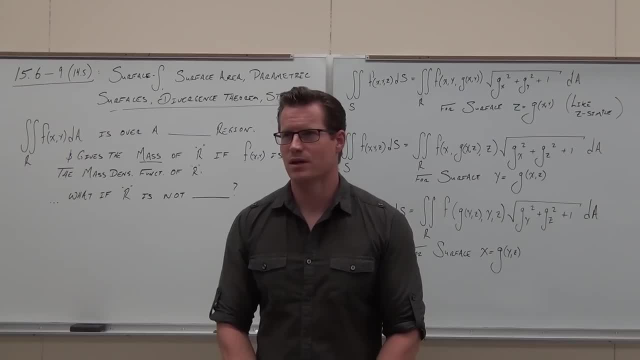 And you can do that, but we always strive for forward progress. This is not a line integral on a conservative vector field that creates a complete, simple, close curve. We want work to be done. We want Green's theorem to apply: Your education has come full circle. 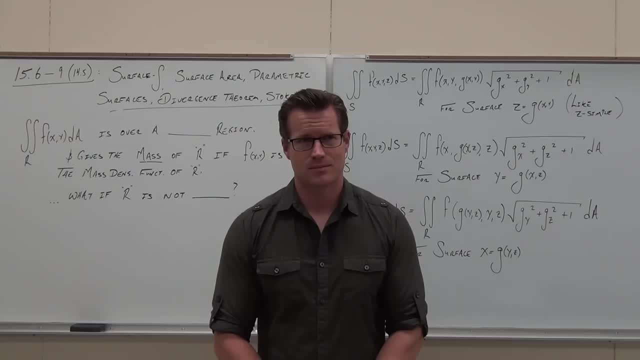 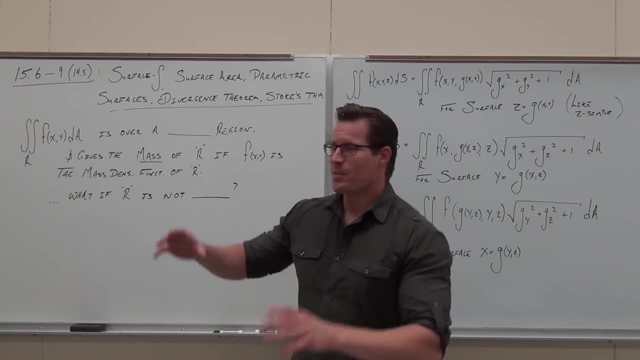 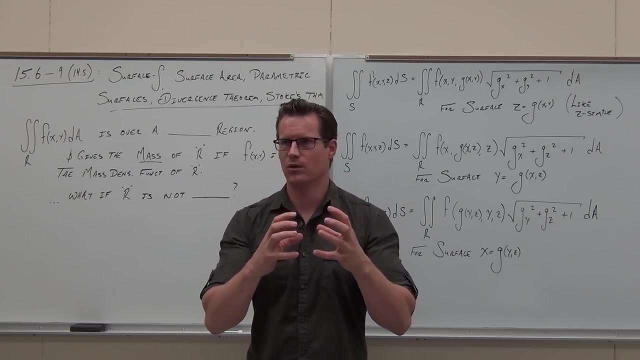 In a non-conservative way. Boom, Boom. Let's just end it right there. We're not done Because we have. we're doing this seriously, though. we're doing the rest of the material for Calc 3 in one go. 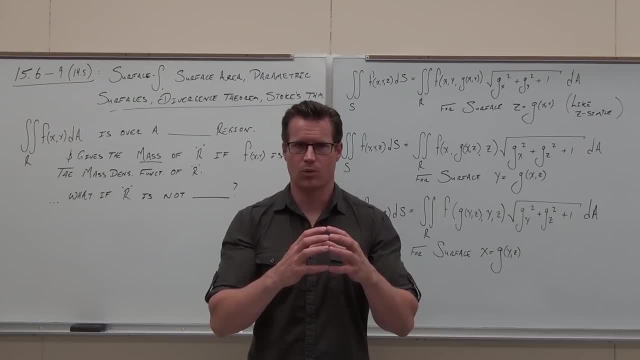 Because it flows very smoothly. I don't want to break it up into four sections, frankly, because I don't have a lot of time. I don't want to break it up into four sections, frankly, because I don't have a lot of time. 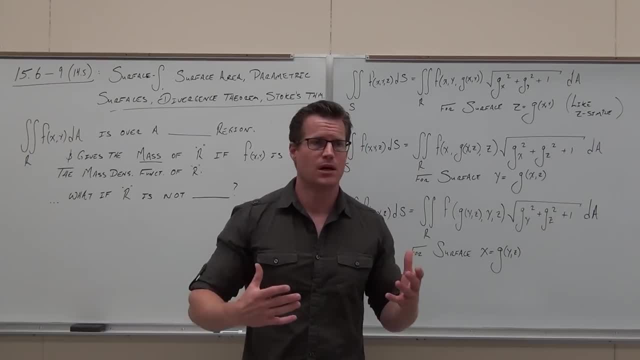 And honestly, it doesn't need to be So how this stuff flows. I'm going to show you How this stuff flows. I'm going to show you Where this stuff comes from. I'll talk about it. We're going to talk about a lot of different things in this section. 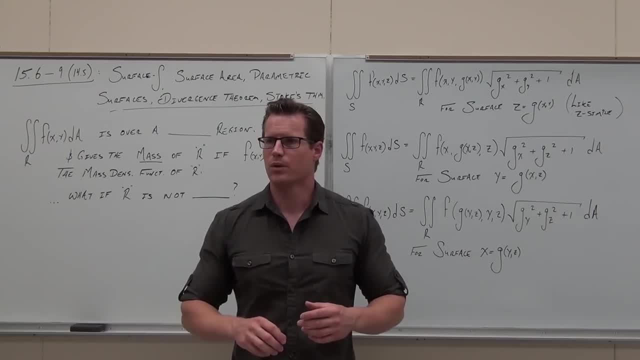 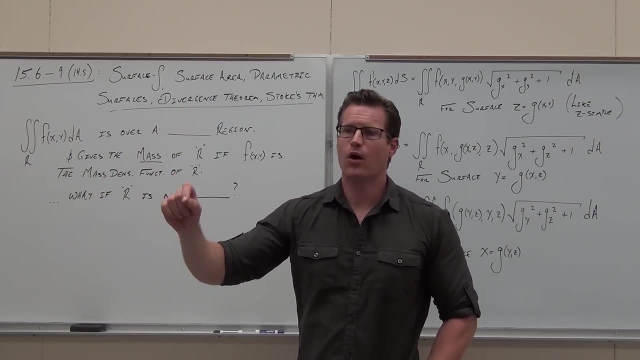 This large chunk of material. What we're going to talk about is a flow from what surface intervals are, how they relate to surface area, how we can parameterize surfaces so that we can find surface area easier. How we can parameterize surfaces so that we can find surface area easier. 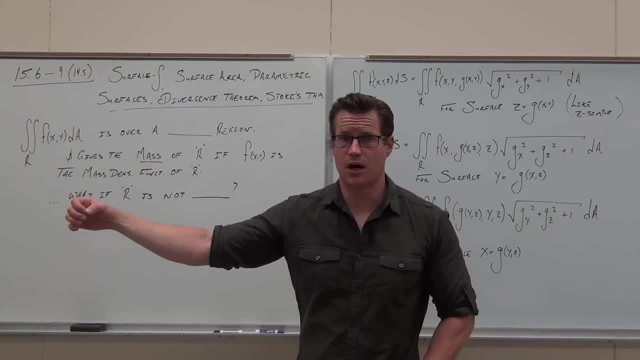 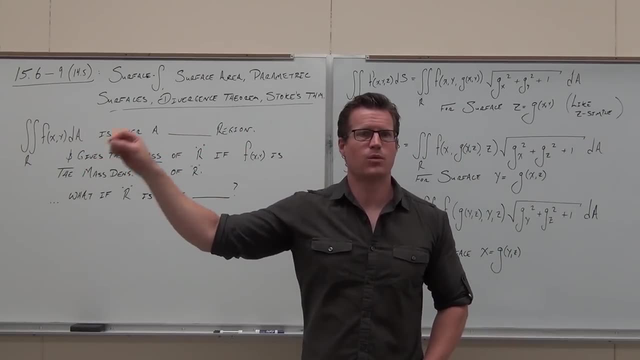 And do work on a vector field a little bit longer. And do work on a vector field a little bit longer, All right, field along surfaces, not just along curves. how we can use divergence theorem to our advantage, what that even means. and then, finally, what Stokes theorem is. 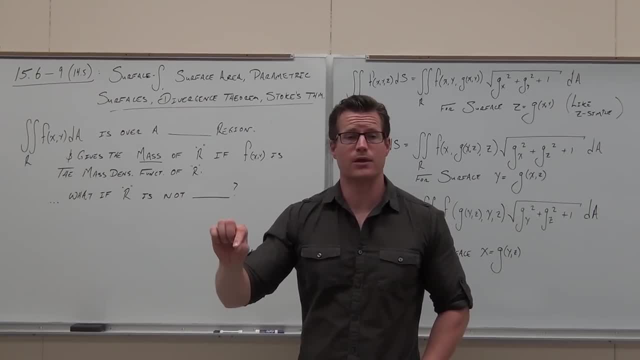 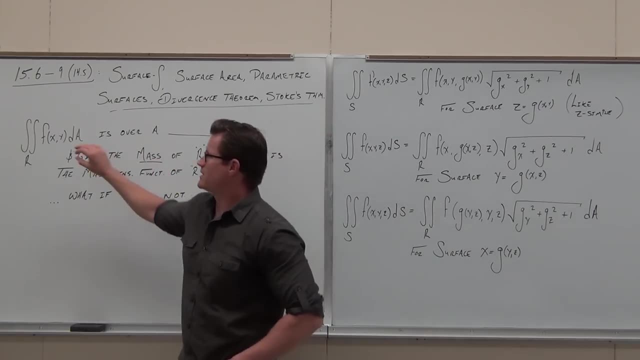 Stokes theorem is a generalization of Green's theorem and we'll talk about how they relate. you'll see how they relate. I want to get into the start of it. we're gonna relate it back to that. you've seen that we've worked on that for over a 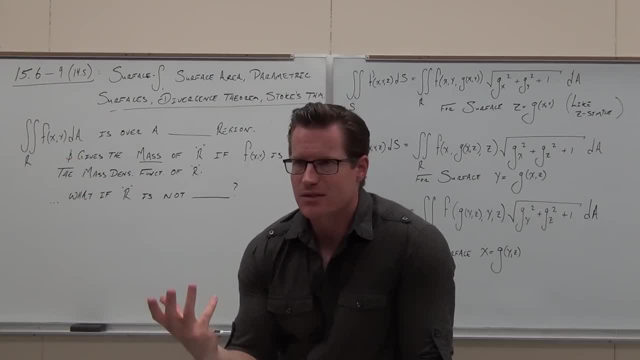 chapter. now, what a double integral does it says: I want you to look at a region. I want you to look at a region, but that region has to be on a. what plane it's got to be on a plane? in other words, R is a flat region. that's how double. 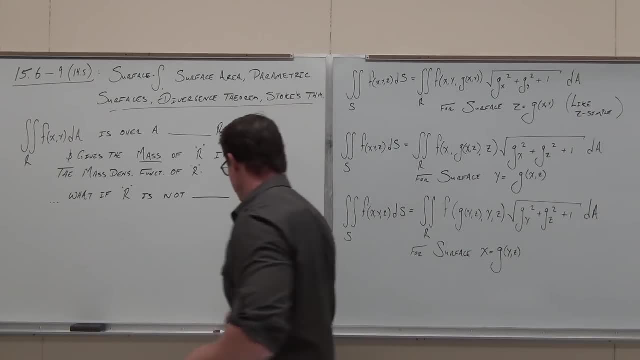 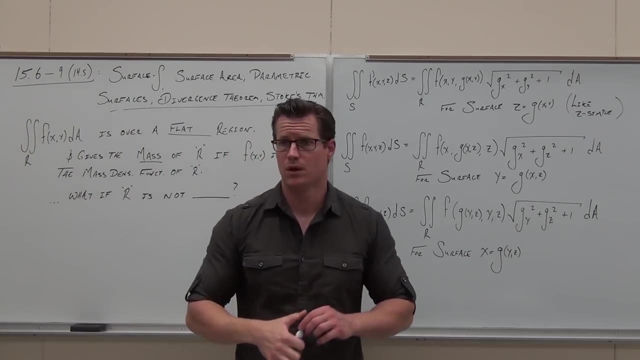 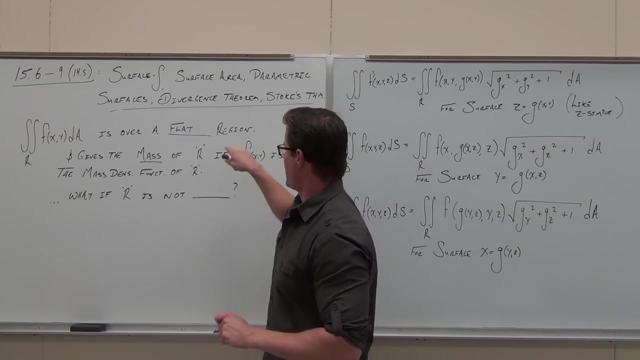 integrals work. they're a flat region. now, what do double integrals do? well, they either give you the volume under the surface over that flat region, or or, if you're looking at a flat region, you're looking at a flat region, you're looking at a flat plane. if f is the mass density function of that little plate. 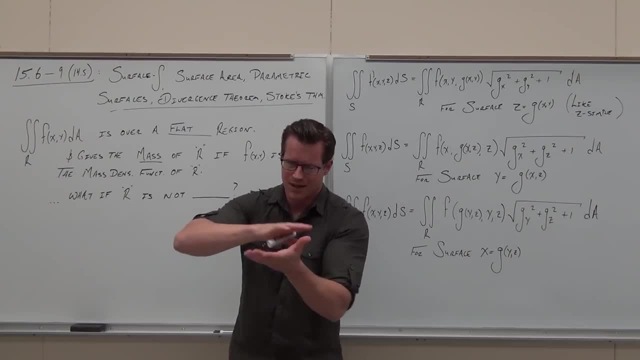 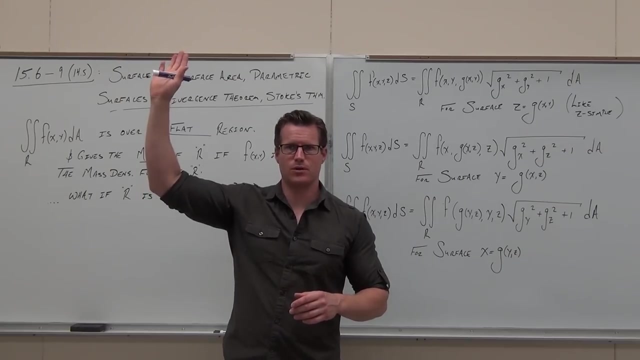 that really, really, really thin plate. remember that a really thin plates that are a point like super flat, like it's not have any real width to it. if f is the mass density function, it's giving us the mass of that plate that occupies the region R on a flat plane to eventually locate with that one. okay, that's what a. 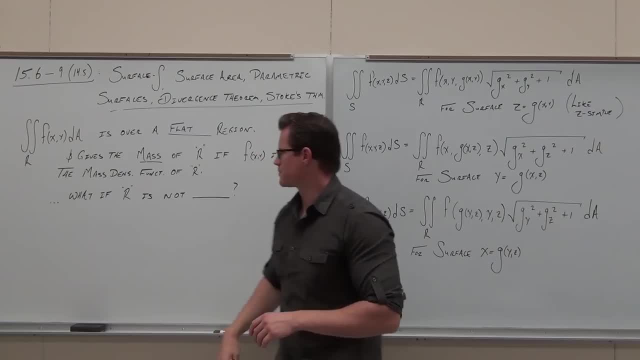 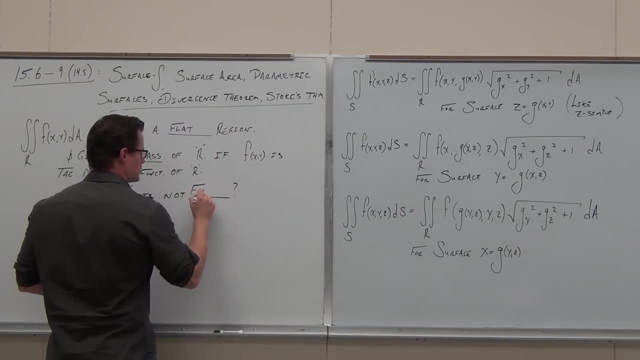 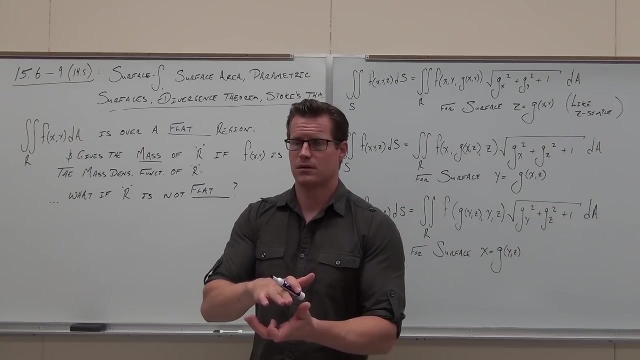 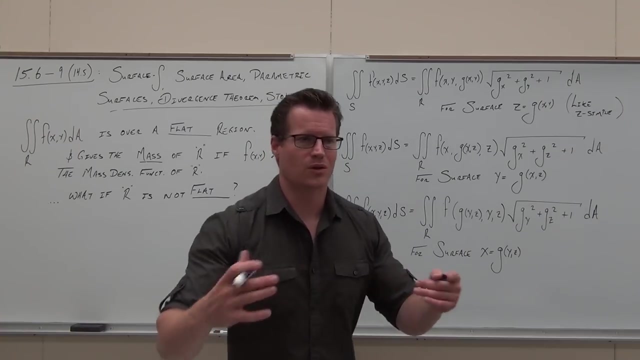 double integral represents. for us now imagine this: what if R it's not flat? if? Well, if R is not flat, can it possibly sit on a plane? If R is not flat, not flat, can it sit on a plane? No, Then R is no longer flat. 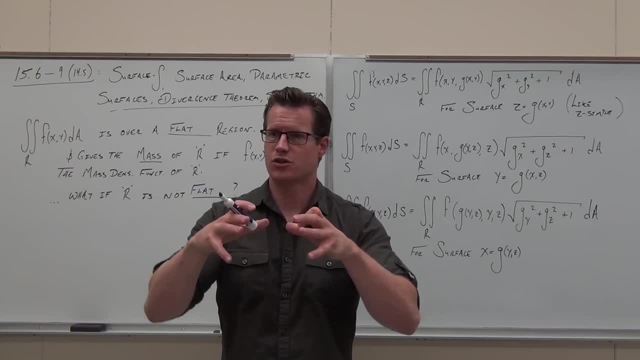 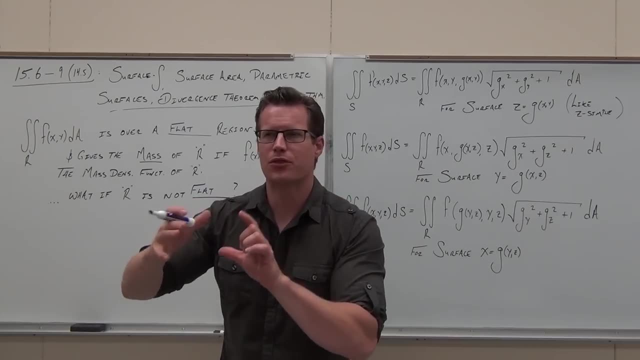 That means R is no longer a plane. R is now a surface. This is what we're going to be considering. What if the R that we have? it's still really thin, but it's no longer flat, It's a surface. 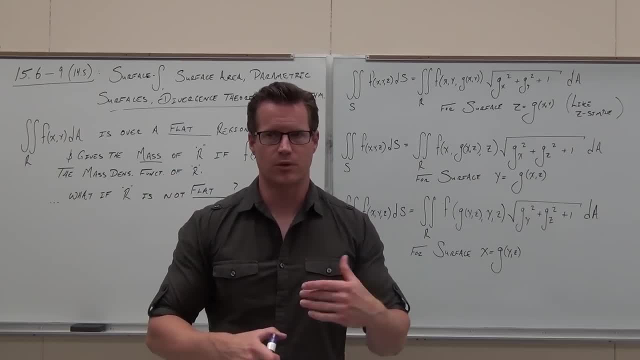 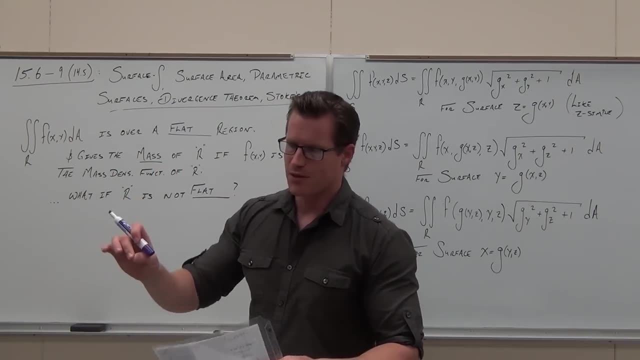 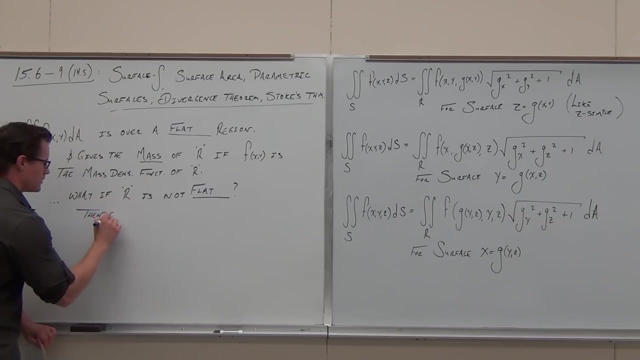 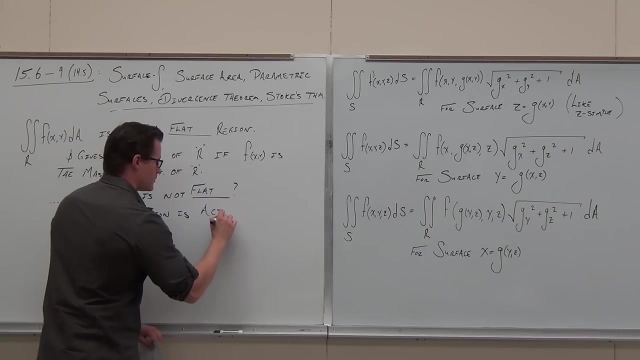 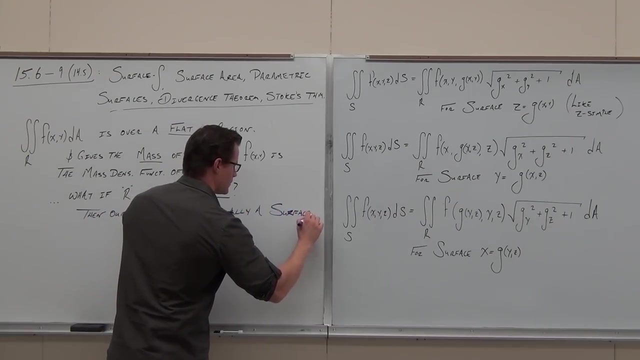 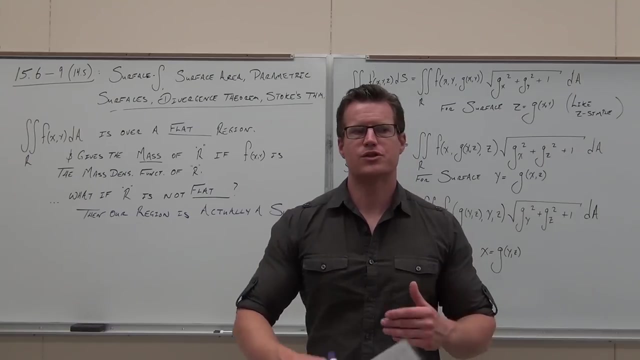 That's what a surface integral starts to describe- how to do double integrals over a surface, And we'll talk exactly about what that means. So if R is still thin but not flat, then our region is actually a surface. This is going to lead us into what surface integrals are. 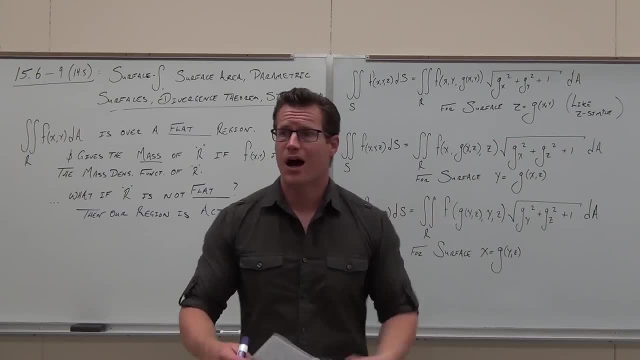 We'll talk about what they are. We'll talk about what they mean. We'll talk about the formulas, what these mean. I'm going to say, hey, we're going to jump back and do 4.5.. It's literally a one-sentence lesson for section 4.5.. 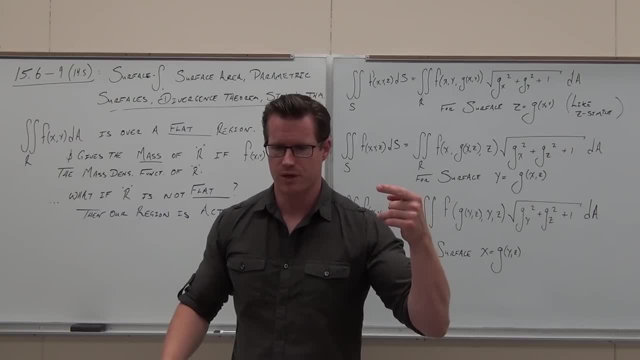 That's why we skipped it. You're like man: we went 14,, 1,, 2,, 3,, 4, 6.. Leonard forgot how to count. I didn't forget how to count. We skipped a sec. 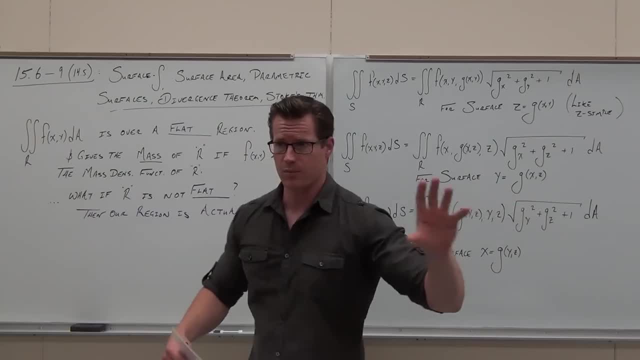 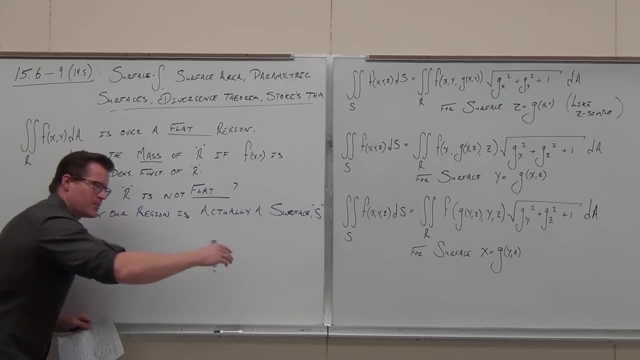 Why? Because it's literally right here, And I will show that to you, I'll prove it to you. I'll prove it to you. So, firstly though, we got these integrals now, these double integrals over these regions that are still really thin, but they're not flat. 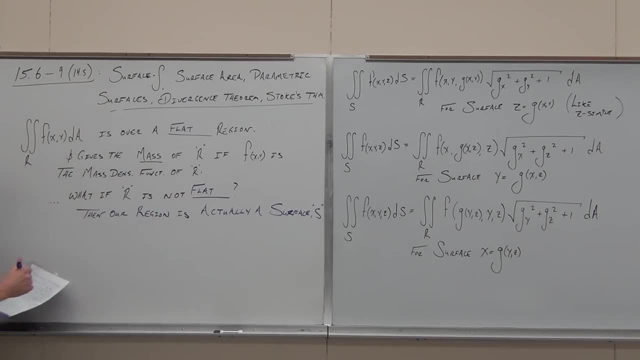 That means they're over a surface. This is a surface integral. So a surface integral it's a double integral over some really really thin plate that's not flat, a surface And some function. what are we going to let that function represent? 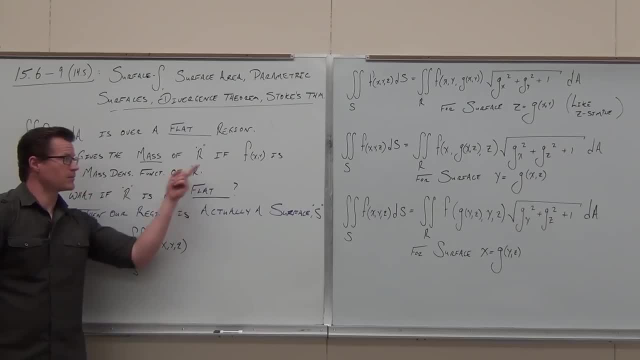 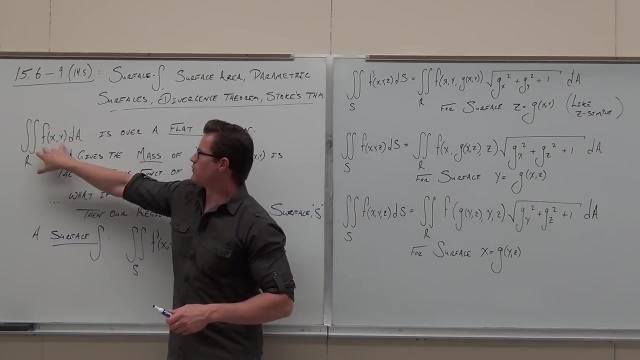 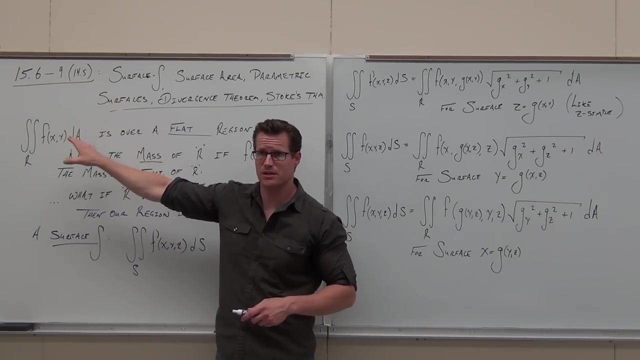 What do you think I want to make? you consider the comparison here. This is a double integral over a mass density function, where this region has some area and we integrate across the area of that region. Does that make sense? Okay, this is the same thing. 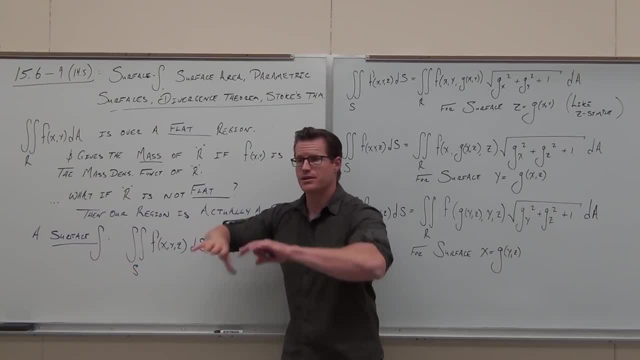 This is a double integral where we have mass density function over some region. that's a surface. We don't just have area anymore, We have surface area. Does that make sense? It's not a flat concept. You can't integrate across a flat concept anymore. 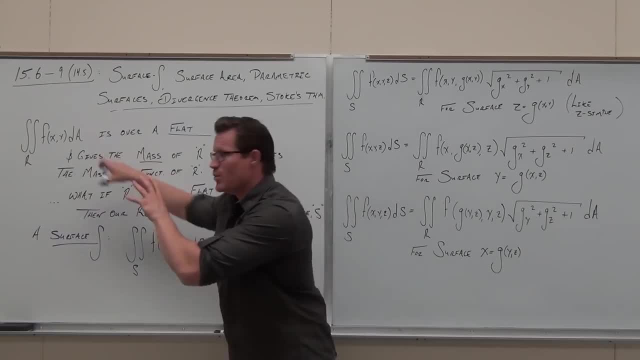 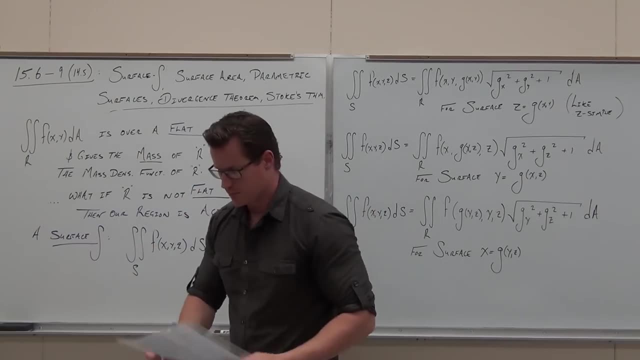 It's a surface area concept. So not just area But surface area, Not a flat region but a curved region, Something that has a surface to it. Now I'll make one more statement. Are you guys okay with that one? 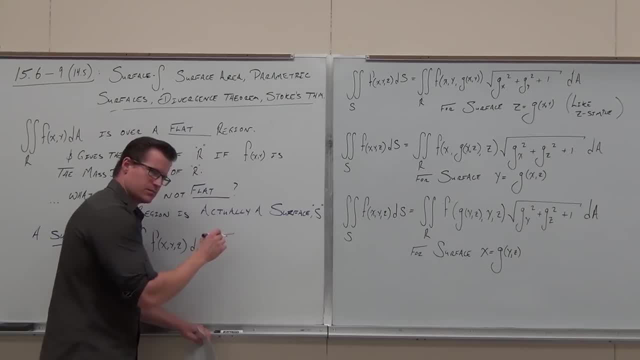 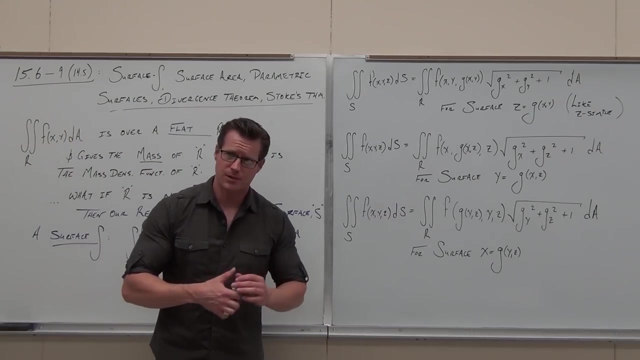 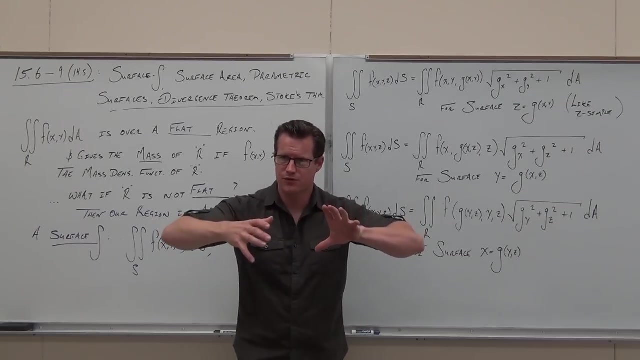 This is a surface area concept, Not just area, a surface area. One more statement. One more statement. Imagine this. Imagine that we have this, not flat plate, So this surface, And I look, I take this surface. Are you looking up here? 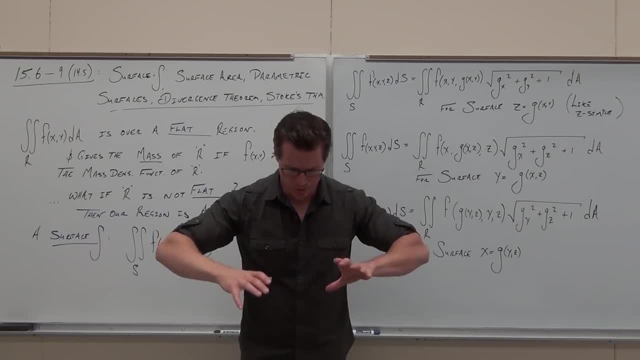 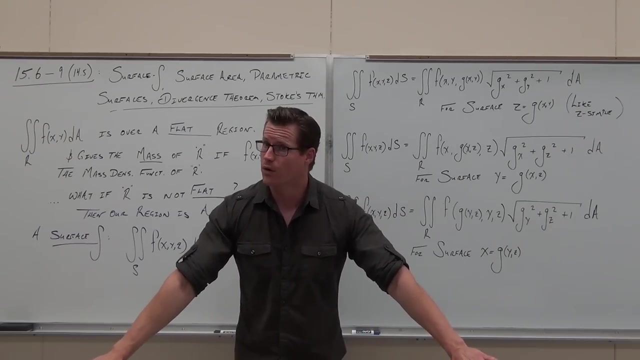 Look up here. I take this surface and I look straight down on top of it. Is it going to look flat? Straight down on top of it? In fact, that look that it has to it, that flat look is a projection onto the xy plane or the yz plane or the xz plane. 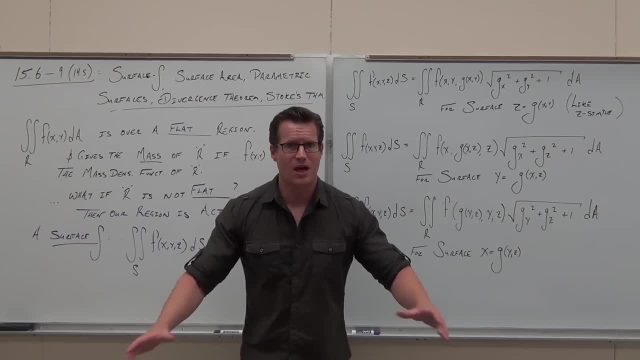 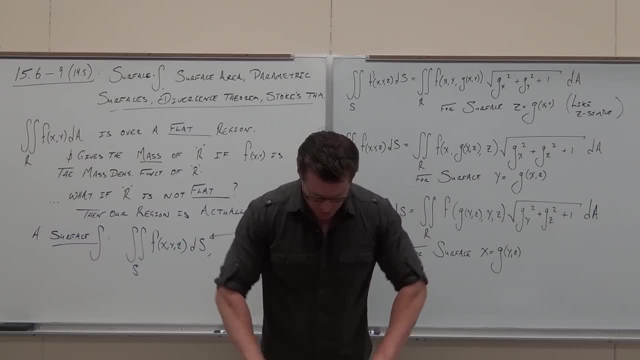 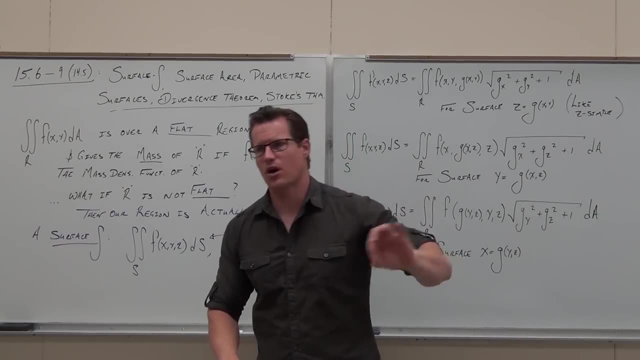 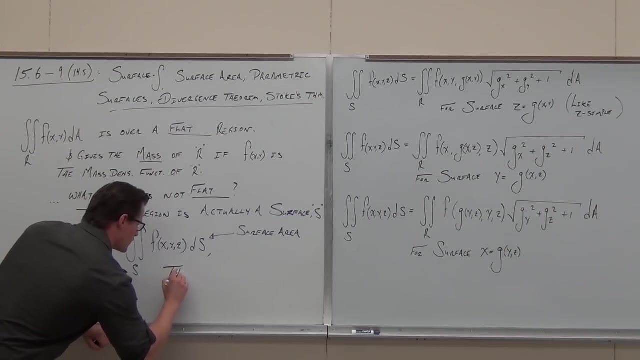 Surface is our region. The projection of that surface onto a plane, that gives us this r that you see here. So the projection of the surface onto a plane is giving us r, Expressing that r to us. If you had that, if you. 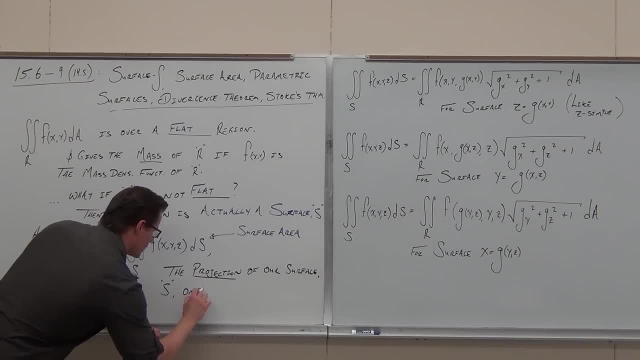 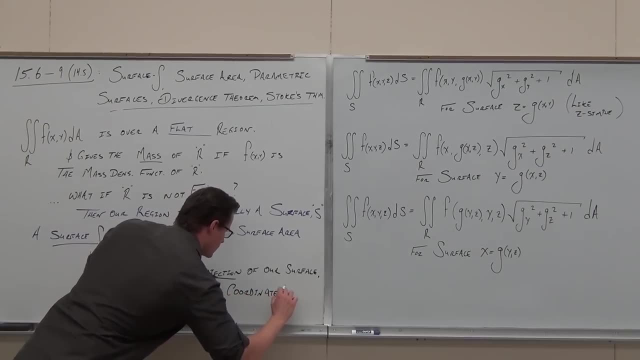 Really well. I don't think it makes sense to watch you wait on that flying on your vacationagad. But it means if you wanted to put in this r to a plane, you wouldn't have to do it on your trip to Vietnam. 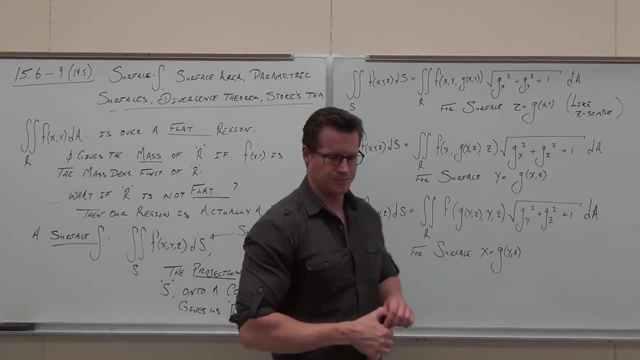 Or you shouldn't have to do it on your trip. It's kind of like gonna ask you: what Do you need to do it on your trip? So here's like maybe a 15-second recap about what this stuff is. We'll run through the formulas that you need to know what they mean. 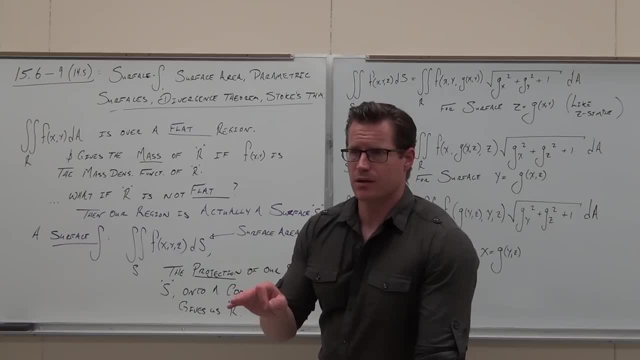 I'll explain them to you and then we'll do an example. very, very quickly to get our feet wet Again. I think I said this before the opener, but basically you're going to have idea, one example: we have to move on. 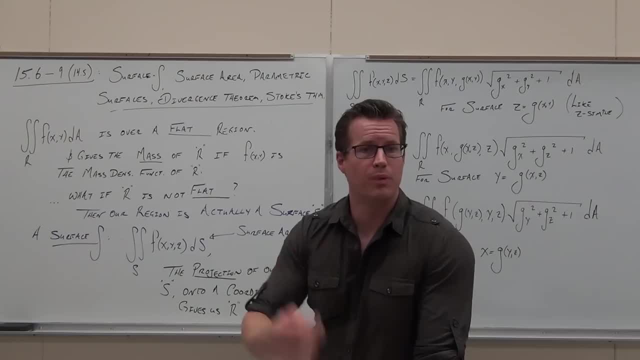 Idea, one example. we have to move on. We're not going to get a whole bunch of examples here because, frankly, they're very, very similar to each other and I don't want to waste our time. I'd rather go on with kind of more of a theory, the lesson part of it. 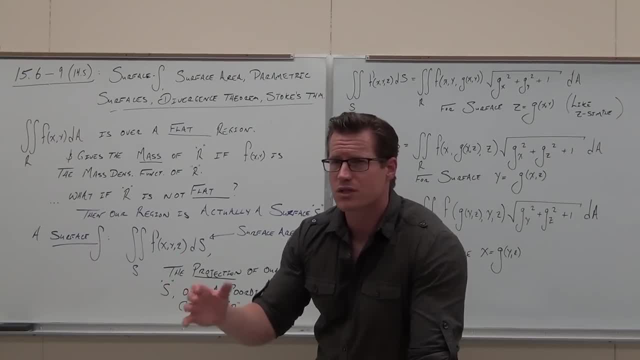 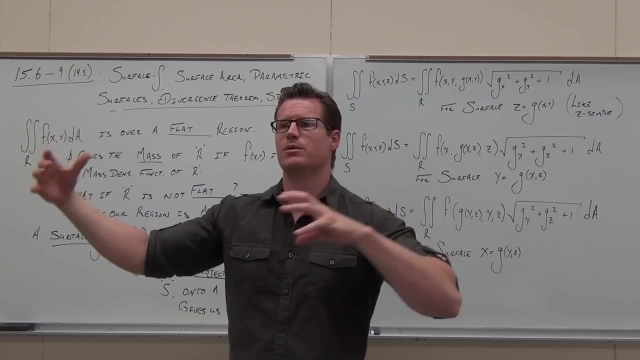 than just crushed examples. We've done a lot of that, Mostly here at this point, since you guys are man really mathematically mature after doing all this stuff. all right, you know how double integrals work. You know how triple integrals work. 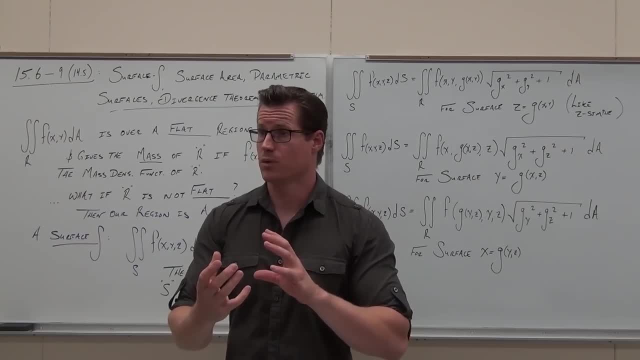 You know how all this stuff works. We're just dealing with a theory behind it. now, How can we use it to our advantage to make our lives easier, not harder, but do different things with it to make our lives easier. Did you guys get that? 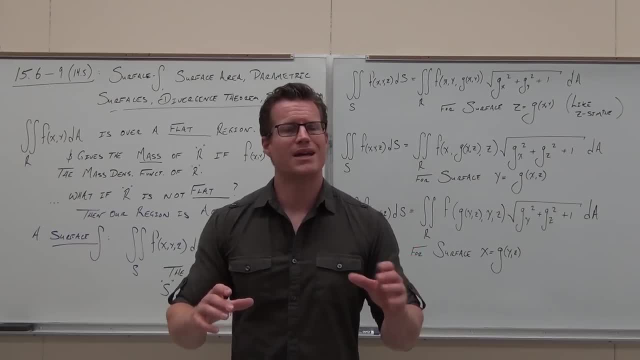 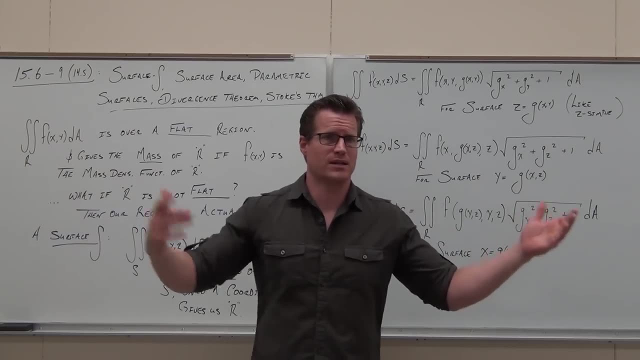 So I'm not going to try to give you really hard examples here. What I'm trying to do is to get you to understand the concept, to truly understand it, because if you get it, then I you can practice the easy examples. 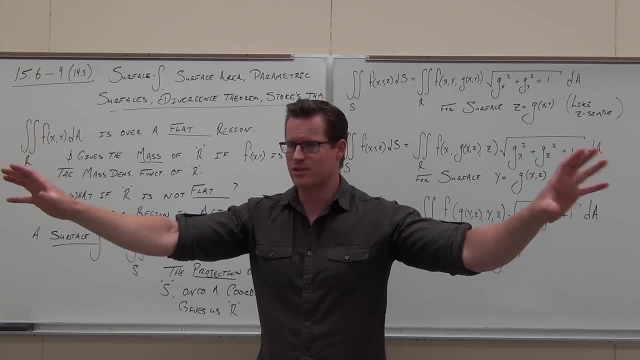 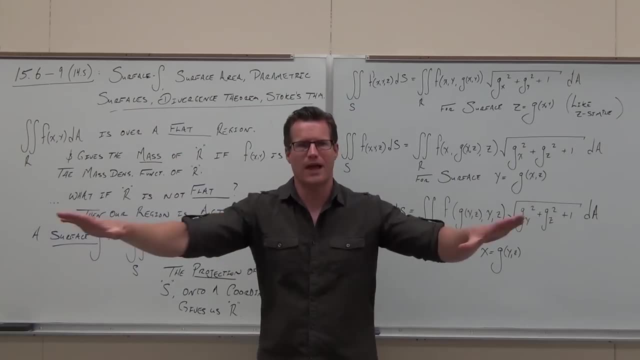 and you can do everything on your own. Does that make sense? If you understand it? that's my job as a teacher: to make sure you get it, if you actually understand the concept. The concept here is: we used to have double integrals where our region was flat. 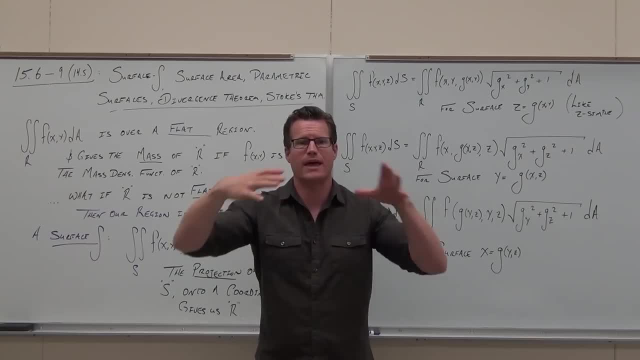 and we used to have this thing that gave us a mass density every point along that flat region. Does that make sense? Really thin little plate. and now we're saying: imagine that plate is no longer flat, That plate is now a surface. 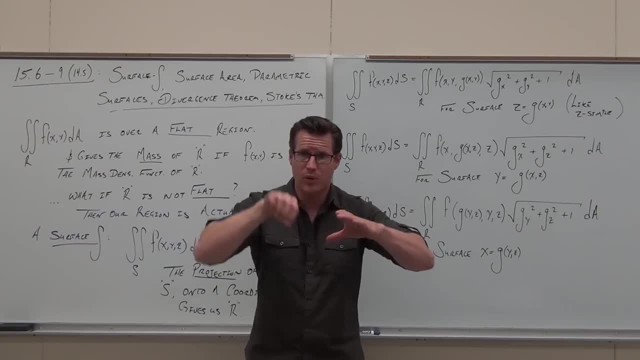 It's still really thin and it's still the mass density function Any point along that surface, on that surface that works. Look, surface three variables. It's creating that mass density at every single point on that surface rather than on the flat plane. 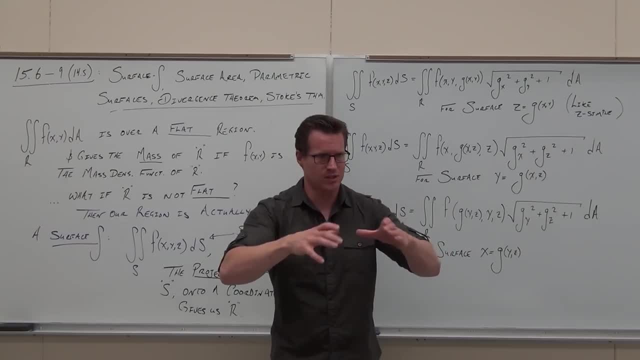 Do you guys see the difference in it? already We go, okay, well, can we still do it? Yes, Yes, we can still do it. In fact, if we look down on the top of that surface, it's going to give us a region on a quarter plane. 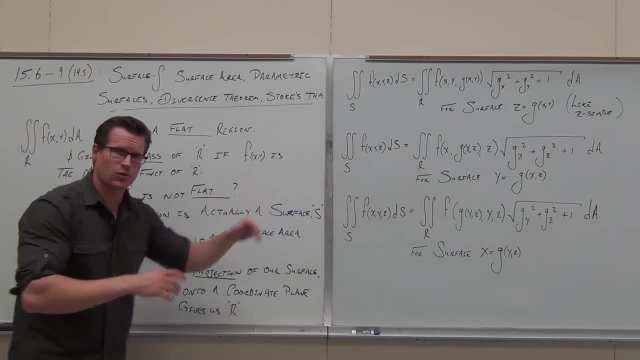 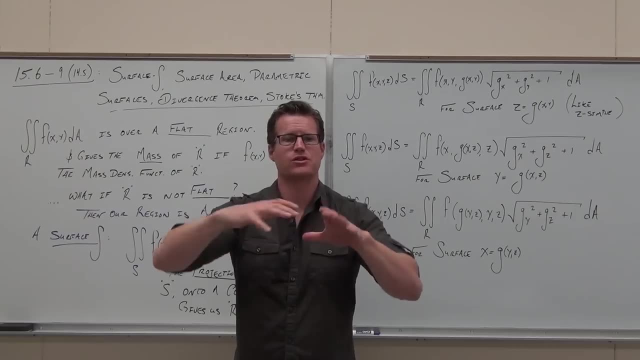 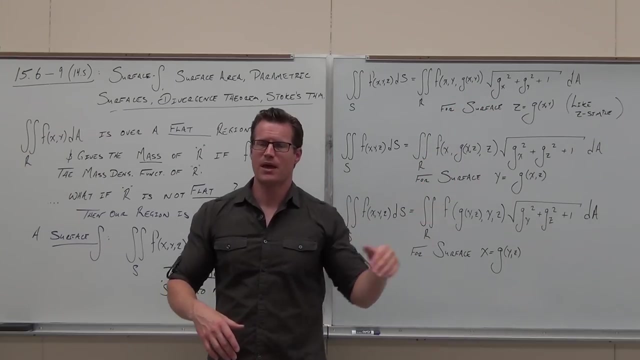 We can structure our surface. So surface integral means basically just find the mass. if I do this, find the mass of a really thin plate that has a surface to it. Does that make sense? And we can do it like this. Now, what in the world is all this stuff coming from? 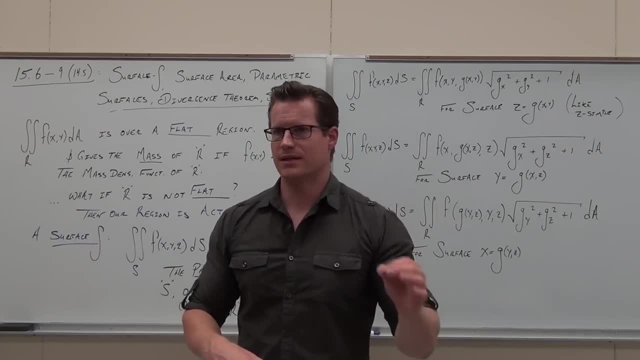 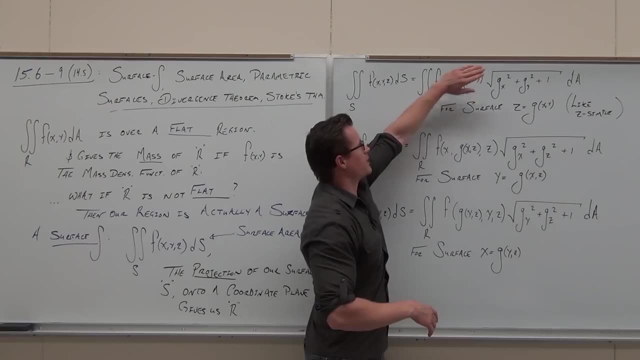 Here's section 14.5 in a one-sentence statement. Are you ready for it? Here it is. If you eliminate this and you treat your function in terms of x and y, so z is a function of x and y. 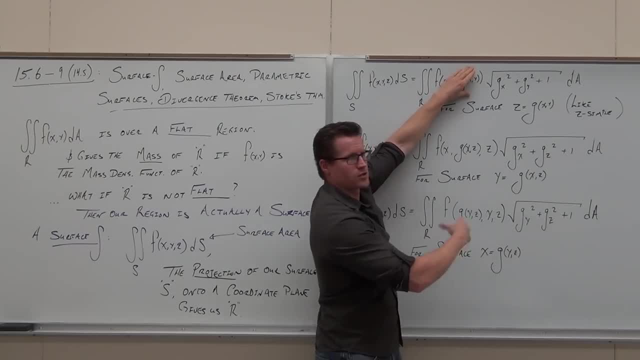 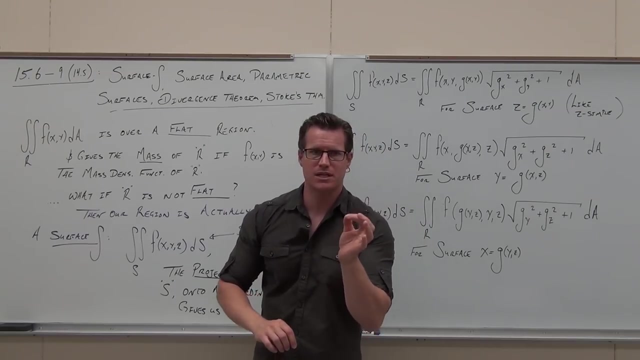 or y is a function of x and z, or x is a function of y and z, or you treat one variable as dependent on the other two. then this right here and this right here and this right here are the exact thing that you see in section 14.5 for surface area. 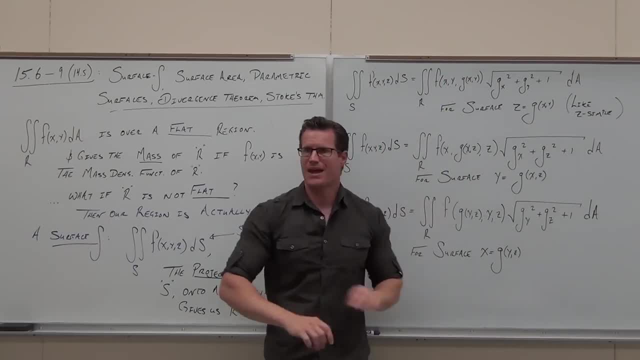 of that function over that region. It's the exact same thing. That was a one-sentence statement. If you read it back, that was one sentence. I use a lot of ands and buts, but still, ah, that was one sentence. 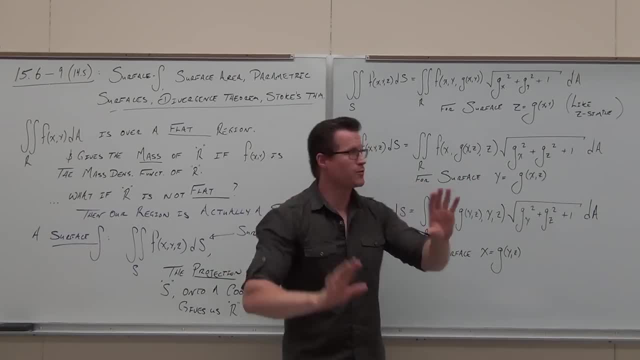 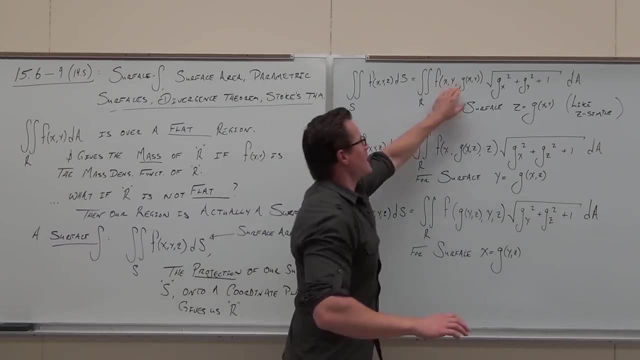 That's 14.5.. So, so watch, Are you ready for it? 14.5 just has this. That's it. Now let's look at it. Let's look at what this does. What does f give us in this context? 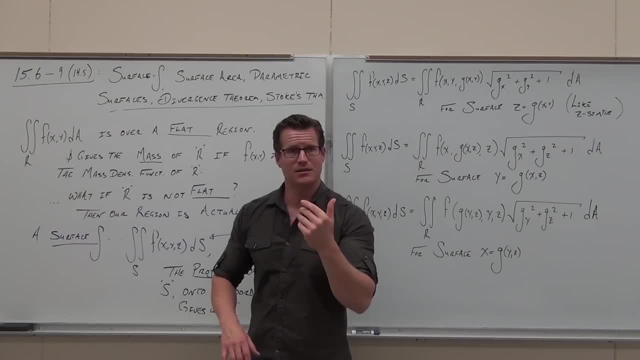 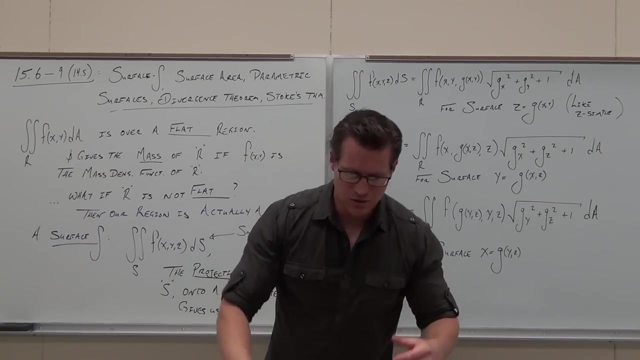 What is that Mass density? What's this p Surface area? It's giving us the mass density at every point on the surface with respect to area. It's just finding the mass and adding it all up. That's literally it. That's what section 14.5 did for us. and now we say: 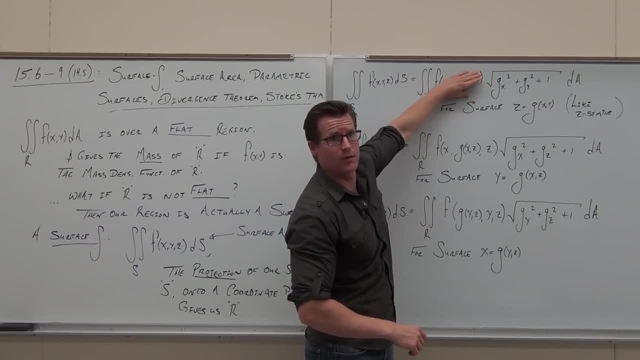 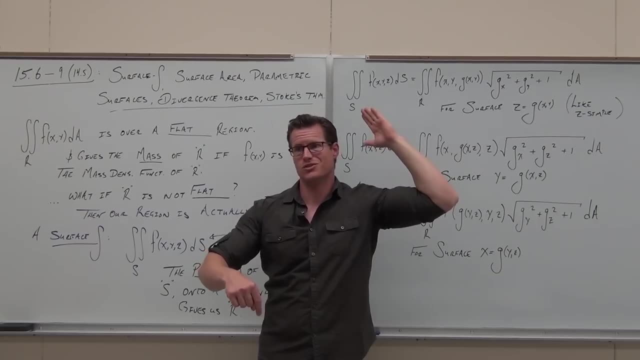 suppose that we also want to find the mass at every point along that surface with respect to its surface area. Boom, That's now this section. That's what surface integrals start to do for us, Do you guys see it? It's kind of cool, right. 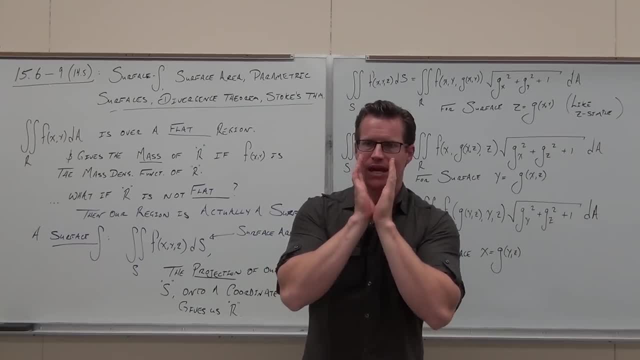 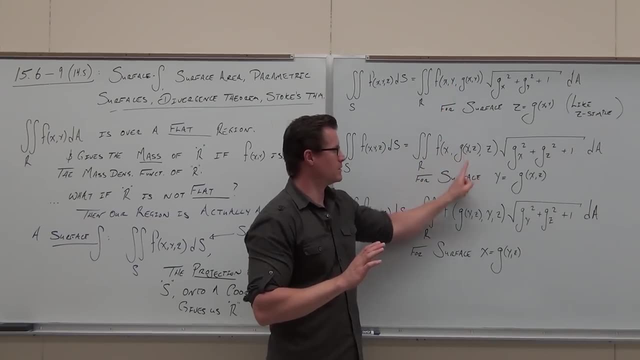 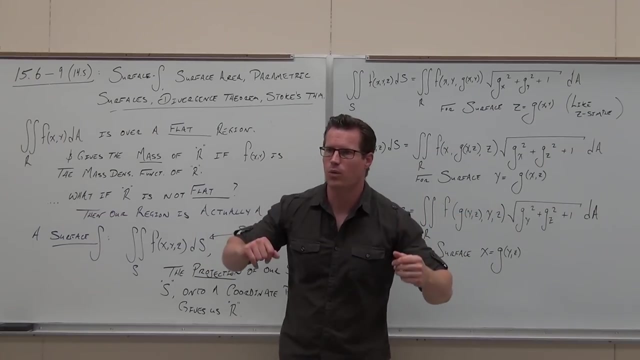 I'll say it to you another way. Suppose that the mass density at every point was constant and had a value of one One, one one. Do you remember talking about that? You'd have surface area and surface area If your mass density was just constant, one every single time. 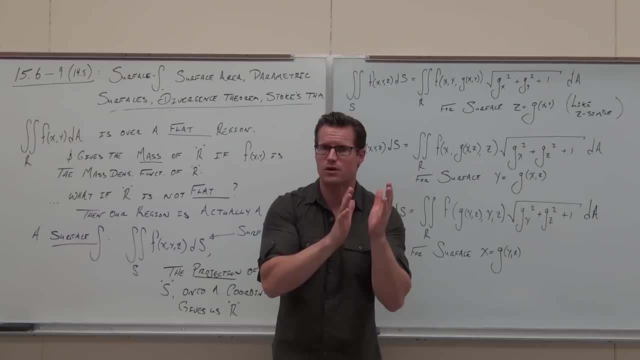 Remember talking about how we can use one and get different things for it. So if you had a double integral of one, actually you'd just give us area instead of mass, or it's given us like triple integral of one: give us volume. 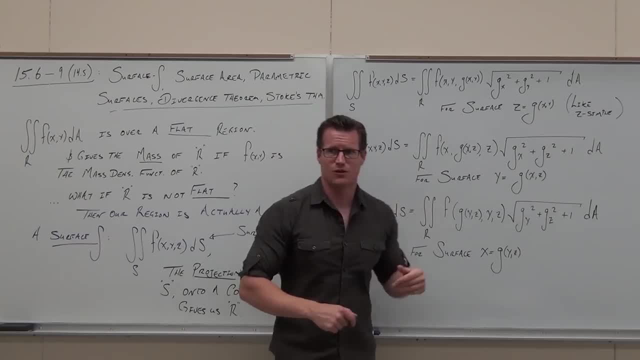 Instead of mass. we can say one for mass density and get surface area instead of mass. That's interesting. Cool, right, That is so. I hope I made the case for you that the reason why we didn't cover surface area explicitly is 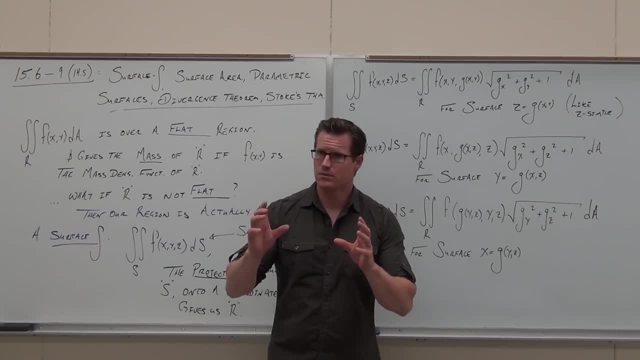 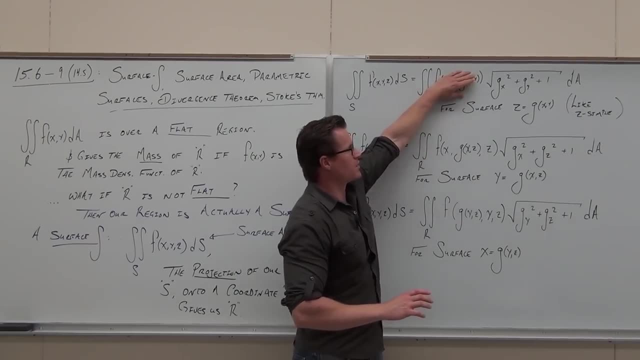 because it's literally covered right now. And if you don't believe me, go back and look at it and say, oh my gosh, he's right. If you just cover this up, you have these three formulas for surface area. And if you just treat the mass as constant one at every point, 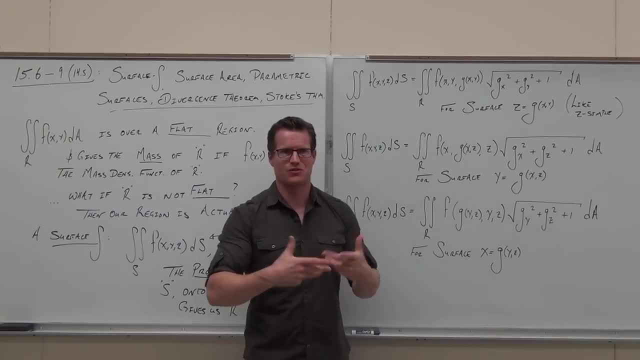 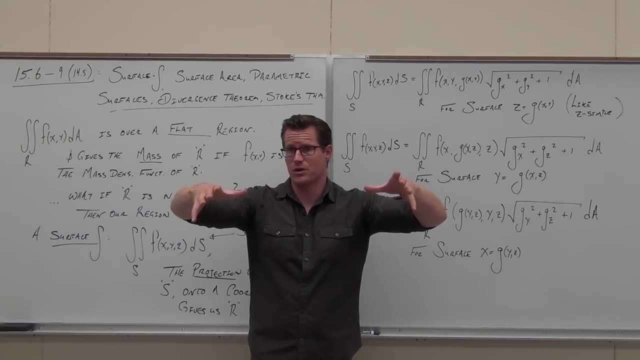 you literally just get the surface area of the region that you're trying to define. That's what surface integrals do anyway. They take the surface area, times the mass and get mass density and get the mass of the surface, the really thin plate. 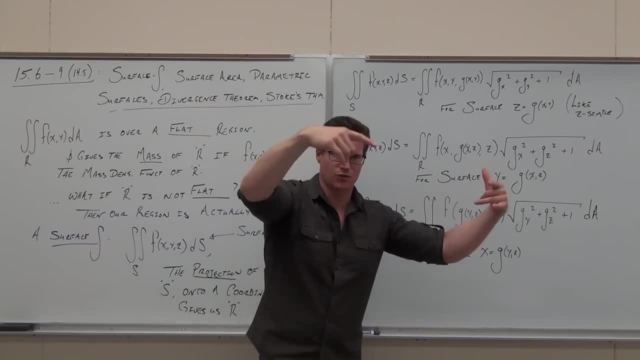 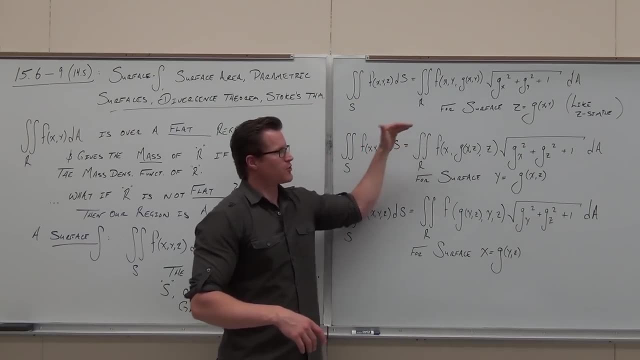 So that's it. So this encompasses surface area force and you're going to see it a little bit later. A couple points I want you to look at. The reason why you have three formulas is the same reason why you had three different options for triple integrals. 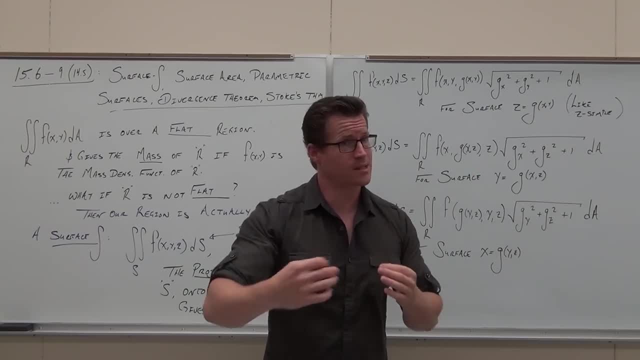 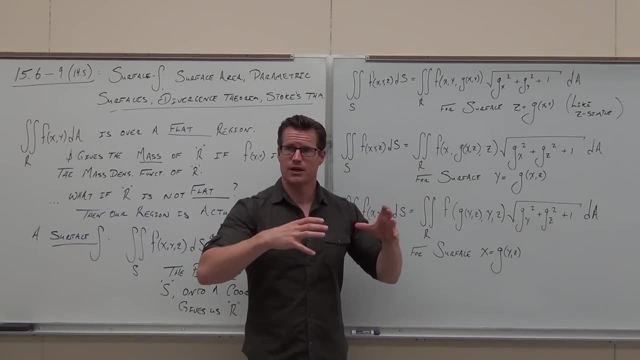 You could choose to do Z simple, Or Y simple Or X simple. first, You guys remember doing that with triple integrals. Well, you can choose to define your surface. Look, your surface would be one variable equal to two other independent. 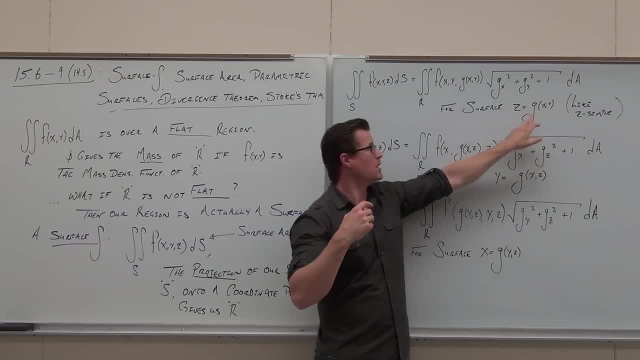 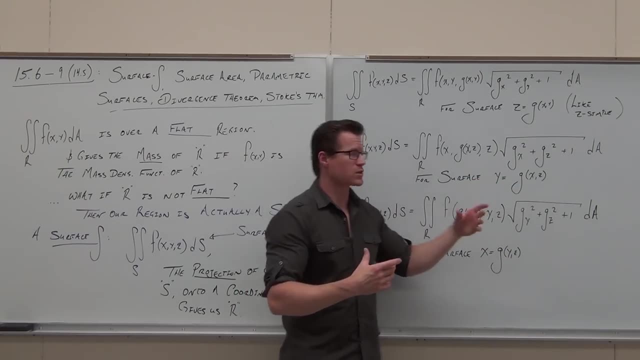 Does that make sense to you? Three total variables, two are independent, one is dependent. You can choose to define it in terms of X and Y, Or X and Z, Or Y and Z. I just want you to look at how it works. 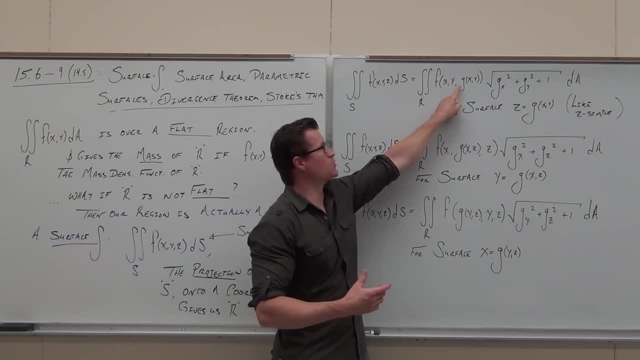 If you define Z as X and Y, then you'd have an X And you'd have an X And you'd have a Y, But you wouldn't have a Z. You'd have a function that's redefined in terms of X and Y. 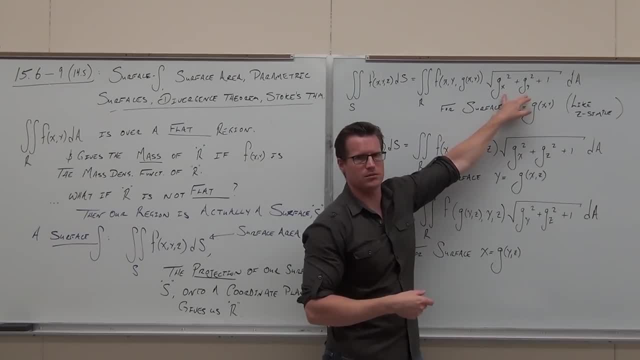 Does that make sense Then? oh my gosh, what are these things? Well, this is the function that you just defined. You couldn't take a partial derivative with respect to Z- here There are no more Z's- But you could take one with respect to X and one with respect to Y. 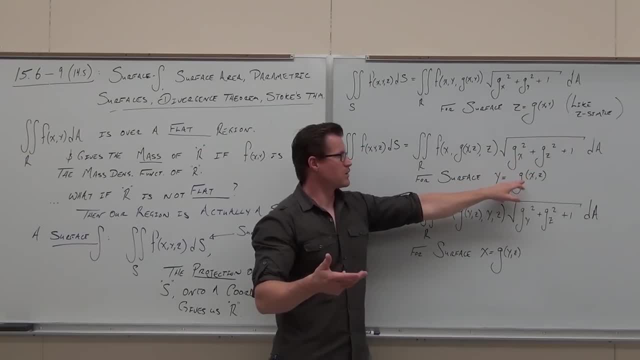 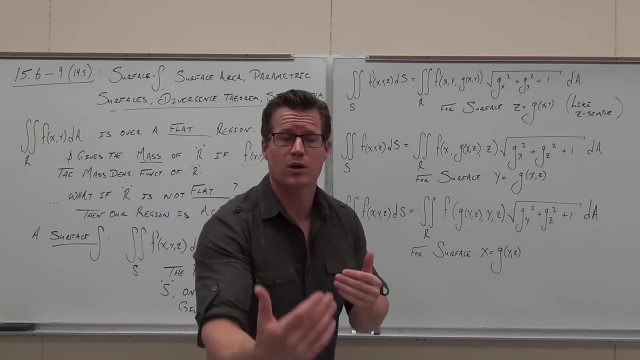 And that's what that's doing Here. you could take one with respect to X and Z, Here with respect to Y and Z, And so it's just kind of the same formula. It just depends on what you want to define your surface as. 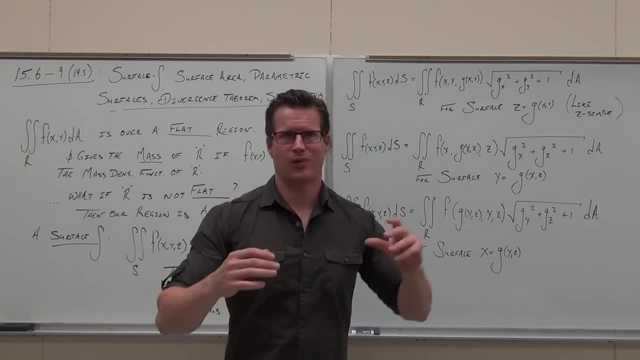 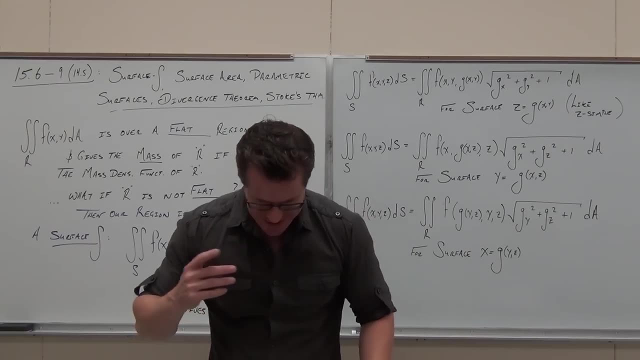 Whether you want Z equals- Think like Z is simple, Y equals- Think like Y is simple. Or X equals- Think like X is simple. Does that make sense to you? So that's the idea. I'm going to show you one example real quick. 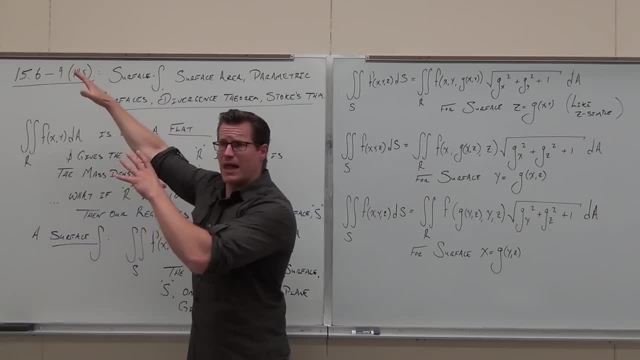 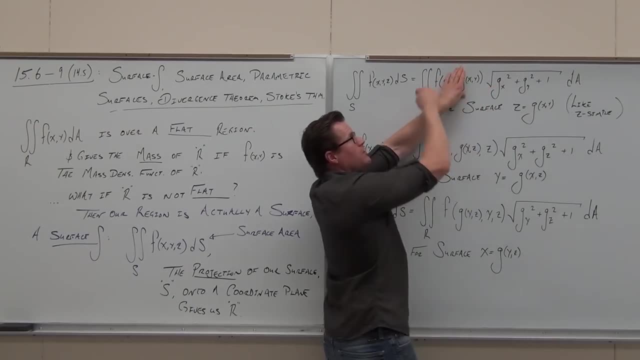 But I really want to know if this makes sense to you, The idea of flat versus non-flat area versus surface area, How you literally do surface area with a projection over R Times, mass density. That's what it is. It's surface area over this. 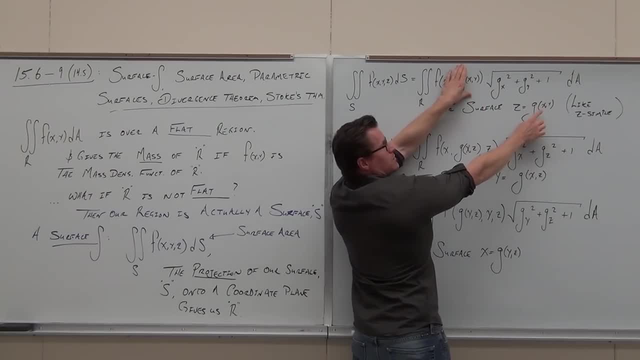 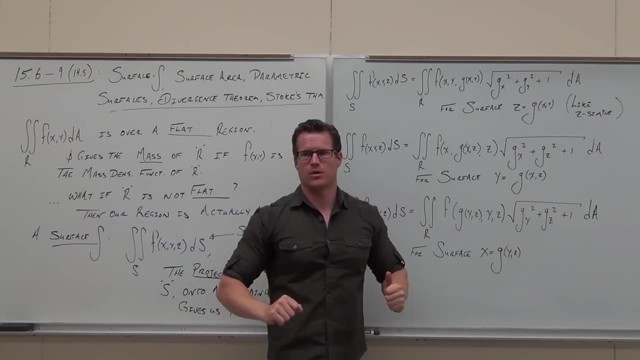 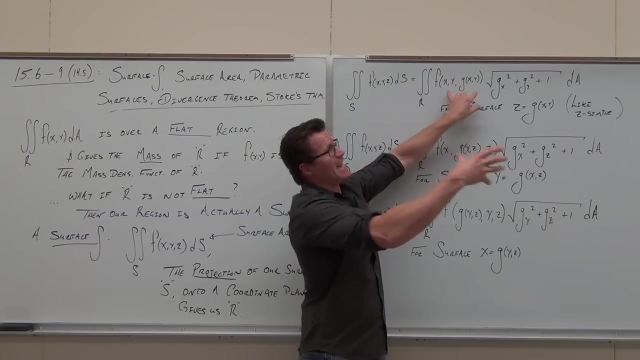 This is surface area of that function, Where R is the projection of that function onto the XY plane Or the XZ plane Or the YZ plane. That's what that is Now. it just says: take that stuff, Multiply by the mass density. at every single point. 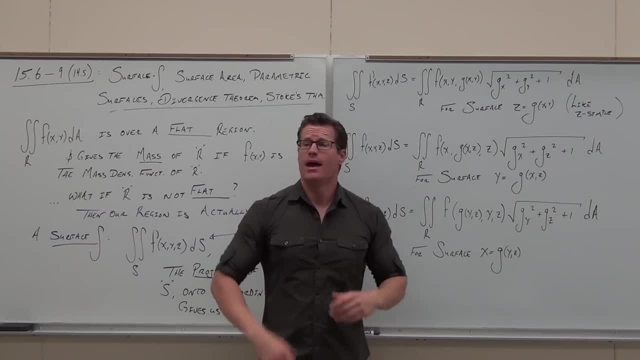 And add it up, like every integral does. It's just an infinite sum, Just adds up the mass density. That's what it does. Gives you all the points, Gives you the mass of the surface where the projection is R onto a coordinate plane. 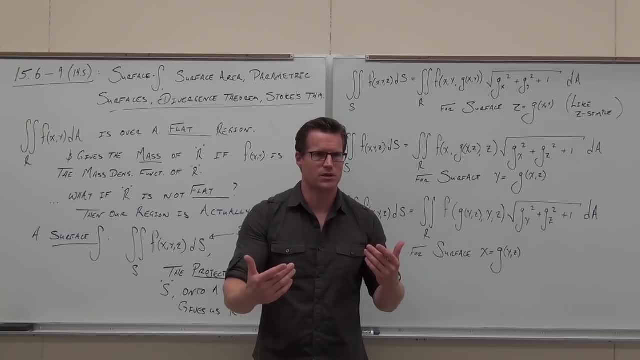 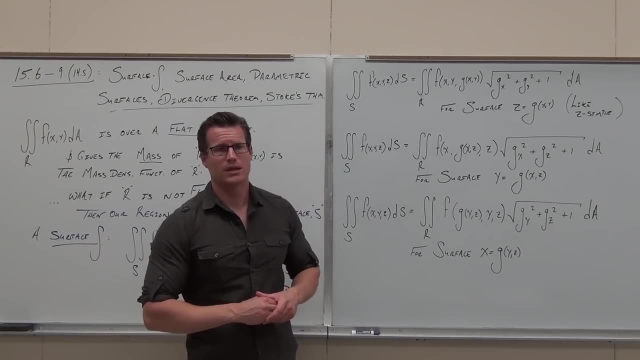 Is that well explained for you guys? I want to make sure that it is. Are you sure? Okay, Now the important question is: how do you do it? It's honestly not that hard. It really isn't. The most important thing you can do is define your function in terms of X or Y and Z. 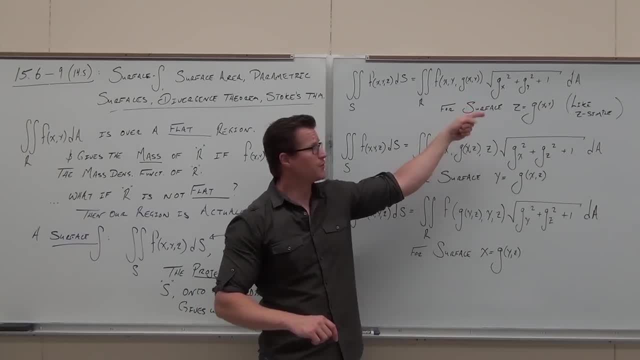 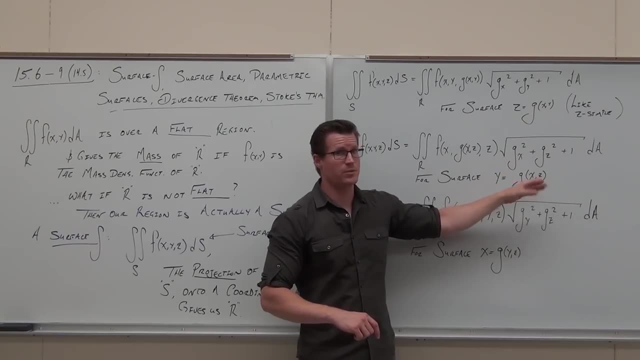 And follow the correct formula. If you do Z equals, then all your stuff better be in X's and Y's. If you do Y equals, all your stuff better be in X's and Z's, and so forth. So let's do one example. 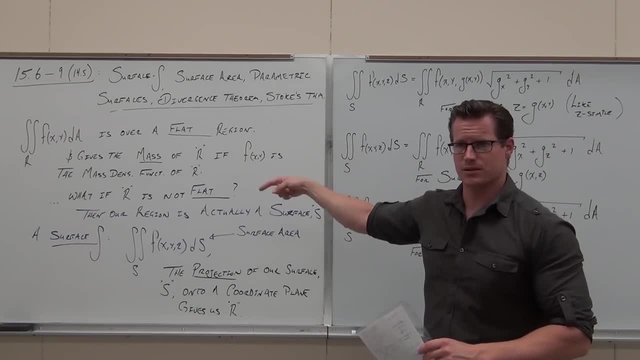 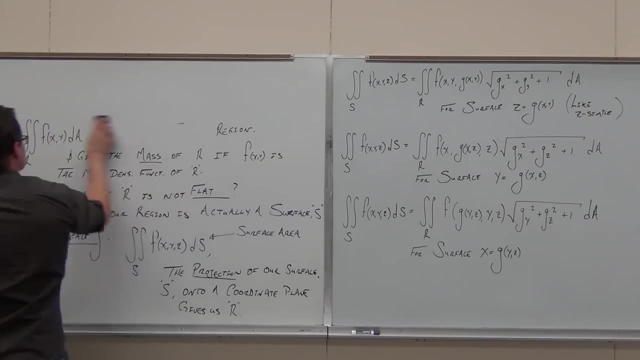 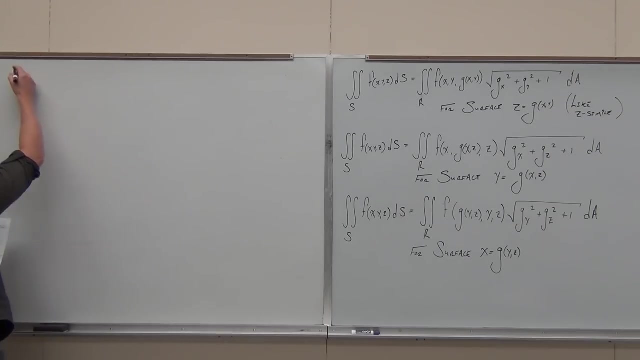 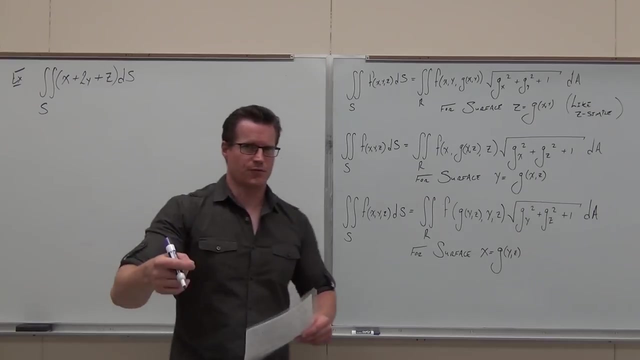 I'm going to have to erase this, so are there any questions on what this stuff means? Okay, Let's check out the look at this thing first. Let's check out the look at it. What is this thing? What is that? 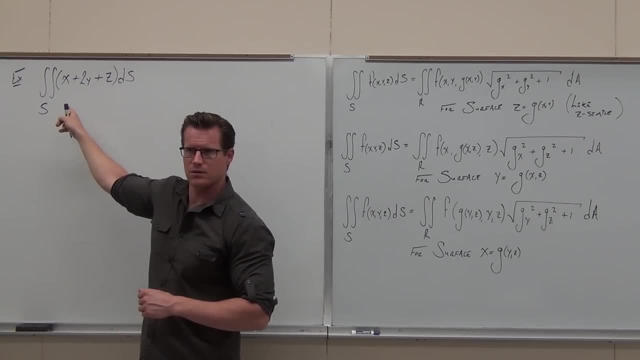 Is that the surface? No, What is it? Mass density, Mass density, That's the mass density function. It gives the mass density at every point on our surface. So, just like on double integrals, I can't just give you this and say: do it. 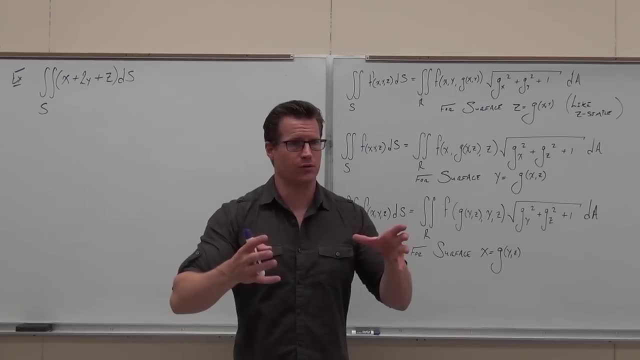 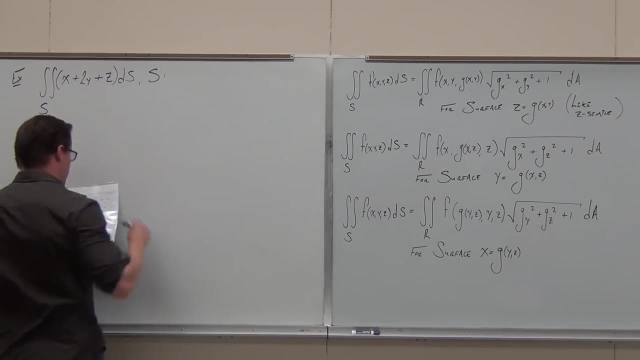 I got to give you this and then I got to give you a surface that you're integrating over that has a surface area. Does that make sense to you? You got to have that, So I'm going to give you the surface. So where S? 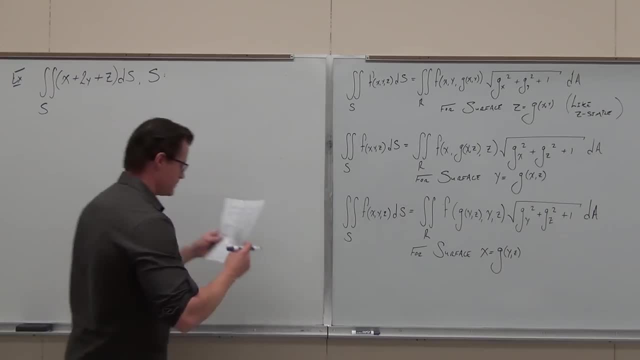 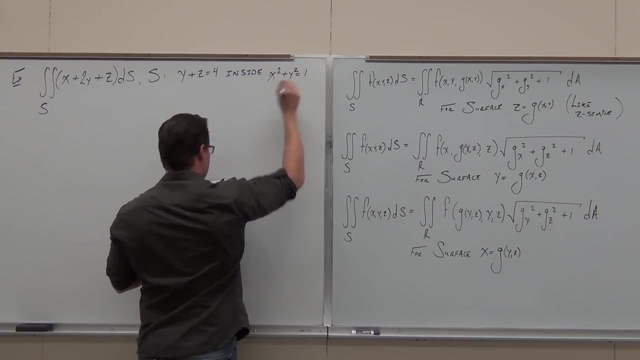 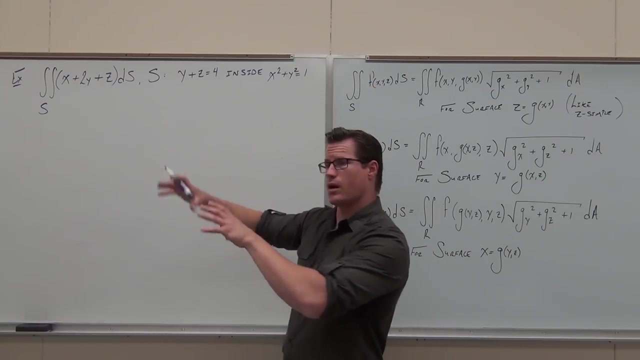 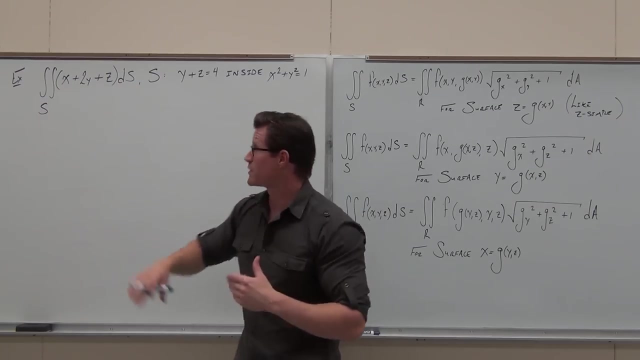 S is a plane inside a cylinder. Okay, So we got this double integral, but it's no longer over flat regions, over a surface region. It has surface area. We have a mass density function at every point on that surface and I've given you a surface. 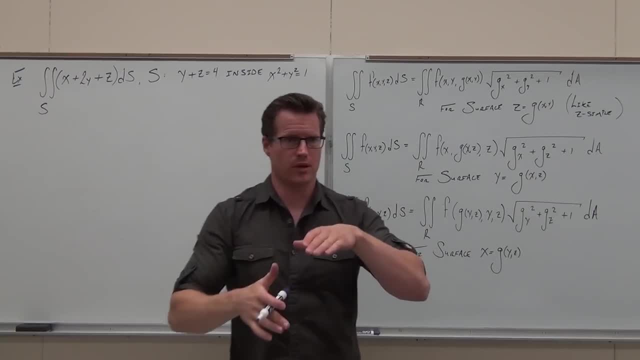 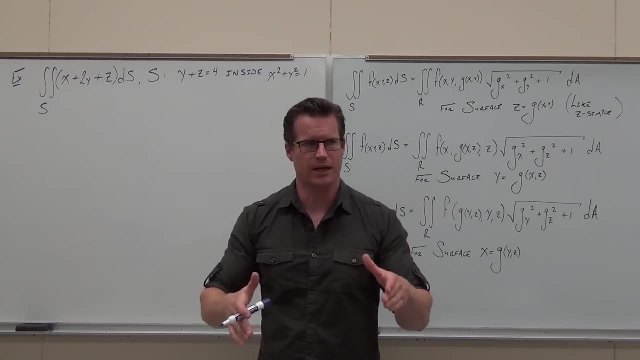 Notice this is not flat according to the coordinate plane. It's not flat. It's going through 3-space, all right, Yes, it is a plane, but not according to a coordinate plane. is it considered flat? Does that make sense to you? 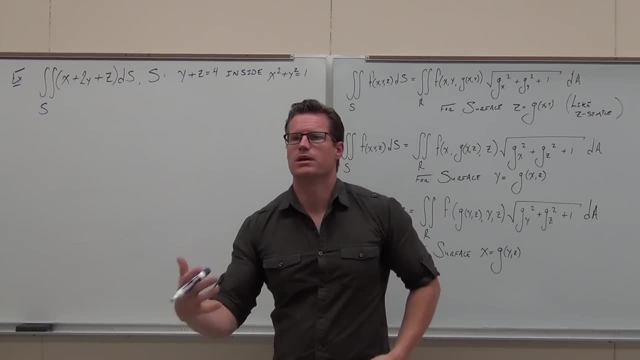 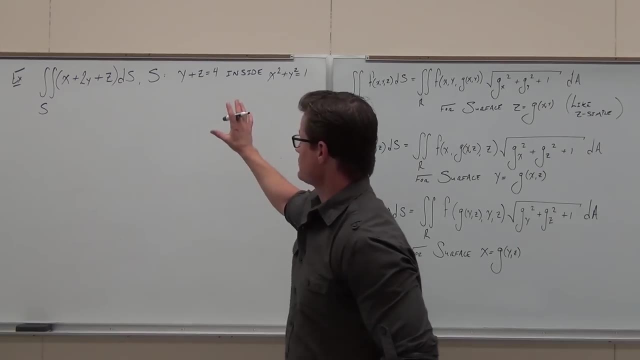 So we go okay. well, what's the most important thing we can do? The most important thing we can do is, like I said before, define the function. Define a function for your surface. Look very carefully, please Do not lose this. 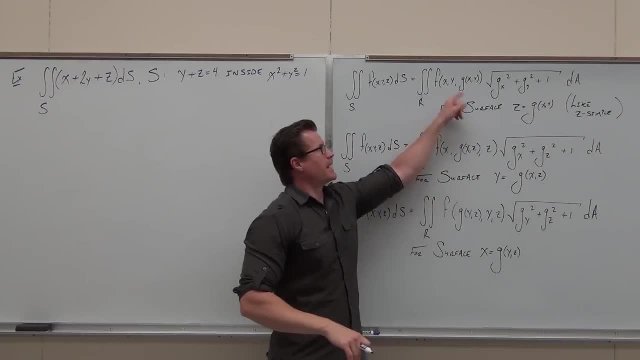 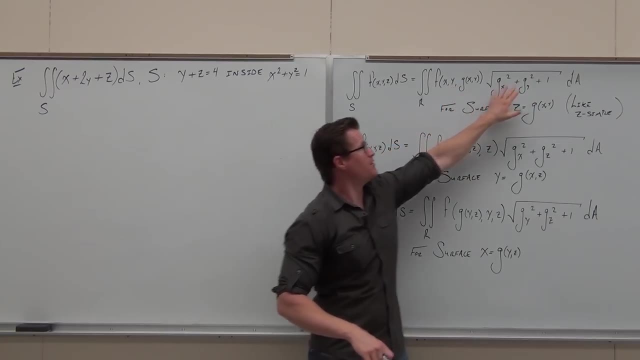 Do not miss this. This surface, it ain't coming from here. This is not your surface. This stuff, it ain't coming from the function inside your double integral. This stuff is coming from the surface that I'm giving you. It's coming from this. 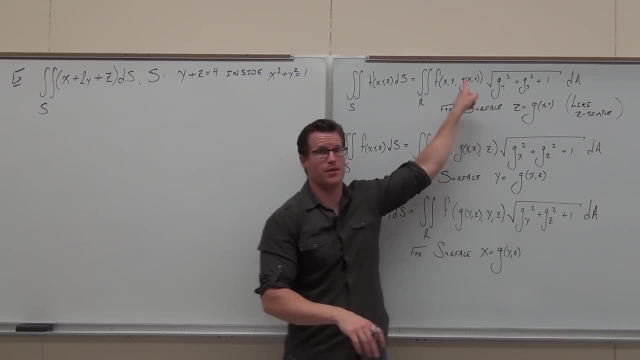 This is what gives you this and this and this and lets you redefine that. Does that make sense? It's all based on the surface stuff. This is just going to get redefined. It kind of plays along. It's second fiddle. 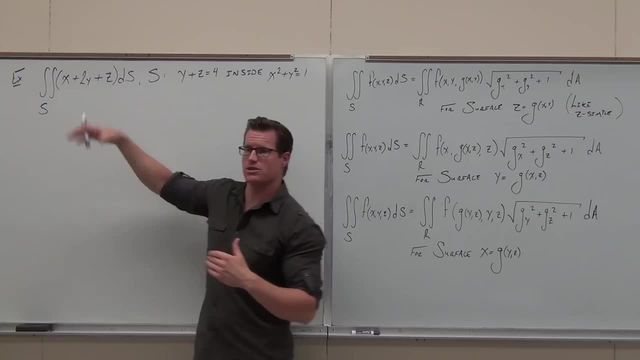 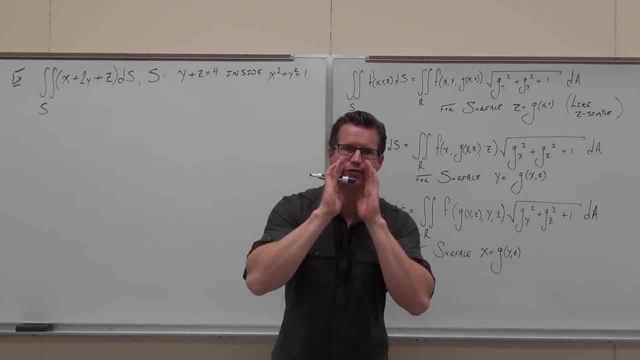 So this is going to stay. well, some of this stuff is going to stay. We're going to redefine one of the variables, depending on whether we want to pick z equals or y equals or x equals. but that all comes from the surface definition. 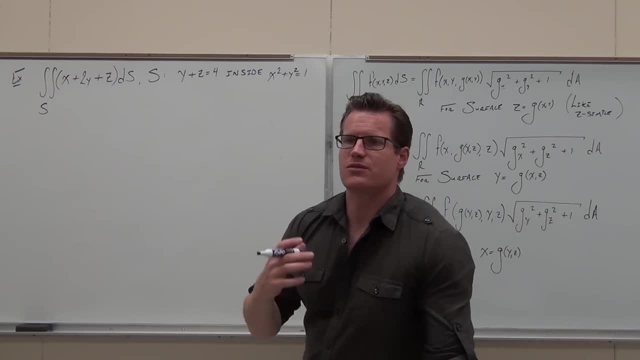 So we're going to look at that. What would the easiest variable be to solve for, Just like it's not z simple because we're not doing triple integral, but kind of like that. or x simple because we're not doing triple integral but kind of like that. 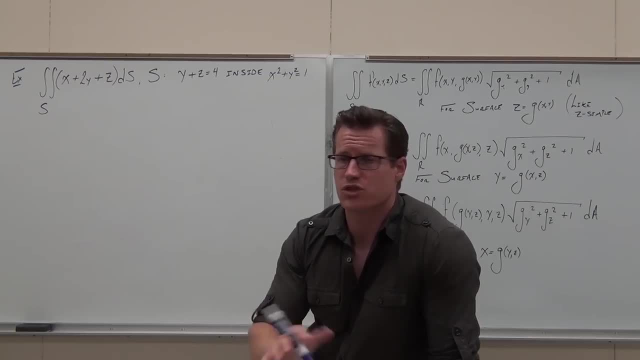 Let's look at the variables that would be easiest to solve for. Let's knock one just right off the top. Let's knock one just right off the table. Y. I would not want to solve for y. Why? Because I have two functions that both have y's in them. 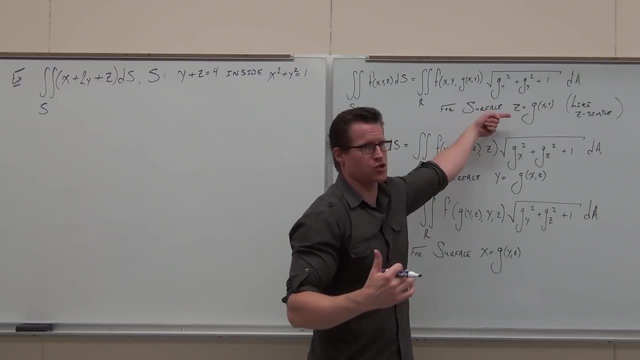 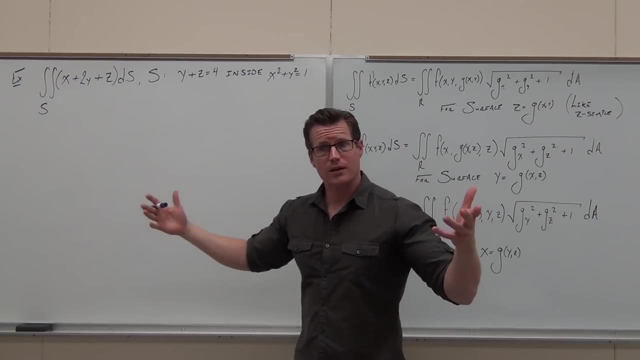 That would be pretty hard to do. if I'm trying to get one function, Does that make sense? Because I have y equals something and y equals something and it wouldn't be the same something. That would be hard. I could do x, I could solve for x over here. but that's kind of funky too, because I have a square root. 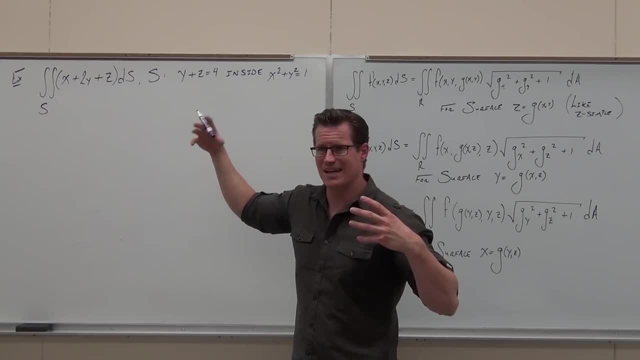 and it doesn't have a z and so I wouldn't be able to solve for that z That would encompass my other variables with that. Does that make sense? I'm going to look at this and go. well, I could solve for z. 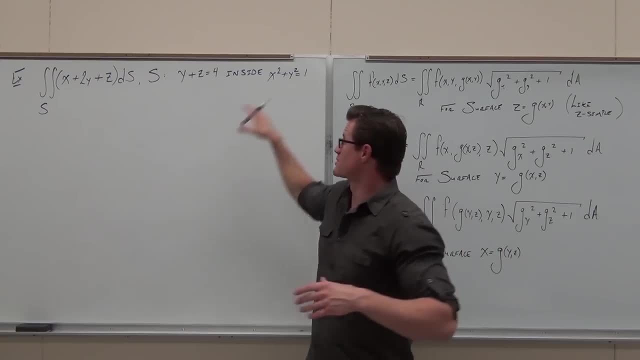 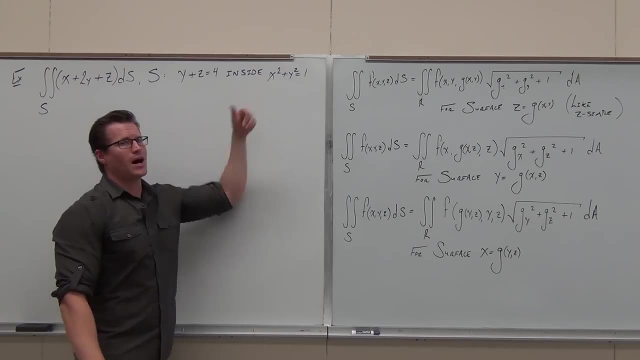 Now it doesn't have an x, but x is wrapped up in a cylinder. This is a cylinder that is plain, cutting through the cylinder In this case, because I don't want to solve for x, I really can't solve for y. 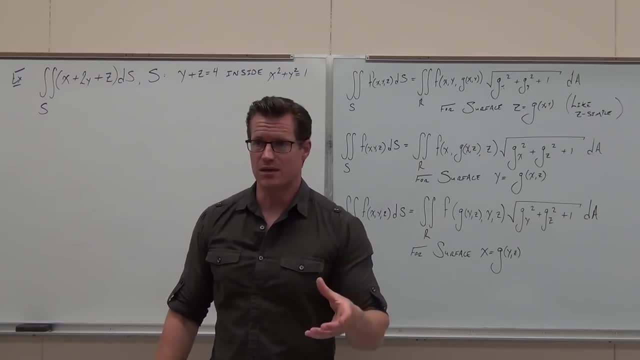 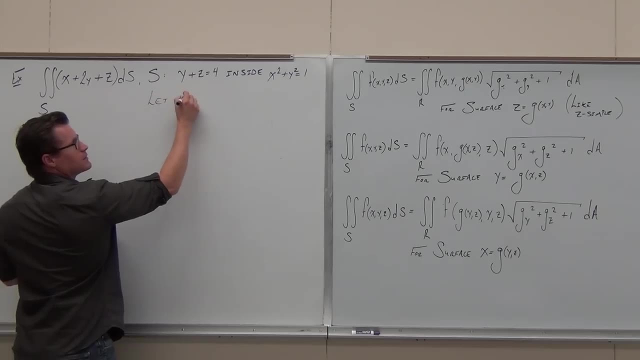 It leaves me with the only option. I've got to solve one of these functions for z. That will become my function Head down. if you're okay with that one, We'd say let's let z equal a function, A function in terms of x and y. 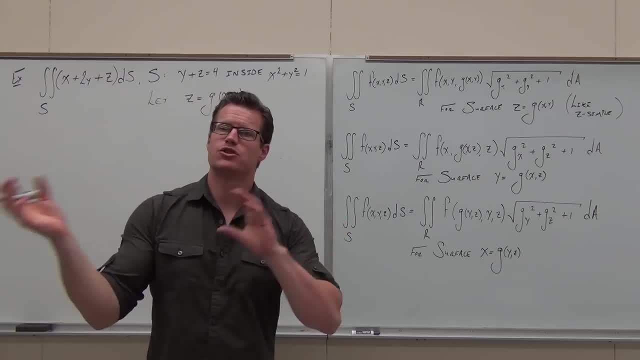 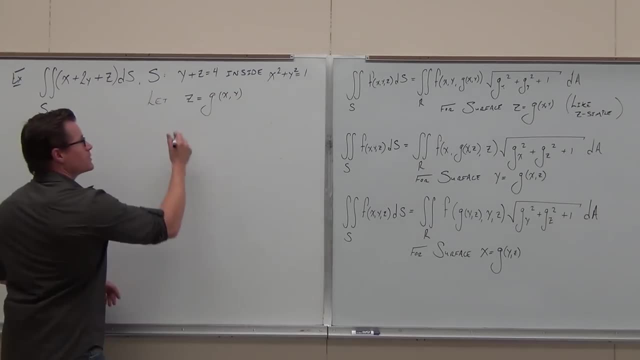 It doesn't have to have both x's and y's, but you can't have two different functions. That's why we didn't pick y. We can't have two different functions out of this thing. You have to have one function. In this case we'd say: hey, z equals 4 minus y. 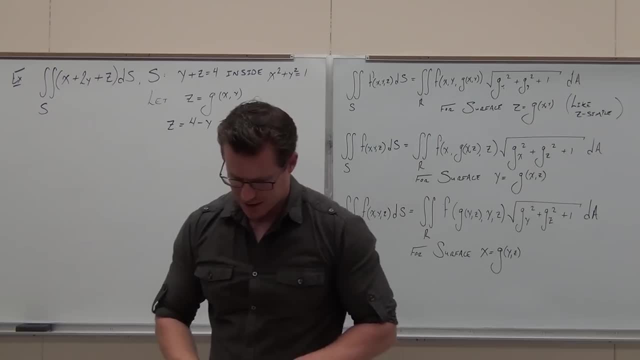 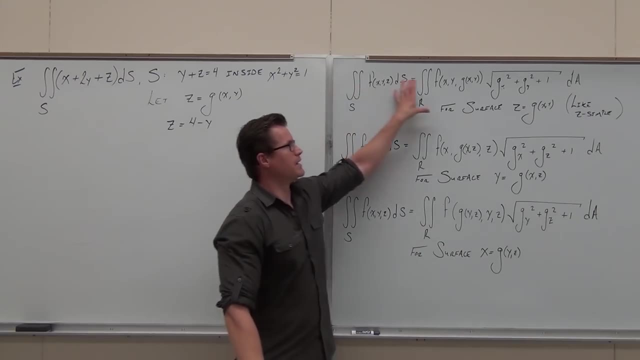 Pretty easy. I wonder if that makes sense to you, yeah or no? We've said no, no, yes. Here's how this stuff works. Please look carefully. I don't want you to lose it Again. you know how double integrals work. 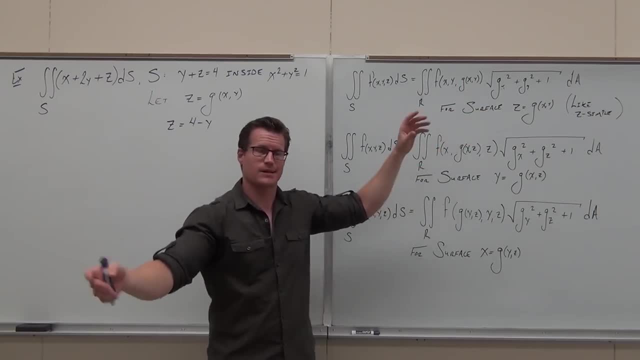 It's just the setup. The whole class has been set up. It's like the first two chapters. It says: well, let's start redefining it. Let's look at our region. We'll do that later. All about set up first, then look at the region. 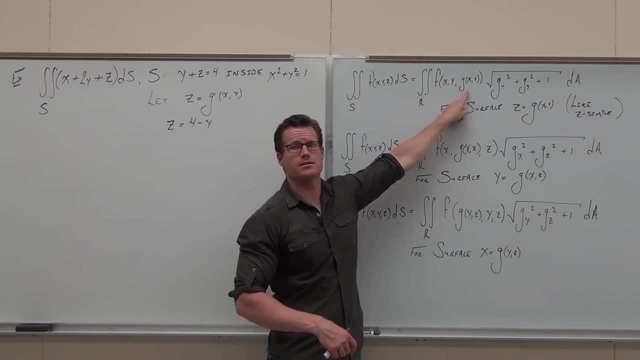 Let's look at the function, the mass density function. Could you redefine this so that you have only x's and y's And if you have any z's, you change them into x's and y's? Could you do that? Now that you've defined this thing in terms of x's and y's, the answer is yes. 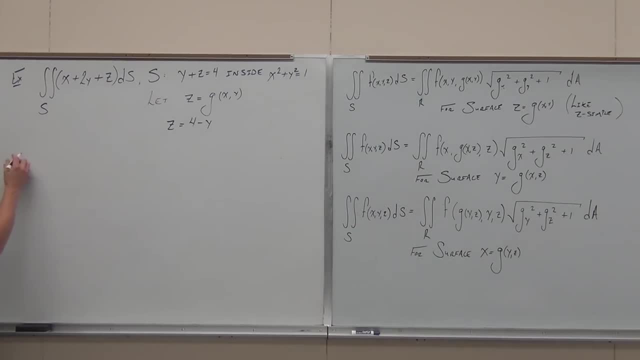 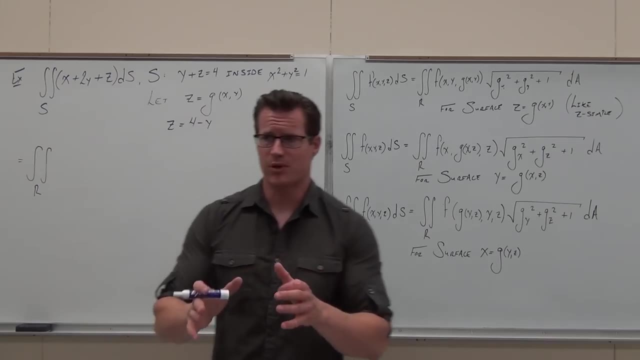 So let's start doing that. So, using formula number one, write your double integral Literally: write your r. Don't skip that step. I told you that last class. Do not skip that step. You'll deal with your region later, but get your setup correct. 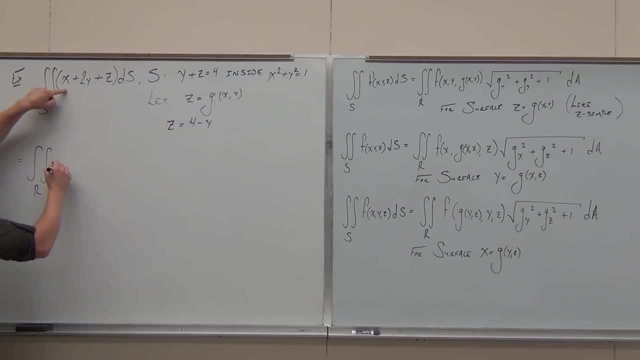 Hey, hey, according to this stuff, do I want x's? Are x's okay, Yes. Are y's okay, Yes, Are z's okay, No, No. So what's our z become? If you can make that jump, you're halfway there. 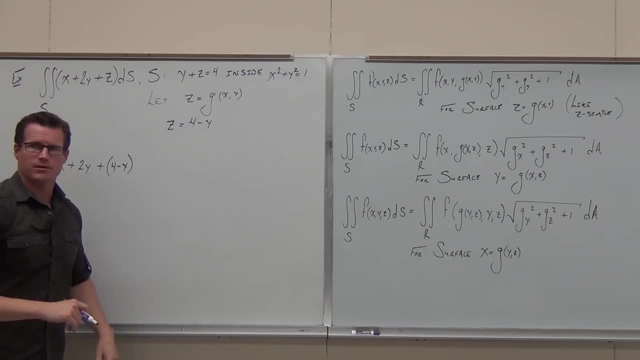 Are you guys okay with where that comes from? You need to find one of your variables in terms of the other two, because we don't have a triple integral, We have a double. That means only two variables, So you've got to pick one. 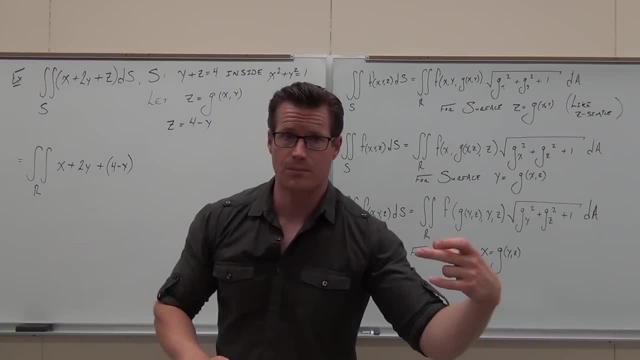 You can't have x's, y's and z's because you're only integrating two times. You've got to integrate two times, You get two variables. That's why we did that. So this is our mass density function as redefined using the surface that we're going to use. 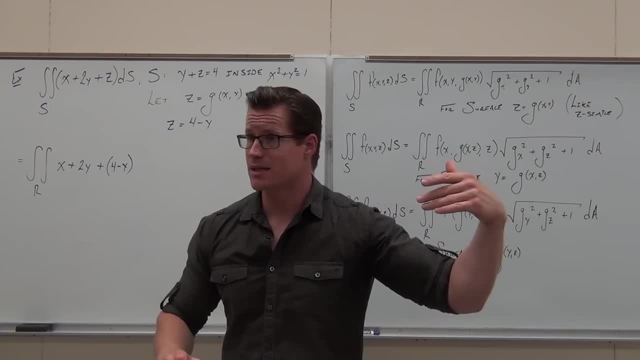 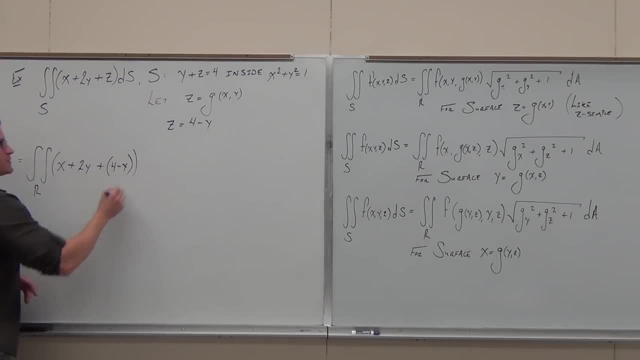 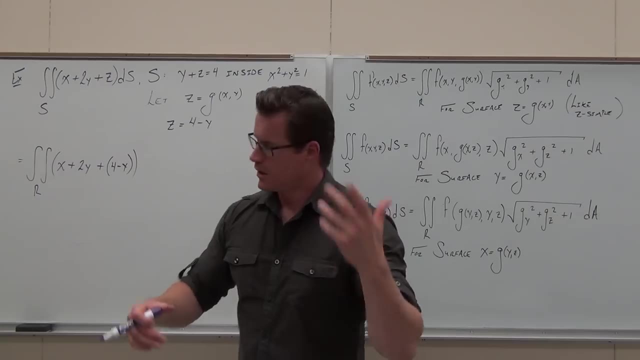 You get two variables. That's why we did that. So this is our mass density function as redefined using the surface that we're going over. That's the idea, And I don't know if you're okay with the idea. Now the df. 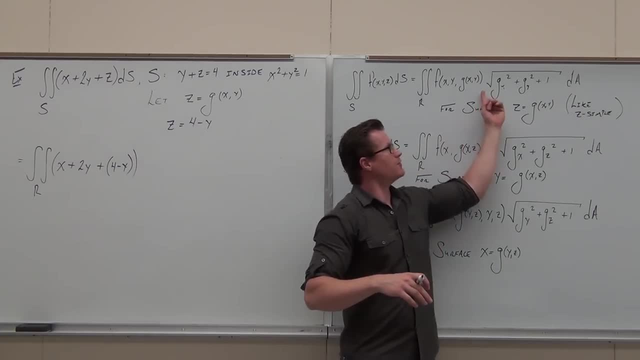 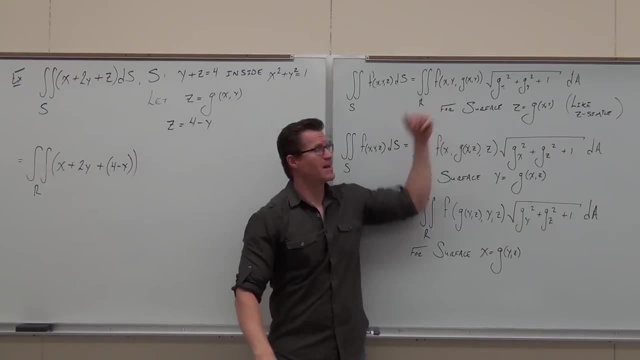 Okay, this stuff. That's the idea of surface. Hey, look at that. If ds is the idea of surface area and that's the mass density function, we still have the mass density function. ds is surface area. right, This is surface area. 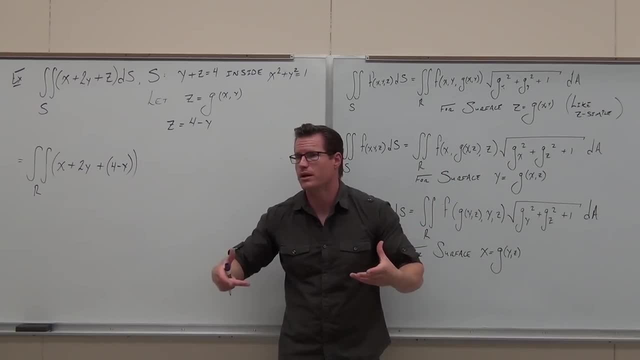 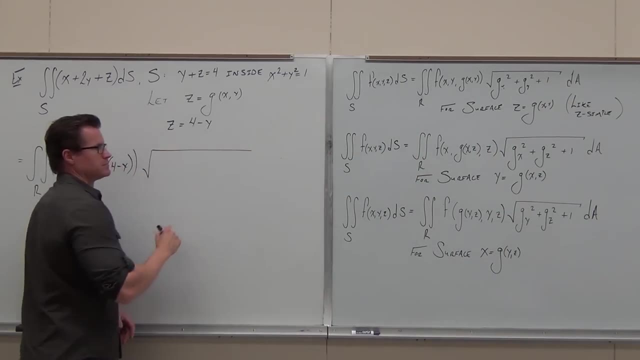 Over that region. the projection of s onto a corner plane? No problem, That's just surface area. So we rewrite it. Okay, Surface area. I know it's going to be a da. Don't change that yet We don't know if it's dx dy. 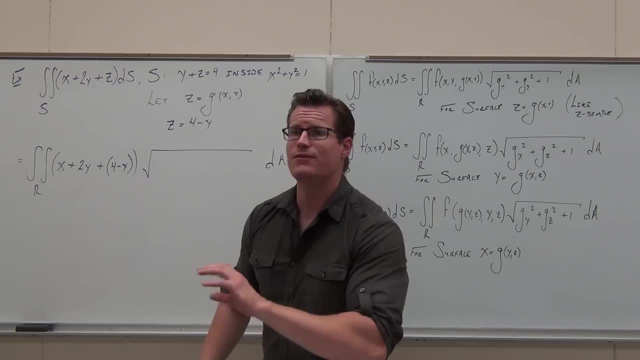 We don't know if it's polar, rd, rd, theta, We don't know what it is yet, So you leave it. Don't do that. Don't do anything until you've actually drawn the region. Are you listening to what I'm talking about? 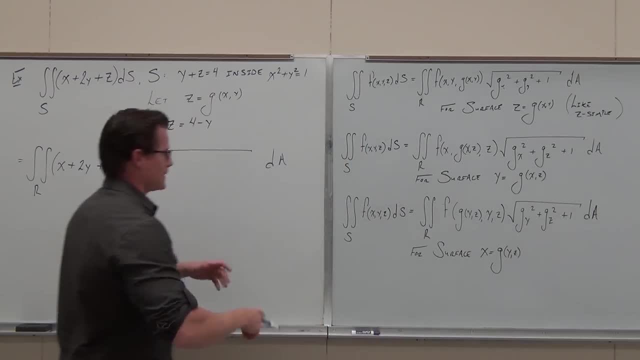 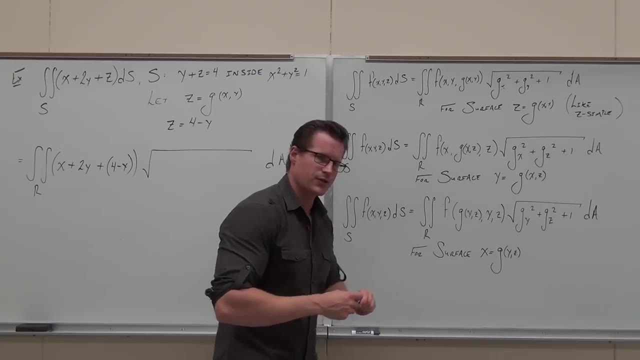 Please don't do anything with this yet, because you don't know what's going to happen unless you draw the region first, Which we're not going to do. Now, what this stuff means, it's kind of some different notation. We're going back in time a little bit. 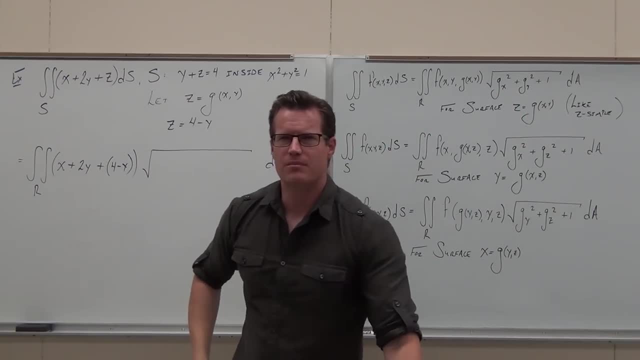 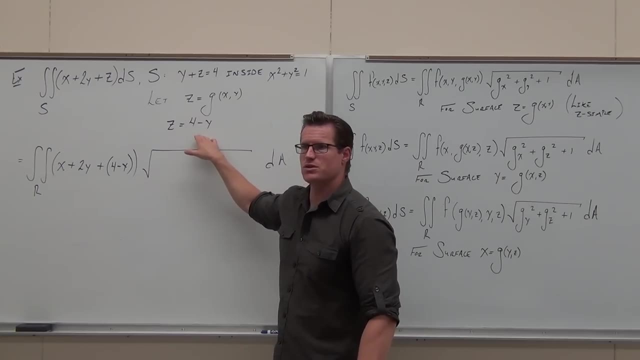 Do you remember what that g with a little x, the subscript, meant Partial derivative of g, whatever you defined with respect to x and then with respect to y, the two variables that you just redefined your function as. So let's do that. 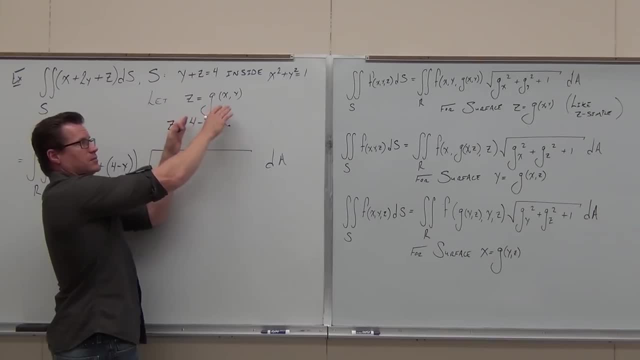 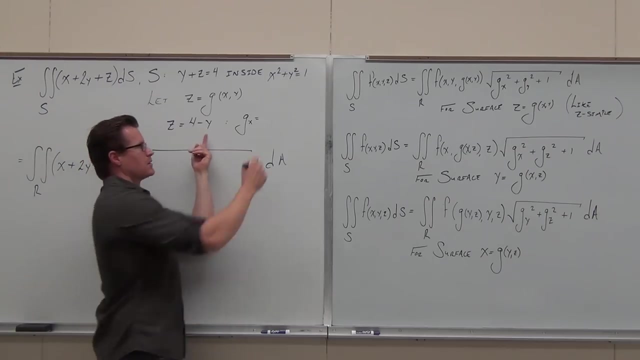 So if this is, look, hey, if z is the function g, then we should be able to find from this partial derivative of g with respect to x: Hey, what's the partial derivative? this is g. Partial derivative of g with respect to x. 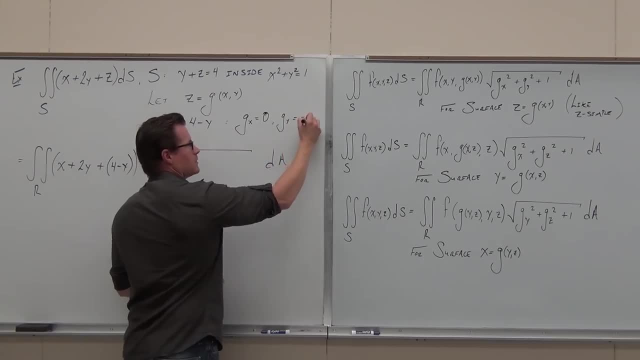 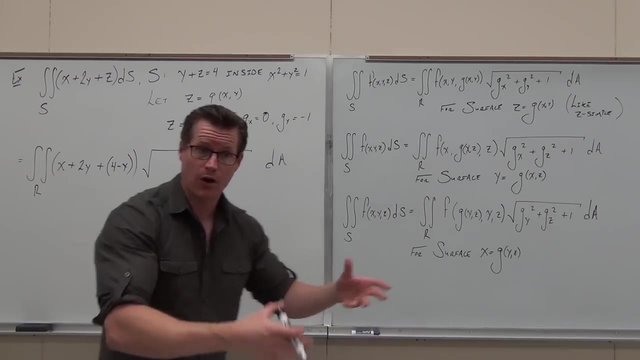 Partial derivative of g with respect to y Hard. You just got to follow it. You just got to know what it means. And if you know what it means, it's easy to follow. Just put that stuff in here, So OK. 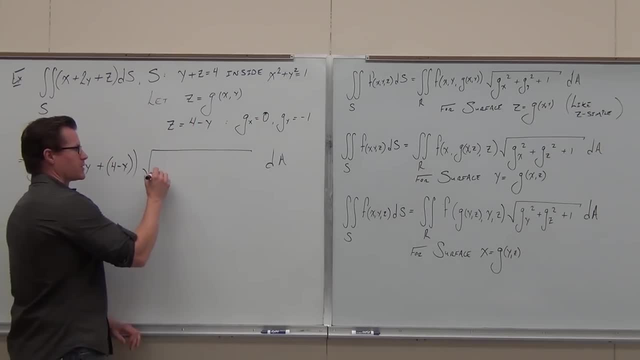 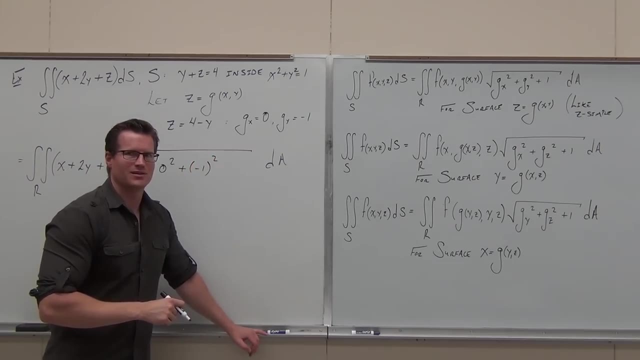 Well, it looks like we have gee tough one: Zero squared plus negative 1 squared. Is that it Plus 1.. You know, some people are going to forget the plus 1, right, Don't forget the plus 1.. 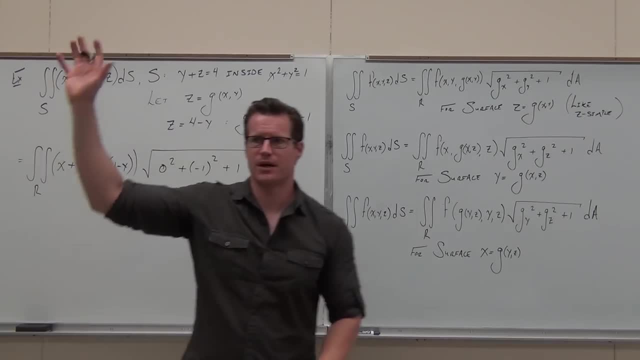 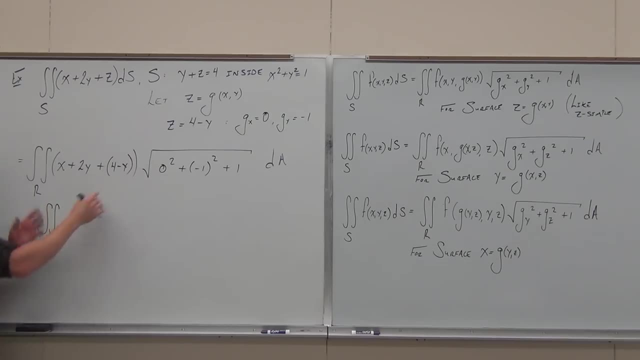 That plus 1 matters, So fancy girl art with that one. OK. So let's clean it up just a little bit. Combine like terms. You know this from basic calculus. You know this from basic calculus. Combine like terms before you do any integration at all, like ever. 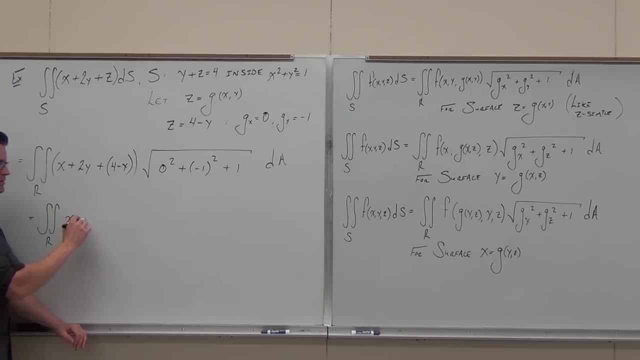 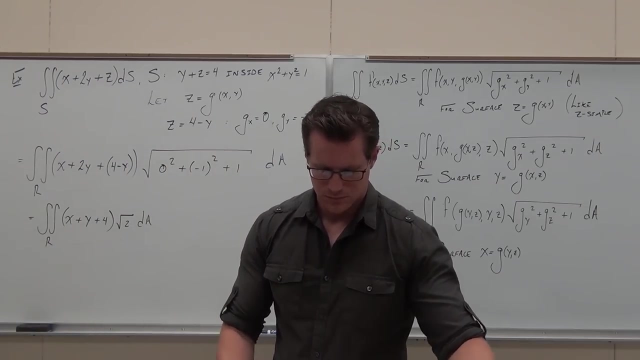 So here we have x plus y plus 4, and then we've got this square root of 2 hanging on dA. OK, Right there, I'm going to do a little pause. OK, I want to make sure that this is totally, totally understood by you about where all. 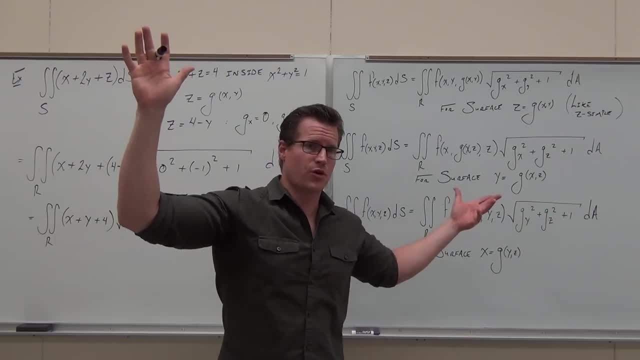 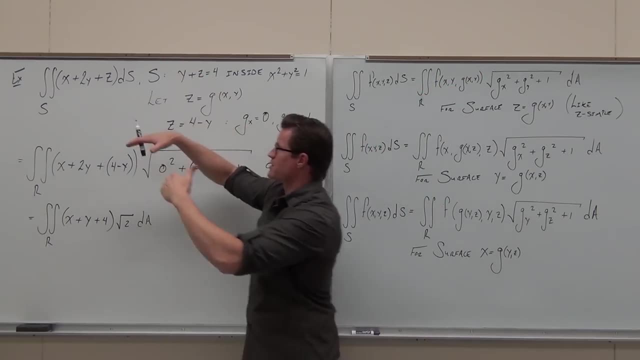 of this stuff comes from. It depends if you feel OK with it. Literally just a formula. It's a surface area from before which we didn't cover, but it's there times, mass density. at each point We make our transition by saying: let one of your variables equal, the other two become. 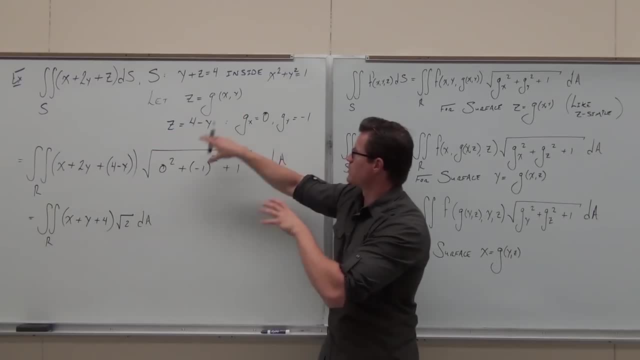 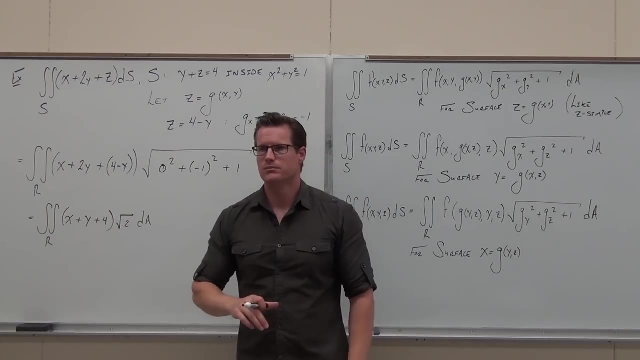 a dependent variable. It lets you parameterize according to those variables, lets you find partial derivatives- really nicely- lets you do something kind of simple and it leaves you with a chapter to go. It leaves you with: hey, if you ignore all of this stuff and just look here at the bottom, 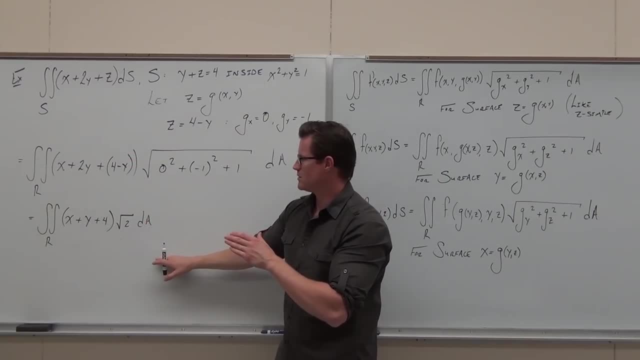 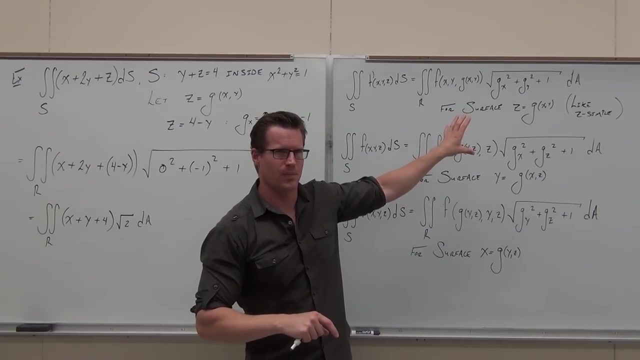 and just look here and say, well, that's a double integral. What's your region? Your region is the projection of this thing onto. OK, now you think back to this. If we let z equal something, it's very much like being z simple. 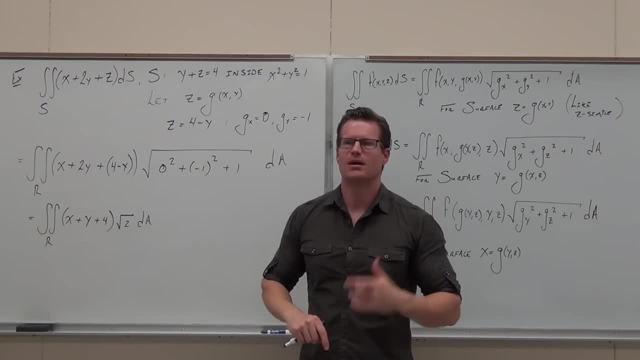 What plane is this projection going to be on? Yes, That's why I said: think like it's z simple, Because it's going to have your brain go. z simple means my r is on the xy plane. That's why I said: think like it's z simple. 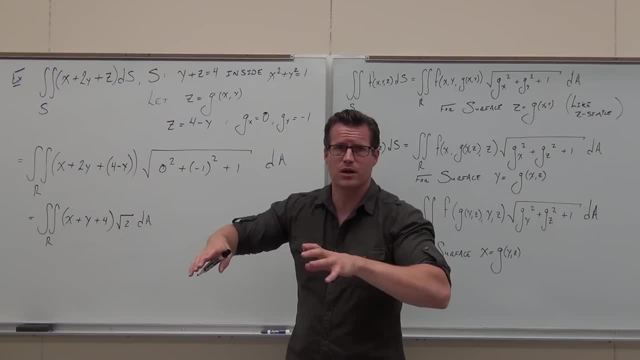 Because it's going to have your brain go z. simple means my r is on the xy plane. That's exactly what's happening. You're kind of cheating a triple integral here. OK, You're kind of cheating a little bit, That's OK. 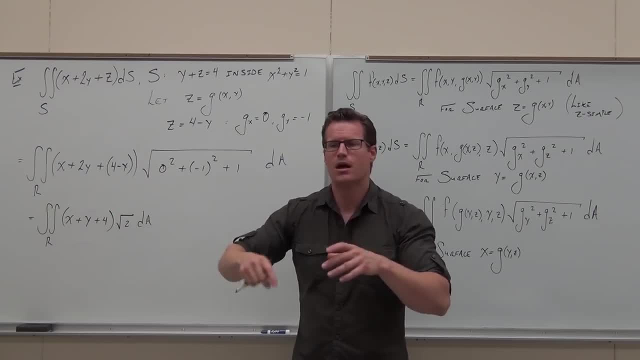 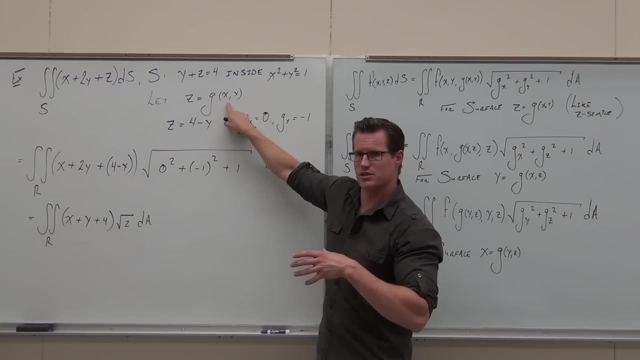 We're just redefining in terms of two variables and using that, The projection will be on the plane that you redefined. as Does that make sense to you? This r should be on that plane. This r would be on this plane. 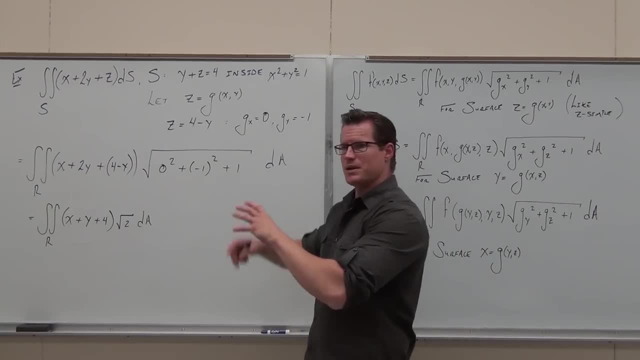 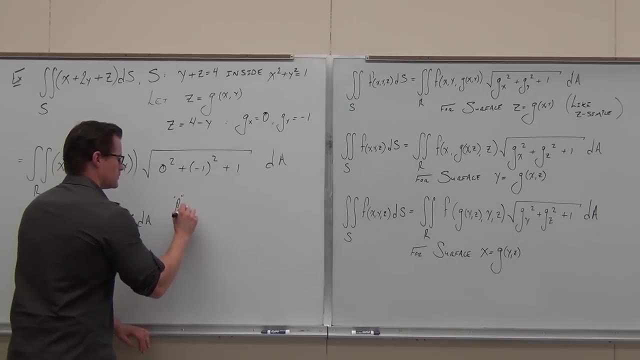 This r would be on this plane. That's where it comes from. So because we picked, z equals function of x and y- our region- our r is on the xy plane. OK, Thank you. So let's do this. This r looks familiar. 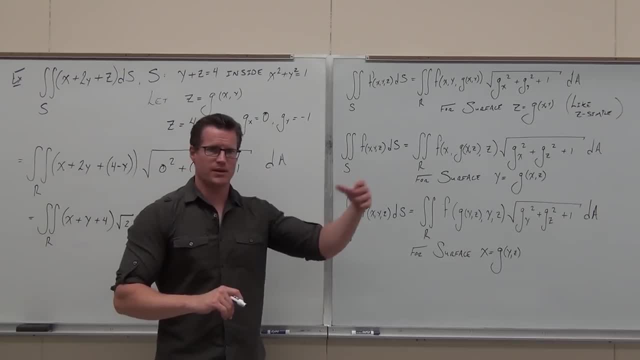 Right before this. for triple integrals, we just let z simple and then we'd have r is on the xy plane. Draw it, Man. this stuff should be coming back to you. We always draw our region, like every time. Draw it. 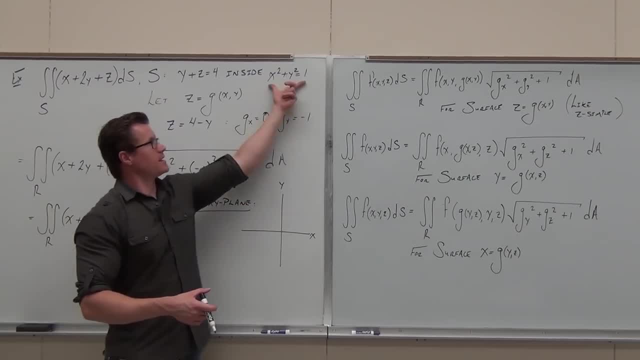 Just draw it, OK. so what's going to happen is this: Hey, can you put that on the? Oh my gosh, look at that. How about that? Can you put that on the xy plane? What is it? 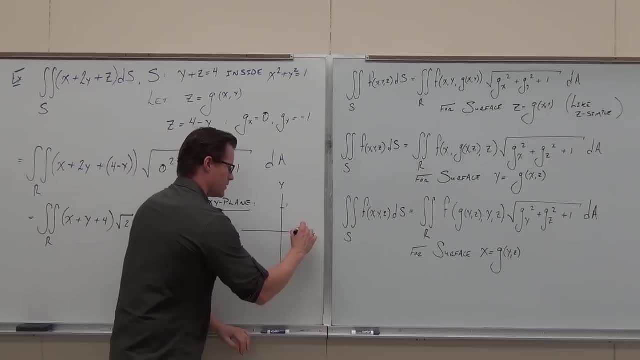 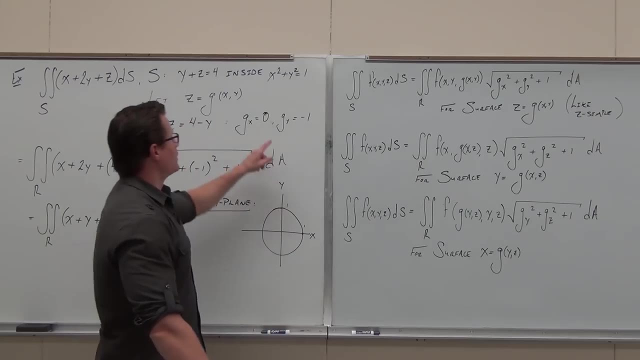 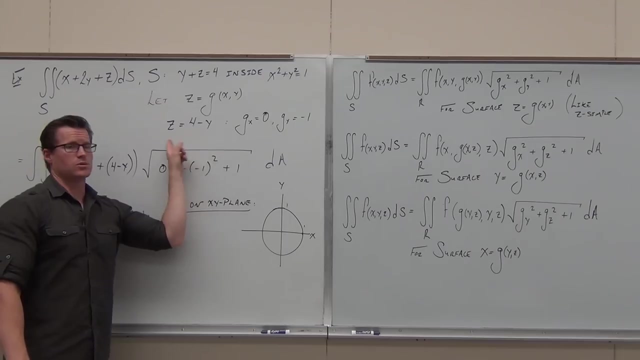 And it's the liberty on the x- y plane. Getting kind of tired of that Same thing. Oh, at least it's nice. Now can you put this on the x? can you put this, this one, on the x- y plane? 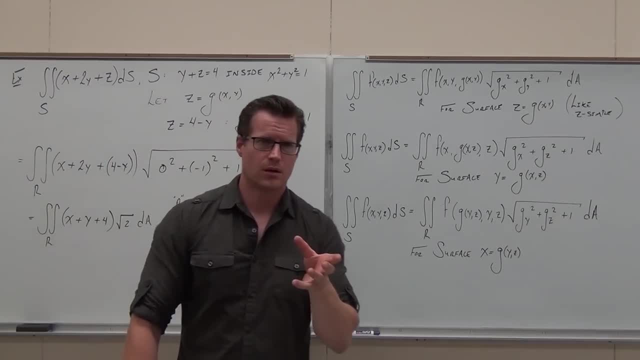 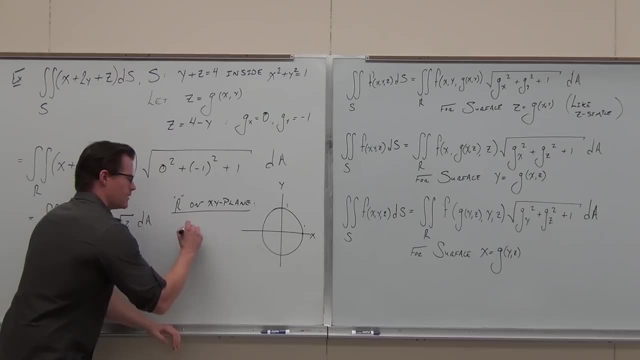 or this, it doesn't matter. Can you put that on the x? y plane? What's the value of z on the x? y plane? So x squared plus y squared equals one. That gave us a circle, Z equals. I'd do it this way probably. 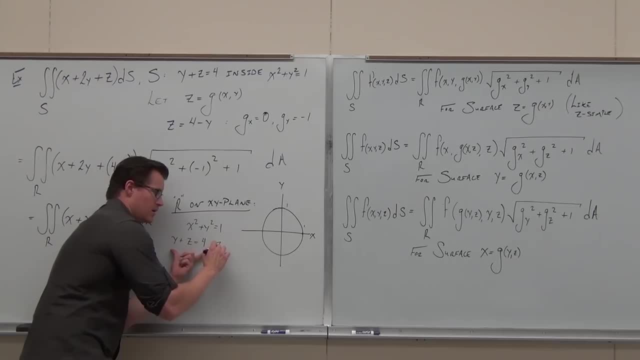 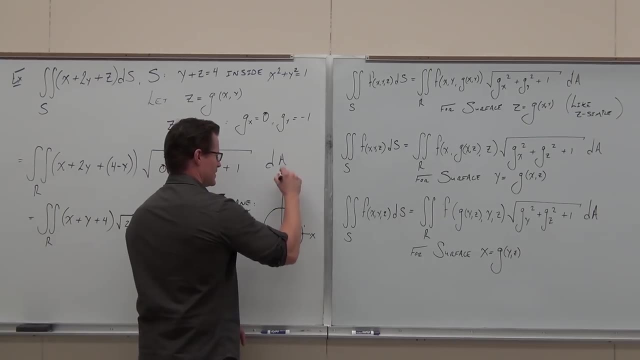 Y plus z equals four. on the x y plane means z equals zero, which means y equals four. You go wait a minute. Y equals four. that's like way up here. That's y equals four. that's what that is. 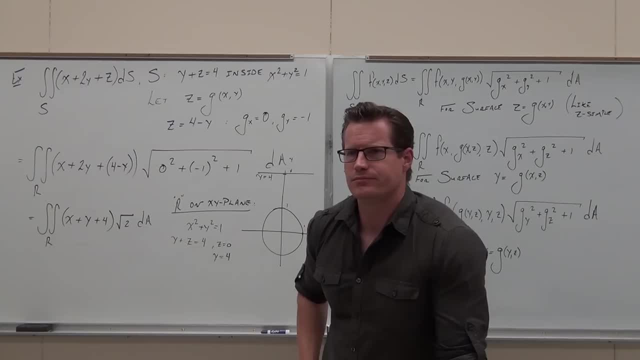 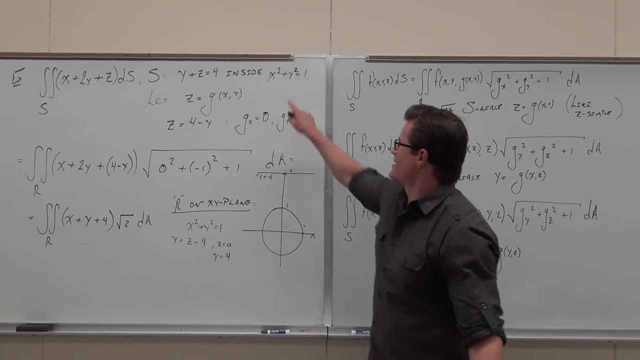 Here's a weird question: Why don't they intersect? Think about what this is. What is this? Come on people. what is that Along? what axis Z? It's going like this at you. What's this? Don't say a line. 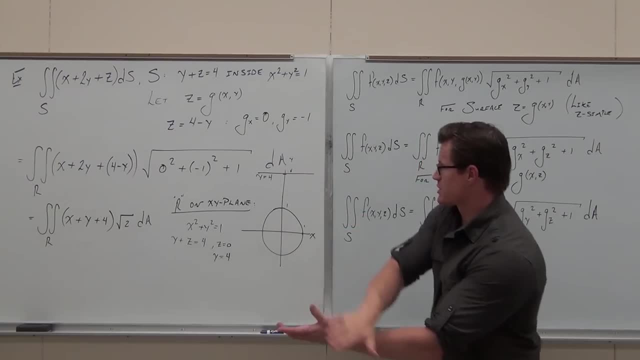 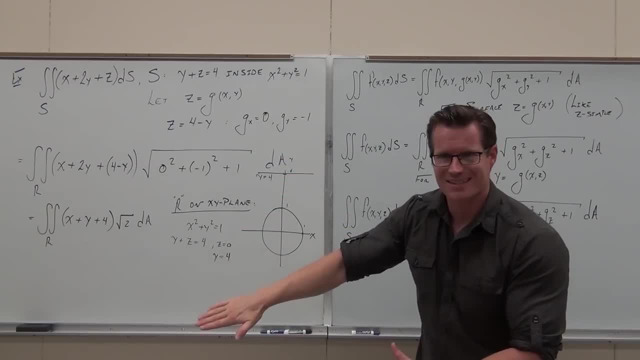 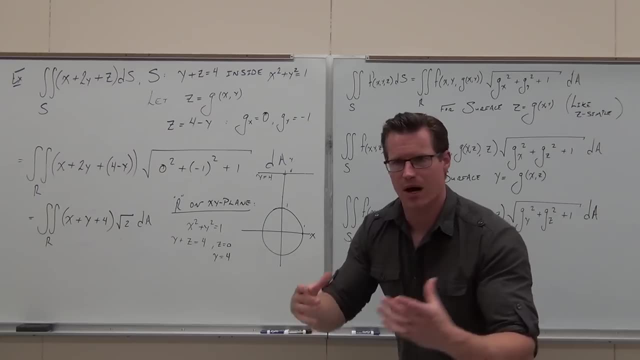 So you have a cylinder, you have a plane. It's slicing the cylinder, but not on that plane, not on the x- y plane. It's just out here in space. So the surface we're talking about is the surface that's created. 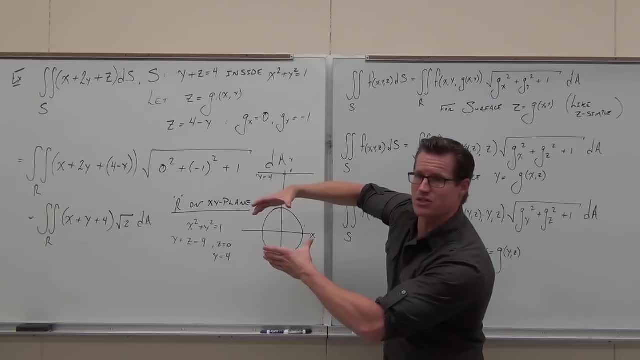 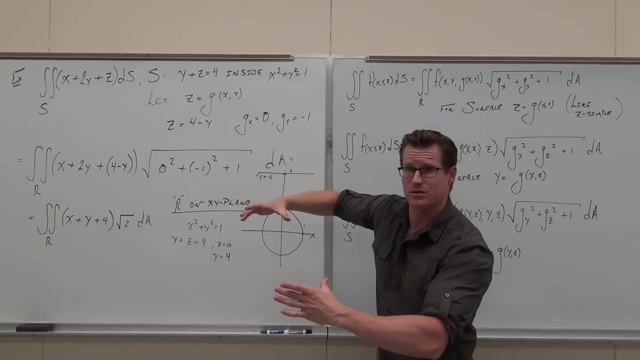 when this plane slices through this cylinder and gives us this oblong shape right in the middle. That's why it's not flat, because it's not flat with any of the chord planes. It's coming through space like this. It gets us a flat. 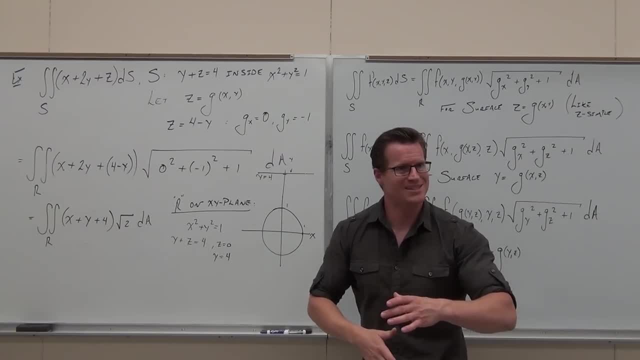 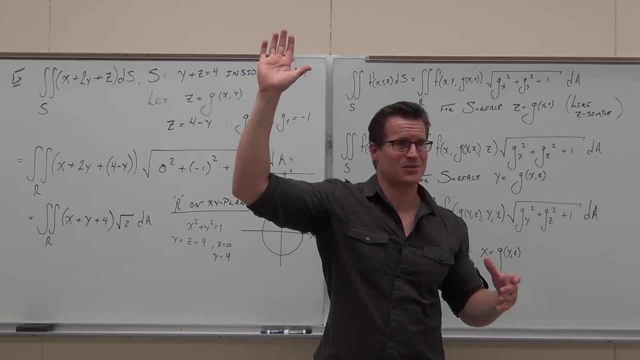 stretch out disc. That's what we have here. Show the fans. you understand the concept. That's pretty cool, right? That's what we're doing. That's why they don't intersect, though They're intersecting in space. Does it bother us? 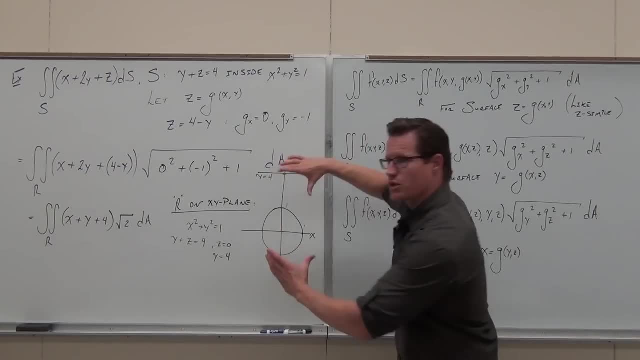 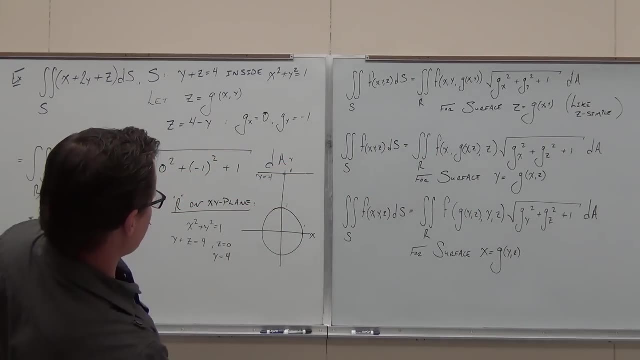 No, No, we don't care, because all that's happening. when you look back at this, you are literally looking where this plane slices your cylinder. You're looking down at it and you're saying, hey, where that plane comes out, it's slicing the cylinder. 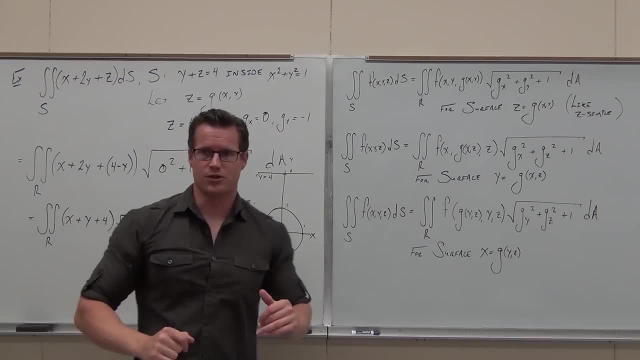 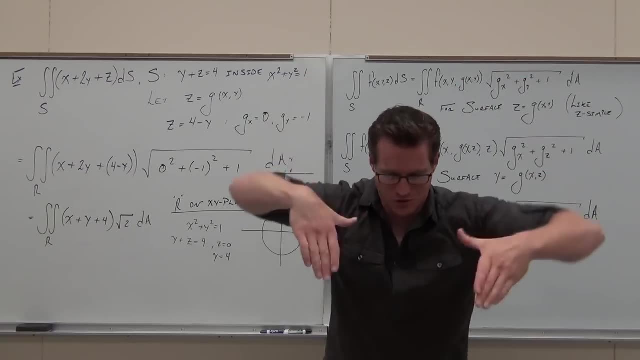 That region is all contained within that cylinder. Do you guys see it? It doesn't matter that it's slicing above. This is still your region, That's still ours. It's a projection of your surface. If you were looking down, right, right down on top of it. 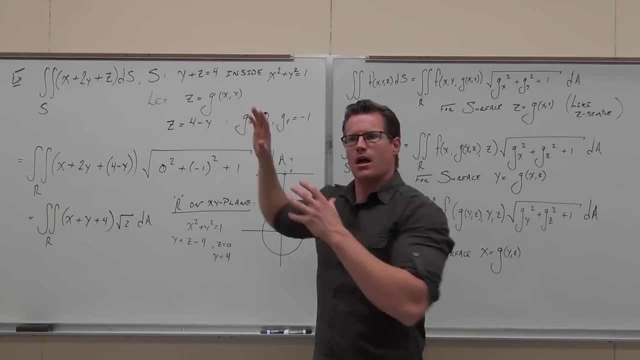 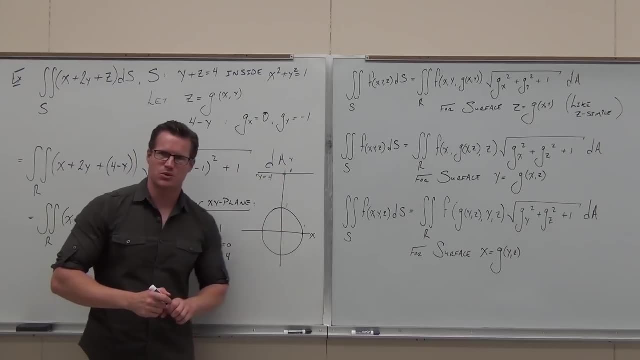 it'd be what it creates on a coordinate plane. So if you're all right with that one, that's your R. Now you tell me, after all the calculus you've done, all the double integrals, how would you choose to define that? 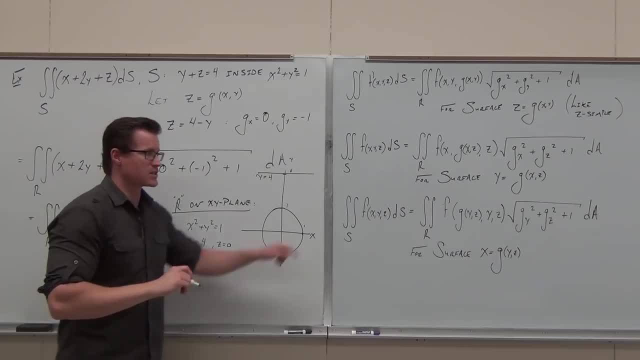 A little lower, A little lower, A little lower. Now you watch carefully, okay, because this is very important for this stuff. As soon as you start doing polar and you start saying this and you start to please watch. 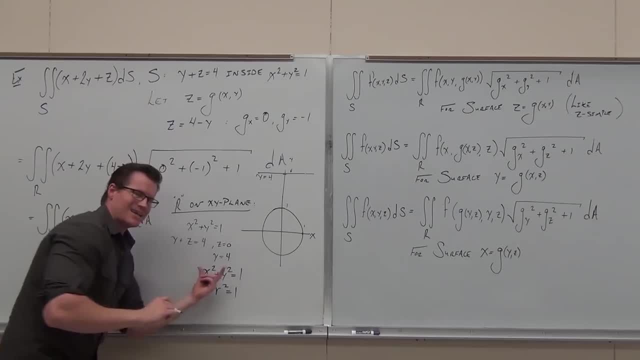 as soon as you start saying: well now, R squared equals 1,, as soon as you make that jump. look carefully: as soon as you make that jump, it doesn't have to be X and Y, right, It could be X and Z or Y and Z. As soon as you make that jump. from now on, 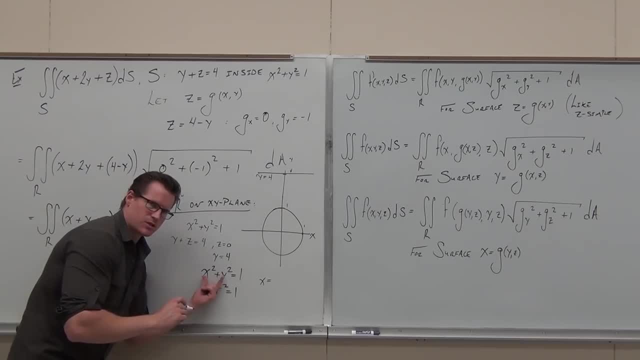 I want you to say: well then, define these two variables, because when you make these two variables, when you make the jump into R, X has to be either R cosine theta or R sine theta, depending on what axis you're choosing. 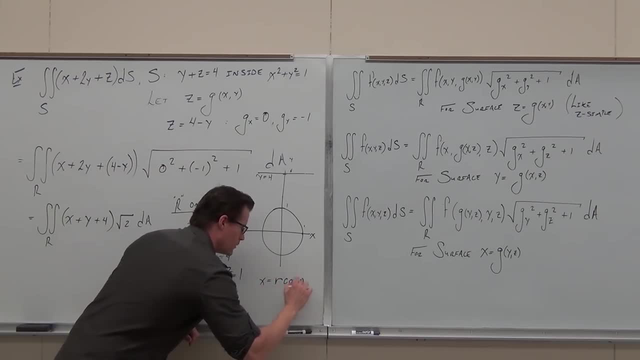 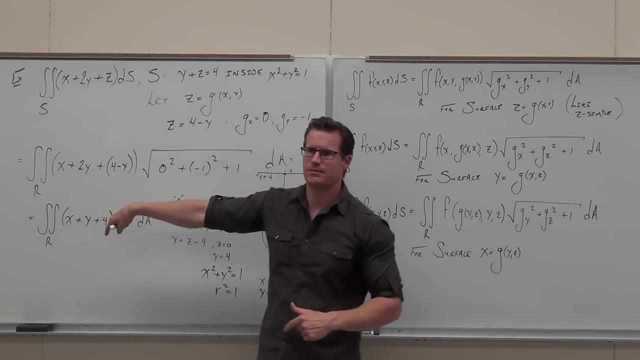 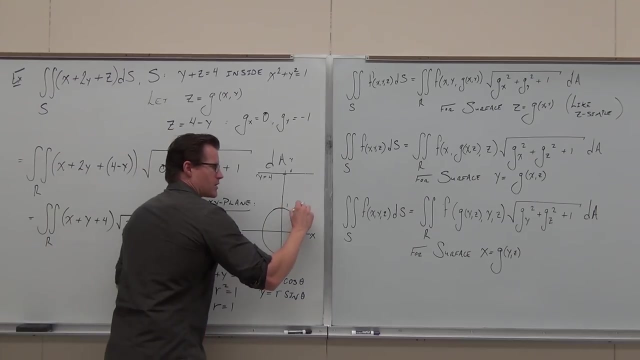 We're going to choose R cosine theta, which means that Y has to be the other one. What about Z? I don't care, if I want to change this, You'll just have X's and Y's. So this is our new function in terms of polar. and now, now we make the jump. 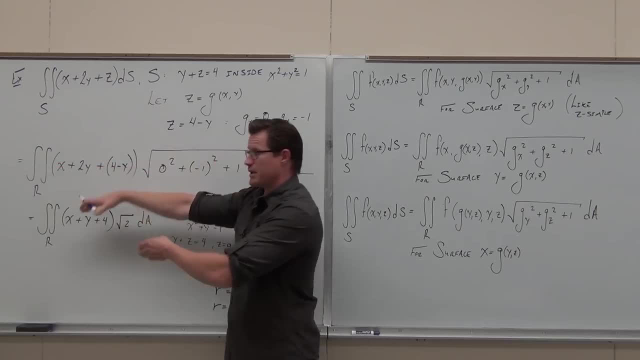 So we don't, we don't have to do that, We don't even talk. look it. we don't even talk about R until we get right down to here And then go: hey, double integral, Project the picture of your surface onto a coordinate plane and look at what you have. 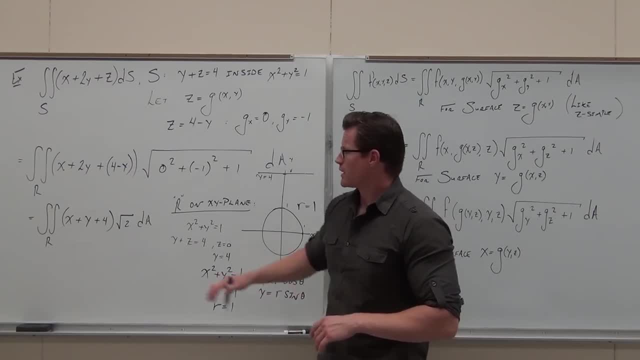 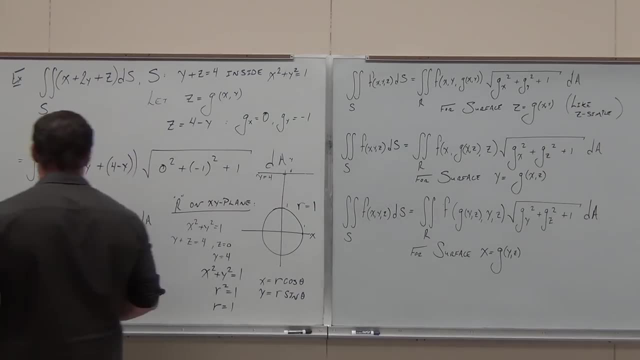 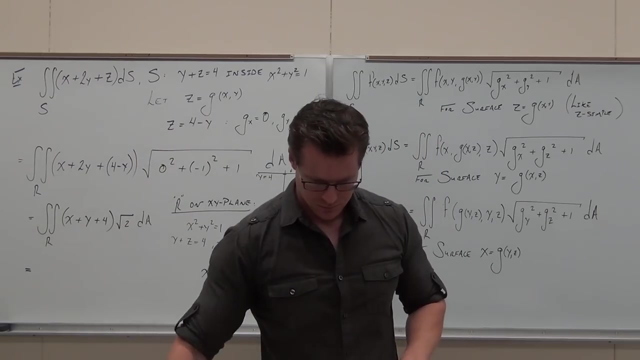 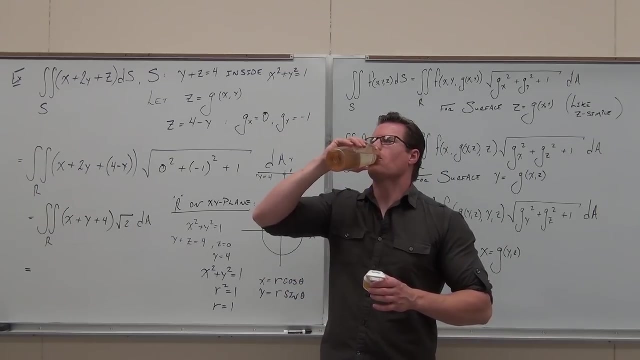 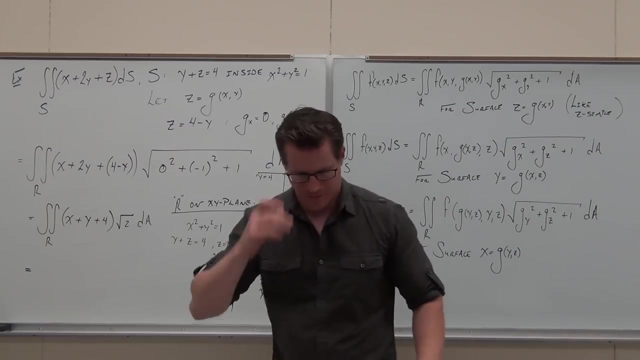 If it's a circle, or that's pretty nice, use polar. Can you please redefine this double integral in terms of the region you've now created? Keep in mind it's a full circle with a radius of 1.. So let's see. 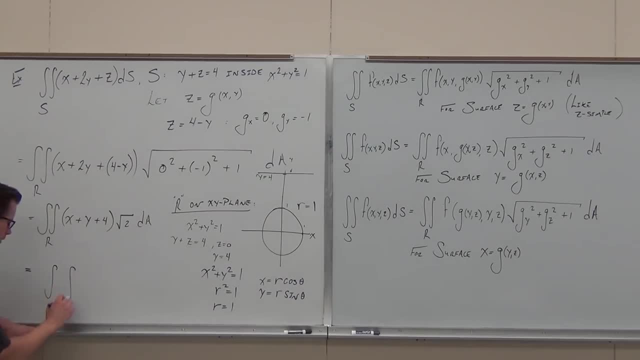 So let's see, Should you still have all of this stuff? Not, if you did that. That's why we wrote this stuff out, because you're not going to get a whole lot. You could, I mean you could get like X squared plus Y squared in here, but you don't have to. 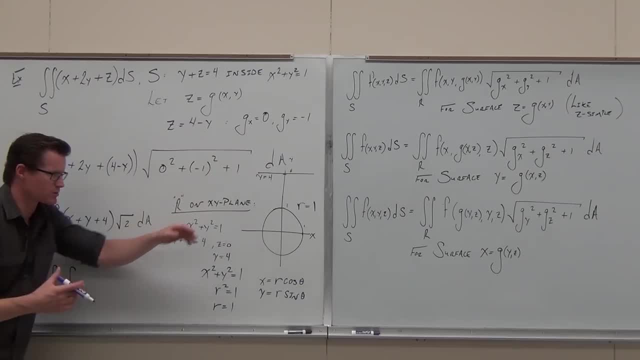 If you get X's and Y's or in other ones X's and Z's, Y's and Z's, whatever, you'd have this redefined already if you did this. So as soon as we choose polar, you have that definition. so let's write that. 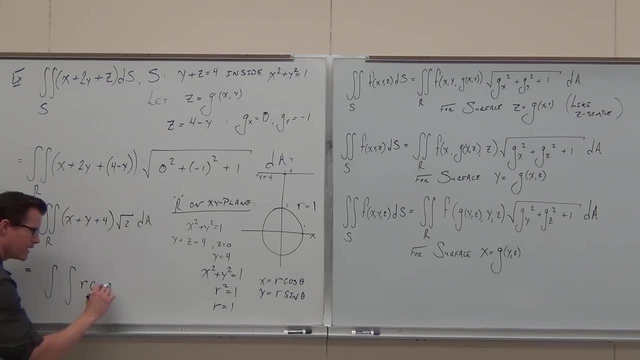 Instead of X, I'd write R cosine theta Plus. instead of Y, I'd write an R sine theta Four. Yeah, Square root of 2.. Yes, Then what? Square root of 2.. Square root of 2.. 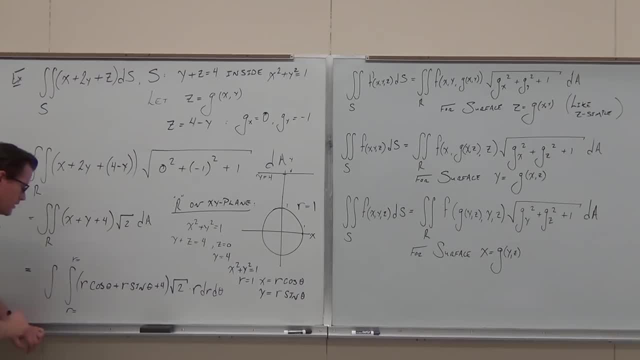 And we know this already. This is old stuff. We always go R to R first, theta to theta last. We've got to match these up. with these things, R goes from 0 to 1.. We're in our region, Right here. 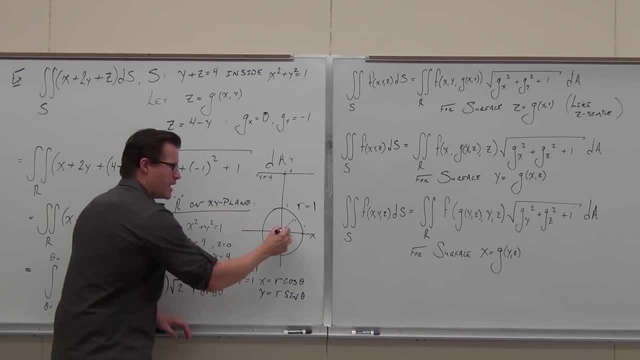 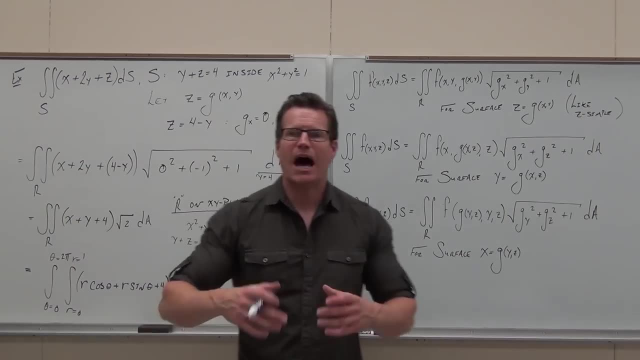 This is literally the region you create when you're looking down at your surface on top of a quarter plane, And then we're going to go around for a full circle: 0 to 2 pi. That's it. After you understand the concept of how to change these really weird things we're creating. 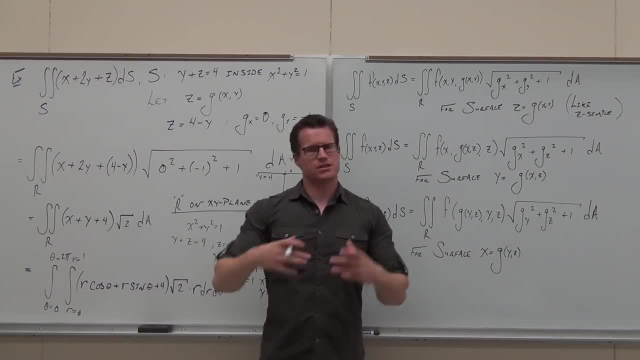 into some double integrals you're used to. this stuff gets pretty easy. It's all about understanding how to go from here to here. After that, it's just double integrals. It's just some regions you're going to be really, really used to. 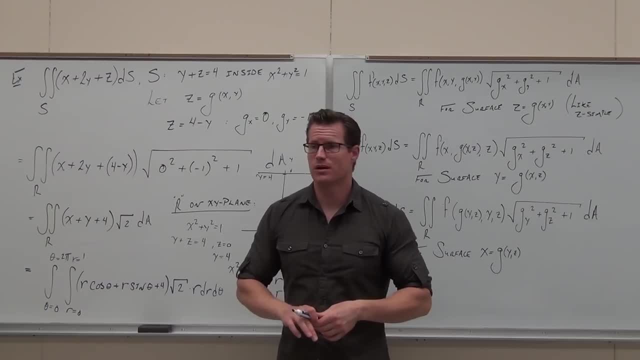 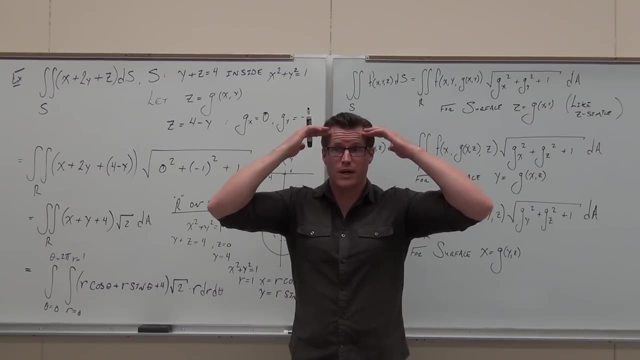 Kind of like Green's theorem: right Makes a double integral pretty easy. one deal with the region, you're done. Sometimes this stuff looks so overwhelming. When you look at it you go dude. these symbols look crazy. What's going on? 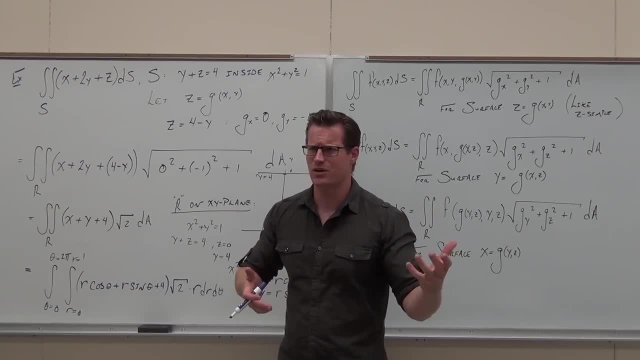 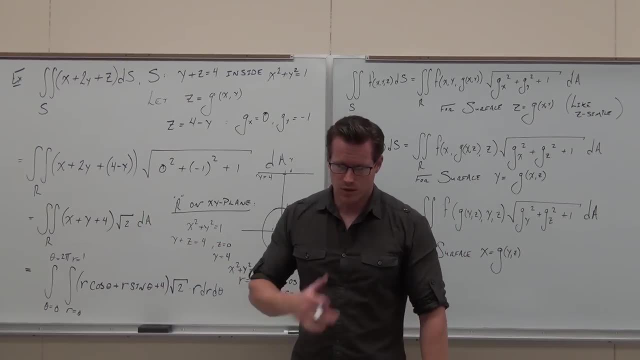 But once you understand them you go: oh that's it, I'm just getting double integrals over a really easy region. That just made my life actually easier, not harder. easier. This is nice. Now you work it out. 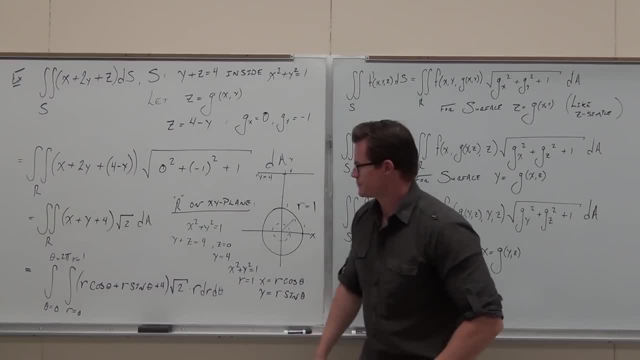 Would you know how to work that out? What would you do? Distribute the R- Don't forget the R. Distribute the R. Integrate with respect to R: Do plug in 0 to 1.. It's going to be kind of nice. 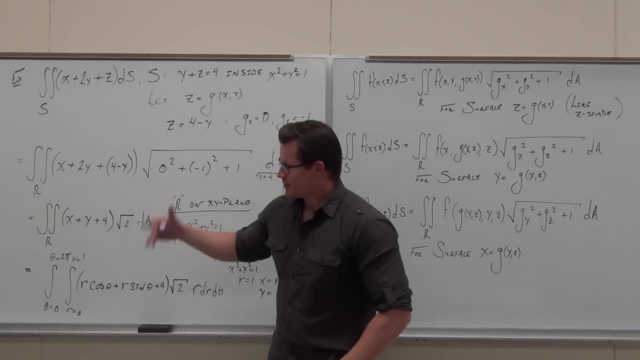 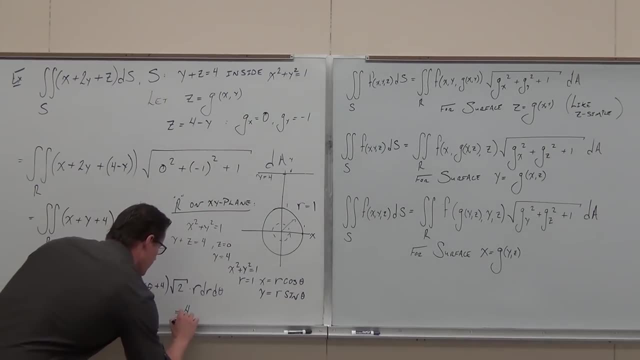 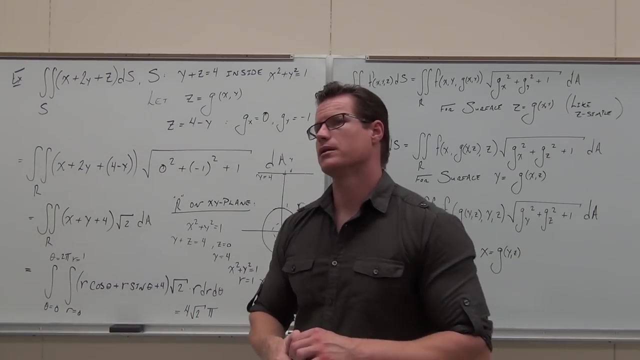 Integrate with respect to theta. You've got some sines and cosines in there: 0 to 2 pi. What you should get is 4 root 2 pi. Now tell me what that number means. What is that? 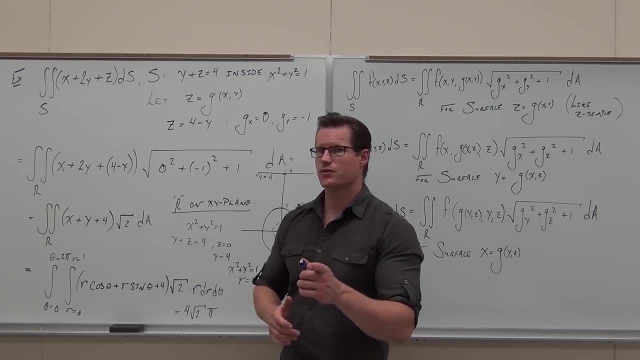 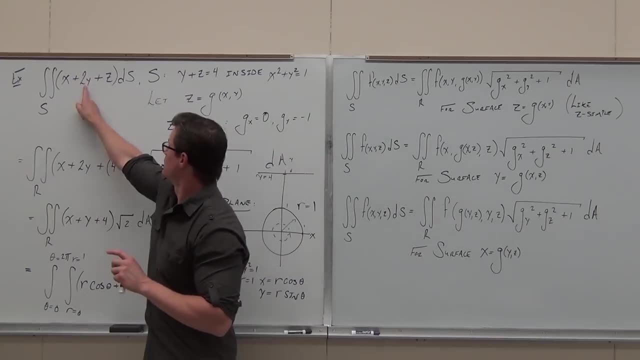 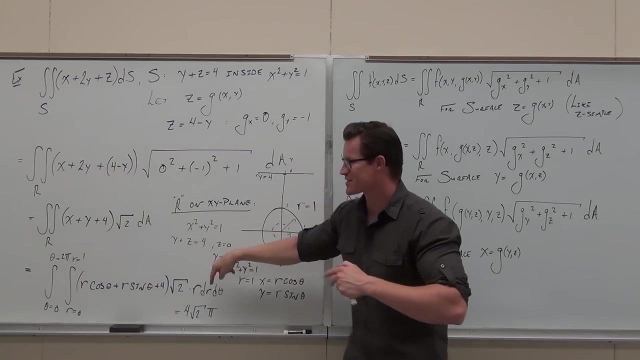 Say it louder: No, it's not surface. Okay, now, this is a good teaching moment for you. If this was 1,, if that was 1, and that was 1, and that was 1,, then this would have been surface area. 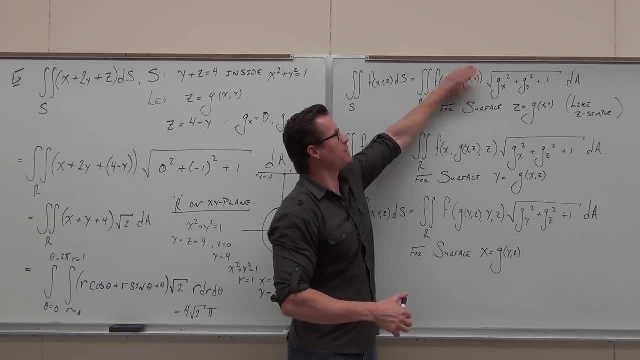 Did you guys catch that? That's the whole point of the 14.5 thing. If that's 1, surface area, Did you guys get it? That's all that's happening. What is that? What is it? Come on. 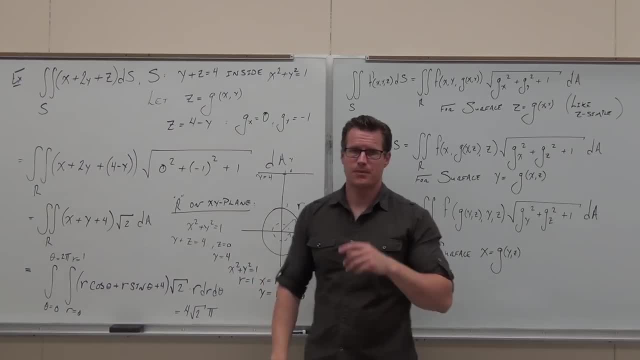 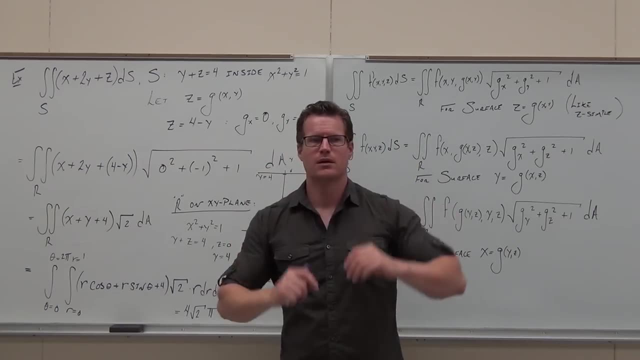 What is it? Mass density? What is this? Mass Of what? That's surface? Mass density, Mass of that surface, A really thin plate That's curved. Perhaps it's not, But really thin plate, That's what that mass is. 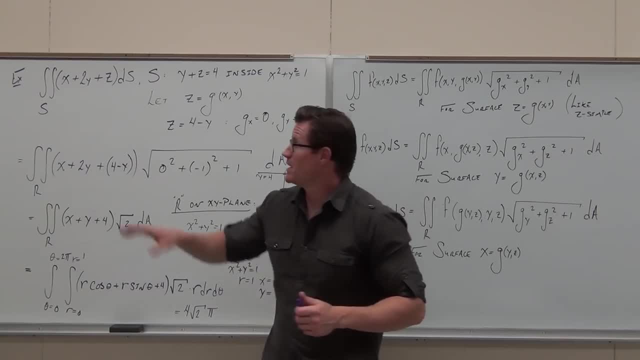 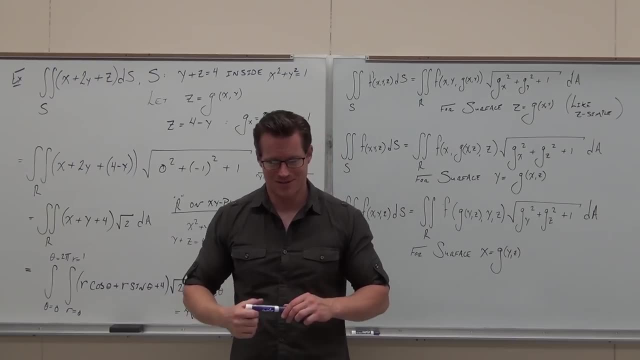 That's what that is. Is it making sense? Again, if that was 1, then yes, that would have been surface area of that plate. Should I be able to answer that one? Okay, That was the only example that I have for just basic surface integrals. 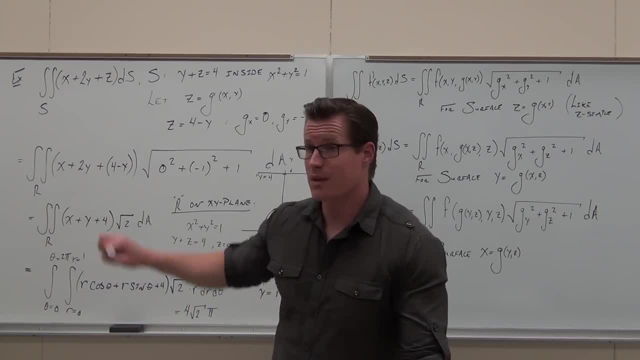 because we're going to move on a little bit. What I want to talk about right now we're going to get back to it. okay, We will, I promise, But I want to show you a different way. But in order to show you this different way, 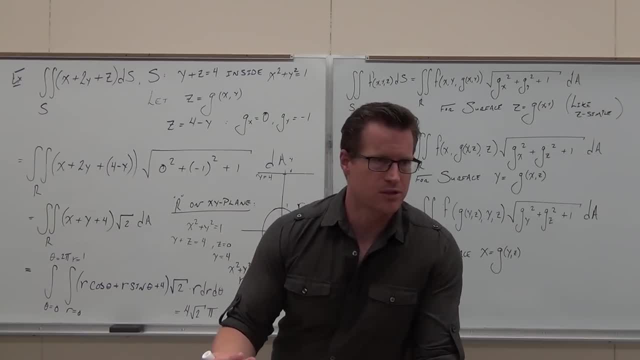 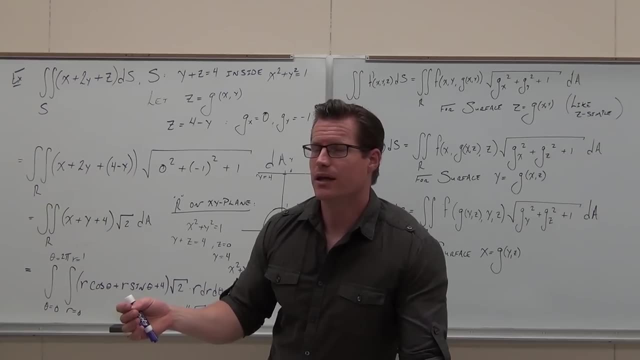 I have to show you how to parameterize surfaces. What that means is treat a surface like a vector function. I got to show you how to do that. It's not necessarily, it can be super hard, But I'm going to show you two techniques on how to do it that are very, very fast. 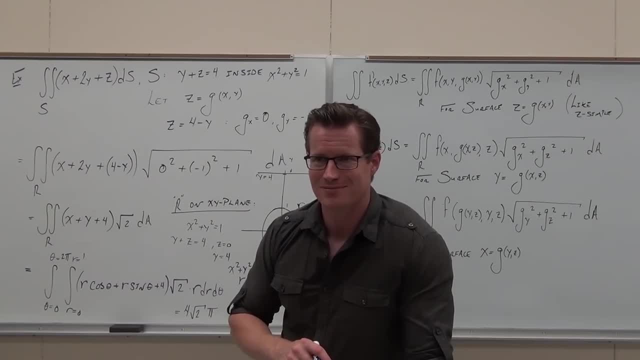 Are you guys ready for it? You're not ready for it? Well, get ready for it. So, are you okay? on surface integrals, for right now, I'm going to leave this on the board the entire time, because I'm going to have a lot of time. 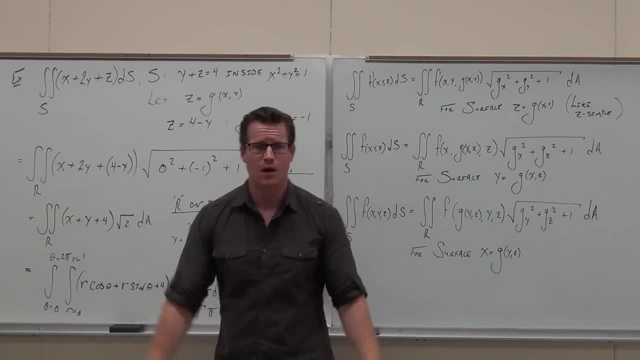 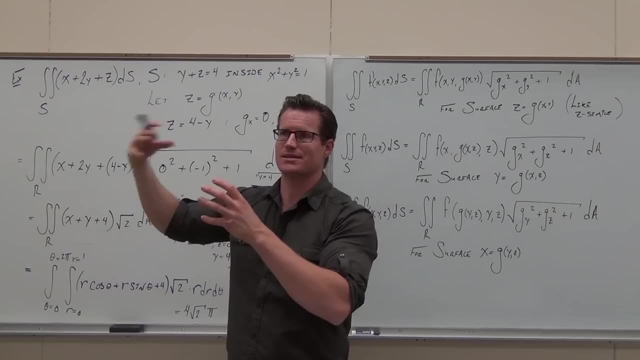 I'm going to come back to it. I want to make the connection with what we're going to be doing, what we've already done, that we don't lose this. This is not like seven different concepts, okay, It's the same kind of the same concept over and over again. 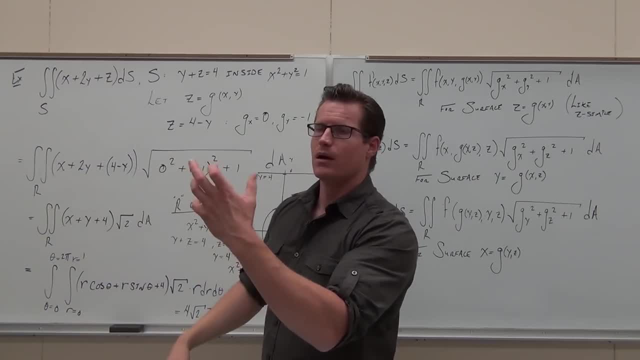 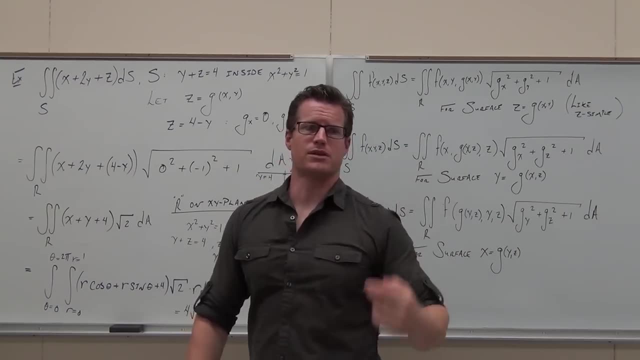 until we get to divergence theorem. And then we start talking about well surface integrals through vector fields, And then we start talking about divergence theorem. And then we start talking about curves through three-dimensional vector fields, And that's Stokes theorem. 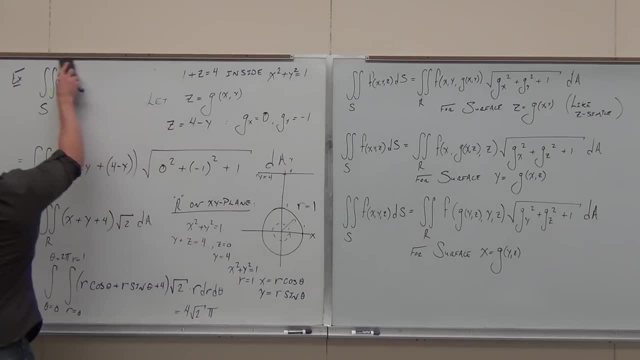 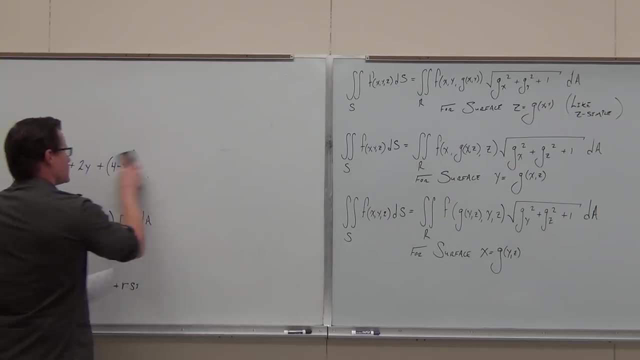 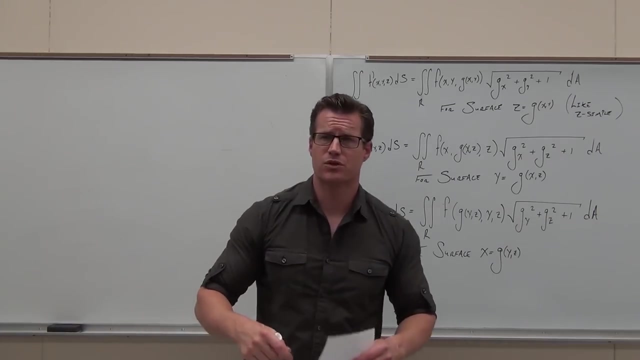 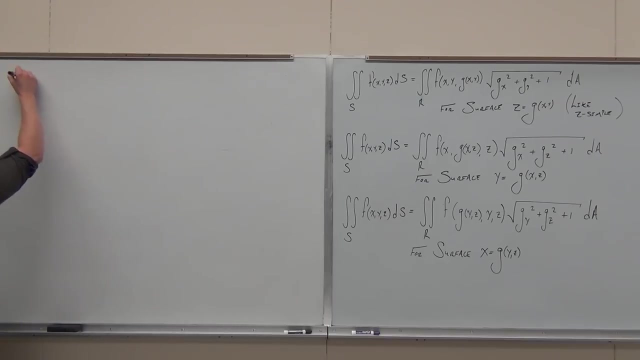 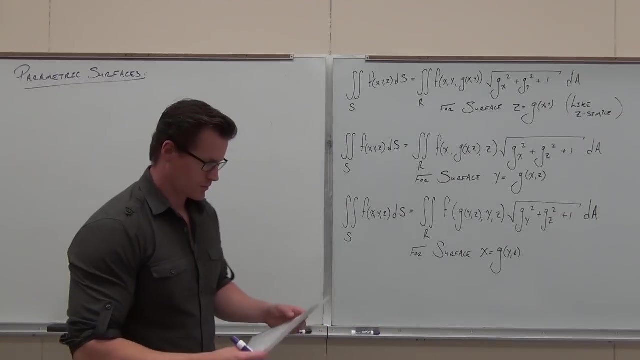 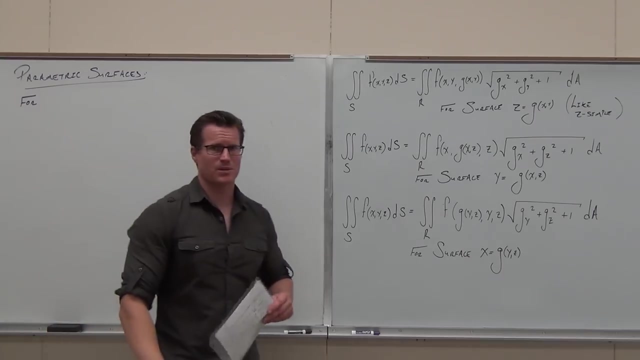 We start talking about that, okay, So you can kind of title this little subsection, just title it parametric surfaces. We're going to do quick examples here to get the concept. So here we go. This is all going to look like gobbledygook at first. 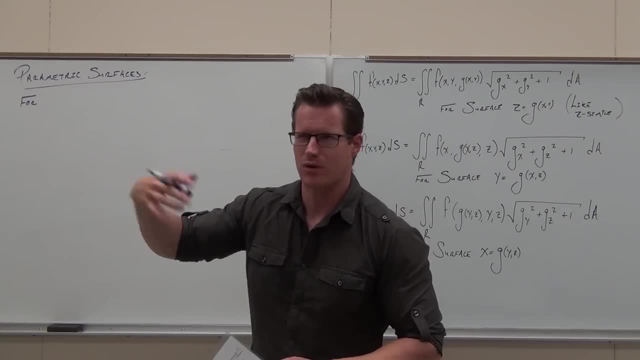 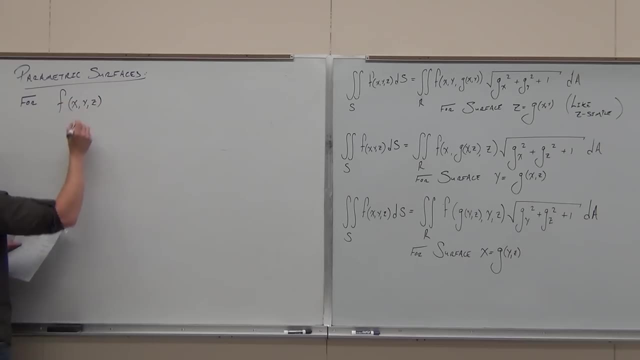 I'm going to make it make sense with a couple of examples. Just write this down. This is like the background behind how you do parametric surfaces. So if you've got this function of X and Y and Z and you can redefine X in terms of a function, 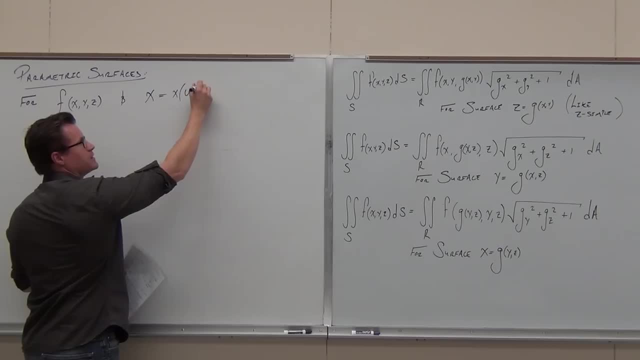 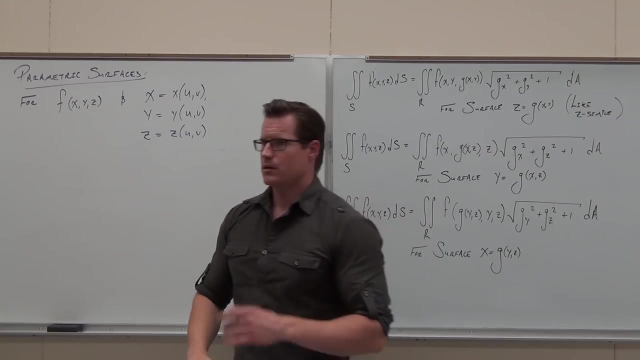 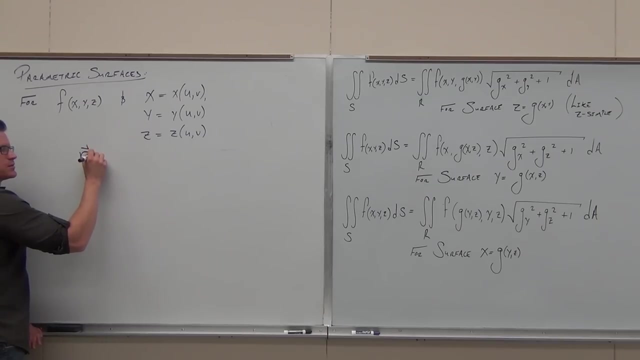 where X is defined in U's and V's, and Y, where Y can be a function defined in U's and V's, and Z, where Z is a function in terms of U's and V's. If you can do that and if vector functions are always the X thing, 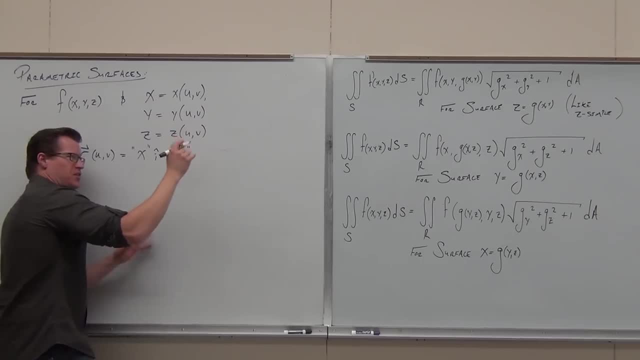 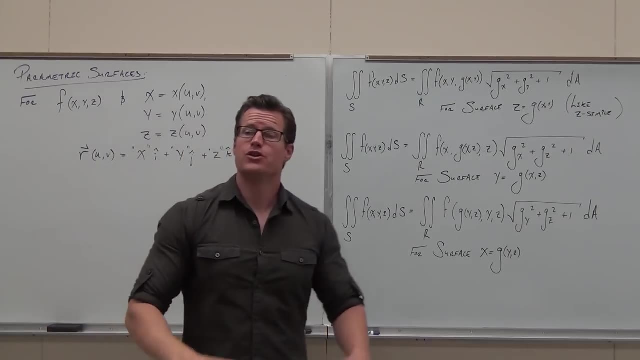 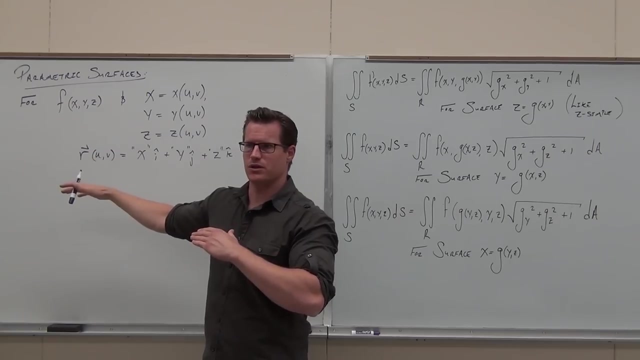 and I, plus the Y thing, J, plus the Z component, K, then you can redefine a surface in terms of a vector function. Why, Why would you want to do that? Well, let's look at it. Verify that this would have three variables. 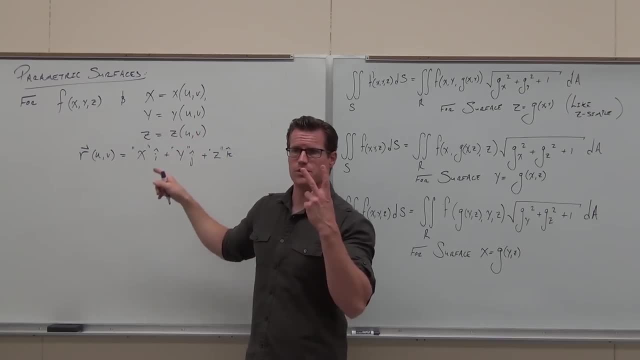 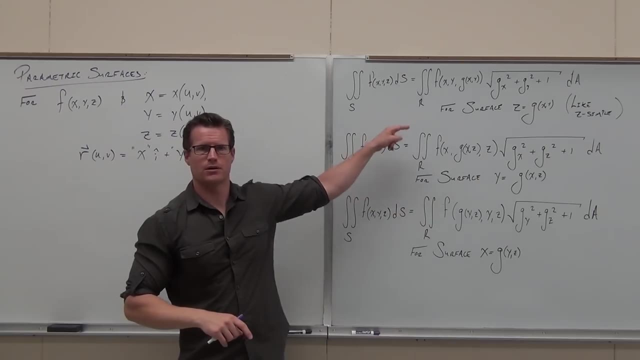 Verify that this has essentially two variables. You eliminate a variable. Now you listen carefully right now, Do you recognize that that is exactly what we've done over here? It's a different way to do basically the same thing, just a slightly different way. 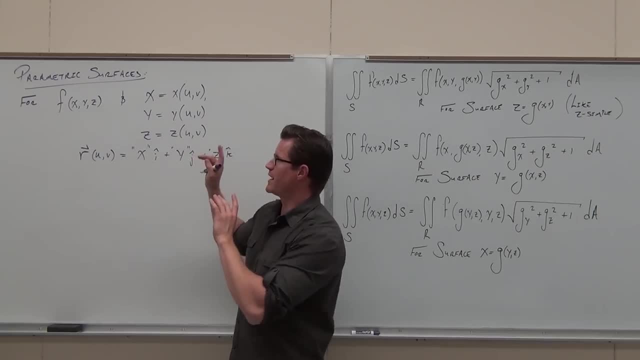 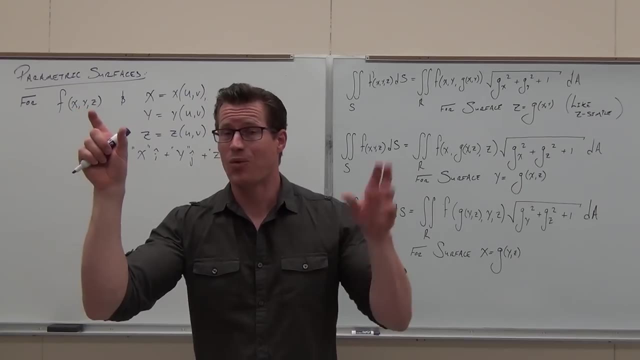 So we're going to deal with this one. but essentially, when you find parametric anything, it eliminates a variable. Remember that back from like Calc 2, when you were like, hey, here's X's and Y's, and you define them in terms of T: X's and Y's both change to T's. 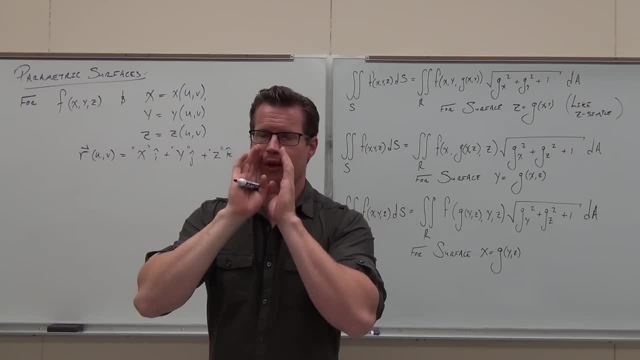 Now we're saying: well, we've got X's, Y's and Z's, Let's define them in U's and V's. We've already done that. 14.8 transformations, Remember that Kind of? do that sort of thing already. 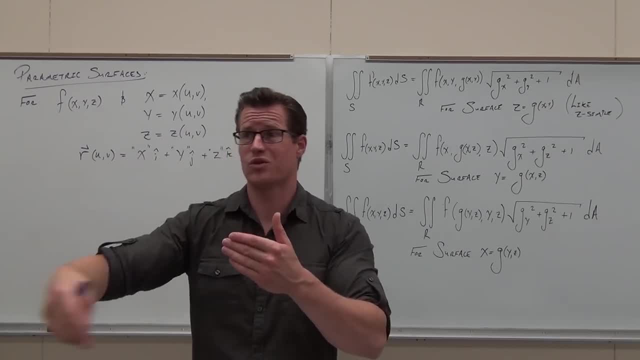 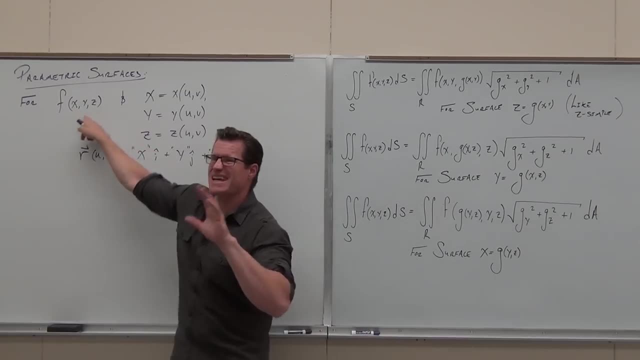 This is just kind of further, just a little bit further. and those were surfaces. We're just kind of redefining the same thing. It's just hey, if you could define something that has X's and Y's and Z's. 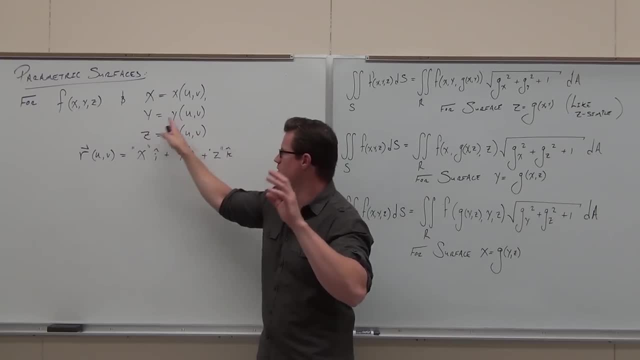 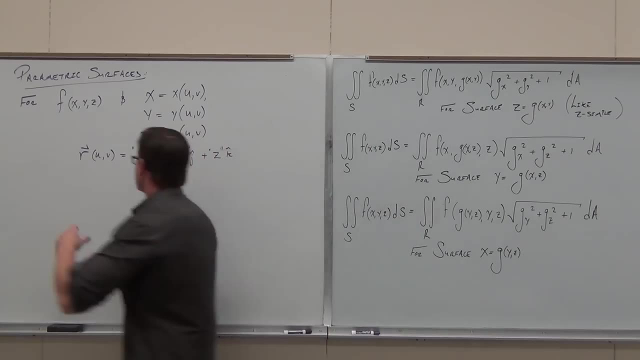 where X would be U's and V's and Y's would be U's and V's and Z's would be U's and V's, and you know that vector functions are always the X component I, the Y component J, the Z component K. then what we can do is we can define. 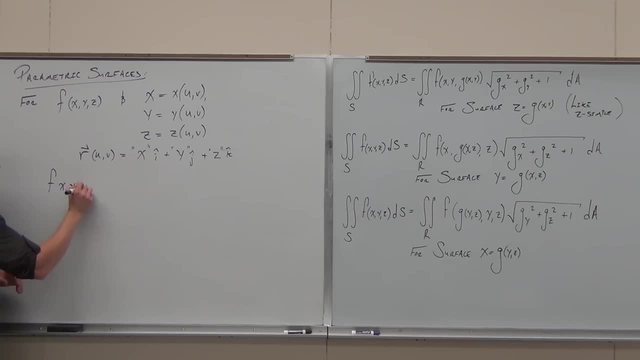 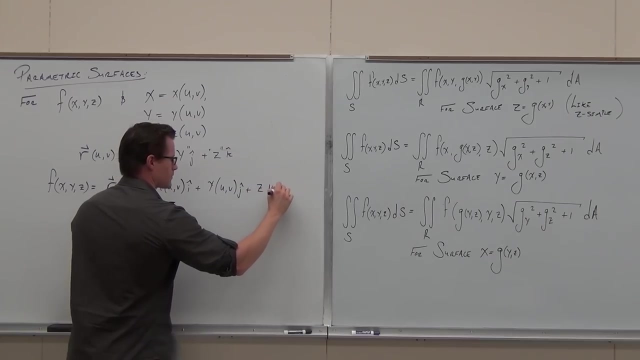 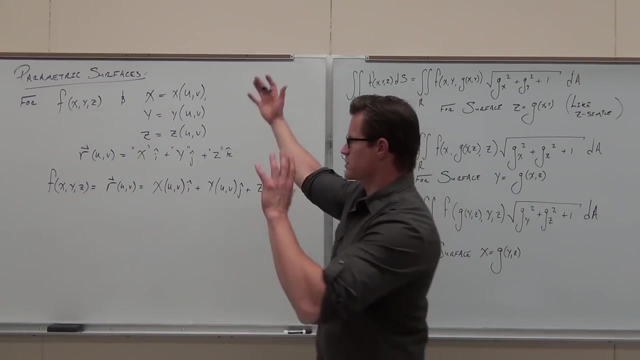 is, we can redefine the surface itself as the vector function and it would give us the same thing graphically. Here's what I want you to get out of this. all this notation It's saying I'm essentially just going to be changing X component into something with U's. 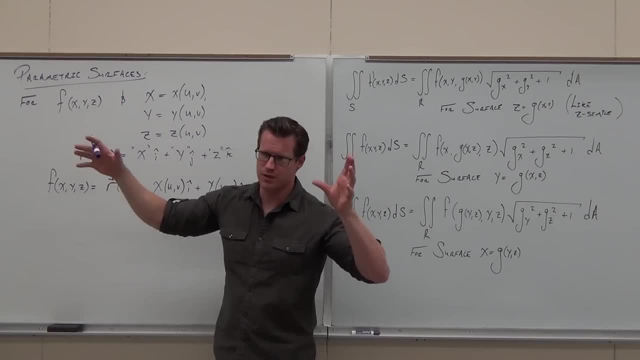 and V's, Y into something with U's and V's and Z into something with U's and V's. Therefore, I can define a vector function in terms of U's and V's, U's and V's, U's and V's. 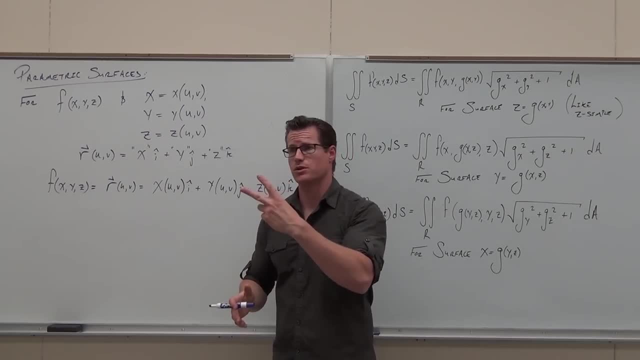 Does that make sense? Three variables change two, two variables, and that makes things nice for us. It also makes the formulas even nicer than the other ones. It makes the formulas even nicer than the other ones Because these don't look very nice. 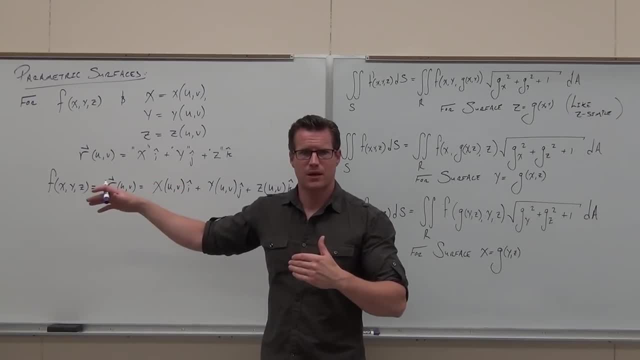 I'll show you how to do that. Are you guys okay with the notation so far? Now I'm going to give you two examples on how to do this. The first one's very easy. It's supposed to be very easy. I just want to get your head wrapped around it. 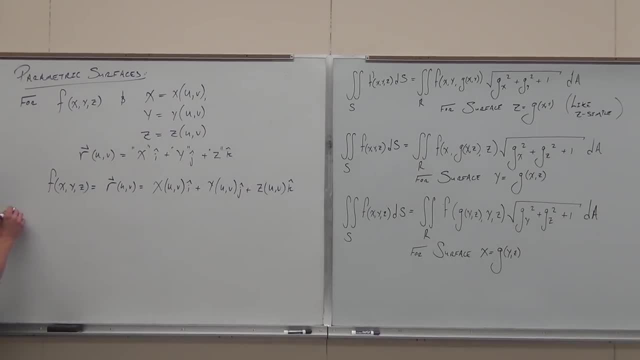 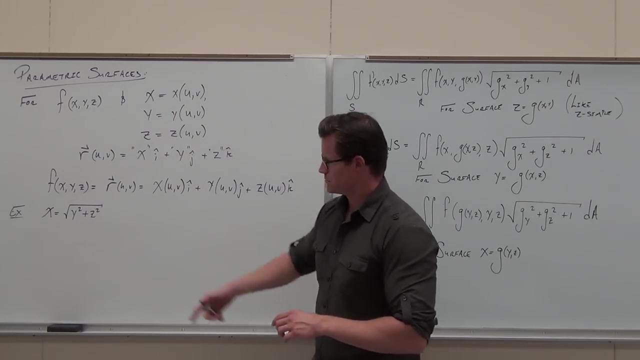 So let's suppose this. Hey, let's take a look at it, What is it? Well, how about this Surface? yes or no? What do you think? Yes, Yes, How many variables? Three Or two? 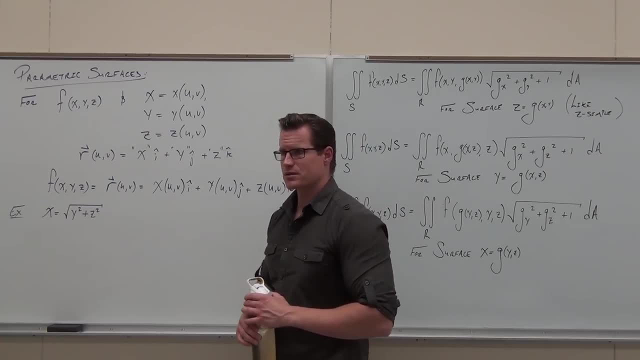 Three variables, Three, Three total variables. X is dependent on both Y and Z. This is half a cone. If you didn't know, that's half a cone Upper, half cone along the X axis. Remember cones at all Square both sides. 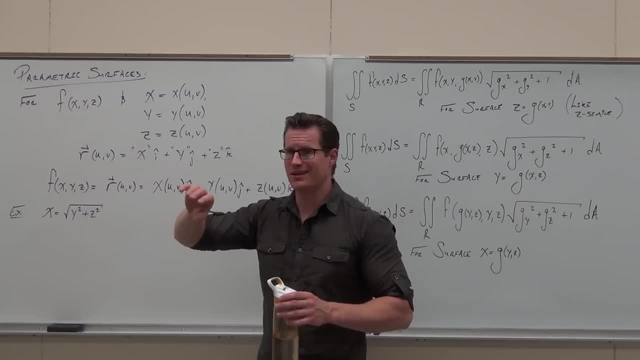 You get X squared equals Y squared plus Z squared. It means, if you solved it, you get zero and you get one negative. It's a long way. It's a long way along that axis, but this is an upper half cone because you've got a square root. 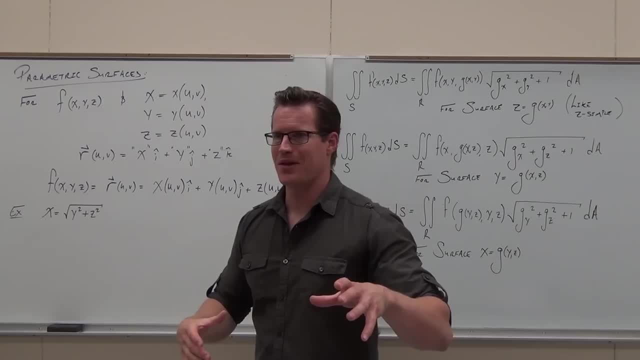 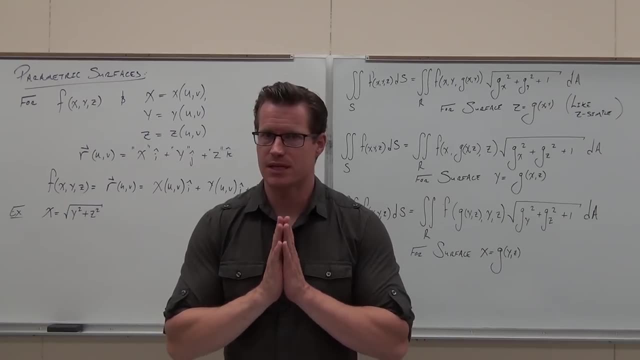 You're not taking the bottom half of that. It's an upper half cone and not very good on that one. So here's how you. there's two cases. One case is way easier. This is the easier case. Please listen carefully because it's going. 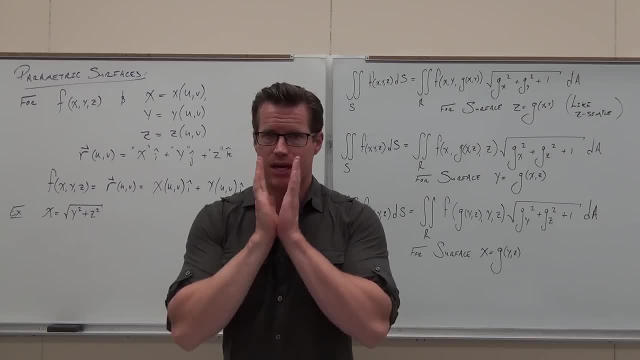 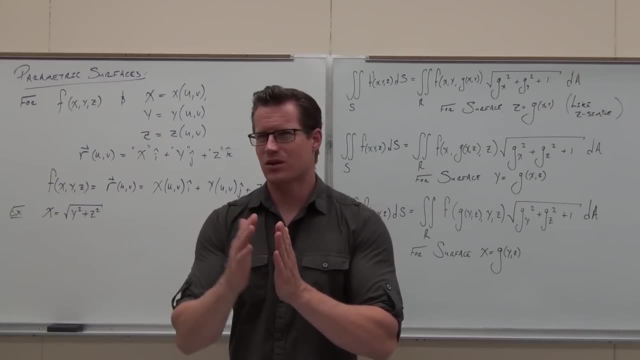 to save you a freaking ton of time. Okay, A ton of time. If you have a surface where it's already solved for one variable, Is this already solved for one variable? Yes, Okay, Then it's already depending on only two variables. 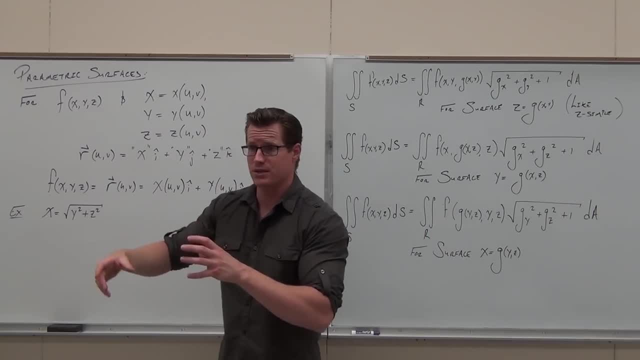 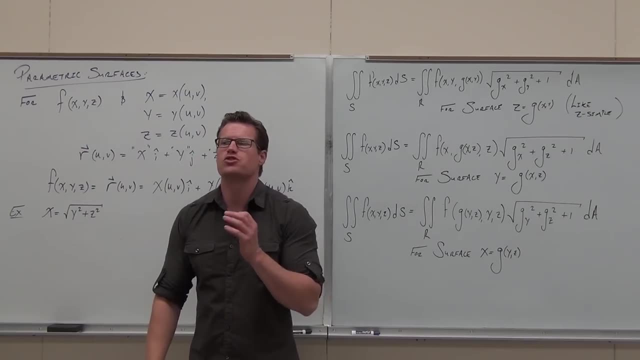 It's already there. Then what you do to parameterize this, Call this U, call this V and it automatically takes care of X. It's the easiest, it's almost it's a trivial. it's a trivial parameterization, but it lets you put this. 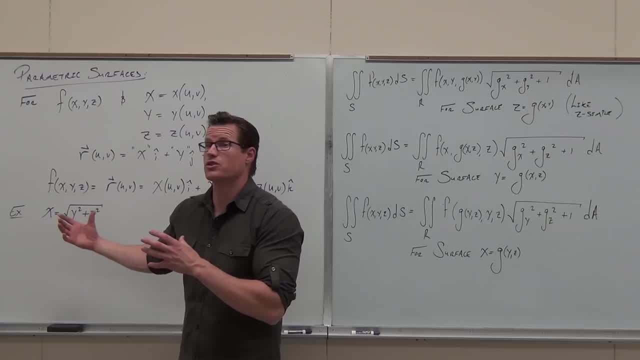 in vector function notation. Does that make sense? You can honestly do it right from here. You can literally do it with X's, Y's and Z's, but if we want to use U's and V's, here it is. 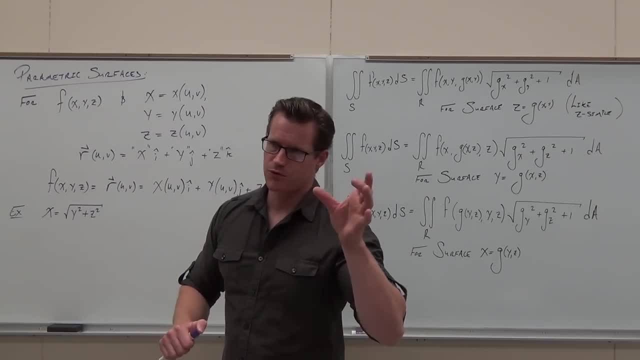 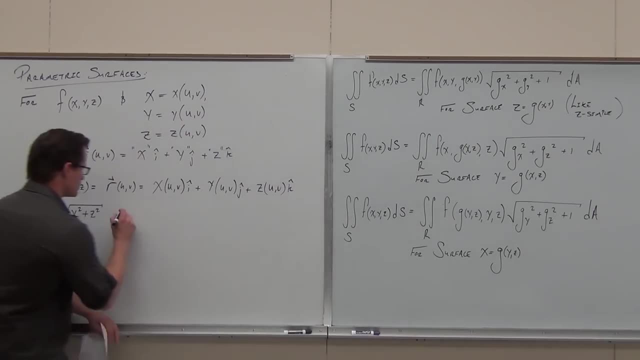 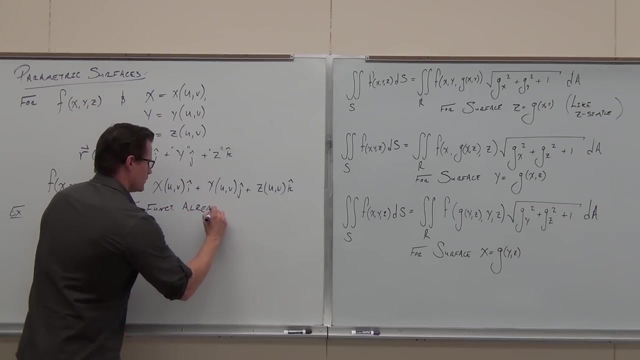 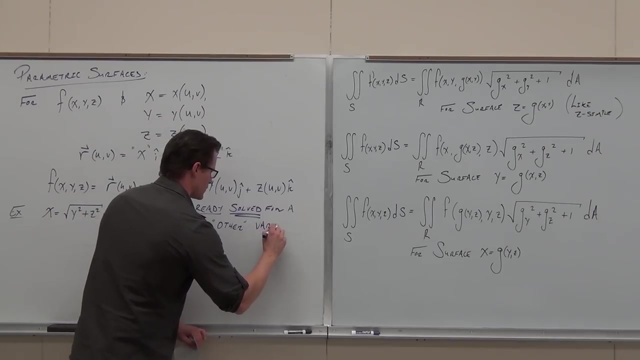 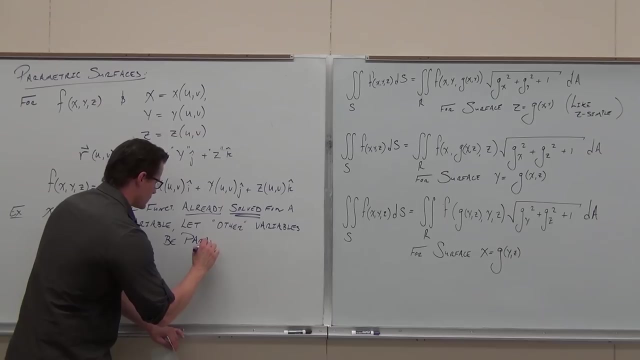 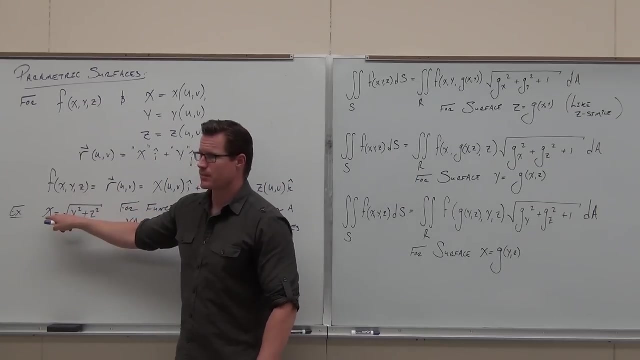 Write this down: For functions already solved for a variable, let the other variables be parameters. It's going to make sense if we do our example. If it's already solved for X, then the other variables are Y and Z. Those variables become your parameters. 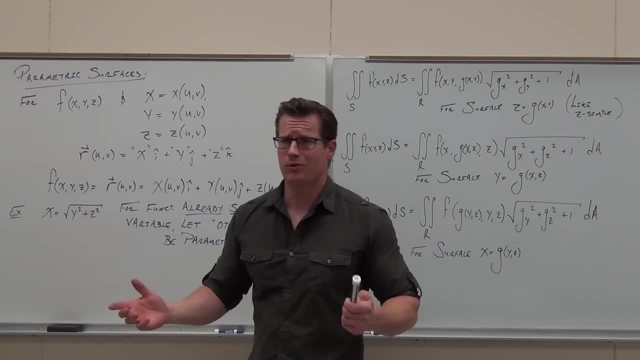 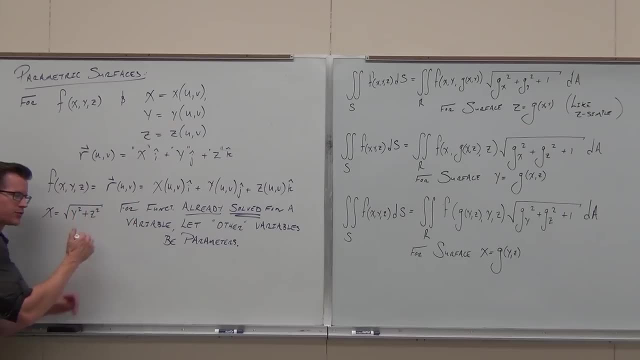 It doesn't matter which one, No, not really. Pick one to be U, pick one to be V. So what do you do? Let's say, hey, X is solved for Y and Z. My other variables, the ones that are not solved for, are Y and Z. 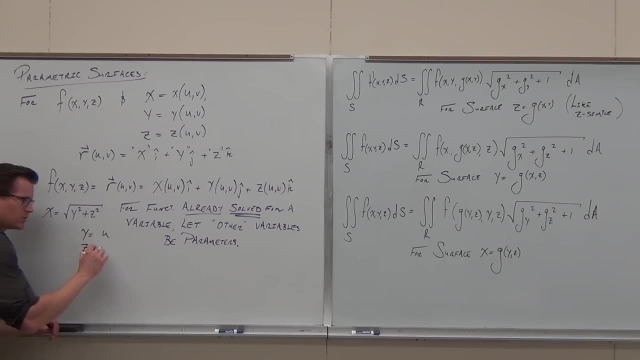 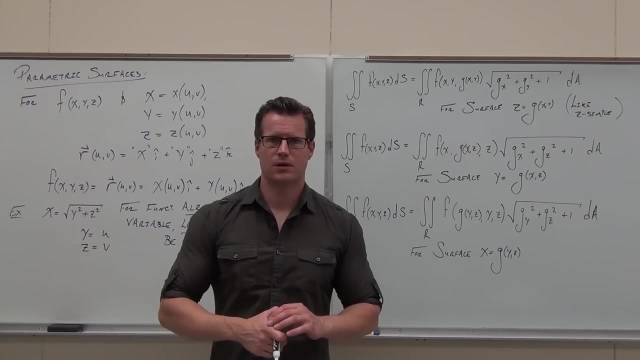 Let's let Y equal U. Let's let Z equal V. Okay, I don't know if you're okay with that. Yes, no, yes, Okay, then what's X? X doesn't really change. That's why it's trivial. 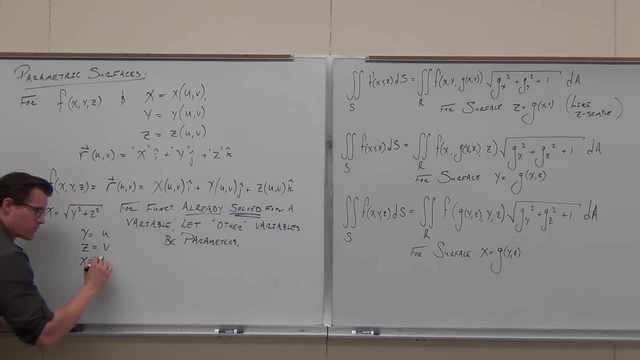 X doesn't really change, Then X is just going to be the square root of U squared plus V squared. If Y is U and V and Z is V, then X is just U squared plus V squared. You're not doing any. that's why it's a trivial substitution. 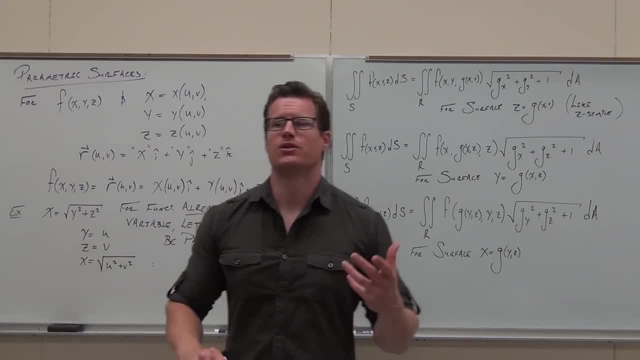 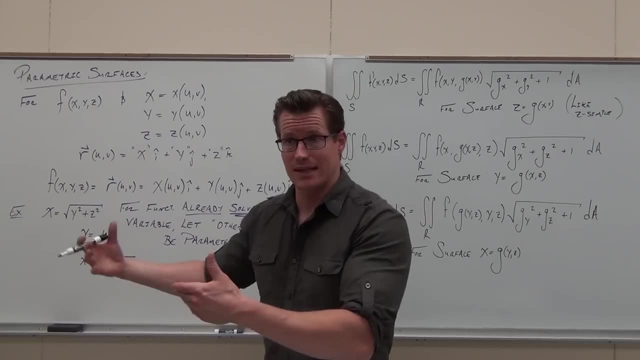 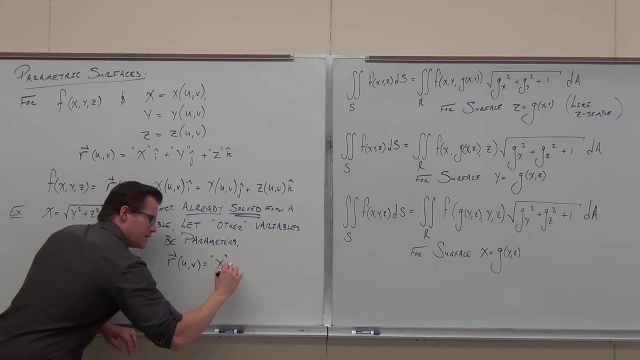 But what it lets you do is easily redefine a vector function into variables. Are you guys okay with the X, the Y and the Z? Okay, so let's continue. Every vector function ever does the X thing, I plus the Y thing, component J plus the Z component. 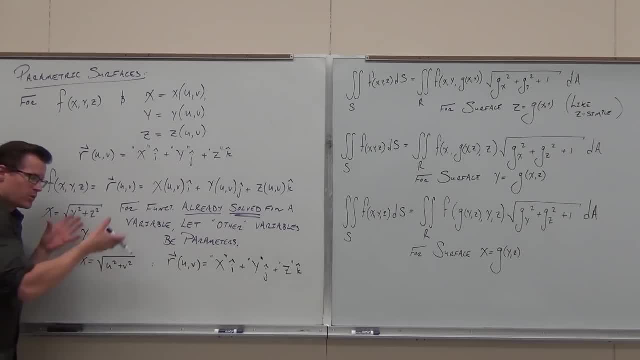 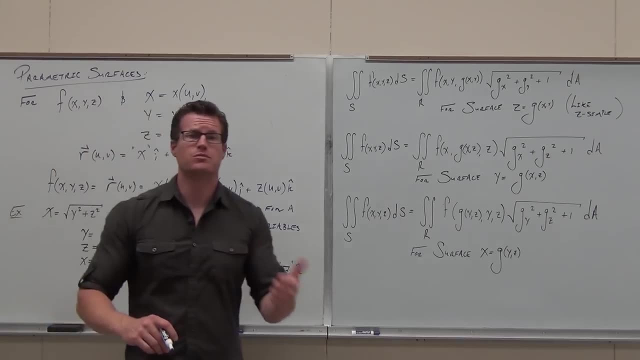 okay, and since we already have that- yeah, it's trivial, but we've already redefined it- Now we can easily define our surface parametrically, and that's exactly what this means to do: Define as a vector function. those are parameters. 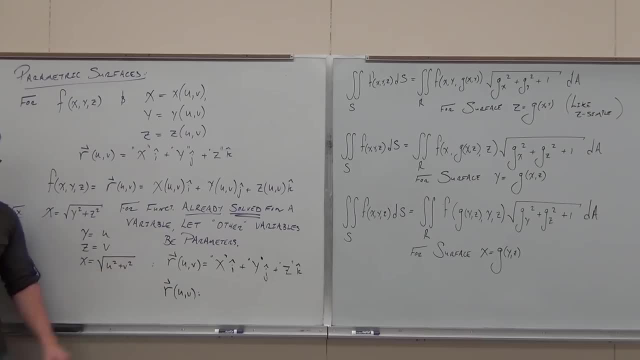 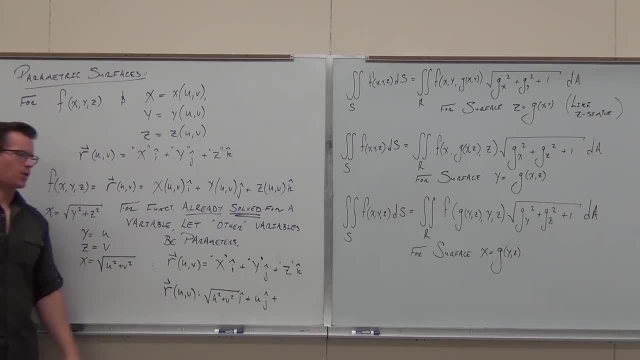 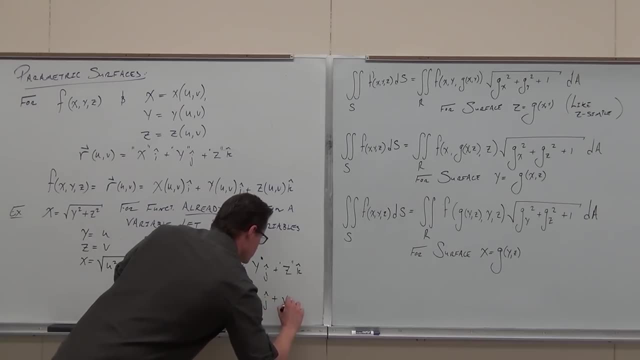 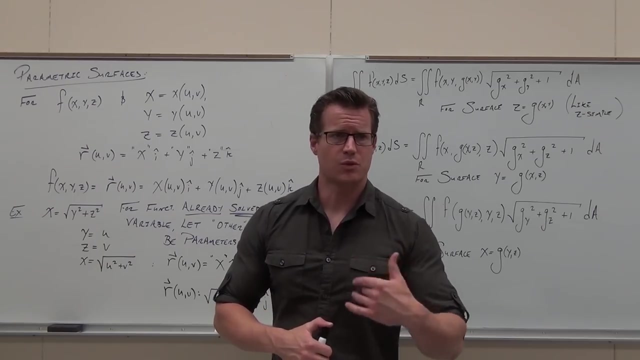 U. What would the Z part be? I don't know if that makes sense to you, But by the way, in case you didn't see it, I keep using this word: trivial. Trivial means it's really not doing a whole lot for you. 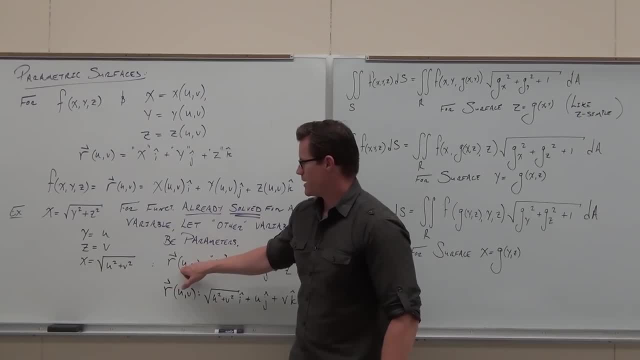 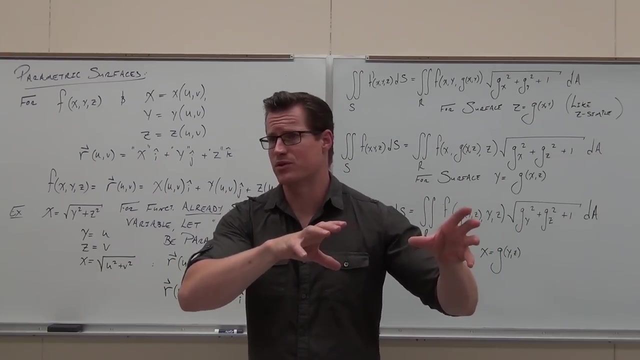 Here's why, If you just called this X or- sorry- Y and Z, you could have Y and Z and Y and Z. We typically change variables just so you're showing that you have a different parameters, different parameters, different parameterization. but 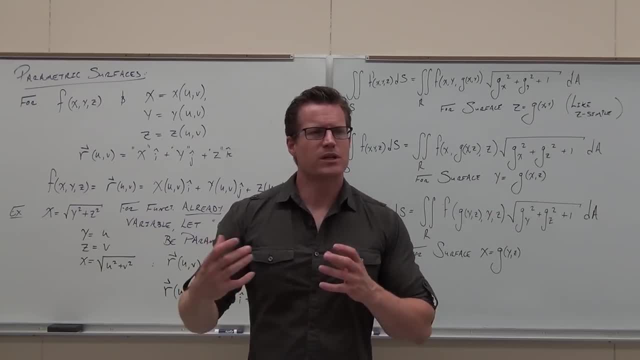 and so it fits our notation a little bit better later, honestly, but we're not really doing much. So this is a really do you guys see that it's a really easy case? It's a really easy case if you're solved for one variable. 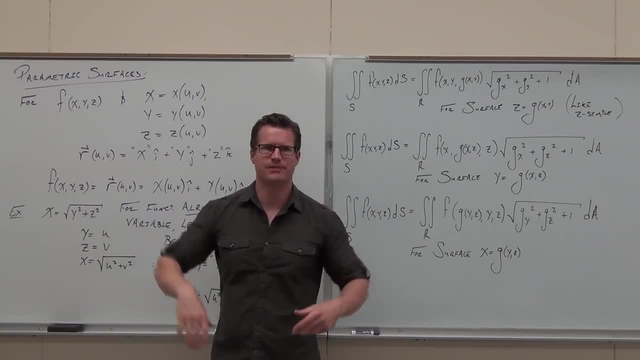 the other two variables become u and v respectively, and you just plug it in. That's all that's happening, so it makes for a given value. Now, a little more difficult is when they're not solved, for We're going to do one of those things and then we're going. 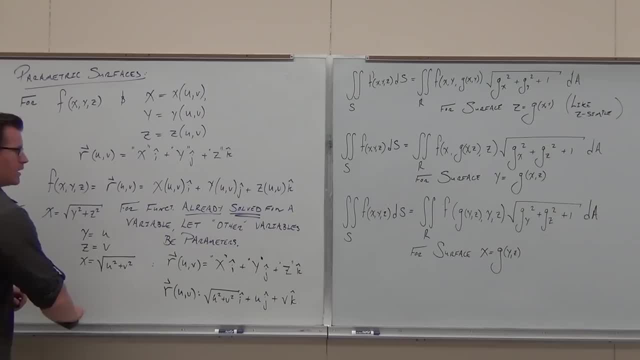 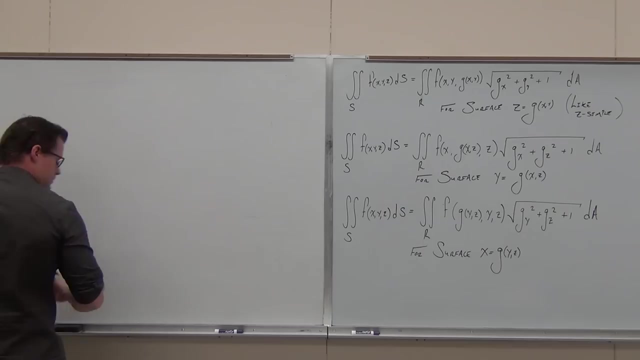 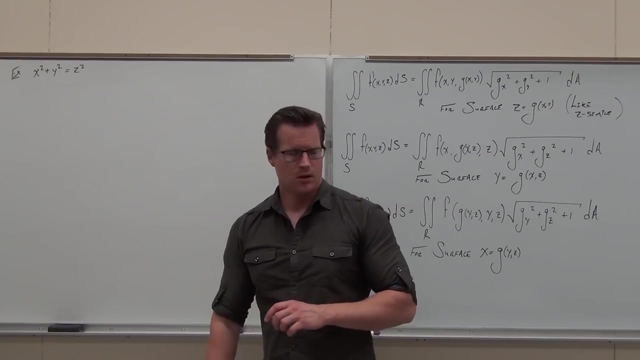 to work with it. do some examples with this. So are there any questions on this right now? Okay, So let's give this one a go. Ladies and gentlemen, is this solved for one variable? Yes, no, No, clearly not. 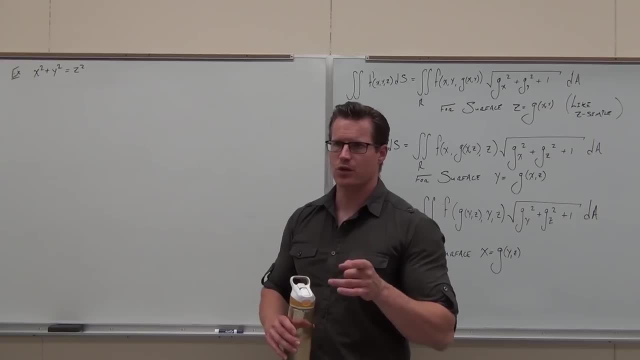 You got x squared, y squared, z squared. Here's my first advice to you: Don't Don't solve it for one variable, because as soon as you start taking square roots, you lose half of this cone. This is another cone, but it's a full cone. 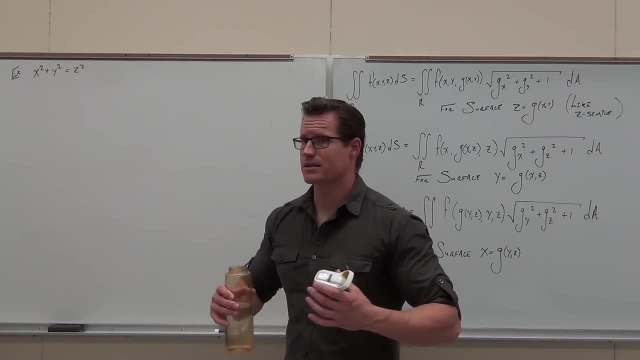 Do you guys see that It's a full cone along the z axis actually? and if we took a look at the z axis, we'd see that it's a full cone. So it's a full cone along the z axis actually, and if we took a look at the z axis and if we took a look at the z axis, we'd see that it's a full cone. 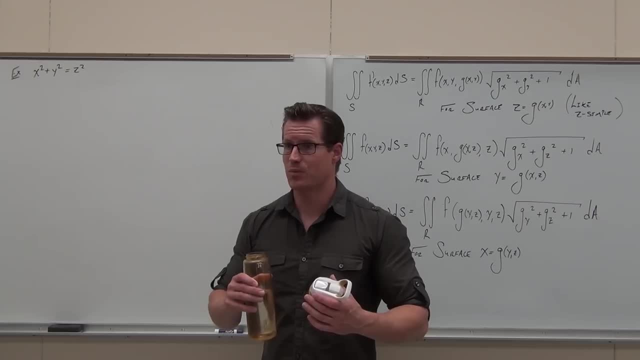 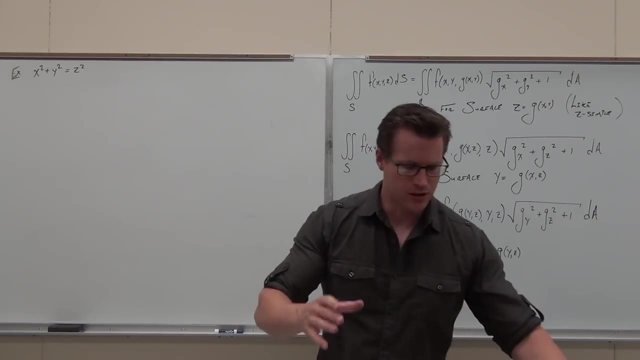 So if we took a square root, we'd be losing half the cone. Did you guys get it? That'd be a problem and I want to do that. So when you don't have a function that's solved for a variable, you're going to be using a non-trivial parameterization. 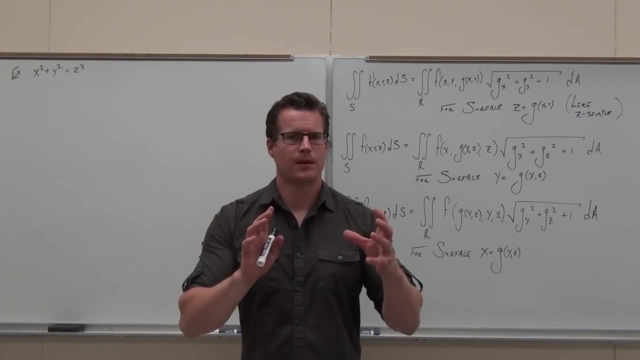 How to pick it. Start with one side, Parameterize one side that looks like it's easy to parameterize and it's awful wording, But start with a side that has the majority of variables, all but one variable. If you have to move something around, maybe move something around. 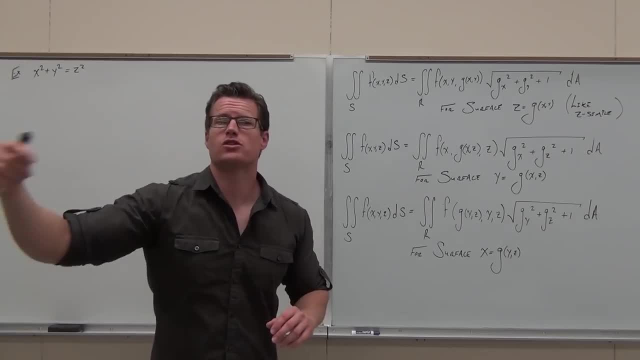 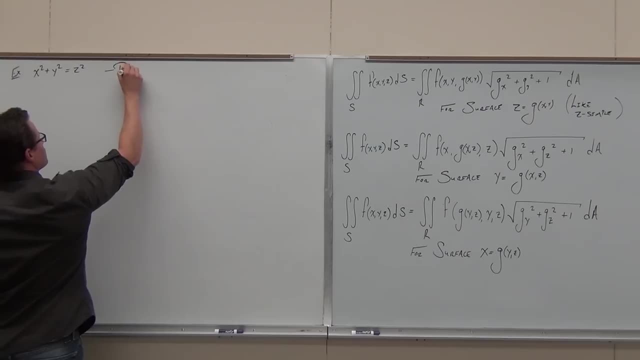 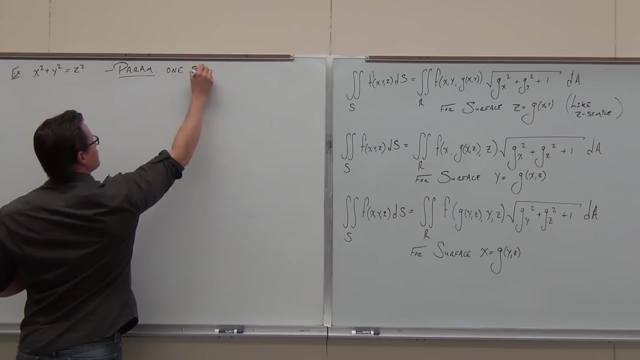 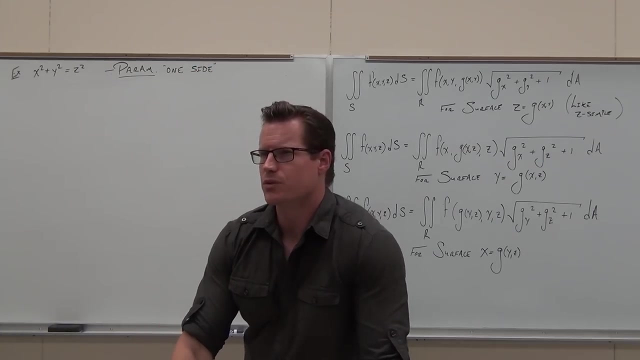 I'd start on this side. So when you're not solved for a variable, parameterize one side and use it for the other side. What side do you think that you would want to start with here? Would you want to start with the z squared side? 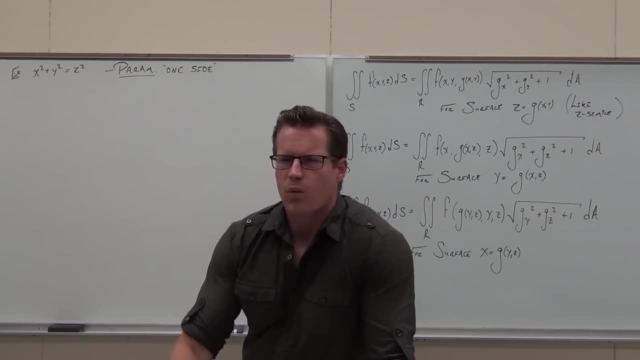 or the x squared plus y squared, Both sides. Why? Why would you want to start with the x squared plus y squared? What's that look like to you? It looks like it's something that you could call something else. That's why we start with one side. 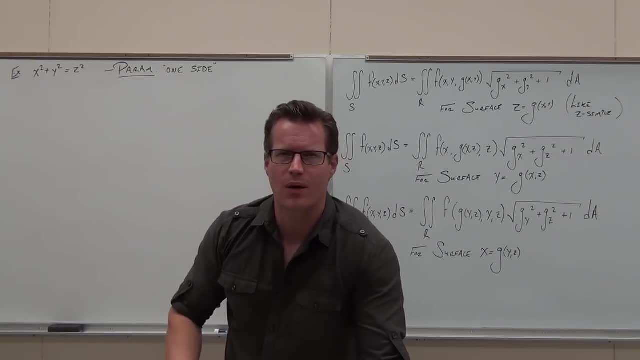 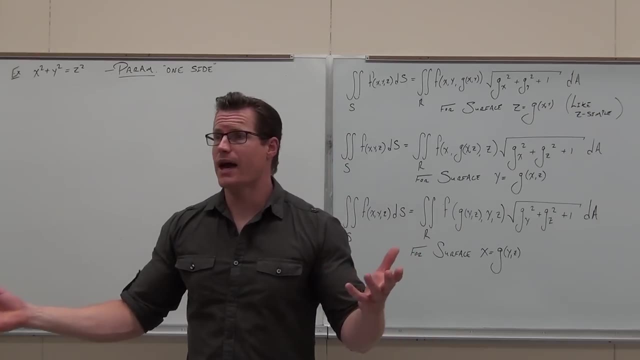 Something that you could call something else. It rings a bell in your memory. You go: hey, x squared plus y squared. Have we ever defined x squared plus y squared before? What do we typically call that? We can do things like that. 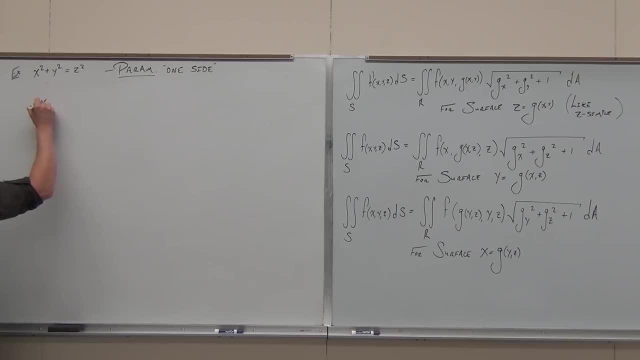 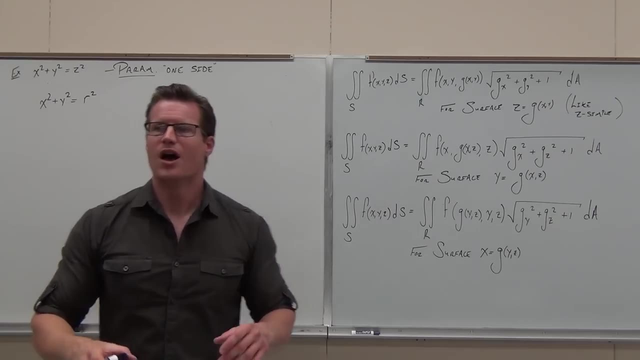 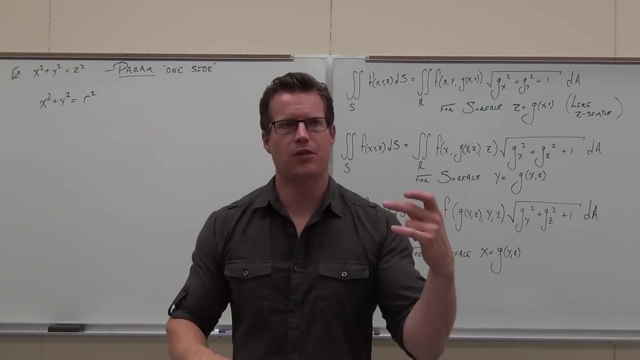 So let's call this, Let's let x squared plus y squared equal Well, r squared. But I told you something about 15 minutes ago. I said, as soon as you do, that you're picking some very specific things for x and y. 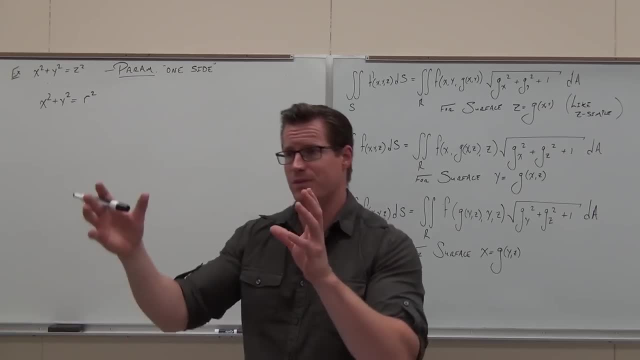 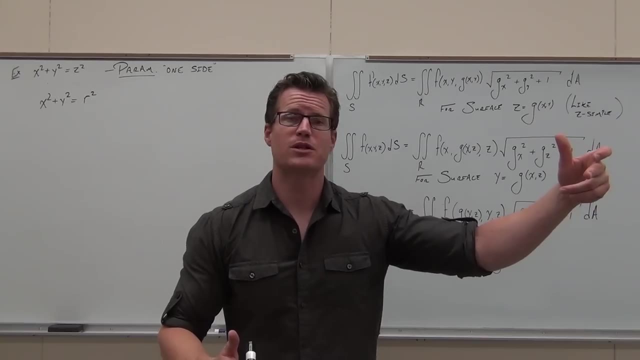 Do you remember that You can pick any two variables? you want to be x squared and y to be r squared, But we specifically chose x and y to be x squared plus y squared equal to r squared. Does that make sense? It means x and y have to be two very specific things. 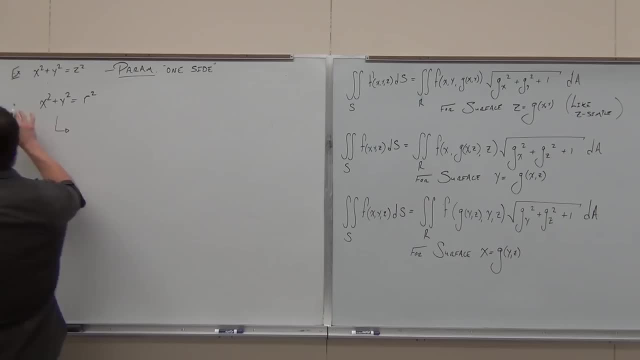 As soon as you do this, as soon as you make that connection on one side, you have to label what they become. So what are you going to call them? What are you going to call x, R, cosine, theta, Exactly, And what are you going to call y? 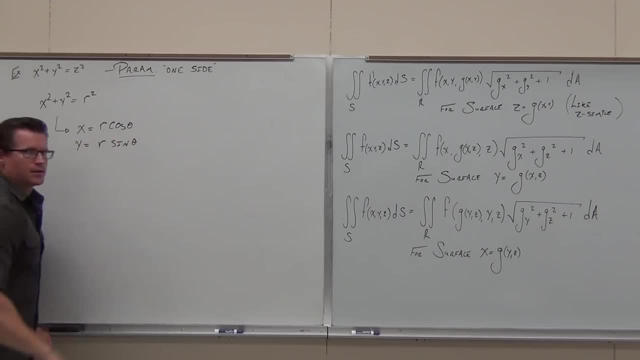 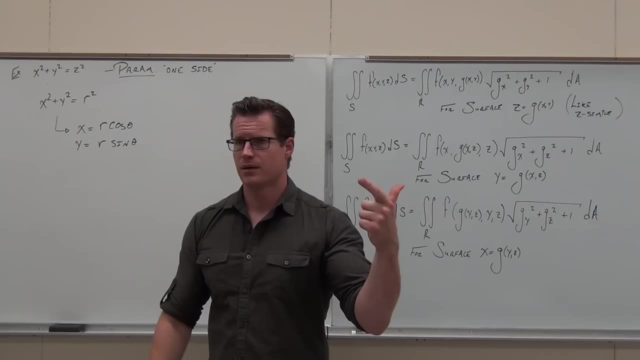 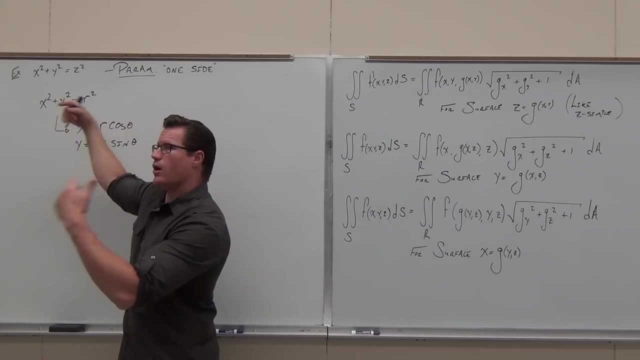 R sine theta. Do you realize that you just parameterized x and y in terms of two variables, r and theta. Are you guys okay with that one? Now let's work with this. If we called this r squared, then that also means that r squared. 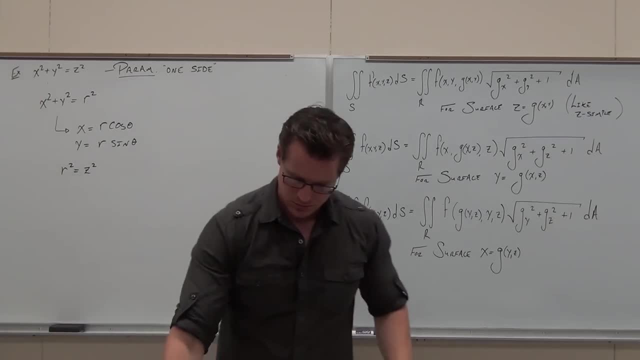 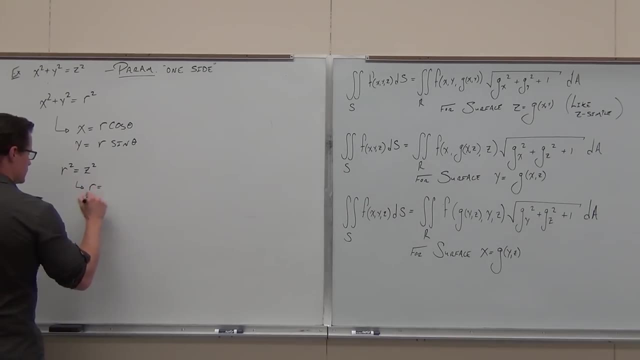 equals z squared, or r equals z. I'll write that away- Z equals r. So I have- hey, look at that, I've got x and y defined in terms of two variables, z defined in terms of one of those two variables. 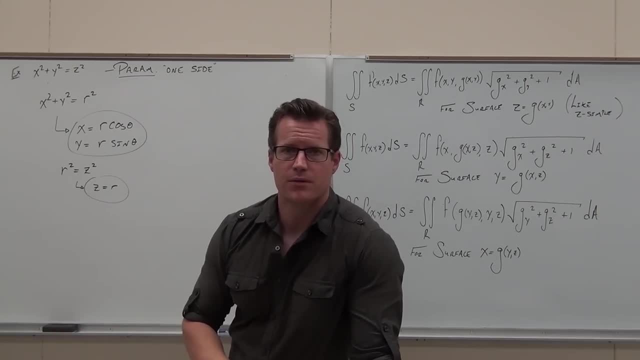 I've literally redefined x and y. We have literally redefined x and y and z. That's parametric. That's how we would redefine x and y. We would define the surface parametrically, at least the start of it. 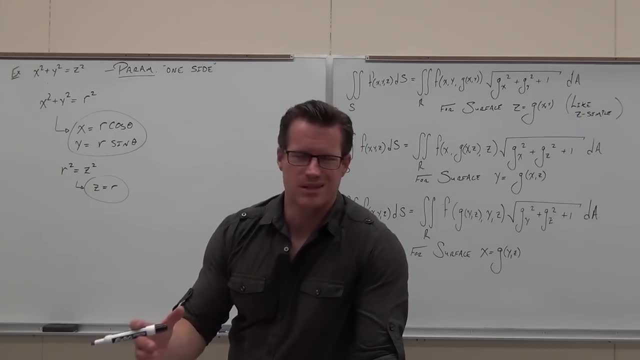 Are you guys okay with the idea behind it? So if it's solved for a variable, it's pretty easy. If it's not, pick one side and start doing things like defining x squared plus y squared equals r squared. if you can Work with that, 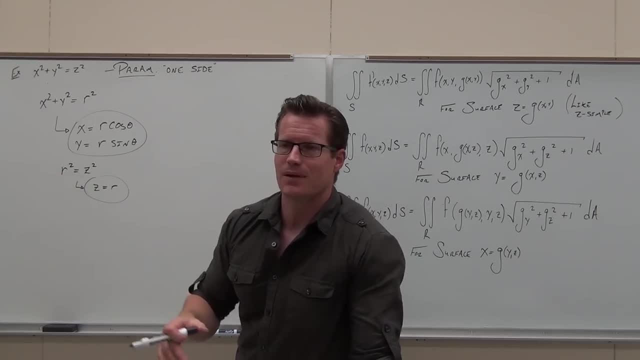 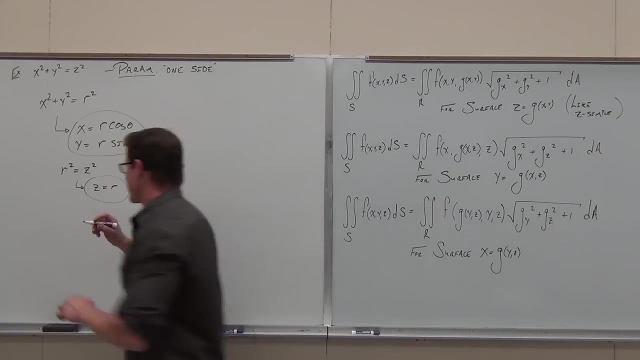 As soon as you do it, redefine those variables. Now I don't even have your attention. I should have your attention because it's important. There's two things that are going to go on As soon as you have this and you know this right. 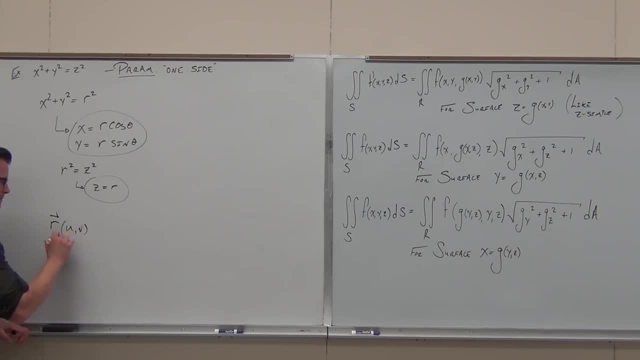 You know that we're trying to get down to this. The x times z. That's the first one, That's the second one, That's the third one, The x thing i, the y thing j and the z thing k. 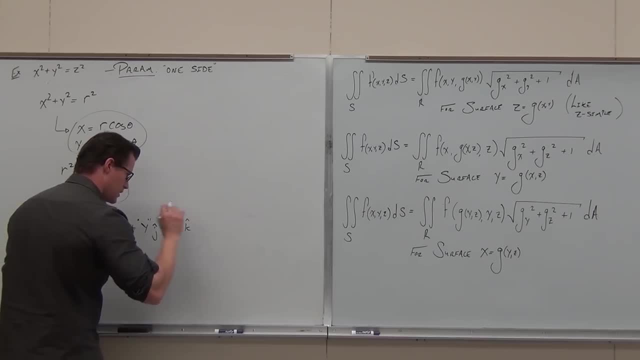 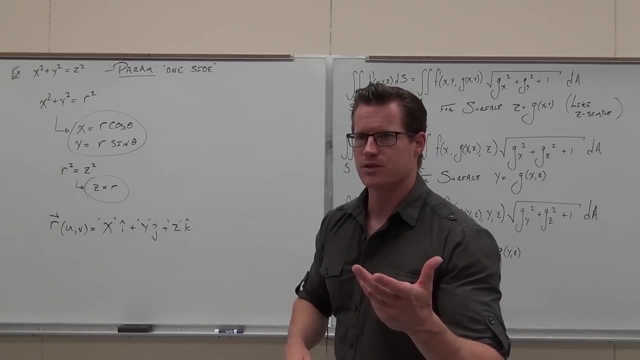 Oops, that's not a k, Not okay k. We're trying to get down to that. Now there's two issues we're going to have. Do you see one of the issues? You don't see one of the issues. 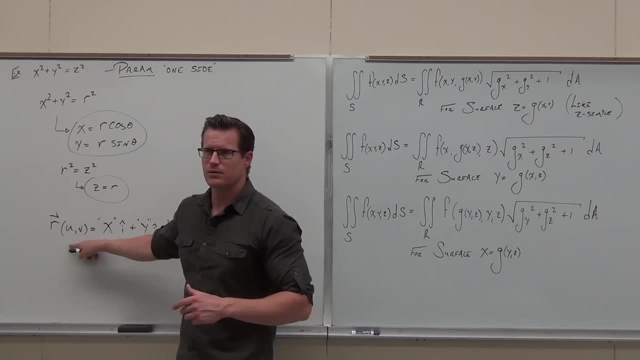 What variables do I want? What variables do I have? Could you just define this as r and theta? Yes, but it looks a little weird because we're going to have a lot of problems. We're going to have a lot of r's floating around, okay, 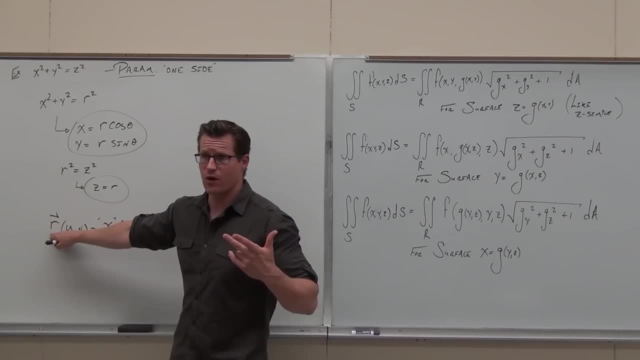 So I really don't want to use a vector function of r and then have a variable of r inside of it. Does that make sense? That looks a little funky. Can you do it? Sure, you can do it, It doesn't matter. 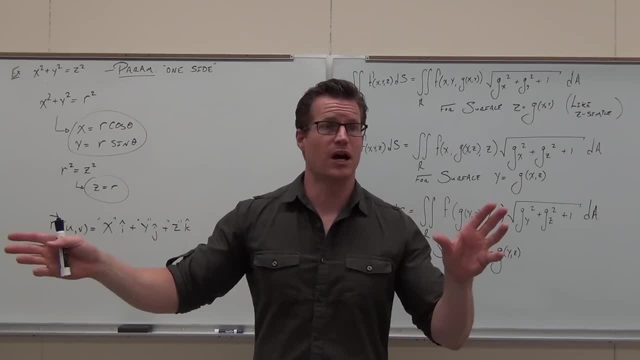 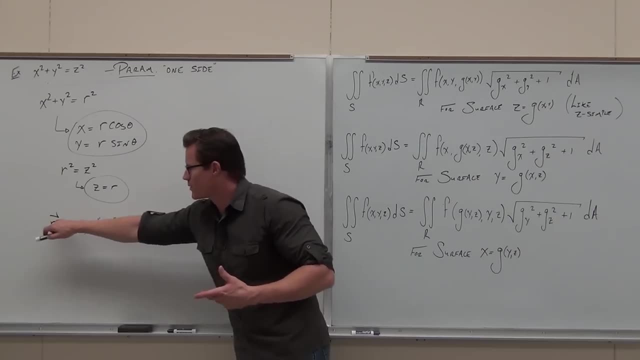 u and v are dummy variables. They don't even matter. Just pick any two variables and you've got rid of one variable at least. So r's and theta's fine, but I wouldn't pick them because I don't want to run into confusion. 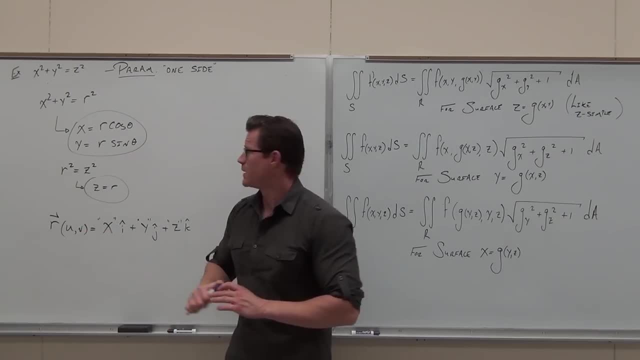 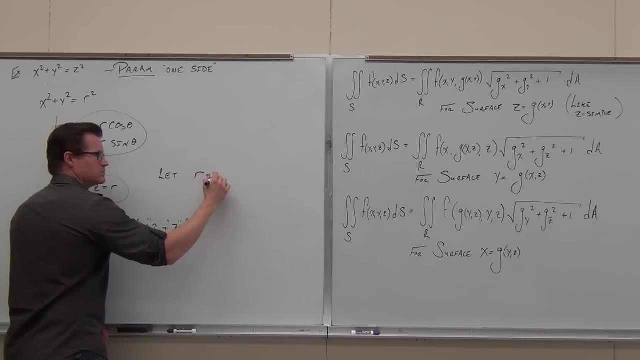 Now should there be confusion? Not really, but you could do something really easy If you just say: well, let's say: let's let r equal u and let's let theta equal v, then we just redefine this thing. 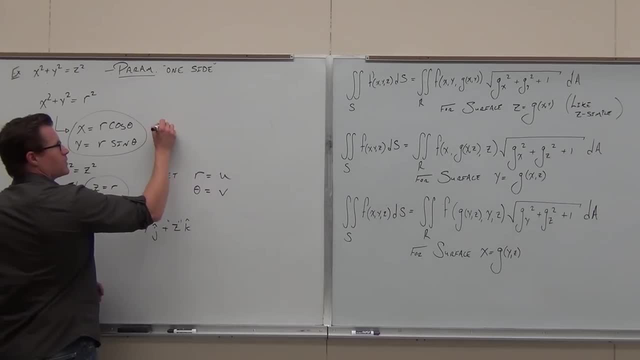 Does that make sense to you? So we go, okay. well then, x is going to be u cosine v, Y is going to be u sine v and z is just going to be u. Okay, And now that matches our notation a little bit better. 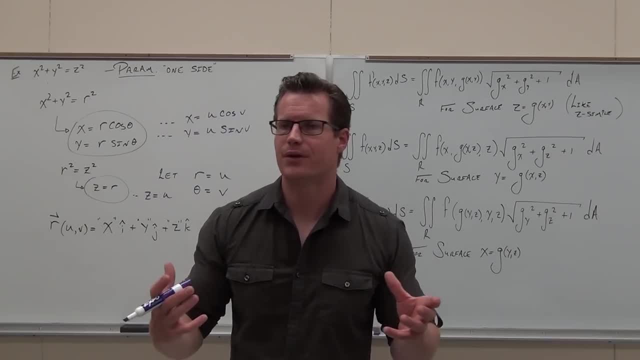 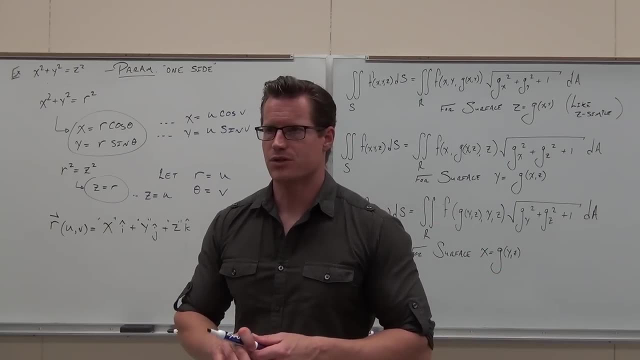 again, does it matter? No, it doesn't really matter because they're dummy variables, but they're going to fit in your formulas a lot better because our formulas are based on using these. If you have r's and theta's you're going to have to make 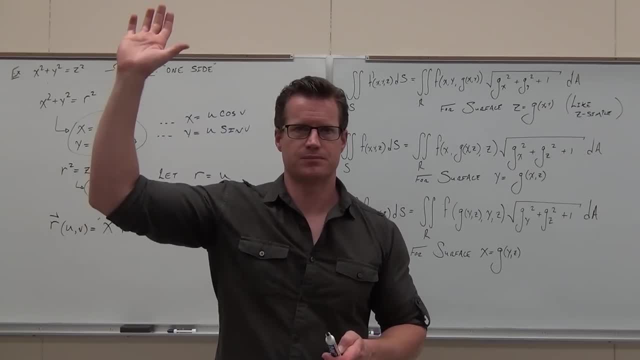 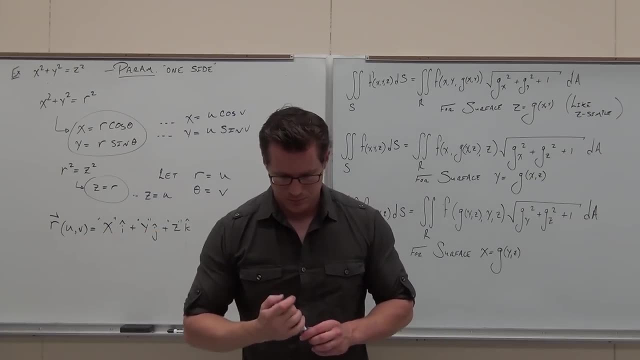 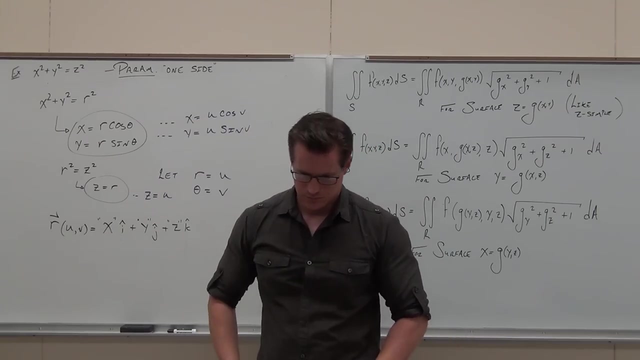 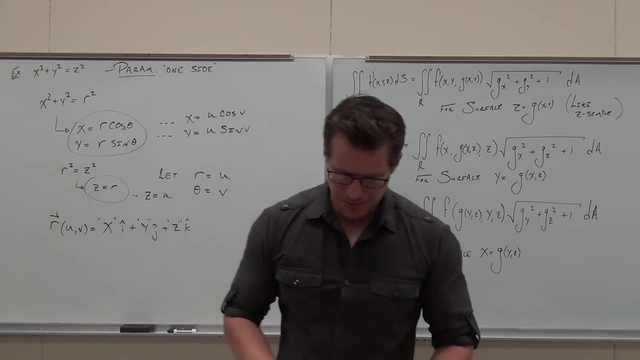 that transition in your head every single time Should have answered real quick with that one. Okay now, what I want you to do right now is take what we've done and build your vector functionality with these. Let's see, I want to keep this all the way up here. 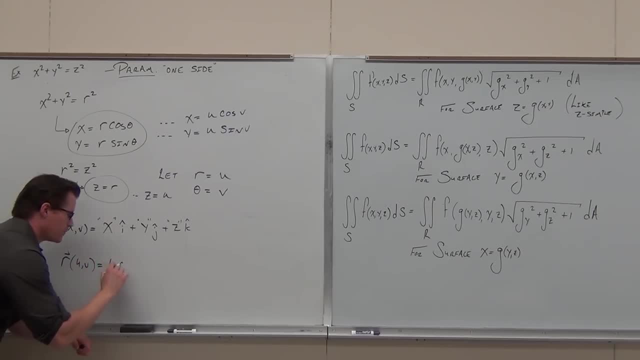 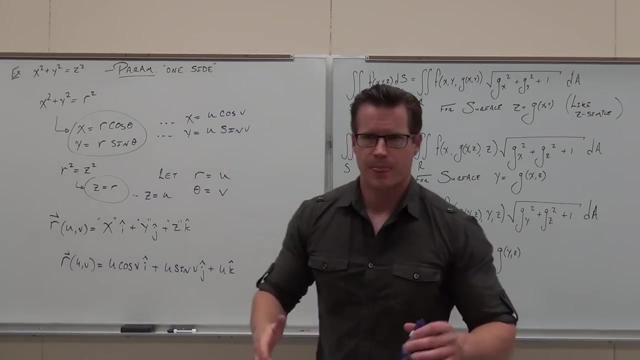 Once you go here, quickly, please, once you go here, U sine v, Perfect. Let's see how this still has an i Plus what u sine v. And Yeah, Here's the point of all this: This will give you the same cone that that gives you. 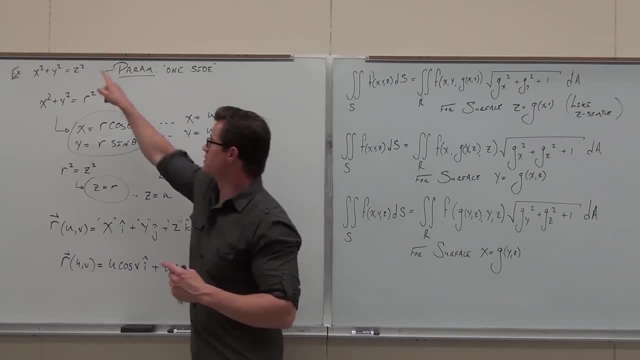 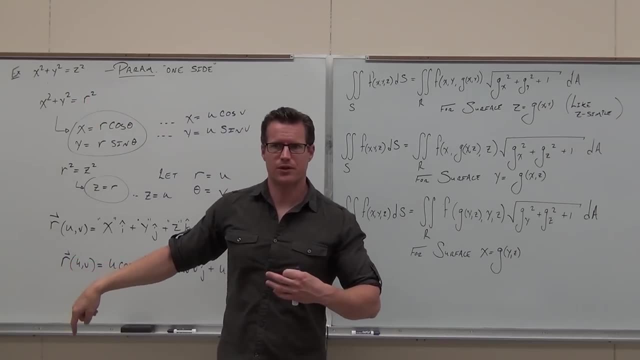 It's the same thing, which means any time I want to use this, but I don't want to use three variables. I either have to solve for z or I could reparameterize and do the same exact stuff with it, which will be the answer to that one. 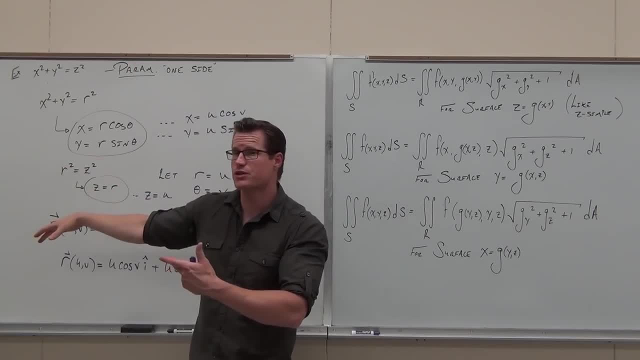 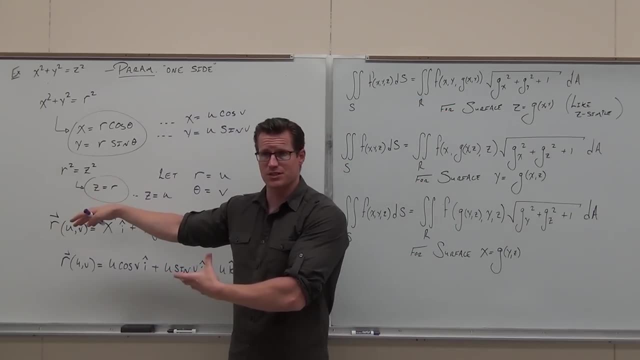 Well, this leads us to the next question: What if you have chosen to parameterize your surfaces, but wait, that stuff's all in regular functions? Can we still get this stuff from these type of surfaces? Yes, Yes, There's a slightly different way that we can talk. 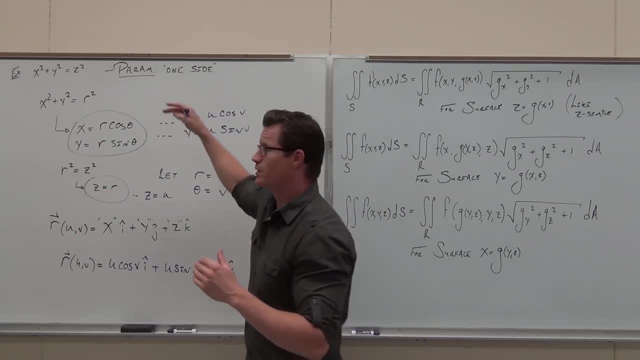 about surface areas, So I need your heads wrapped around this. Firstly, I've only given you two examples, but they illustrate pretty much how to do this. Are you guys okay with parametric surfaces? How to take a surface and parameterize it? 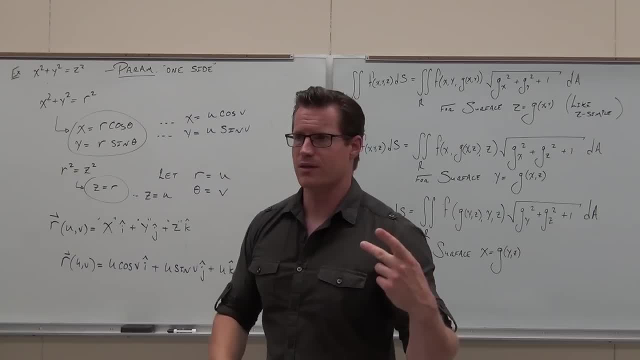 I'll give you two ways. Most of them fall into one of these two categories where either they're solved for variable already- piece of cake If they're not, pick a side- And then, as soon as you pick a side to parameterize. 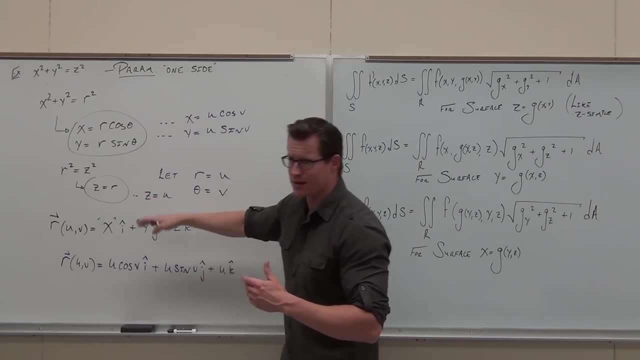 then the rest of it just kind of flows, And then you create your vector function x, i, y, j, z, k and you're basically done, You guys, all right with that one. So let's suppose that you've done that. 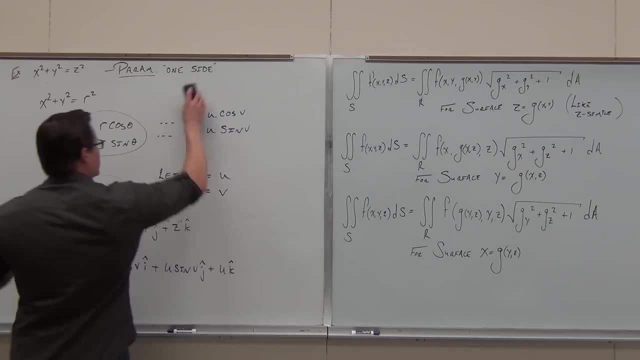 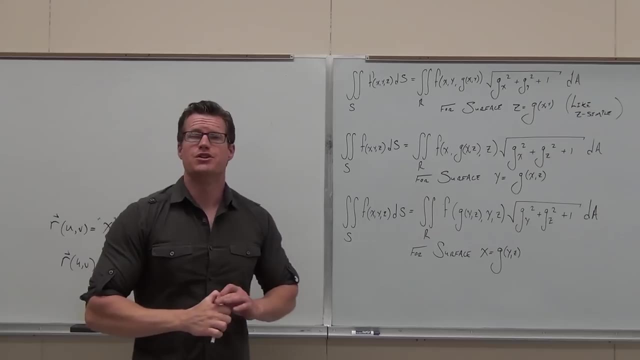 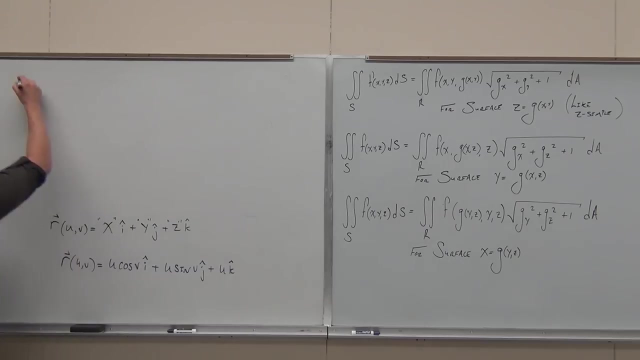 So you've got this vector function. it looks like that And it's a surface. Then there's another way that we can talk about surface area. The second way we can talk about surface area- This is an- Would be this. Now imagine, okay, if you just did all this work. 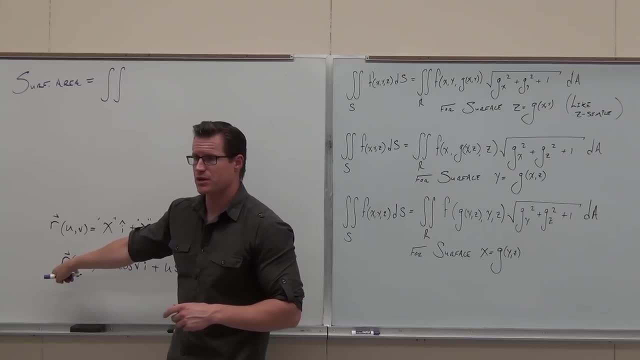 and you have this vector function represents a surface. What two variables you got. Could you take a partial derivative with respect to u? Yes, Could you take a partial derivative with respect to v? Yeah, Let's go back to the previous data. 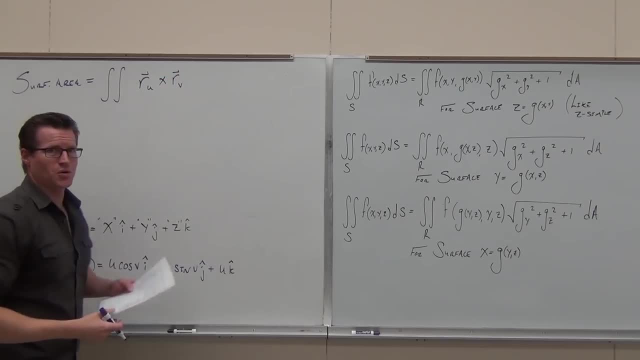 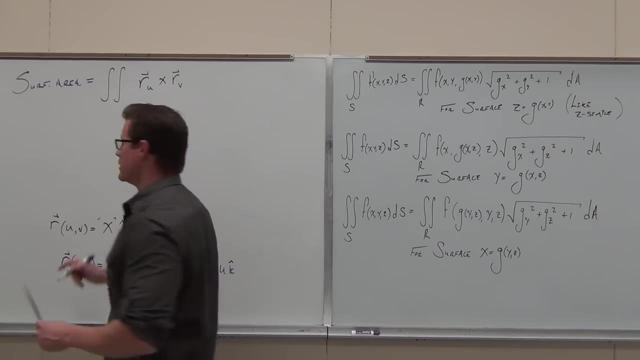 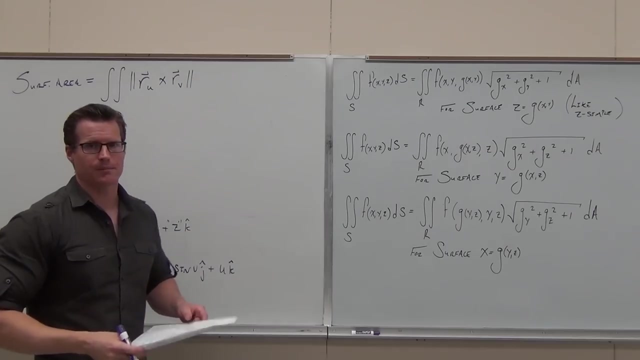 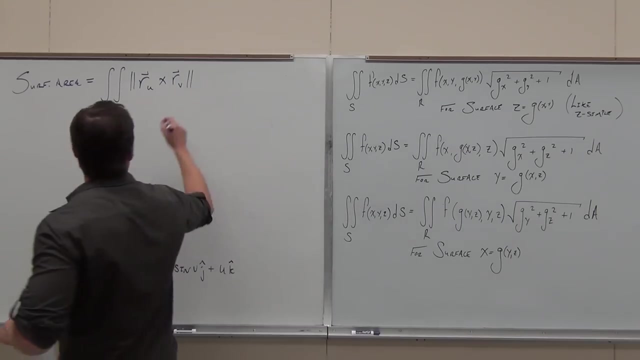 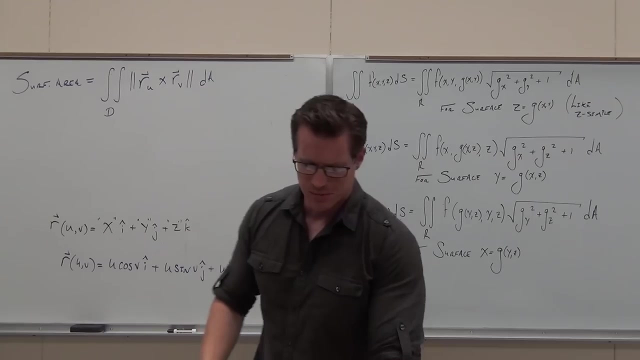 Could you cross product those vectors that you will be getting with respect to u and v? Yeah, Could you take the magnitude of it? Yeah, Here's the nice part about it, Here's the cool thing about it: The d. so what this means is very, very similar. 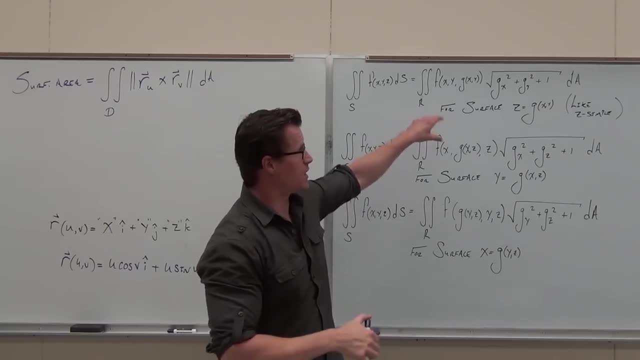 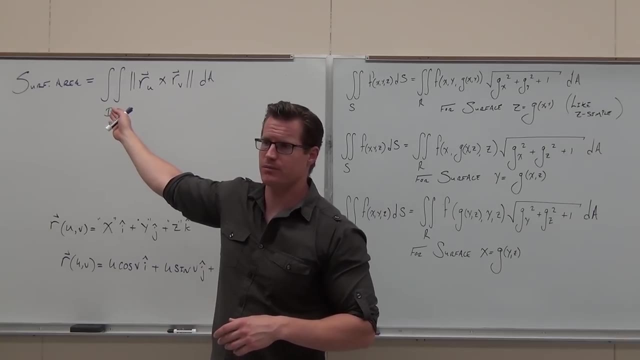 to what we did with this stuff. where r is the projection onto a plane, d is just the balance of your parameters u and v, That's all it is. So d is the- basically you call it domain Domain of the parameters u and v. 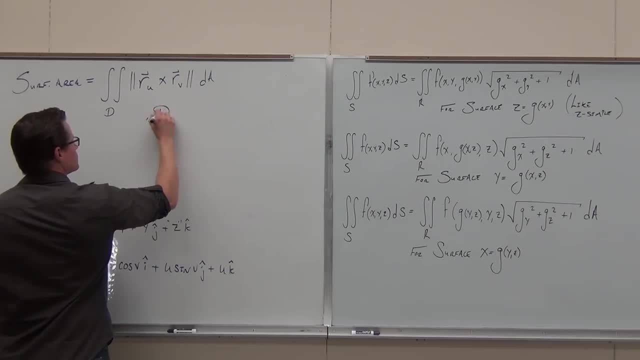 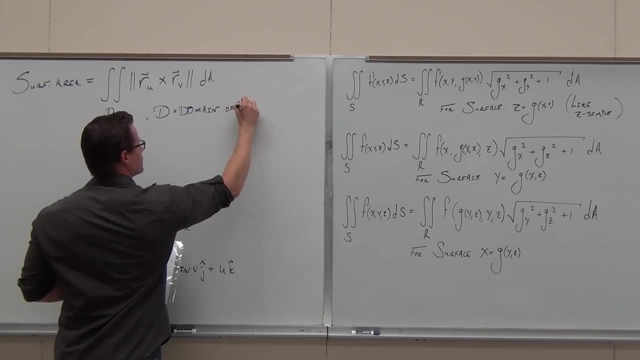 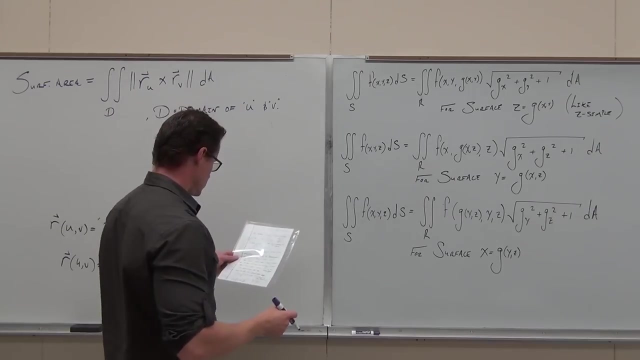 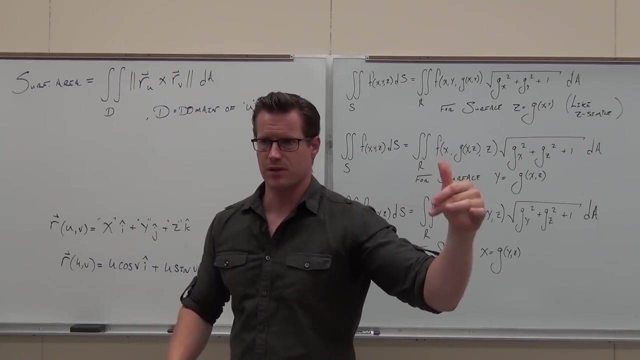 I don't really want to run, do you understand? that's a notation for the partial derivative of the vector function r with respect to u and with respect to v. Same like that was. that was the same for g. All right, So what's d a going to have to change to? 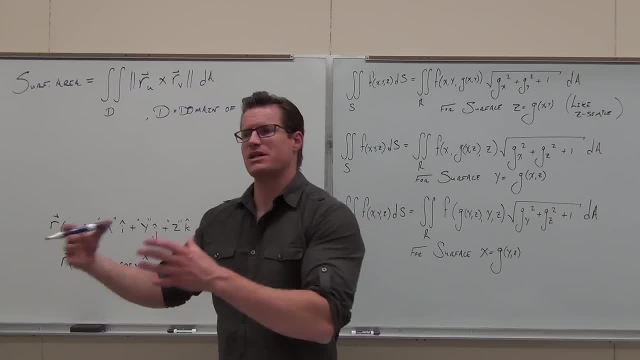 D u d v. Yeah, it just have to be d u d v, because our variables now are just d u d v. Is that all pretty straightforward to you? Because I'd like to do an example here real quick. 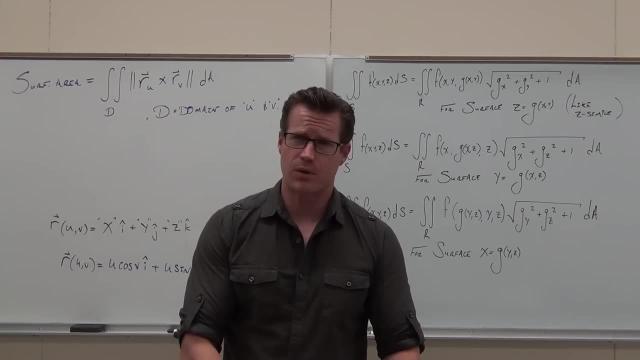 but I want to make sure that we're good on it. Are we? Are we okay with it? Am I losing you? You falling asleep? There's some wake up juice here Now. we have talked a lot, but the idea was: 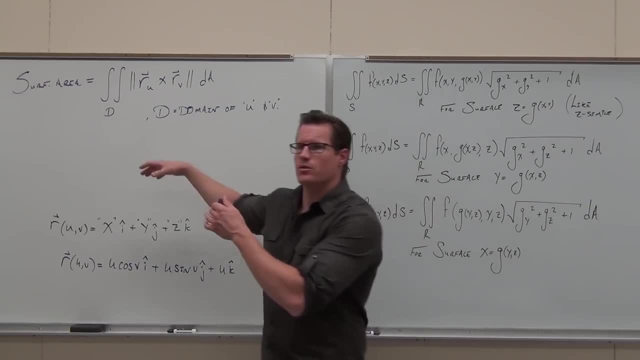 I'll answer your question in a second. the idea is: hey, if you can parameterize surfaces, can we work with that? Yes, Now, now have your eyes on the board here real fast. please Put down your phones or your whatever you want. 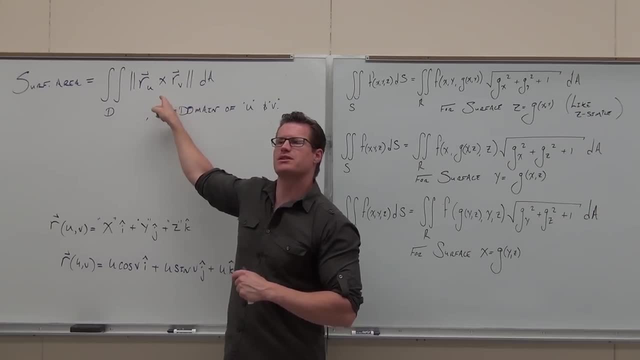 Just put it down and listen. What is this? This is the surface area. This is the surface area of whatever this vector function gives you. does that make sense? Look at the board right now. What's the mass density function? What is the mass density function? 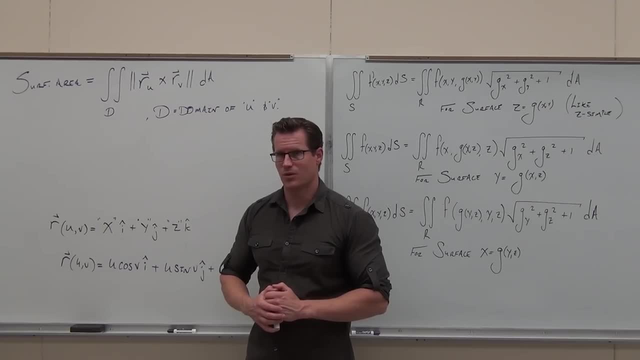 Is there a mass density function? What is the mass density function? One, One, One. We're right here. Look at the board. We're right here. Do you see it? Same thing. We've just defined our surfaces parametrically. 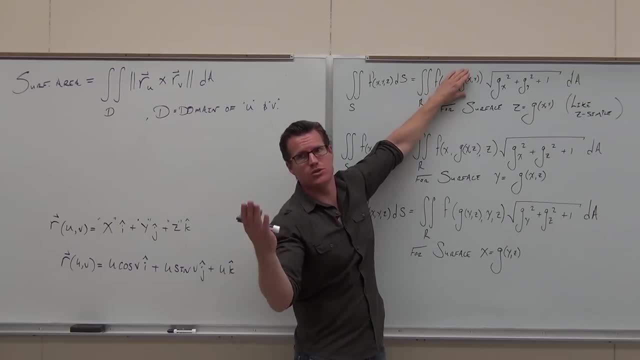 Same thing, In fact. look, I'm begging you to stop with the freaking what you're doing and look at the freaking board. I'm begging you. Do you have to beg? I'm going to beg you. Stop and look. 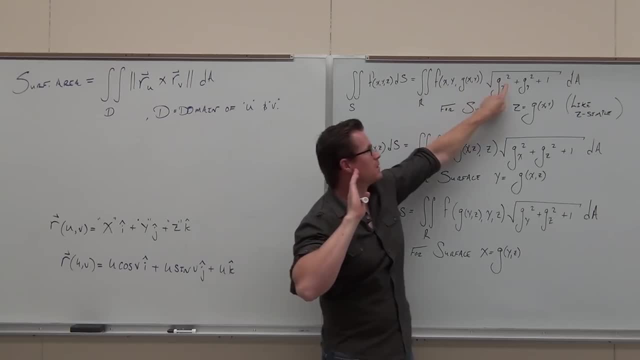 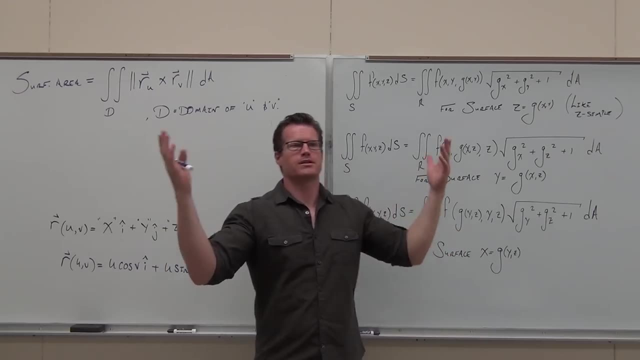 How do you find a magnitude? It's practically the same thing. You're practically doing the same: Squaring them, adding them, squaring them. It's the same thing. You're just doing it parametrically. That's all that's happening. 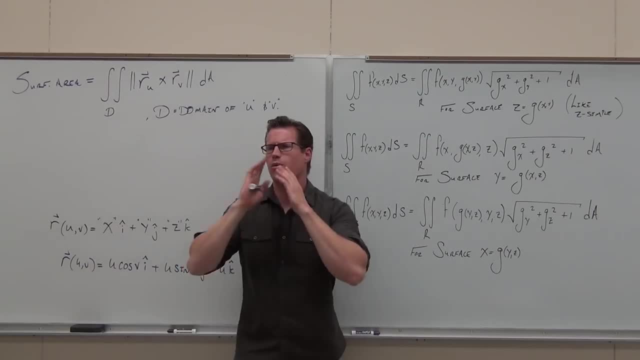 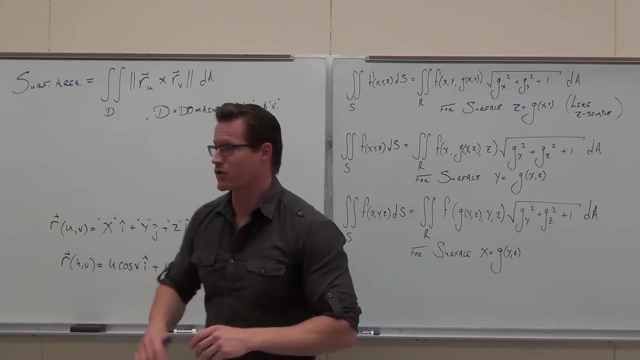 Your mass density function is one giving you surface area. Oh, wait a minute. So how could we go about and change this into getting a, a surface integral with a mass density function? What's going to go right there? A mass density function defined in terms of u's and v's. 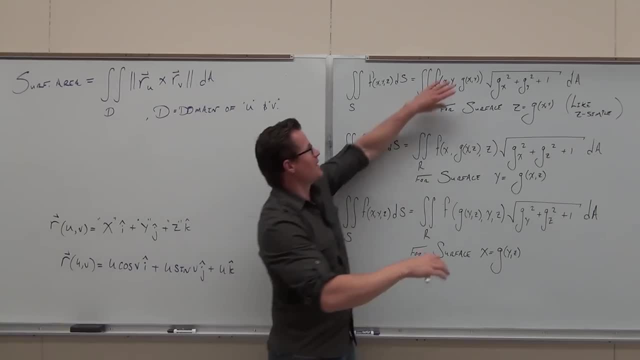 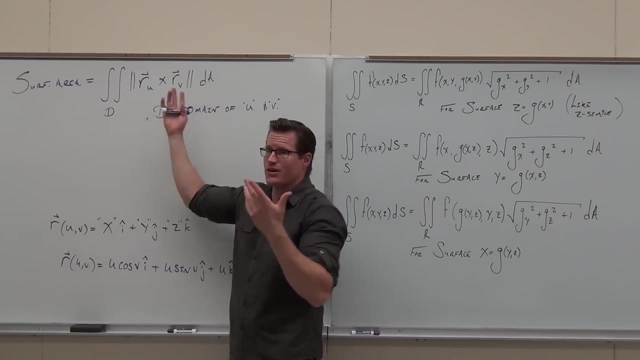 and we make the jump. So right now we have basically 14.5 again, but just with parametric surfaces. All we're doing is finding a magnitude of the cross product, That's a vector. Find the magnitude of the vector. We're basically getting this, this surface area idea again. 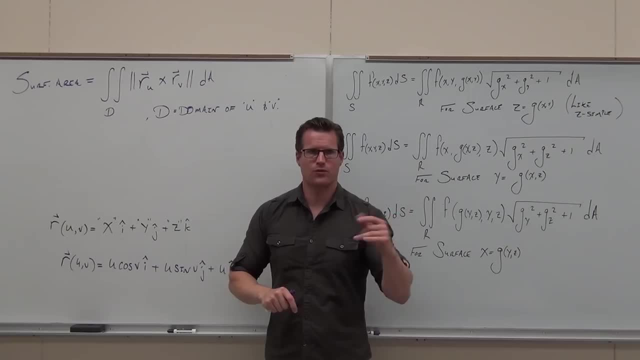 If we put a mass density function right there, we'll have a surface integral finding the mass of whatever the surface area is. We're going to get a bigger mass density function. So I'm going to build in a vector surface that that vector function finds. 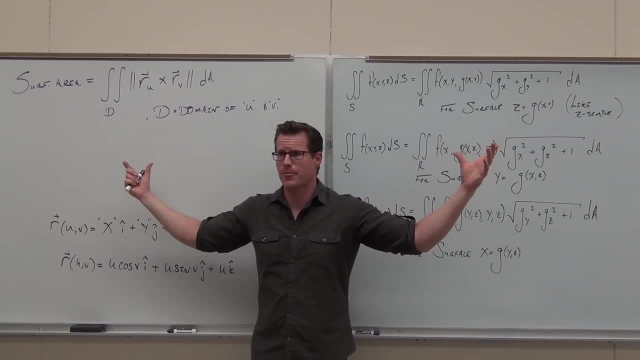 Is it making sense? You guys see the connection. I can't have it be separate. I've got to have it be the same exact idea, just a slightly different way. Should I be okay with that? And so I teach it this way? 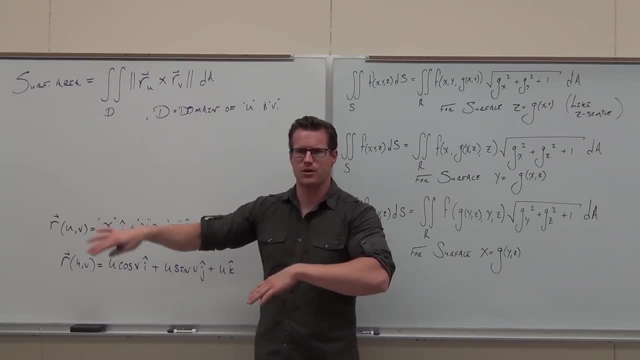 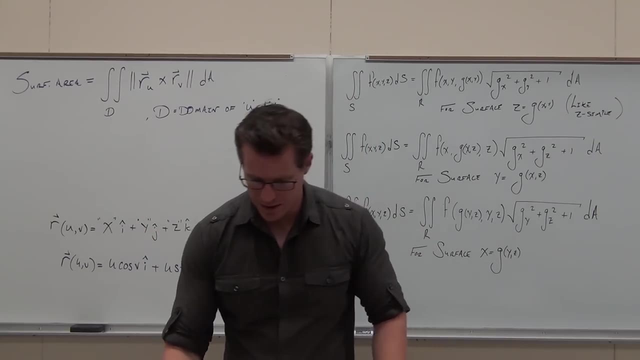 It's got to flow. You can't just say, oh, parametric surface, that's a long time ago. It doesn't make sense, It's the same stuff. It's the same stuff. Now, what I'd like to do, we'll probably just do one example. 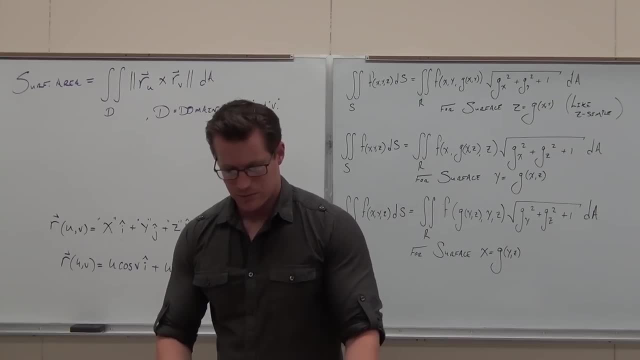 And then I'll show you the- yeah, I'll call it parametric surface. It's a little bit different. Okay, I'll show you what I was just talking about and then take a break. So what I'd like to do right now is find the surface area. 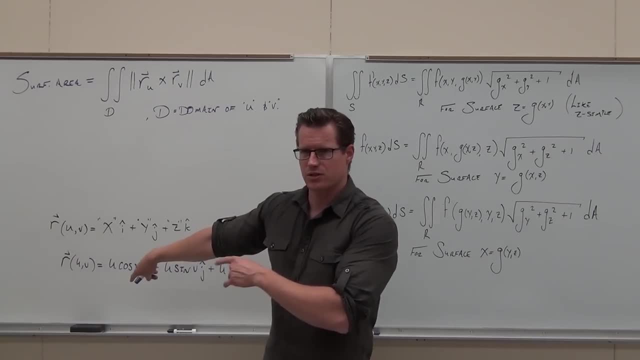 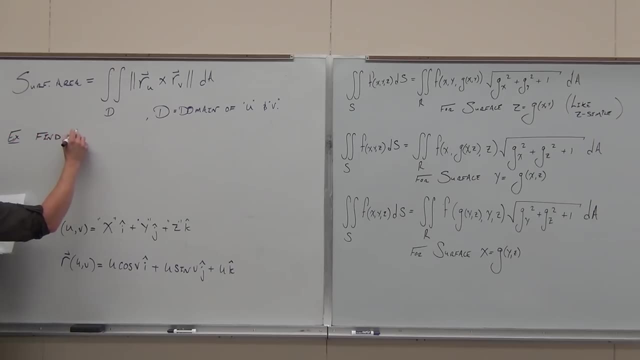 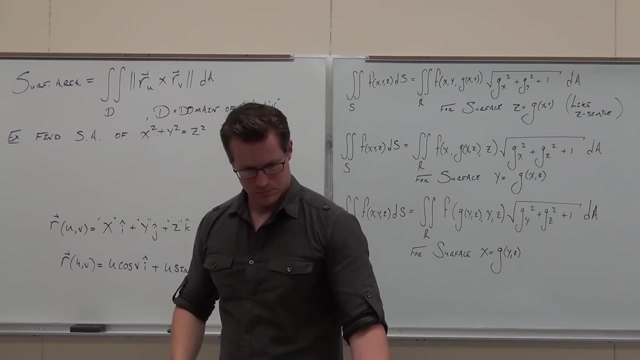 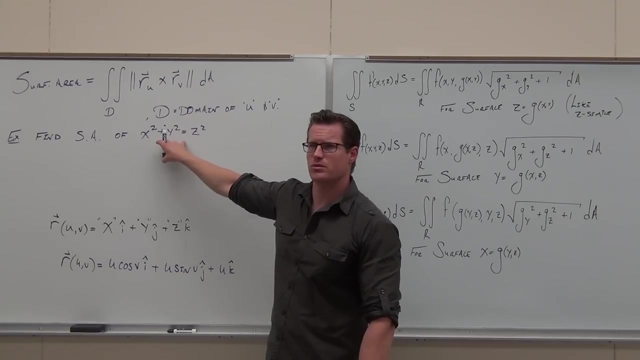 of the cone that we just parameterized. Okay, so I want to do that, So let's go through it. Hey, find the surface area of this thing. Could I write that in terms of a function z? Yes, but I have to take a square root and I don't really want to do. 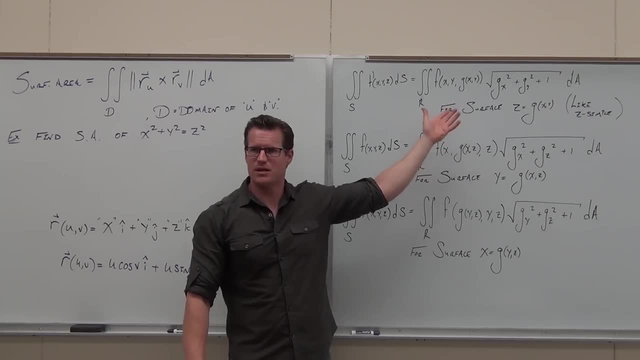 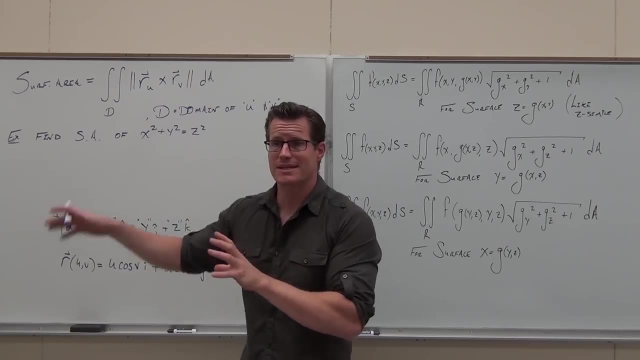 that, because I might lose half my cone. Is it a problem? Well, maybe, maybe not. You could always double it. if it's a symmetric cone, probably double it. Could I do it a different way? Yes, yes, Can I reparameterize that surface? 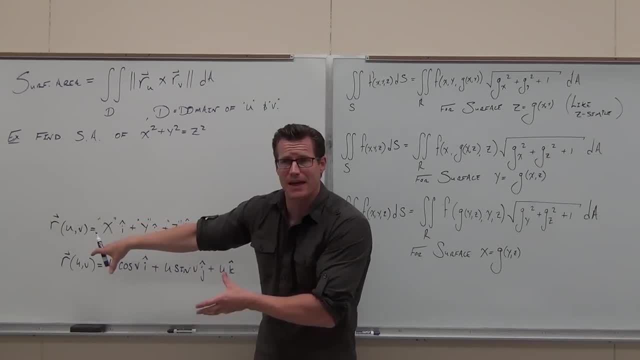 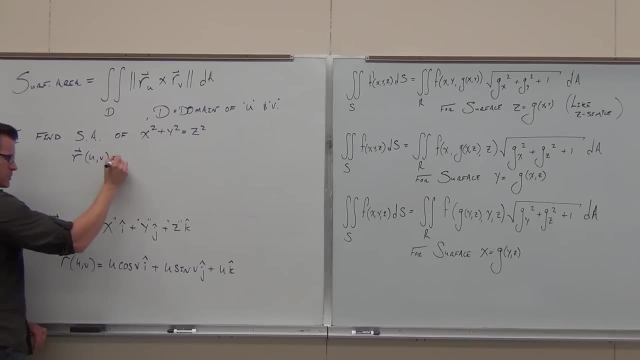 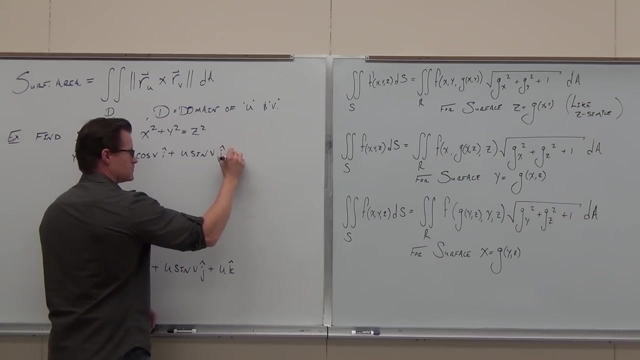 Yes, in fact, we've already done it. I don't want to go through the process, but we've already done it. We just did that. That was why I did that example. So this says: okay, if I define this in terms of this, this and this. 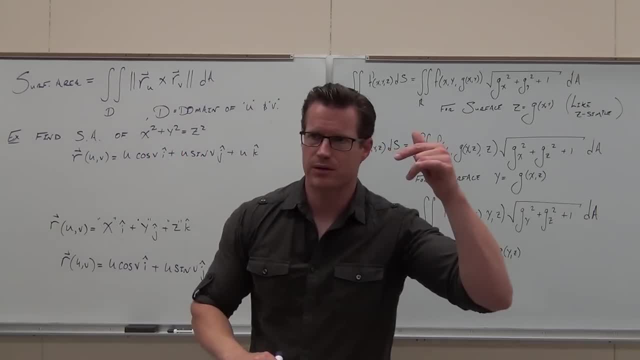 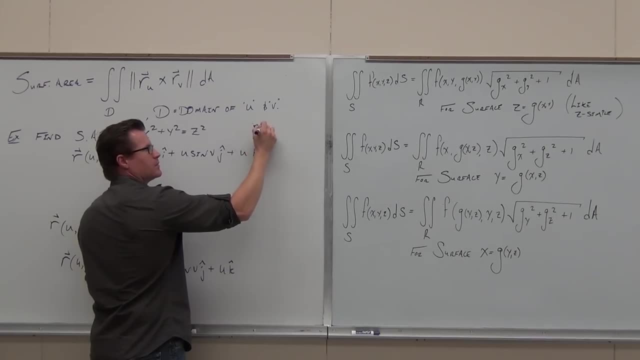 I'm going to write a little side note just so, because later on I'm going to come back to this. I'm going to prove it to you. okay, Just a little side note. remember that r was u and theta was v. 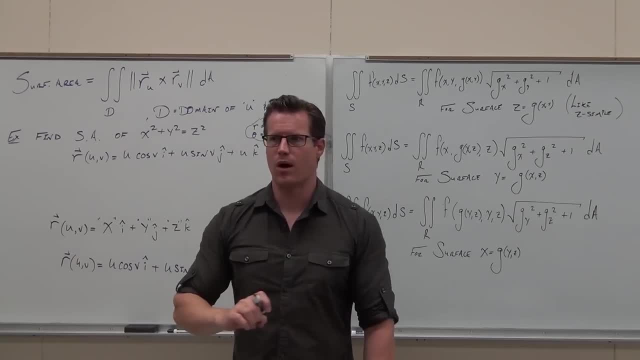 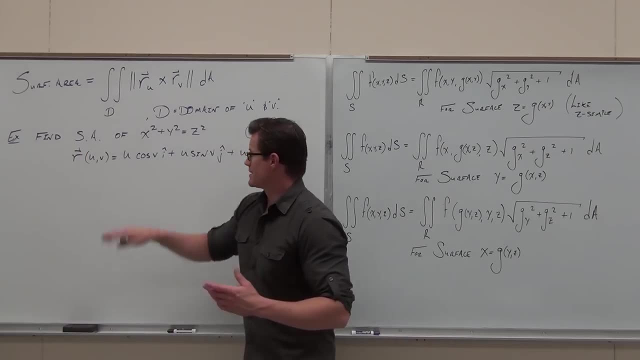 Just keep that in the back of your head, okay, I want you to remember that for a while. So that's our vector function. Here's the first thing I need you to see. Do you recognize that this is the same full cone that that is? 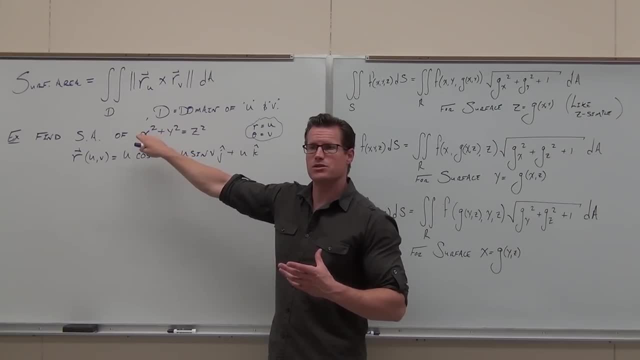 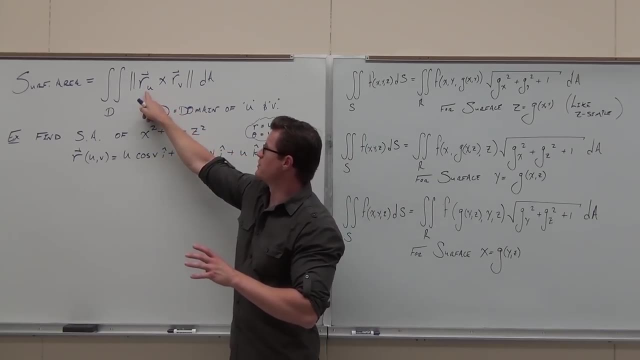 Do you guys see that It's the same exact thing. So let's start working with this and treat it as a vector. So this is our vector function that defines our surface. Can you find the partial derivative of this thing with respect to u? 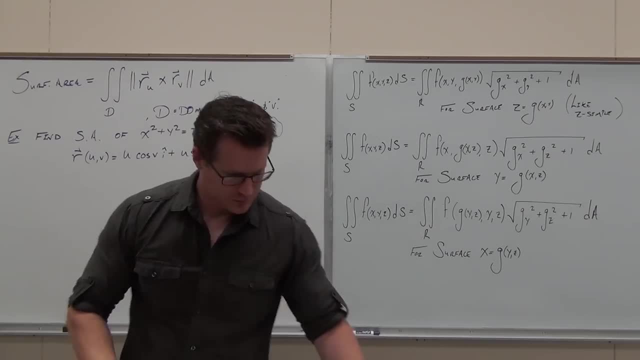 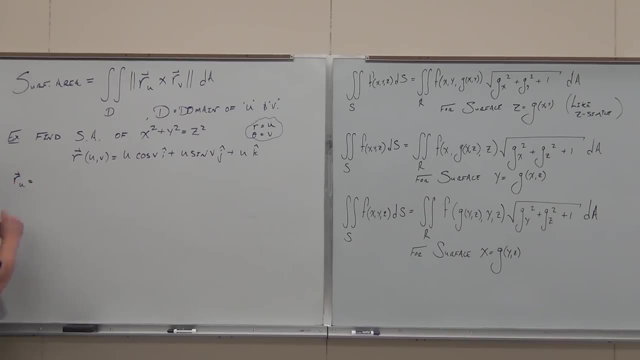 Okay, let's write that down. Tell me what it is. Cosine Cosine V9.. V9.. I And Sine Sine V10.. And Sine Sine V10. V10.. 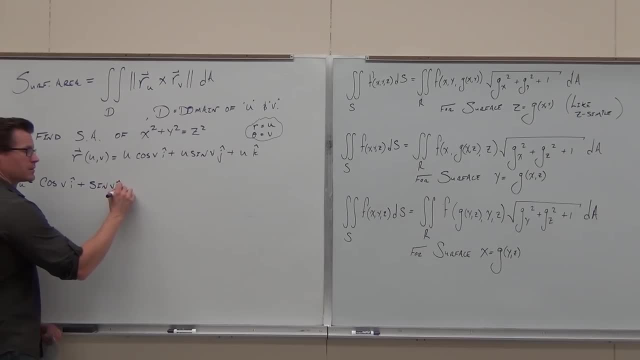 V10. And V10. And V10., V10., V10., V10., V10., V10., V10.. Cool Oops. Can you find the partial derivative of this with respect to v? Can you do that? 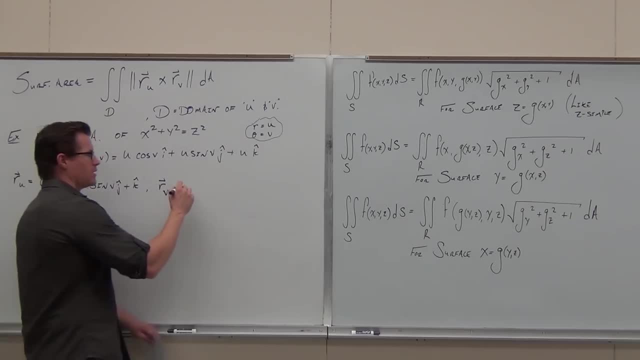 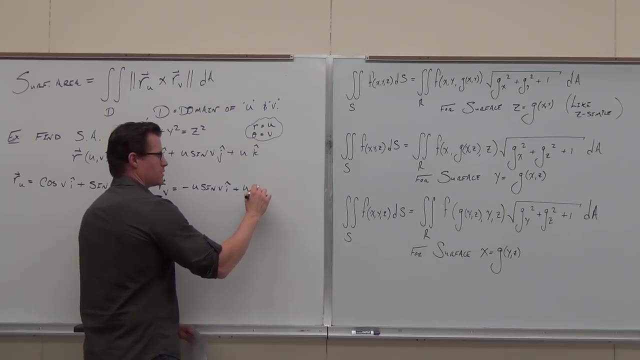 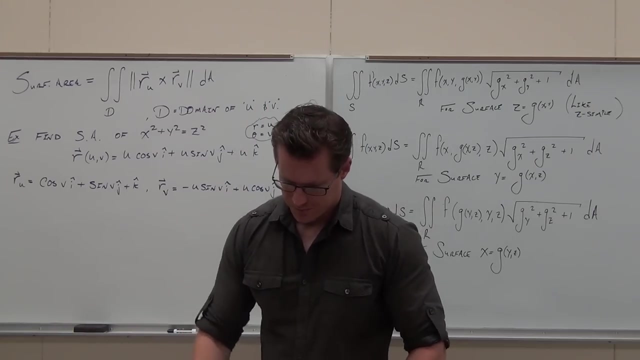 A little bit more complicated because you got some trig function up there, but we should get negative u sine vi plus u cosine vj, And that's it. There should be no k because there's no v component of that. So what's this? 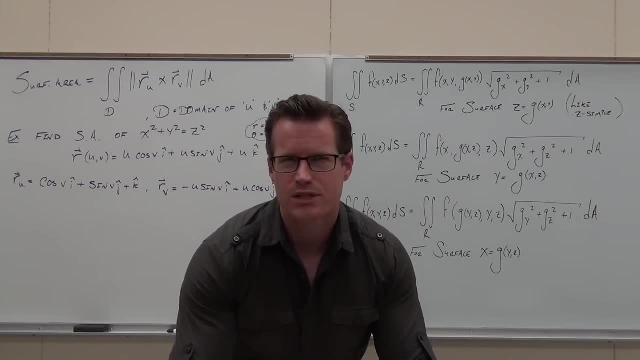 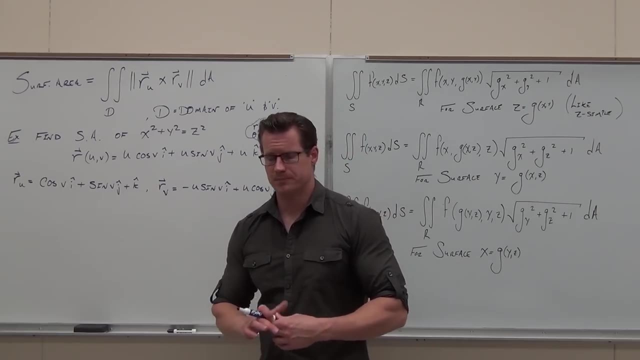 V1., V2., V2., V3., V4., V4., V5., V6., V7., V8., V9., V10., V11., V12., V12., V13., V13. 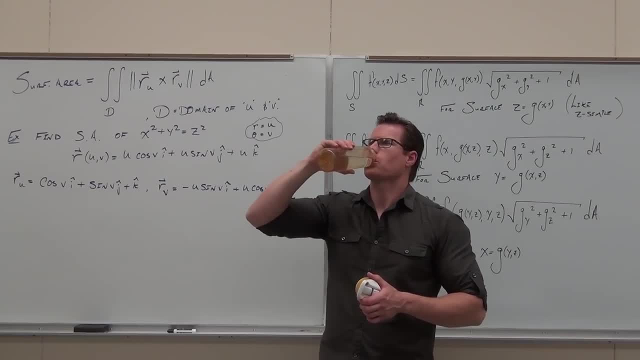 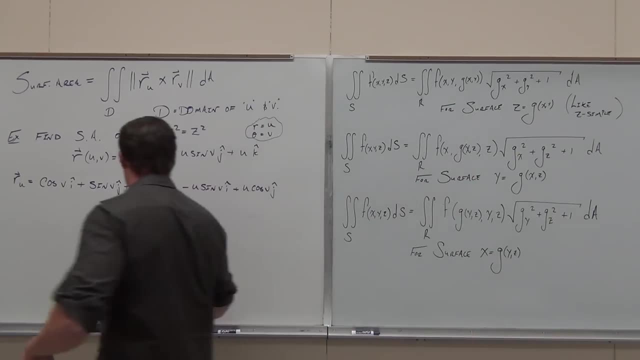 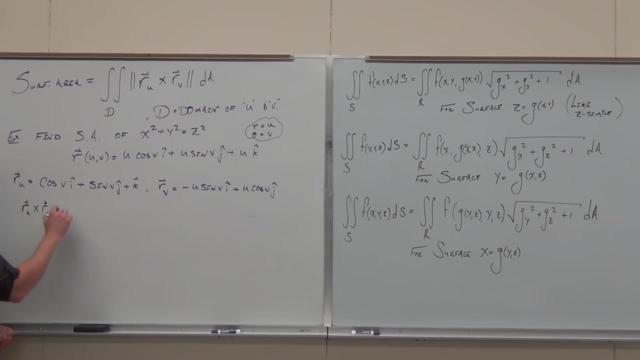 V14., V15., V16., V17., V18., V19., V21., V22., V23., V24., V25., V25.. Hopefully you made it that far. Did you make it that far, At least set up. 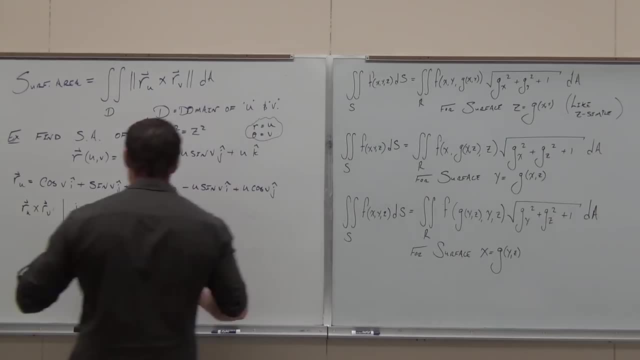 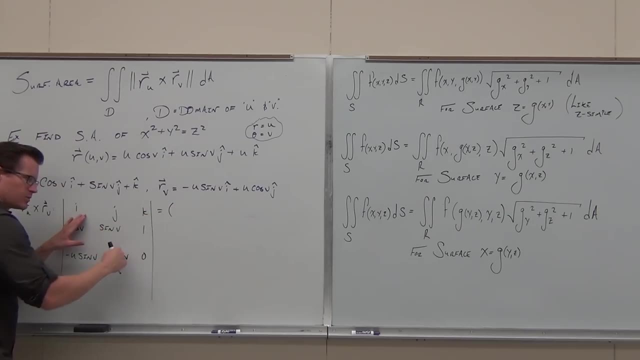 Do you all remember how to do it? If you remember how to do it, it's kind of a cover-up method. I cover up this. We multiply, subtract, multiply, So multiply 0, subtract and multiply negative u, cosine v, and then we have an i. 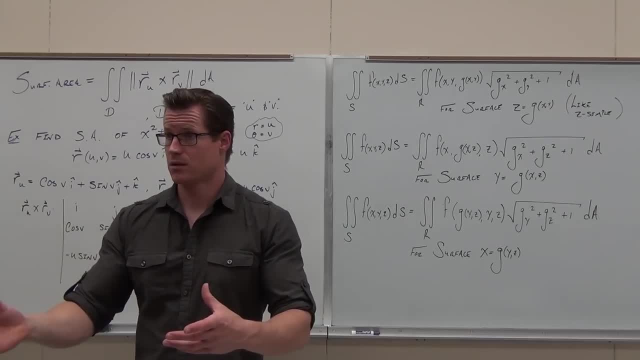 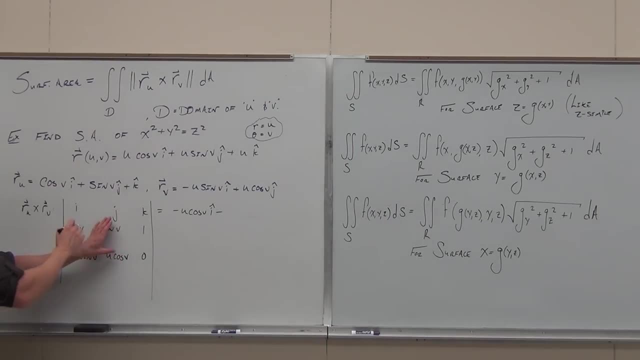 You guys. okay on the negative: u cosine v: i Did you get the same thing. Next thing, Before we do anything else, what's the next sign? Minus. Make sure we're okay with that. Minus. Okay, cover this up. 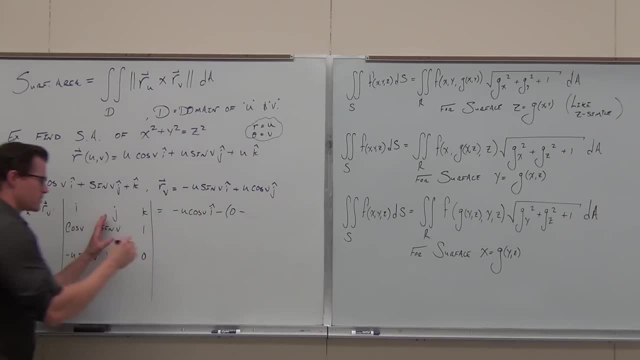 Multiply, That's 0. I'm going to show this one so we don't get all screwed up on it. Subtract and multiply gives us minus a negative. That would be plus u sine v, j. Are you okay with that one? 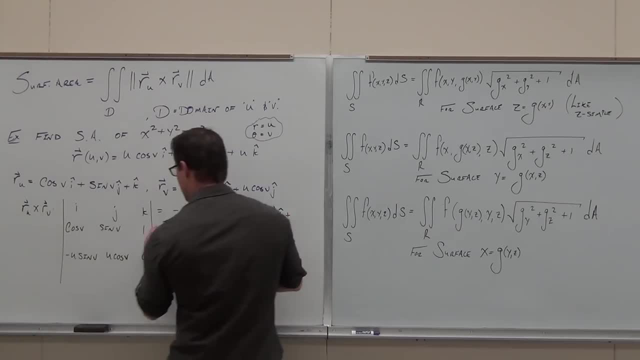 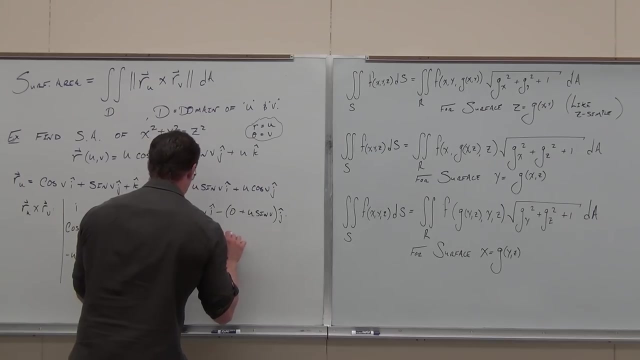 Okay, Lastly, we got a plus. I'm going to go okay. well, oh yeah, I'm going to break it down. Bless you. Multiply, we get u cosine v squared Cosine squared v Minus. 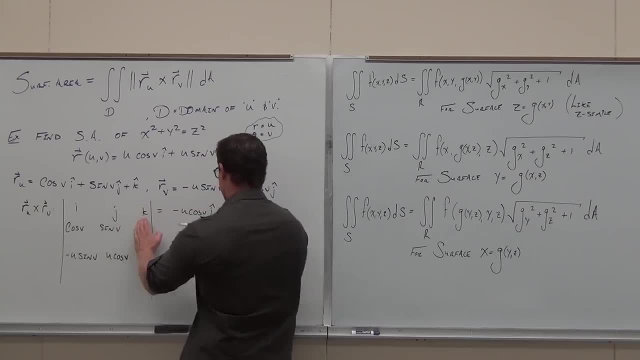 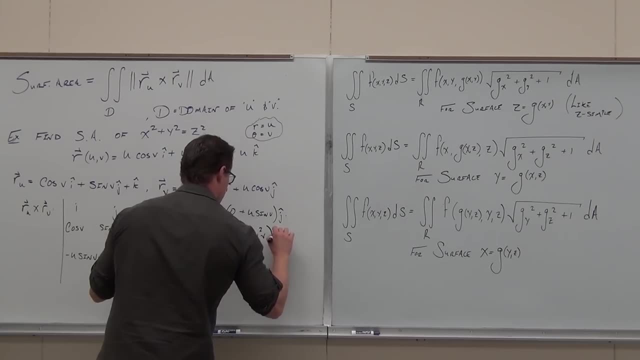 Well, if I subtract, I subtract a negative here. So plus u sine squared v and then k: Okay, I'd like to show fans if you're okay with the cross product, if you're all right with that one, Yes or no? 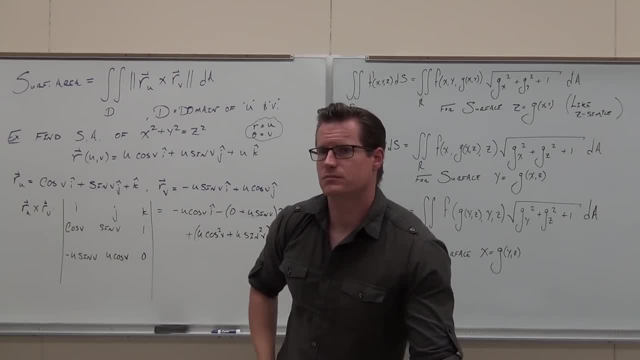 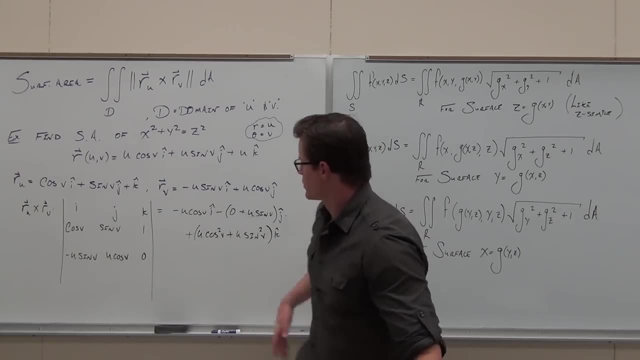 Yes, What now? Before that, Simplify as much as you possibly can, because I don't want to start in magnitude. if you have to simplify these pieces, What's going to happen here? specifically, Factor the u cosine squared plus sine squared v is: 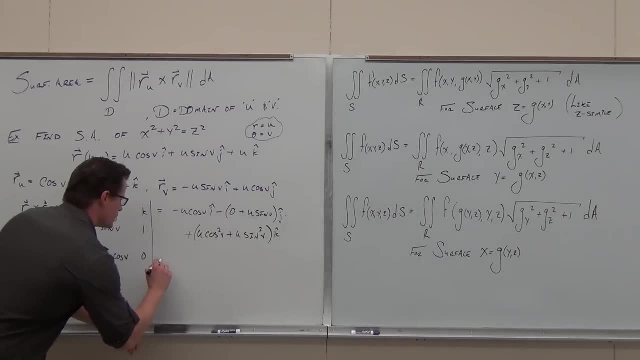 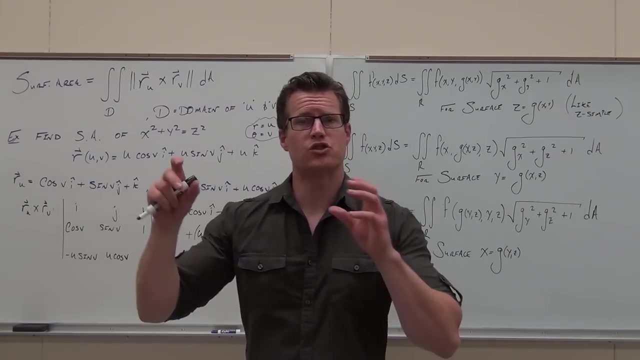 So this is just u Simplify that, Simplify that. We'll do it again Now, find the magnitude. Remember, with magnitude we square the components. add the components and square root them. Try it, Okay, Okay. All right, all right. So we got the root sine f squared. And when we multiply our knowledge of that value, what we add is: If y equals 12 times the inverse of y, F gain polygon y times z, And we get an H and y equals m ž dou MOOUS m. The third element- dangerous to remember, but here we can also say- is: Aim to learn outros to to the 정확ality. But instead of using this- and you're not going to want to be negative- 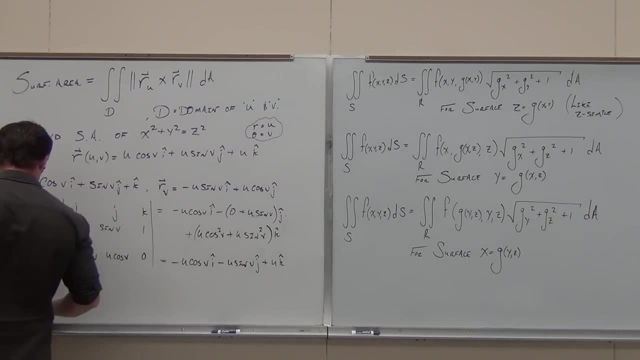 Now find them right there. A have the measure of magnitude. we square the components, add their components and square root. let's try it Right now. Thank you, We can have some simplification. that's going to be taking place. What do you think? 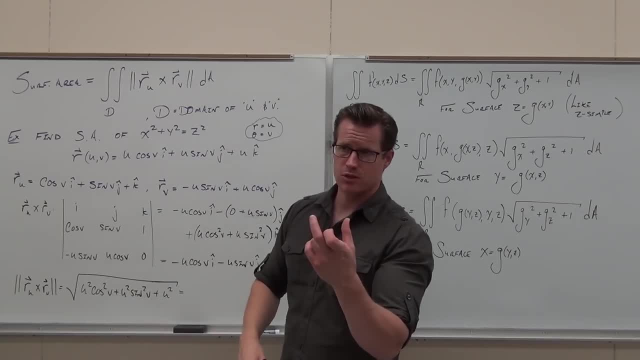 They all got u squared. Factor out a u squared. You're going to get a cosine squared plus sine squared. That's going to give you 1.. But then you also have another 1.. Can you guys see that this is going to give you a 2u squared inside of this square root? 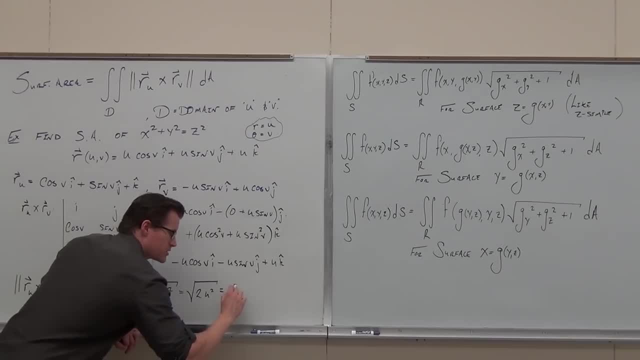 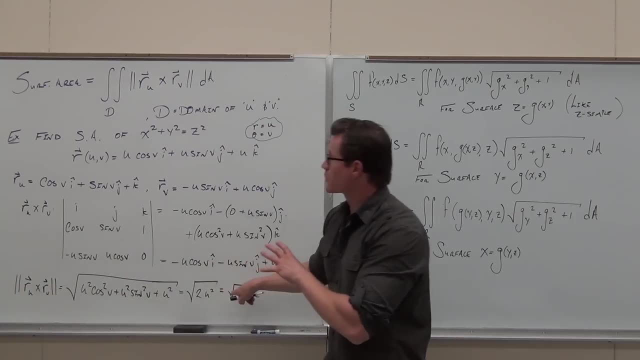 If we simplify a little bit further, then this is simply square root of 2u. Now, what is that? That's now the argument of your surface area. This is just the only thing that you're going to have. That's it. 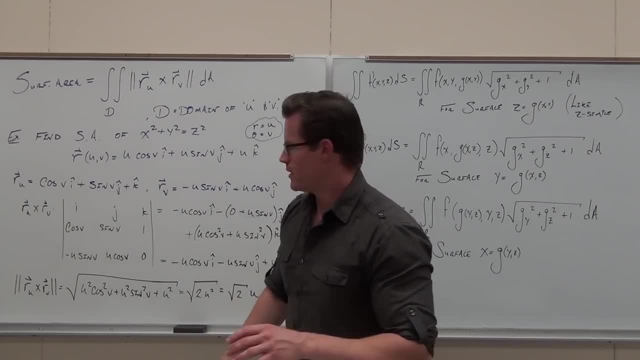 That's all you've got to do, And so I want you to set it up. So, right now, all I want you to do is take this piece, put it in there. Do I want you to deal with the d? No, 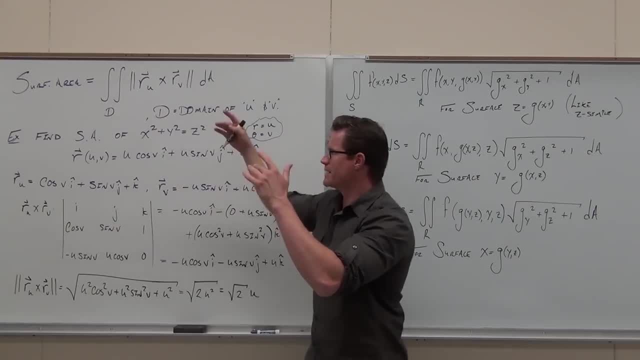 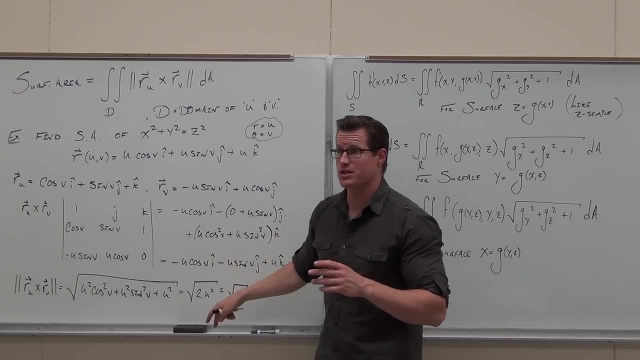 Do I want you to deal with the d8? No, I just want you to set it up. So the whole idea here is: if you can parameterize a surface, find the partial derivatives, do a cross product, Find the magnitude. All the hard work is done. 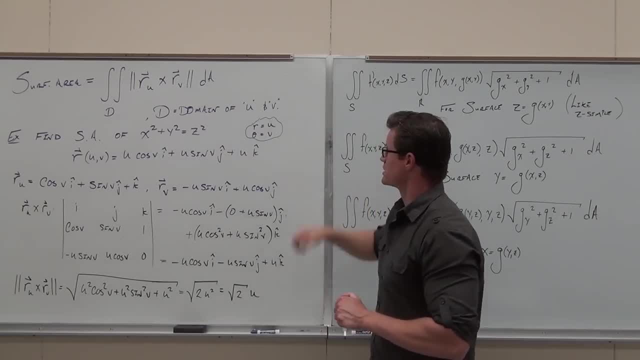 Just set the double integral. I'm going to have to erase this again. I wanted you to see. Well, at least you kind of saw the connection there. I want to make one more connection, But I'm going to erase this here real quick. 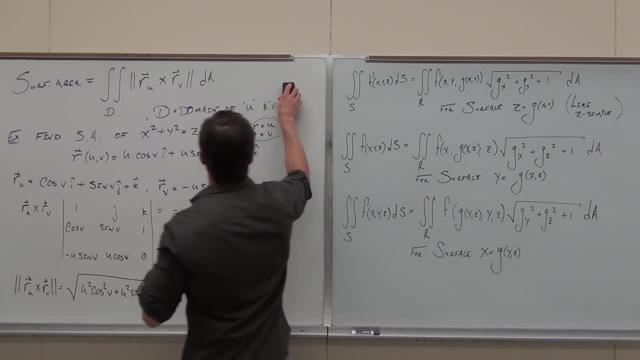 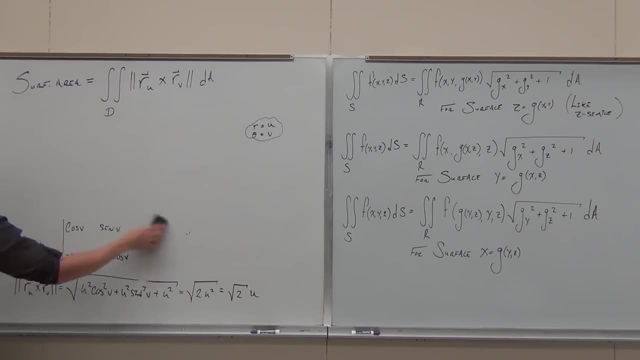 Are you guys okay making it this far? So, when everything's all said and done, Don't skip this step. We have 2 square root u d8.. Yeah, that's not the same thing, is it? Good thing I had you guys here. 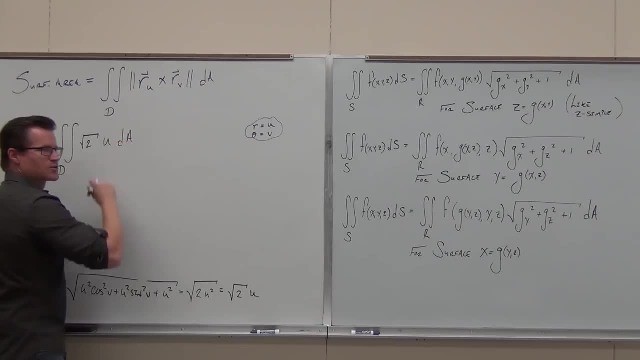 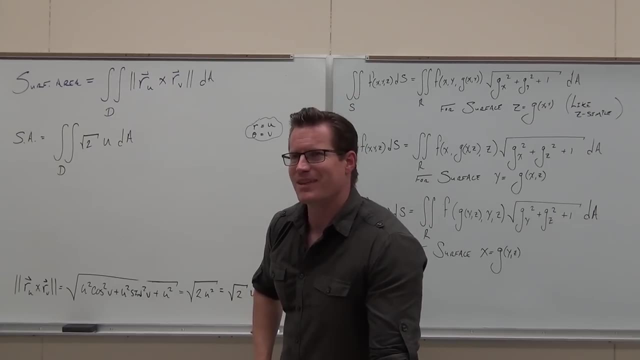 Thanks, So I'm going to miss you. I'm going to miss you all when you're gone. Other classes they just let me go And then 20 minutes later I go. thanks a lot, guys. I appreciate your paying attention. 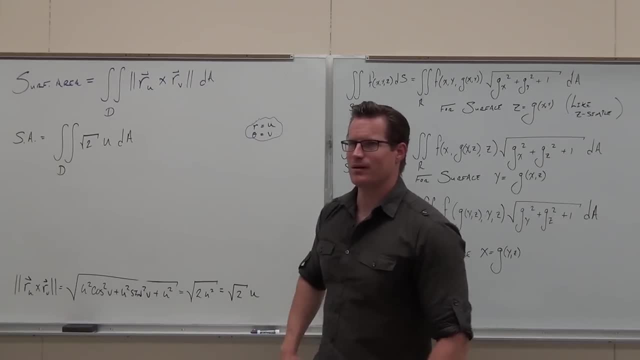 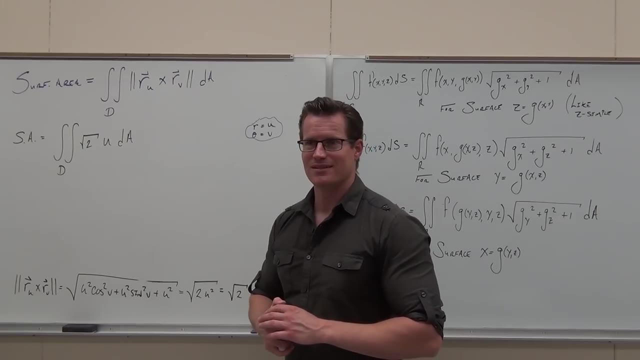 I failed them all. Ha ha, ha, ha ha. Anyways, not you guys, though. You're all getting A's. Yeah, okay, Really. No, that's a joke, It's a meme, It doesn't happen. 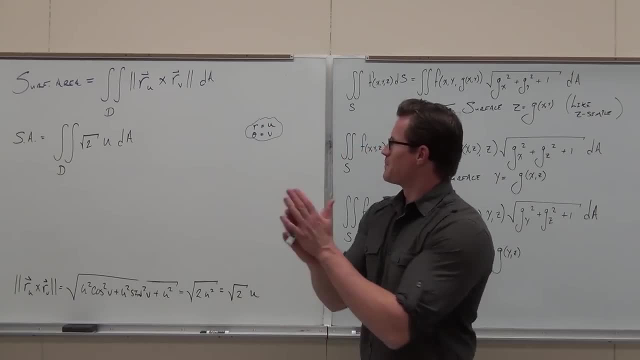 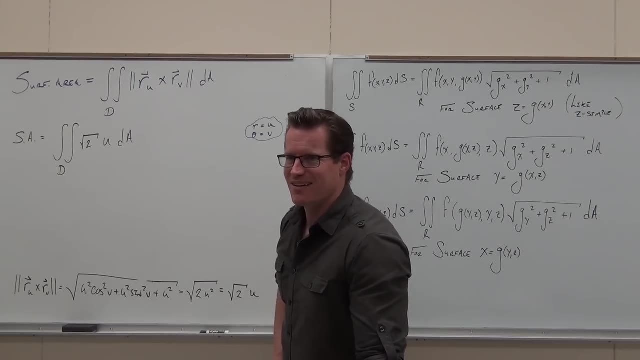 It doesn't happen. Yeah, it's unfortunate, But there are a lot of A's. It's good, Especially on the third test that I have for you. You know that. huh, Yeah, it's good. Anyway, what do we do now? 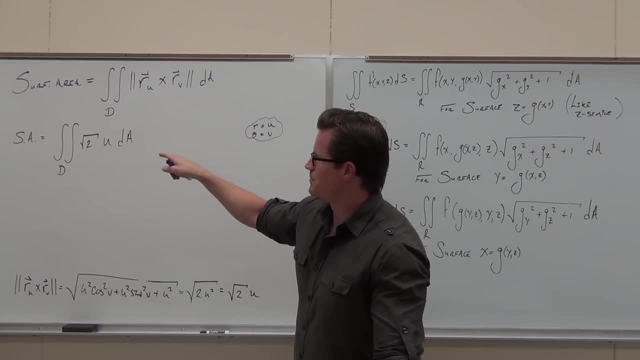 Well, d, what d is, is the domain for our parameters u and v. This is why I had you write this down. Why don't you look at this? If this thing's a cone, okay, if this thing's a cone. 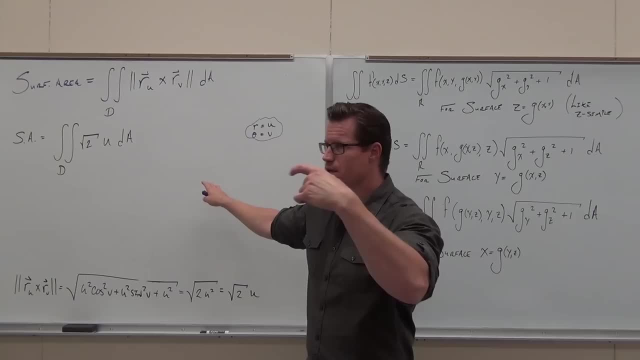 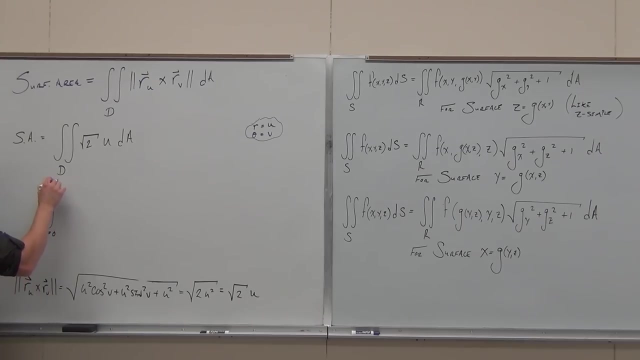 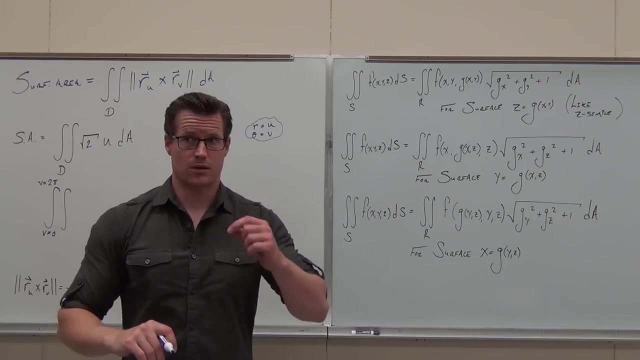 and if u equaled r and v equaled theta to go full circle around that cone, our theta would go from where to where. If I wanted to go along the r, well, I have a choice to make. Look carefully. 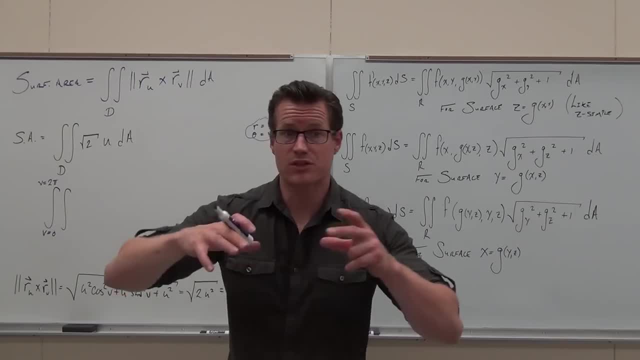 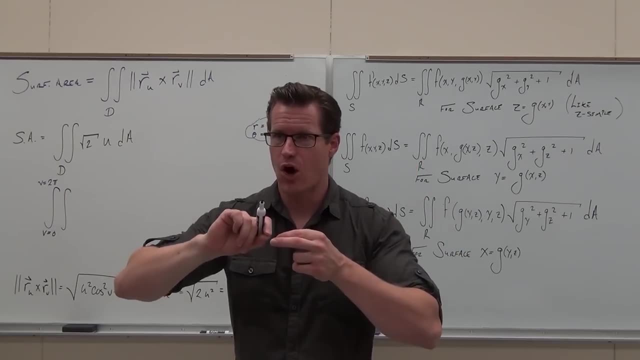 Please listen. Remember: this is surface area, right, And we're dealing with a cone. So this is finding the surface area of a cone, That's it. If I just stop at any r ever and go full circle, it would give me the surface area for whatever cone I want. 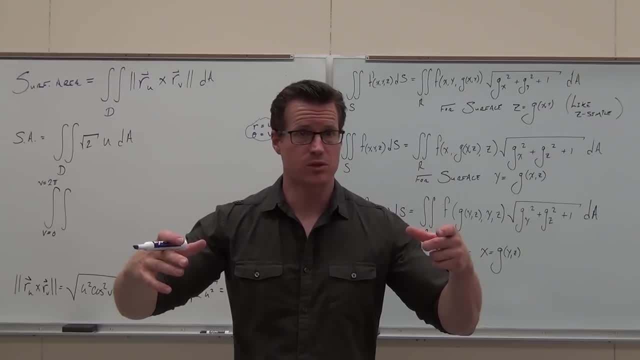 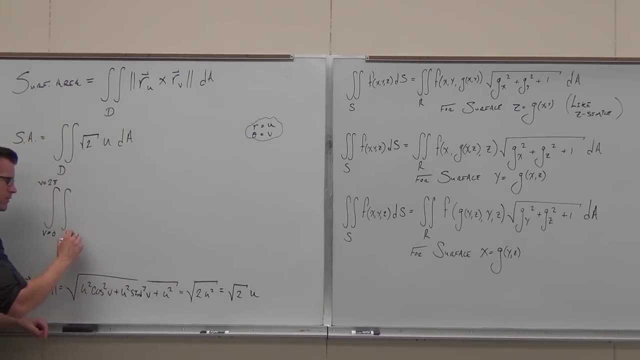 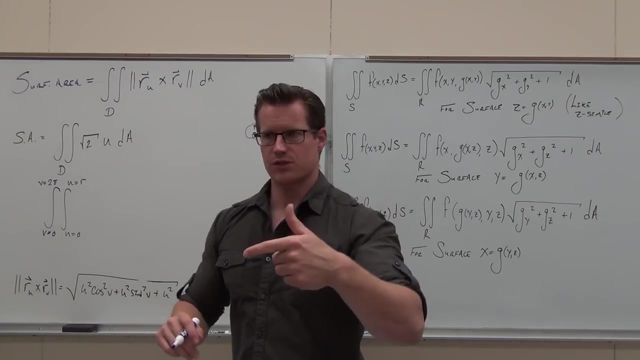 with a given radius. Does that make sense? That's what it would do. Well, what if I let the u- because again, u is the radius, It's all it is- Go from 0 to r? Then what it would give me is a formula for the surface area of a full cone. 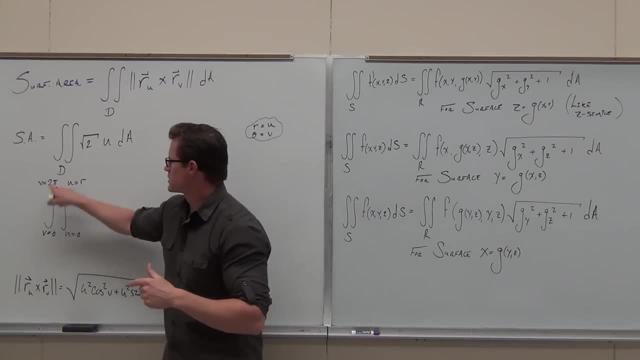 That's what we're talking about here. So again, if I went from 0 to 2 pi, that's just going full circle, Full circle around the cone. OK, If I went from 0 to, like, 4, it would give me the surface area for a cone. 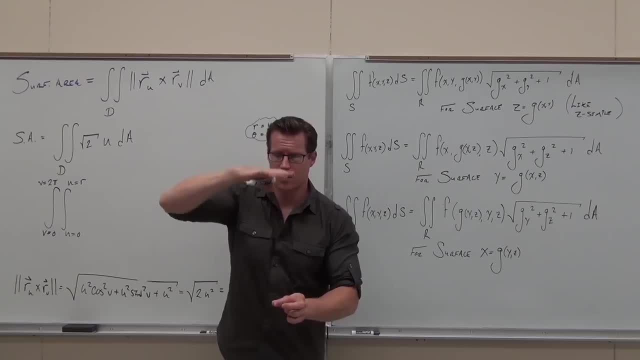 that's stopped at a radius of 4, from 0 to 4.. Does that make sense? If I went from 0 to r, it would be 0 to anything. I could look at r later and find a formula for the surface area of a cone. 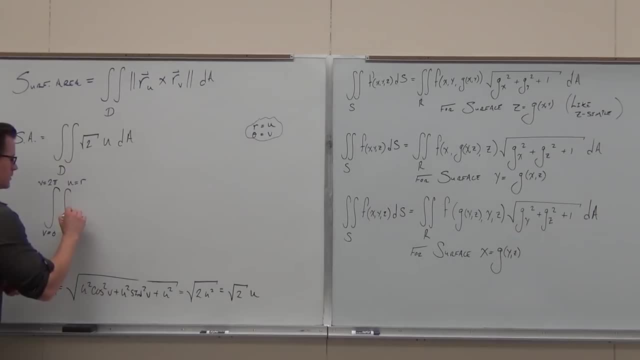 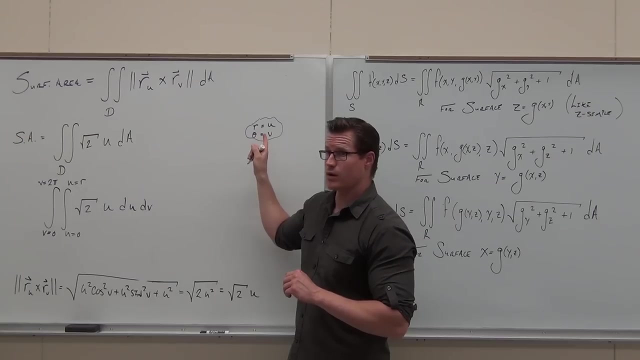 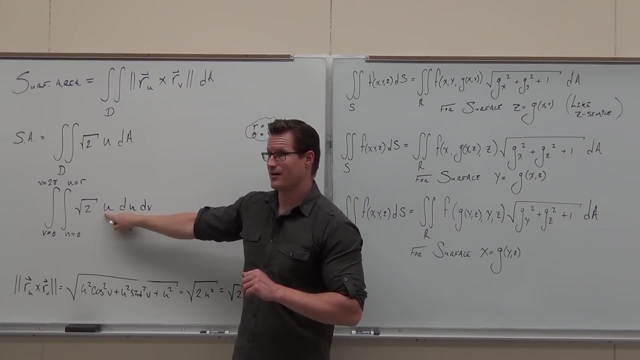 This particular cone root 2? u. Oh, my goodness, You're going to see some magic happen. Who wants to go first? D u d. Where did the? u come from? r? Where did the v come from? 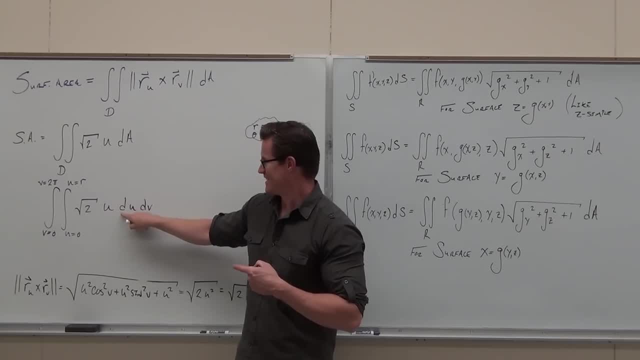 Say it. I'm not going to say it for you. r r, dr, dr. What That's crazy Magic coincidence. There are no coincidences. This isn't right. No, Could you integrate that? Are you missing a u right there? 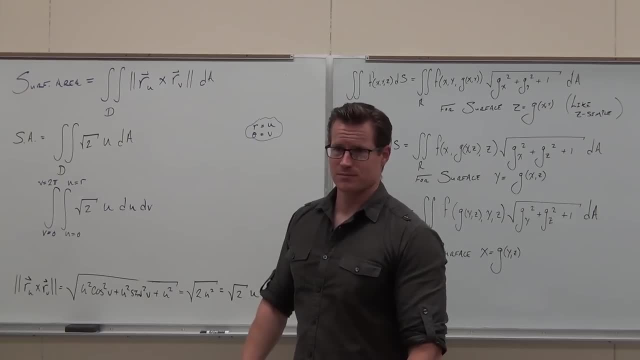 No, Are you missing a? u right there? I'm not missing u This dA, this is just dU, dV. I'm not changing to polar because I already did Already did it. That's the whole nature of letting u equal r and v. 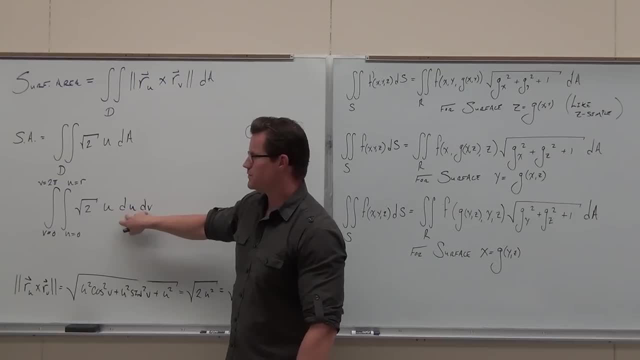 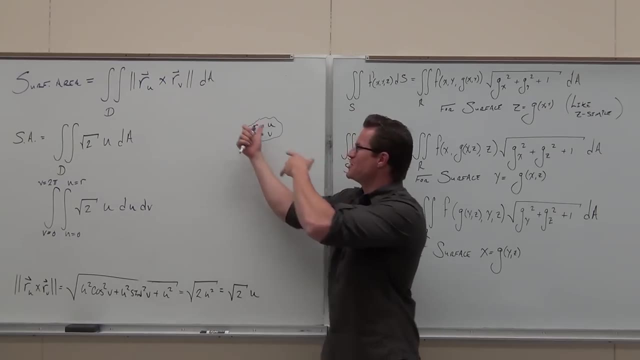 It is polar, You can see it, It's already there, It's right there, It's already done. It's just infinite. It's a single. It's just infinite. It's a single. It's a single, It's a single. 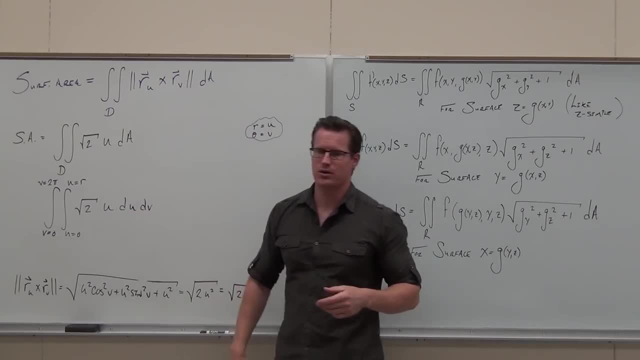 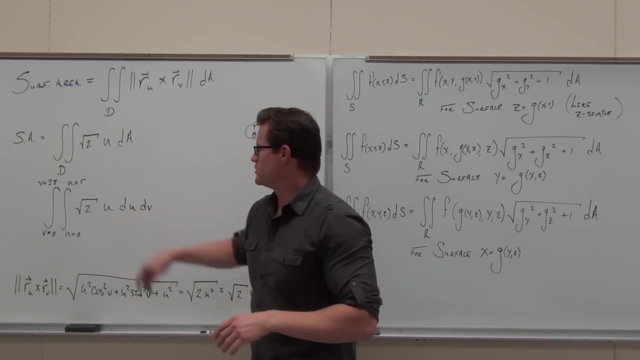 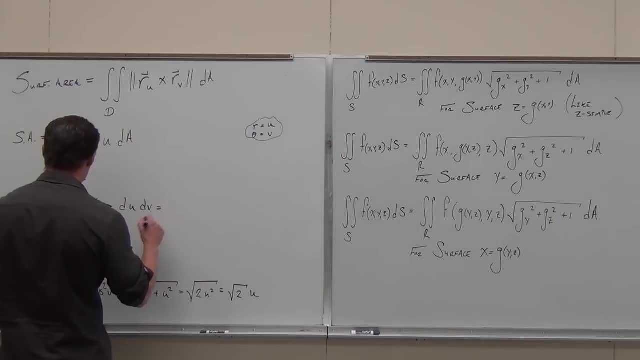 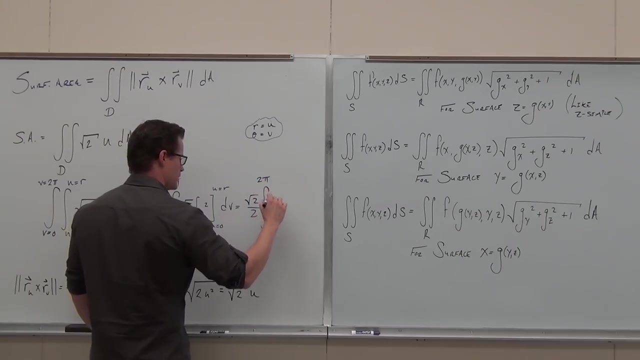 did not too bad. let's see we'd. uh, yes, we could do this one. yeah, I think sort of works. right, this is up. looks like we got our square DB now. wait a minute. I thought that we couldn't end with with with a variable R. but keep in mind, keep them. that's why we chose you instead of. 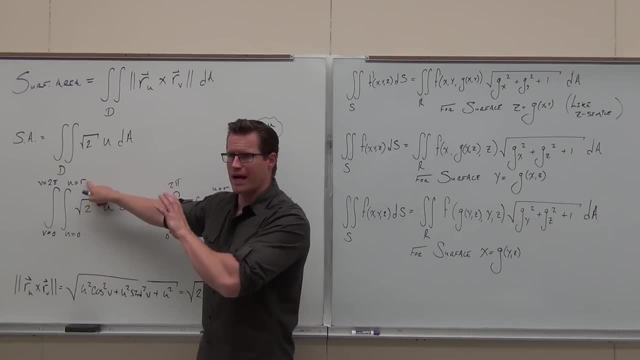 our. if I want to go from zero to R, I need to plug in R for a different variable. this is very well, could have been a constant is a constant. I'm just getting to plug in the constant later. do you guys see why we chose you instead of? 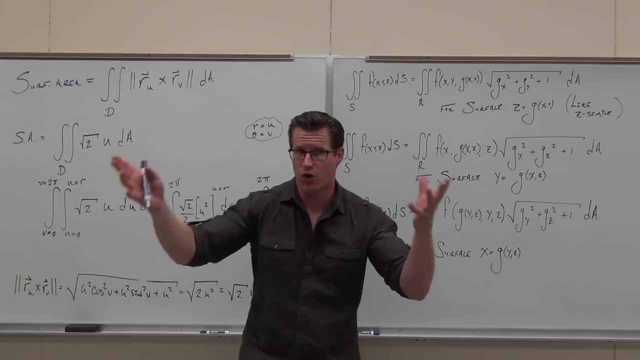 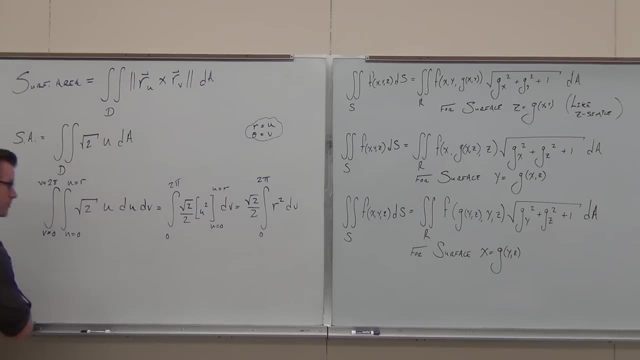 R. we allows us to plug in R into something that's not R and get a formula for this with respect to R. so DB would give a us. well, just V, this whole thing. V where V goes from 0 to 2 pi, okay, well, what's that? 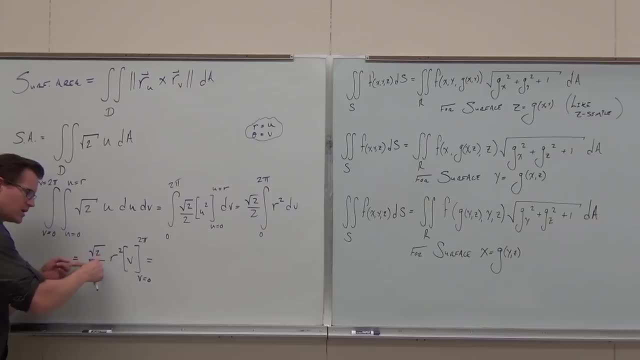 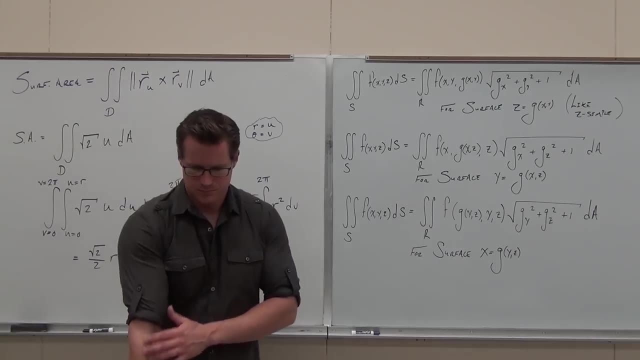 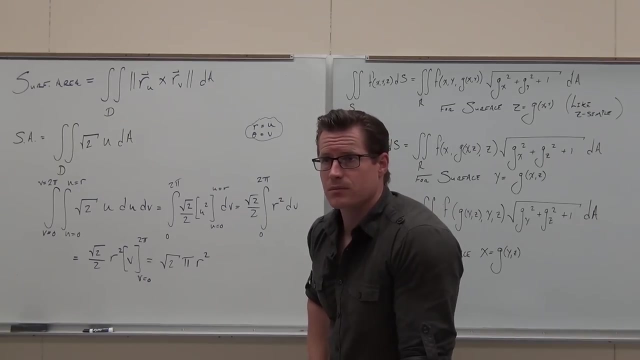 what's that mean? but plug in 2 pi and spread 0, I get 2 pi. 2 pi times 2, that's just giving us the square root of 2 pi. R squared, but not 1 pi, is the speed of 0.. oh and plus 1 pi degrees of What is 1 pi degrees. 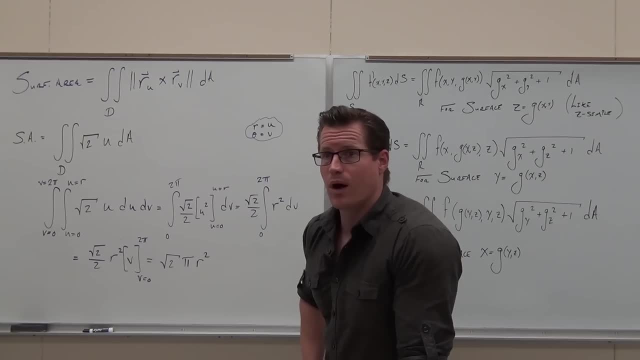 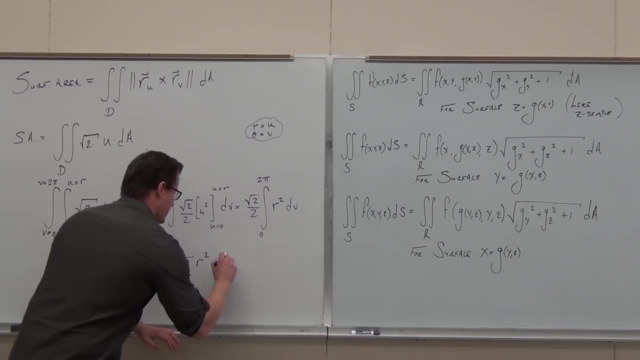 of star for 1 pi. I'll give you the answer. are you good with this? That's correct. yes, I, amalal. I would have knowngio, if you're okay with the math behind it. now, what is it? Is it mass? Is it mass? No, What is it? 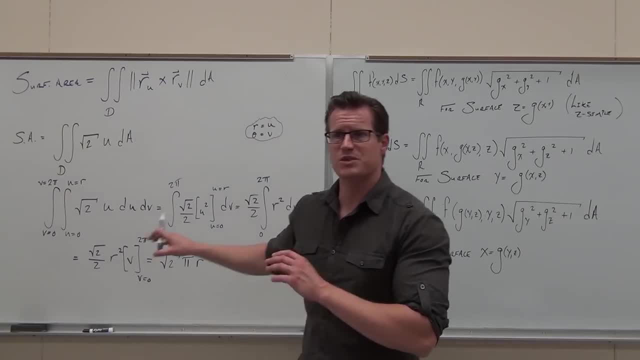 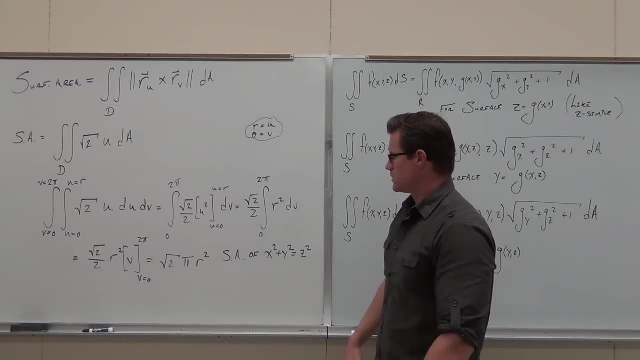 surface area of what Of cone? This is the surface area of the specific cone. Does that make sense? For however far I want the r to go Now, what if we do it a different way? How about this? Check this out. 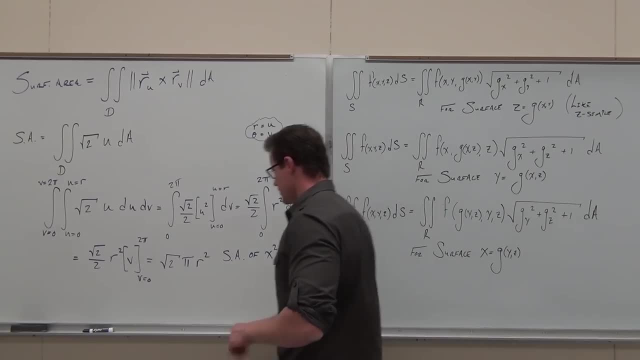 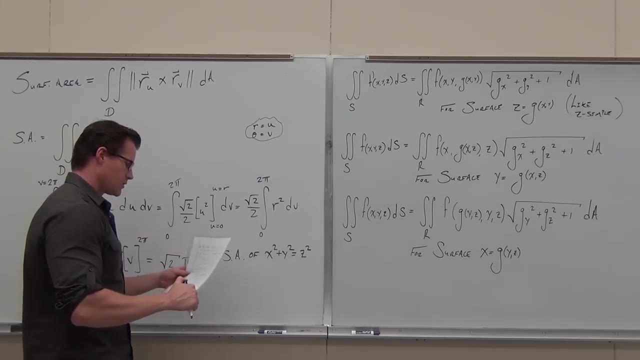 If that's a cone, and I go well if I let this equal r squared, which I'm going to do that. So I want you to check Here. watch Now, if you look up surface area of a cone, like Google it or something, you get that. 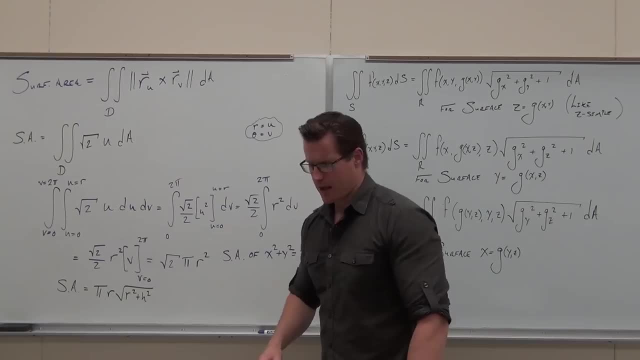 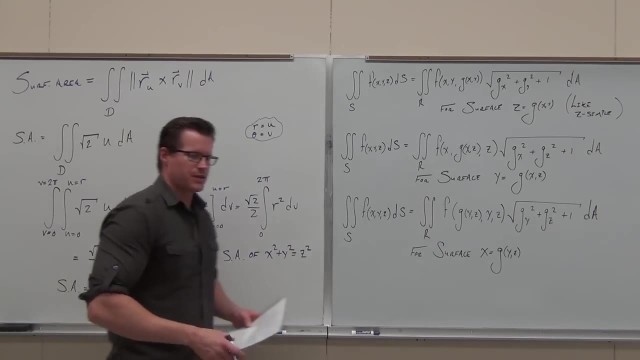 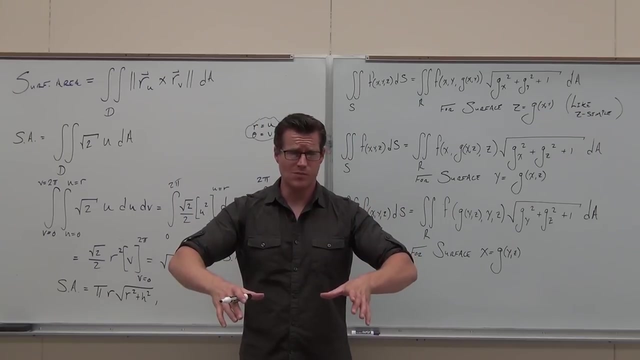 You get something like that. Okay, well, how does that relate? Well, I'll show you If I think about this cone. this cone is along the z Axis. Are you seeing what I'm talking about? That means that z is the height. 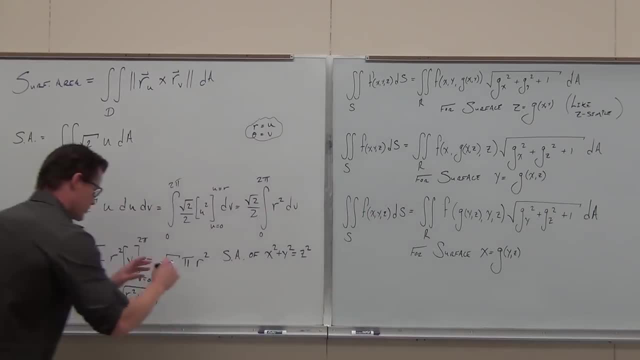 Z is h. Are you following that? Okay, so z is h, But wait a minute, Z is also or z squared. I guess is also x squared plus y squared. So if z equals h and z also equals the square root of x squared plus y squared, 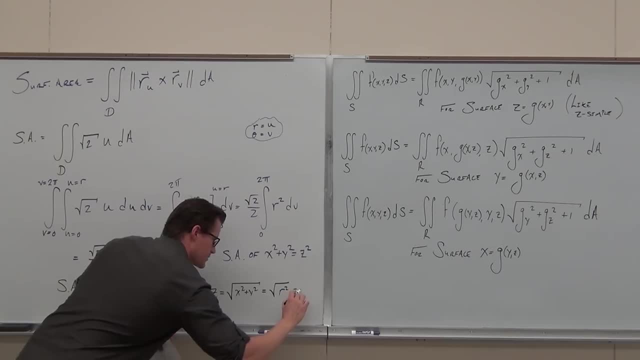 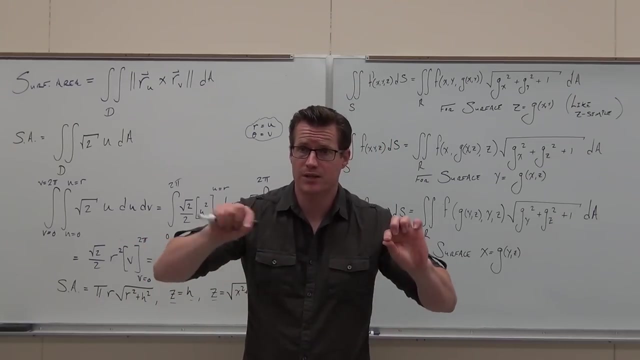 then this is the height And this is the square root of r squared, and this is r. If z equals h and z equals r, then for this particular cone, h is the same as r. It's like a cone that has the slope of one. 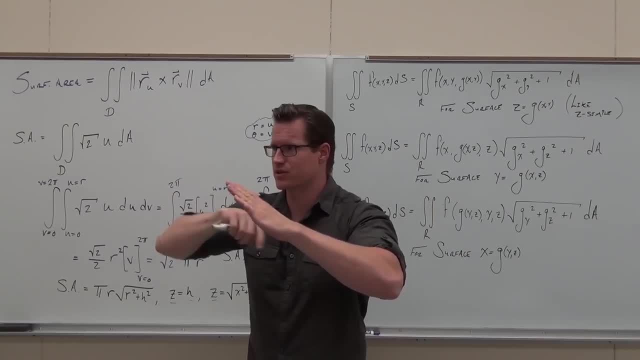 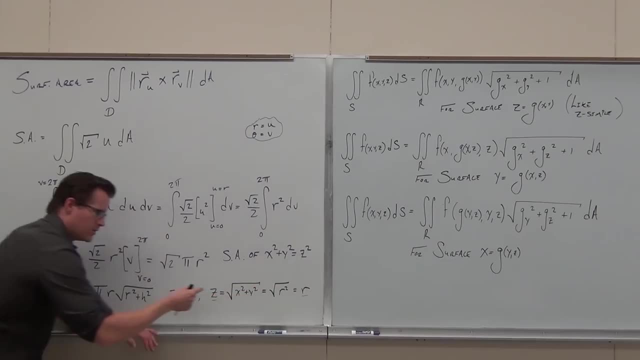 It's making like a square. That's basically how, again, the diagonal would make a square out of it. So for this particular cone, if z equals this and this equals r squared, then z equals r. But if z equals h, 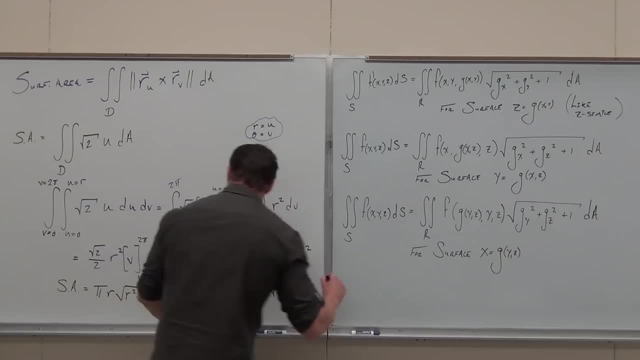 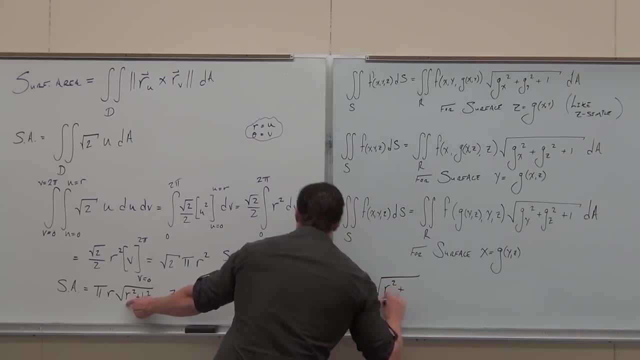 then h equals r for this formula- I'm going to move over here for just a second- So from here we'd have r squared yes, h squared no. Since h is z, z is r, that would be r squared. 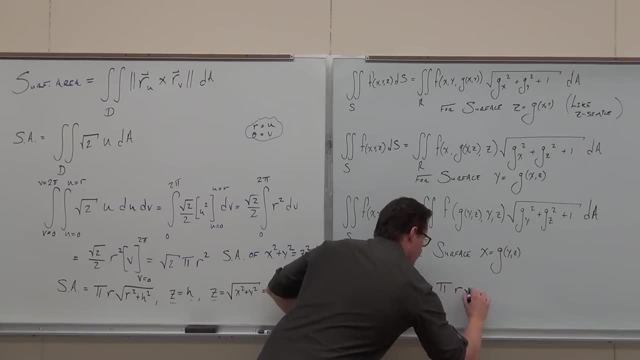 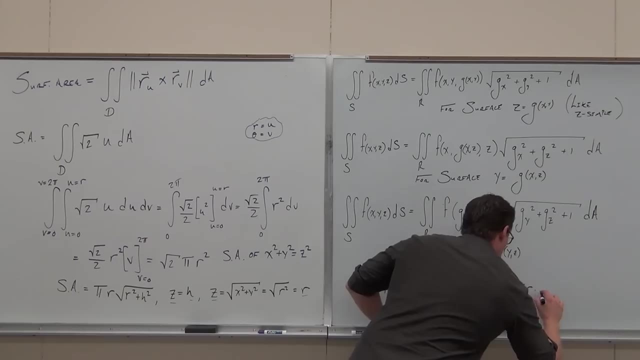 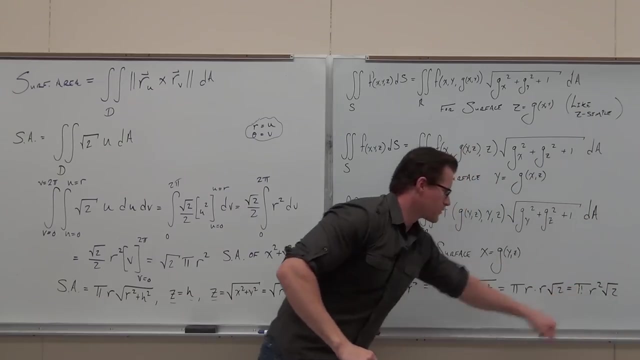 No, wait a minute, That looks pretty nice. Pi r squared root of 2r squared. Hey, what's the square root of r squared? Well, it's r. I'm going to move over here for just a second Surface area of this cone, where z is the same as r, z is height. 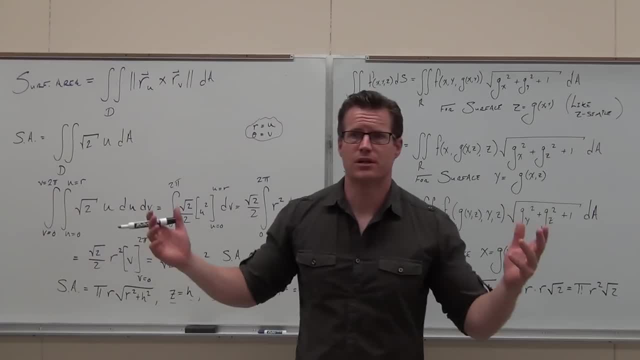 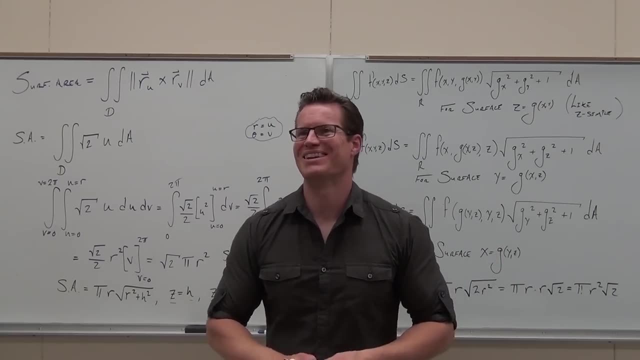 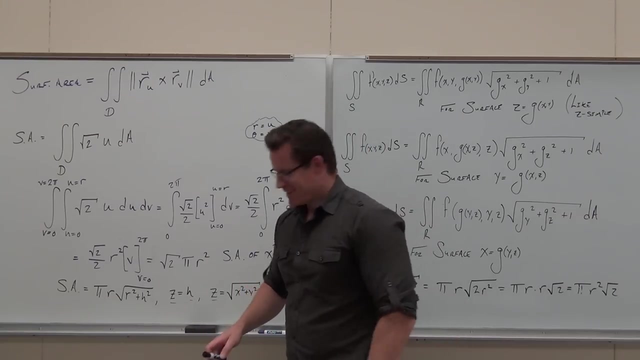 Surface area of this cone where z is height. Same surface area Done, geometrically Done, calculacy Done. either way, That's funny. Come on, lighten up. It's too stressed out. Take this stuff too seriously. I just wanted to prove that this was a good formula. 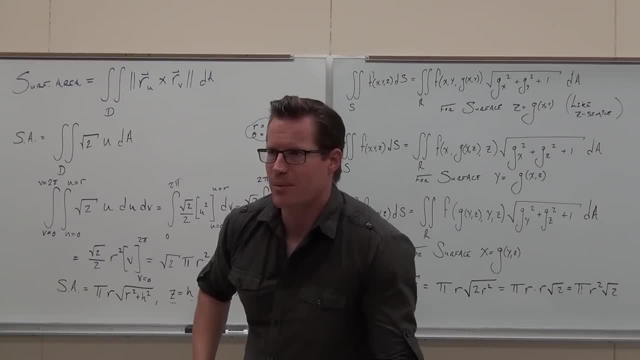 I'm going to go back to the table here. what we're actually doing. okay, this is. this is real stuff. it's not fake stuff. I'm not making this up- you know which? I could make it up and freaking awesome. I've only done that one time. okay, it was a fake lesson. I got really in trouble. 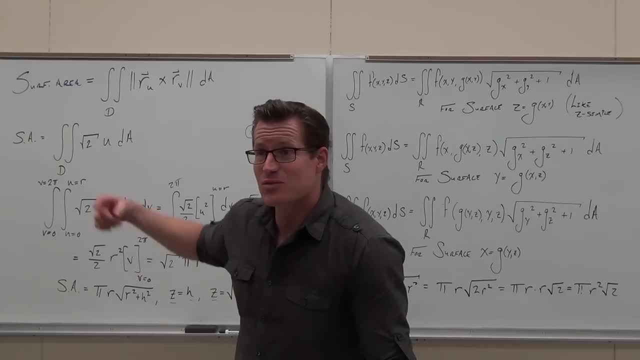 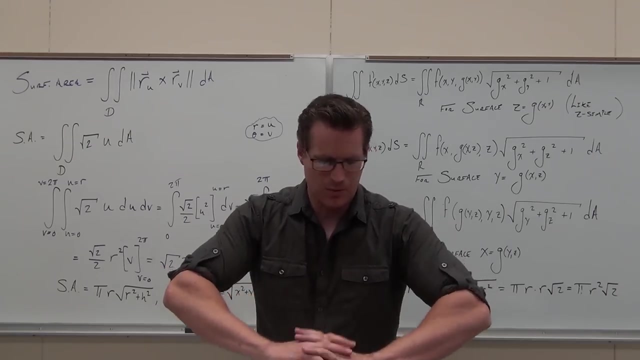 for doing it. never do it again. but this is real. it actually makes sense with geometry. it's it's analytic geometry. okay, sorry, yeah, we're doing geometry, calculus wise. I'm gonna leave you with one thing: that we're come back and do an example now. you know what. we'll take a break now, because I think we need one. 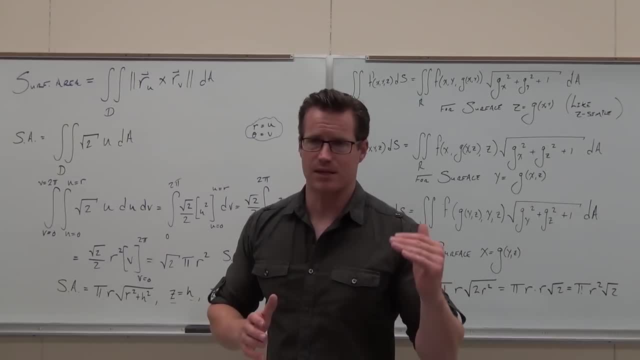 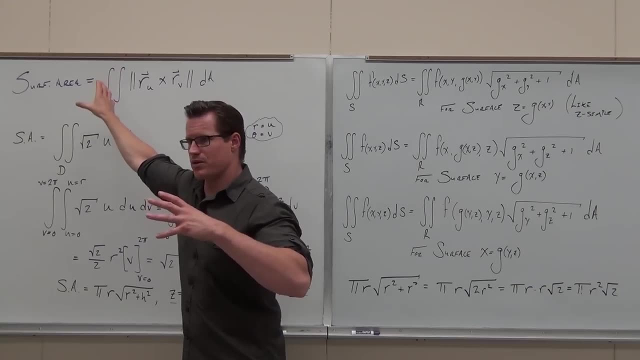 really let our heads get refreshed a little bit. we'll come back and we'll say this, and I've already said it: if I can do surface area with this, I should be able to do surface integrals with this by just putting in a what here: yeah, I. 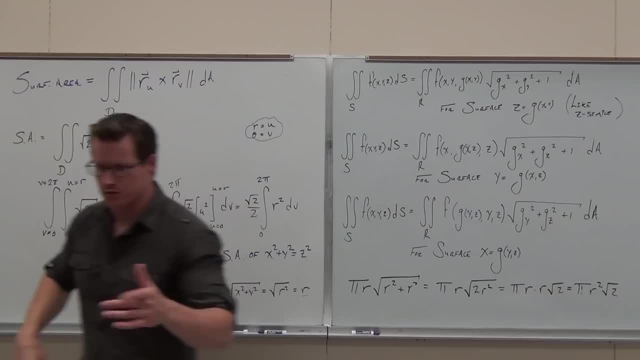 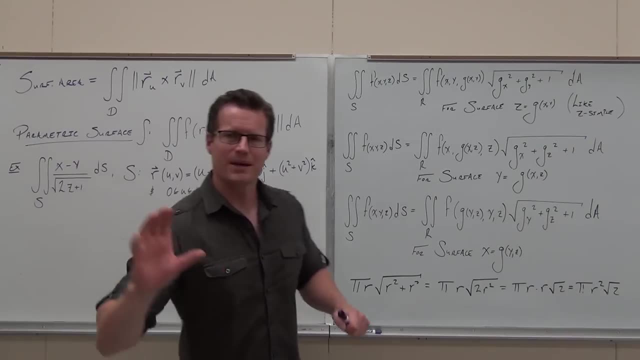 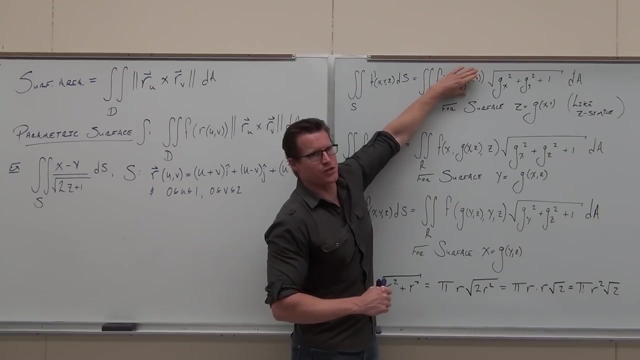 should be able to find surface integrals, to find the mass of this surface. we'll do that later, okay, so hey, you know what we're gonna make. the jump right here. what I told you before was: the only reason I left on the board was if this is 14.5 version of surface area, which it is, and this is our now. 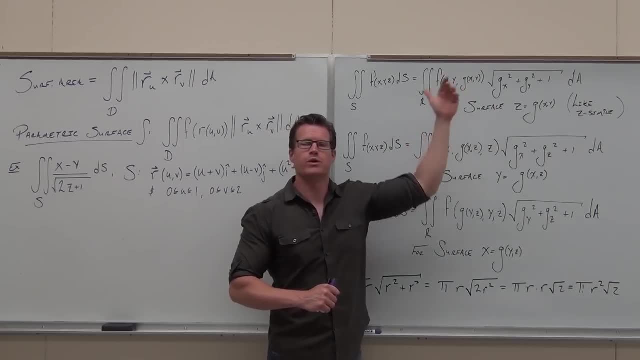 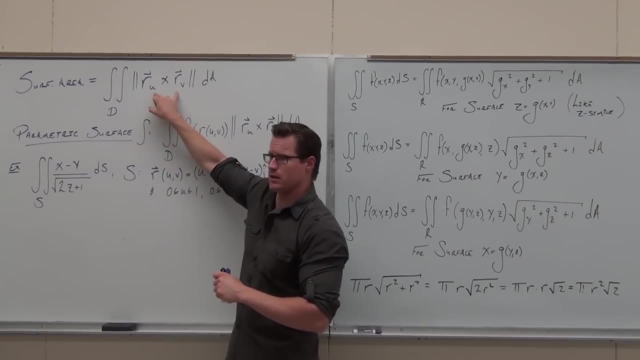 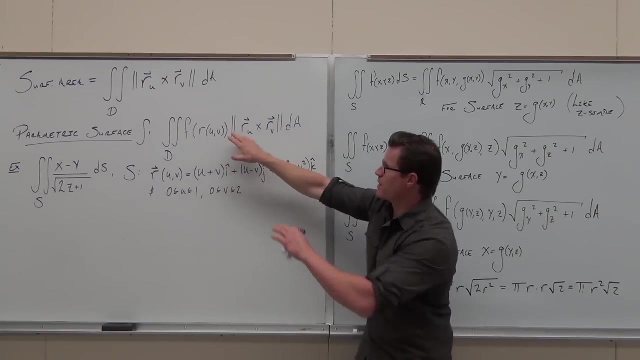 surface integral, where that's a mass density function, then we should be able to make the jump here. if this is surface area of the surface parametrically defined and we just take and put a mass density function right here that we have surface area, the idea is that we should be able to make the jump here. if this is. 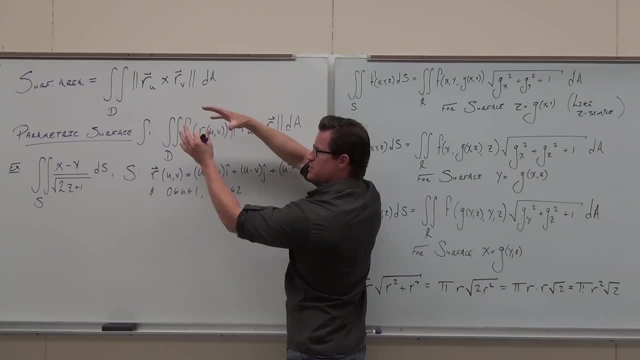 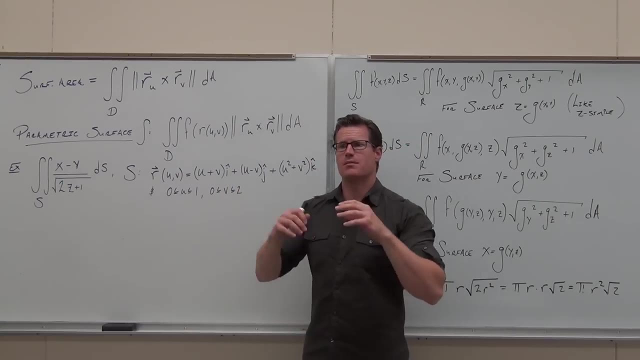 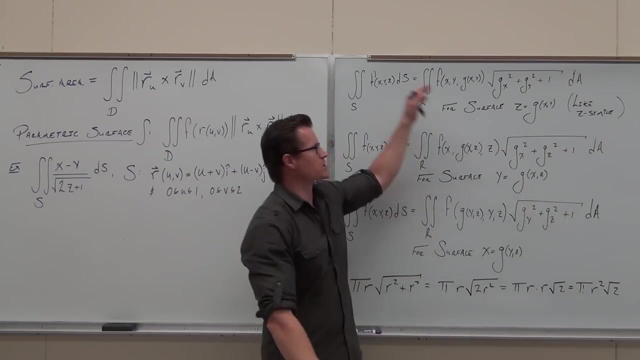 surface area of mass at every point across the surface and add it all up and this should give us the same thing that this does, which gives us mass of a surface. if that is the mass density function, so it has to be okay with that one. so, just like we've done surface integrals before, now we should be able to: 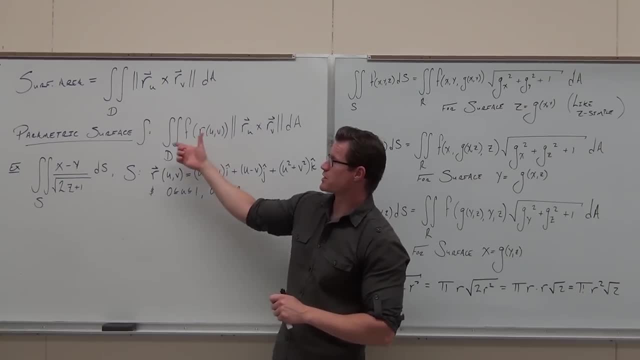 do them parametrically as well, and that's what we can do. so parametric surface integrals look just like this: do the exact same thing as you would do for surface area. it's just now. you also have to. you know, man, that looks a little weird. 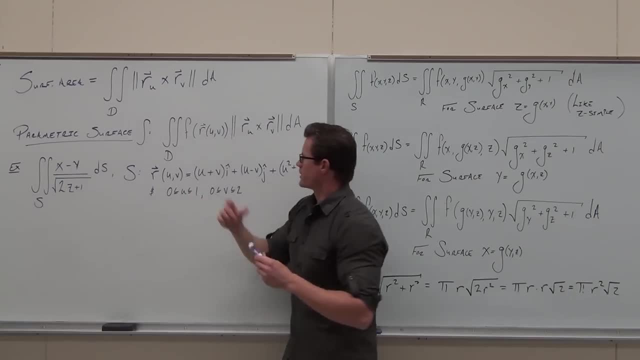 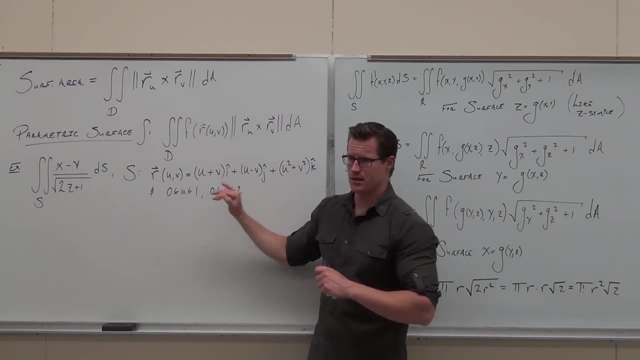 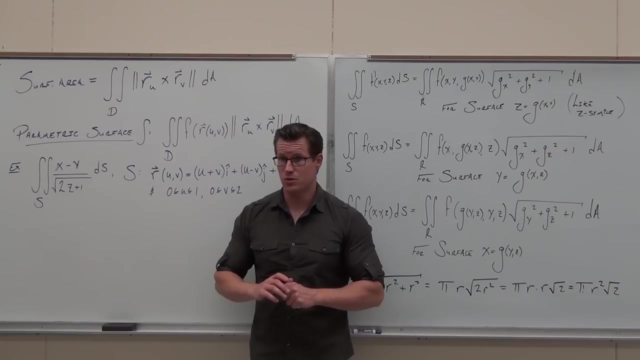 well, sorry, that looks a little weird. well, that just means that you're redefining your function in terms of the pieces that are given to you right here, and not if you're okay with that one. now I've given you kind of an easy example. someone- and it's not generally easy to do someone- has already defined your. 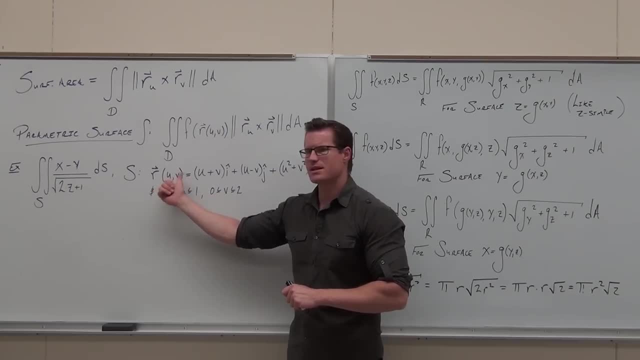 surface. look at this. look, do you guys recognize? that's a surface. it's a vector of two variables. it's giving you a surface there. this is a surface and someone's given it to you. they're also giving you the domain for u and v. that's. 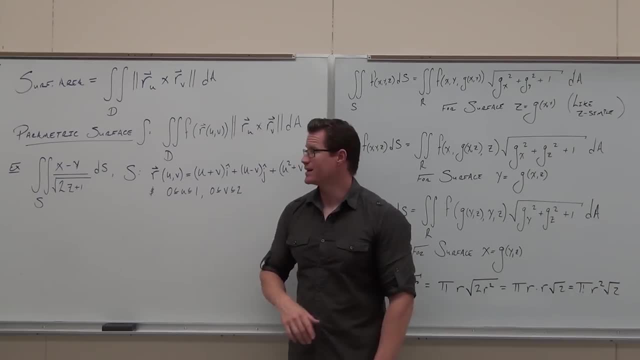 really convenient. here's what I want you to do. firstly, recognize you are going to have to change all of your variables into u's and v's. do you guys see that you're gonna have to do that? so right here, you're gonna need to find out what. 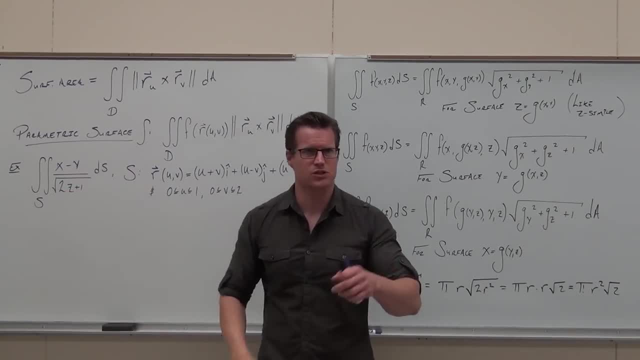 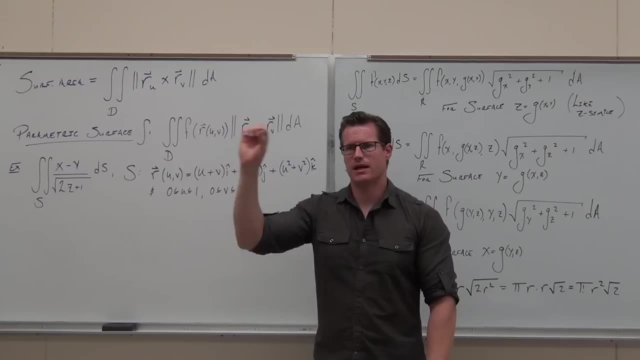 X is what Y is and what Z is. so if, if you're given a surface in terms of this parametrically defined surface or a vector function, I want you to just write above them, write what X, Y and Z are. that way we can make a little. 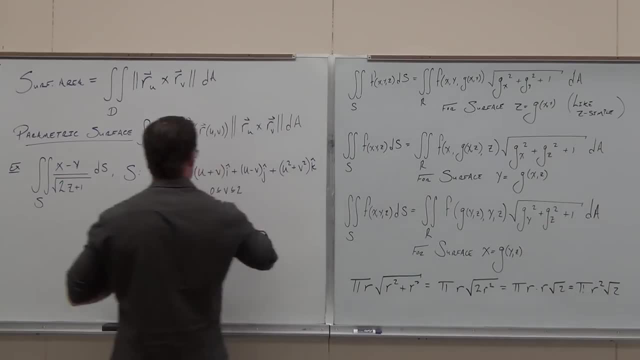 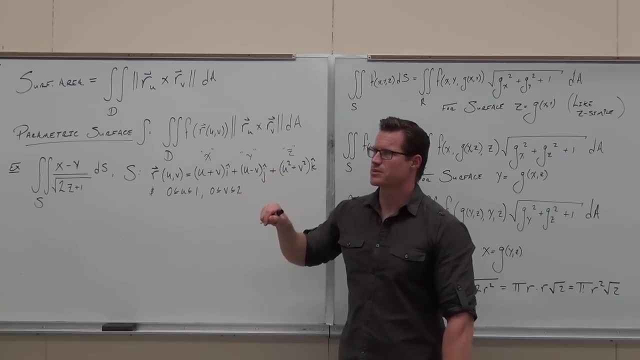 substitution later. so what's the X thing? and this is Y and this is Z, you guys? okay with that one? then we just run through the formula. what we're gonna do here is: well, now let's, let's be real careful. is this the surface? no, I'm not. 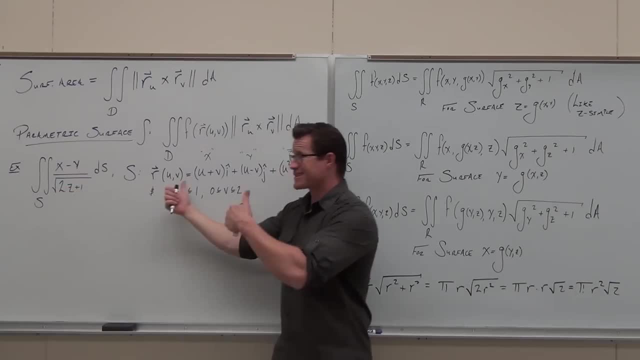 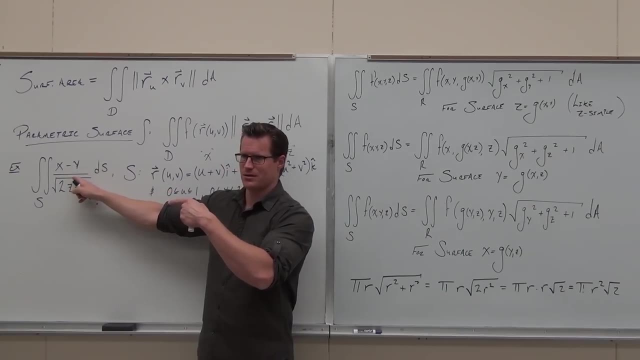 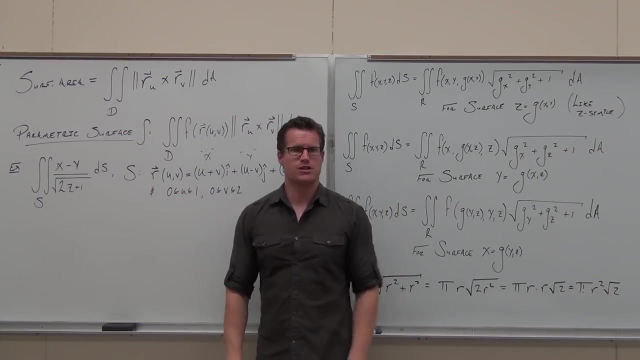 I'm trying to kind of see if you're with me on this stuff. that's the surface guys. what is that? if this is one, if this is one, then this formula gives that thing. does that make sense of what I spoke about earlier? if that's one, then we just get surface area. 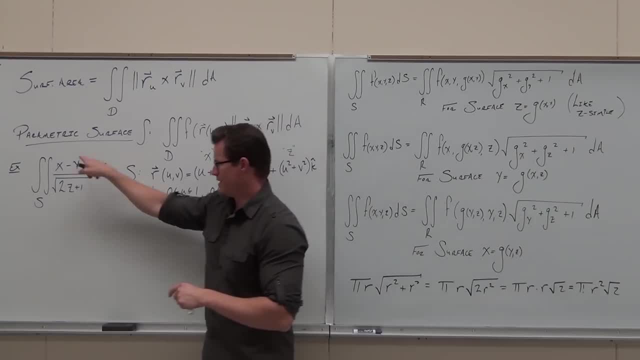 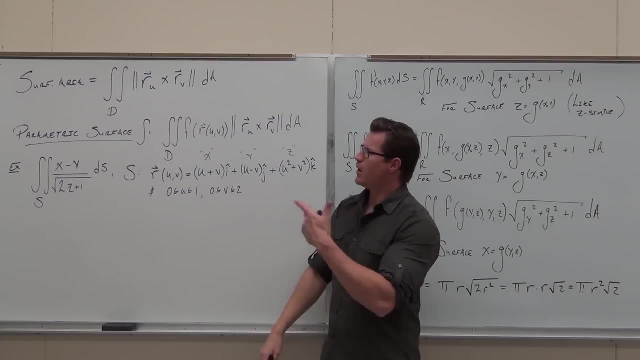 if it's not one. that's a function based on what the points are, so this all has to change. this stuff based on X, Y and Z. we also need to still find this in the formula. so how I would start this: I start with these two things, so find the. 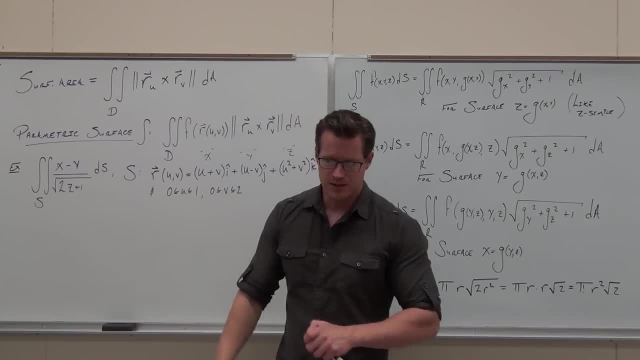 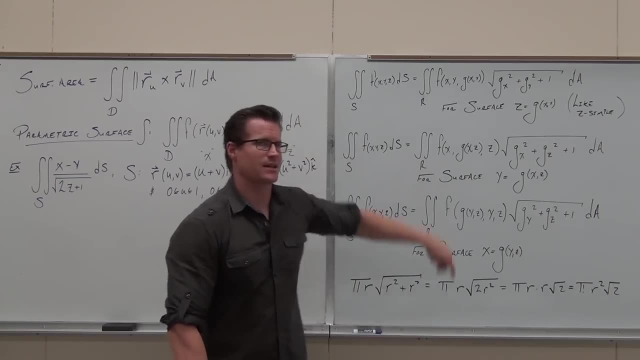 partial derivatives. cross them, find the magnitude. that's a what i want you working on right now. about every 30 seconds, i'm going to put a step up on the board. it's going to take a little while i'm going to erase this, since i made my last connection to 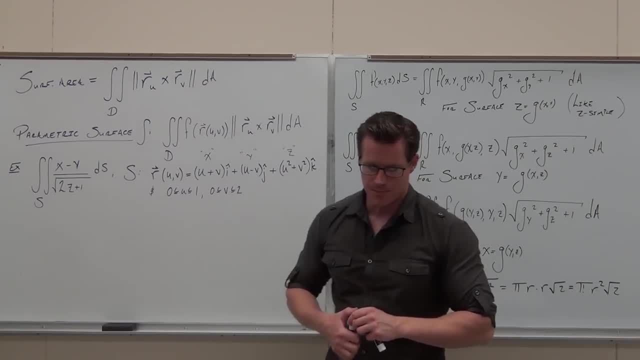 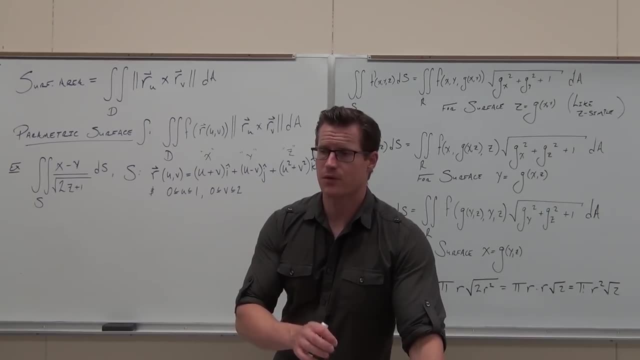 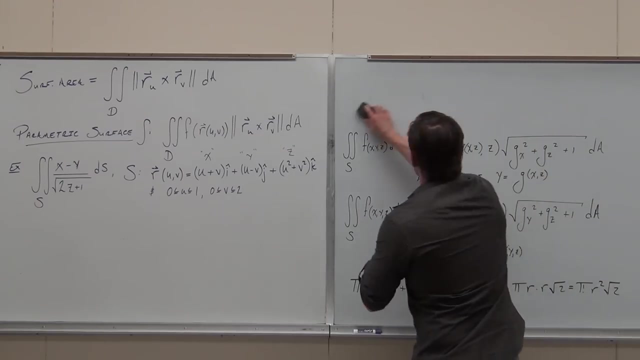 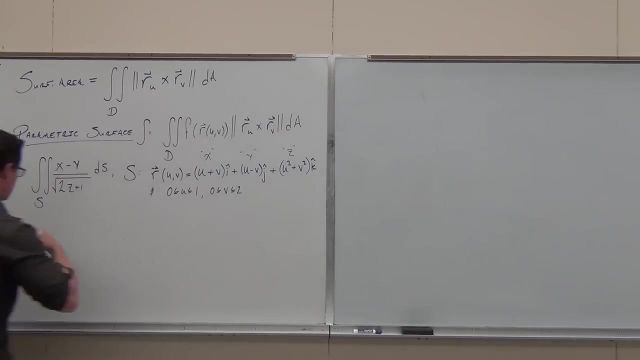 it. i'm going to start working mostly on that side. so i want you doing- doing just two things right now- i want you finding the partial derivatives and crossing them. if you've made it that far, then i want you to start working on the magnitude. okay, so 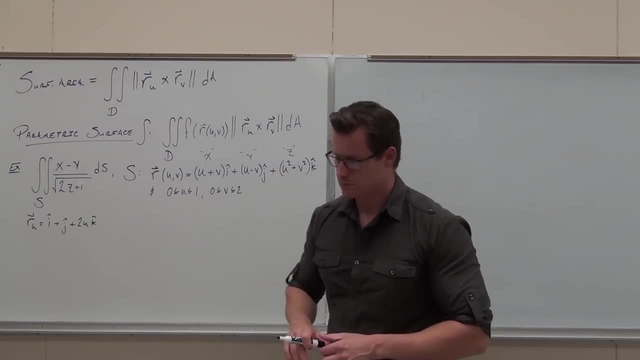 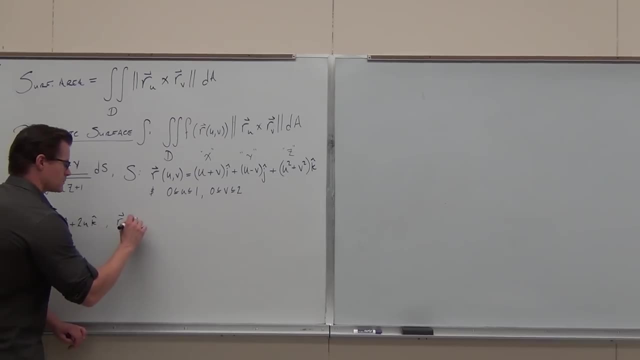 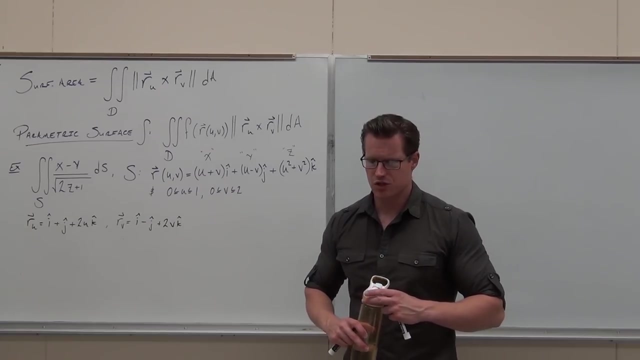 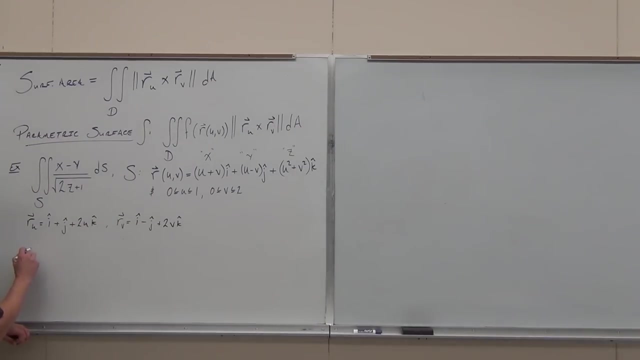 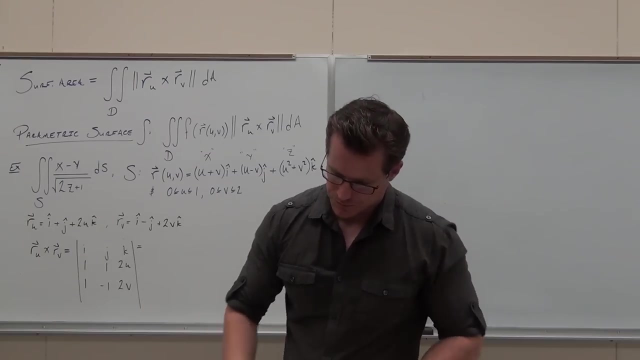 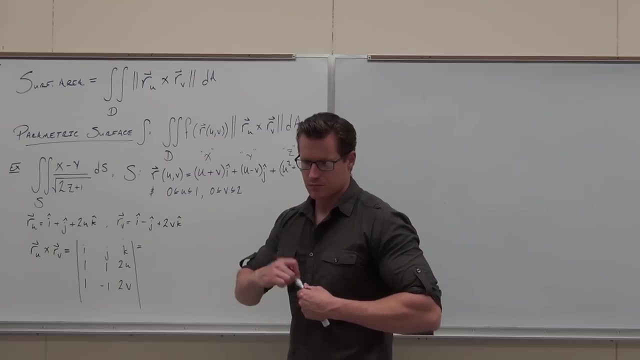 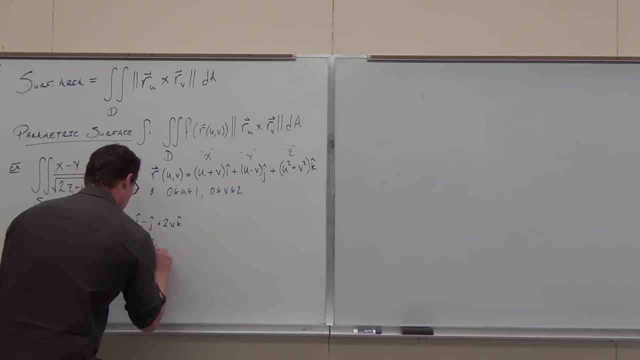 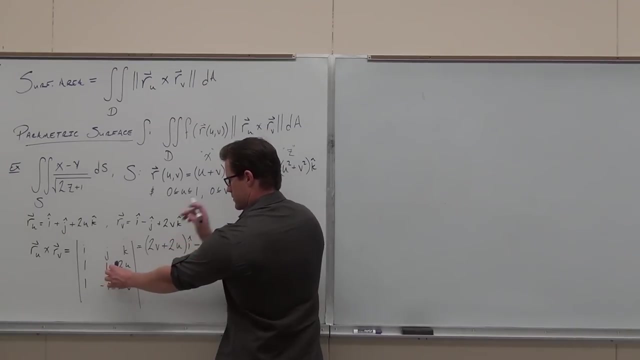 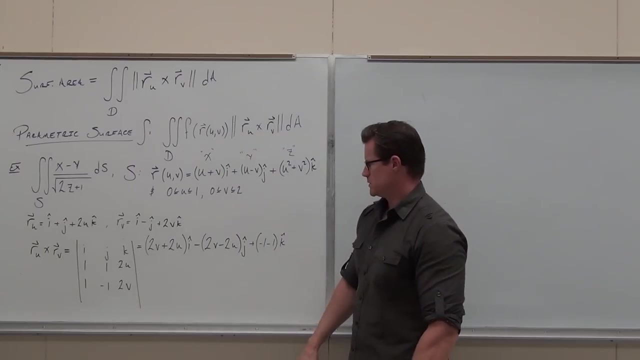 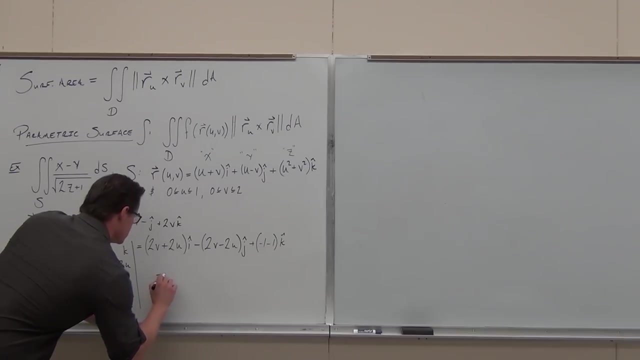 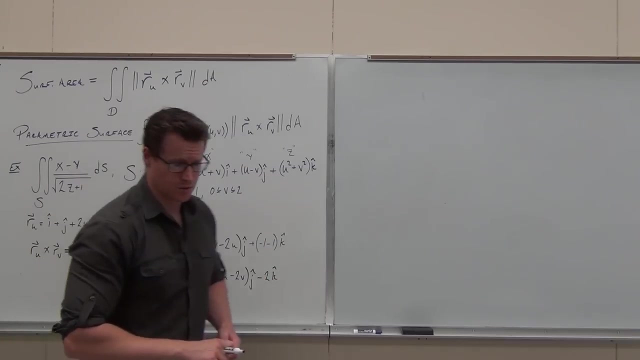 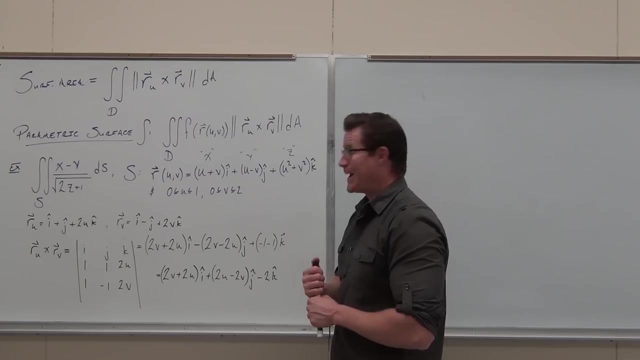 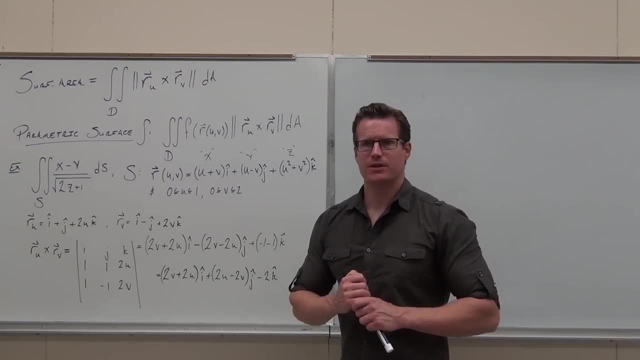 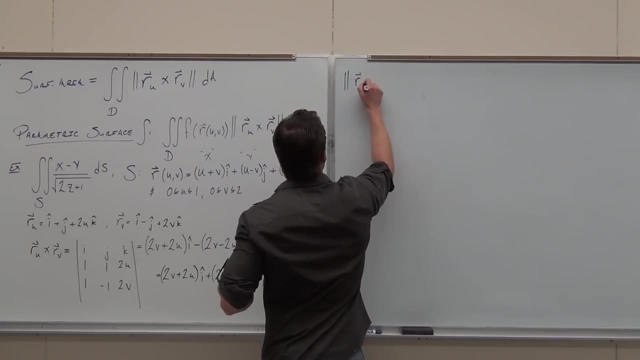 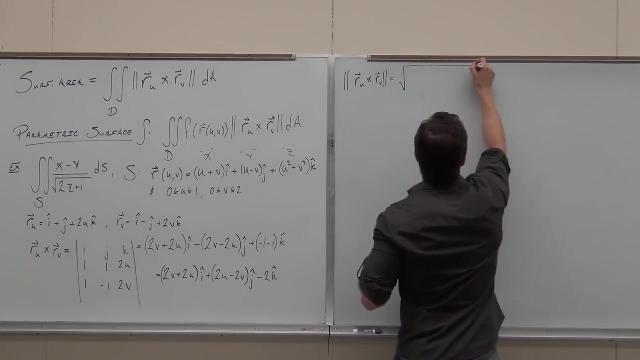 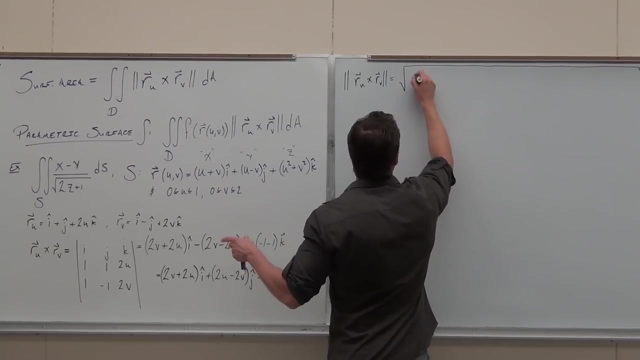 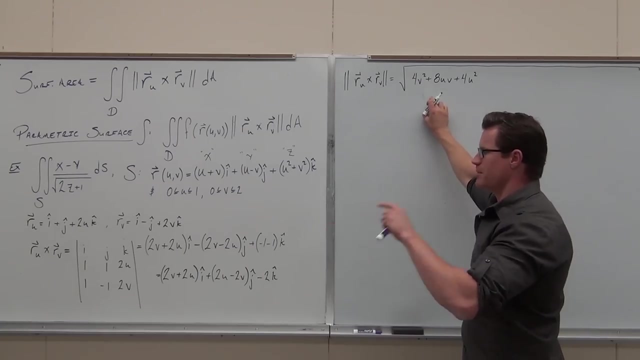 Magnitude, magnitude, Work on the magnitude. That's what I got for the x components squared. So we square them, we add them and we square root them. I got that when I squared that thing. Can I get a double check? 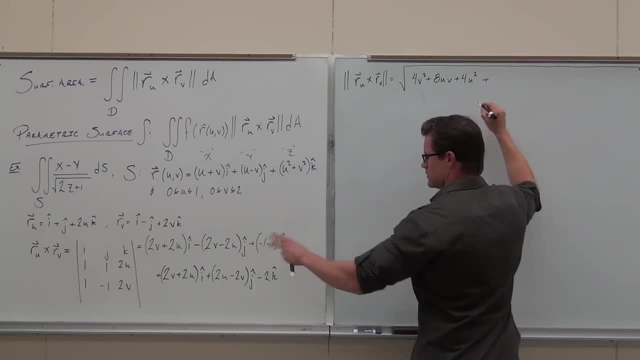 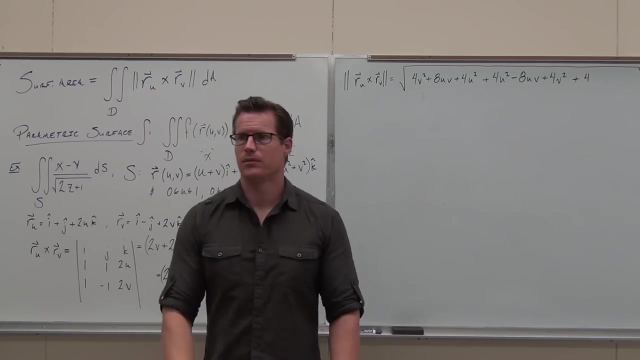 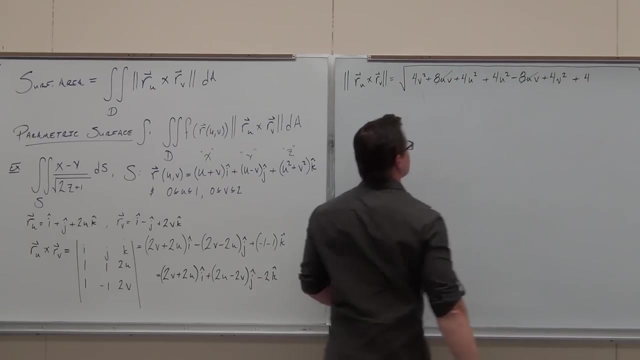 Did you get the same thing? I got that when I squared that, And just 4 when I squared that, And I don't know if you're okay with that one, What now? Simplify a lot of stuff. 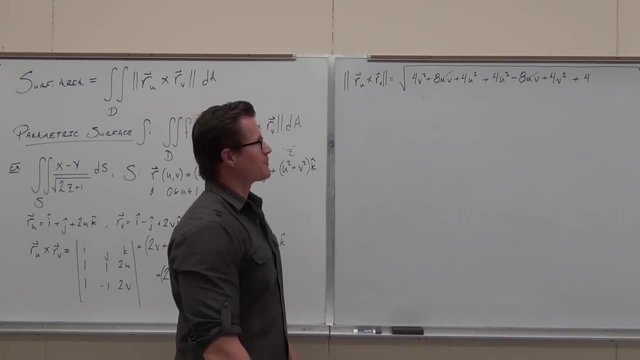 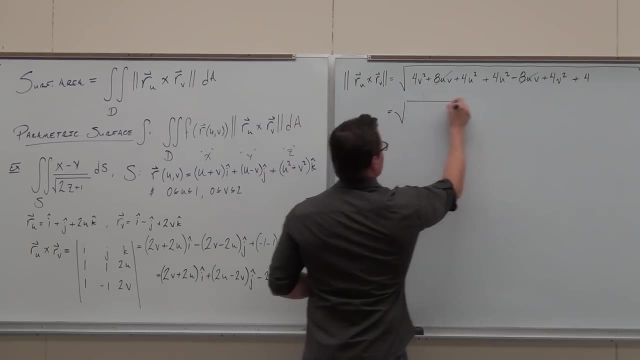 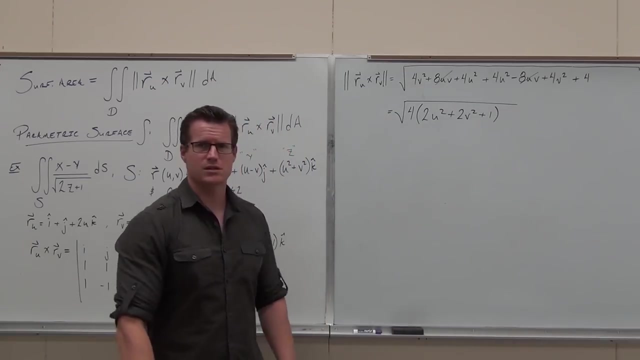 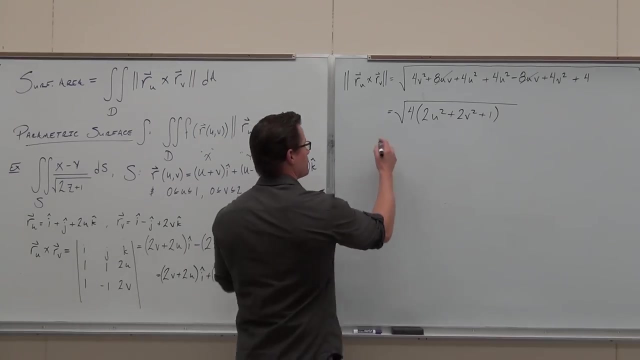 Also you know everything's got a 4 in it. Just factor out that 4.. If we factor out the 4 from everything we get. 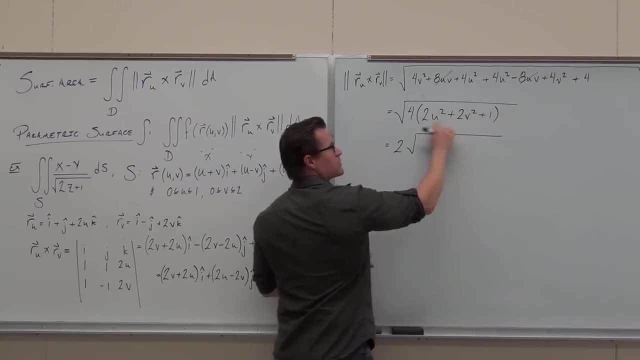 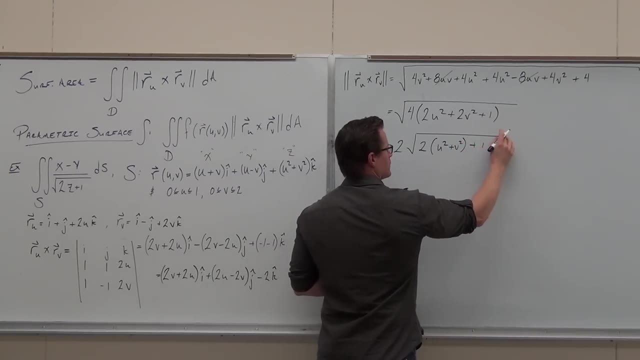 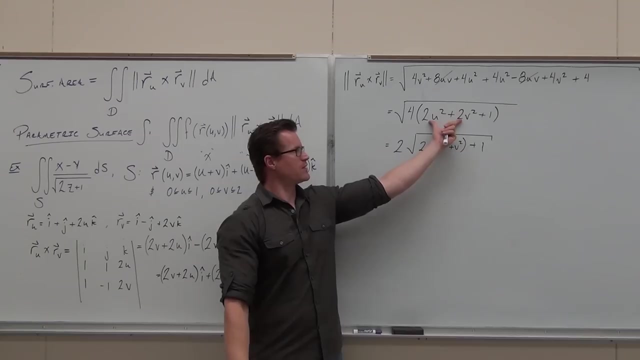 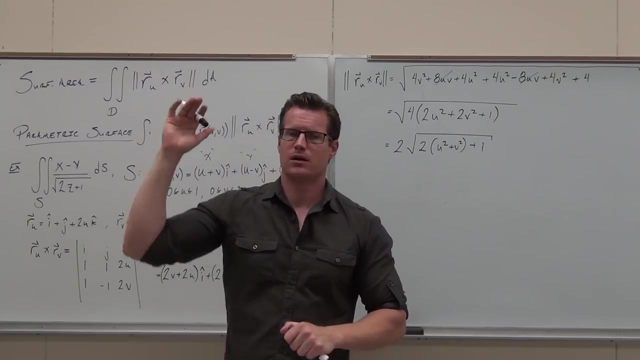 Not that one. so we have this: 2 times the quantity of u squared plus u squared, and then plus 1.. So if we can follow the algebra on that one, what now? 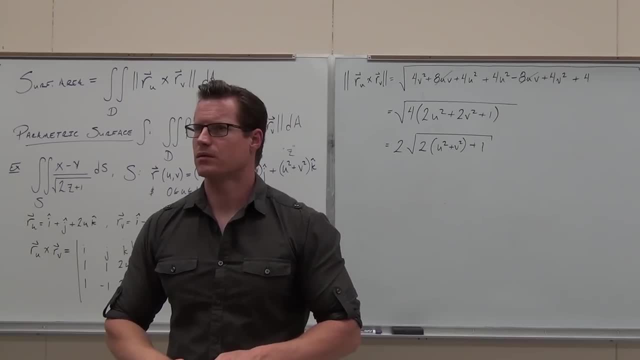 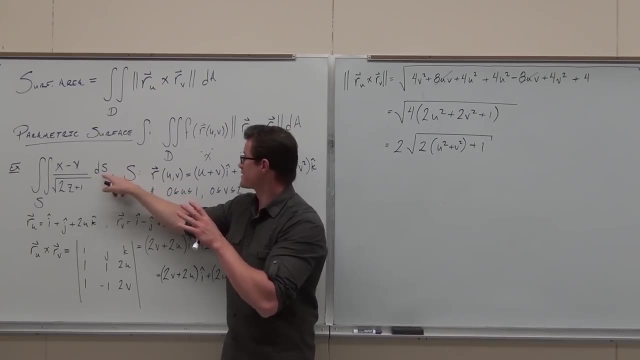 What now? What do you think? Well, what have we done? We're trying to figure this out, right, We're trying to figure this out. What we've basically done is just figured this Right now. this is this part. 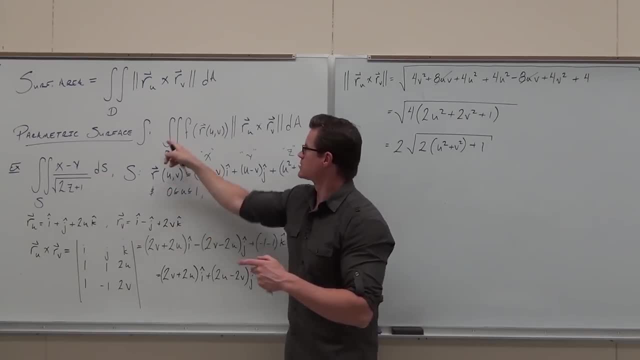 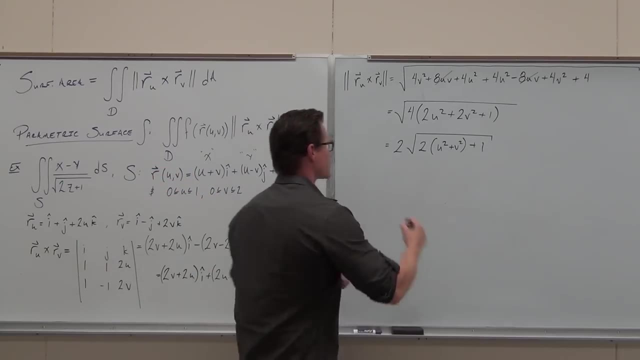 Surface area: surface area. That's basically it. Let's start setting this thing up again. Don't worry about your region, your domain, right now. We'll deal with that in just a second. Right now, I want to see your setup on your double integral. 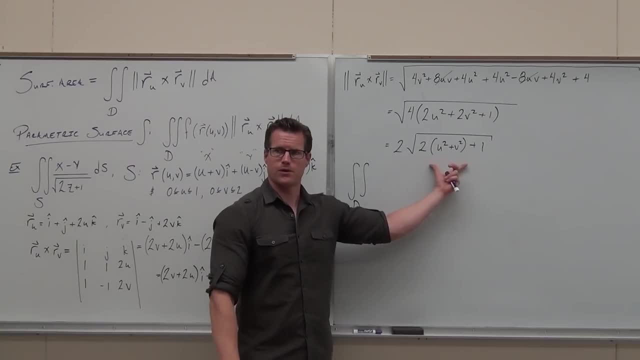 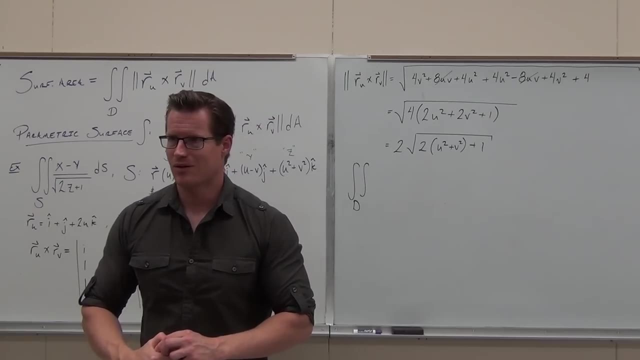 Start with this first. Change this stuff accordingly. I'm going to give you about 30 seconds to do that. Are you guys okay with what I'm talking about? What needs to happen to all the x's, the y's and the z's? 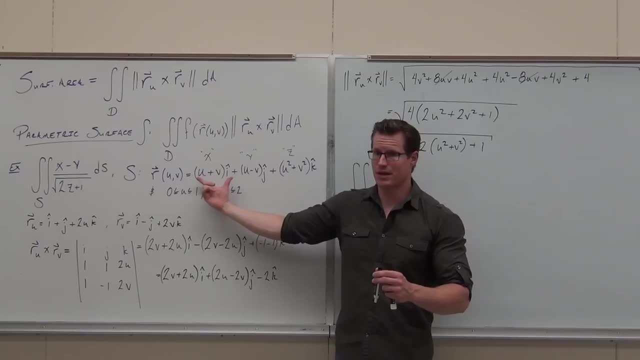 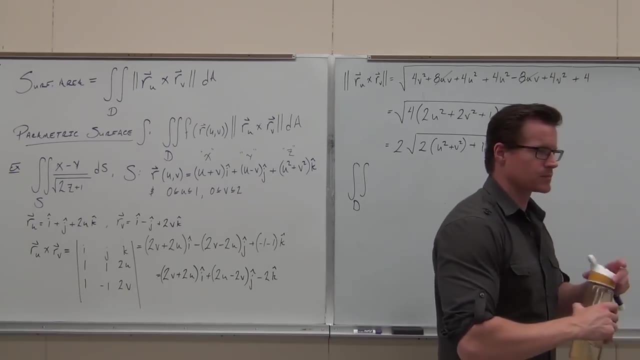 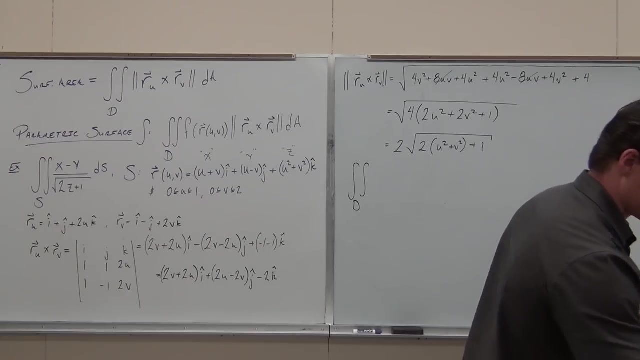 We've got to be using v's. Can we do it? Thankfully, yes, Okay, Come on. come on, try it. If you haven't done it, try it. You've got to try it. Come on, you got to do it. 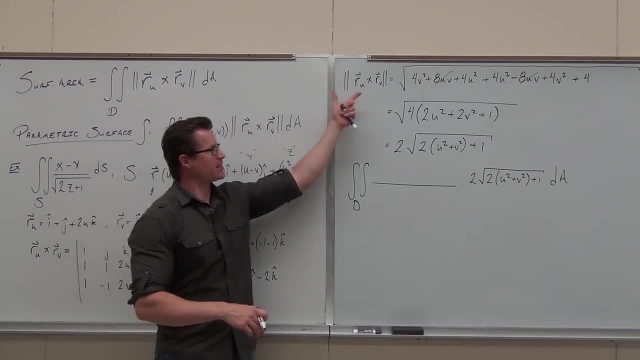 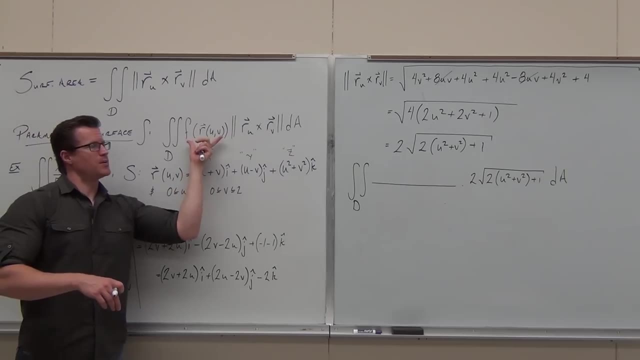 Okay, So I got this. I found the cross product, I found the magnitude. We simplified as much as we can and we have it right there with the d8.. That's exactly the same thing This piece, this says: look at the mass. 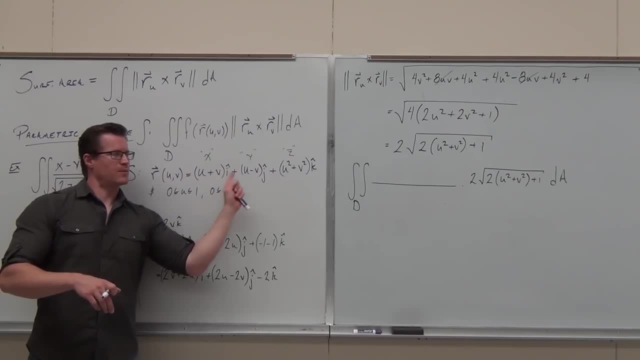 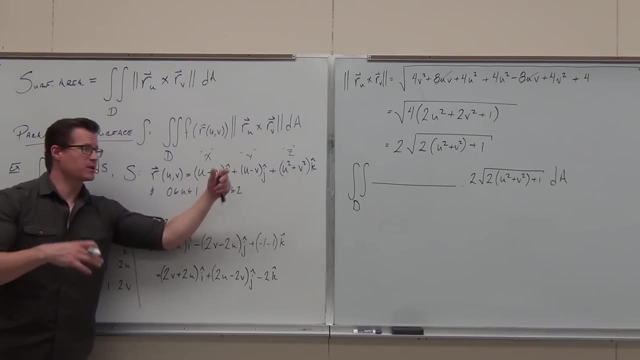 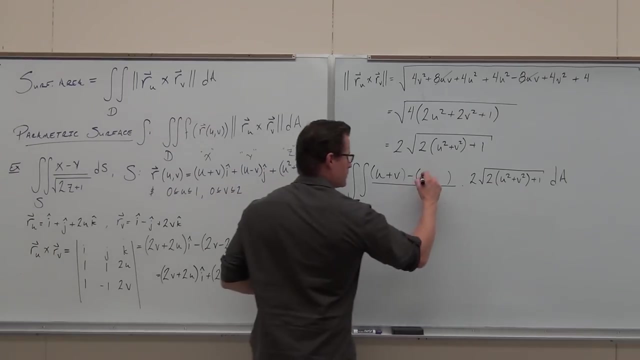 density function and x's, y's and z's. use your parametric surface to change it. X becomes this, y becomes this, z becomes this. every place you see it. So in our case we have x minus y over nasty square root. the 2 doesn't change, but the 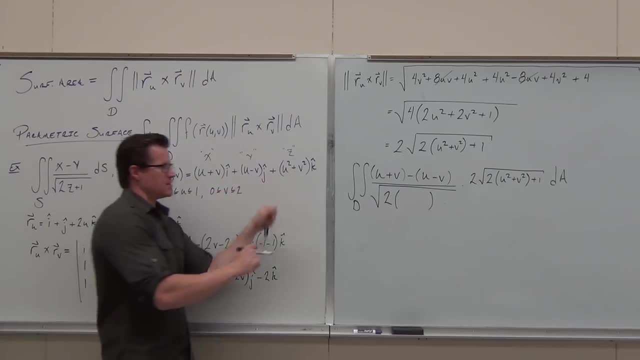 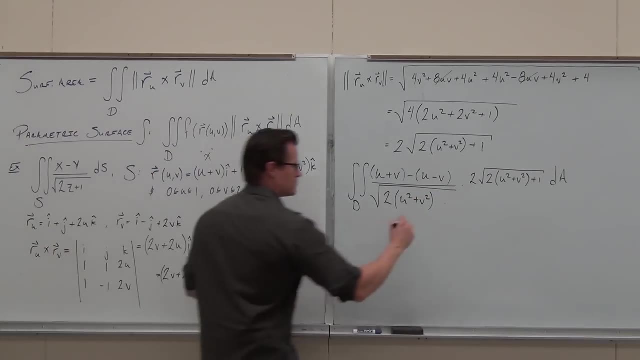 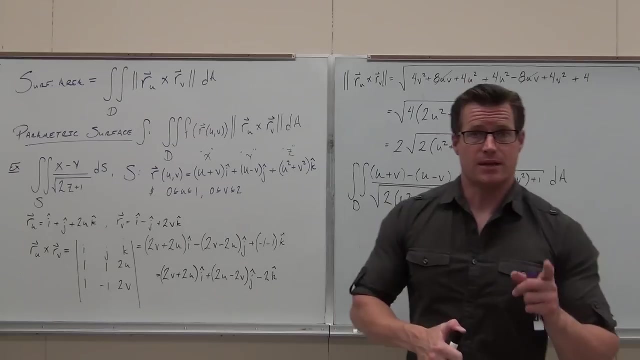 z changes 2 times z. What else? Hey, I want to see if you can make it that far in your minds right now. Can you guys see where all this stuff is coming from? Why are we changing x's and y's and z's again? 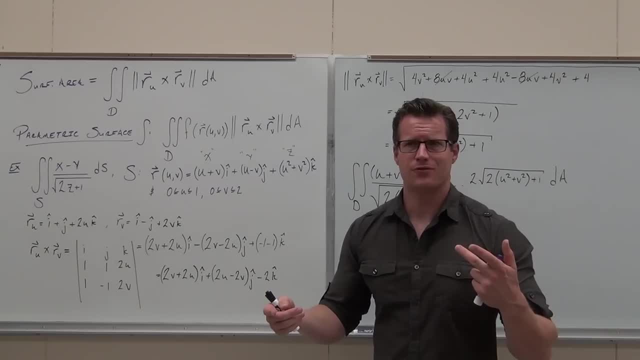 Could you even do the double integral? if I didn't do that? We have like 5 variables. We have u's and v's and x's, y's and z's. That's crazy. So we're using our parameters here to change our. 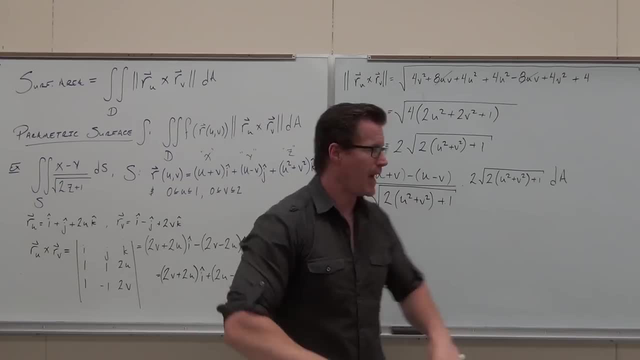 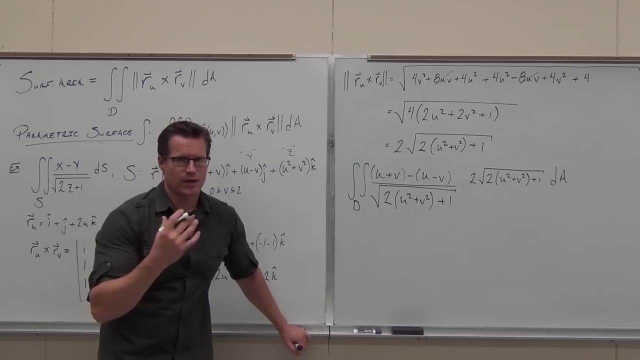 our mass density function. That's legal, It's on this surface anyway. We're talking about that. What now? What could you do now? Simplify it before you even worry about your region or your domain here. So this is gone. 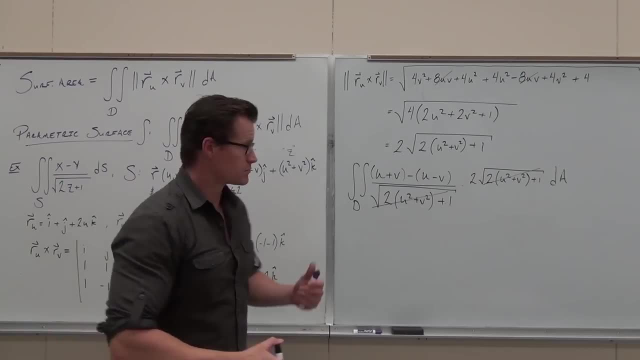 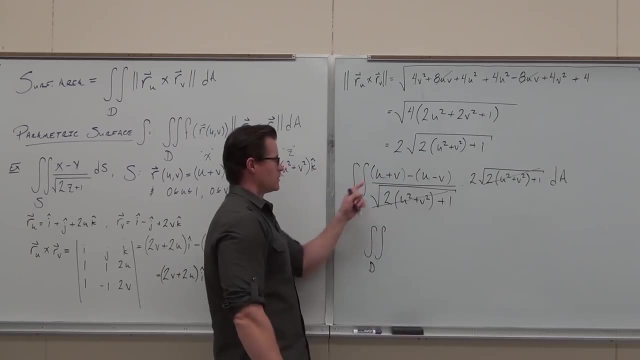 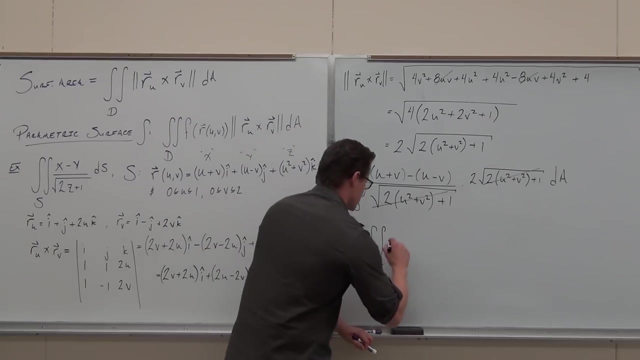 Tell me what else you could do, So this all becomes: u's gone, You got 2.. You got 2.. You got 2.. You got what 4v? That looks a whole lot nicer than what we just had. 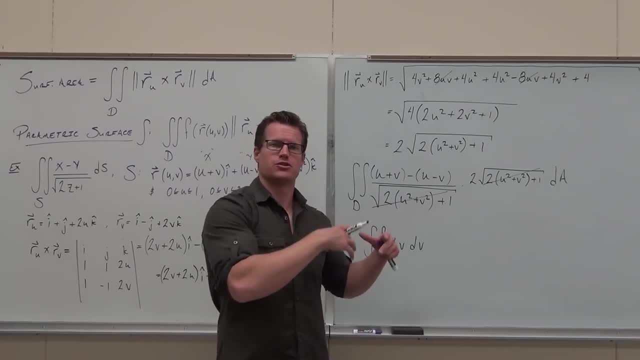 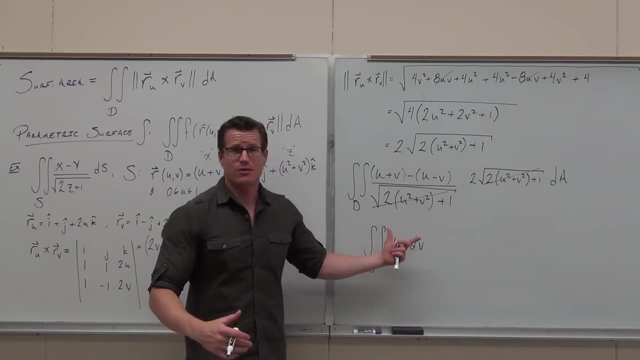 A whole lot nicer Now. now go back and fill out your double integral. So all this stuff, all of this is just setting up your double integral. That's what I'm talking about. This set up is the most important part. Once you get this, you have a very simple region. 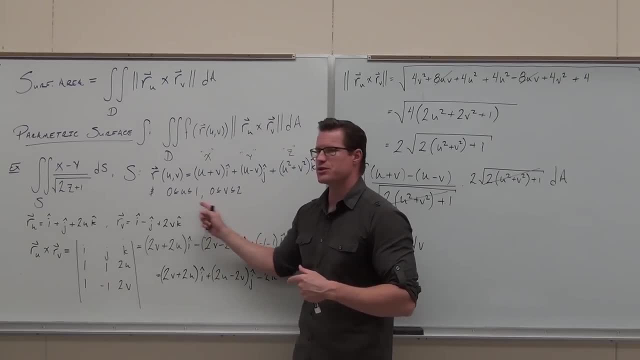 In fact, if you look at the region, the region you have here is: What type of region is that? where u and v are both- Say it louder- Rectangular, Rectangular region. Set up any way you want. You can do du dv. 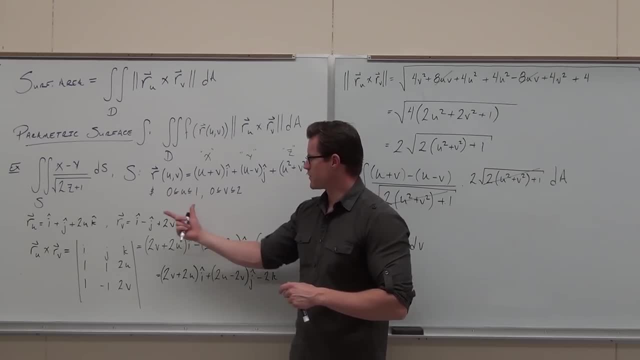 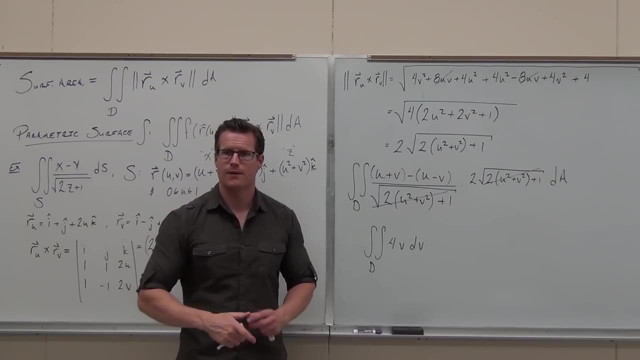 It doesn't matter, As long as you go constants, constants. I would go du first and then dv Also, so I don't have to deal with that v. So I do just a u integrate done Question: Is that supposed to be da? 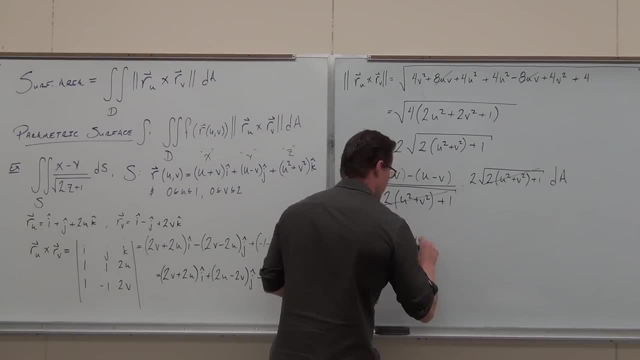 Yeah, I'm sorry, Thank you, It is supposed to be da. I got ahead of myself. Now change it. So I'm going to do 4v, I'm going to do du, Then change, Then change, Then change. 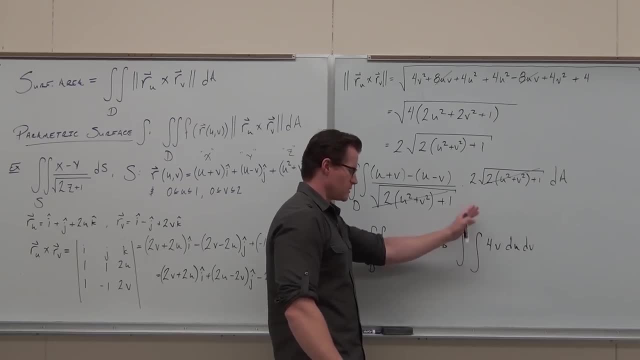 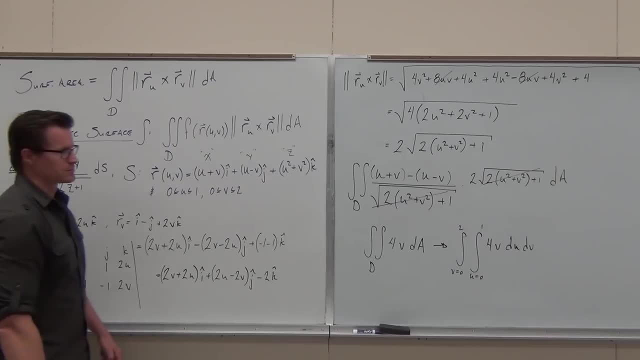 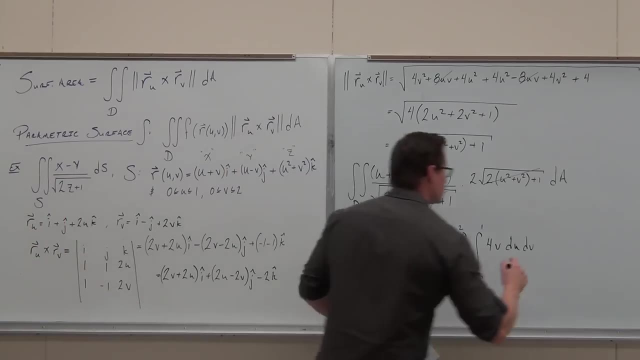 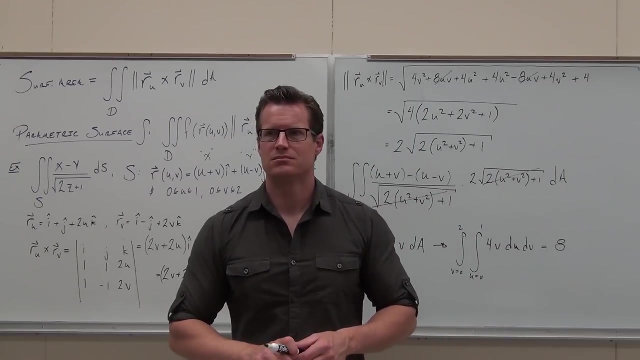 And v is 0 to 2.. Should have finished my work with that Easy medium hard. Plug some stuff in. You end up getting 8.. Now, what is that? What's 8?? It's the surface area. 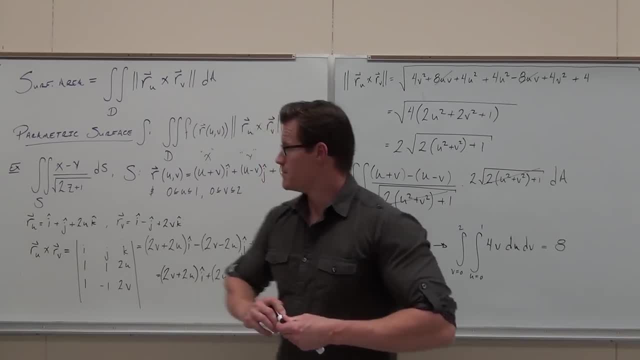 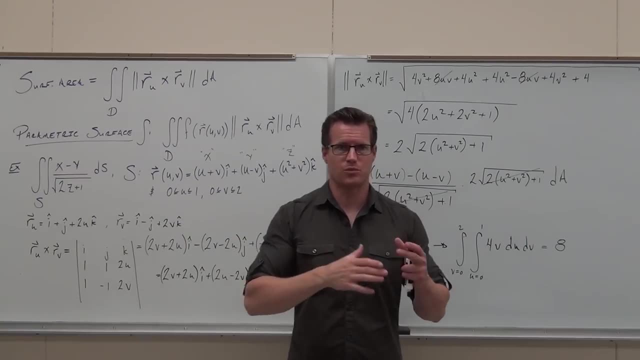 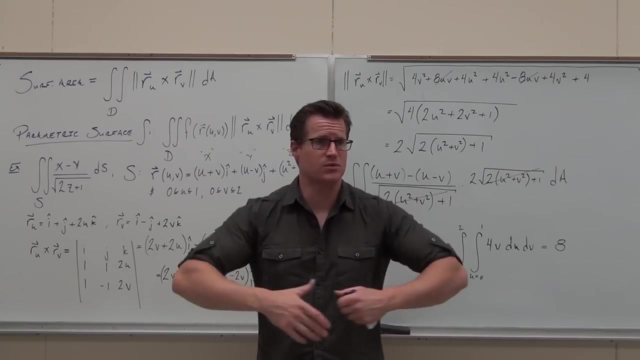 or not. it's the mass. it's the mass of this parametrically defined surface between these numbers, between you goes from so one and V goes from zero to. that's what it's giving, the mass of that's that surface, the plate that's been stretched into a service. that's what's happening and I feel okay with. 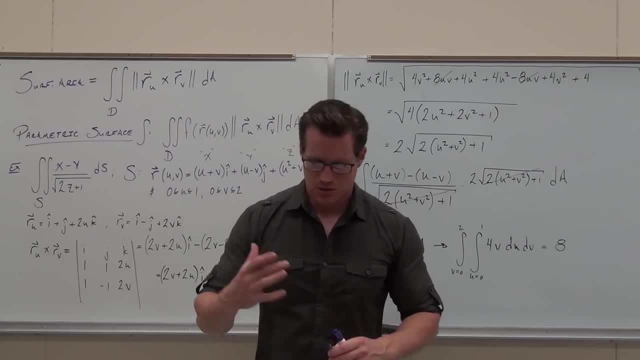 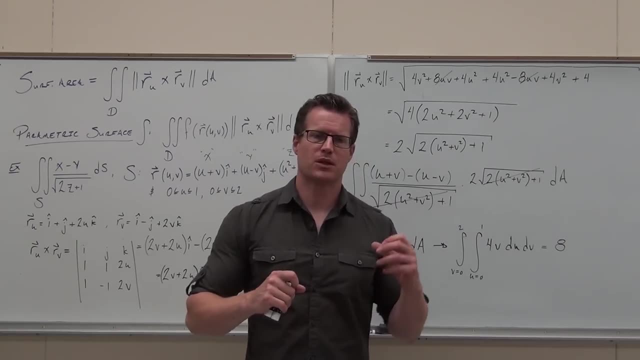 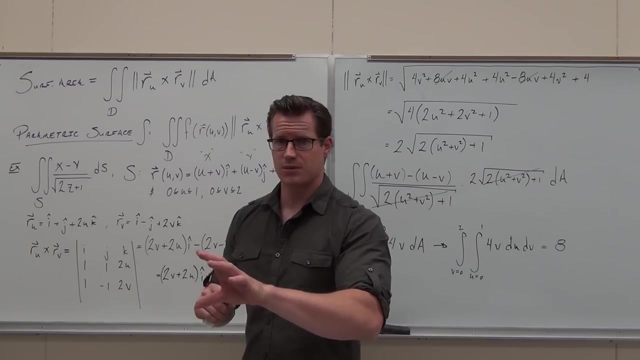 that kind of cool right now. but the next question: if you, if you want to go back to what we did, we did line integrals that we said: well, let's put a line integral through a vector field and let's see what happens. now we have surface integrals. we got to see what happens when we put a surface through a 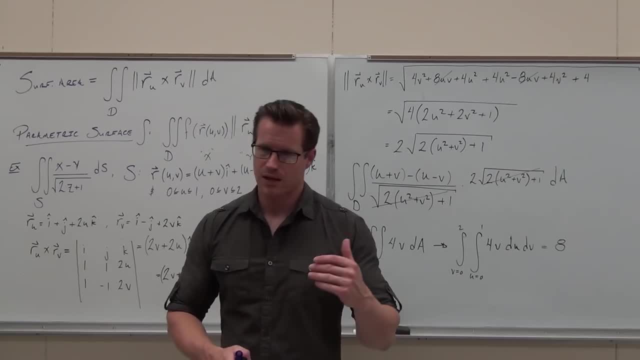 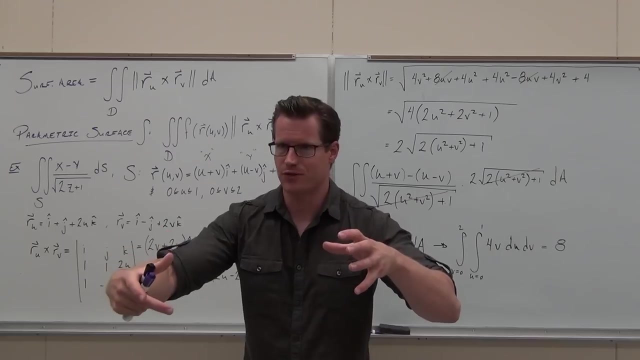 vector field. so we're going to talk about surface integrals, or surface integrals on vector fields. that's we're going to start discussing right now. so I want you to think, think about it this way: think that a vector field you or think of a surface on a vector field, so that that that vector field contains. 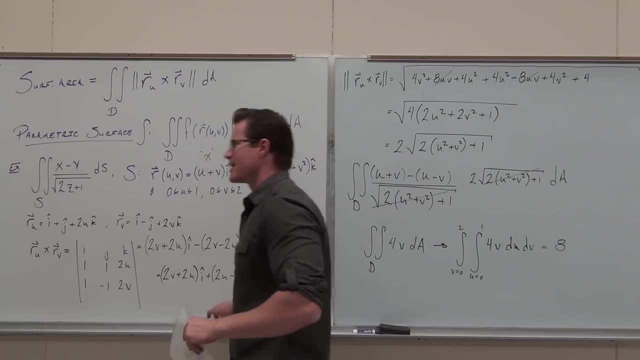 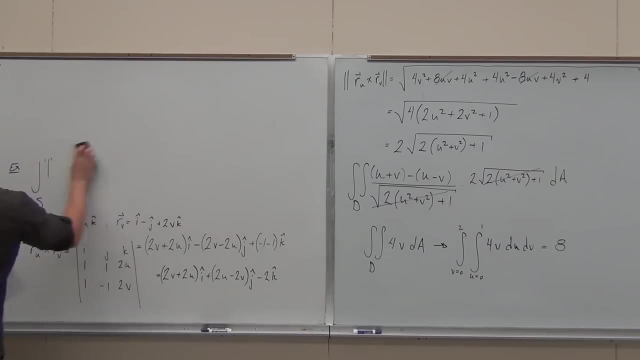 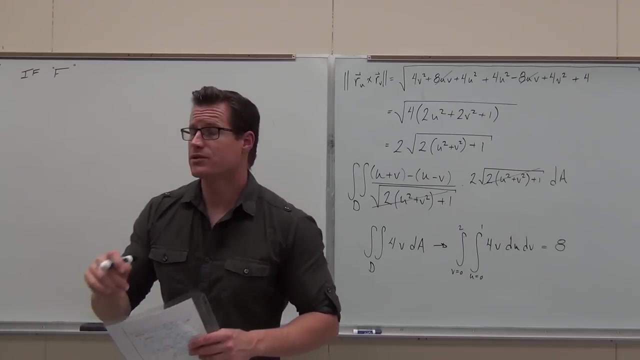 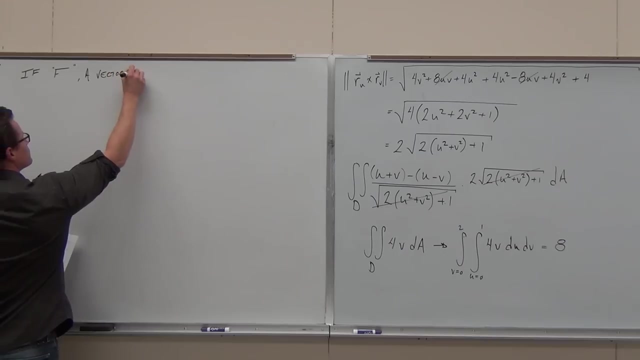 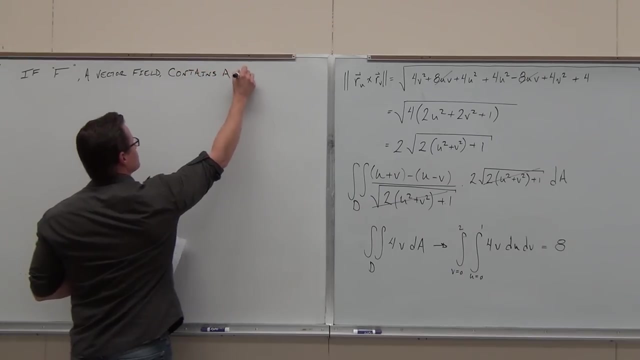 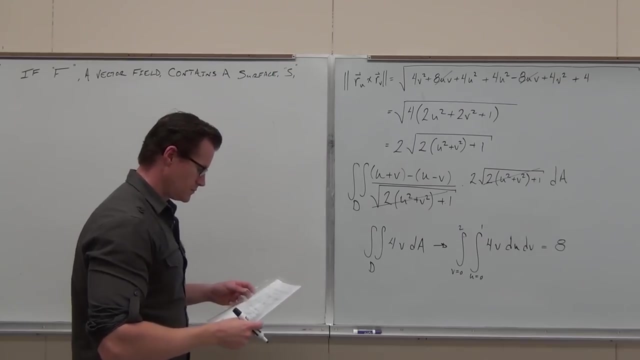 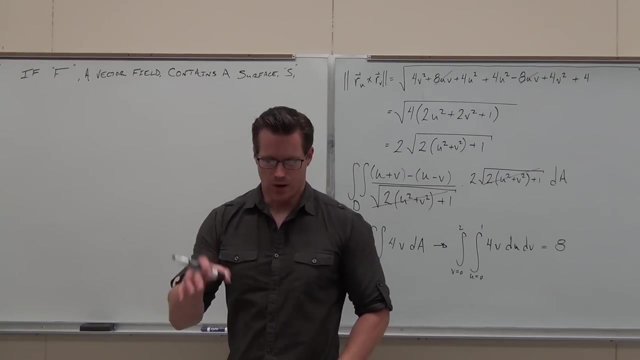 the surface. that's why it's got a couple things about that. you, if f- let's call that a vector field- contains a surface, you, you, you, kamu, then F describes the velocity of the flow or the fluid. we talked about that. I remember talking about vector fields, how they describe the like, the flow of 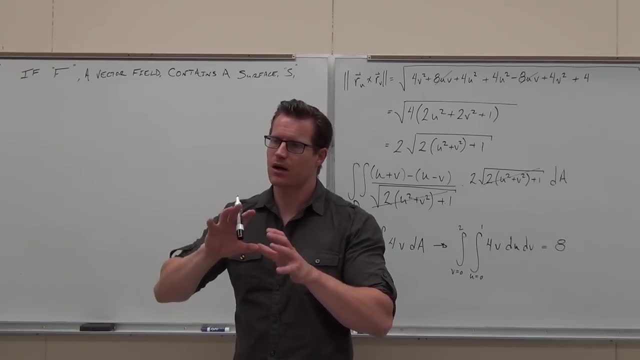 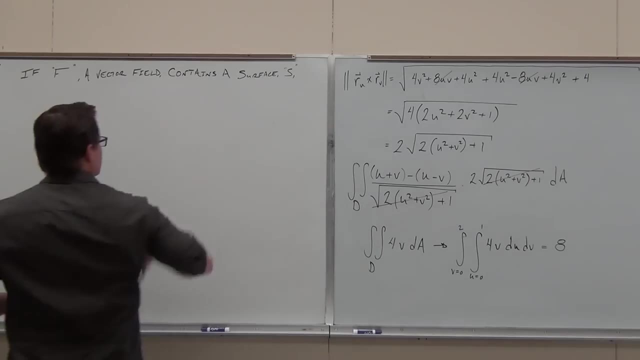 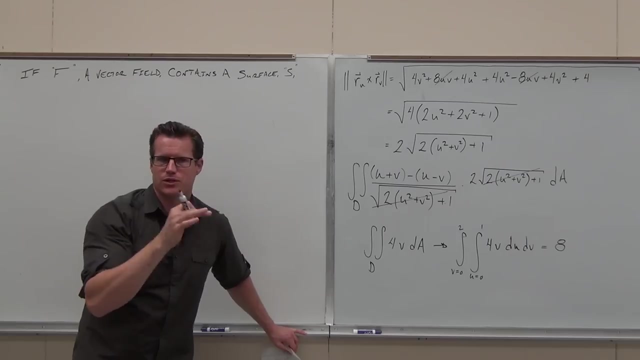 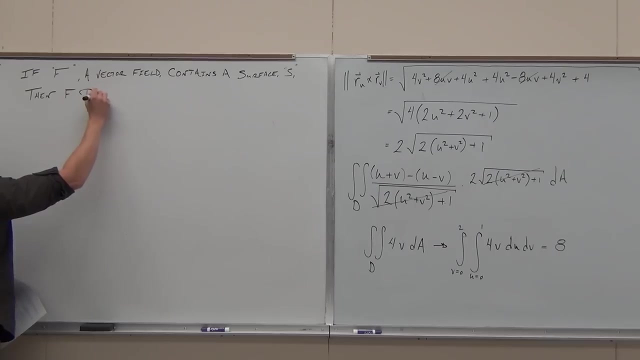 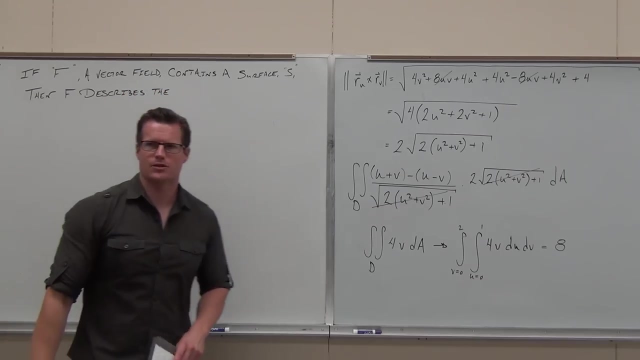 fluid or some substance at any point across the surface. so if our vector field contains a service s, then the vector field describes the flow or the fluid or the velocity of what that flow of fluid is, what it's doing at any point across the surface. Why am I using the word velocity? 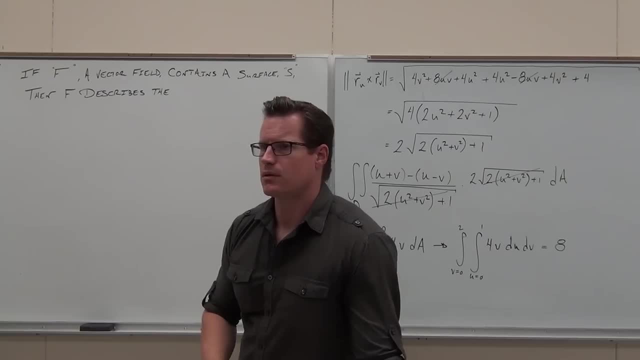 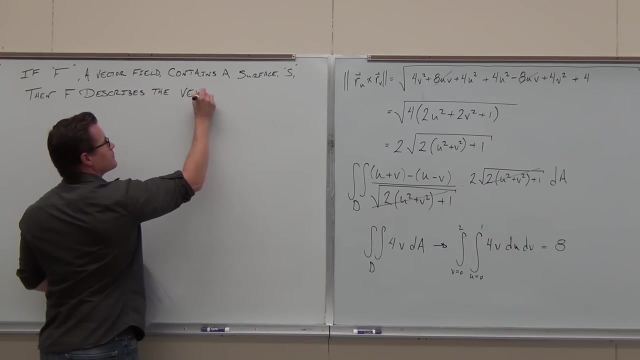 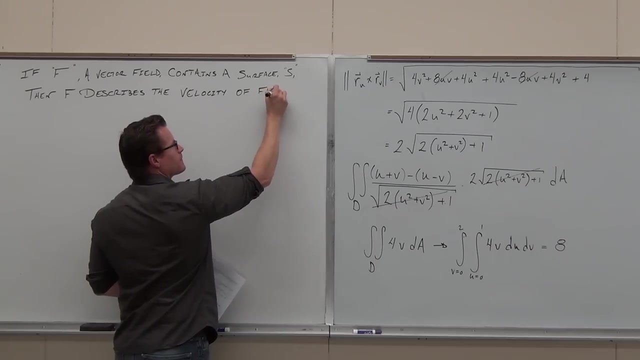 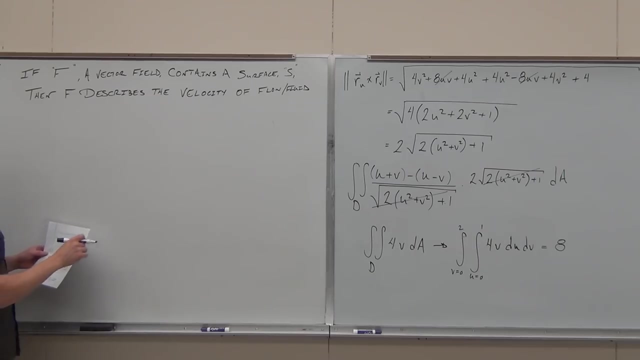 What two things does velocity have? Speed, Good, So basically just a vector. So vector fields describe velocities. That's what they do. So what F describes, the vector field describes, is the velocity of the fluid or the flow, however you want to think about that. 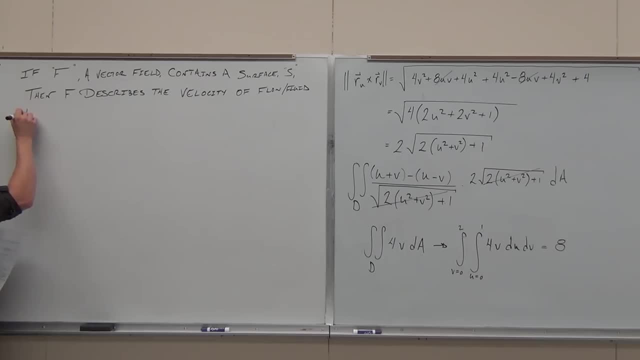 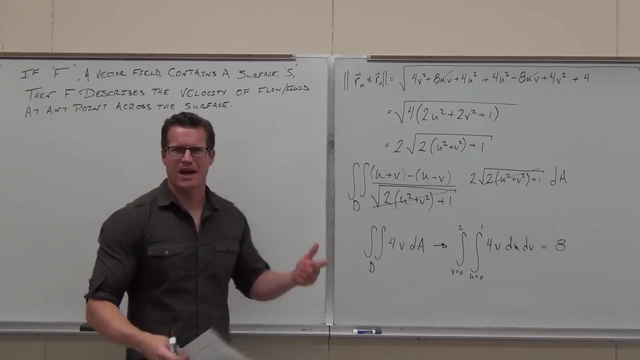 at any point across the surface. You know, it's kind of like before, kind of like before we had that. It's just right. now. we don't have just a flat flat plane, We don't have that, We don't have a flat figure. 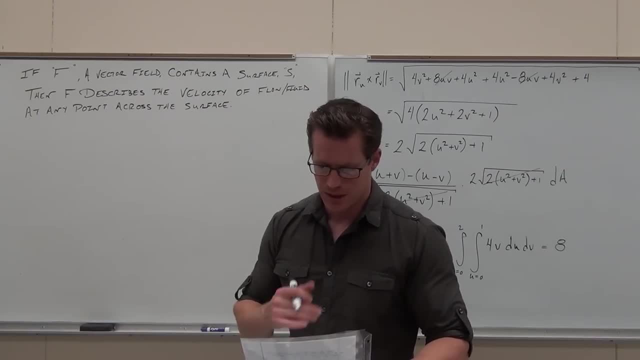 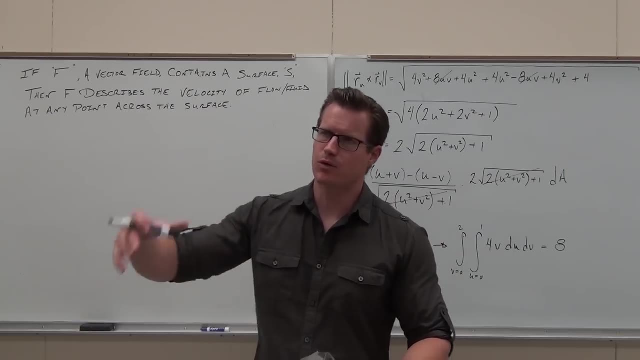 Right now we have this, this surface. It's going through a three-dimensional vector field. By the way, I can describe something for you: The rate of flow. so the amount or the volume of the flow going across the surface is called something called the flux. 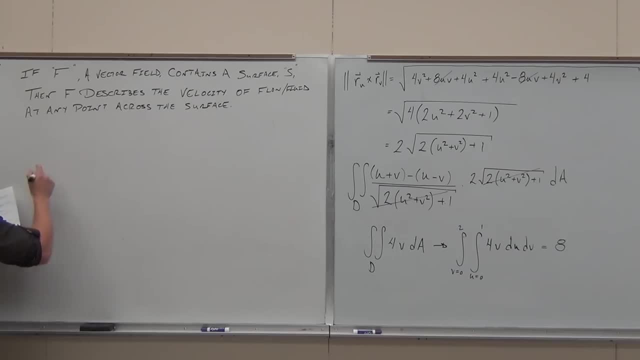 Okay, Let's see what it's going to look like. Okay, So these are the two things: the speed, the velocity. the velocity and the momentum of the flow across the surface. So how much velocity am I gonna have? I'm gonna have. what's my rate of flow? 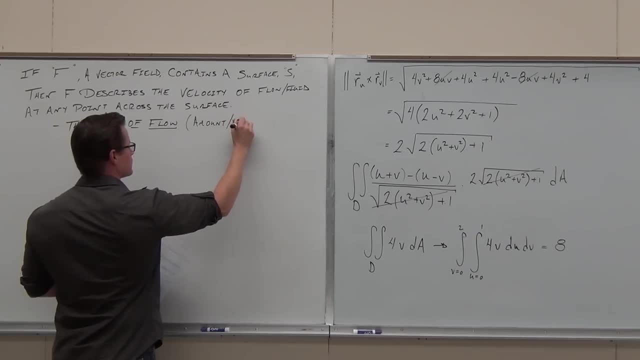 Minus one. Let me see here: Okay, What do we currently have? What's our rate of flow? We have 90-point velocity. If I multiply that with one, it's going to be 2.5.. Okay, So that's. 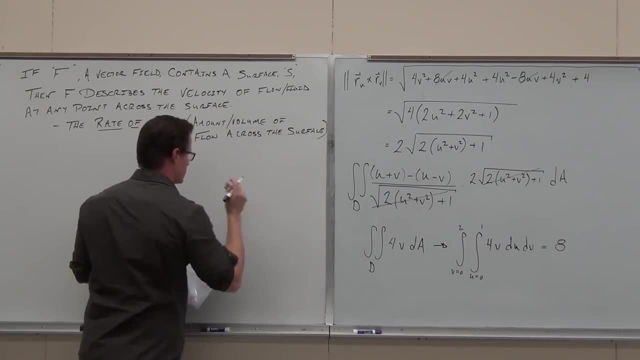 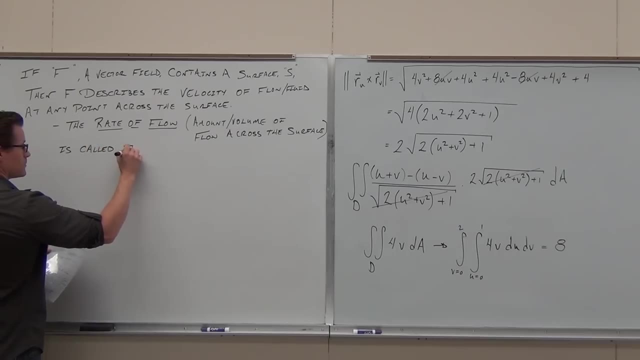 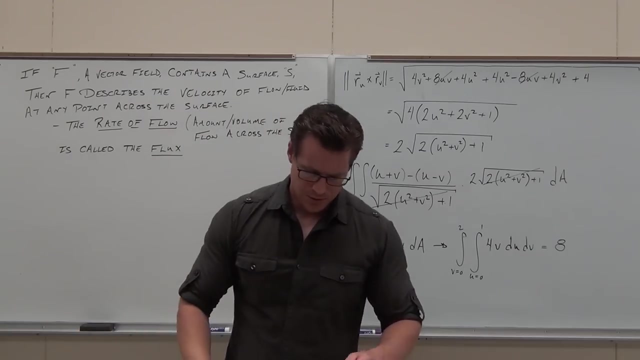 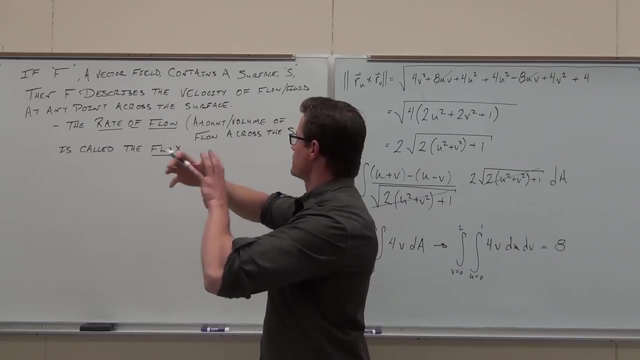 Okay, So let's see. It's also called flux. Now we're going to deal with something, but I want you to hang on to this idea. Can you do that for me? Hang on to the idea of the amount of the flow going, or the volume of the flow, the rate. 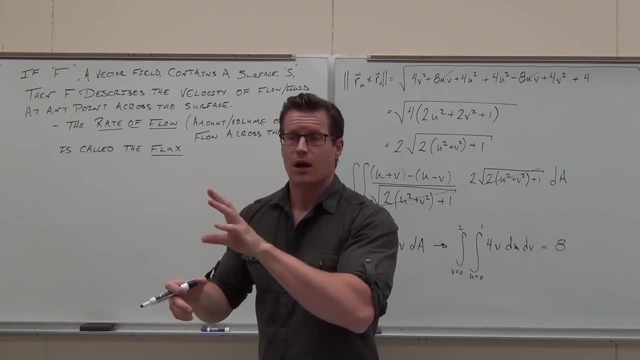 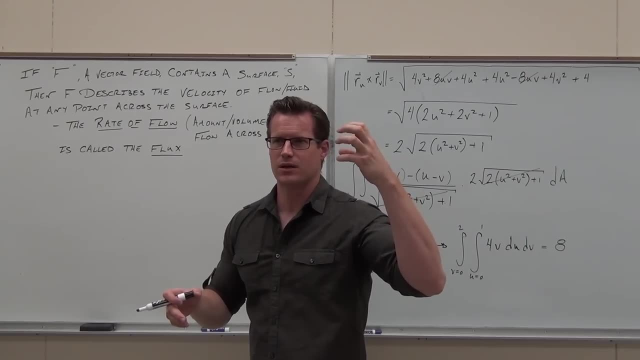 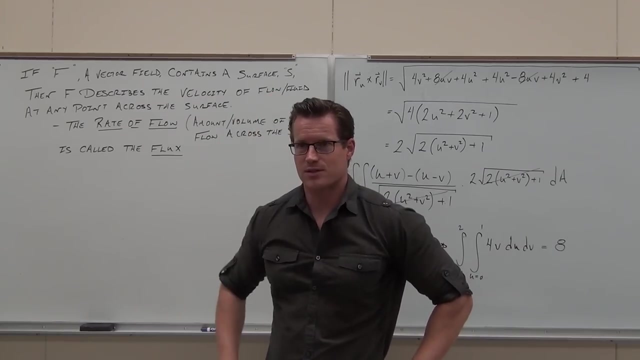 of flow across the surface. What's that called, again, The flux? I want you to hang on to that idea, like that, one thing in electricity that holds on to charge. What's that thing called The flux? That's right, I want you to be a capacitor for the flux. be a capacitor for the flux, be a. 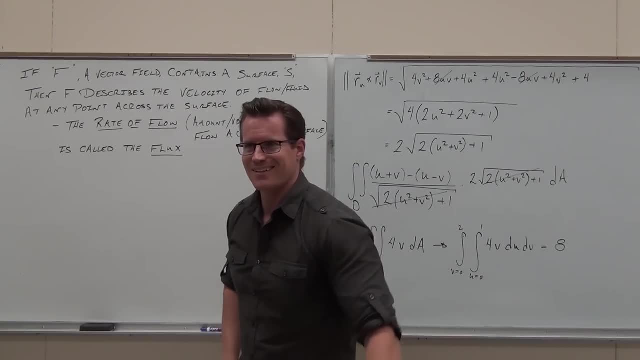 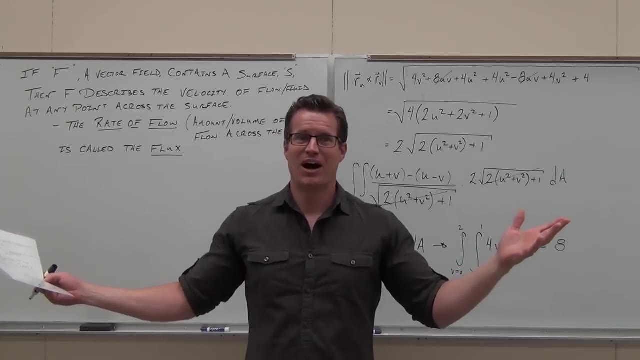 The flux, The flux. You got it. Boom, I had to throw one more in. It's the last lesson. I'm pulling all the stops here, guys. I can't use it later. man, it's the last video. 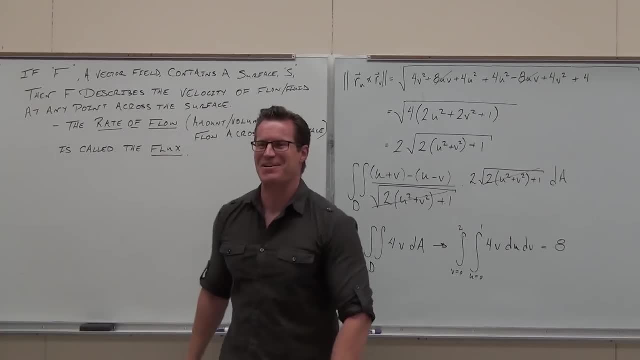 Two, I need a flux capacitor. Dang it, That's good stuff. What I worked on that all day, just for this moment right now. It was like lesson prep jokes. That's what I'm doing: Cheesy, cheesy, back to the future jokes. 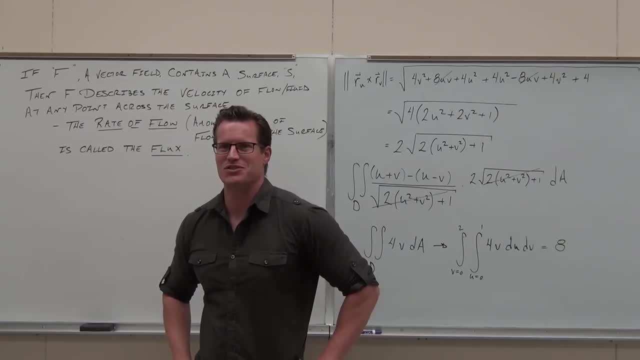 Seriously, though, it's called flux. I might make that up. Let's talk about the flux Now. let's think about this: The flux is given by. I'm going to give it to you, but I'm going to show you why it. 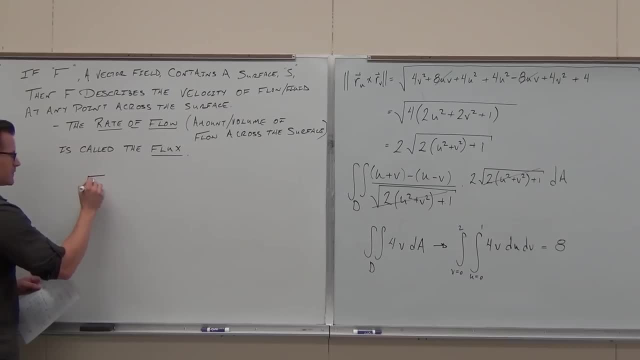 makes sense. The flux is given to you by this, The vector function is given by this. the vector field dotted with the normal vector surface area. You go well, what's this really mean? This is a vector field dotted with the normal at any point of that surface. 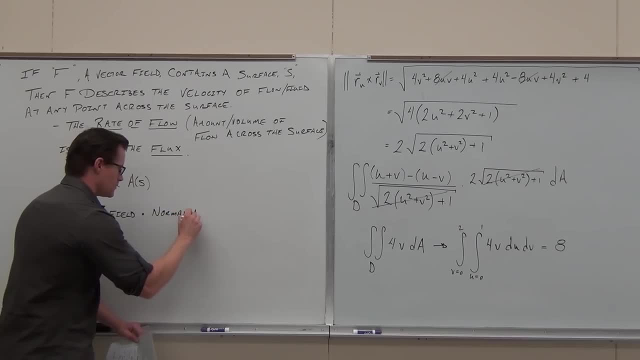 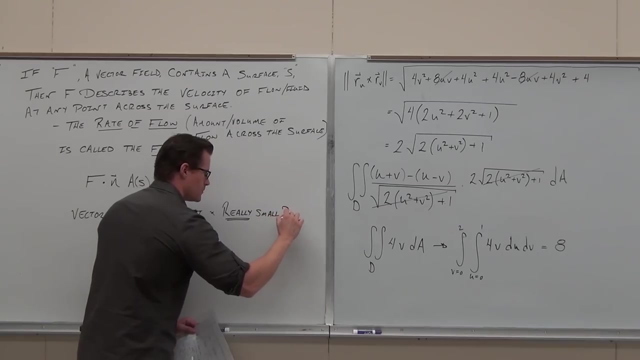 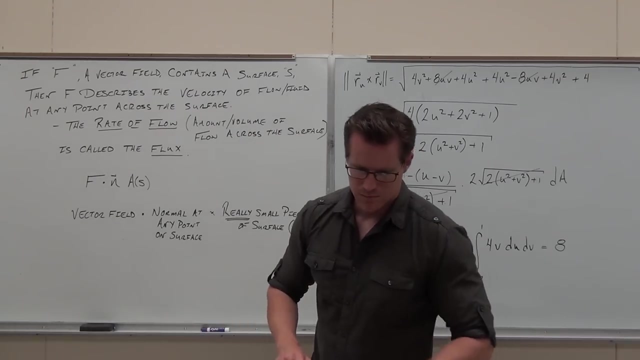 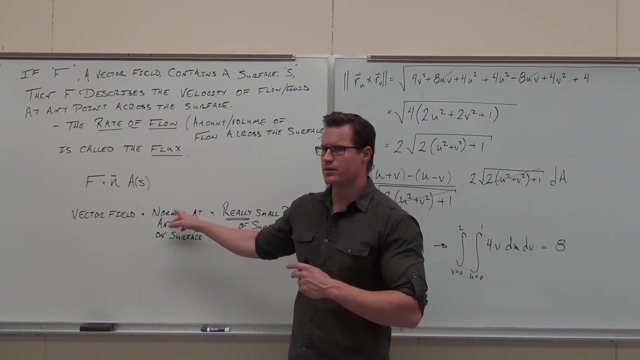 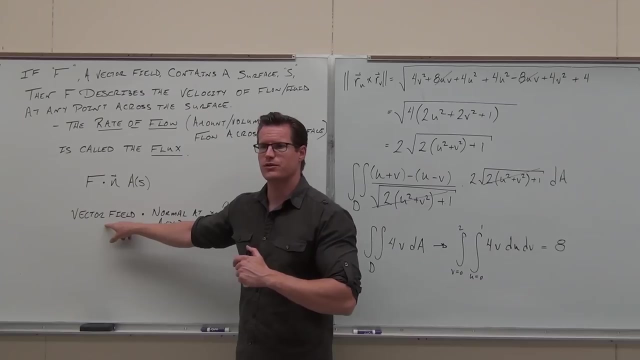 Not cross just a little times multiplication, The area of a really small piece of the surface. So surface area, What's it given us? Well, it's given us a normal to that surface and the flow through that surface according to the vector field. 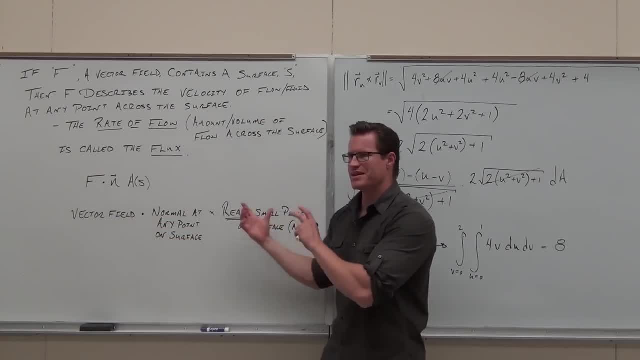 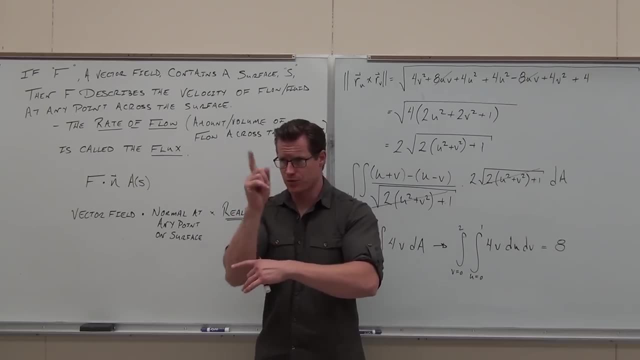 So it's given us how much is crossing this region. This is the idea here. Think about the idea. please Listen. Normals go through stuff, right. So if you had a surface normal, it's going through that. It says okay, vector field's describing that flow. 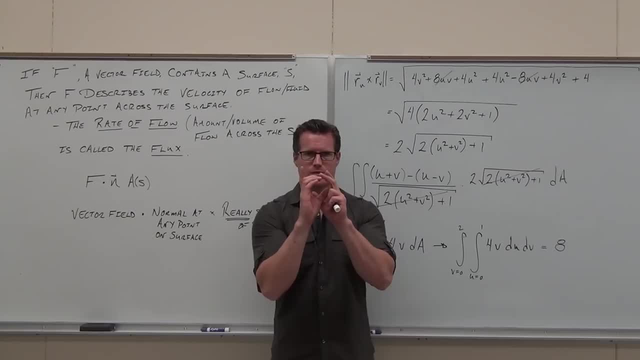 I take a dot product. This is the amount of the flow times, the size of that region. Basically, this is the amount of the flow going through a little teeny bitty region. Now we want to do this for the entire surface. 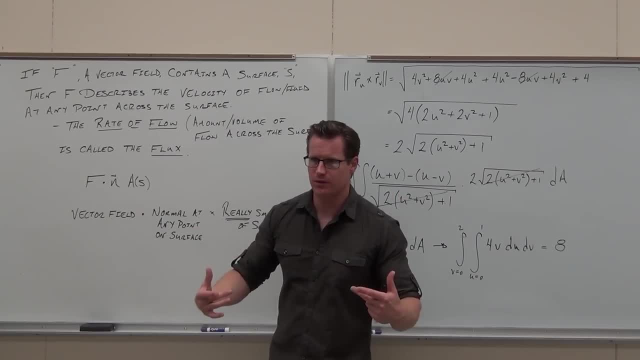 And then we want to add it all up. What adds up stuff in calculus Integrals. So surface is two-dimensional idea over the region. Think the region Two-dimensional idea. We're going to be adding up all the flows across little bits of surface. 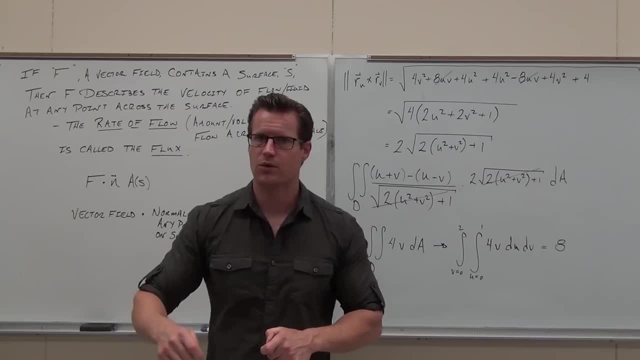 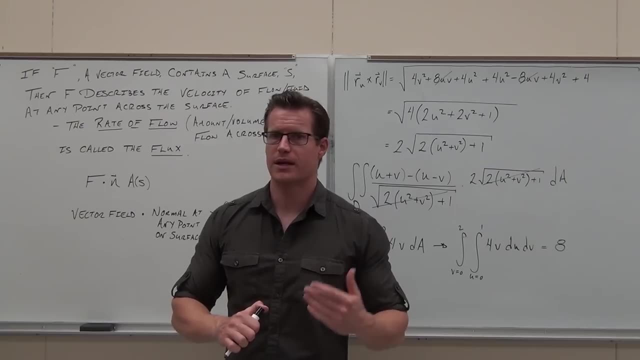 That's what this is called. It's called a flux integral Or typically we call it that. So this would be a surface integral through a vector field, Or we call that a flux integral a lot, Because what it's describing is the rate of flow or the amount of the volume that flows flowing across the surface. 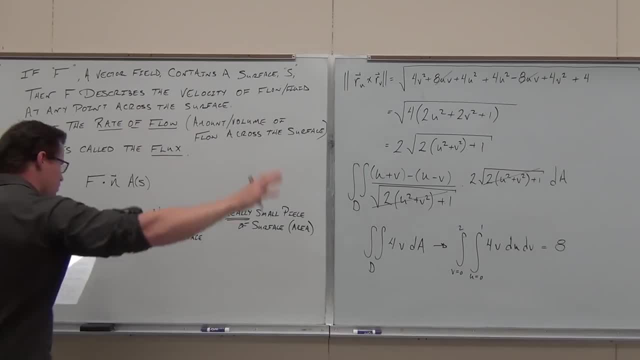 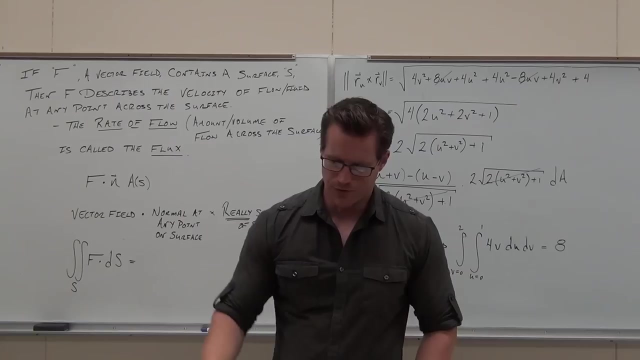 And not, if you're okay, following the idea. So if we do this for the entire surface, well then we have a surface integral changes a little bit. So we'd start saying, well, if we can describe this, as I've got to make a little fine point here, 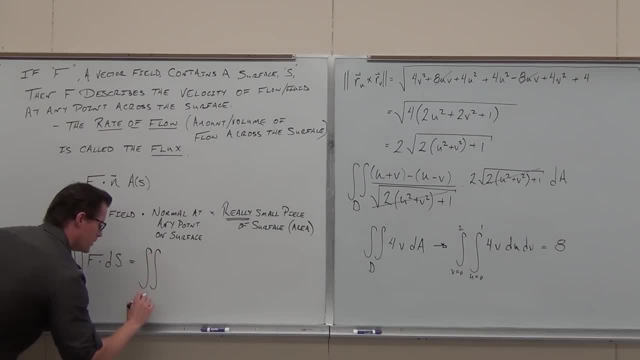 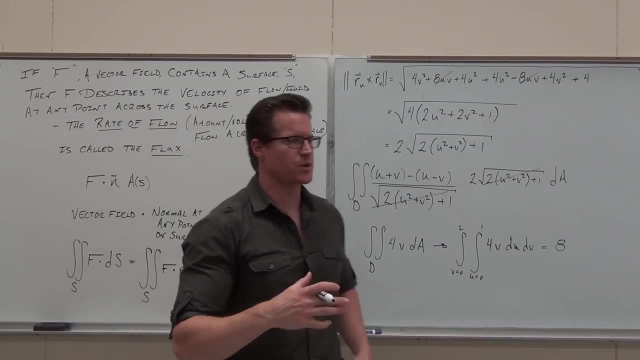 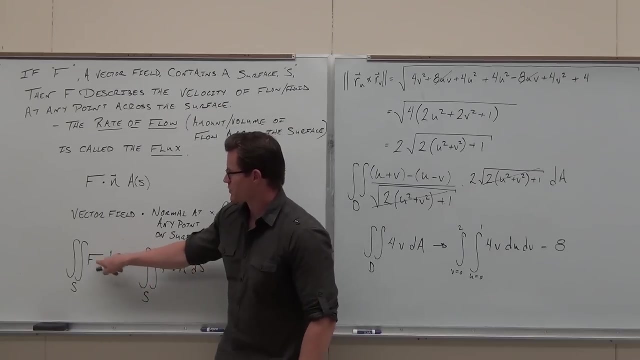 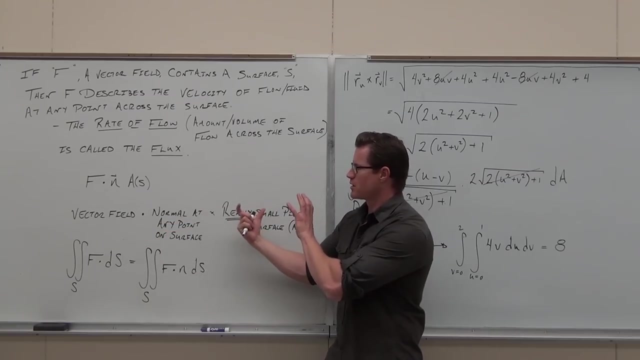 Here We'd say, if we want to do a surface integral where our surface is going through a vector field- that's what this says, A surface integral through a vector field- We go. well, what are we going to do? We're going to think of this as the vector field dotted with a normal times a really small part of area. 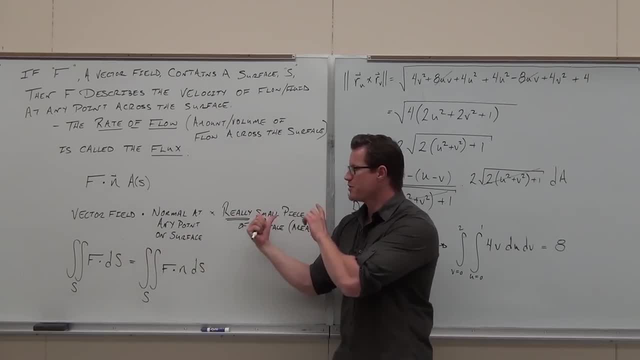 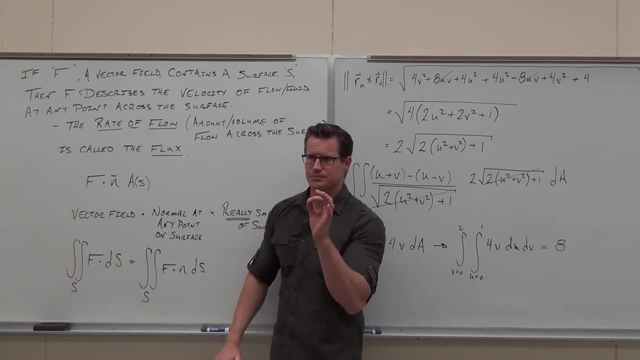 This is the amount of the fluid going through that area. That's what this means. I need to make a little point here: Much, much like The switch between F dot, DR and F dot, that that R prime DT, this S is slightly. it's a slightly different S. 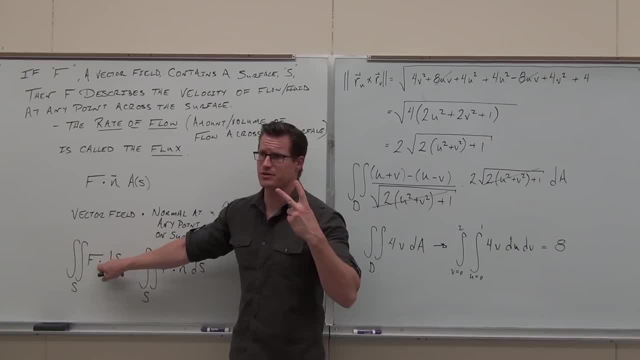 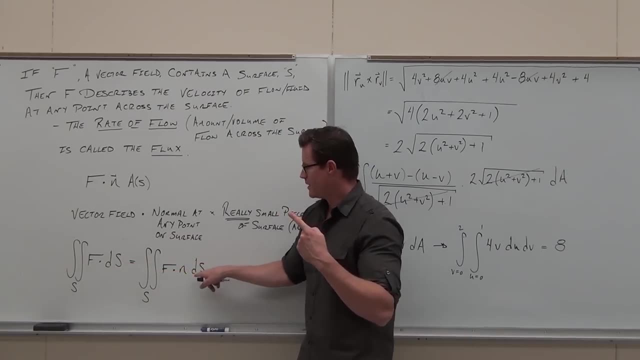 Notice the difference. Dot product has to happen between two vectors. Do you see it? These are two vectors. This includes the vector portion of it. This one does not. This is a dot product between F and N. This is just the idea of the area itself. 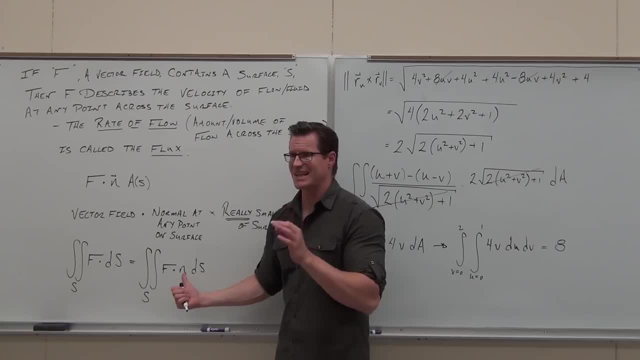 It's not a vector. Difference between a vector and a scalar. Does that make sense? It's slightly different. Now, fortunately, we don't have to deal with this a lot. We're going to make another jump here in just a second. but the idea is: is this idea? 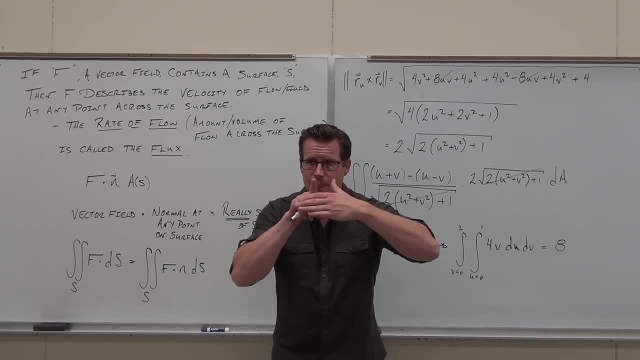 The idea is we're finding the flow that's going through a surface, a little little teeny part of that surface, and then we're adding up all that flow and that's giving us a flow through the surface over a given region there. 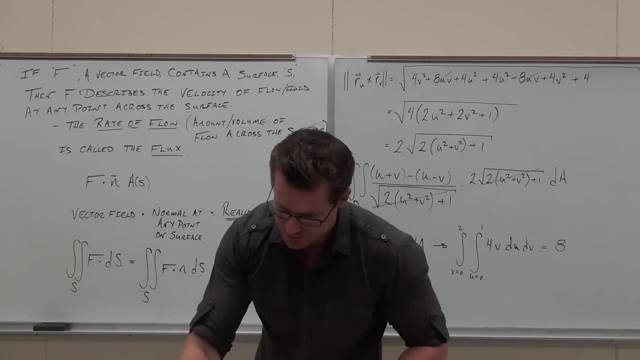 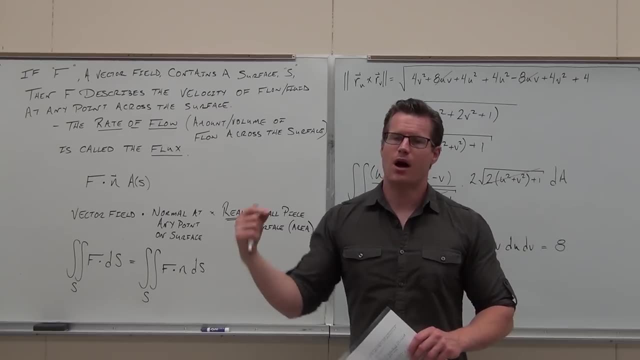 It depends if you know it, if you understand it. So this is, this is the idea. This is called a surface area, surface integral through a vector field, or we often call it a flux integral. Why? Because it describes the flux. 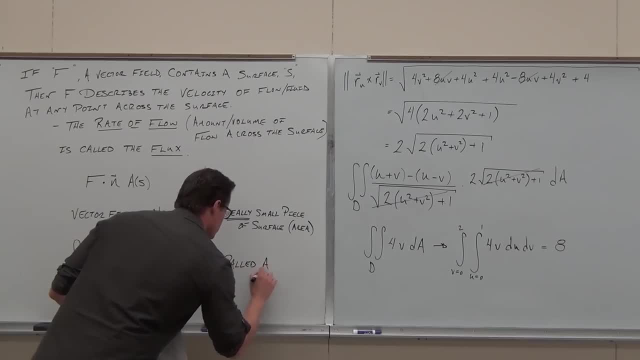 We say we're going to add this over here and it's going to give us a flux integral to this surface and we'll be doing that over here and over here, and over here, and over here, over here. but if we're adding those together it's going to be draw a fraction of the material. 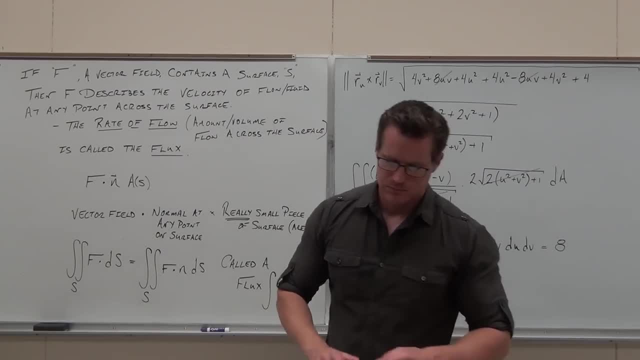 that's going to be coming from this surface area and that's going to be the Well, we're going to do that over here. That's not going to be the fixed surface area. Now one last statement. then we get to. 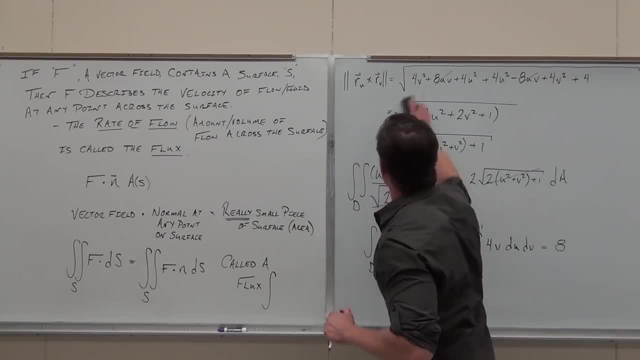 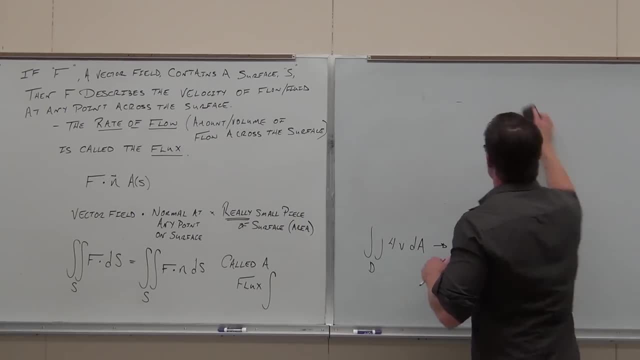 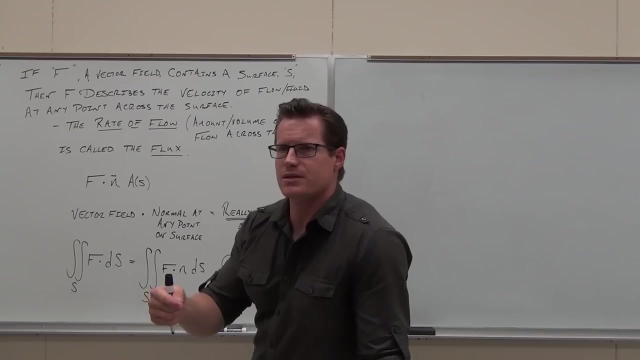 get to the kind of kind of cool part, how to do it. You know, I hope that you're kind of sticking with the idea, because a lot of calculus builds on this idea of the same idea over and over again, which is applied to different things. 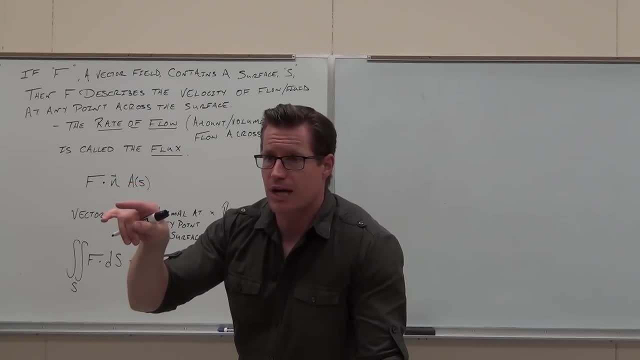 When we had a double integral of 1 DA, that was just area of the flat region. Make sense, Put a function in there you find a mass of the region. You get it. When we had surface area of mass density, function 1,. 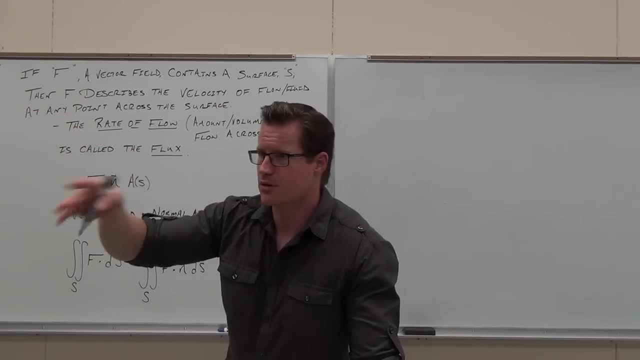 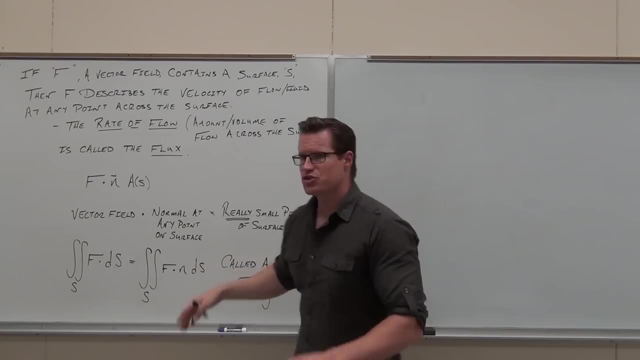 which we just had it. that's giving us, well, just the surface area of the surface. We put a mass density function, then we get the mass of that surface. This, right here, is just giving us the amount of flow through a surface, across a surface. 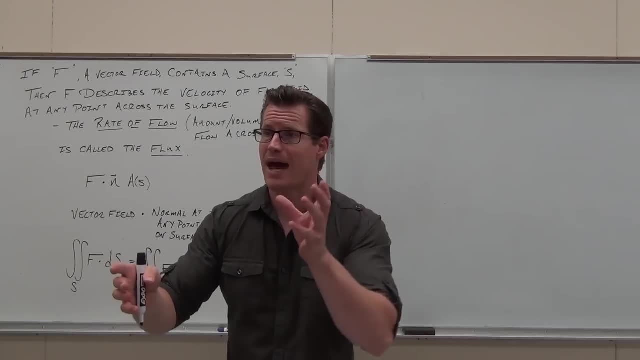 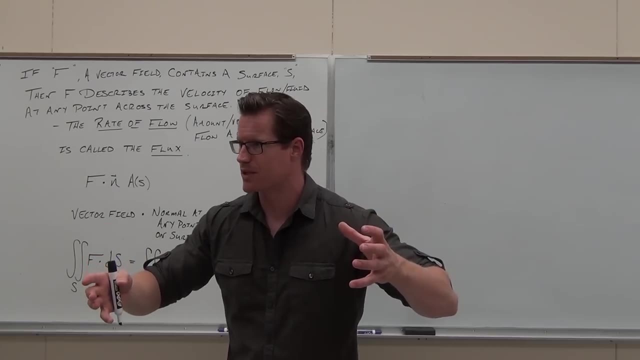 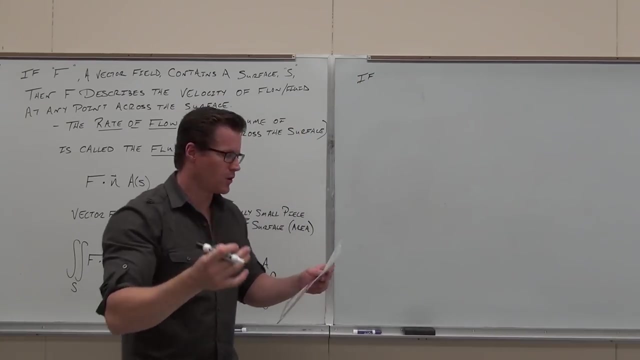 Does that make sense to you? What if that flow has a mass density function? Then it would give us the mass of the fluid crossing that surface. Does that make sense? So, if I want to find this, so if the fluid or the flow has a mass density at a given point, 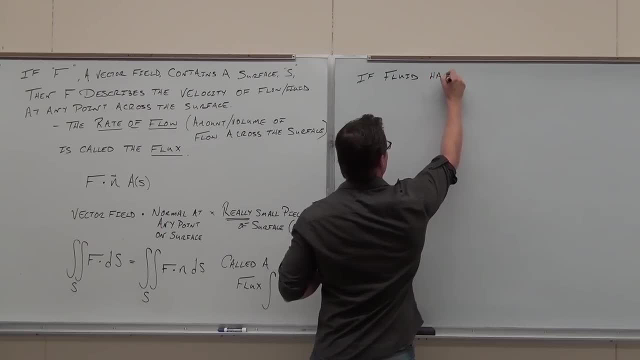 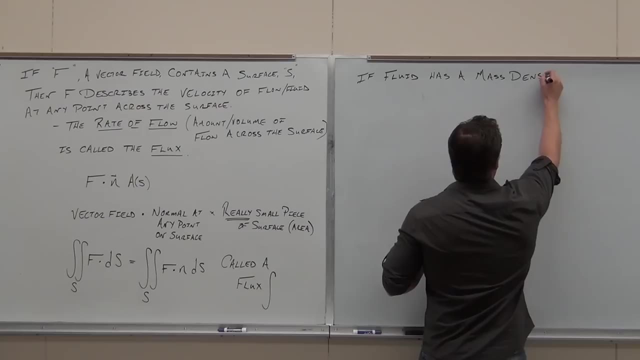 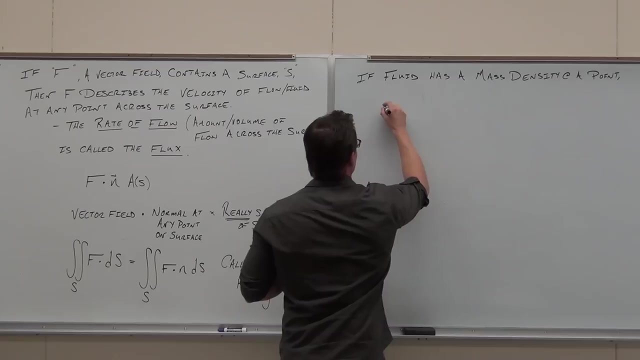 then we know the mass density function of that surface. This is just that of the surface, But we see this line here. What You mushrooms leave? a small wave. Your bins are big, That's why I am overriding it. Yes, Thank you. 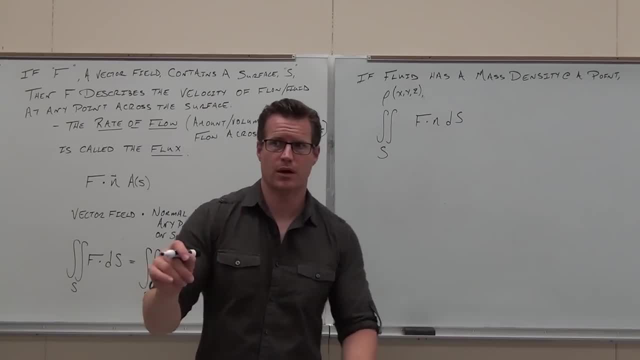 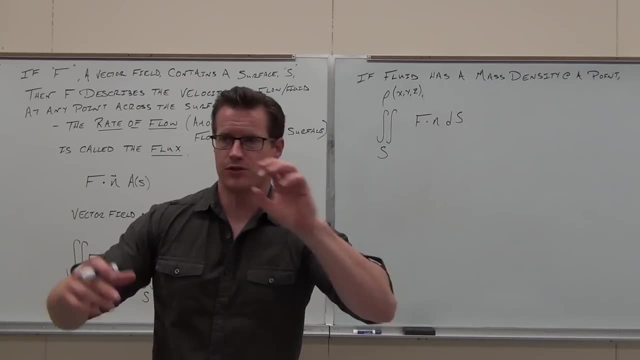 Okay, please watch carefully. I want you to get it. I really want you to see the scenario play out for you. The same like double integral over region with one and versus a mass density function, Surface area with one and then surface area with mass density function. 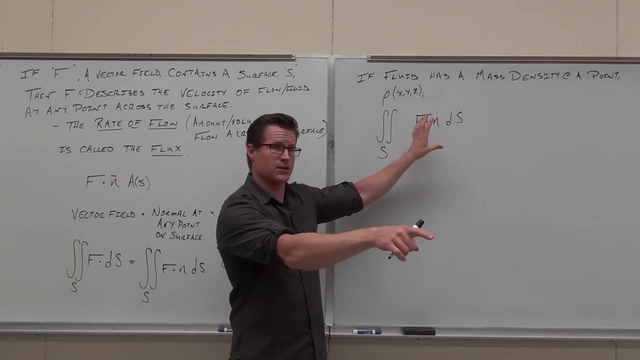 What's this? give you? What's that called Flux? That's a flux integral. So this is describing the flux, the amount of the flow going through that surface. whatever that's defining, I don't know if you're okay with that one. 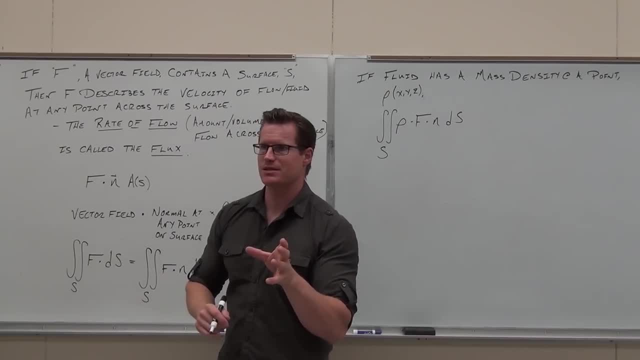 Then that gives you the mass of that fluid. Does that make sense? It's very similar to the previous concepts. we've had Amount of flow, mass of flow. Get it Like amount of area, mass of the thing that's occupying that area. 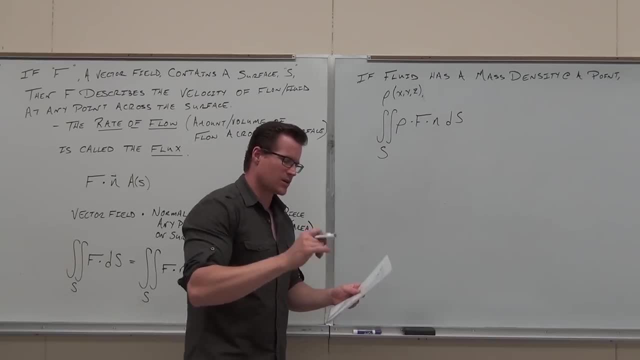 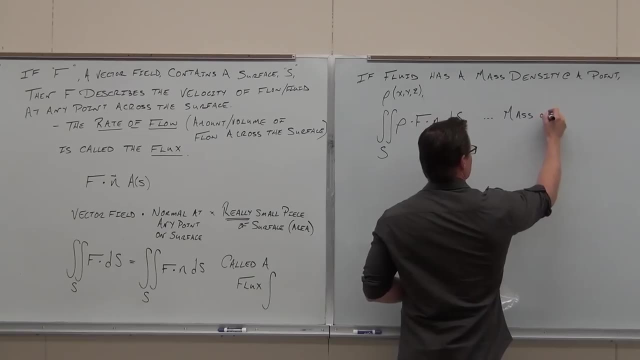 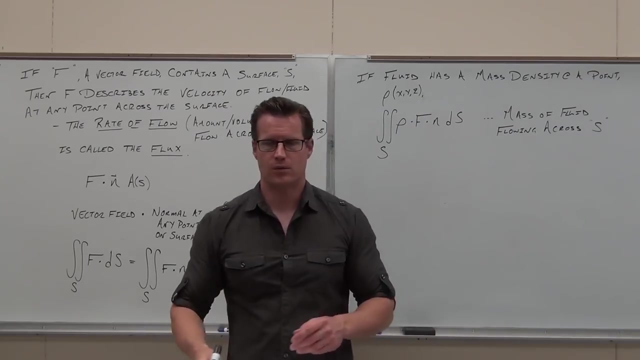 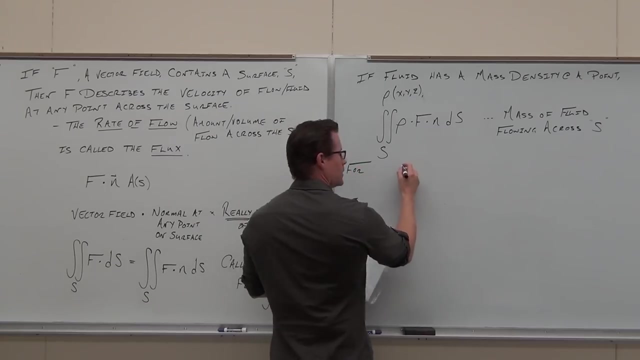 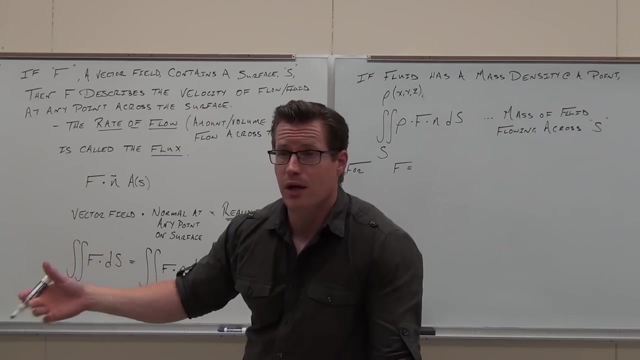 Very similar idea. So this would give you the mass of the fluid flowing across the surface S. Now how will we actually do it? Obviously, I'm going to have to define a few things for you, right? Any time we do this stuff through a vector field. 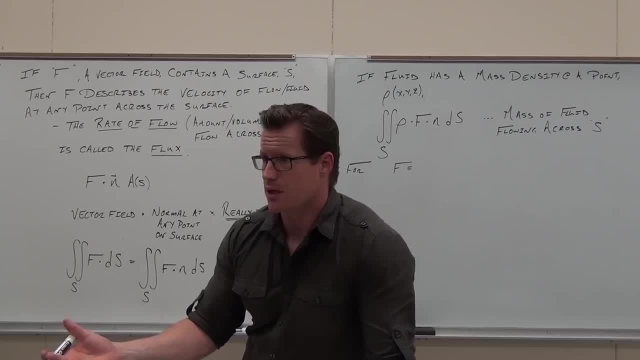 you need to know what the vector field is It matters. You also need to know what the surface is. It matters for right now. So we need those two things. So let's define a vector field. It's this thing, It's normal. 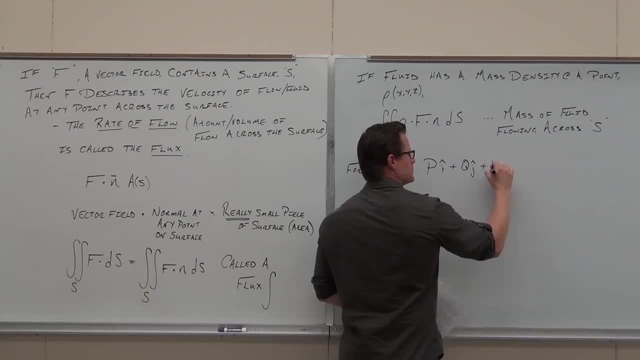 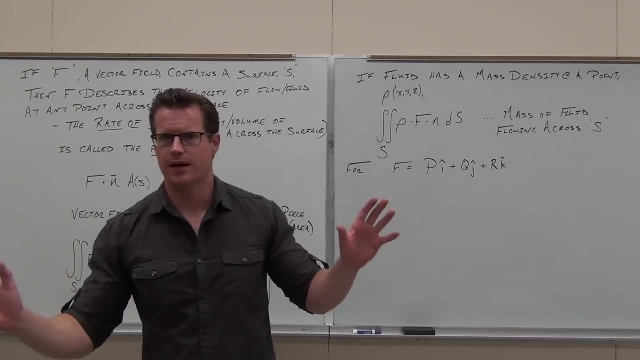 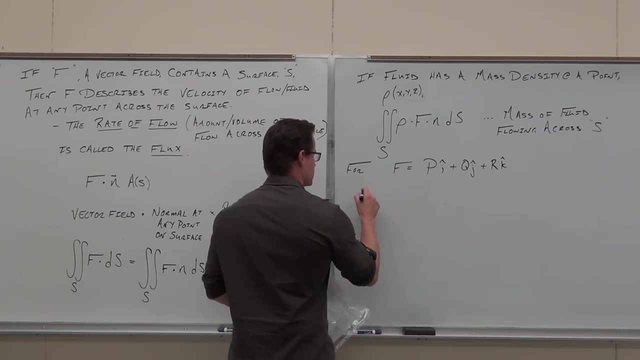 P, I, Q, J, R, K. So just a function-defined vector field, Hit not. if you recognize the idea of a vector field, That's our vector field. Then the flux integral. This is where we started. This was hey. 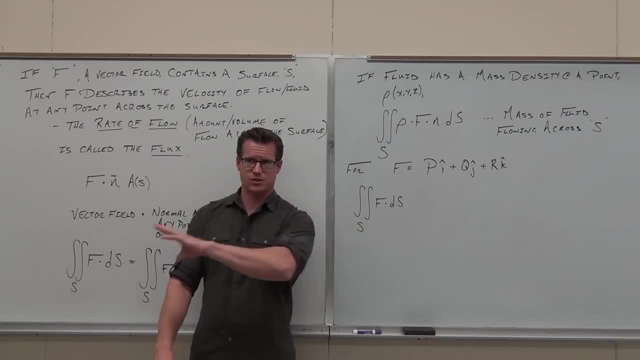 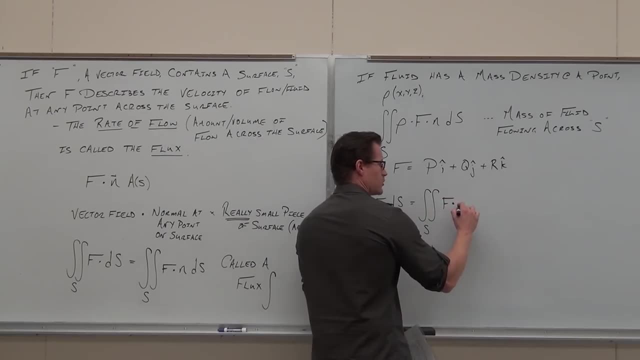 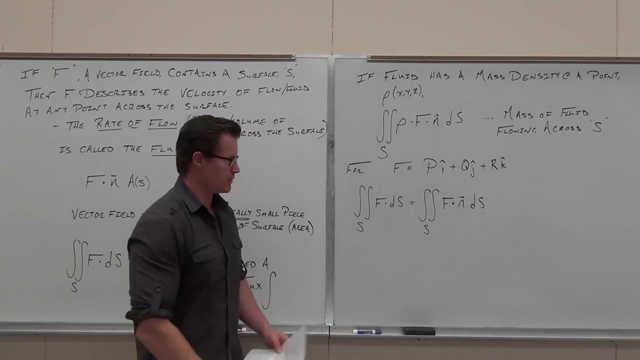 This was a surface integral across a vector field. That's where we started with: So well, this equals this, This is a surface integral, and we changed it a little bit. We said, yeah, that's the same thing. We talked about that. 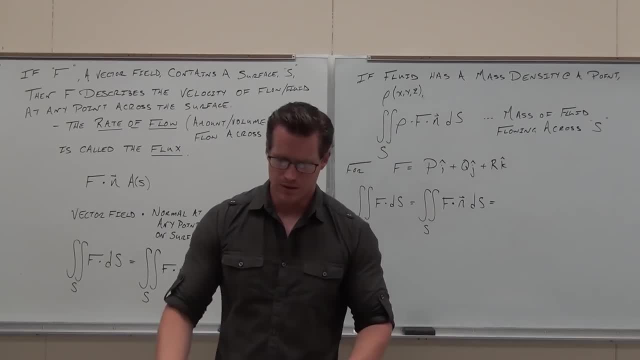 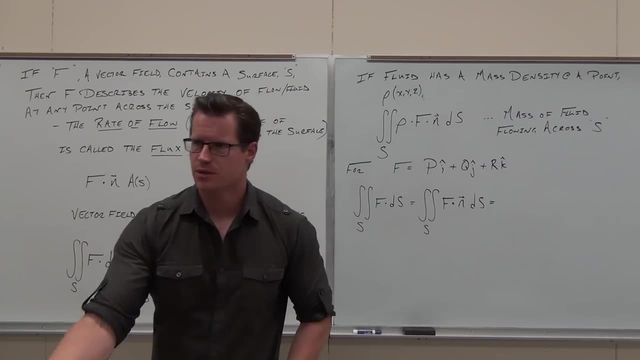 We go: okay, here's how we actually do it. This is a formula. I'm going to just state it without proof, but it's going to make your lives really nice. Here's how we actually compute, And the formula is this: 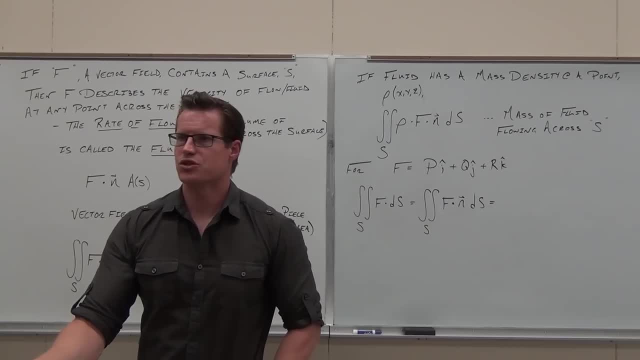 The proof. I believe it's in most of the Calc 3 books out there. You can just check the proof out. It's not beyond you. It goes back to some summation notation. It just adds up the little areas. If you made it through the other proofs in this class, you can look at it. 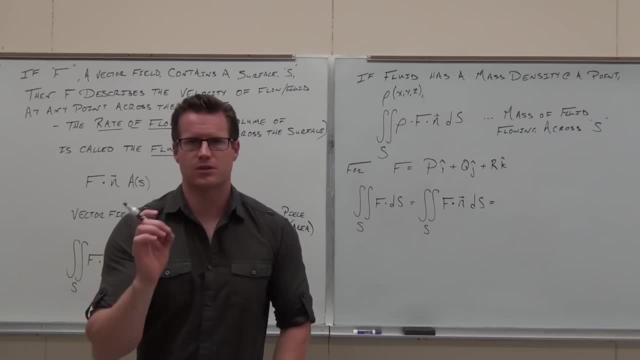 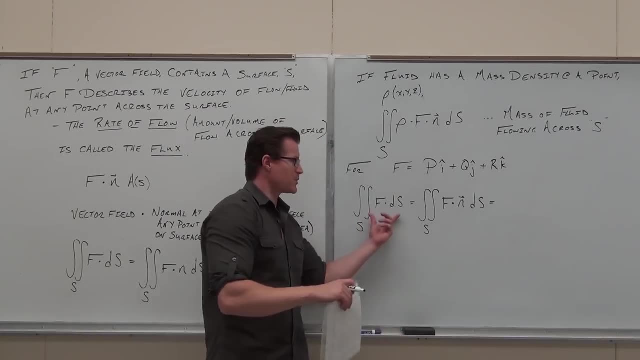 You can do it yourself. You really can Just take a look at it. It involves some cancellation simplification, but it's not beyond you. So here's the how we do it, though Do we get wrapped up with this? 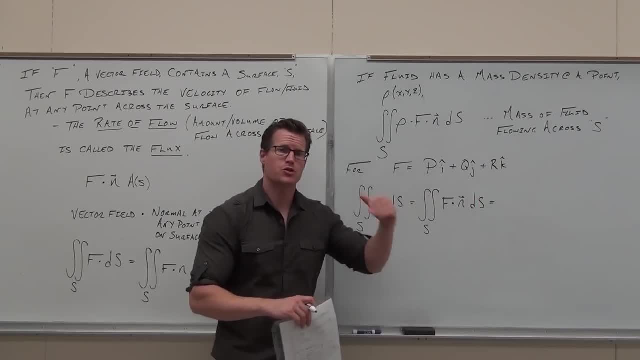 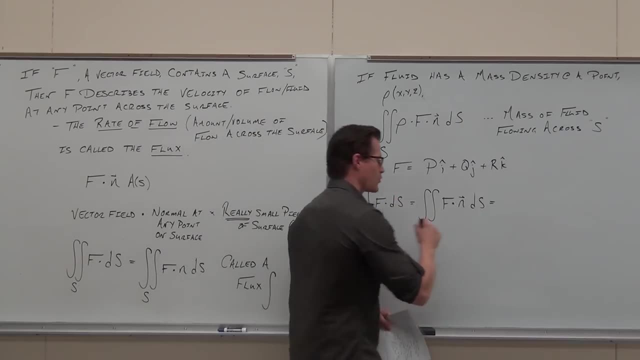 No, Or this: No, Here's how we do it. If we're trying to calculate the flux of a vector field across a surface, we can use this formula. It's going to look kind of nasty at first, Don't worry about it. 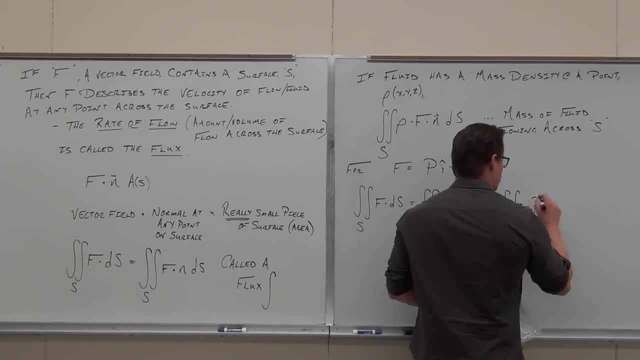 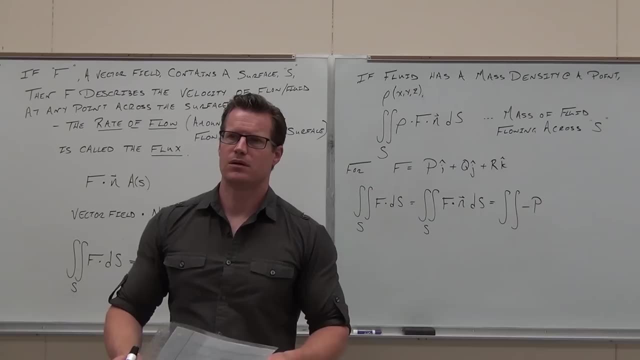 I'll show you where everything comes from. Negative p: Where's the p coming from? The max: No, The p, not the rho The p. Where's the p coming from? That's what the p is. It's just the x component of the vector field. 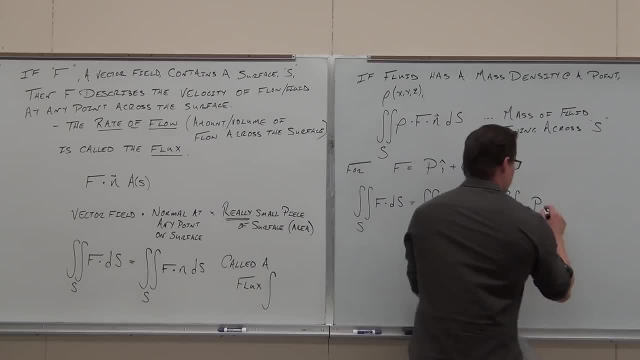 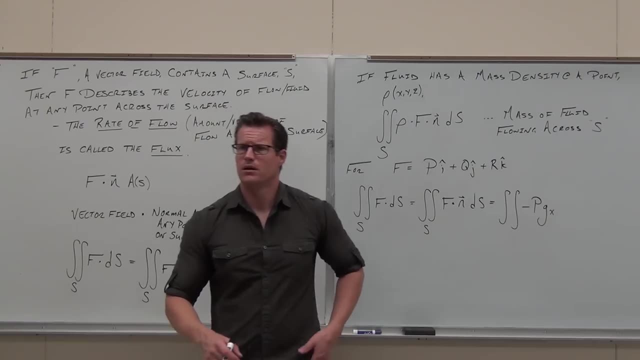 They put a negative in front of it. Does that make sense? What's that mean? What's that mean? Partial derivative of g, G? Where's g? This would be for a surface that's defined. z equals a function, x and y. 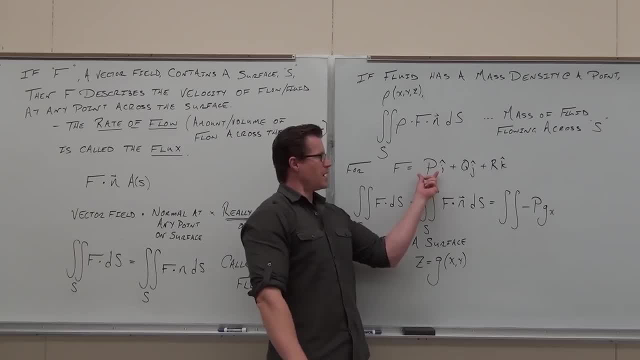 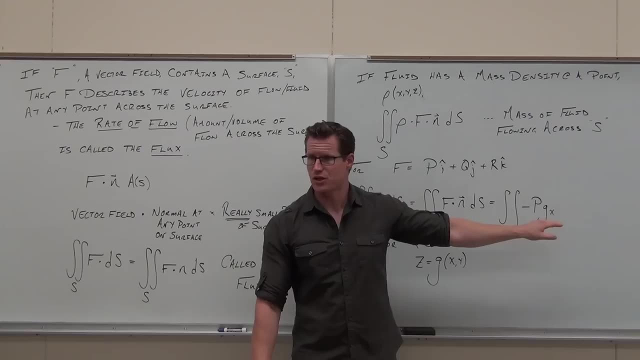 So we start off with x, component partial derivative with respect to x. They match up. Make sure they match up Minus what do you think the next thing is going to be? Just use your intuition. What do you think x is going to be? 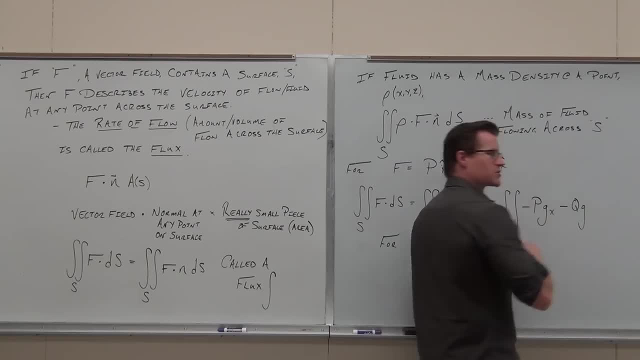 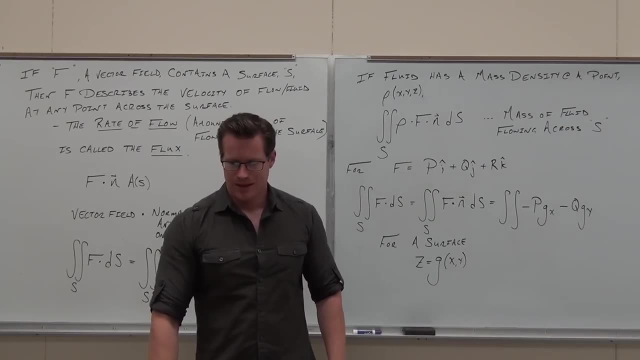 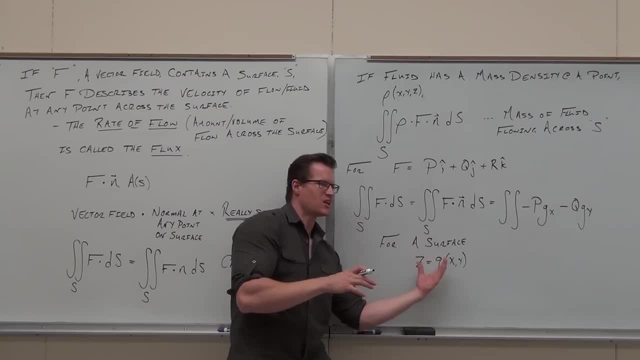 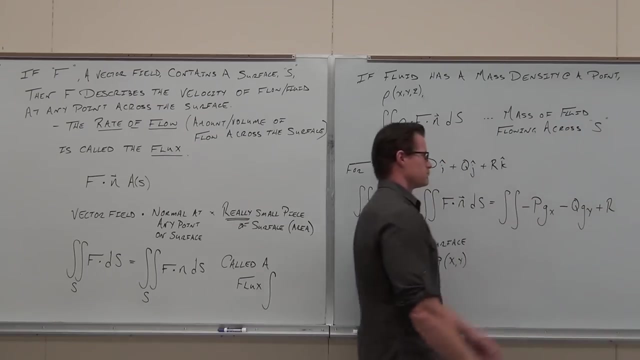 Y, Y, Y, Y Y. If I've defined the surface as z equals a function of x and y, can there be a partial derivative with respect to z? If there is, it's one. There is none for z. 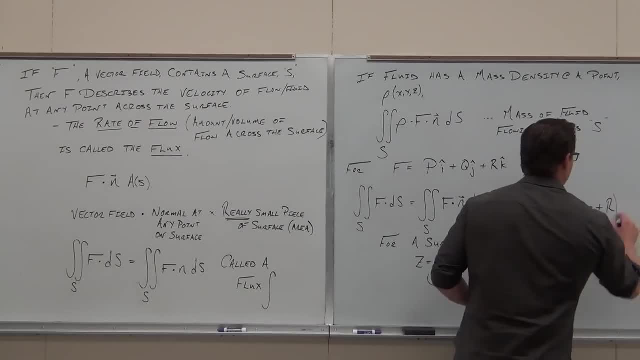 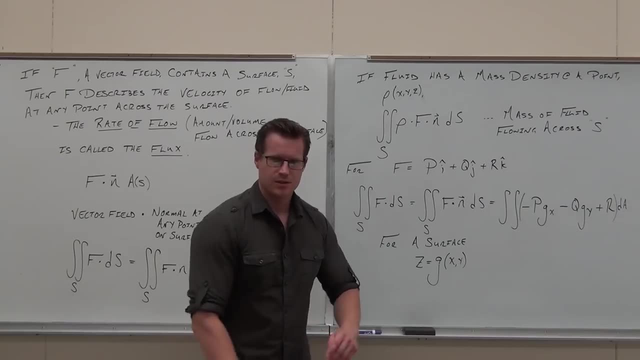 It's defined as a dependent variable. dA Over. I need to explain this to you. I'm going to use the letter d here, The letter d. listen carefully please. I don't want you to lose this. The letter d is the letter r. 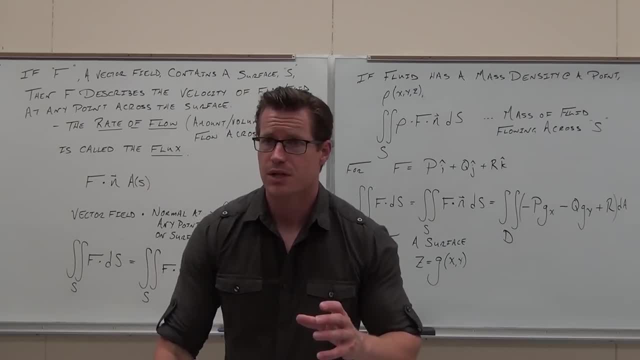 It's just the region, It's the projection of the surface onto the xy plane. Why the xy plane? Because we define this as z equals x and y. Does that make sense? It's on the xy plane. I can't use the letter r because it gets very confusing with that letter r. 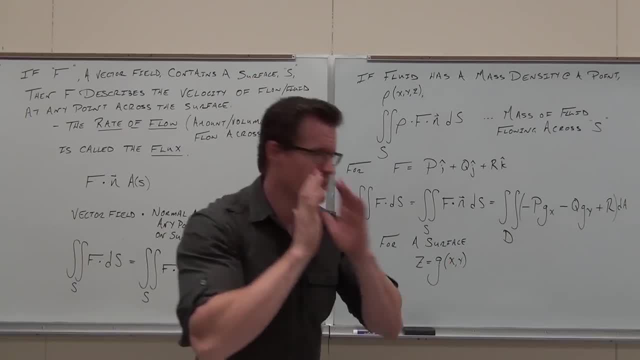 Does that make sense? You want to avoid that when you can. You don't use the same letters. So here's what this says: If you want to calculate a flux of z, you're going to have to use the same letters. So here's what this says. 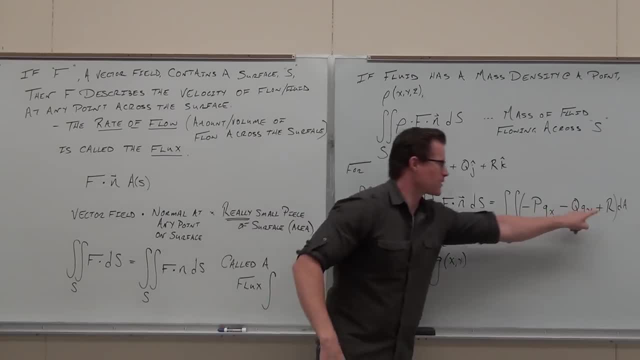 If you want to calculate a flux of z, you're going to have to use the same letters. So here's what this says. If you want to calculate a flux integral, all you have to do is this: You need a surface, which you'll have. 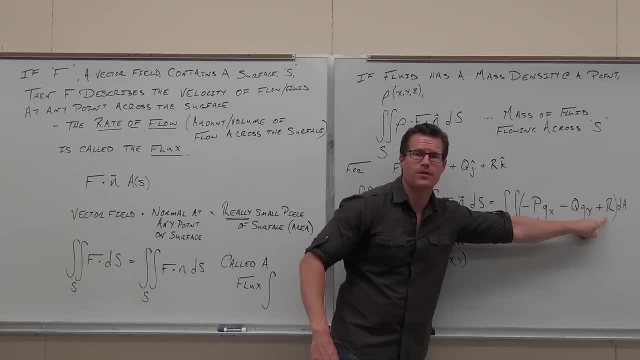 Just solve it for z. You'll need a vector field which you'll have, Literally, pqr, partial derivative of the space of x, partial derivative of the center at z. Come on, it's only going to take a few minutes. I've given you a little bit for the thickness, but it's going to take a few minutes, But we'll get to that later. So if you're using the sphere, what you'll have to do is you'll want to use the same. 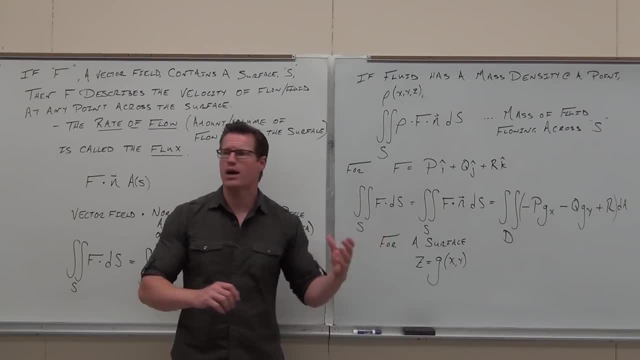 numbers. So here's what this says. So if you want to calculate a flux integral, You're going to have to use the same letters. Do a simple sequence. You'll need a vector field, which you'll have. You need a surface, which you'll have. 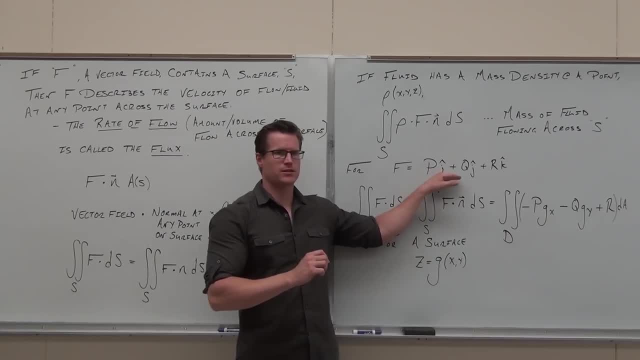 Just solve it for z. You'll need a vector field which you'll have, Literally P, Q, R, partial derivative of the respect of x, partial of the respect of y. You're done, And just look at what the projection of your surface is doing on the xy plane. 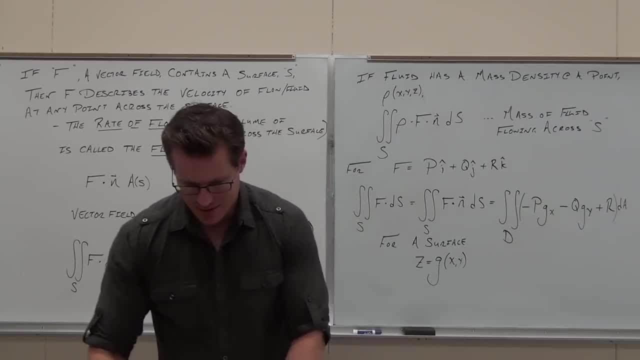 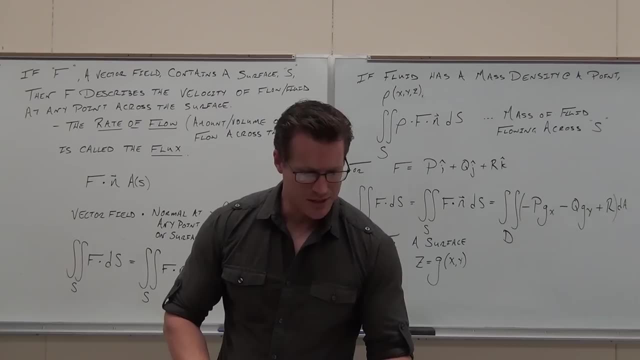 Okay, now, if you're okay with that, that's it. Now we've got some time, Sweet, Let's do at least one example, and then we start getting to the last. This is crazy, the last two theorems ever for you guys. 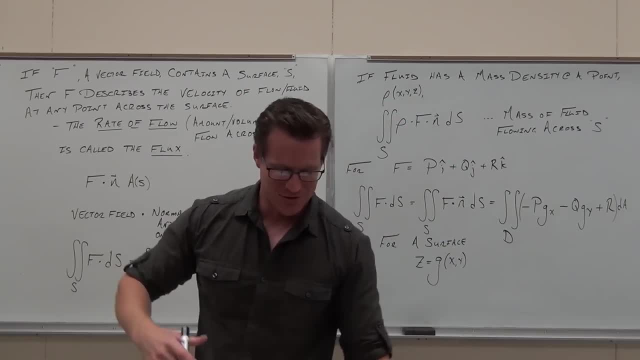 This is so nuts. Oh my gosh, it's blowing my mind right now. It's so good. After all this work, we're coming down to the last part. So did you catch what d is? What's d again? 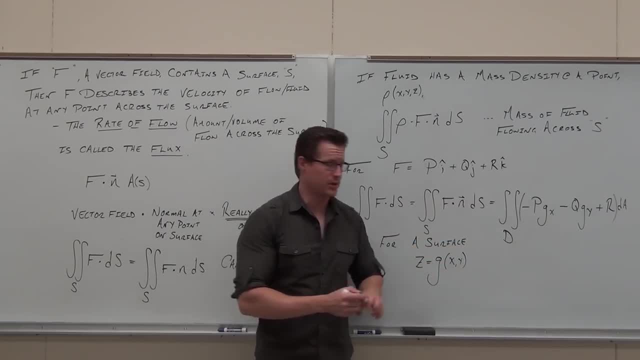 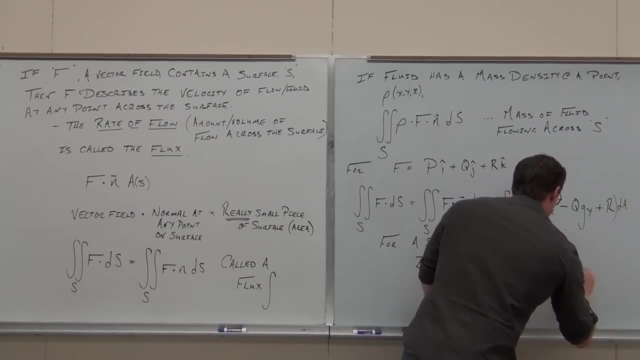 The projection of this surface onto the xy plane I'm 1, g 1,, 2,, 3,, 4,, 5,, 6,, 7,, 8,, 9,, 10,, 11,, 12,, 13,, 14,, 15,, 16,, 17,, 18,, 19,, 20,, 21,, 22,, 23,, 24,, 25,, 26,, 27,, 28,, 29,, 30,, 31,, 32,, 33,, 34,, 35,, 36,, 37,, 38,, 39,, 40,, 42,, 34,, 35,, 47,, 48,, 40,, 49,, 50,, 51,, 51,, 52,, 53,, 54,, 45,, 56,, 57,, 50. 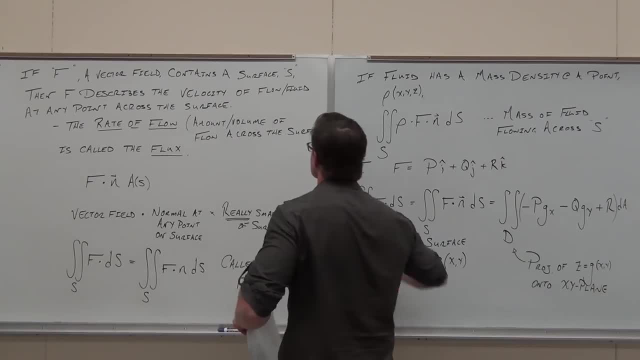 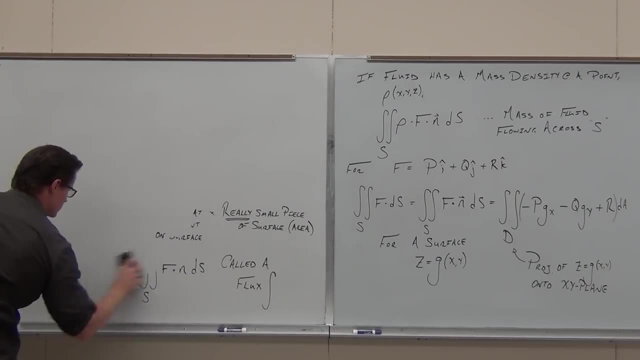 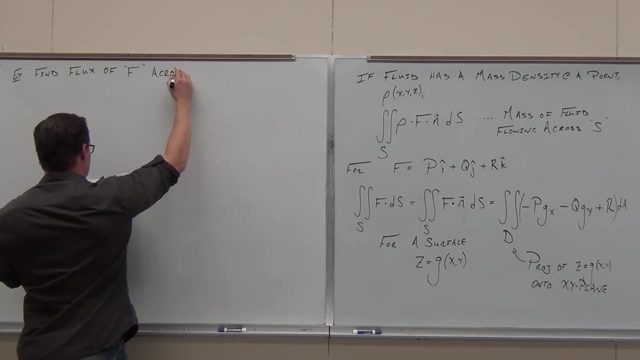 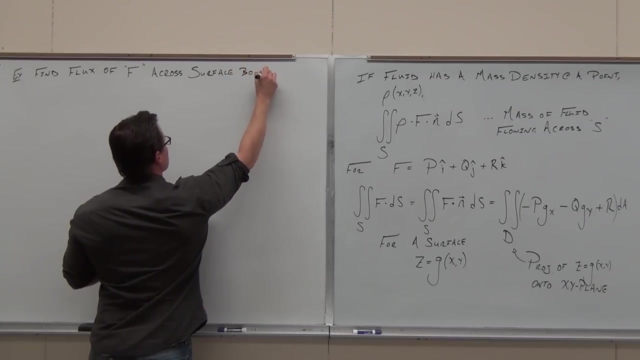 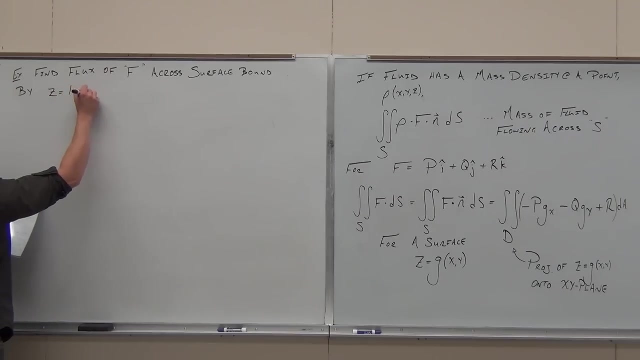 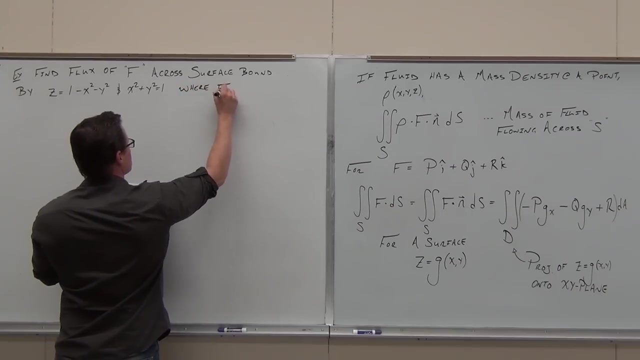 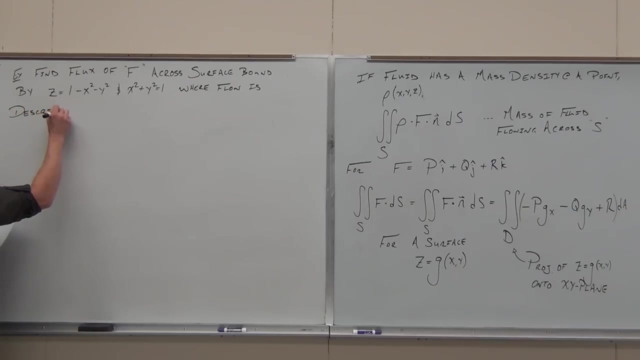 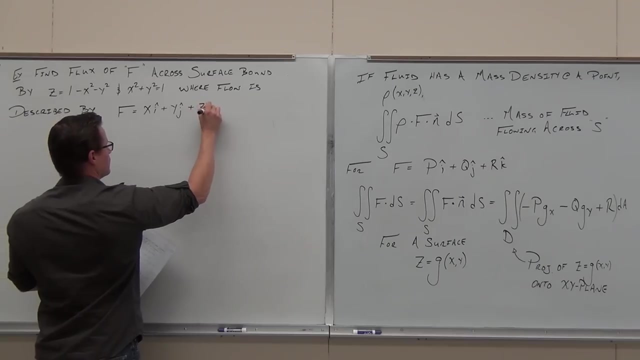 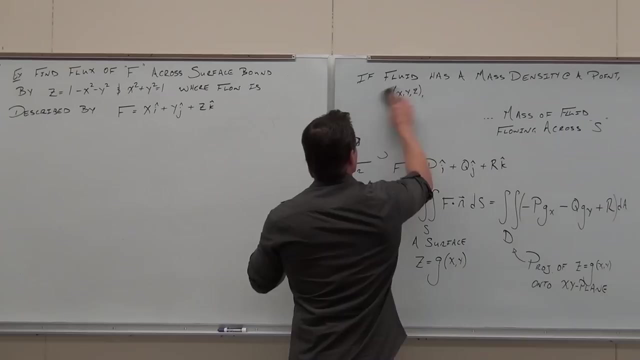 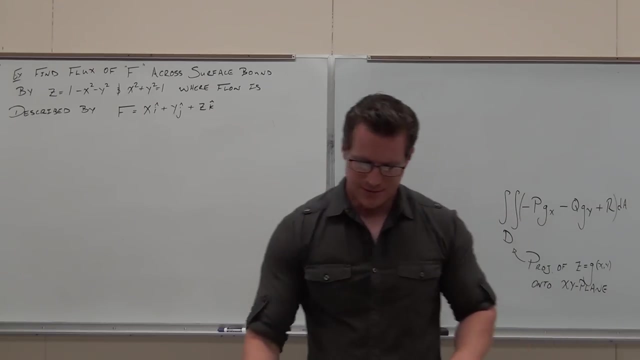 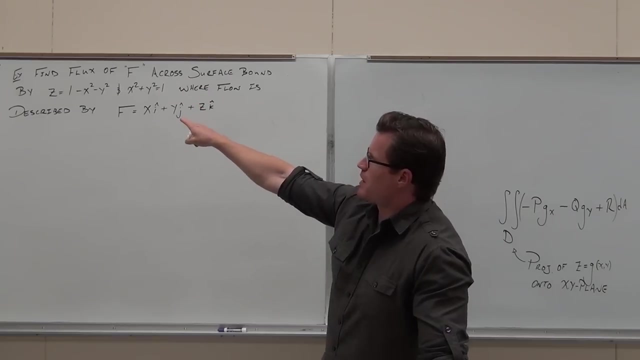 So let's give it a try, Okay, Thank you, Thank you, Thank you. Okay, let's give it a try. We've got to find the flux of the vector field across the surface, which is The surface bound by those two functions. 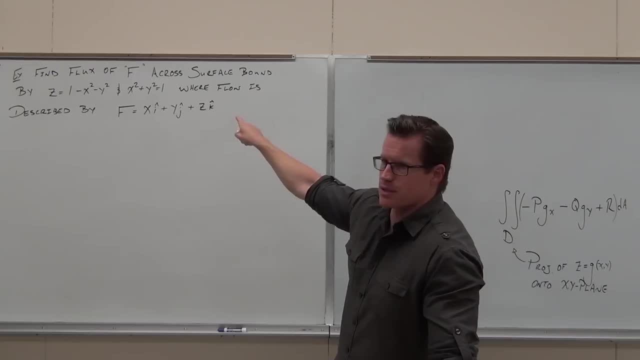 where the flow is described by that vector field: xi plus yj plus zk. Do you guys understand the idea of what we're about to do? So we're trying to find the flux integral That's going to give us the amount of flux there. 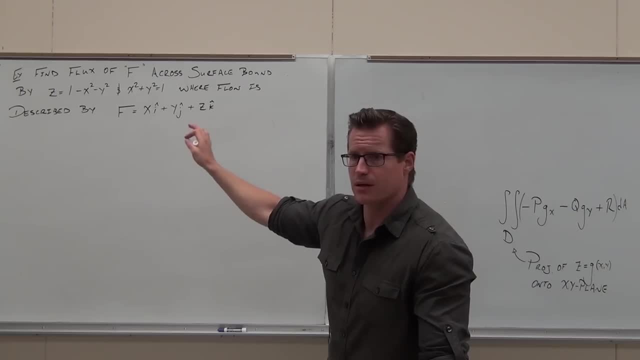 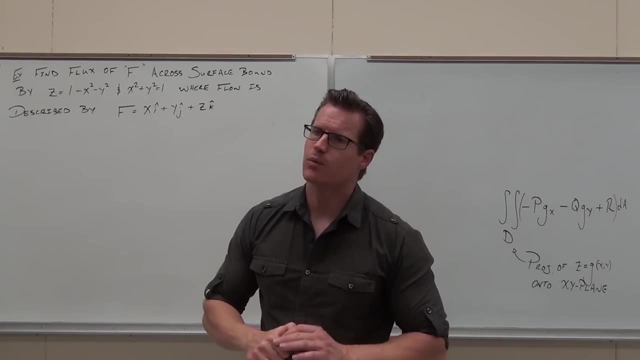 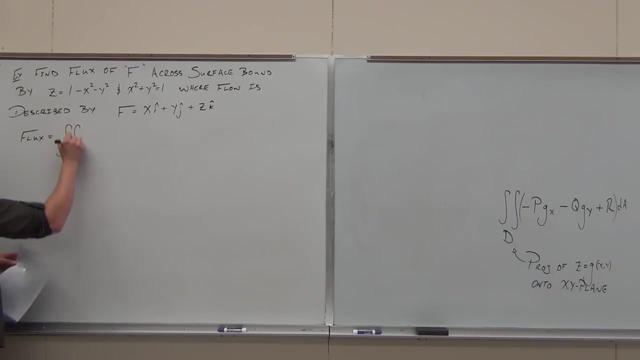 We're not talking about mass here, just the amount of flux across that surface given by that vector field Make sense. That's what we're doing. How you start Number one: write out what you're trying to do. Flux A flux integral is originally that. 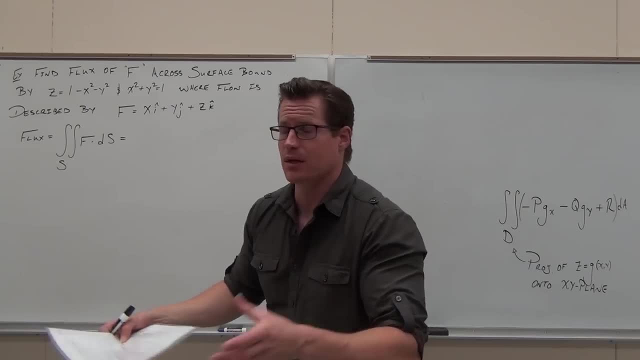 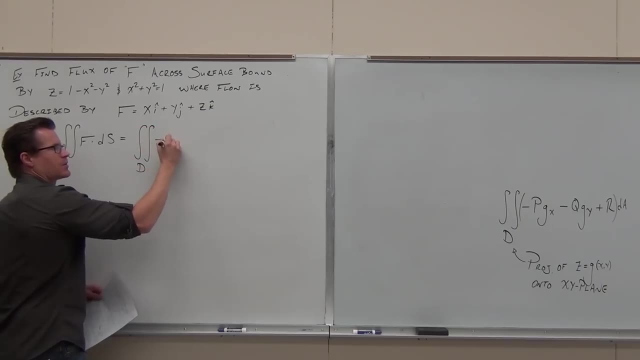 It's a surface integral through a vector field. That's all that's happening. But we have a formula for that. now The formula says: okay, this is the idea, but the how we do it says: I want to find p times the partial derivative of g. 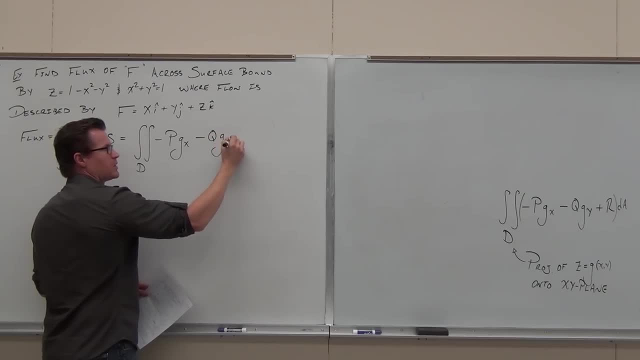 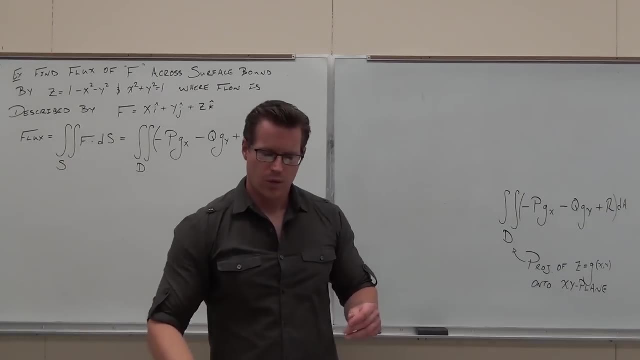 with respect to x minus q, times the partial derivative of g with respect to y plus r, and then da. This is our goal, This is what we're trying to find. So, right now, what I'd like you to do, what I want you to do, is: 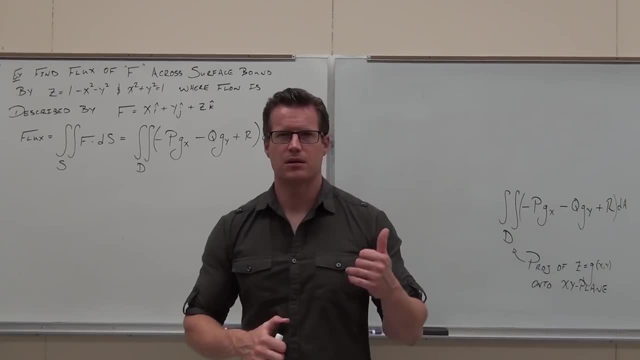 from your vector field, you should be able to identify p, q and r. It should be really easy right now. Can you identify p, q and r? Maybe just write a little letter above them: This is p, this is q, this is r. 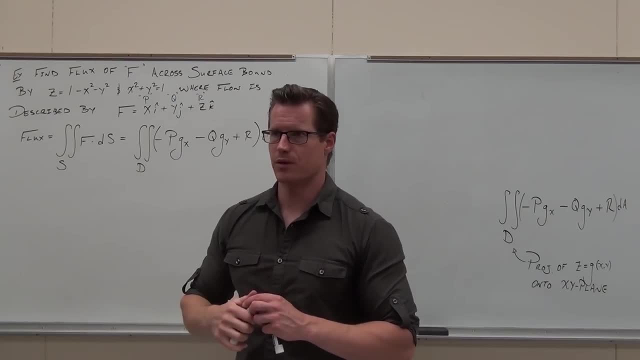 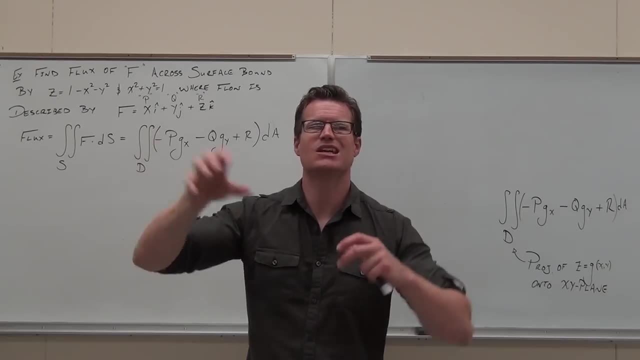 Your vector field always gives you the p, the q and r. I had not mentioned with me on that one. Okay, next step, we also need a surface and we need that surface to be defined for us as z equals some something in terms of x and y. 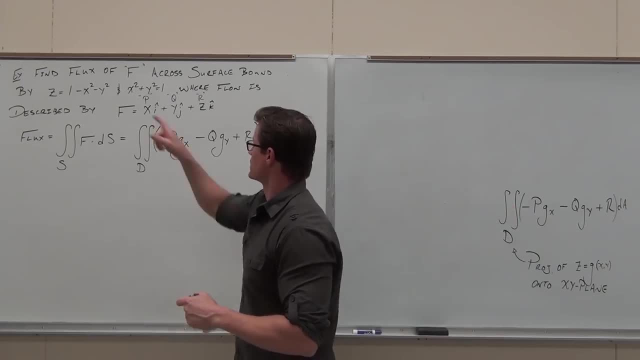 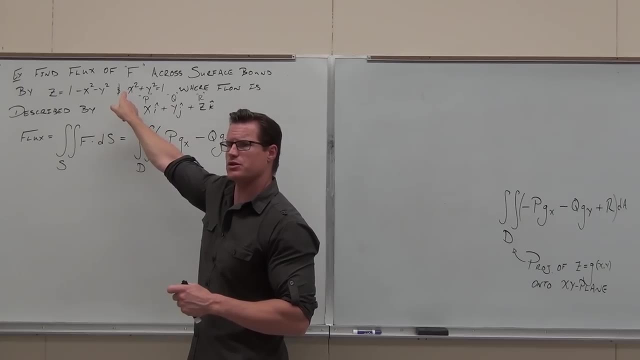 Do we have one of those? Okay, so which one does? this one? This one? Okay, what about that one? Does it matter for us so much? It's not going to matter right now, but it's going to matter for the region. 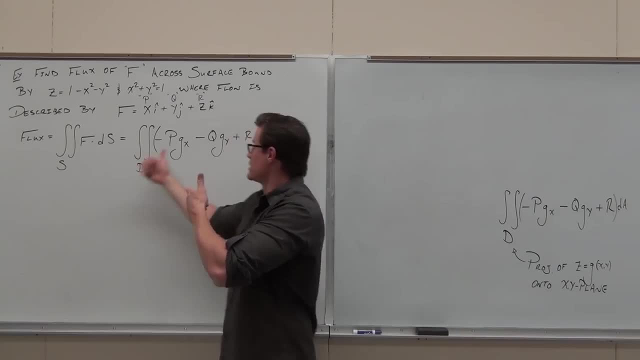 It's going to matter, for I'm going to call it the region. That's what it is. We just have to use d. I don't want to do that, Okay. Okay, I don't want to mess up the r. 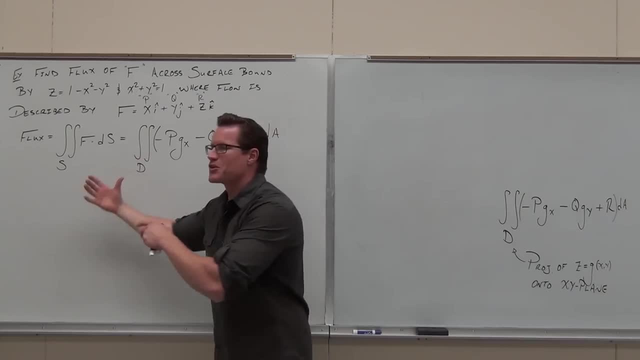 So that is our region. We're going to do that later. Again, it's all about the set up first. then you look at the region. So let's just find the only function up there that has a z in it. That's the function. 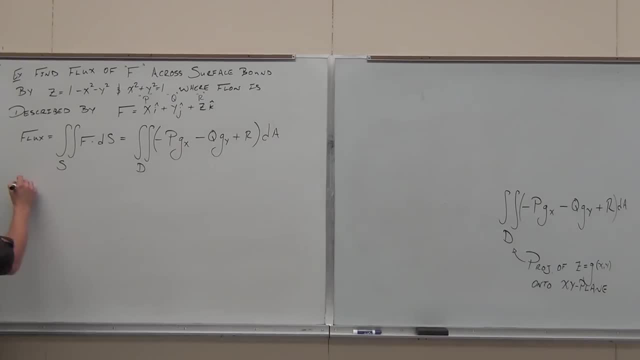 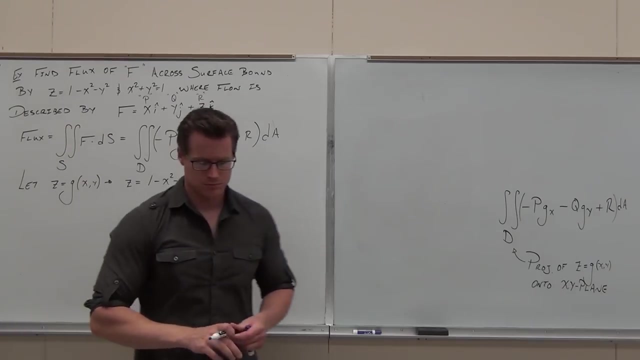 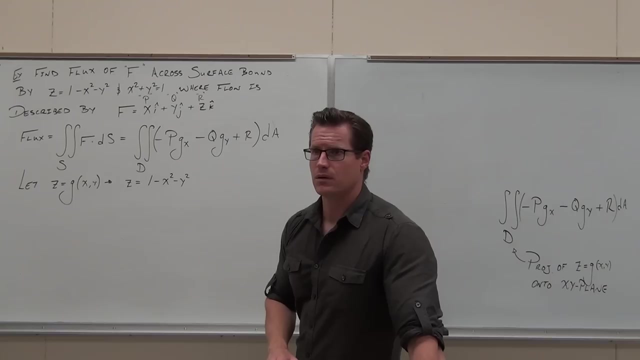 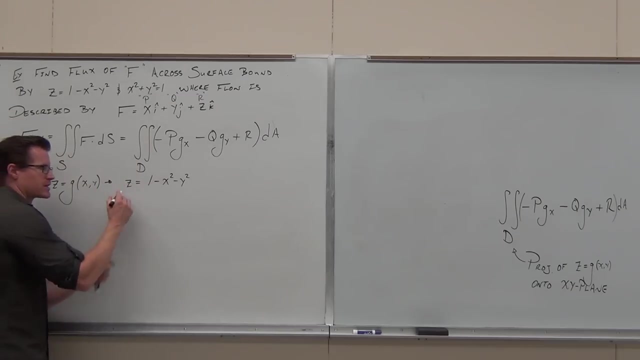 So let's let z be a function in terms of x and y. That means for us, z is this function 1 minus x squared minus y squared. Are you okay with that? Hello, yes, no, yes, okay. Well, if z's are our g function and z equals this, then our function in terms of x and y. 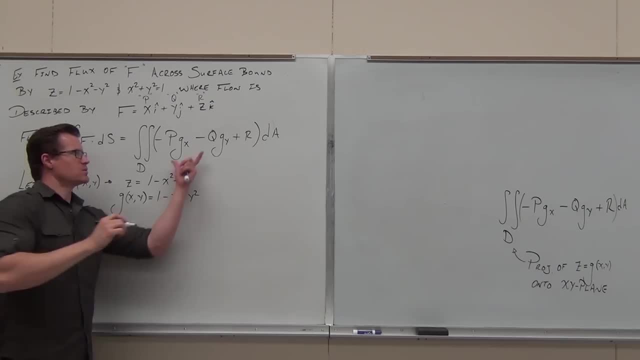 it's just exactly the same thing, but it allows me to use this stuff. It allows me to take partial derivatives with respect to x and y. Notice there's just x's and y's, So I want to right now find the partial derivative of g with respect to x. 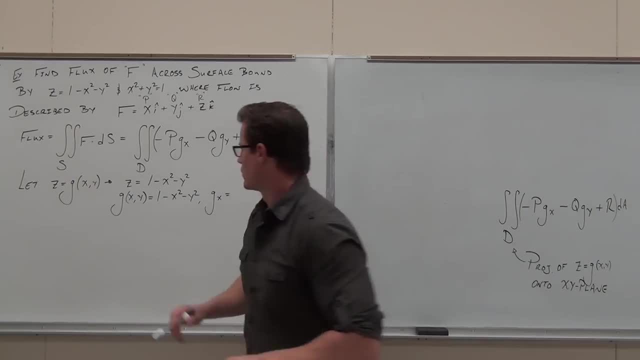 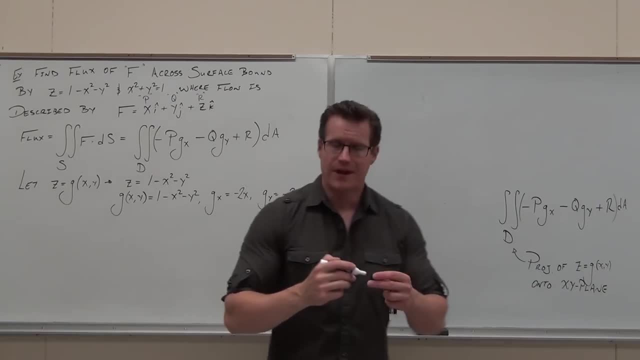 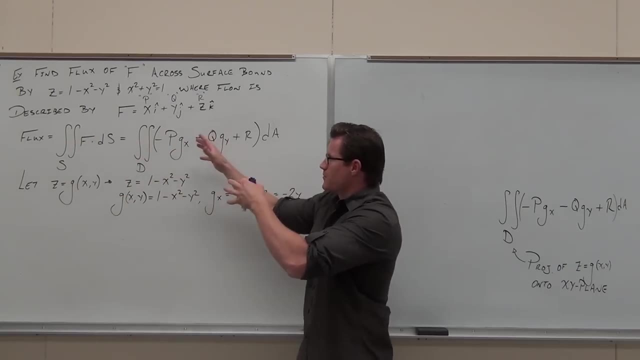 Negative. That's it. So the vector, look it's nice. The flux integral is nice. okay, You take your flux integral, but you've got a nice formula for this, Given by a super cool region, just a projection onto an xy plane. 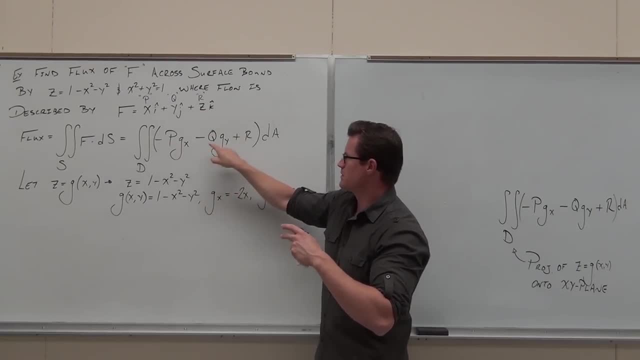 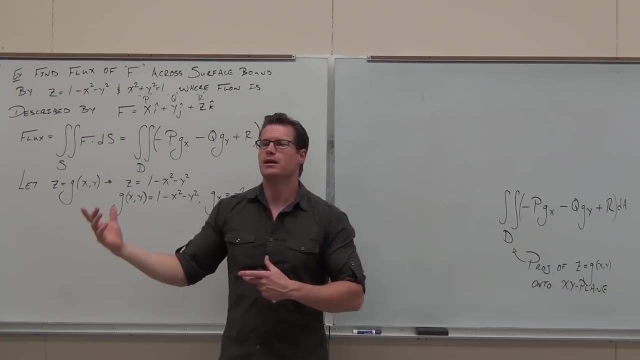 You have p, you have q, you have r from your vector field. You have g, well, partial derivative of g with respect to x and with respect to y, from whatever function is given to you. So we take our partials, just plug them in. 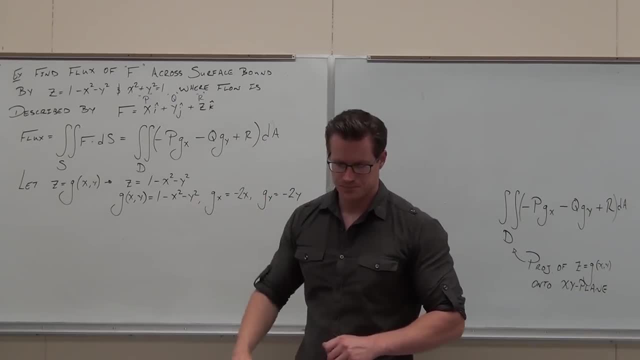 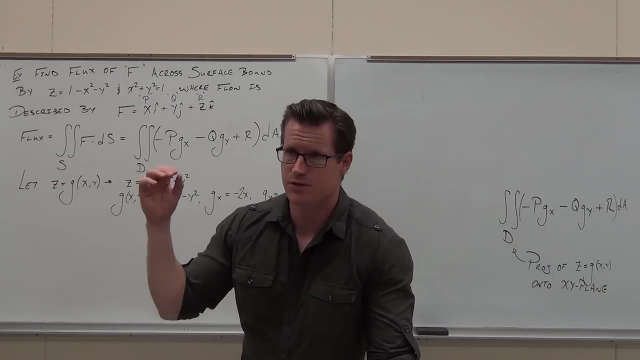 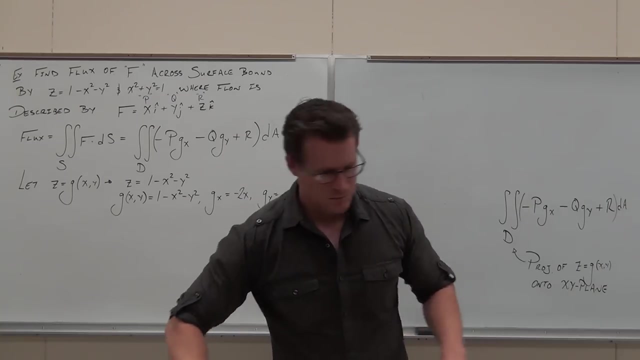 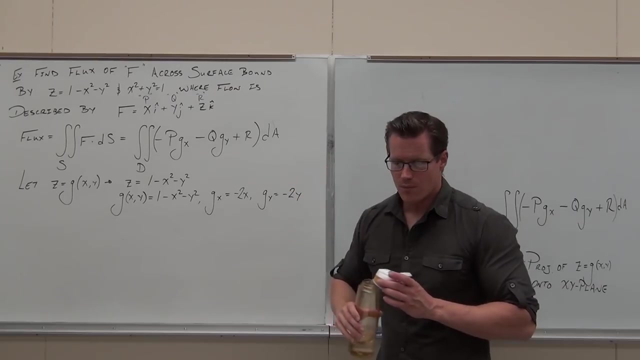 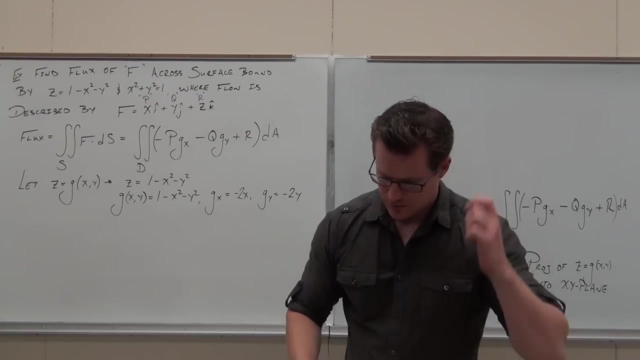 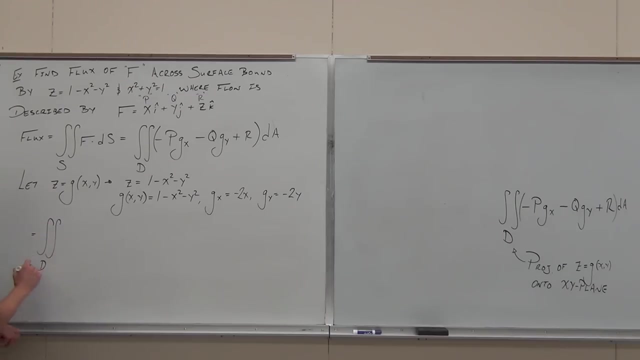 See if you can do it. Once you take your values, plug them into that. By the way, have we even looked at our region yet? No, Don't even worry about it until you've simplified your double integral. Let's see. 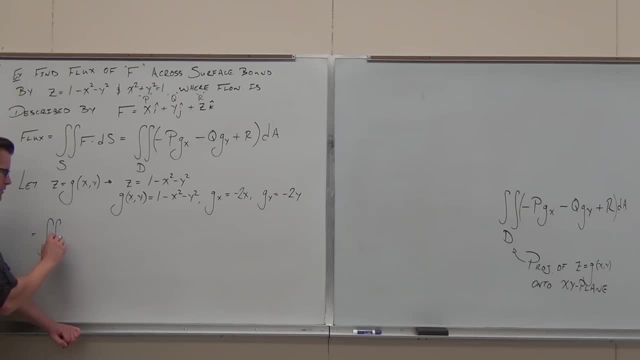 What should we have? What do we start with? I'm not going to do any simplification with my hand. We'll put everything on the board, because you know this about calculus, The biggest mistakes are sign errors, simple things. What do I have? 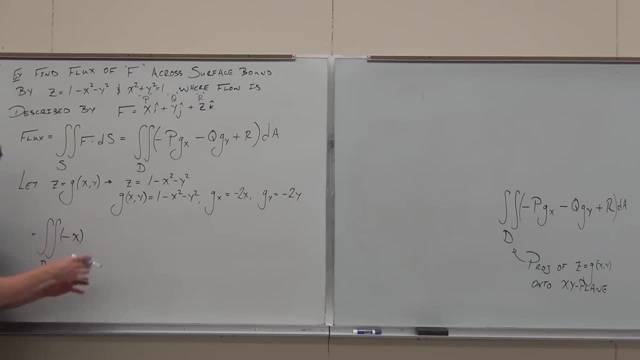 Negative- I'm going to put it in parenthesis because I'm multiplying it and you know it's negative. x. Then what Are you noticing? the x components go together Minus. what's the next thing? Y, Y from here. so negative, I have the minus. 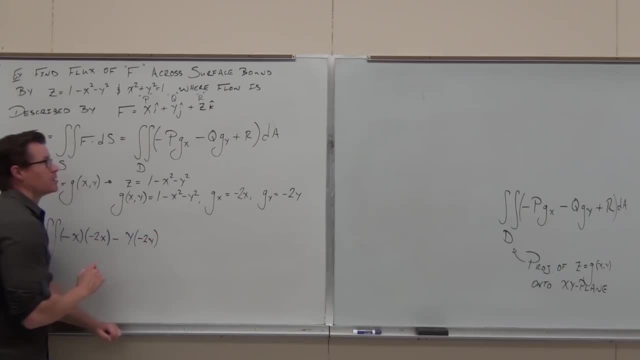 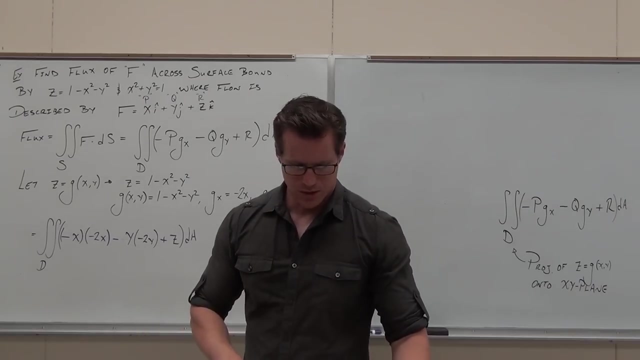 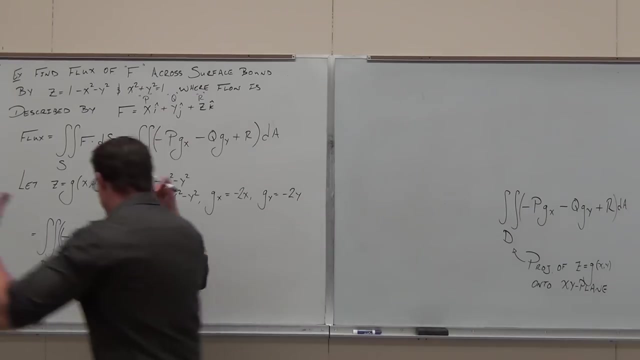 Y and then, And then plus r, What's our r Z? Are you still okay with it? Hello, yes, ma'am. Yes, Let's do ourselves a favor, Let's start simplifying this thing. If we start simplifying this thing, then we have a double integral. 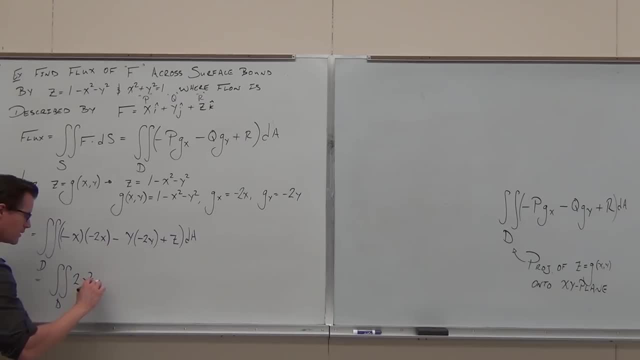 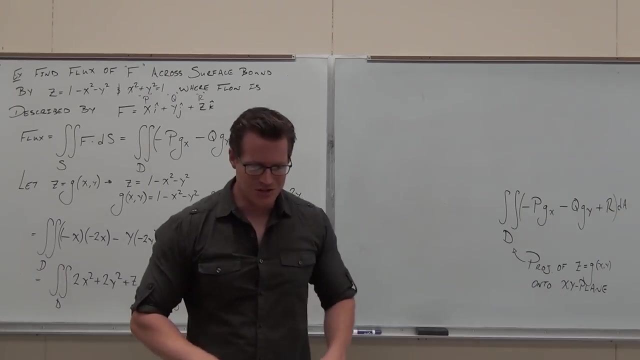 Here's d, just our region. We've got 2x squared plus 2y squared plus z dA. Are you still with me? I'm going to factor out the 2. Why? Because I want to Now. you know enough about math in this class to know. 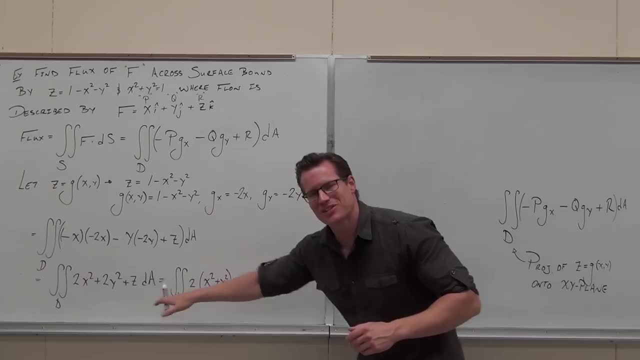 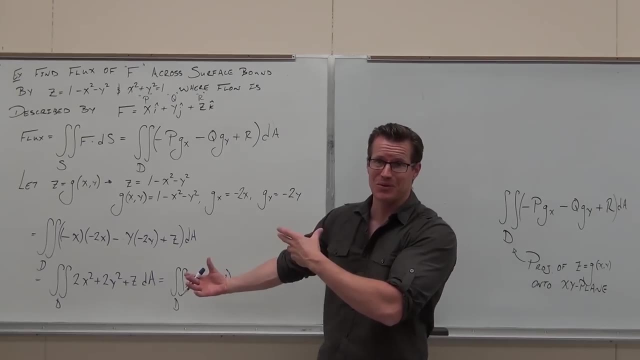 that there's something seriously wrong with this picture. What's seriously wrong with this picture? Because of z. Why? Why is the z bad? Because we've got two integrals and three variables. Oh wait, a second, wait a second, wait, a second. 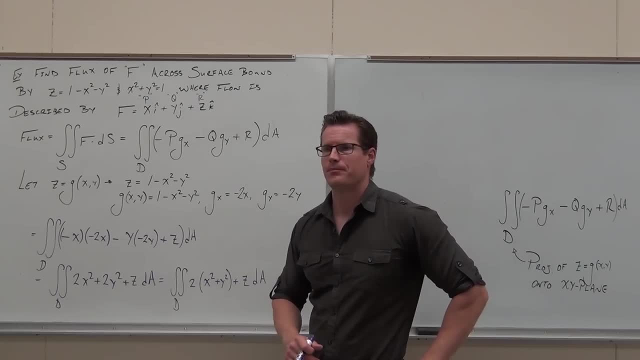 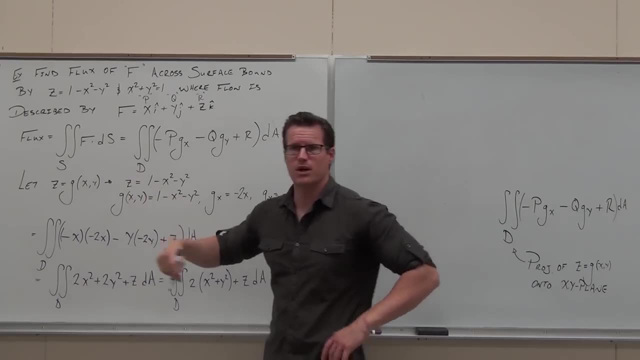 Which variable needs to go: A, X, y or z. Z Why? Because we're on the xy, Because you chose z as a function of x and y. Just plug it in, Just change your z, Whatever variable you have. 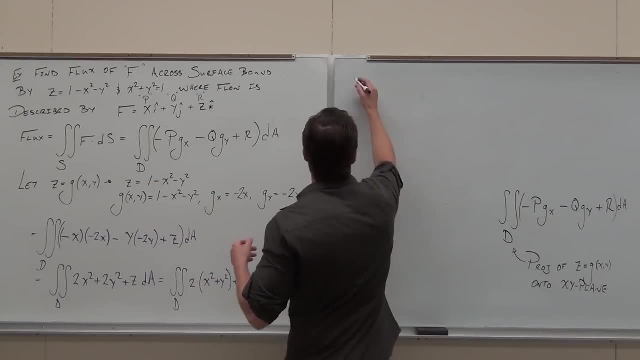 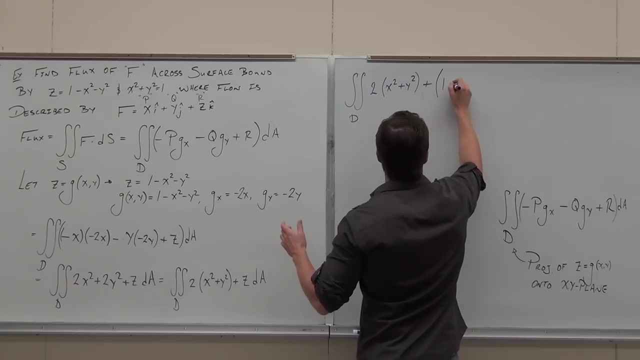 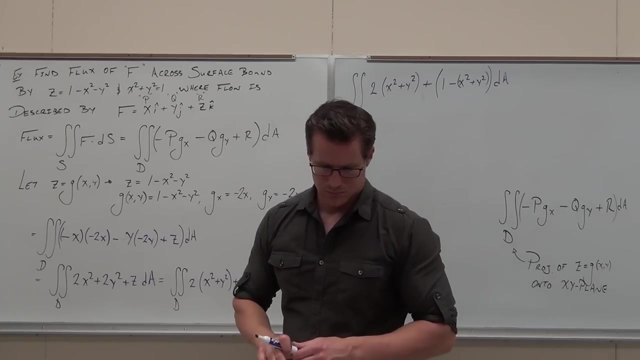 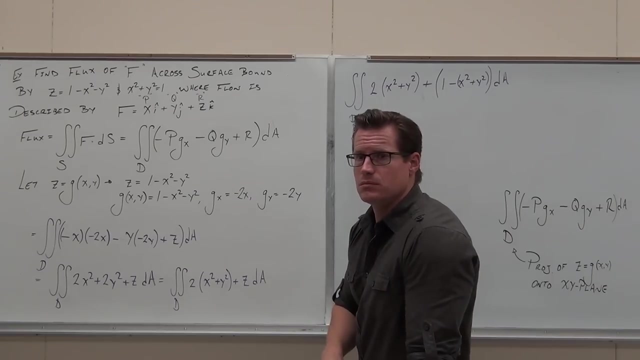 Hey, you should have a function in terms of the other two. Change it. If z is this whole thing, It gives us something. If z is f, z is nothing but x, Well, 9.. We know where the solved figure is. 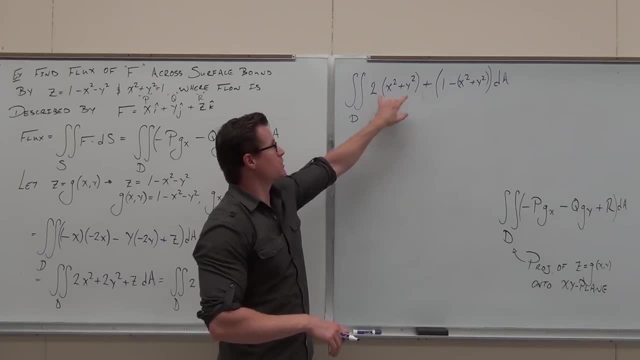 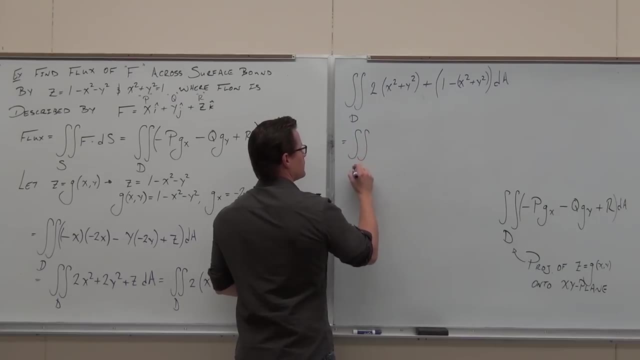 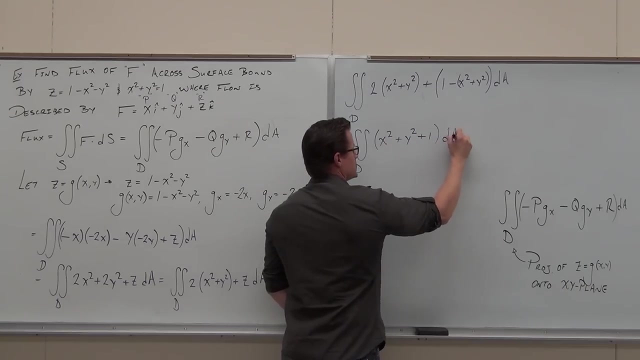 Well, now you can simplify it. Hey, you got this was factored, but you got 2 of these things minus 1 of those things. So can I simplify it one more? You've got one of those things plus 1, dA. 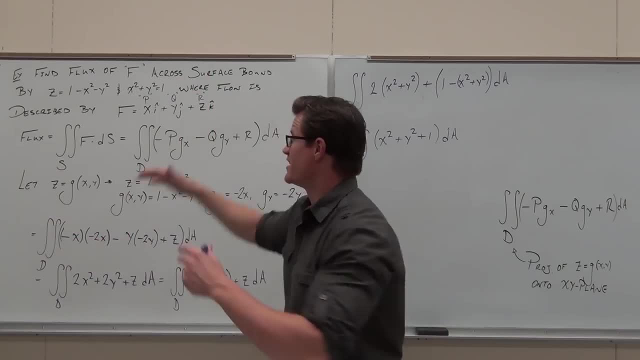 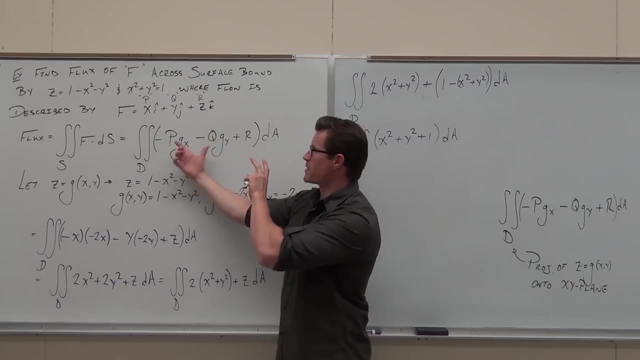 Should have answered for that one. Now, we've done all this work. We said, hey, flux integral or surface integral through a vector field. yes, We have redefined it by the formula that I gave you. We had vector field. 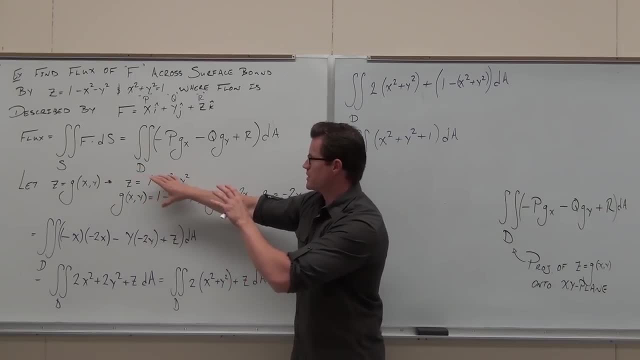 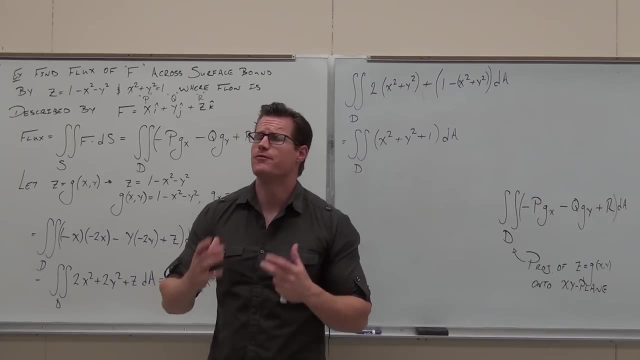 We used p, q and r. We have a surface. We defined it in terms of x and y. We took a partial derivative, We plugged in the formula, We simplified, We simplified, We simplified. Now you have a very basic double integral over a region. 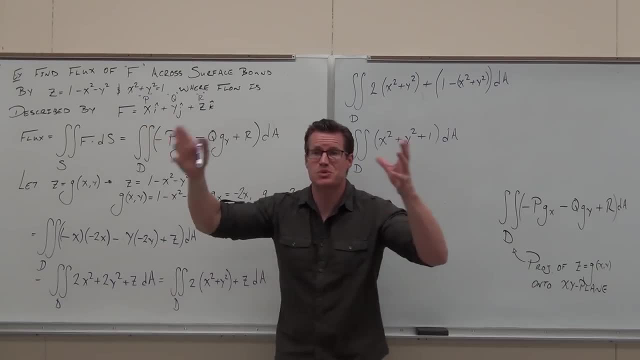 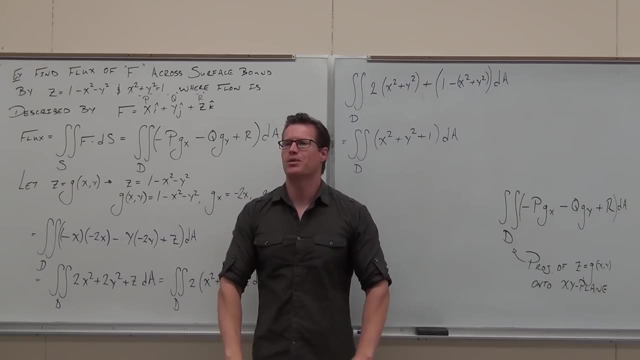 All you have to do is look back at what's given your surfaces, And here's what's happened. You go: hey, let's look down on top of the surface, Look at what's happening between these two surfaces and draw it on what plane. 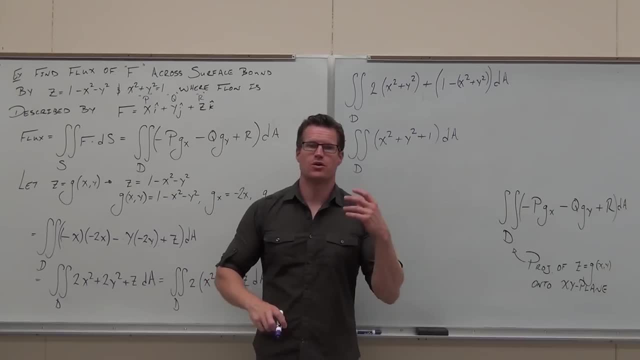 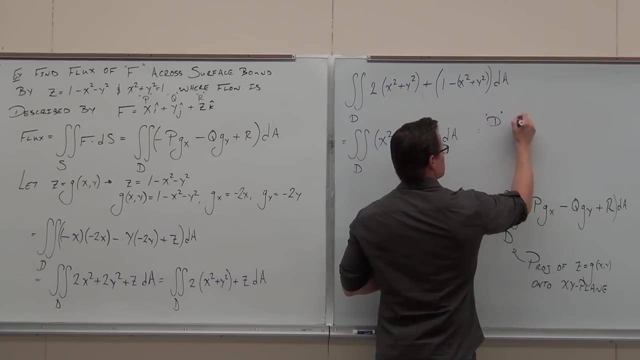 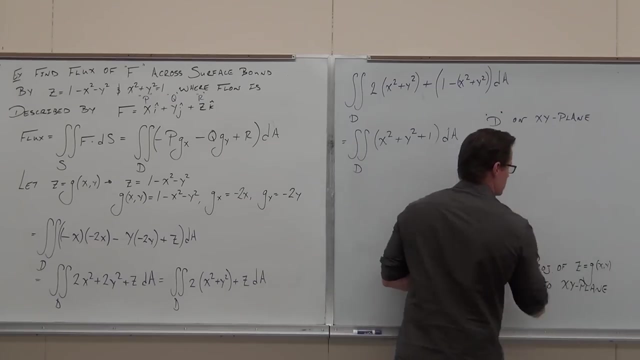 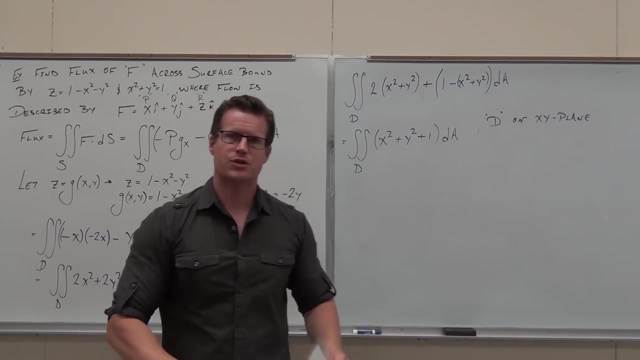 Come on, people, what plane You're basically doing? z simple, Your r, your d, in this case, should be on the xy plane. So d It's on the xy plane. I want to show you something, because some of you guys. 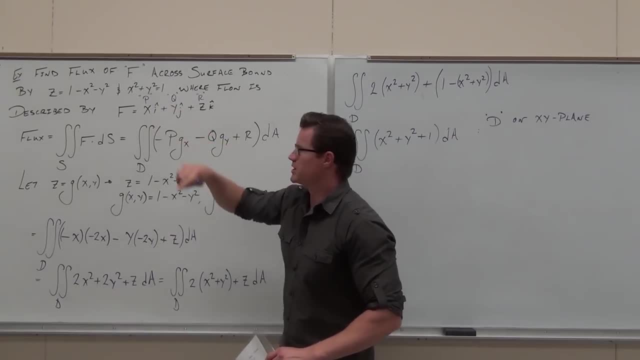 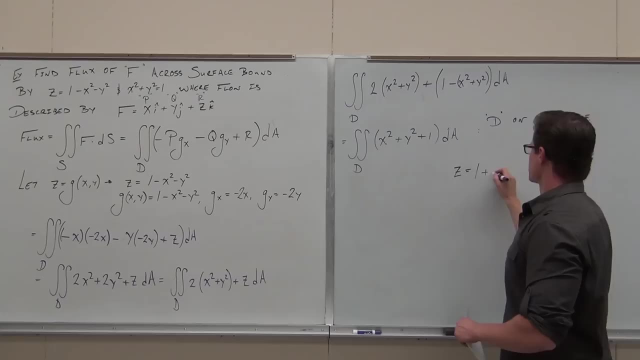 are going to try this. You'll go wait a minute. This is the surface bound between two things, So you should clearly set them equal to each other. So if I have z equals 1 minus x squared plus y squared, And I also have x squared plus y squared equals 1.. 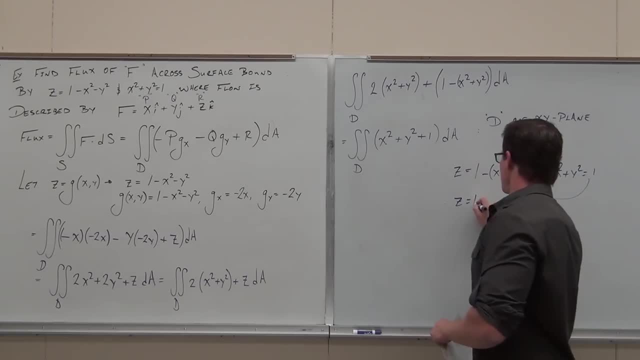 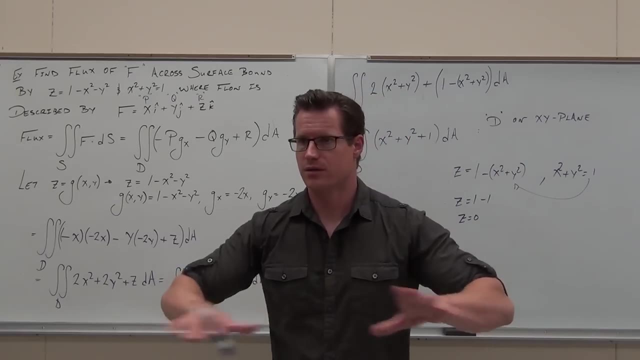 Then I should be able to substitute this, And so z equals 1 minus 1.. z equals- oh crap, What happened? That just means that your intersection is on the xy plane, Which means that your level curve, that you're getting there. 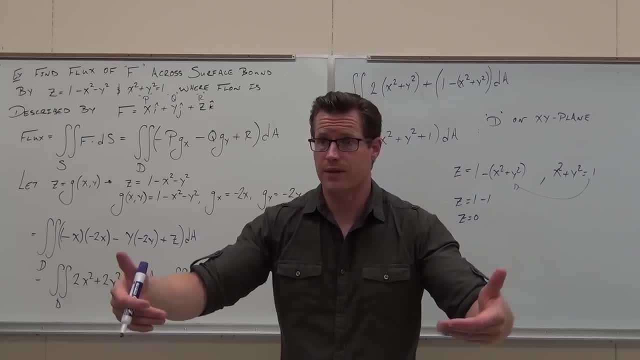 is literally on the xy plane. So don't fret. If it's on the xy plane, then z is 0. Just plug in z equals 0, and you'll have a very nice picture of that. Does that make sense to you? 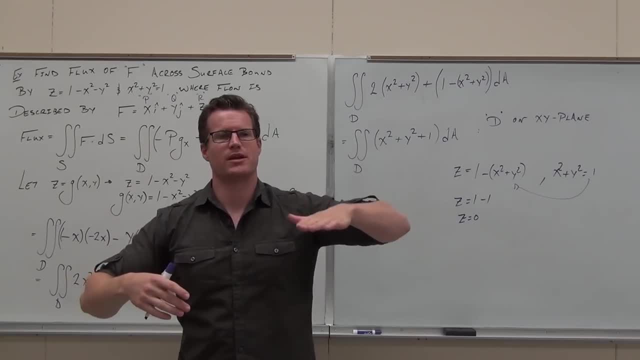 So if your intersection is like it 0s out, what's that mean? It just means your picture's on the xy plane. So basically just draw this Or plug in 0 and draw that, Because you know what You're going to get- the same thing. 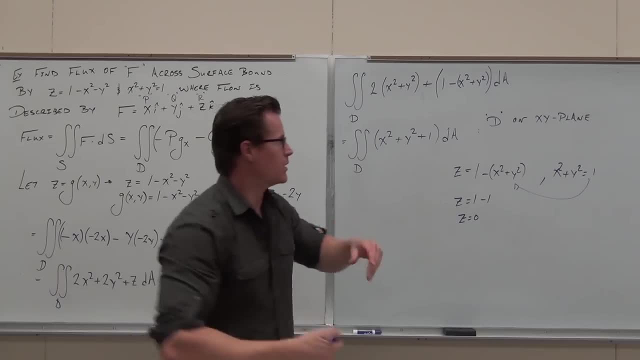 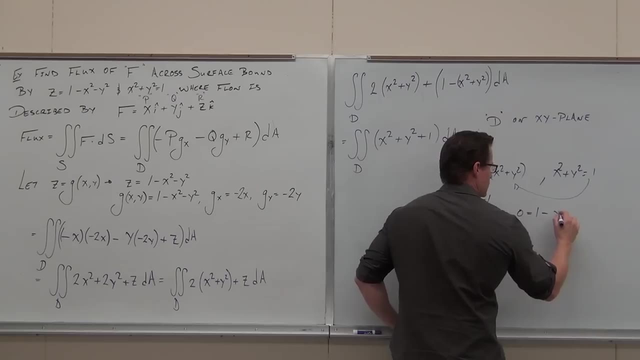 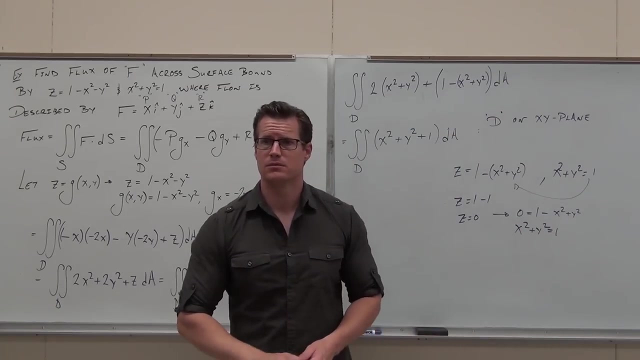 Because it's literally meeting on the xy plane. Does that make sense to you? So z equals 0, whatever, That just means that this is 0.. Can you draw a picture of that? What picture does it give you, Circle? 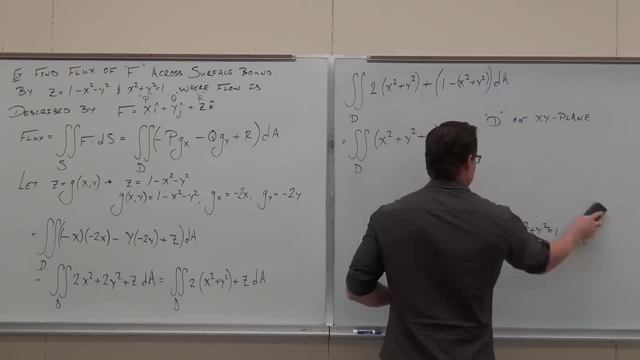 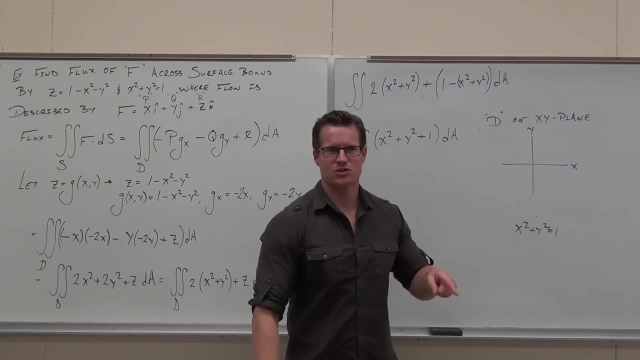 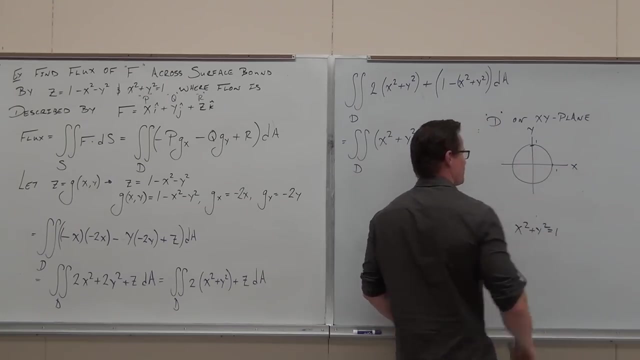 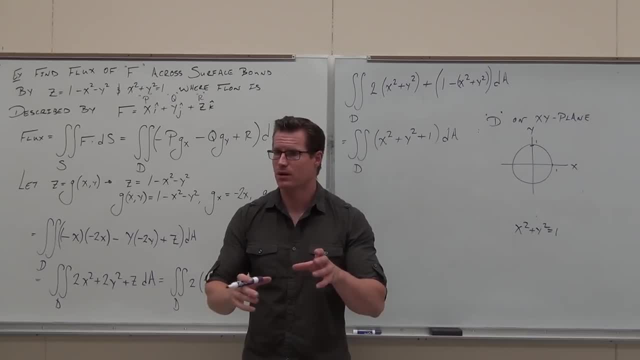 That's your region, That's what that is, And I feel good with that. So, oh hey, What do you do with circular regions? This is why you don't define this stuff until you get your region, because you can start doing all this work and trying to define X and Y. 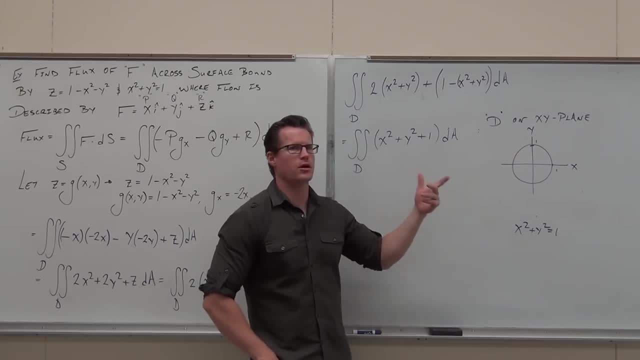 but you don't even know what it's going to look like yet, So you simplify all the way down. Let's draw the region now. It makes our work a lot easier. Well, if this is, R equals 1, and that's a full circle, then here's the point, though. 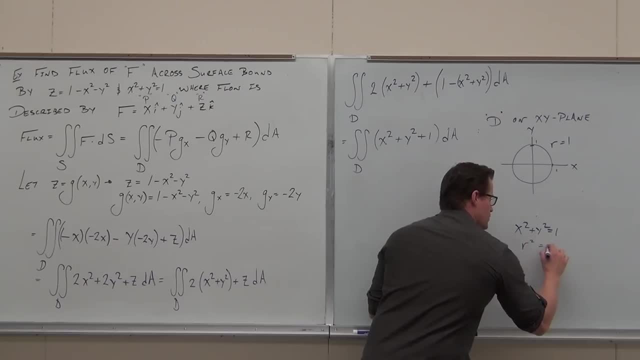 that you need to do this As soon as you let this equal R squared. as soon as you do that, then you're automatically calling X R cosine theta and you're calling Y R sine theta. You have to have those pieces, okay. 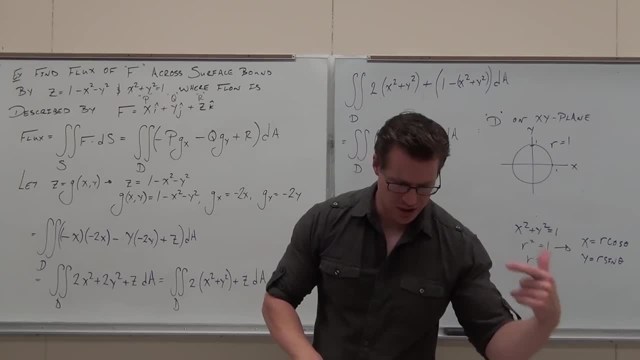 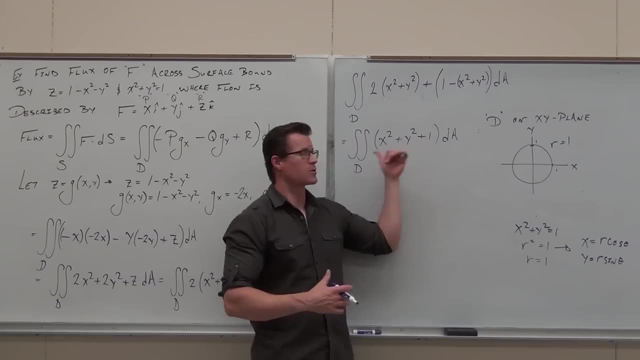 That matters. That's there. So if you have to use that later to change your stuff, then you need to have it. I write it out every time, Even though we're not going to use it here. you write it out because if you didn't have X squared plus Y squared right there, you'd have. 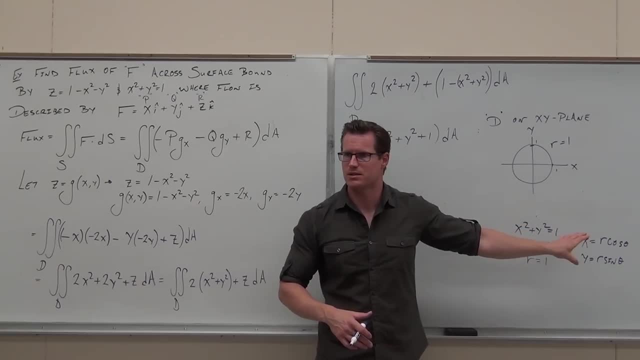 if you just had X and Y, you'd have to have those two pieces. I wanted to show you that. Does that make sense? So here we go, Hey, hey, we just defined this in terms of polar. Fix your double integral, please. 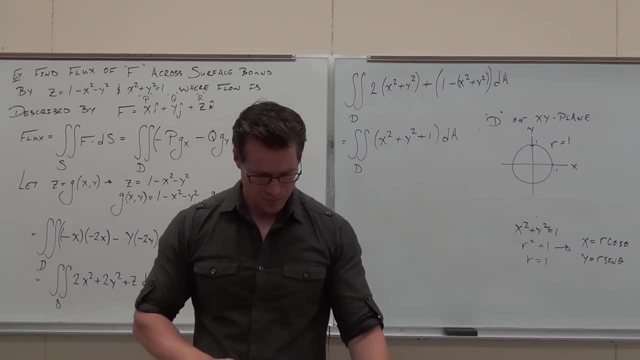 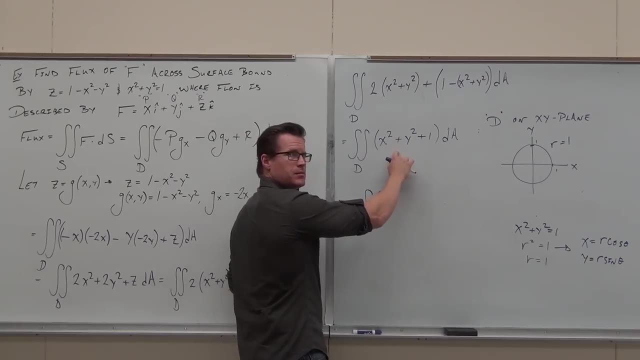 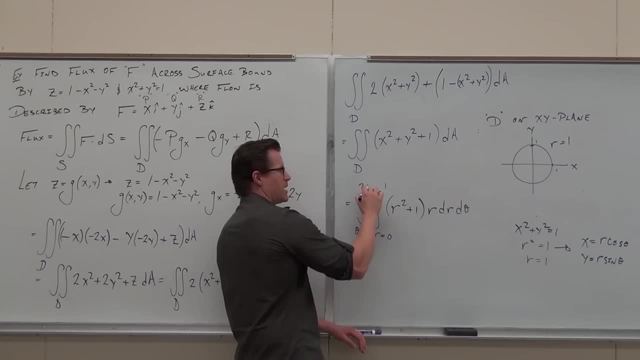 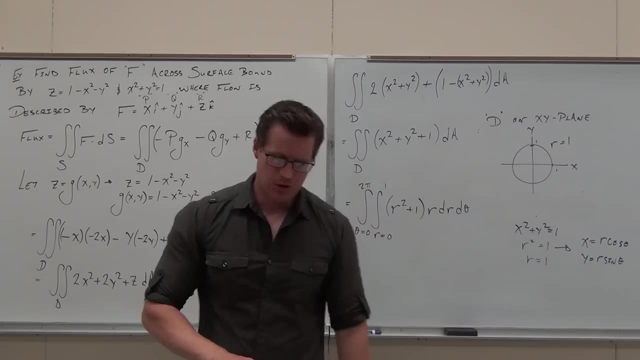 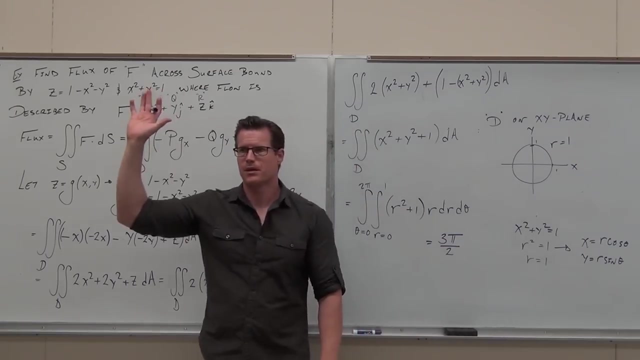 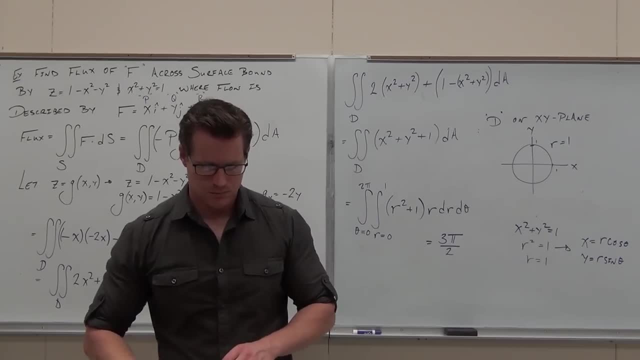 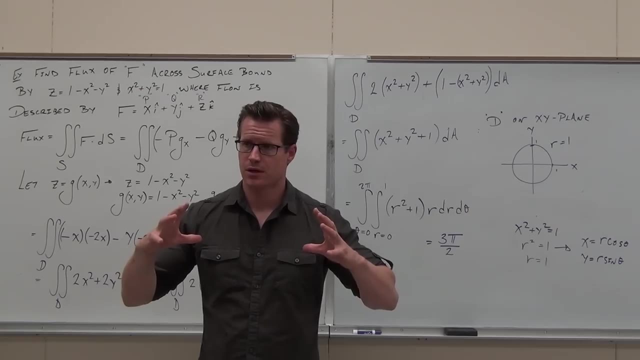 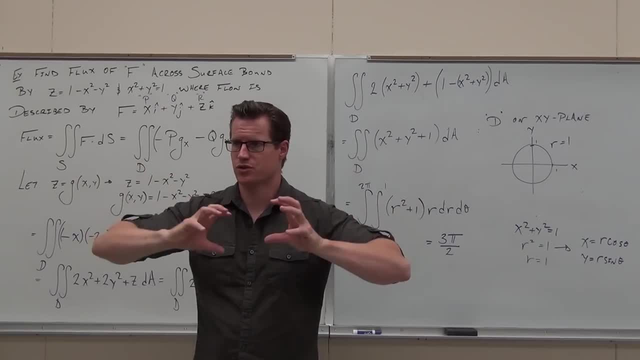 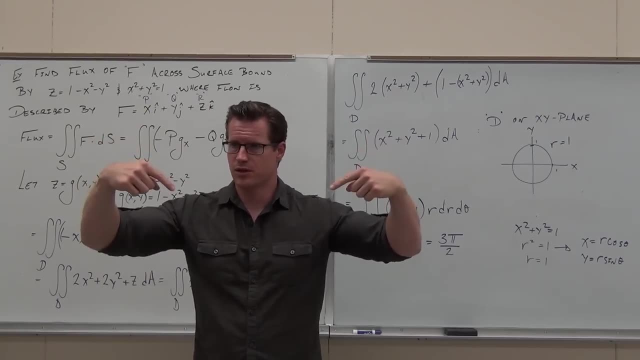 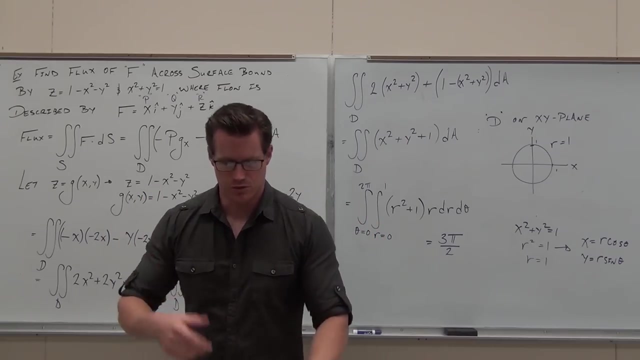 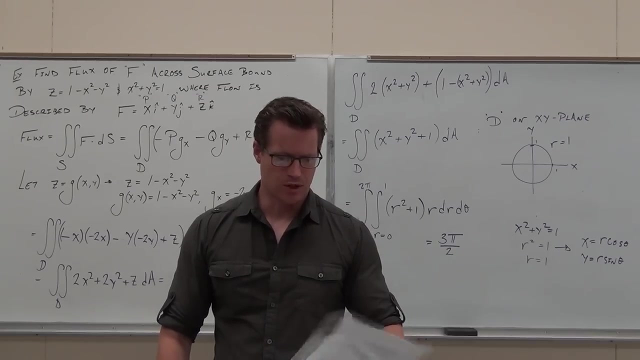 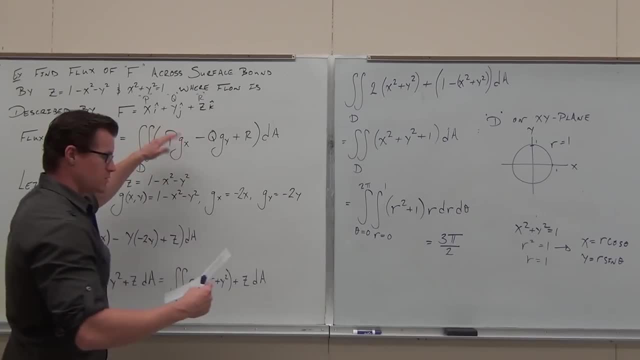 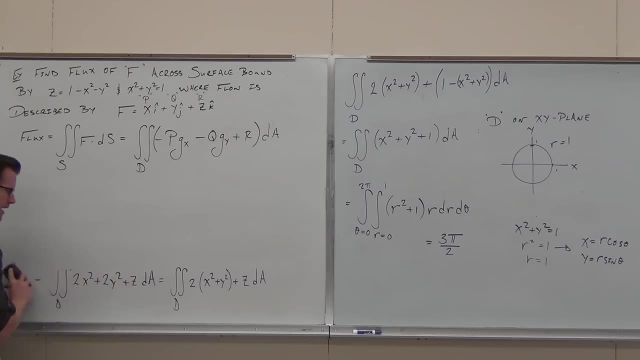 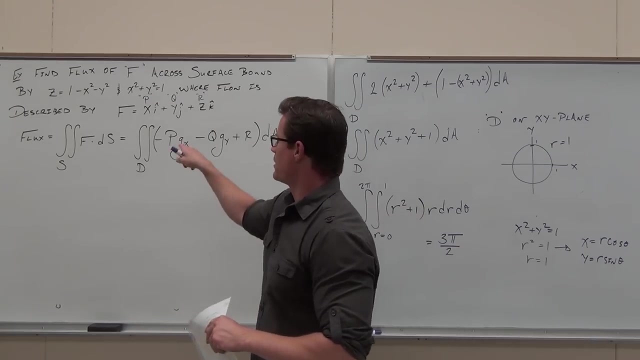 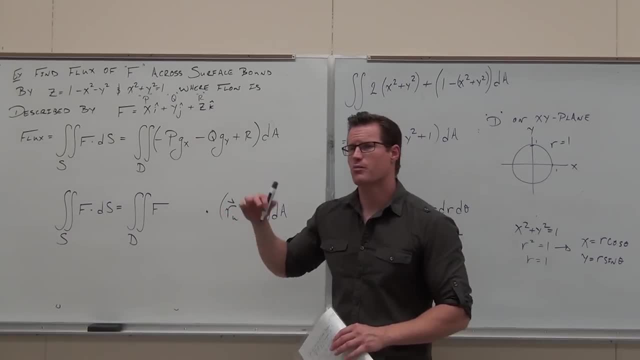 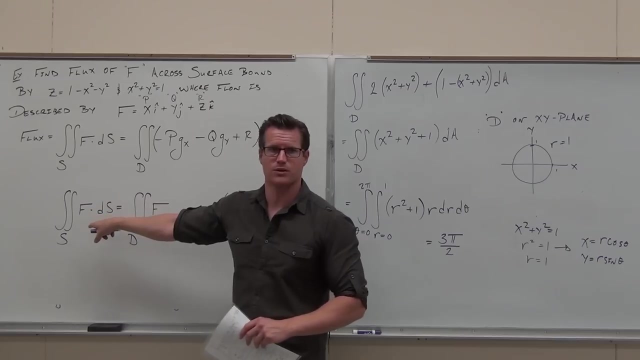 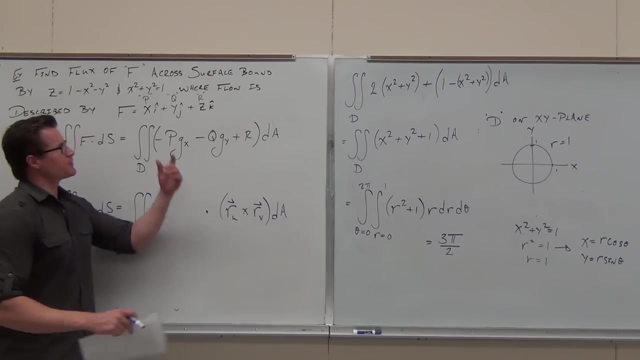 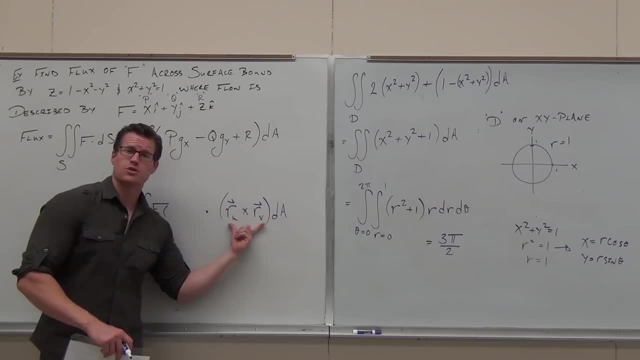 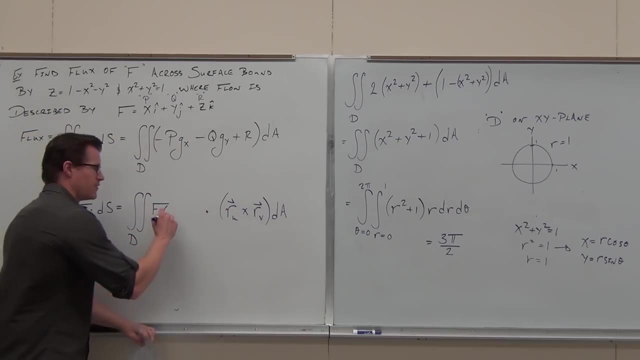 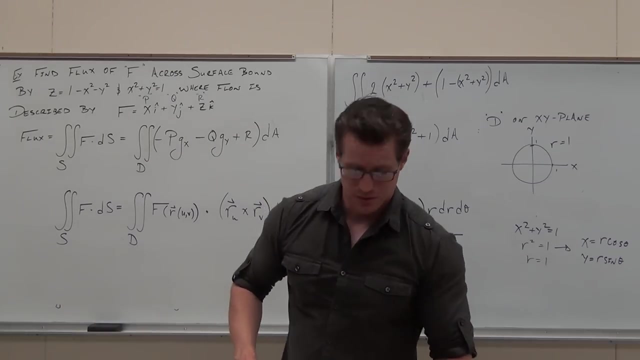 y, z and you have this parametric surface in terms of u's and v's. could you use this parametric surface to redefine your vector field? Then this would have to be defined as: whatever the parametric surface is defined as The way that you would do it, you'd start off with your 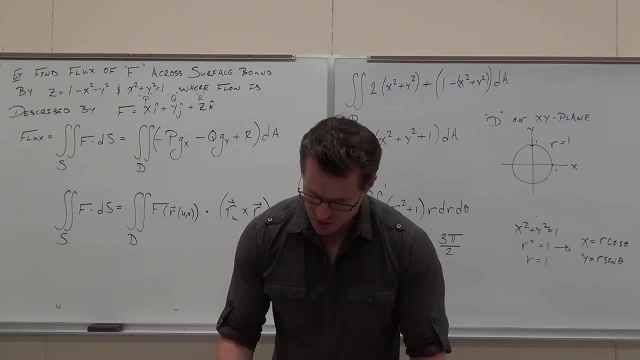 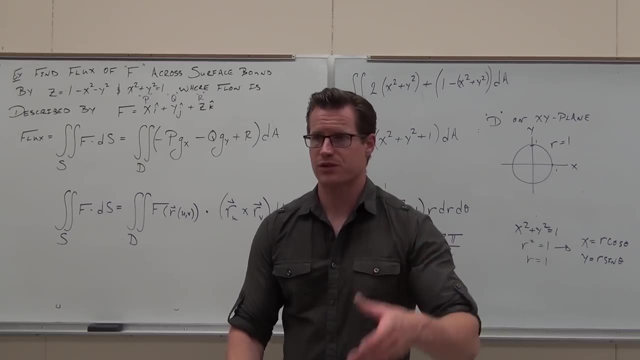 it'd be. listen, we did this a couple few examples ago. when we did, we did a surface integral across or with parametric surfaces. it's very, very similar. it's just now you've got a vector field instead of that function. 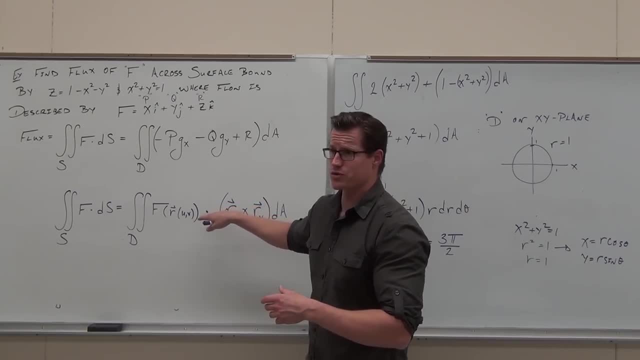 So you'd find it'd be given to you. just find a partial derivative. in both cases. do a cross product. redefine your vector field with x, y's and z's in terms of u's and v's. is that hard to do? 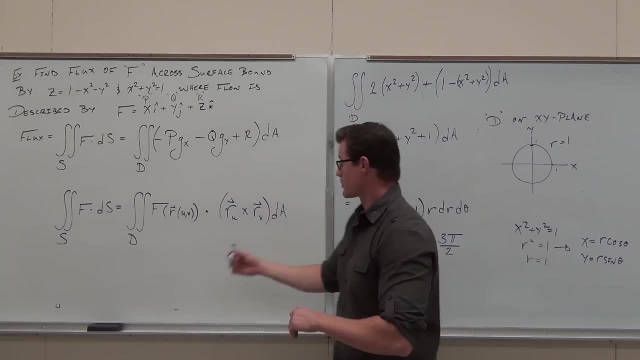 No, and then you just dot, product them and you do an integral With whatever the. the d here is the same thing as the vector field. It's the same thing as it was before. It's the bounds for u and v. So it depends if you think you can do that on your own. 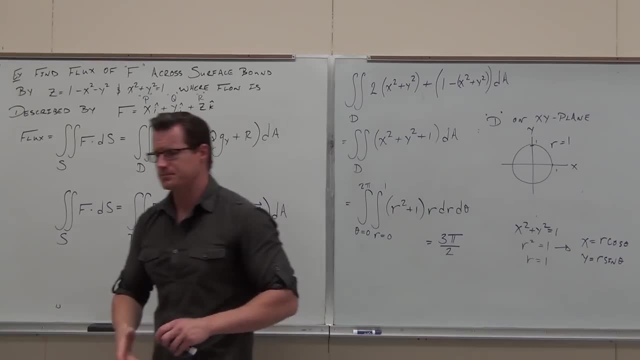 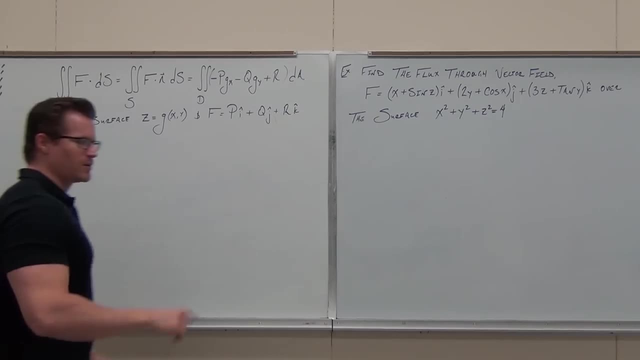 I don't really want to go over examples very, very similar. Just try it. try it one time. So last little bit: we we were right in the middle of something. What we were right in the middle of doing was taking these things. 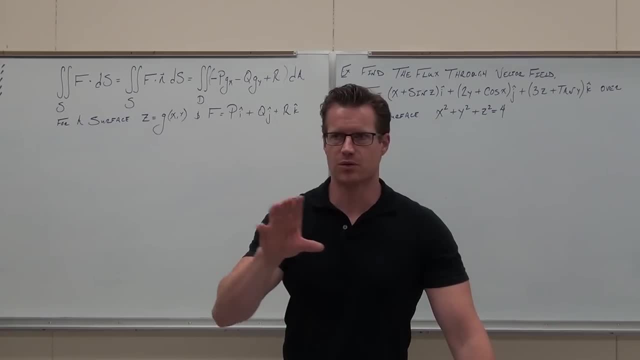 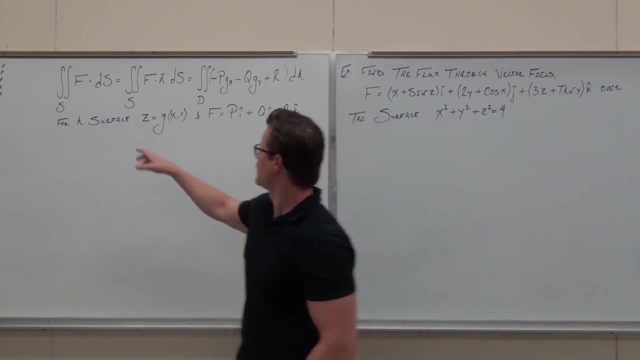 called surface integrals, and finding surface integrals of vector fields, like saying, okay, well, what's what's that even mean? And we had a special word for it. we said, well, you know what this is, this is what the, the format is. 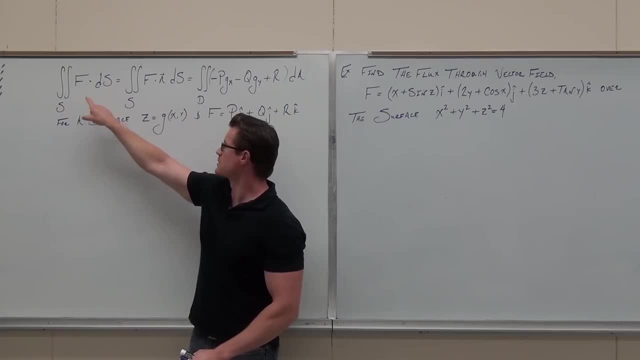 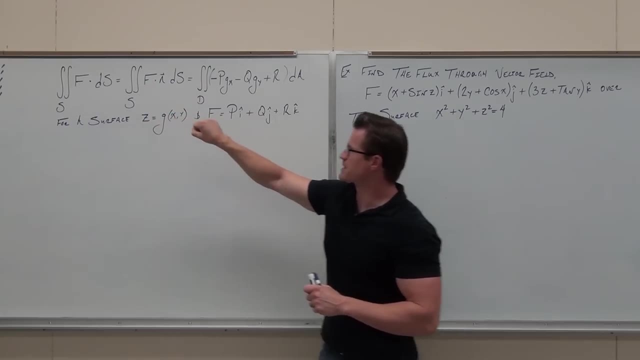 We're doing a surface integral. it's a. it's a double integral of a surface over a vector field, or or or through a vector field. Okay, so we we found out that it's the same thing as a dot product of the normal to that surface at any point. 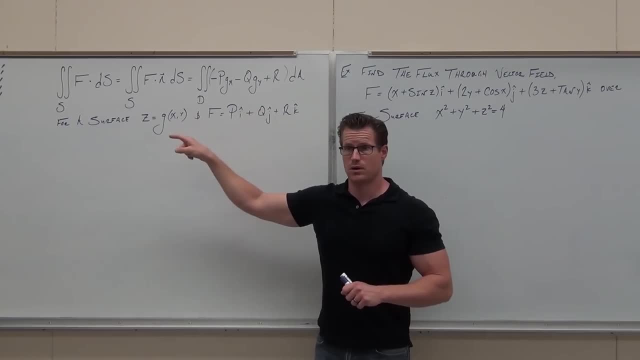 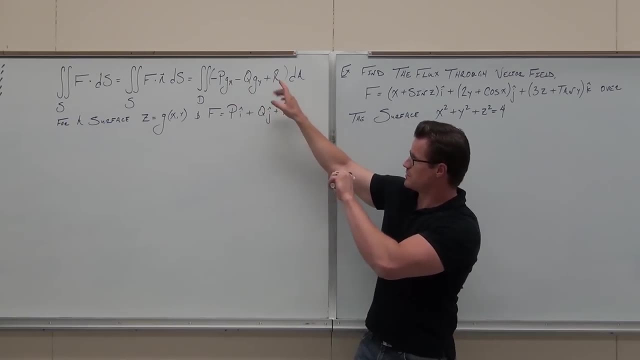 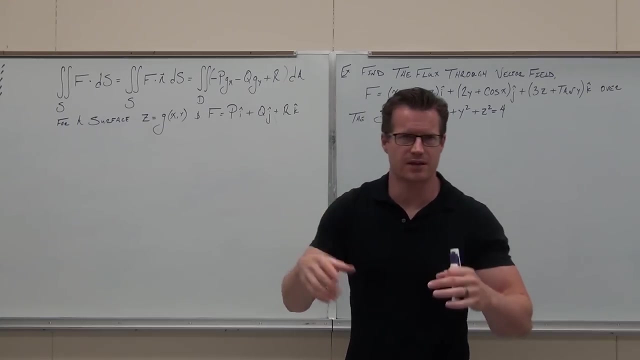 dotted with the vector field. And then we said: there's an easier way to do it, though. What? what if we took the pieces of the vector field p, q and r, put them in this? this double integral defined the surface as z equals some function of x's. 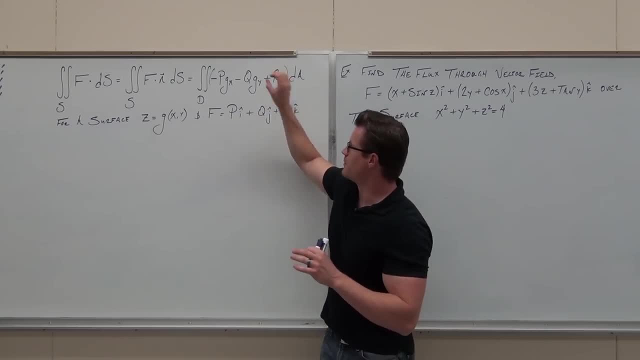 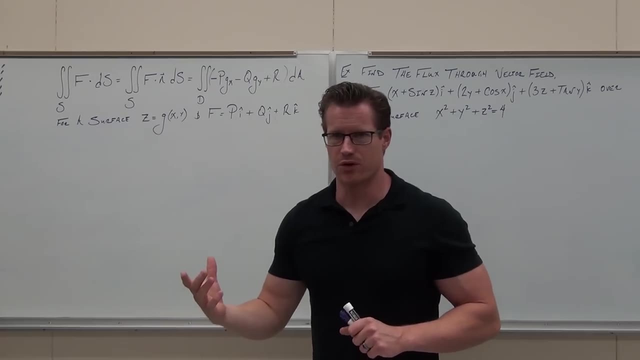 and y's took partial derivatives, then this represented the surface integral of a vector field. But what did that mean? What was that special word? It was the, the flux. Do you remember what the flux I'm talking about? I worked on that one. 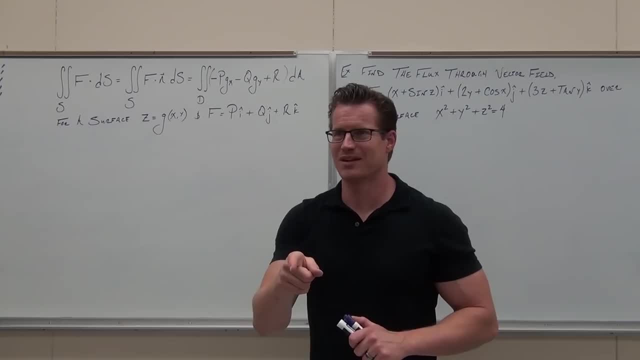 I told you I got to pull them all out, this one. No, nothing, not even a little bit. That was funny. Come on, I worked all day on that stuff. I was like people taking Calc 1 finals, whatever. 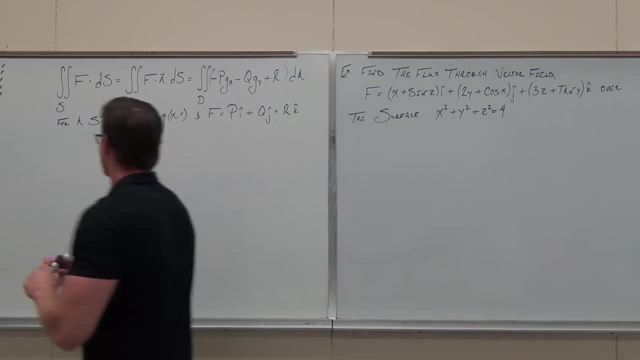 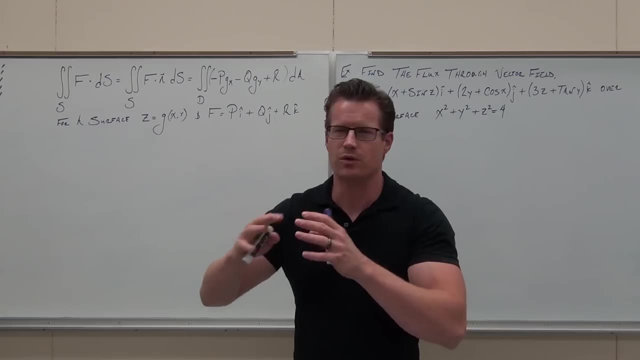 I'm working on what the flux you're talking about. Okay, Anyway, this was called a flux integral And and what it? what it's talking about is the, the rate that the the fluid or the flow is, is. 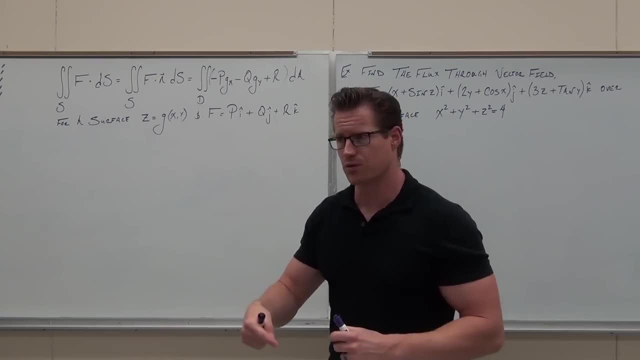 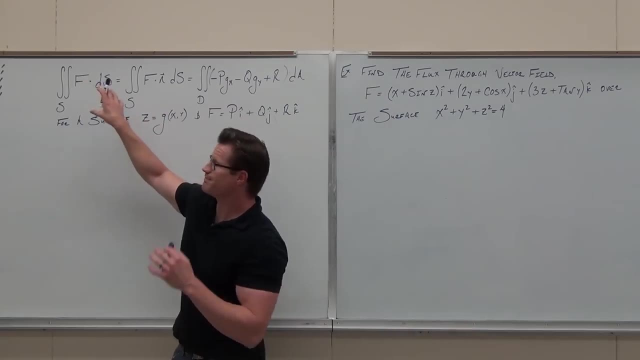 is going across the surface. That's what this is talking about. That's a surface integral of a vector field. It's called a flux integral And now that you're you understand the concept. this is what. this is what it is. 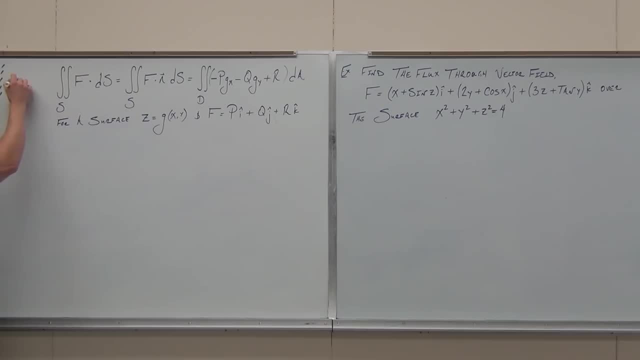 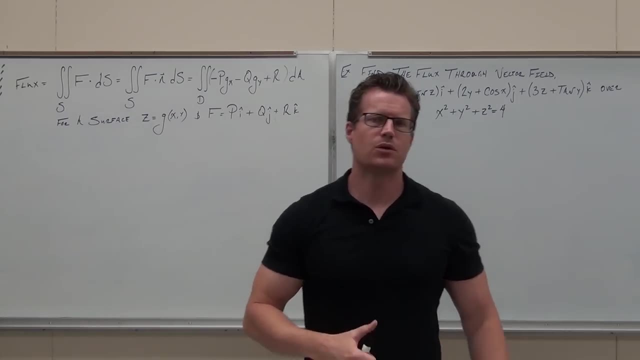 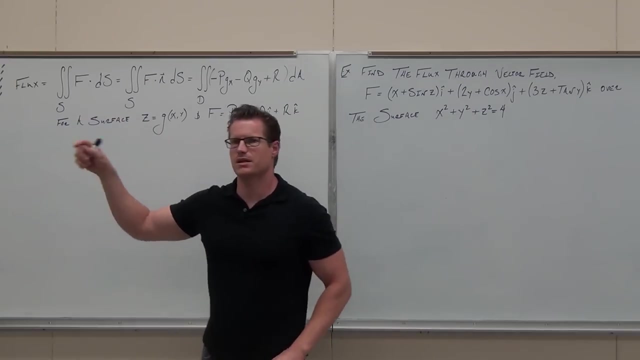 This is how we do it, And what it is is flux. Now here's the whole point about where we're going for the last two theorems you're going to get out of this class. What the flux? integral man. I just laugh every time I say that. 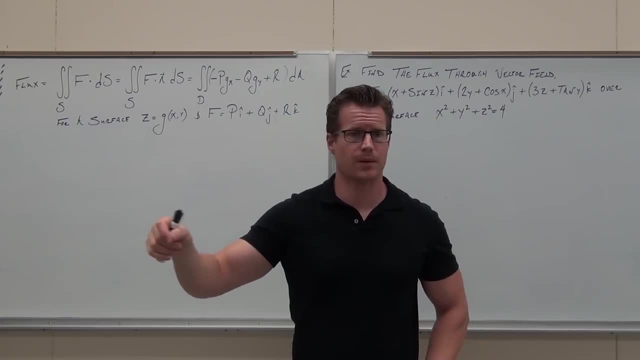 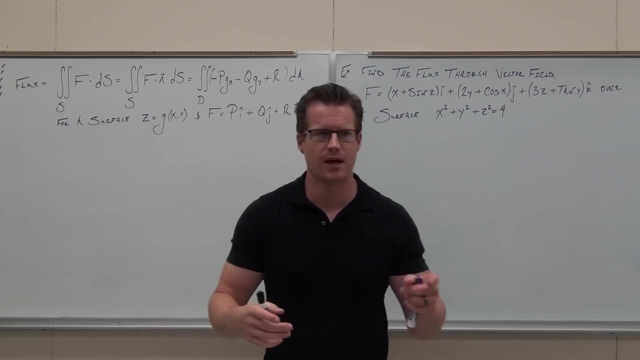 What the flux integral does it. it is a surface integral of a vector field, but it kind of depends on what that surface is and how we can define that surface Here's. here's the main question. that leads us to the next theorem. 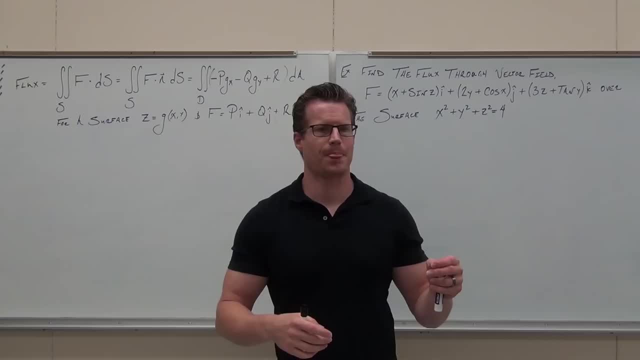 What if that surface? it has a very special case. What if that surface is not just any random surface, but it's a simple closed surface? Does that phrasing ring a bell to you at all? Yes, Do you remember simple closed curves? 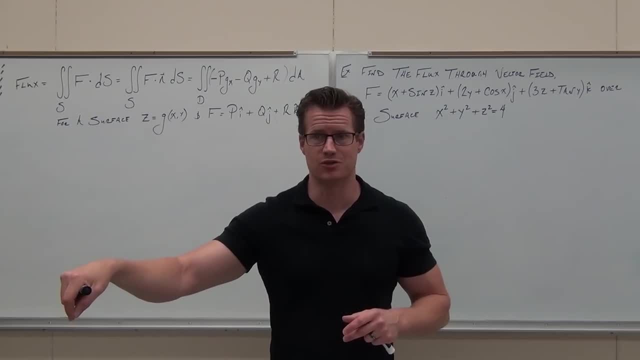 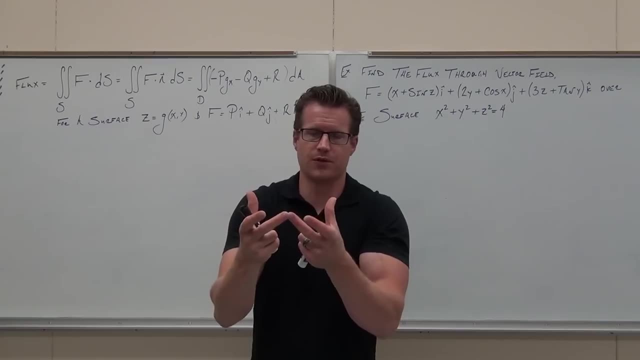 And if we had them, we had Green's theorem and it made it work a lot easier. Do you remember that? What if our surface is a simple closed surface? Means that it's this thing that if you, you filled it like a balloon? 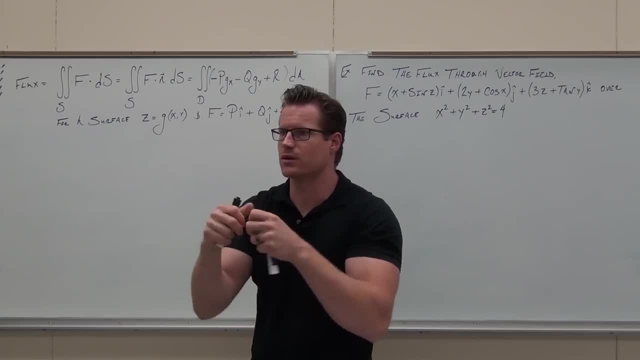 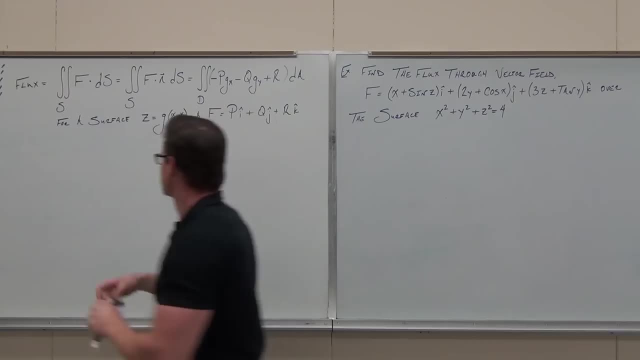 You filled it full of air or something or water, it would hold it all inside. okay, so it's. there's no openings to it. It's simple. It doesn't intersect itself in any way. What if our surface is a simple, closed surface? 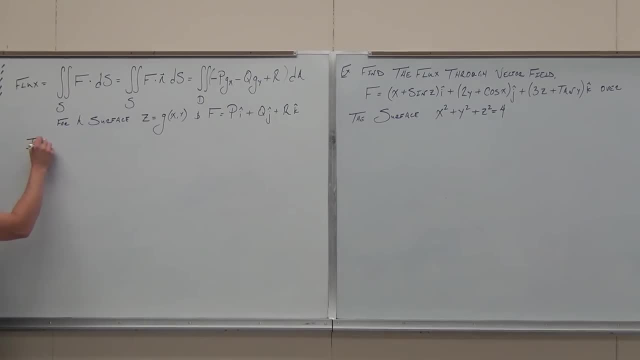 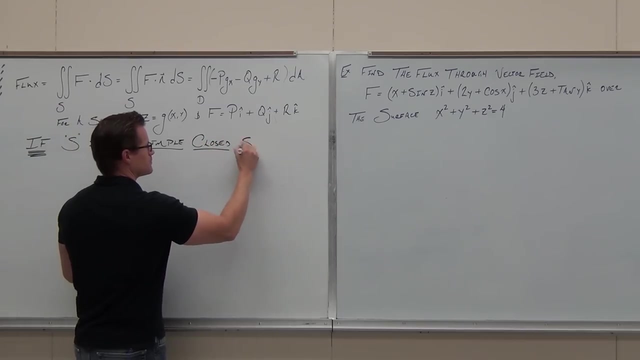 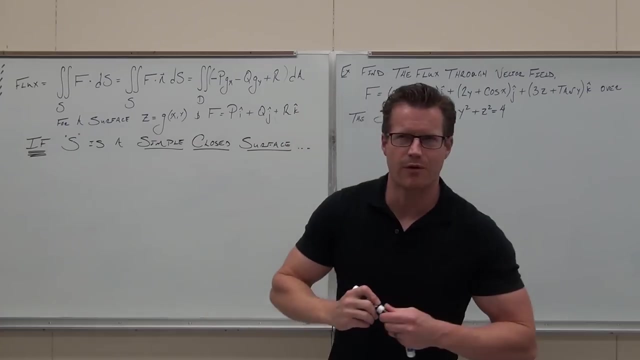 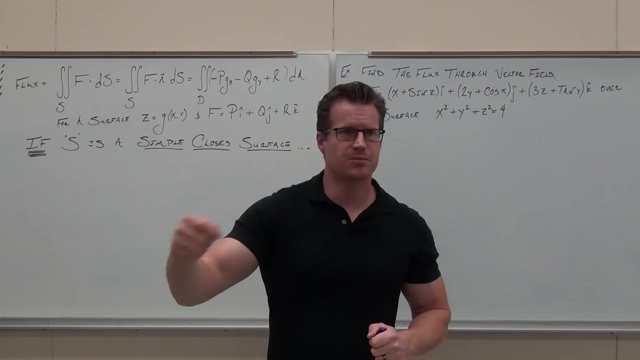 So let me make the case for you here real quick. We've already got surface integrals of vector fields. We know how to do them. They're called a flux integral. but just like before, if we have simple closed surfaces, like simple closed curves, we can make this easier. 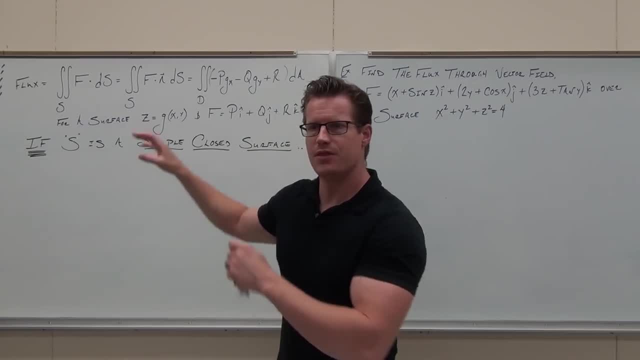 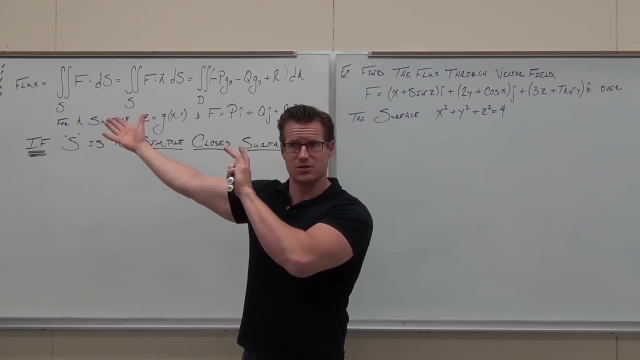 Green's theorem made things easier, not harder. This next theorem is going to make things easier, not harder. So, if you guys get the idea of where we're going on this, we have these things that are called surface integrals. They represent the flux and if 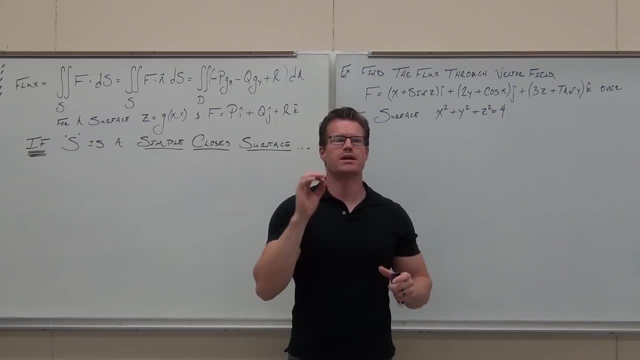 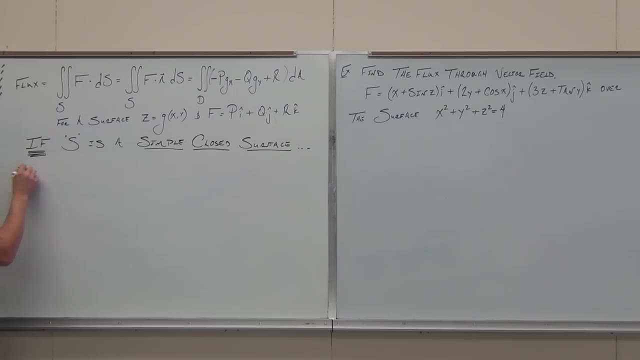 if we got the flux, we're going to get the flux. If we got the surface- it's a simple closed surface- we can apply this thing called the divergence theorem. You know what in the world is that? Where's that coming from? 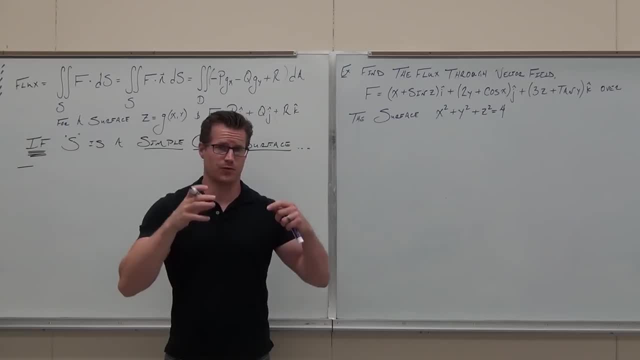 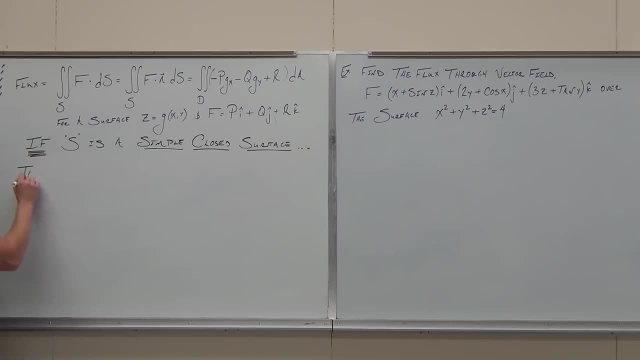 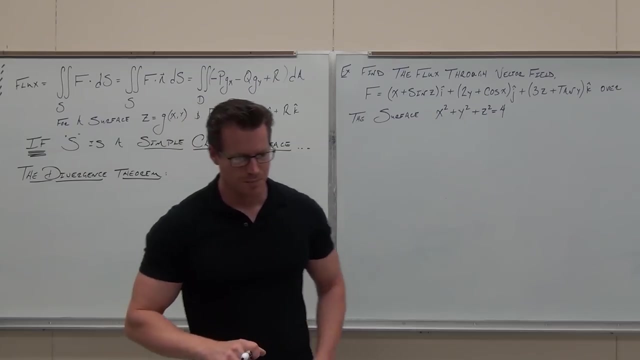 You'll see it in the formula. The name for the divergence theorem comes with for how we calculate it. not because of anything up here right now, but because of how we calculate it. Here's what the divergence theorem says. It's still a way to do surface integrals of vector fields. 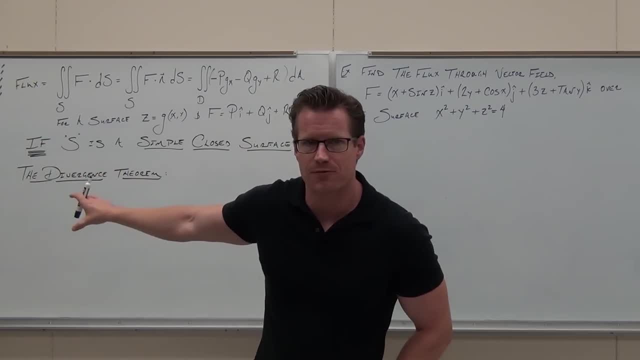 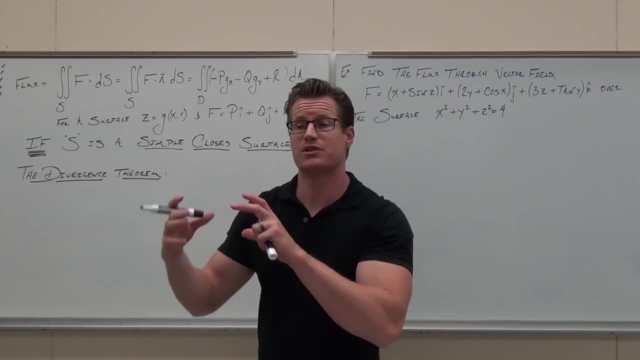 It's still going to calculate the flux force. So is this still going to be a flux integral? Yes, it's still going to be a surface integral through or of a vector field. It's just that if we have a simple closed surface, 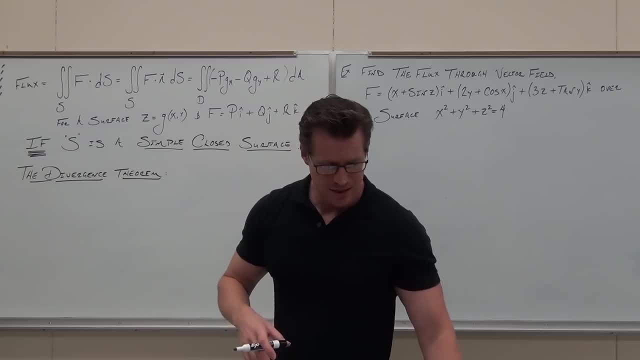 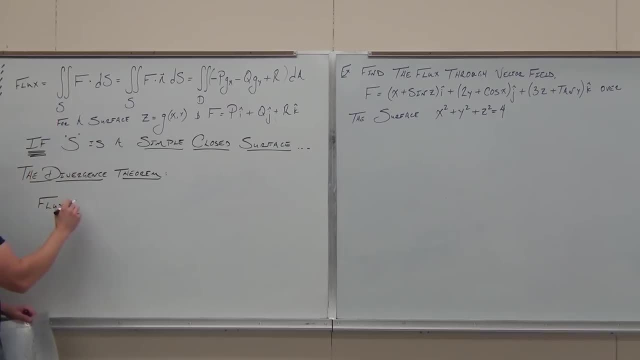 it makes these things easier, And here's how it does it. It says: if you want to calculate the flux, which is normally this, If we have a simple closed surface, we can change it, Instead of thinking about this as a double integral. 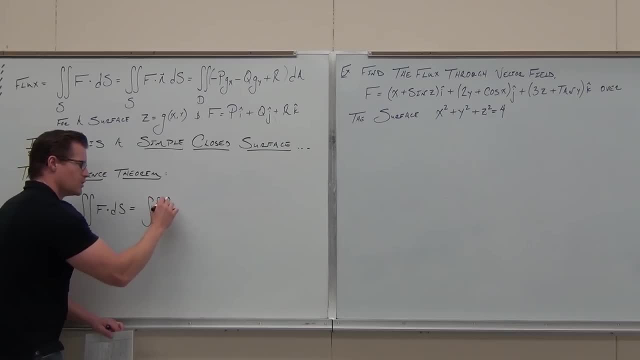 over the surface. we can think about it as the triple integral over the surface, So we can change it. Do you remember using that? These things were surfaces, 3D surfaces. Do you remember that If this surface is a simple, closed surface, 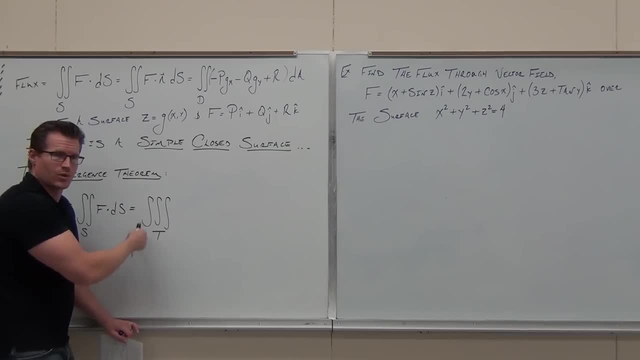 I can redefine it in terms of a surface for a triple integral. It says: well, what else is going to be up here? Take the divergence of your vector field. Hey, do you guys remember how to find divergence of your vector field? 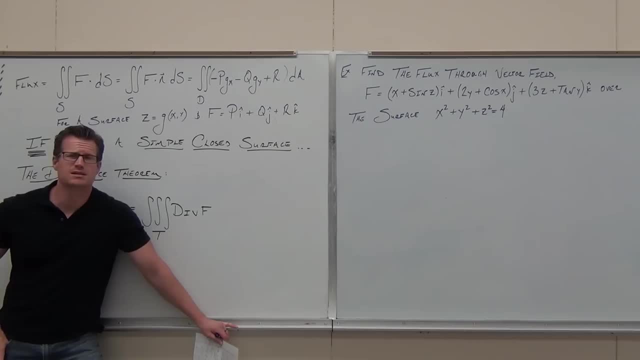 Yes, no, yes, yes, yes. Remember how to do that. It was a really easy thing. In fact. it was a dot problem, Dot problem. It was a dot product of an operator, this thing called del dot, your vector field. 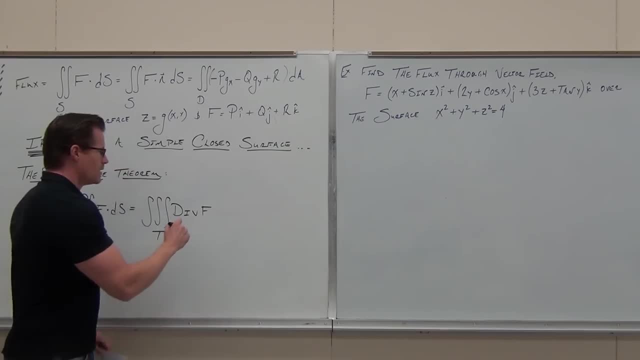 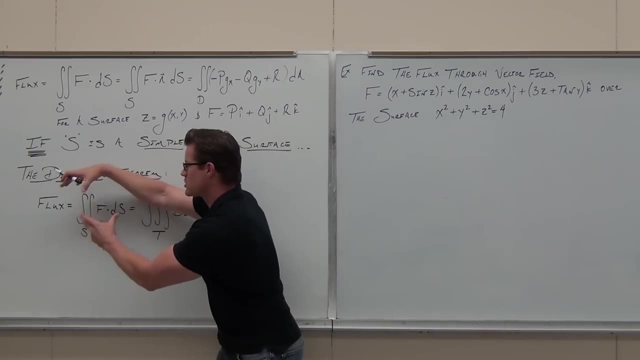 Is this ringing a bell for anybody? Yes, Okay, a lot of head nods. That's good DV, Just like before, with all of these theorems, with all these formulas. our main goal is to change this. Make sure it's satisfied, man. 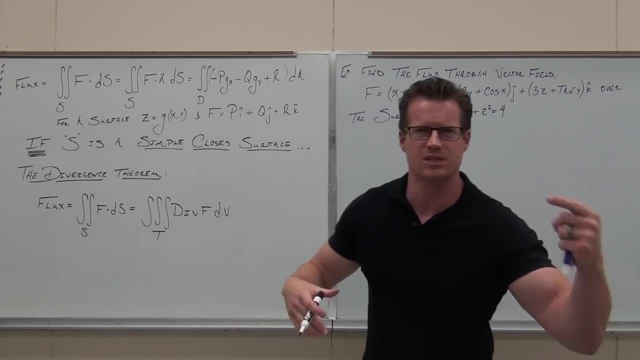 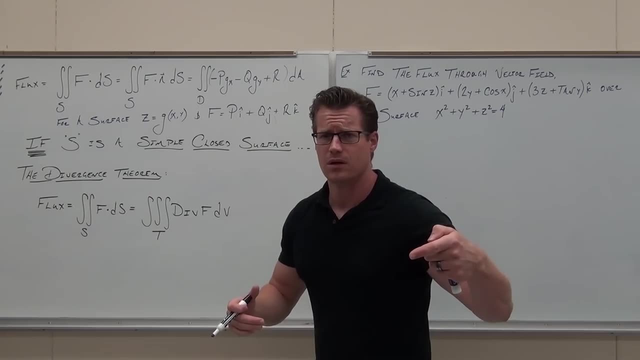 You've got to make sure the divergence theorem is satisfied. What's going to satisfy that divergence theorem? Tell me right now what's going to satisfy the divergence theorem? What type of surface am I looking for? It's a global. If I don't have that, does this work? 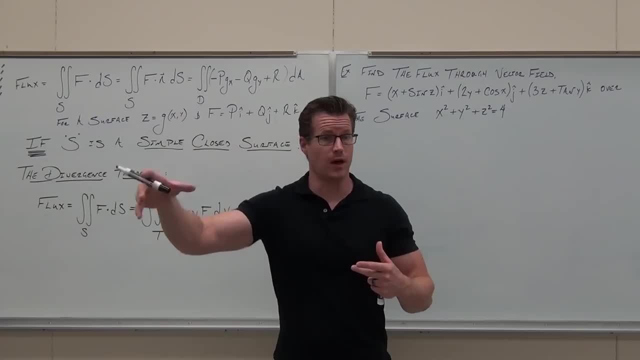 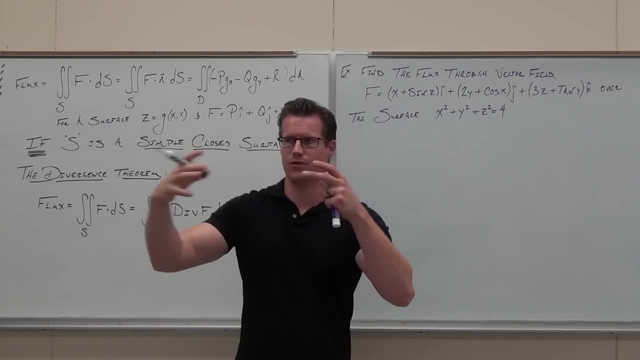 So you've got to satisfy that. So, firstly, I want to be finding the flux, because this thing still finds the flux. Does that make sense? So the wording up there says: I want a surface integral of a vector field. I want to find the flux. in other words, 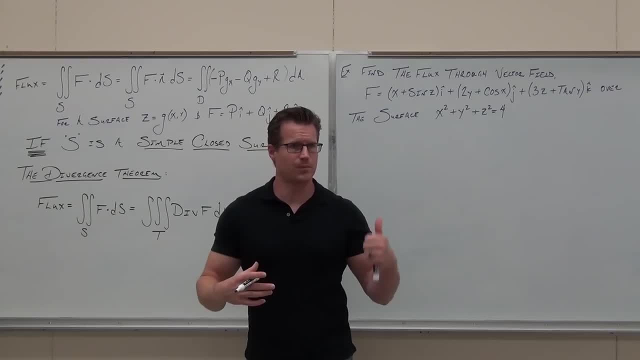 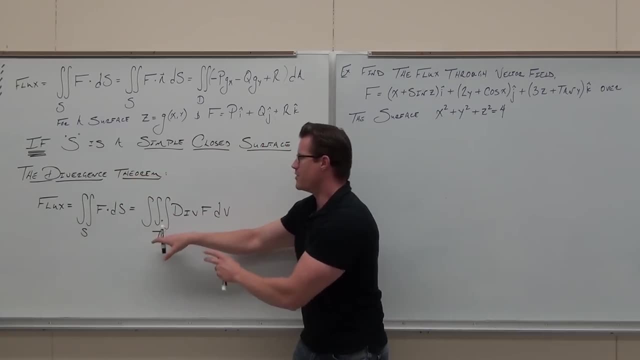 And then we've got to verify that the surface we're dealing with is actually a simple closed surface. Head nod that you're with me on that one. If it is, then satisfy divergence theorem. write this form and then look at what your surface is. 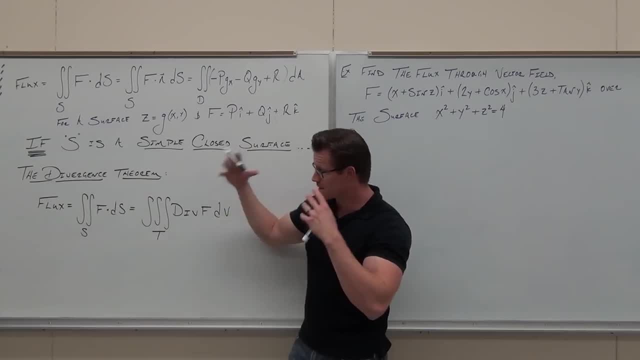 Remember, we never skip this step, Like ever. So in our example we're going to find the divergence of F. We're going to put it in there. Then we're going to start looking at that surface. Head nod, if you're with me on that one. 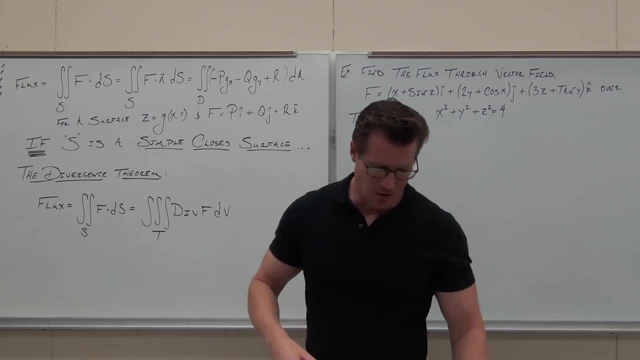 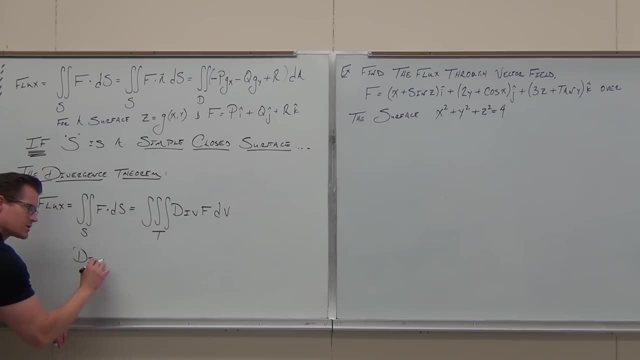 That's it, That's all divergence theorem says: Is it hard? No, You do got to remember what divergence is. So if you're drawing a blank you're like, oh my gosh, I don't remember. The divergence of a vector field is this: 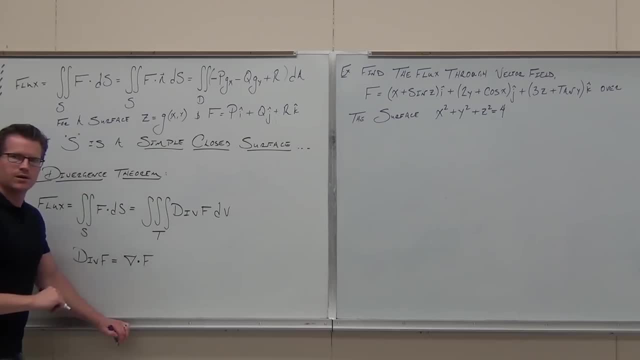 It's del, dot, F. Del was this idea of the partial derivative with respect X, then Y, then Z added up. Does that make sense to you? And then F, is this PQR? So if you really just wanted a formula for it, you're like: 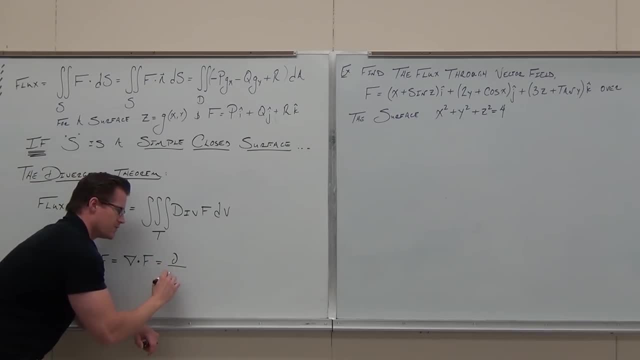 I don't really. it doesn't make sense to me. It says: take the partial derivative with respect to X Of what Well of the P first, Then take the partial derivative with respect to Y Of what Well. the next thing, the Q, Because it's a dot product. 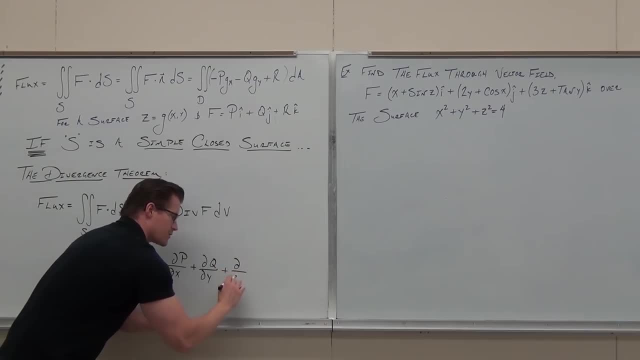 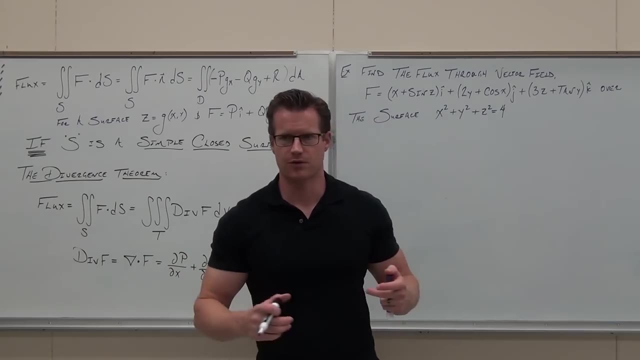 it matches up the components of a vector And then the partial derivative, with respect to Z, of what Well R? That is what divergence it always is for a vector field. Is it hard to find? Yeah, it's pretty, super easy to find. 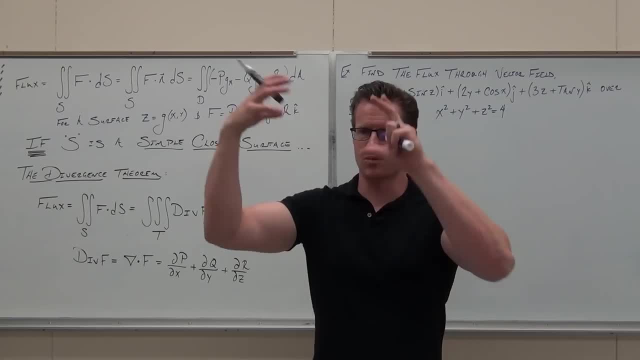 As long as you know partial derivatives and you can match up X with X's, Y's with Y's Z, There's no switcheroos here. It's partial derivative with respect to X of the X component, Y with the Y component, Z with the Z component. 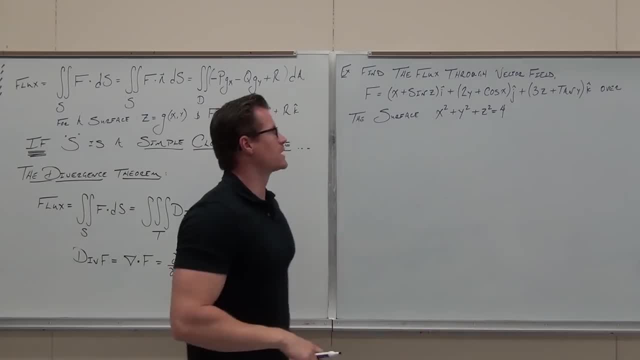 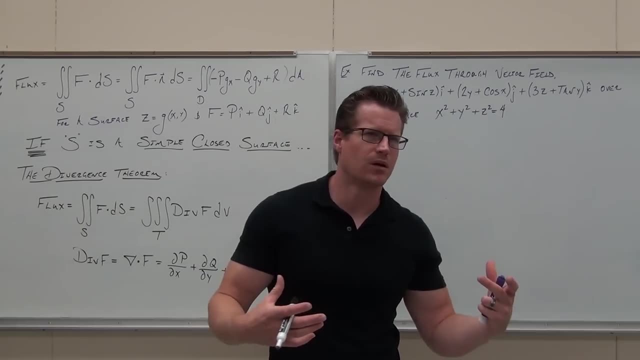 Show your hands if you feel all right with that one. Now let's go over here and look at it. Firstly, tell me something: What's flux? What it? what it? what's it? what's it coming from? It's a it's sure. okay, it's the rate of. that's what it means. 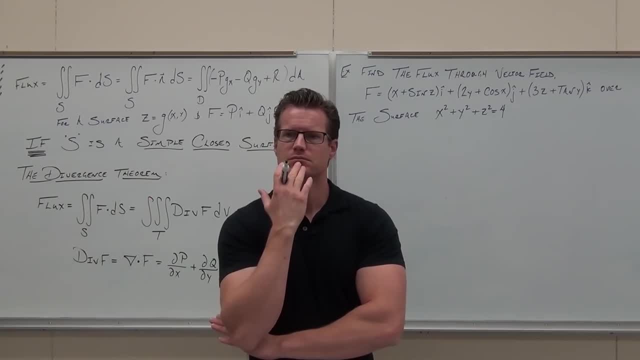 What gives it to us, Gives us the flux. What are we doing in this whole idea here? What are we doing? What's that? I know it's integral. What type of integral? Yeah, there's like those little symbols, like all over the place. 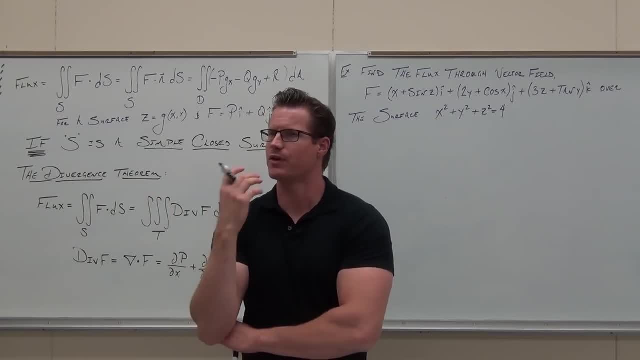 I don't know what you're doing with integral. What type of? what type of? come on folks. what type of integral, Surface integral. Don't, don't lose it now. We've had 33 days of this, okay. 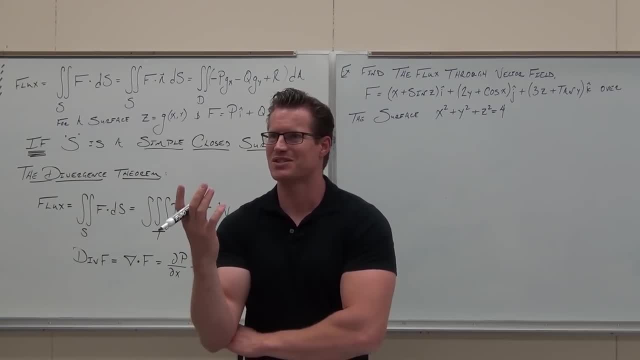 This is the final day. Don't lose it now. I got all of you here. I want to make sure it sticks, because this puts a lot of stuff together for you. okay, I don't want you to leave this class not understanding some. 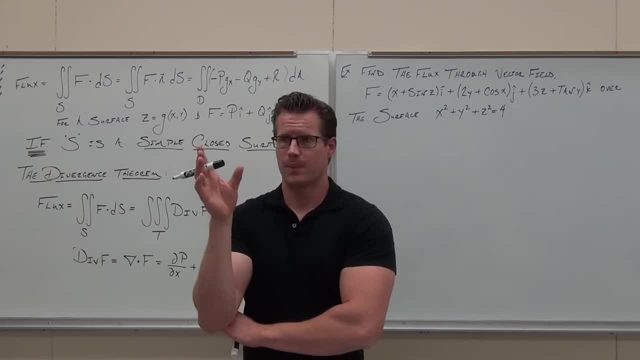 of the connections I want you to make in the next 30 minutes. So, firstly, what gives us the flux? Some of you guys are saying it kind of: What gives us the flux? Surface, A surface integral of what, The integral? 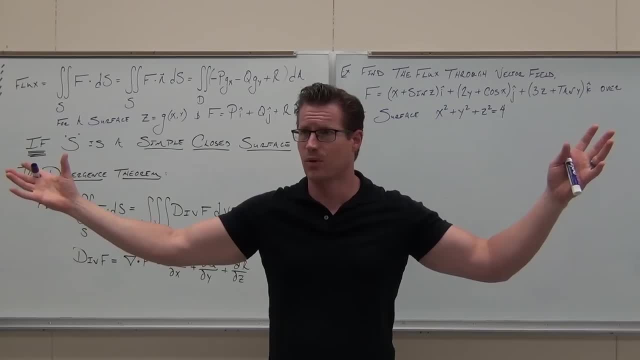 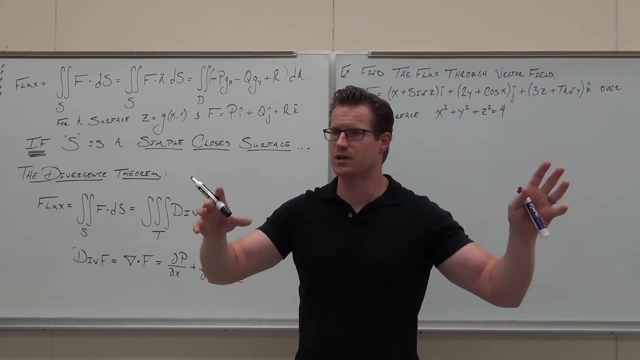 The integral? Through what Surface? What things are we dealing with here? So it's a surface integral of a vector field. That's what's giving us flux. Does that make sense to you? That's what this stuff is. How can we calculate it? 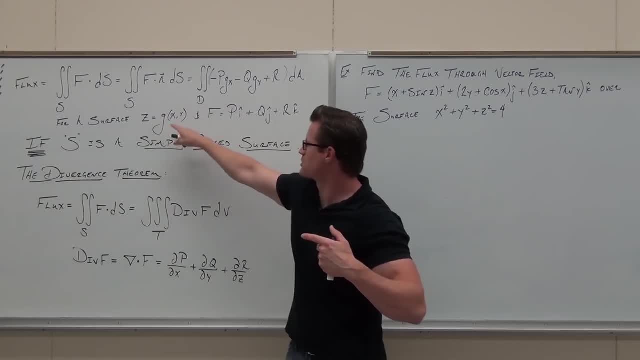 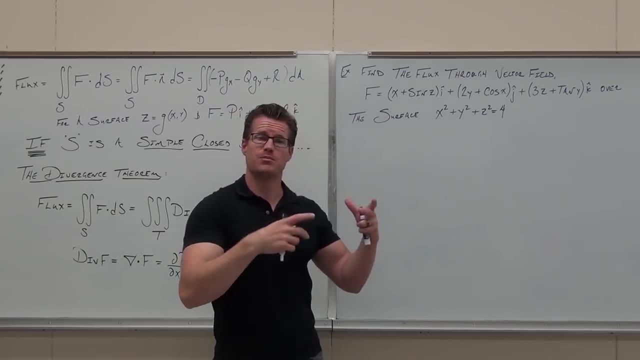 One way, just like that. If we can define z as a function or the surface as z equals a function of x and y, we can do it just like that. We've already done that. If we have a simple closed surface, things get even easier. 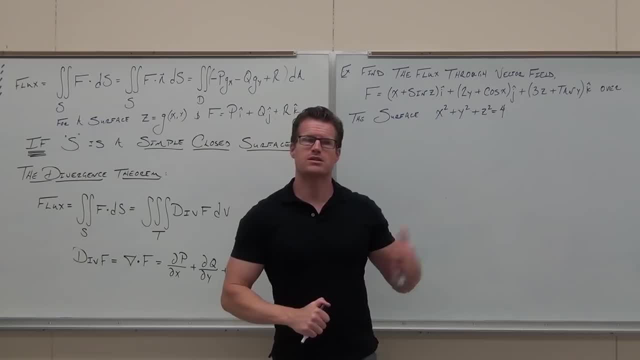 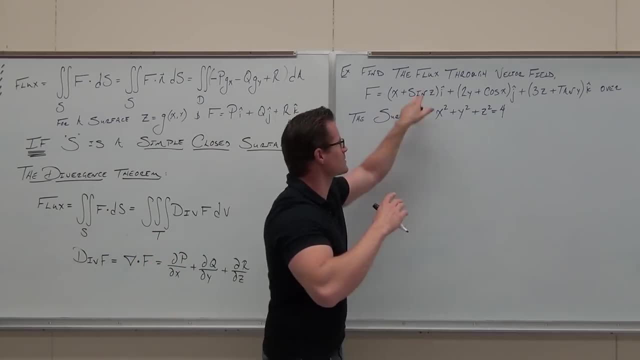 You can go. triple integrals are easier. They can be. Let's take this example out. Firstly, tell me again what's the flux? Well, what's it talking about here to you? Read it in English. It says: flux means I'm finding a. come on people. 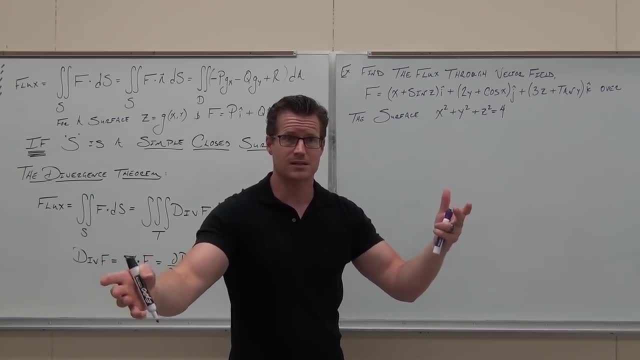 Surface Surface integral of a. That's a vector field. That's fantastic and it's going to give us the rate of flow across that surface. That's what's happening here. okay, What surface Does it give you a surface up here? 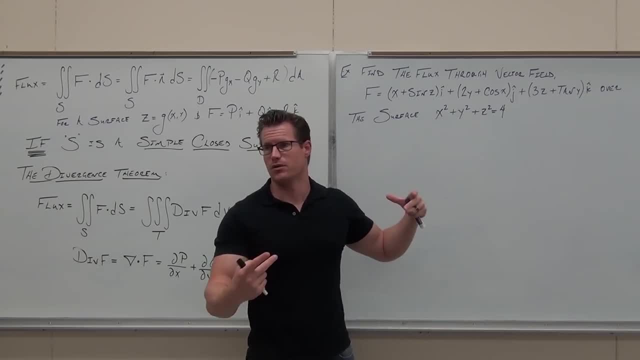 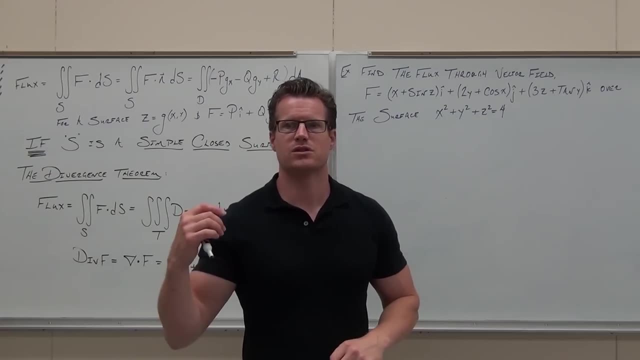 Yes, Yeah, It has to. Does it give you a vector field that you're working with? Yes, It has to. Now, here's how we did it. Here's how we determined whether the Divergence Theorem works. You've got to look at the surface first and say, okay. 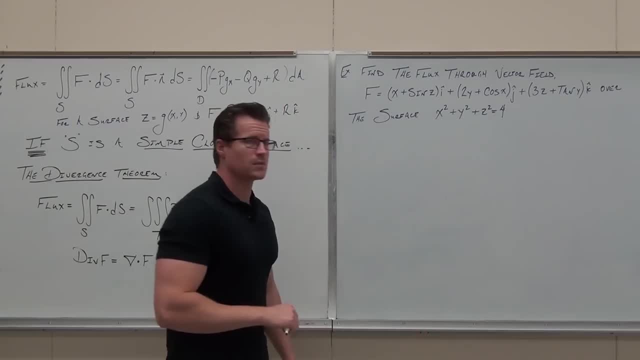 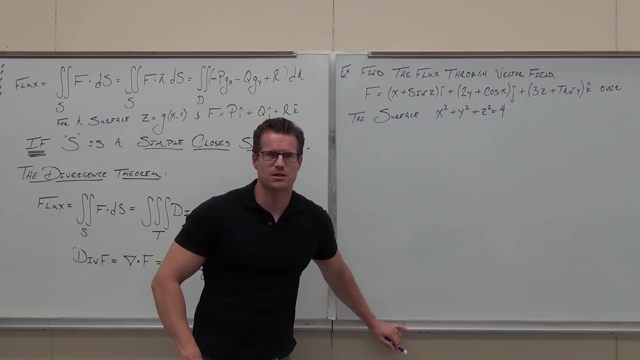 what is the surface? Well, what is that surface? It's a sphere. It's a sphere with a radius of what Hey. are spheres simple closed surfaces? Yes, Will Divergence Theorem apply? Yes, Here's why. 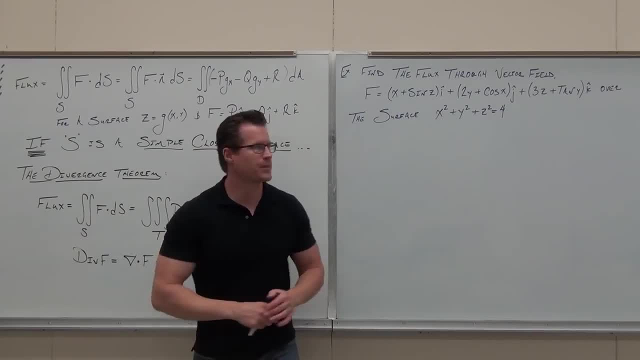 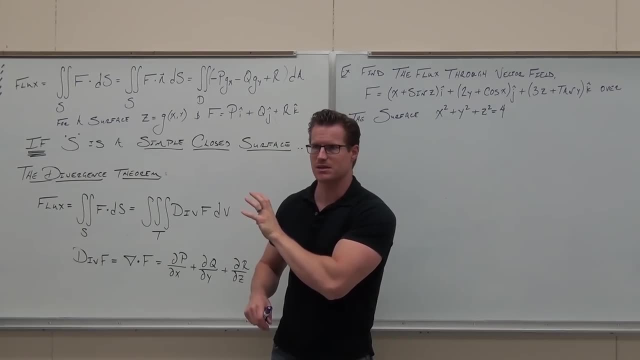 You've got to get this. It's a surface integral of a vector field where your surface is a simple closed surface. That's what Divergence Theorem says to us. Does that make sense? So you check the application first. It's not just a surface integral. 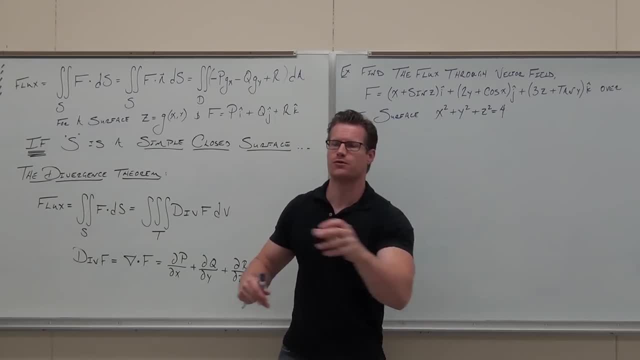 It's a surface integral of a vector field And the surface is a simple closed surface. Those things have to be met for us to use this stuff. You don't just arbitrarily throw triple integrals in there. okay, This has some qualifications and we meet both of them here. 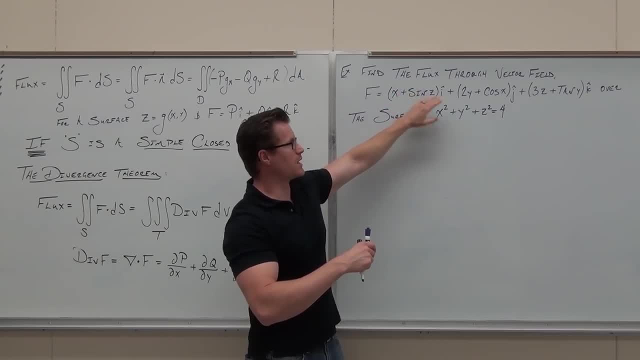 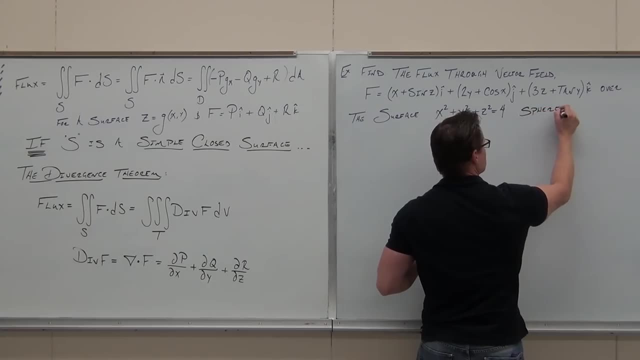 Flux. yes, that is a surface integral of a vector field and we've got a simple closed surface. with me It's a sphere, Okay, Sphere, That's simple. closed, it means it's going to apply. Here's how it works. 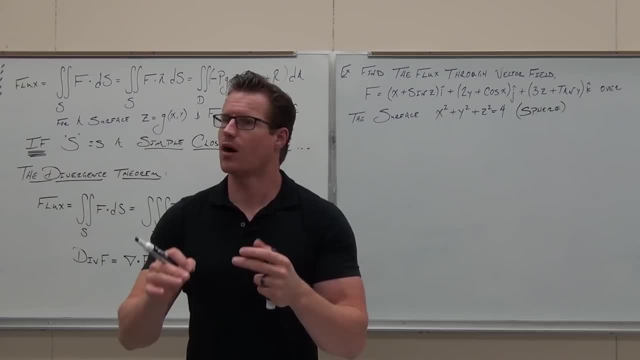 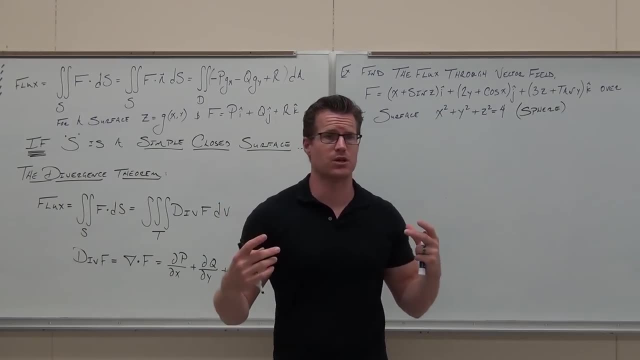 Literally all I want you to do right now: calculate the divergence. Our main goal is getting the setup right. Don't even worry. Don't even worry about the T right now. Don't even worry about the 3D region. 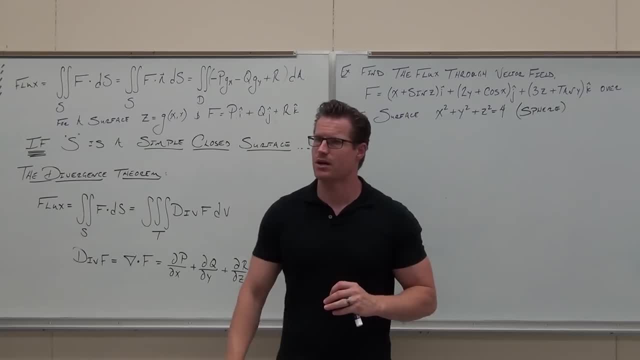 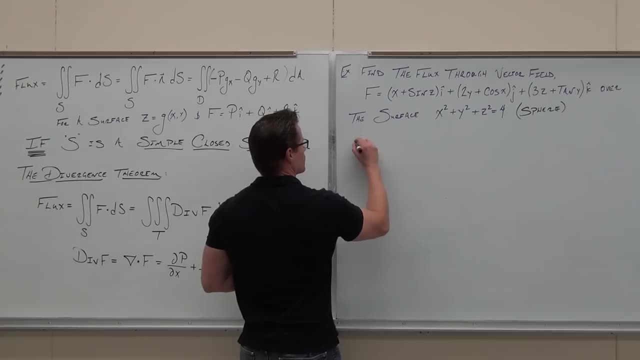 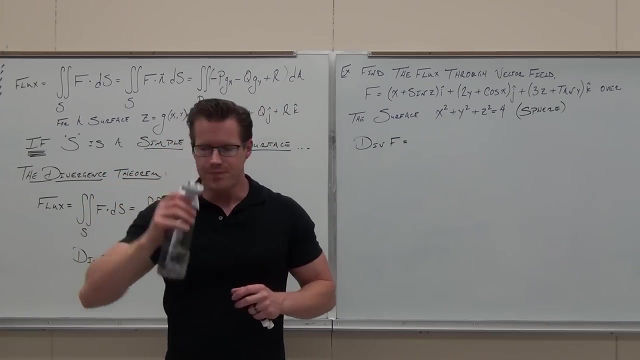 Don't even worry about it, Just use Divergence Theorem. Can you please try that right now? It's good practice for your final. all right, Try to find the divergence of that, please. Did you find it? Was it hard? 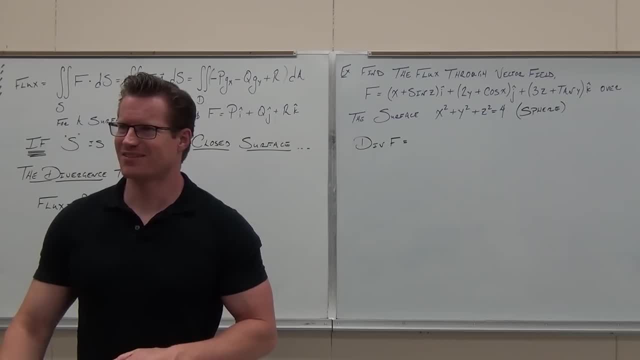 No, It kind of looks like it's going to be hard right, Like, oh man, that sucks, It's not really hard. Well, let's look at it. The divergence of F says: don't do this okay. 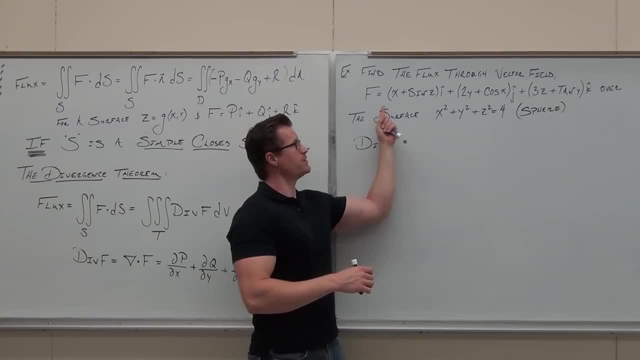 This is from F, the vector field. Go, take the partial derivative of, and you know what You might want to label this. just in case You know these things get mixed up or whatever, Or if you can't use that divergence theorem. 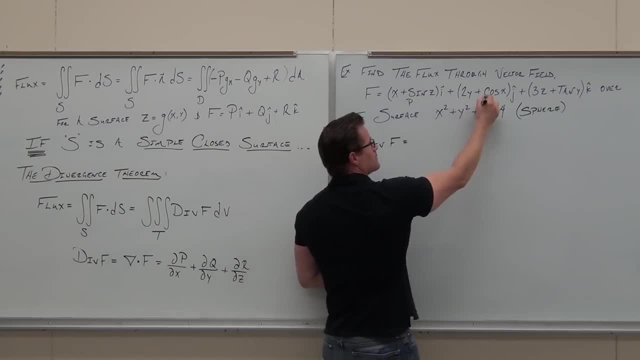 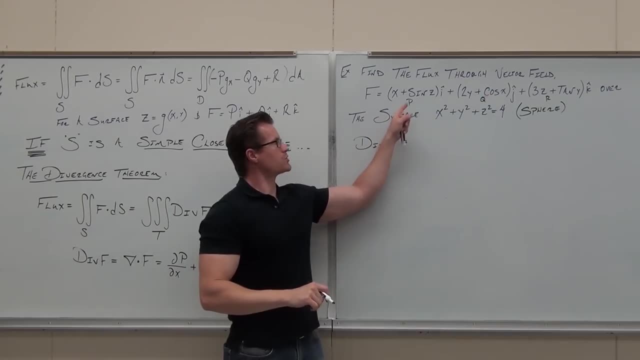 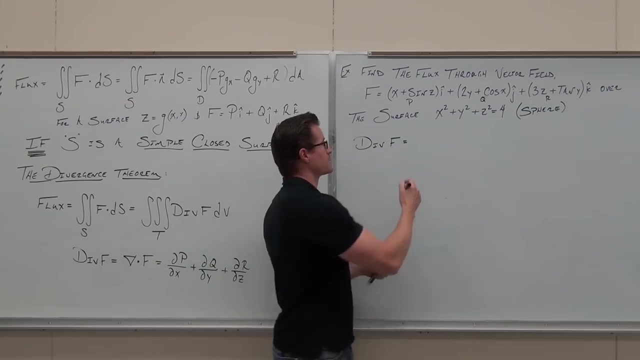 you have to know what P, Q and R are. Maybe P, Q and R Take the partial derivative of P with respect to- seems pretty straightforward. Partial derivative of the X component with respect to X. It's not bad. 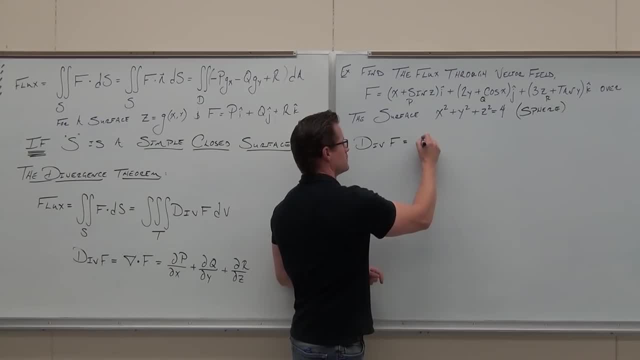 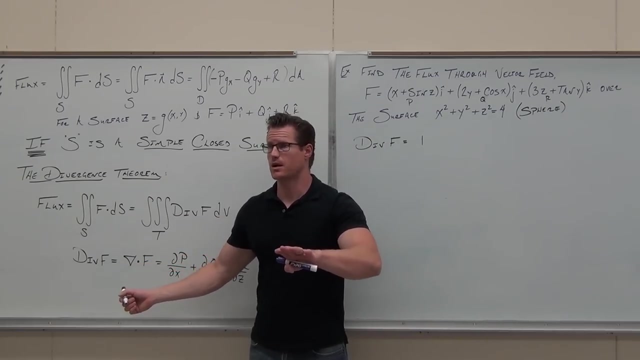 It's just what One, Not I. What divergence does? do you see any? I's up here. If you're dotting, if you're dot producting things, you can't even get a vector. Dot product gives a scalar. 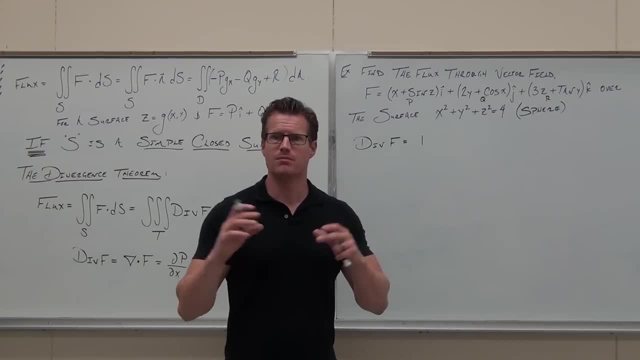 It's a scalar, At most a scalar function. Does that make sense? At most you have X's, Y's and Z's. No, I's, no J's, no K's. I don't know that. you understand that. 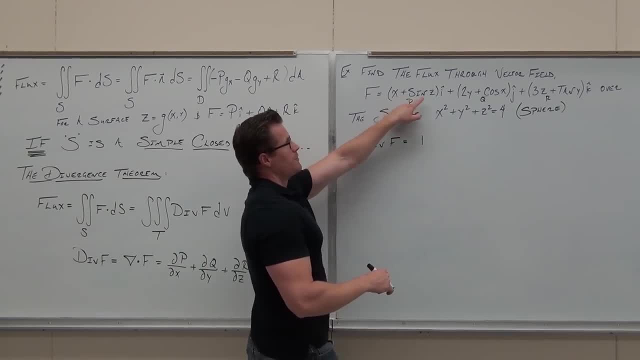 Dot product is really important. you understand So partial of this. just this: that's the P. This doesn't involve the P. The P is the thing in front of the I, So partial derivative of this with respect to X is one. 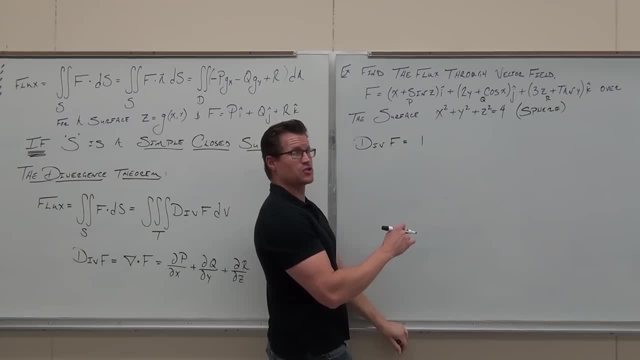 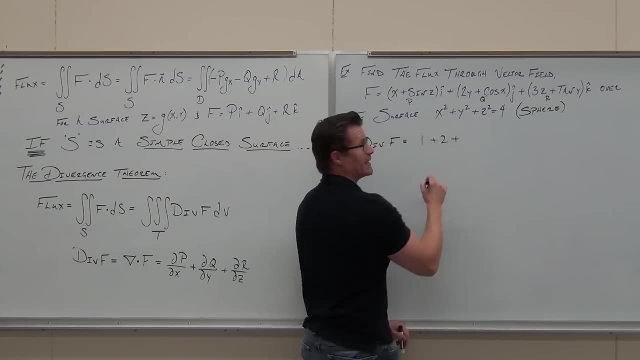 Partial derivative of Q with respect to Y. Y is Two, Two, J, Three, Three, Wait, oh no, J, No, No, No. And Three, Three, Three Equals Six, Six, Wait a minute. 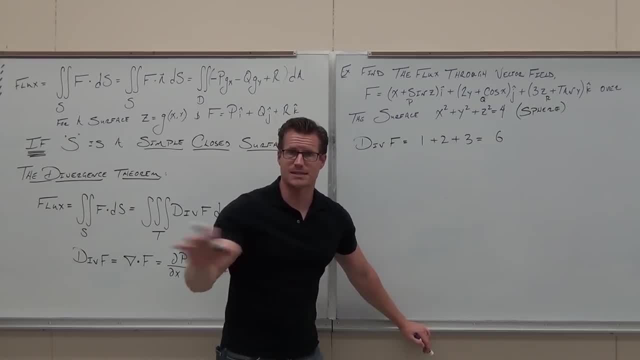 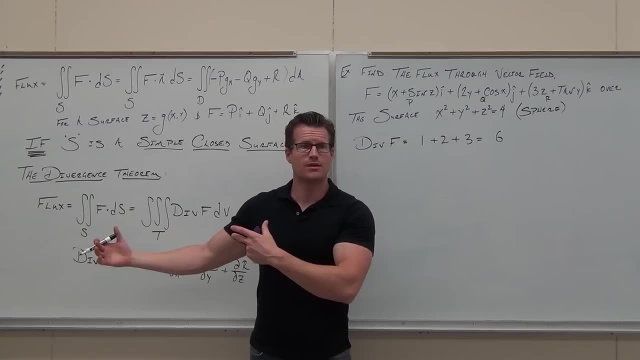 That's it. That's all. Yeah, That's it. I told you this stuff doesn't get harder. The theorems people create aren't intended to make your lives harder. They're intended to do one of two things: Either make the hard stuff possible- not necessarily easy, bless you, but maybe possible- and make the 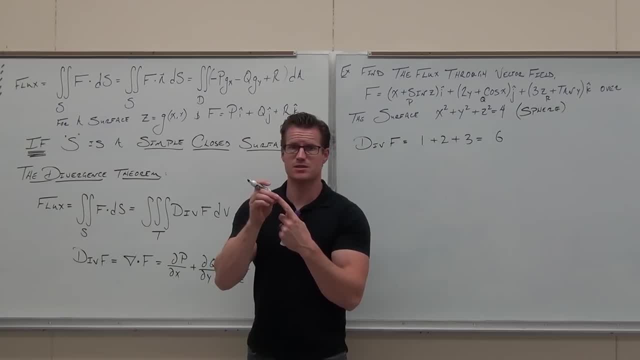 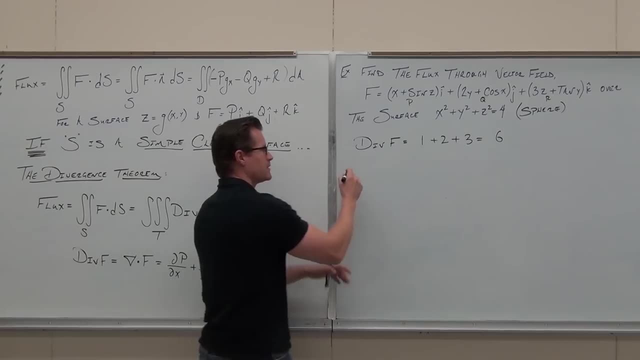 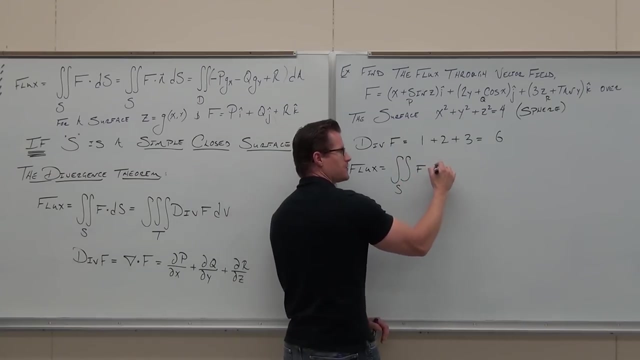 Bless you, Bless you, Bless you The hard stuff that is possible easier. Does that make sense? It's designed to make it easier, So here we go. okay, well, let's set it up. Then the flux which is normally defined as a surface integral of a vector field over that surface. 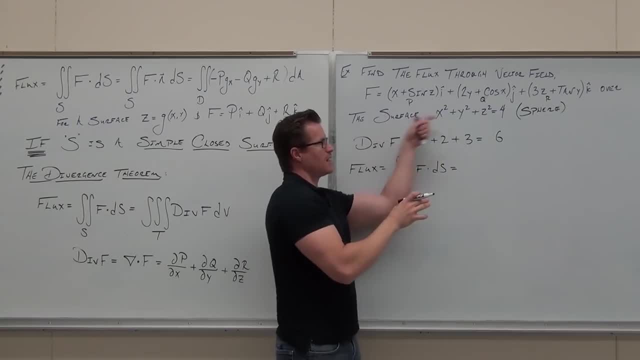 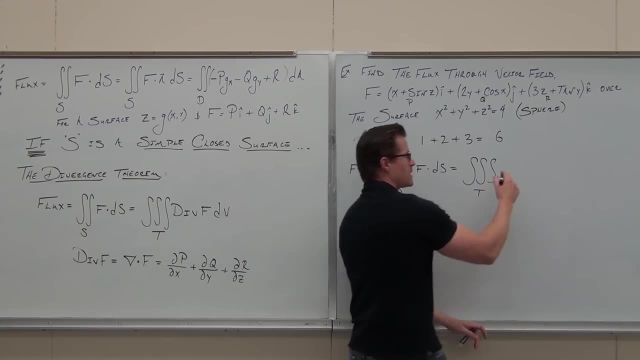 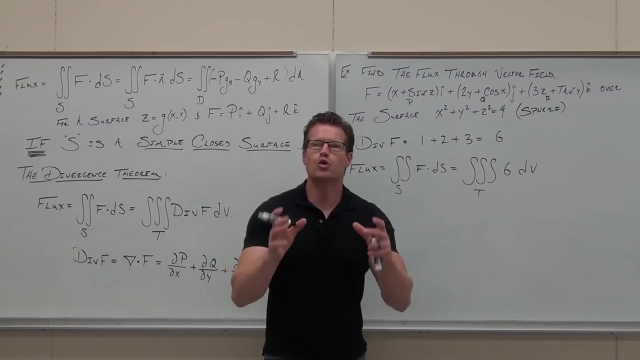 says: because we have, because it's this, because we have a simple closed surface, this is now a triple integral by the divergence theorem over the surface that's given to us of the divergence of F? dv, just like that. Look what it does. 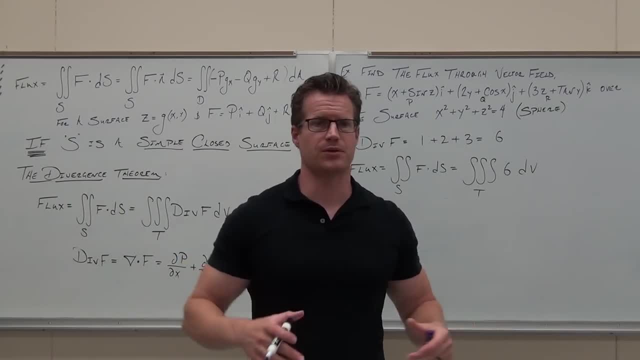 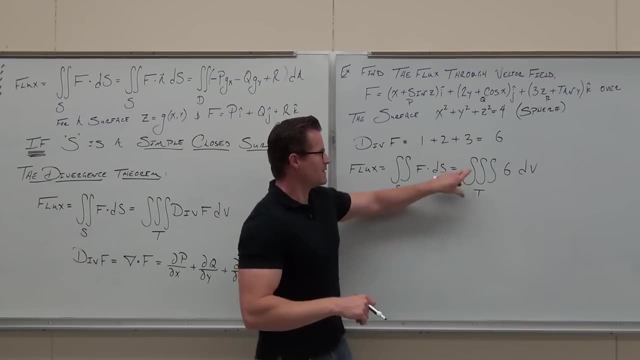 It literally takes you back an entire chapter. Do you guys see that These theorems take you back to old stuff which we've conquered already? Now you tell me something If I give you this and I tell you what surface you have: this simple, closed surface. 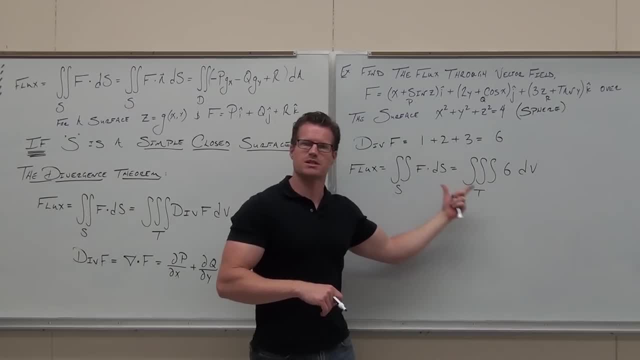 can you do something with that triple integral? Do you understand why we don't skip this step? We don't even skip. We don't skip this step because we want to have this down and then start thinking about what region we're working with. 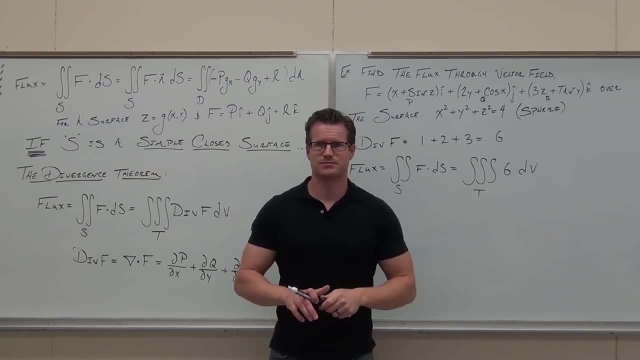 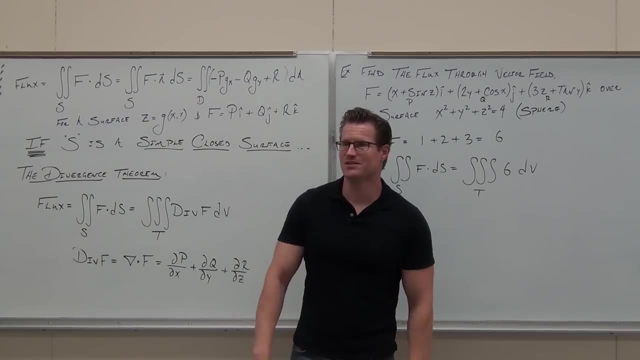 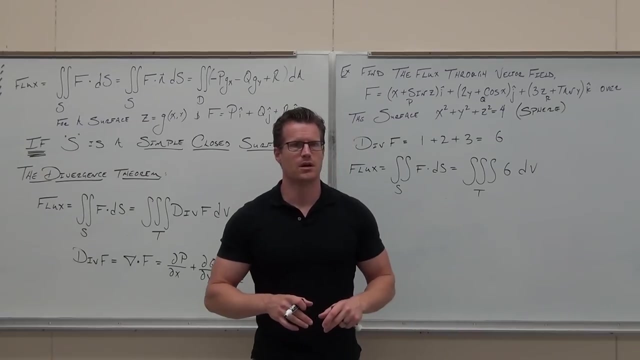 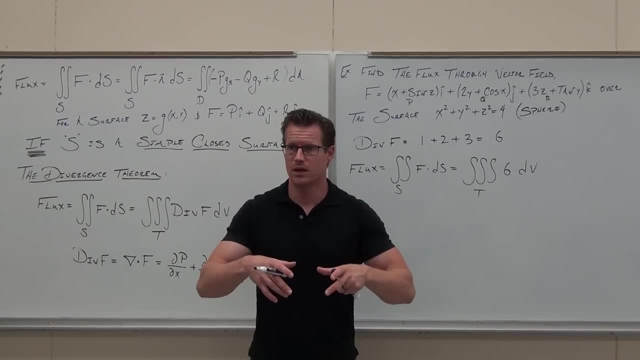 For those 3D regions that are cylindrical in nature or conical, sometimes, use cylindrical, And for stuff that's planar in nature, use rectangular. That's why we learn all that different stuff in Chapter 14, is that we can apply it here. 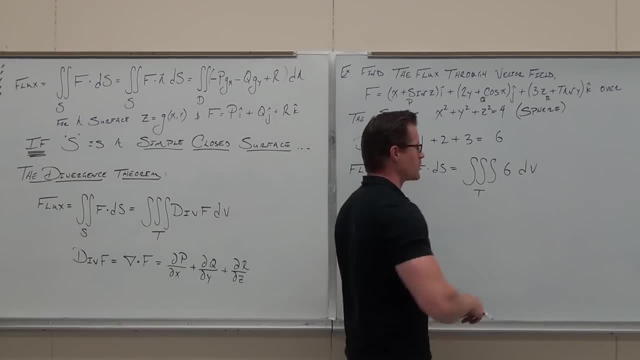 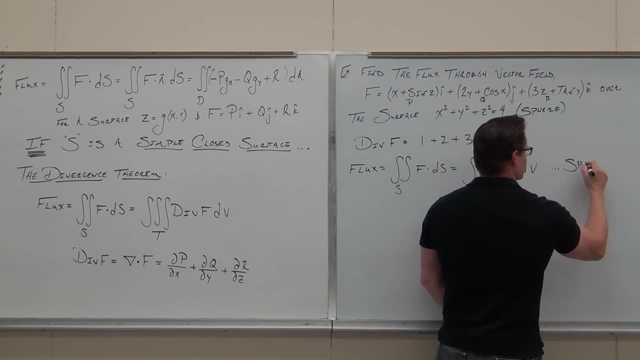 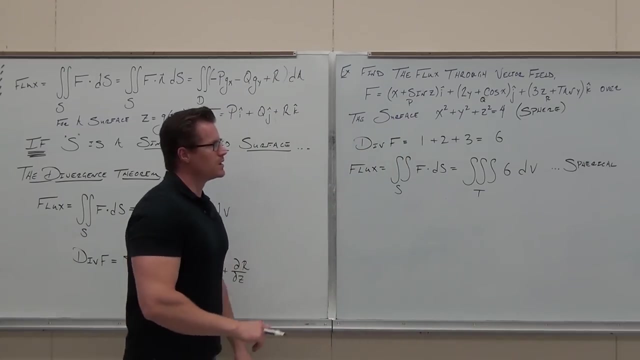 and have an easy time with it. It makes our lives easier. It takes us back to Chapter 14.. You go okay. well, hey, let's use spherical, Let's use spherical. Tell me a couple things about this. Do you remember how spherical is defined? 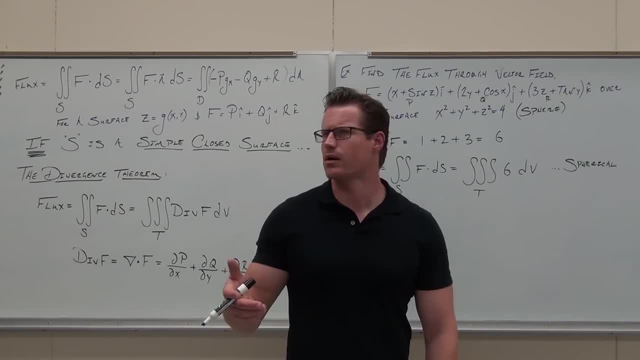 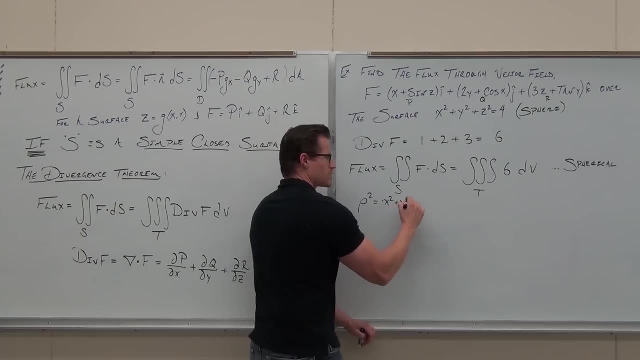 No, Rho, Rho, Rho, Okay, Rho, squared is what? Okay? So if rho squared is x squared plus y squared plus z squared, then from right here rho squared is 4 and rho is 2.. 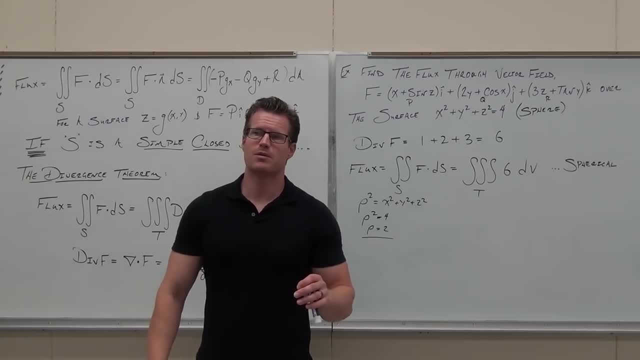 Rho always has to be positive. Does that make sense to you Now, if you remember this? the way that spherical works, you always do what first. We always do rho simple first, Then we do that phi and then we do the theta. 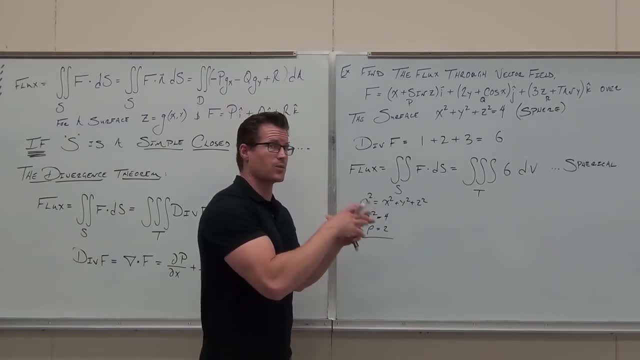 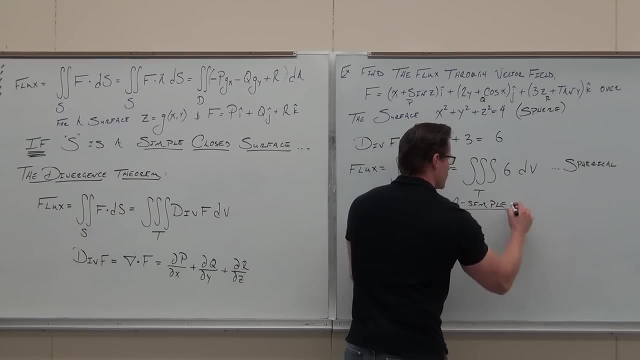 Is that ringing a bell to you? I'm going to walk you through because it's been a while, but that's got to ring a bell. So, firstly, we're going to do rho simple Now it should be pretty easy here. 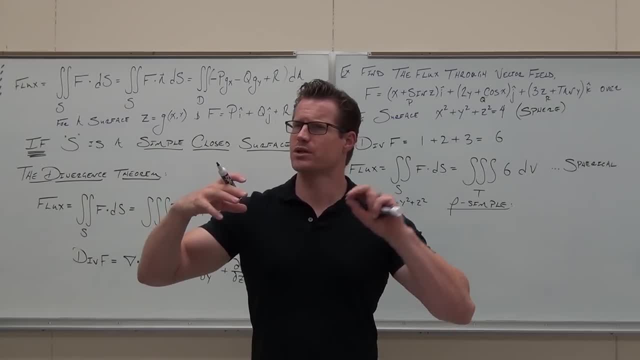 I mean, it's just a ball, guys. Our rho is going to go from what to what? Zero to 2.. It will be zero to 2.. But if you don't remember that or if it's hard for you to figure this out, I told you. 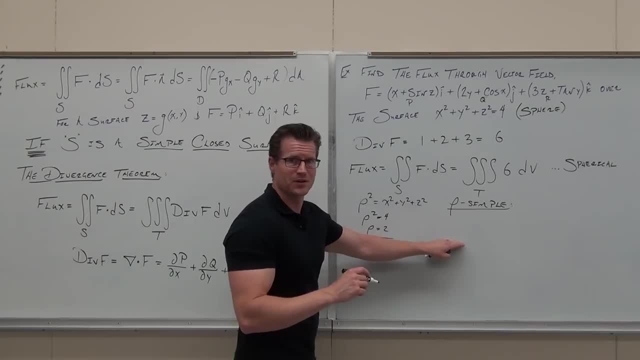 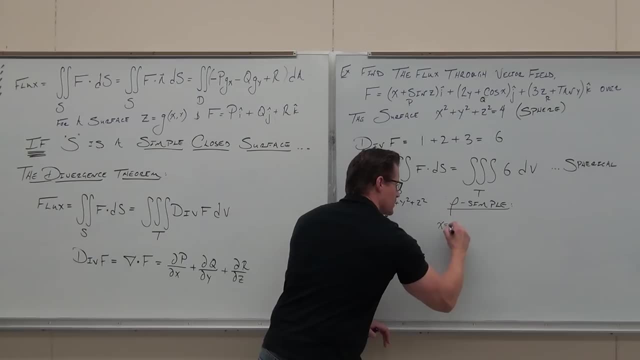 to do something I said for rho, simple, and for phi, simple. It's two for two birds with one stone. Set x, x equal to zero, and you'll get both. So if I set x equal to zero, what we end up getting? x equal to zero gives us this: 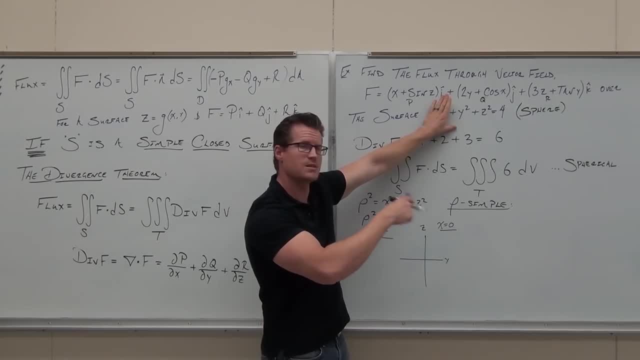 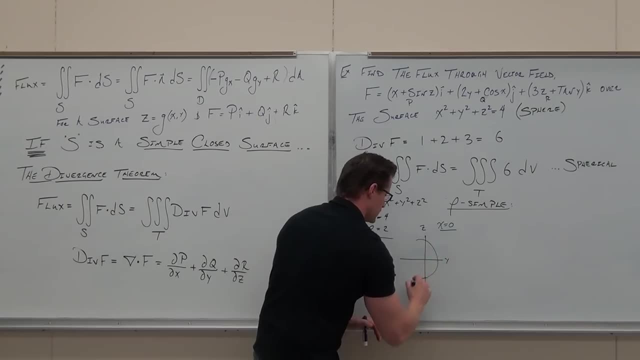 That's just a circle. That's the trace on the yz plane. Is this making sense to you? And it says: okay, it looks like this: 2 to 2.. The rho is the thing that goes from the origin through the root. 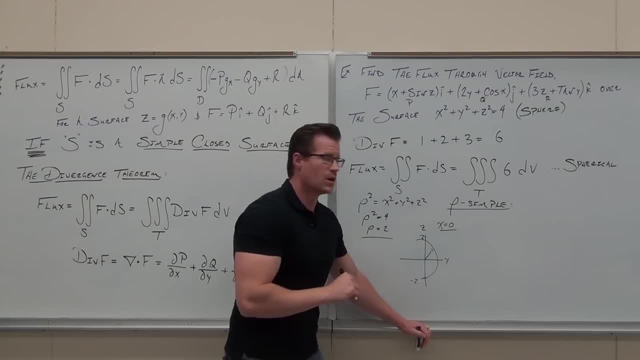 The rho is the thing that goes from the origin through the region and hits the outside of that ball. So the rho, for sure, is going from zero to, and another two with me on that one. But this also gives us our phi. Now, if you notice something, I haven't drawn the left side of this circle. 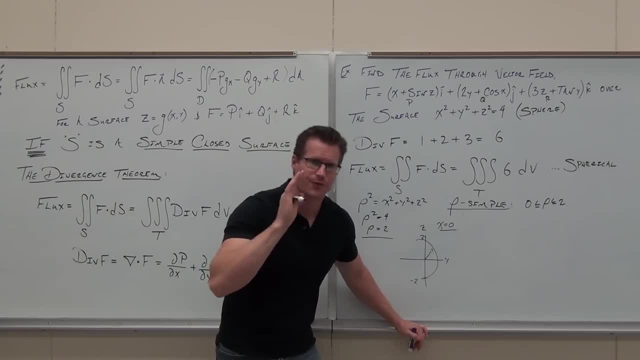 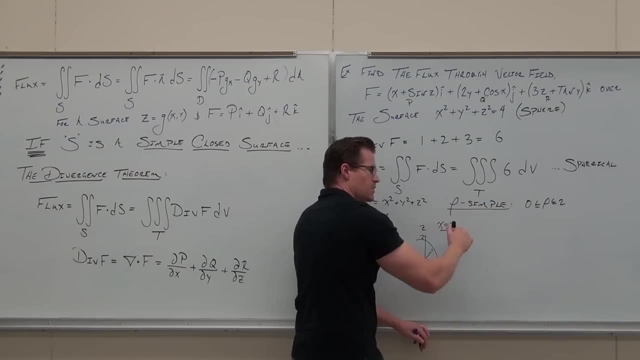 I do that on purpose, because our phi can never, ever, ever go past. what value Pi over 2.. Pi over 2. That's right. So this gives us two things. It gives us rho simple. Then it tells us that our phi 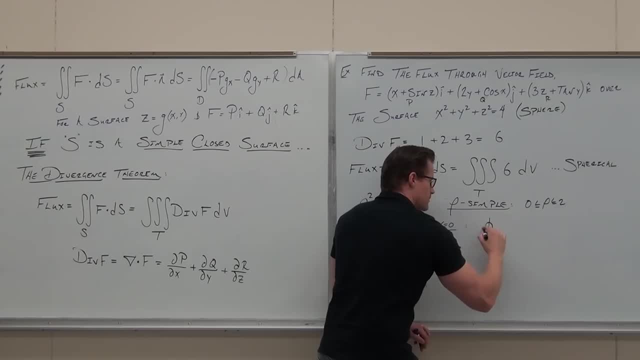 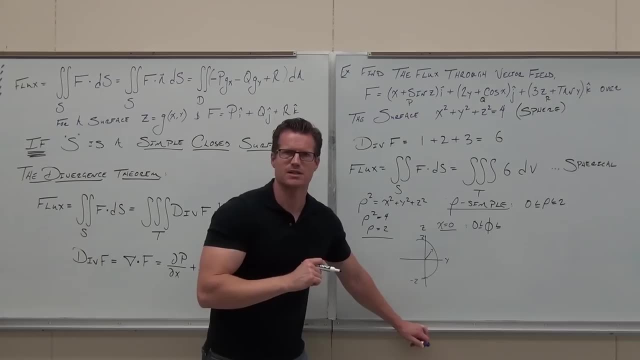 It gives us rho simple. Then it tells us that our phi, I'm sorry, What did you say? Did you say pi over 2? It should be pi, not pi over 2.. I said, yeah, you're right. 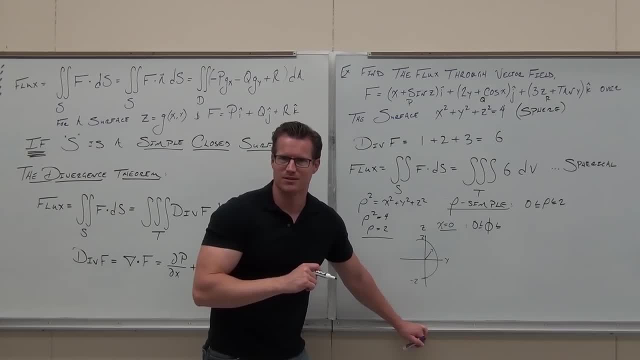 But I was just thinking that you had trusted you. That won't happen again. No, I didn't hear anybody. I was sure pi over 2.. I'm like, yeah, that sounds good, man. Last lesson, Let's get the flux out of here. 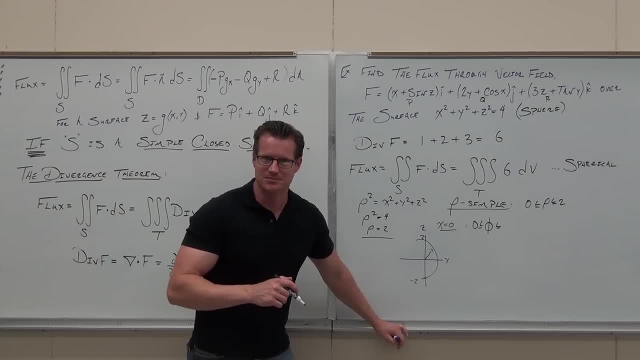 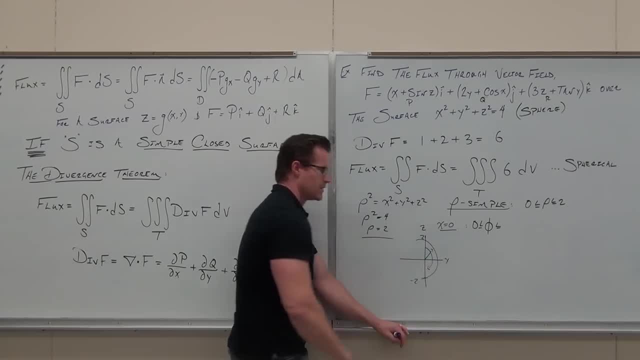 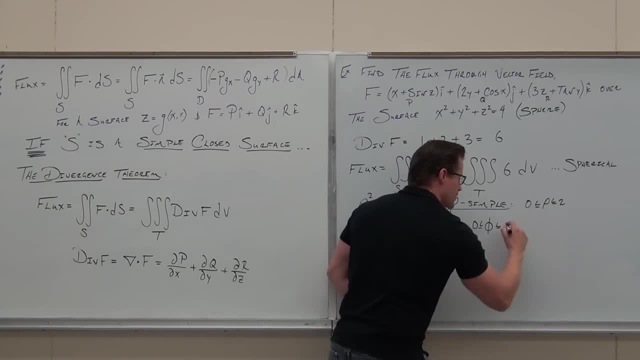 Make sense. So it goes from 0 to pi. Not 2 pi, But pi Make sense. Now, if you wanted to figure out what the theta is, Theta is always on the xy plane. Always, You set z equal to 0.. 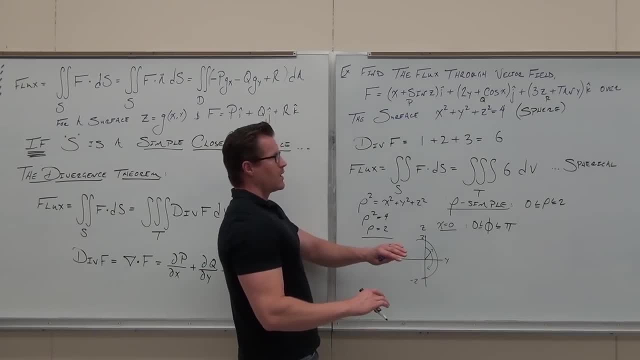 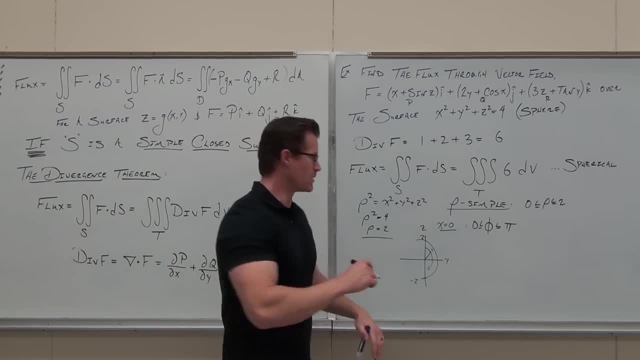 We're going to do it again. We're going to do it again, But you know it helps us out. with a little review right now. If we set z equal to 0, we get x, We get y, But look. 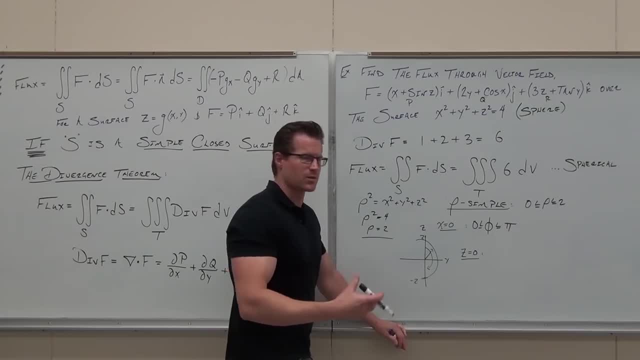 It's a sphere, guys. The traces all have to be the same. If it's centered at the origin, they'll get the same. So it's just going to be a radius of 2 again. Tell me something about theta. Does theta go all the way to 0?? 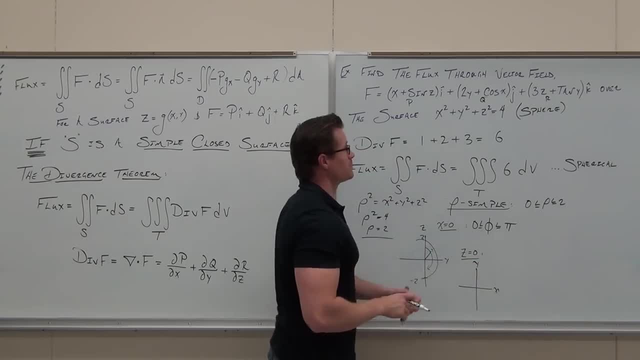 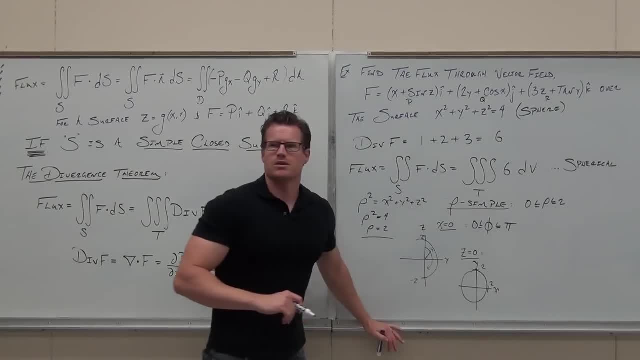 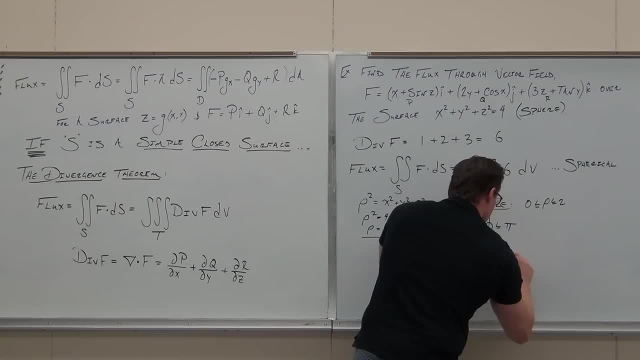 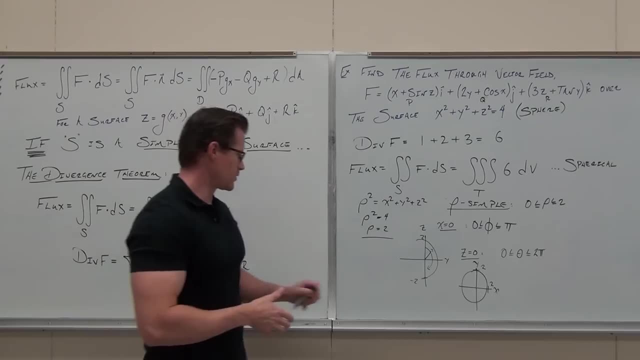 Yes, OK. So phi's the only weird one. It goes just from 0 to at most pi. OK, I'm going to stop real quick. I'm going to do a little recap, just to make sure you guys are with me. 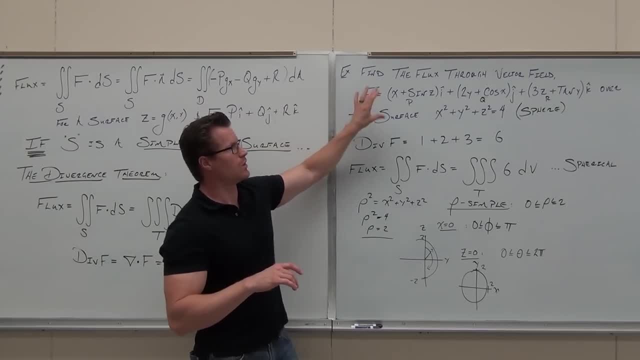 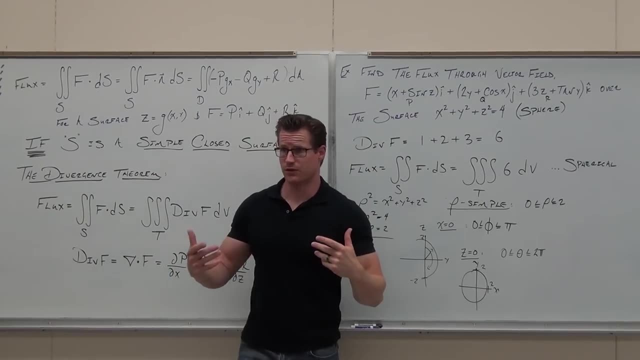 Firstly, we're doing a flux integral, That's a surface integral of a vector field over a surface And you go OK, Or the surface, And they go fantastic. Well, it's a simple closed surface. Divergence theorem applies. 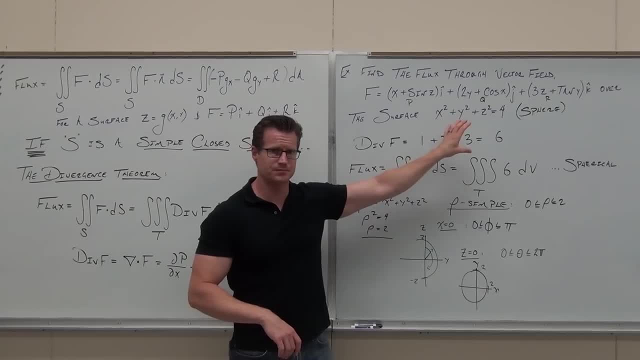 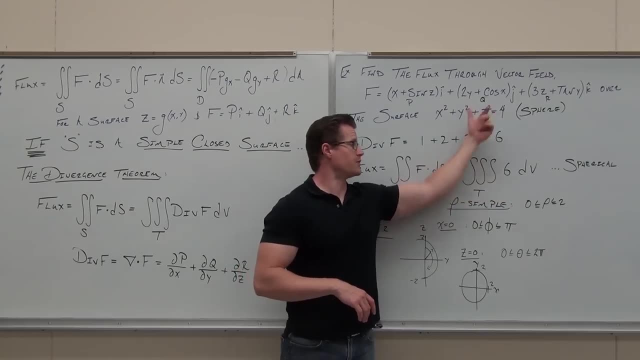 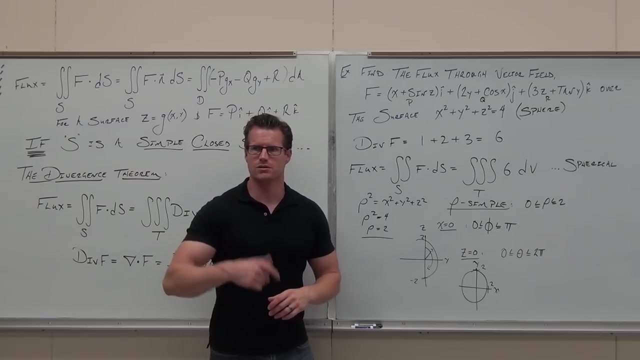 Find the divergence of the vector field. It's typically really easy: Parts and derivatives like normal. Put it right here as the argument of your triple integral And then define your surface, your 3D surface, like you normally would If it's a spherical. our rho is 2, 0, 2.. 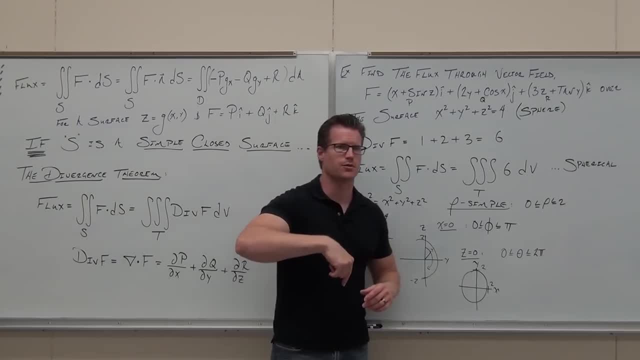 It's a full ball. We're going 0 to pi for phi, We're going 0 to 2 pi for theta, So that one. Can you please set that up appropriately? Set up our triple integral, okay, And then we're going to work it through. 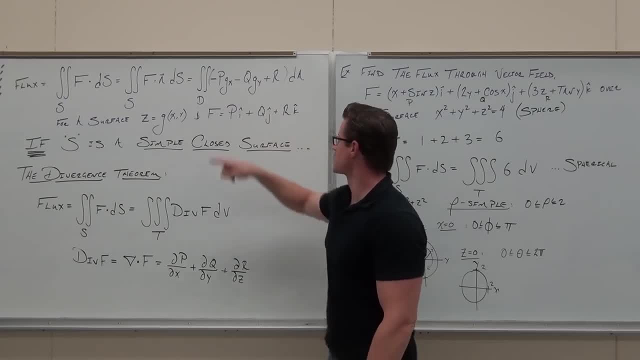 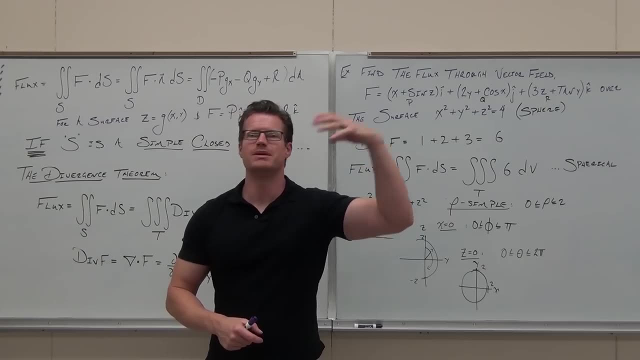 By the way, if you're wondering, just out of curiosity, why we don't use this for this example, When we start defining this in terms of z, we get that square root, the plus and minus. We basically eliminate half of our sphere if we choose one. 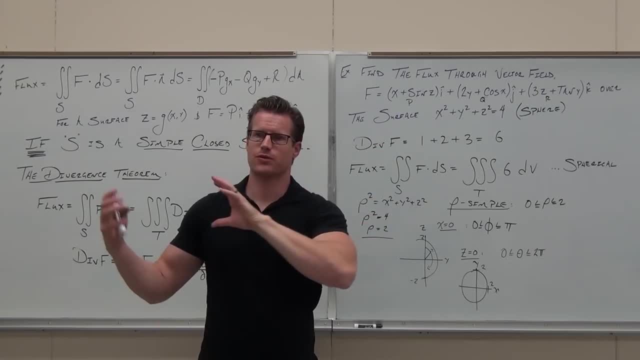 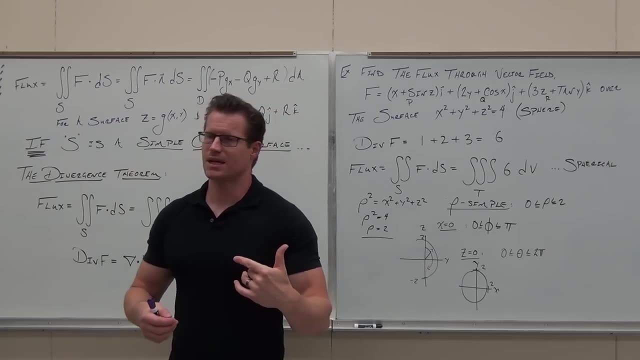 Does that make sense? We'd be eliminating stuff, So it's easier for us for simple closed surfaces oftentimes to use divergence theorem, so we don't have to start redefining our surfaces. That's kind of a nice idea. 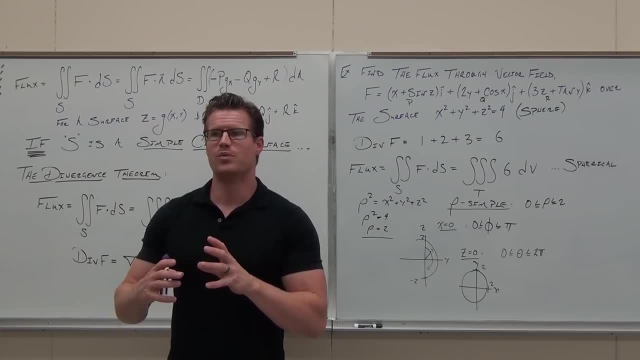 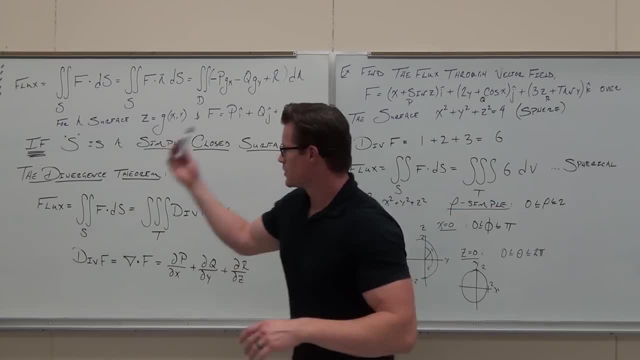 All right, All right, Okay, Did you set it up? Let's start doing it. I'm going to do it over here. Are there any questions on this? the divergence theorem from flux integrals: Do you see where it comes from? 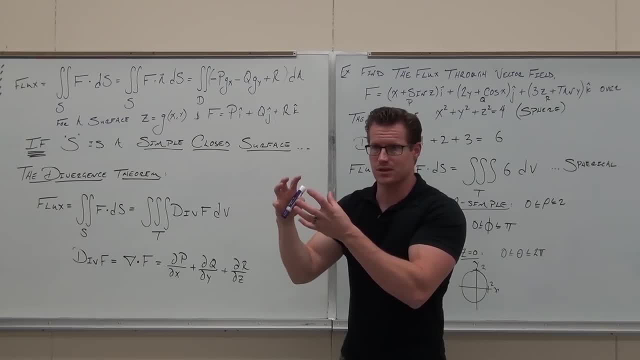 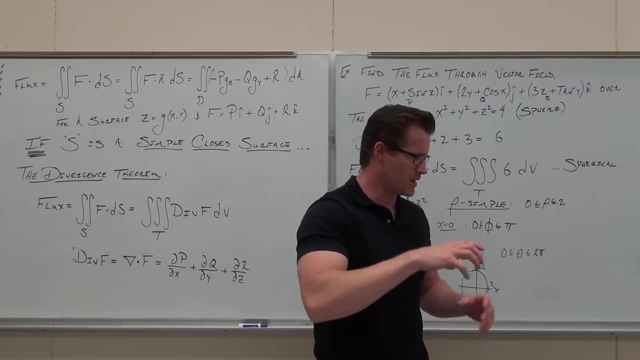 Do you see that it's doing the same thing? it's just over a very specific type of surface. Yes, no, Yes, Okay cool, Just like Green's theorem. Green's theorem was a specific thing of a very sorry. 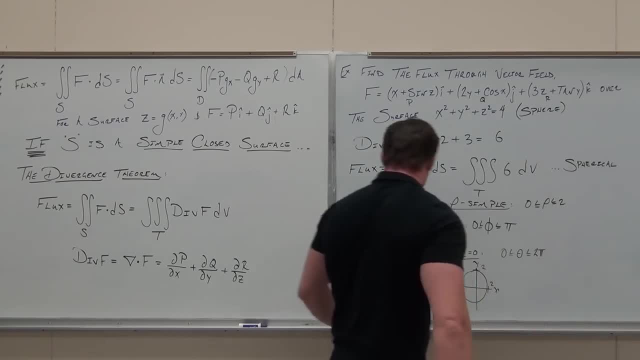 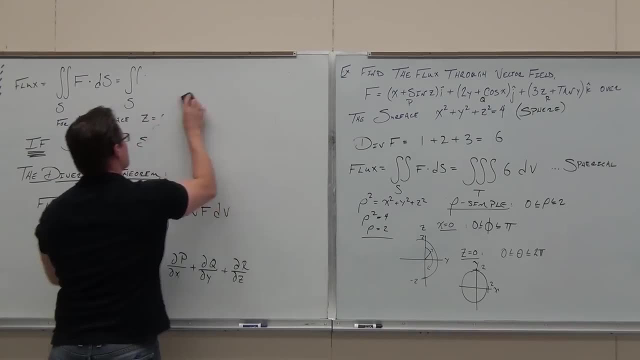 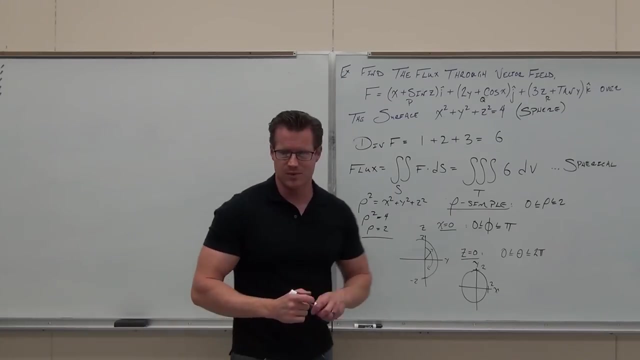 the same thing as a line integral. I put that just over a very specific setting where we had a simple closed surface, A simple closed curve. Okay, tell me, come on, you only get like two more times to show me that you know this stuff. 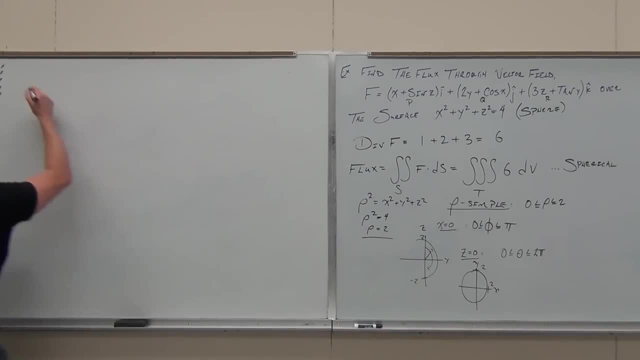 Tell me how that thing turns into a proper triple integral. What's it? look like A bit of a triple integral, Yeah, okay, yes, A little bit of a triple integral, Triple integral. Six, six, rho squared sine Six. I like the six. 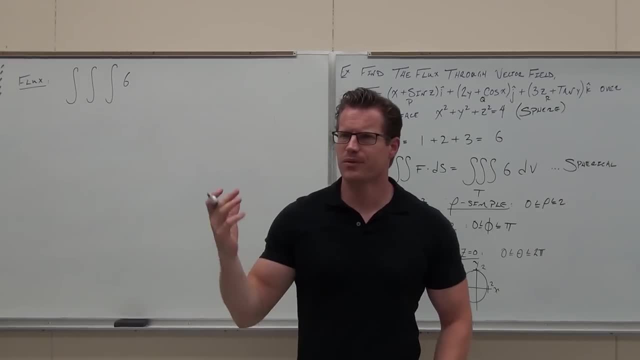 Wait, wait, I'm sorry. What's the next thing you put up there? Rho squared sine phi. Why did you put rho squared sine phi? Jacobian, Jacobian, Jacobian, Love, how you said Jacobian. Yeah, that's Jacobian. 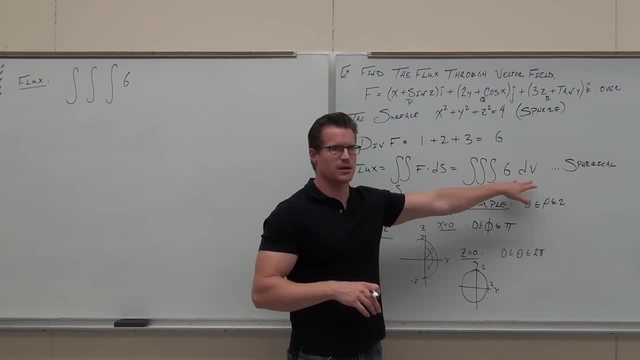 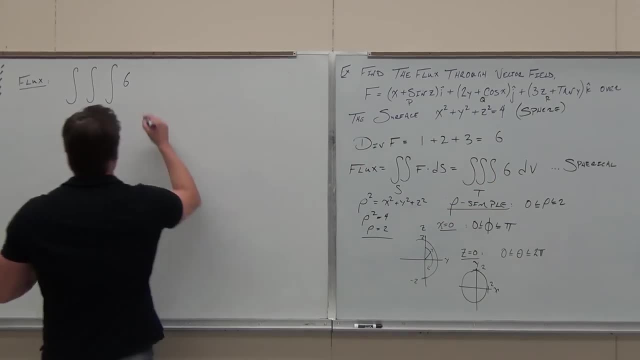 It's the way we transform dv- something that's just a three-dimensional volume of that region- into spherical, So it's got to be there. every single time we do that: dv, dv, dv, dv, dv, dv, dv. 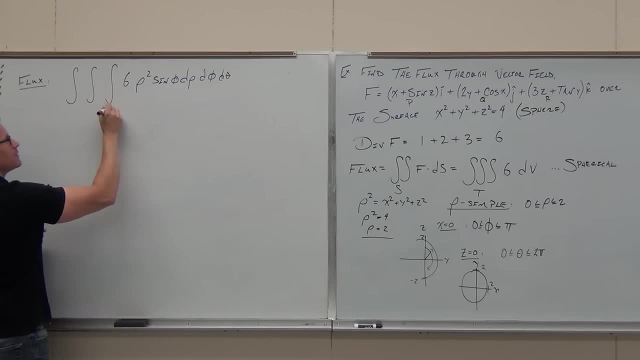 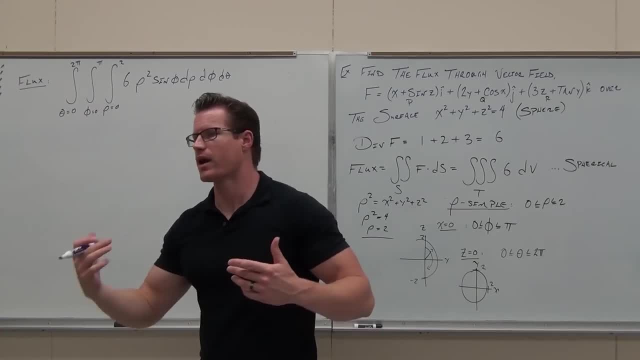 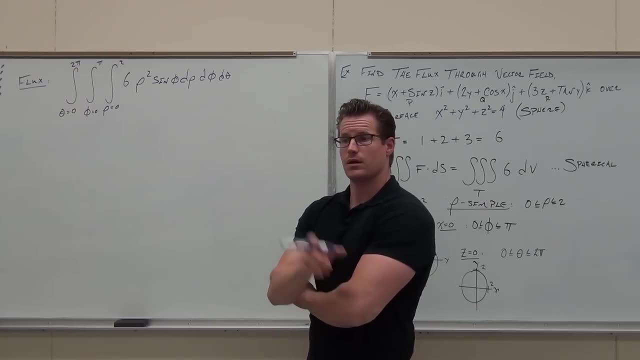 I want to see you work this one through. Let's practice this. We haven't got a ton of practice with spherical in a while. Let's work it through together. What's the first thing that you would do? So when we get the rho, we'd have that rho cubed over 3, yeah. 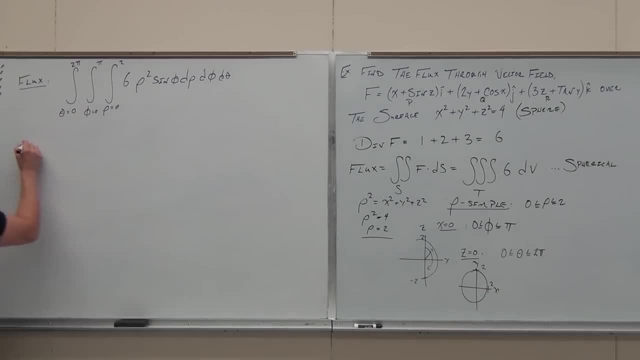 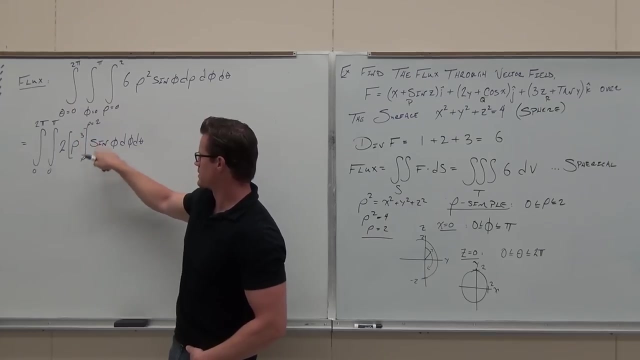 3 with a 6 is going to give you 2.- 2. And then our row is going from 0 to 2, from 0 to 2.. If you plug that in- yeah, I plug in the row- that's going to give me 8,. this is going to. 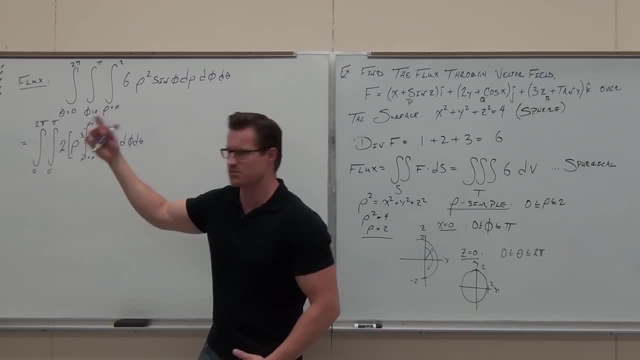 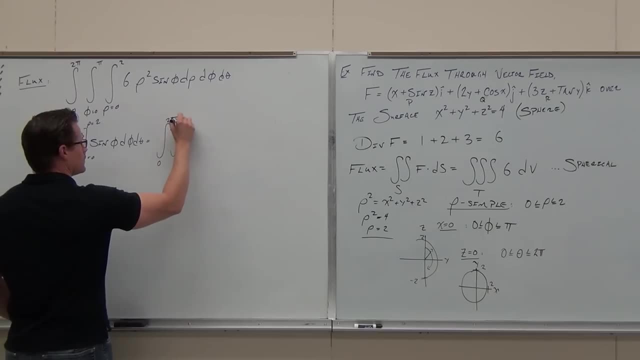 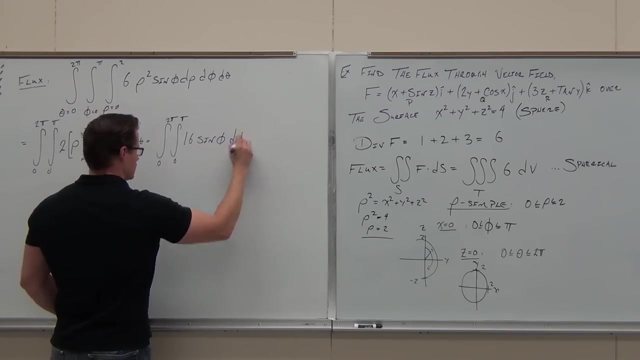 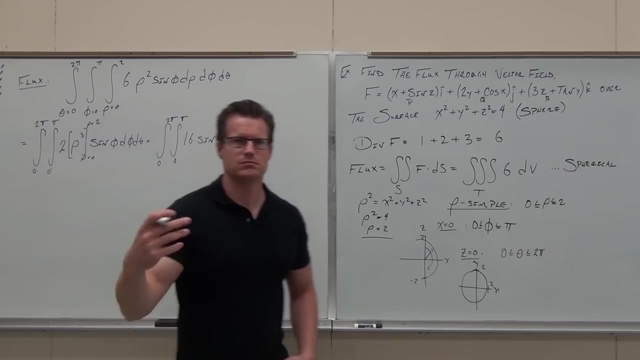 give me 0. So I'm going to just have 8 times 2, I'm going to have 16 there. did you guys get the 16? Sweet. Next up, let's do that one Real quick integral of 16 sine b d phi, what's that? 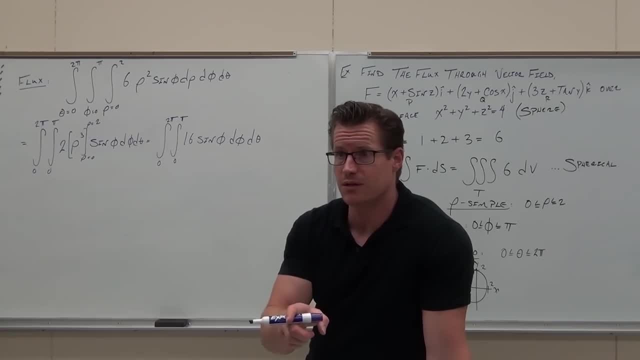 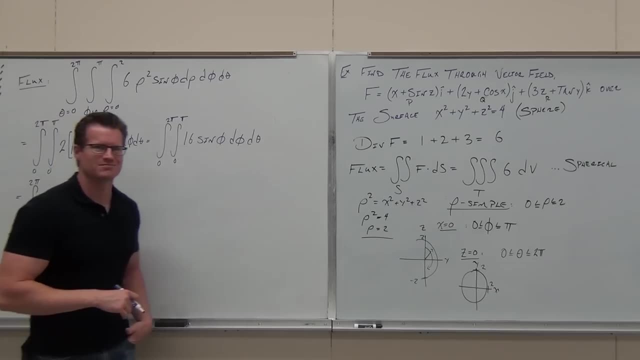 Negative, Cosine, Negative. Did you catch the negative? It's a big deal, Man. it sucks to get all the way down here and do something silly, right? It's like: oh yeah, it's cosine, yay, Well, the derivative, yeah. so then it goes backwards. 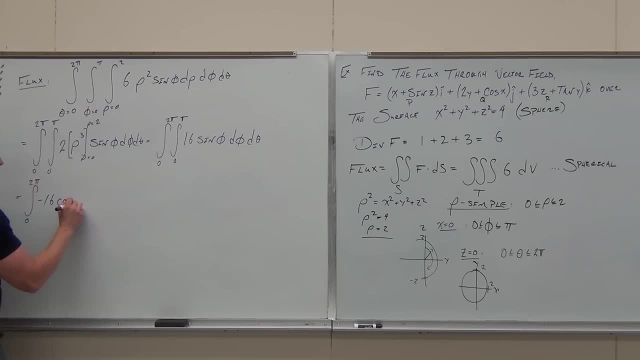 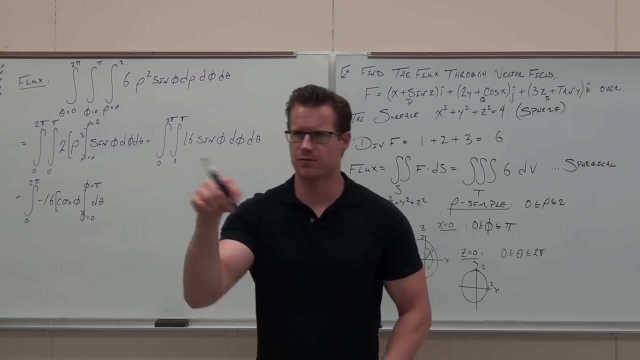 So here we have negative 16 cosine phi and then we're going to evaluate that from phi equals 0 to phi equals pi d theta. Okay, Cool, Hey, what happens? what happens when you plug in cosine of pi Negative 1.. 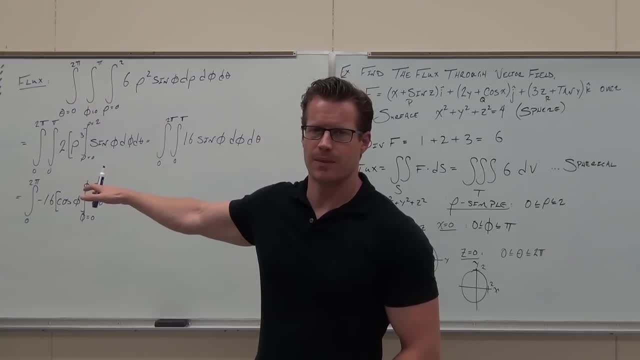 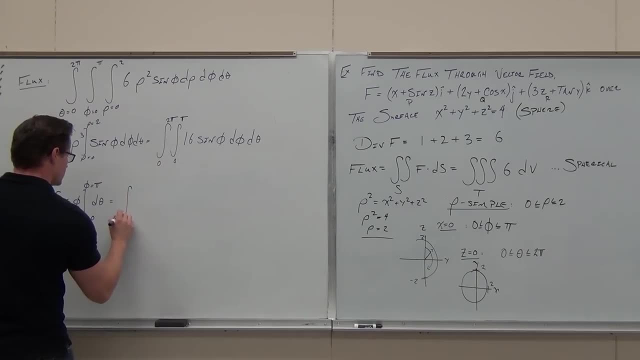 But then with 0, you don't have to plug that in, right, No, Or do you? You do, Why do you? It'll be 1.. It'll be 1.. Okay, So I got the negative 16, I've got. cosine of pi is negative 1, minus cosine of 0 is. 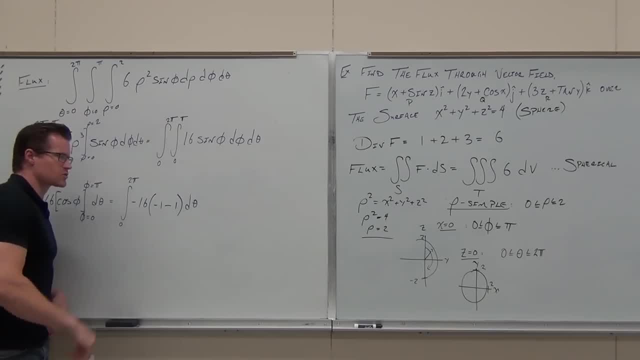 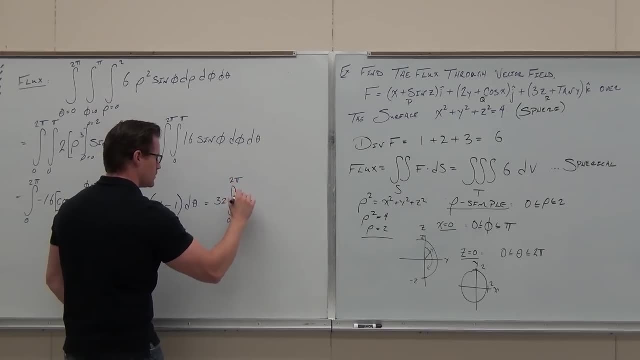 1. If we don't let our signs screw us up, that's 32.. Negative: 2,, 16,, 32. That means that we're going to get, if you look at it, we have this 32 theta and we're. 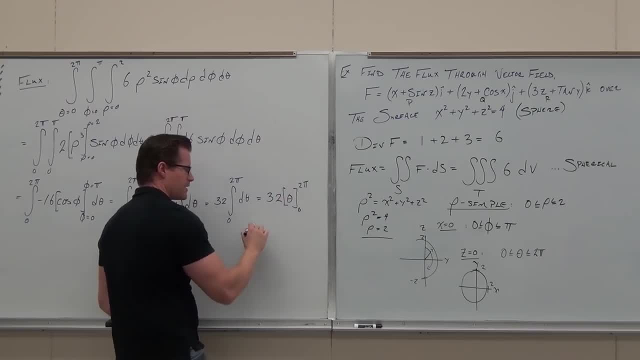 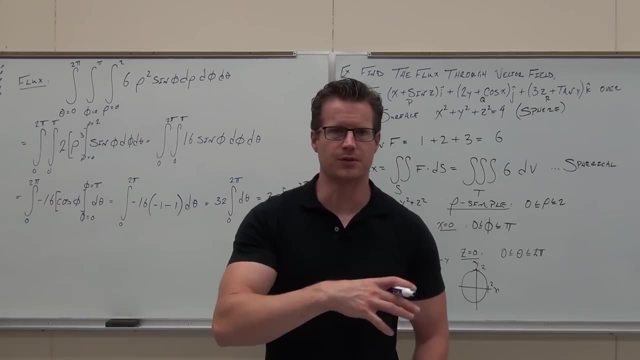 just going to evaluate that from 0 to 2 pi. How much is? our final answer: 66.45.. And then we're going to get the flux across the ball of that vector field is 32 pi cubic units per unit of time. 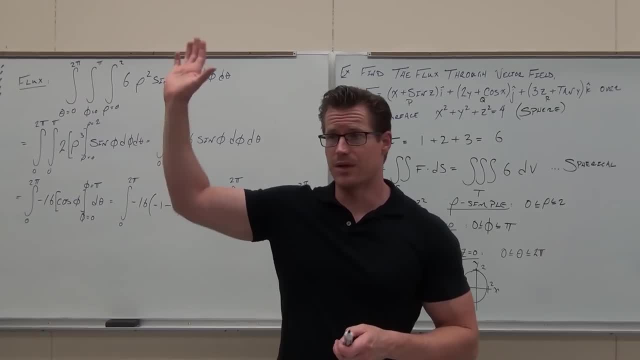 That's the idea here. That's what's happening. Should the fans feel all right with that one, I'll tell you what I'd like to do. I want to try one more. I'm going to have you do most of this stuff and then we're going to do the last theorem. 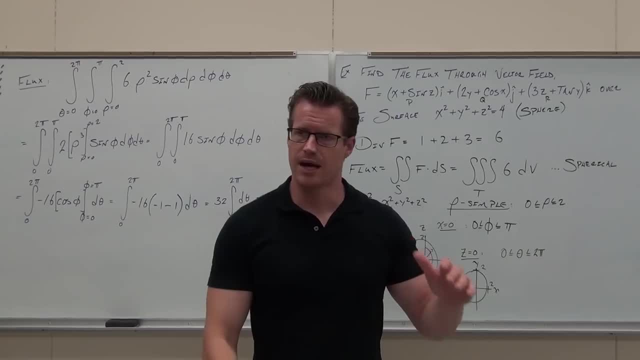 the last example: Just get the chills a little bit. Kind of cool, You're not as excited as you should be. This is freaking awesome. All right, Goodness, Any questions? So we're going to start here and work that way. 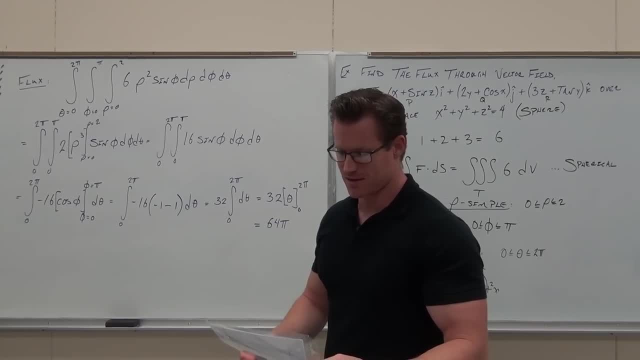 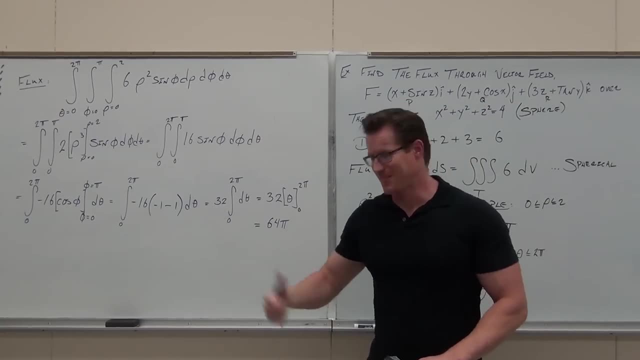 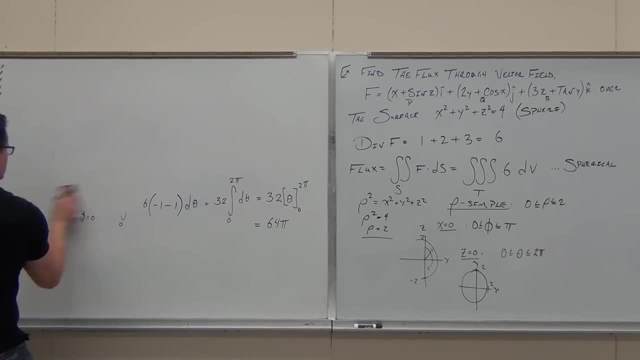 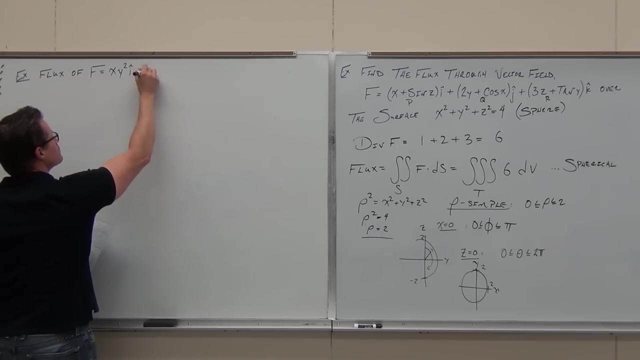 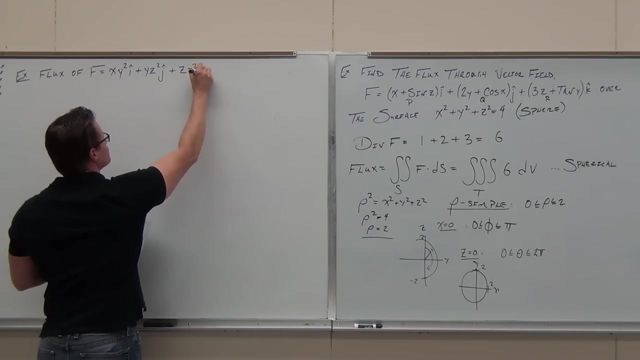 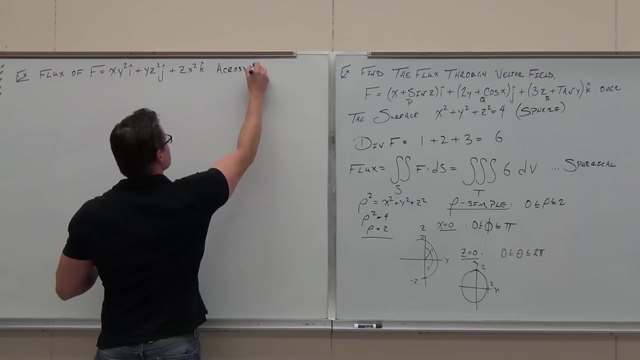 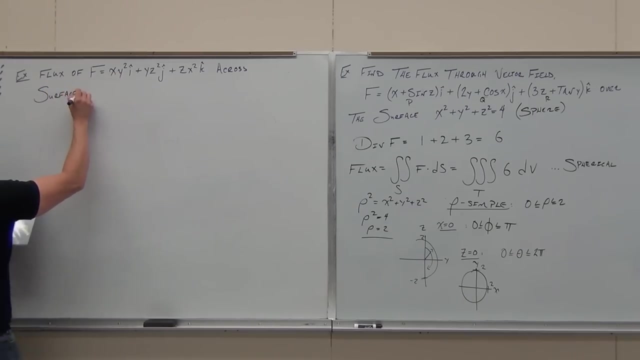 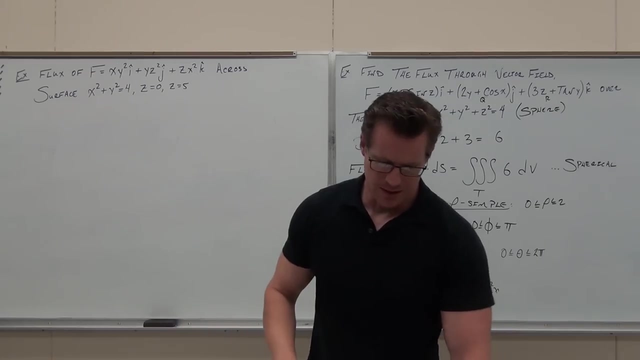 Yes, OK, All right, We got everything. We all got it, All right. Thank you, Okay, come on. I asked you to kind of put all this stuff together, so I want you to answer the question. this time I'm asking you for the flux. 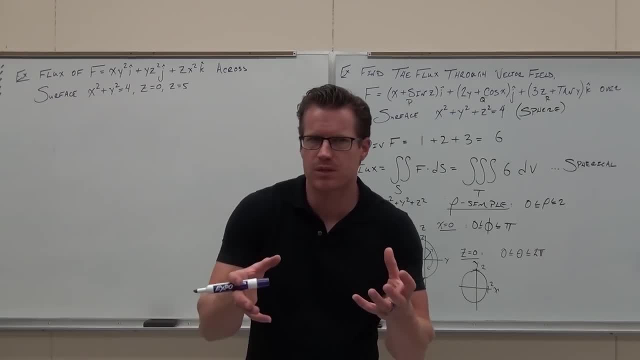 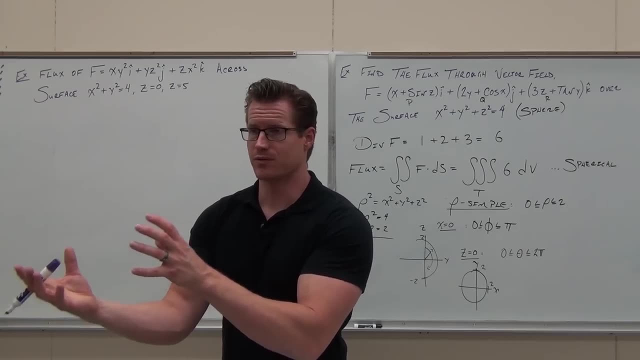 What's that mean? What gives us the flux? What's that mean? Surface integral of the vector field. Very good, Do we have a vector field? We have a surface Surface integral of that vector field, for that surface gives us the flux. 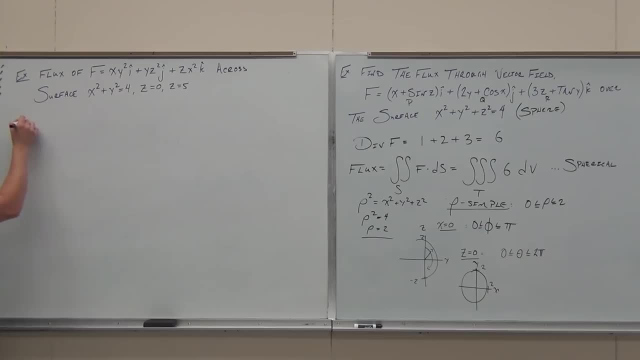 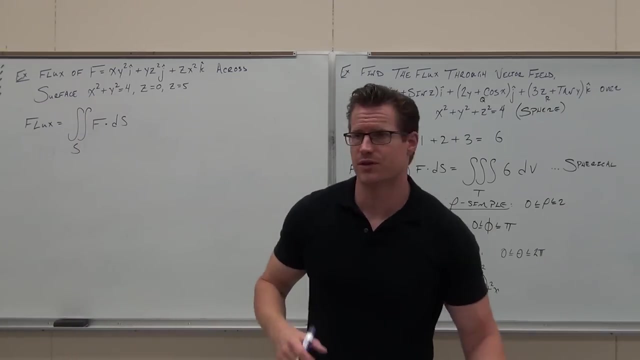 So I know, I know that this integral because of what we talked about, I'm sorry, the flux is a surface integral of that vector field over that surface or across that surface. That's what's happening Now. we're going to try to make it easier. 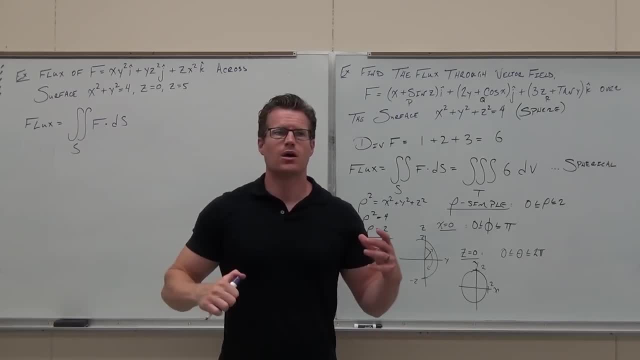 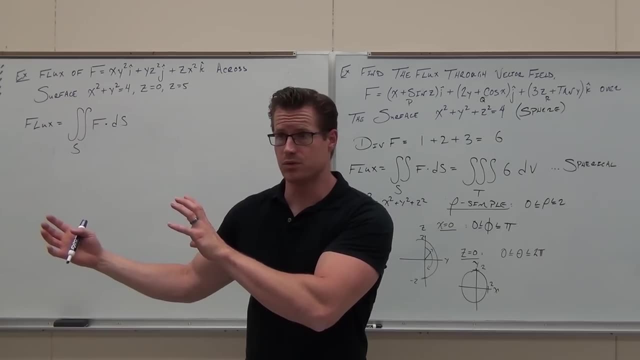 because this thing doesn't have to be real nice for us. So there's two thoughts: Either we have a non-simple closed surface in which we cannot use, or we have a non-simple closed surface in which we cannot use the divergence theorem, Divergence theorem- and we have to go back to the old stuff. 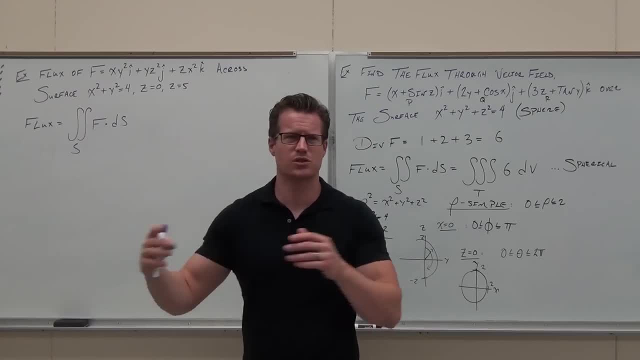 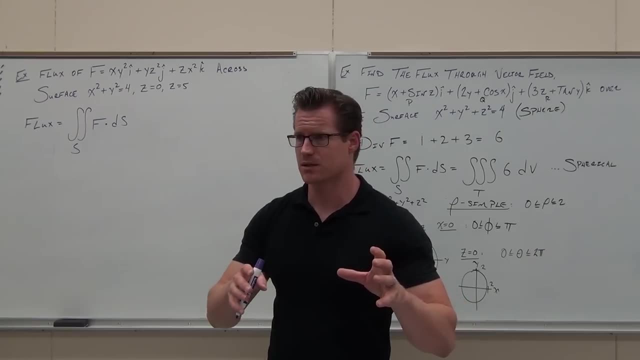 Oh, we do have a simple closed surface and we can use the divergence theorem. So, number one thing: recognize what you're doing, man. If you're doing flux, you're doing a surface integral of a vector field over surface. Make sense to you. 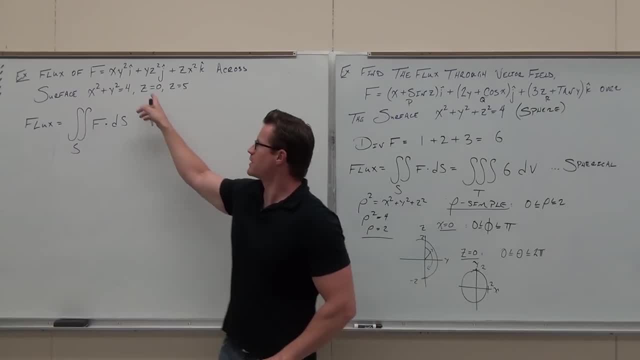 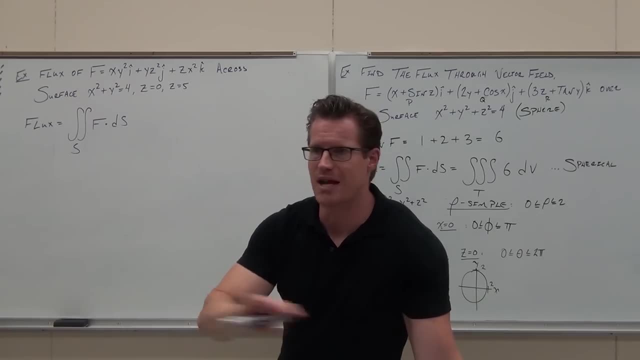 Then we start looking at the surface. Well, what's this look like? If I'm looking at the surface like that, this goes all the way back to Chapter 11, your understanding of surfaces. Do you recognize that this has never left you the entire class? 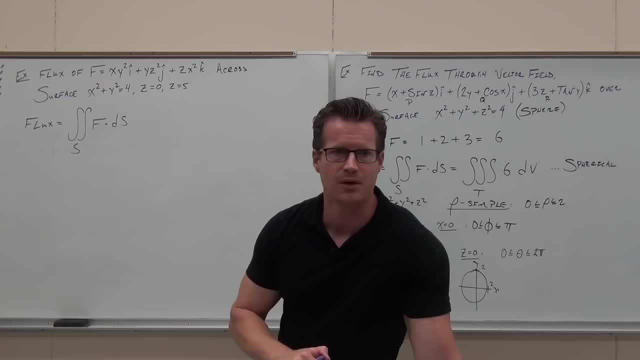 You've always gone back to how you think about graphs. It's crazy, right? I told you it was important. Sometimes it doesn't sink in until, oh my gosh, Like every chapter, we have done the same exact thing: dealt with these surfaces. 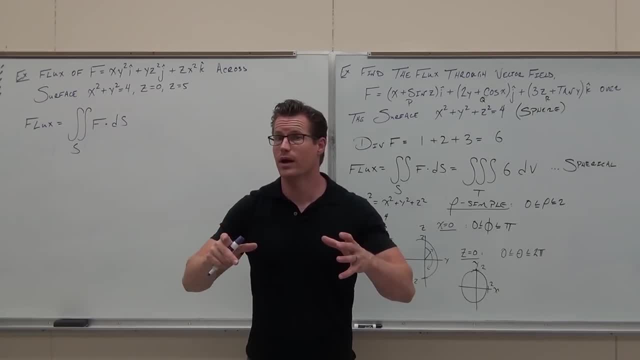 What is that Cylinder? Ah, Cylinder. along what axis? The axis, What's this? A plane? It's xy-y. It's xy-y. What's that one? The xy-y. So this is a cylinder with a top and a bottom, a basic, just a basic cylinder. 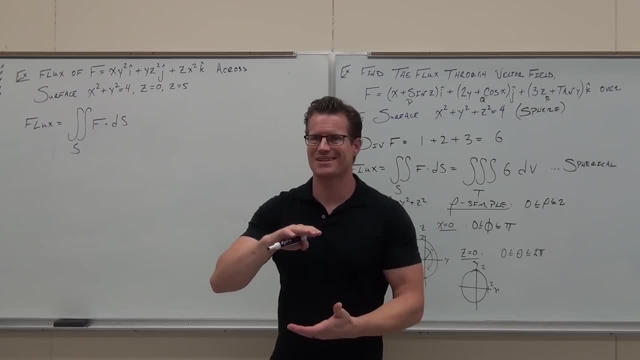 It's a soda can. Yeah, it's like a soda can with a top and a bottom. Does that make sense to you, Is it? Well, now, how about this one? If this is a surface integral of a vector field, does divergence theorem apply for us? 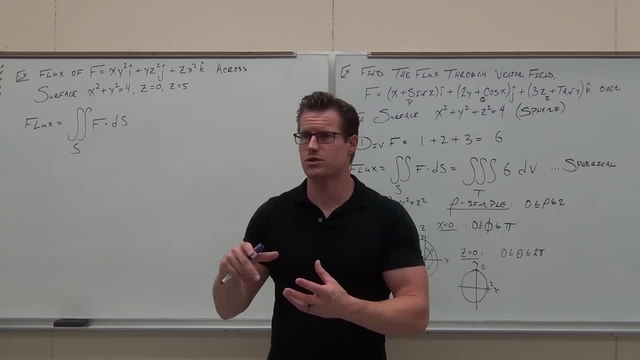 Yes, Is it a simple closed surface? Yes, It doesn't intersect itself weirdly but basically cross like a curve would cross. It doesn't do that. It's closed. so if you had a soda can, nothing's coming out of the soda can right. 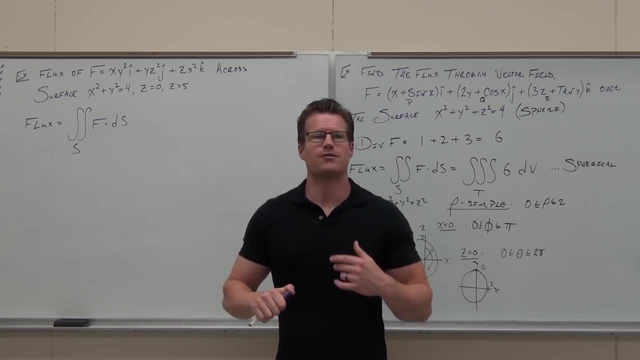 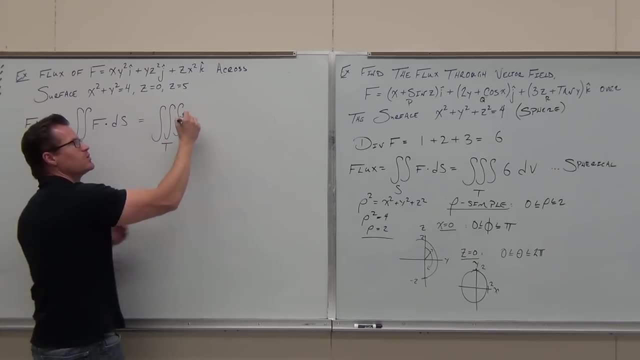 It's a closed thing. That's what this thing is. So divergence theorem: Divergence theorem does apply and what I want to do right now is show that divergence theorem does apply and then we focus on setting it up. Right now, I want you to do the complete setup, please. 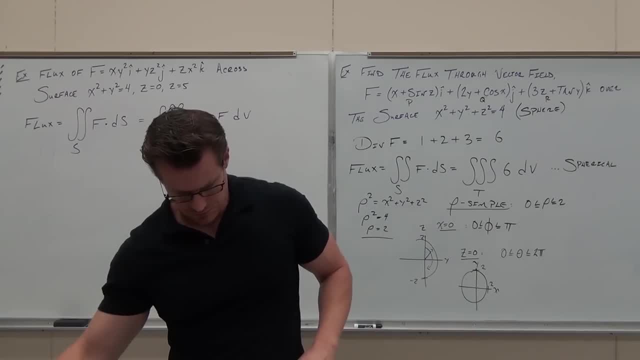 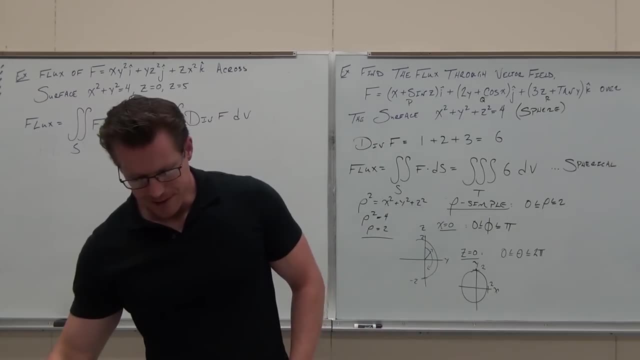 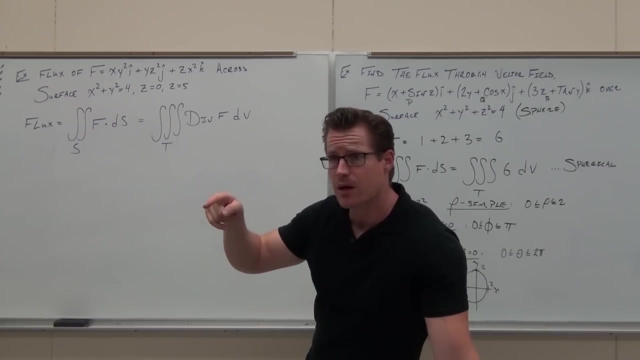 So, as you're working, I'm going to be talking. so when we do this, will we recognize a surface integral of a vector field? We look at the surface first. If it's a simple, closed surface, this is typically the easiest way to do it. 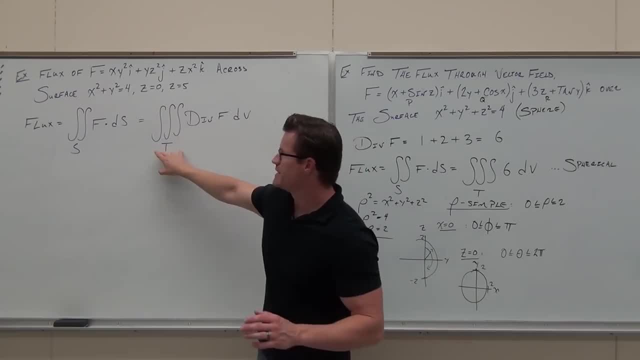 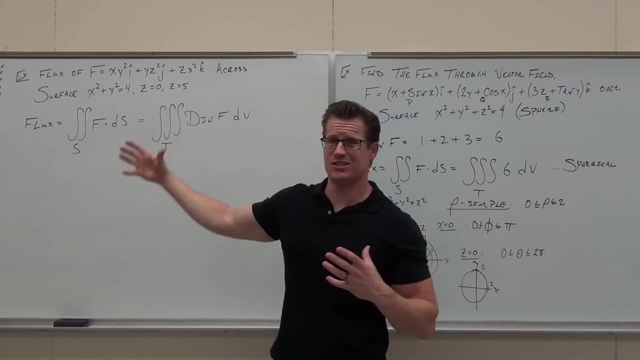 Divergence theorem makes it easier. You set up a triple integral where your 3D region is the surface, and that's nice, because we know how to define that really easily. Divergence of F- that's easy to do, guys. 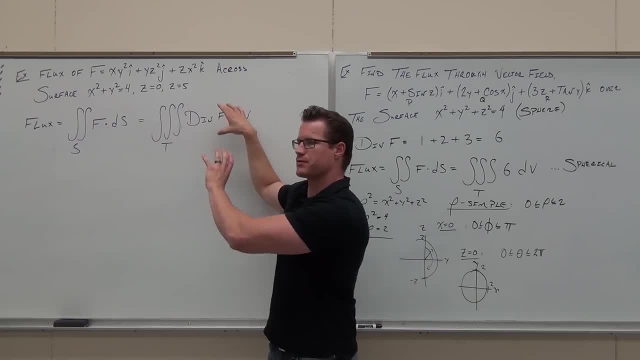 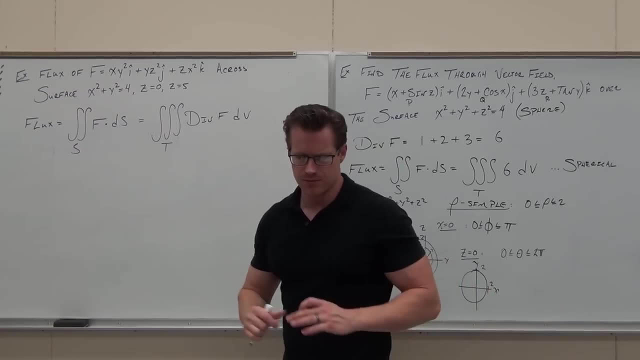 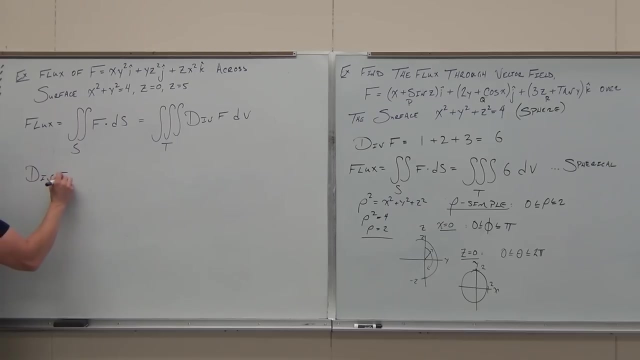 That's partial derivatives. and then, once we translate it by divergence theorem, then we start looking at the region. not before that, not before that. Have you made it through the divergence of F? Yes, I always write off to the side and make sure that I get this thing right, because it's 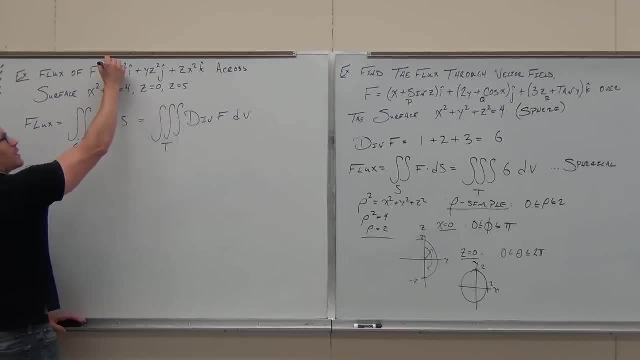 irrelevant if you know what you're doing after that. if you don't get that right, I'd probably label this P, Q and R. I want to take the partial derivative of P with respect to what X, So that gives us. 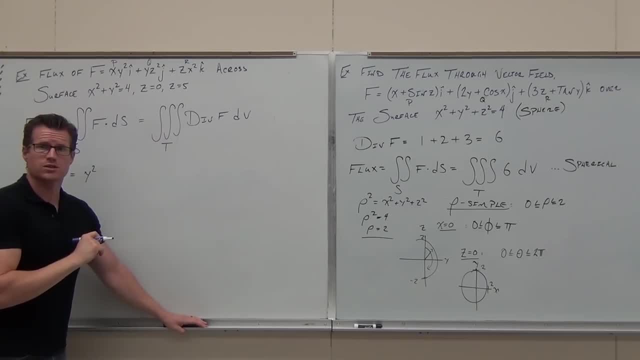 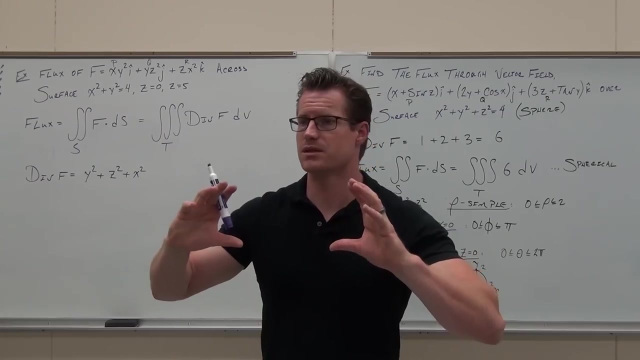 I, I or not. No, The products don't give. I's Plus, I, I, I, I Plus, I, I, I Plus I, I, I Plus. Perfect, That's great. 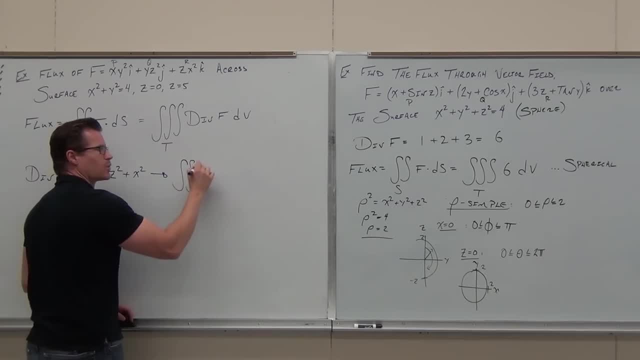 That's all you got to do. That literally becomes your integrand what's right inside the argument of your triple integral? Let's translate it. I know that, our triple integral. I'm not even worried about the region right now, I'm just 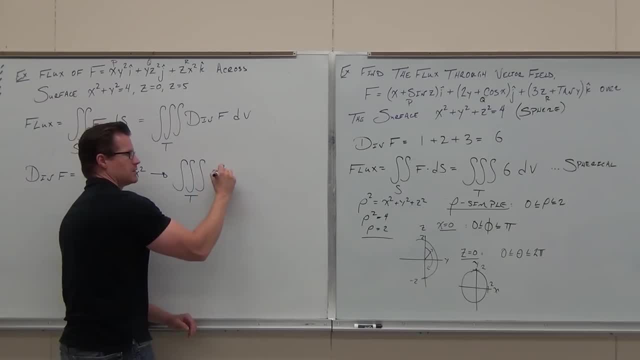 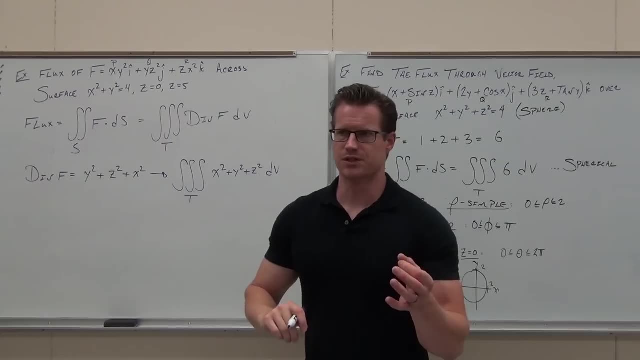 going to write this. I'm going to write this here, I'm going to leave it dv and then I'm going to start looking at the surface. Now, hopefully you recognize I'm doing this on purpose. I'm giving you a lot of the old concepts to refresh your memory for your final. 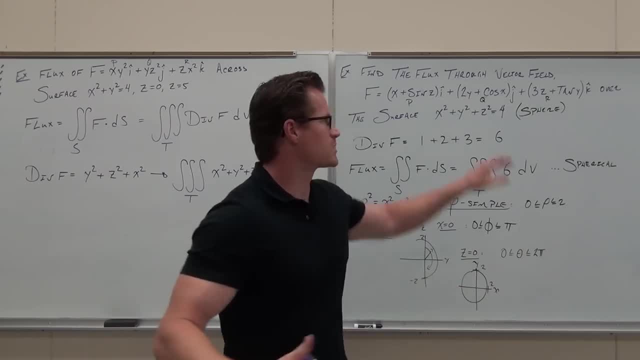 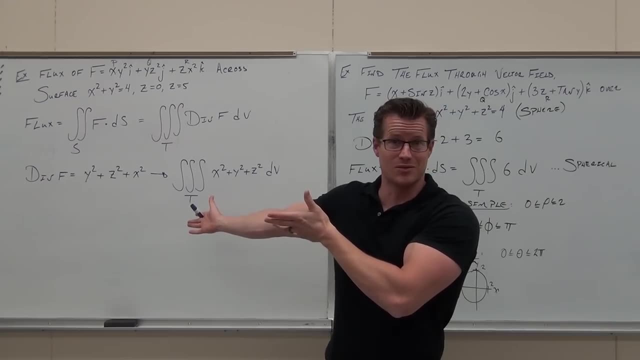 That way, we're getting some review in right now and you're also seeing: oh, spherical still applies. Is it a big surprise? we're going to use cylindrical with a freaking cylinder. This is why it's nice, because if you use divergence theorem and you change 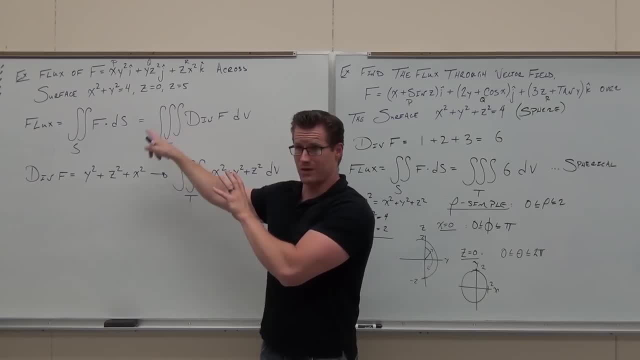 if you change the surface into a triple integral, where it lets you easily deal with the surface, and you've got things like spheres, you get spherical Things like cylinders. hey, we can use cylindrical coordinates for triple integrals. It makes it just very, very straightforward, very, very nice. 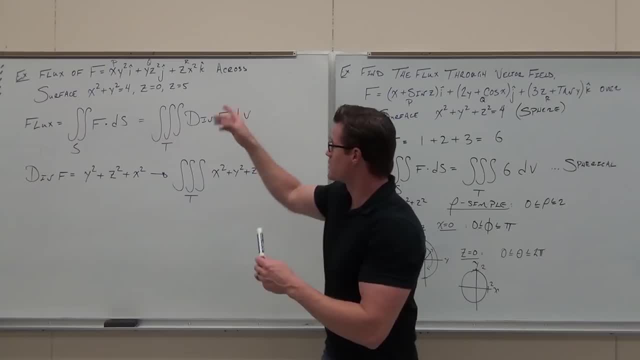 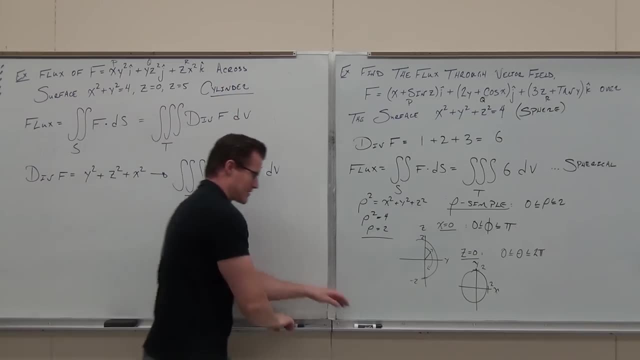 Are you seeing the point of doing this right now? So let's look at that. So this is obviously a cylinder, which means that, hey, we've got a 3-D region of the cylinder. We're going to be using cylindrical 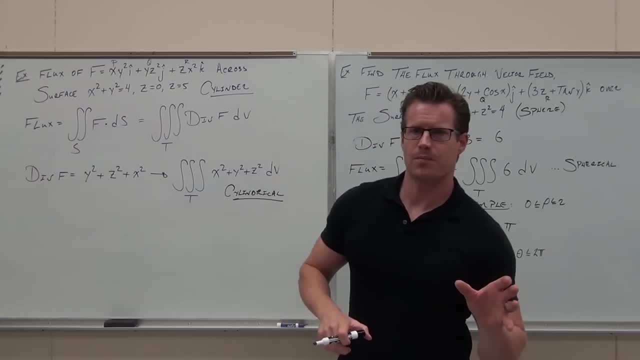 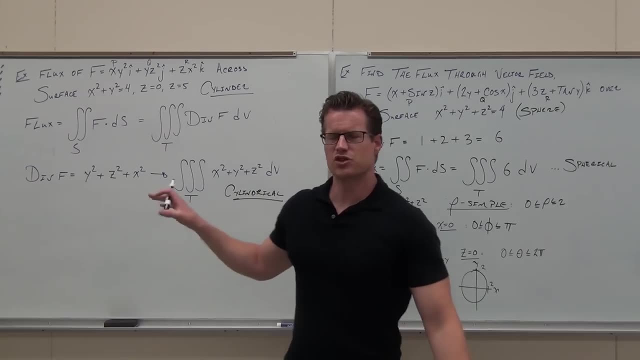 Now you might have to dig down a little bit on this one With cylindrical, with spherical, we did row simple first every single time With cylindrical. do you remember what we do first every single time? Z-simple. We have to use z-simple. 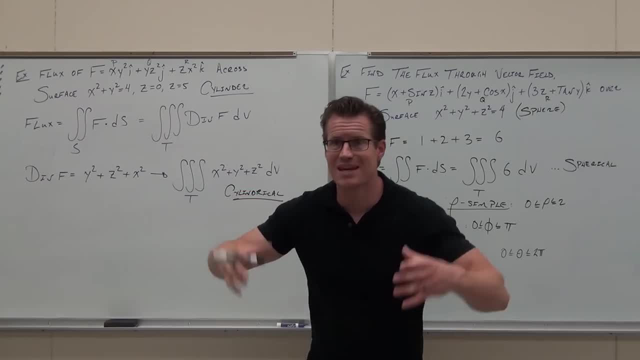 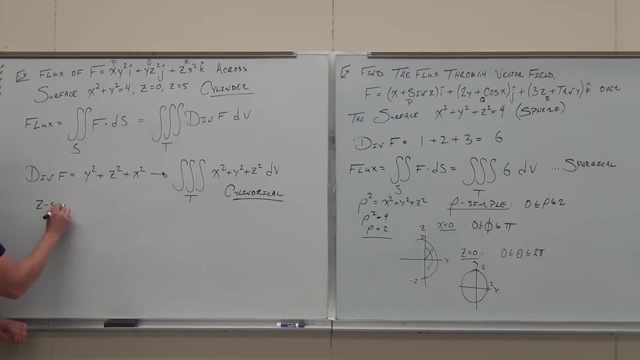 Is that convenient for us? Yes, Yes, With cylinders along the z-axis. yeah, you better believe it, That's awesome. So if we do z-simple, literally all we're looking for is: hey, we've got a 3-D region. 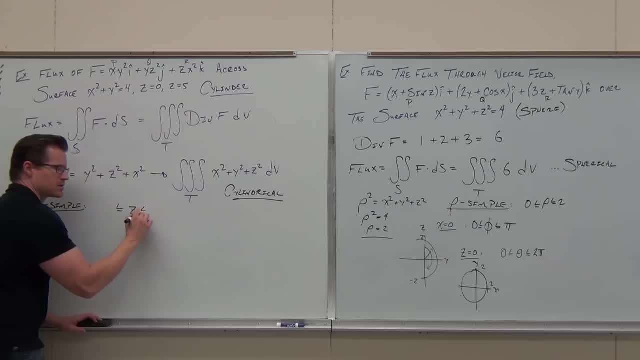 Hey, what two functions can we match z between? Well, that doesn't have any z's in it. That's 0,, that's 5.. It's literally right there in front of you Again. that's why this makes it nicer. 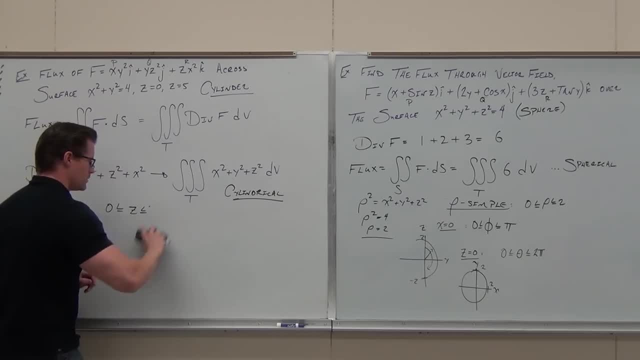 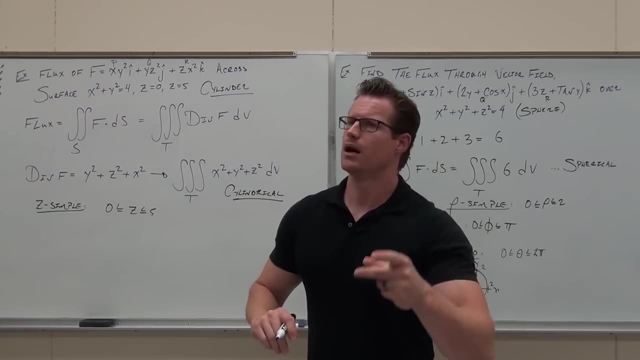 Not harder, not worse, nicer. Okay, next thing, Come on next thing. What's the next thing? The xy Before that? So I did z-simple and what I'm trying to do is set up my triple integral. 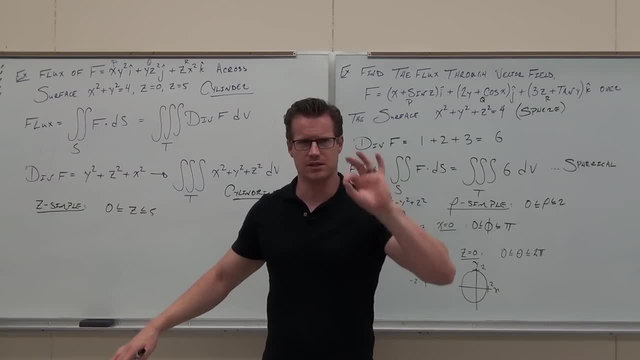 So cylindrical does z-simple first and then it deals with two other things. It deals with r and it deals with a. Okay, so we have to look at our region. If we're doing cylindrical and we did z-simple first, our region is on the what plane? 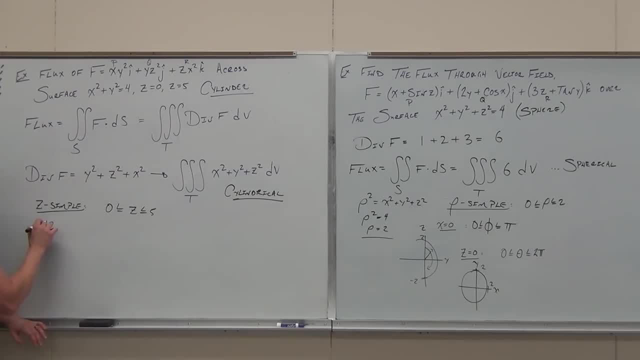 xy. Okay, So that means that I'm going to write it out the same way every time to keep consistency. r is on the xy plane, So let's graph that, Look for everything that has x's and y's and put it on that plane. 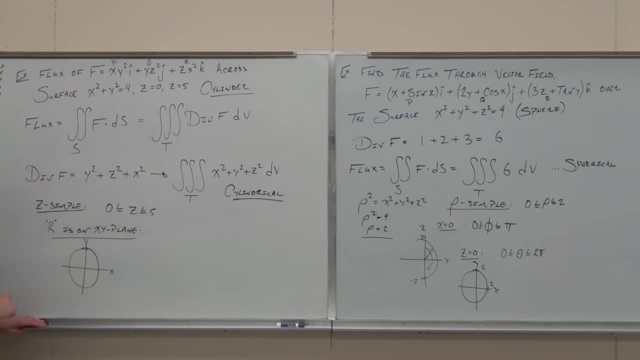 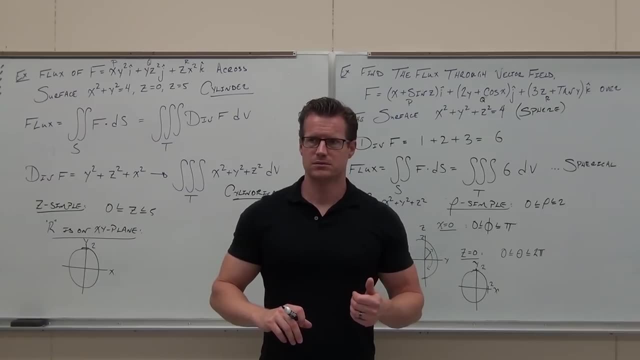 In our case it comes pretty nice. We have a circle with a radius of 2 centered at the origin, And then we go, hey, cylindrical is basically just take care of the z and you got polar. It's the same stuff. 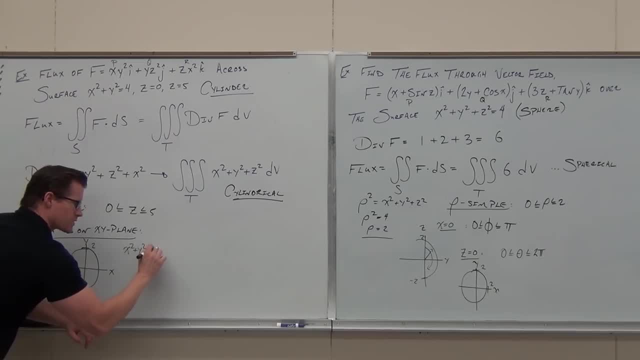 So when we start defining x squared plus y squared equals r squared, well, that means that r squared equals 4, or r equals 2.. And now we get two things. We have to match r. We have to match r between two functions of theta, and then theta between two constant angles. 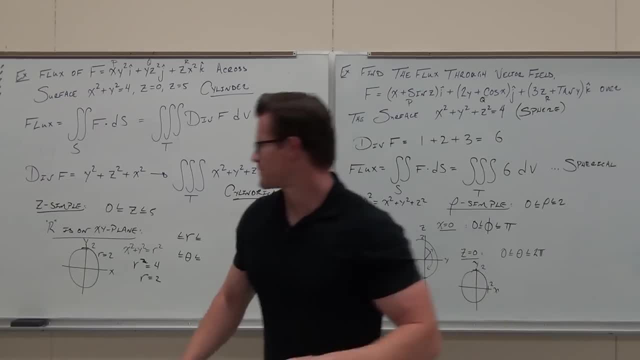 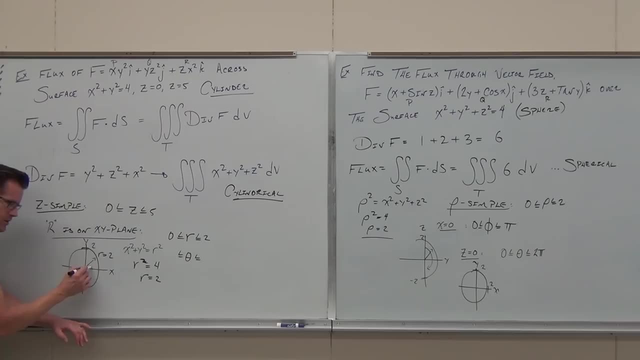 That's what we've got to do. What's the r between, between where and where? We've had so much work on this. So the r goes through our region, the xy plane from 0 to 2.. The theta goes all the way around. 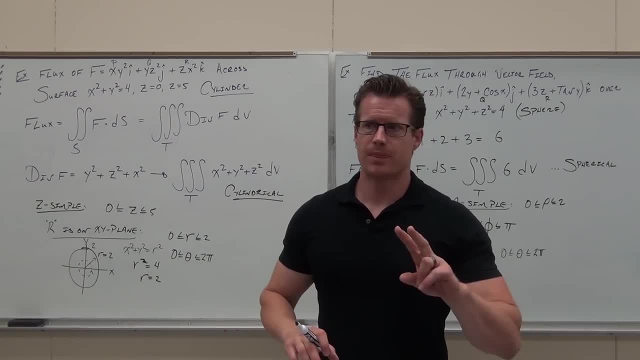 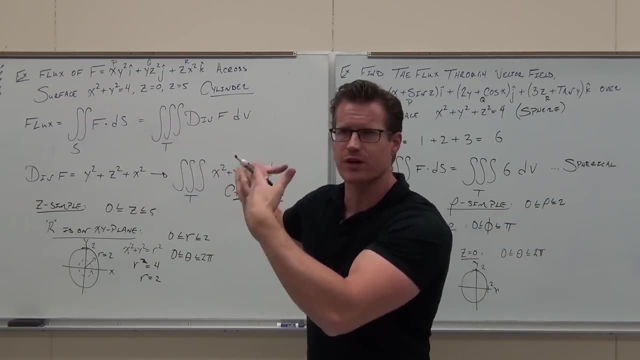 That's it. We're going to do two things right now. The first thing we're going to do is set, just like we normally did: set up the triple integral, set up the bounds of integration, Set up the d, whatever's over here. 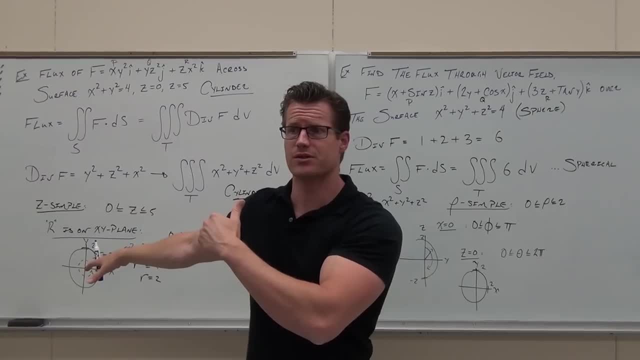 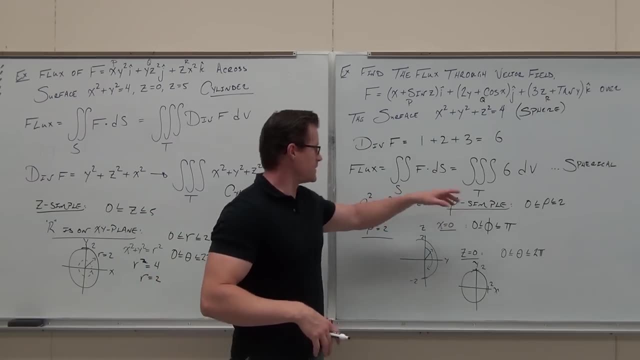 Make sure you understand that we are in cylindrical right now and we just changed to polar. That matters. Okay, the way I taught you was that way. I said we do z and then we have polar, So you're going to have something special up there, just like we had the d phi. well, 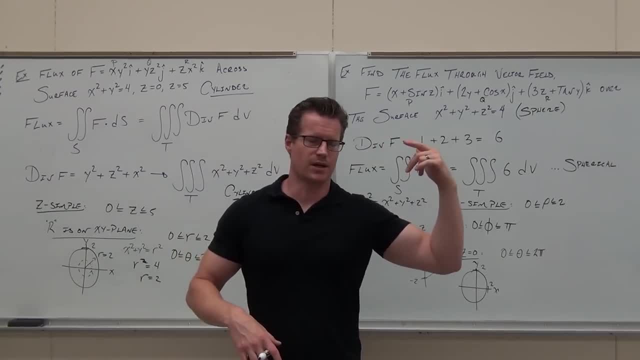 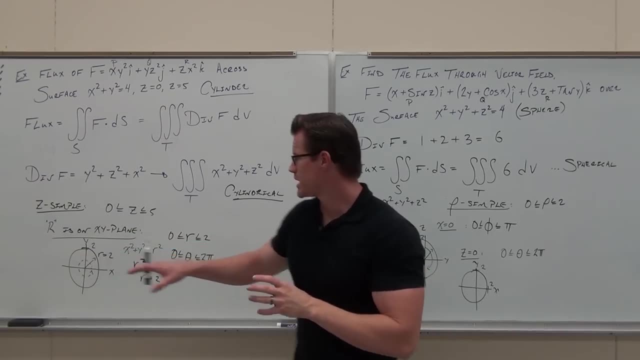 we're going to erase it. the d, sorry, the rho squared sine phi d rho d theta, whatever that was. We're going to have some special stuff here, So I want you to set up right now the bounds of integration and change this piece, please. 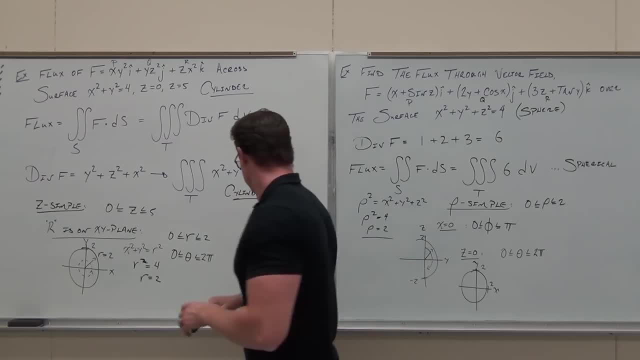 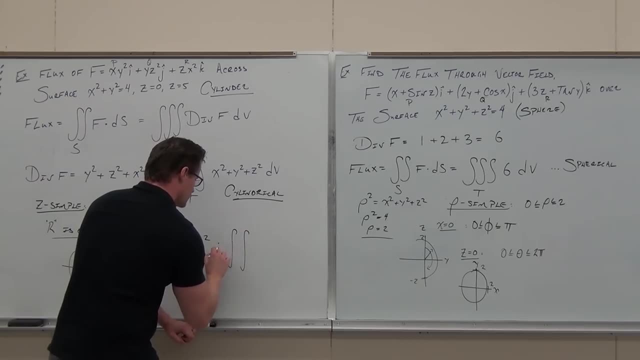 Okay, Well, we're going to do this. We're going to do this. We'll worry about this in a minute. With cylindrical, what goes first on the most inside integral, From where to where? Zero, Zero to the top. 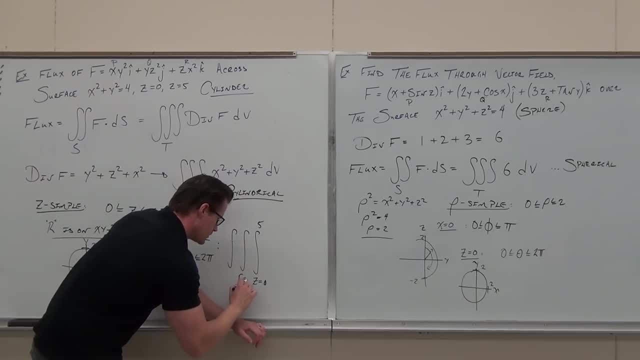 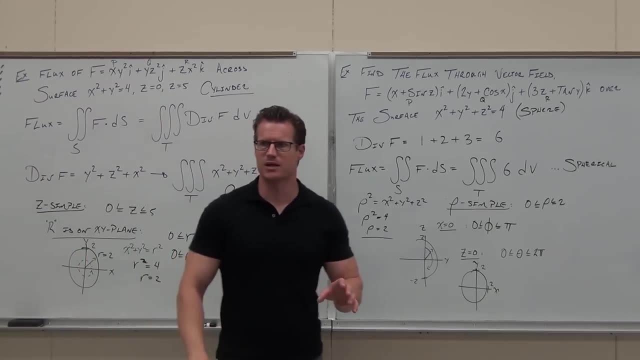 Beautiful. What's next Part of it? Part of it, Zero And, lastly, Fantastic. that's exactly right. That's exactly how you balance an integration. Look, show of hands. if you got it, Is it way easier now than like the first time we did it? 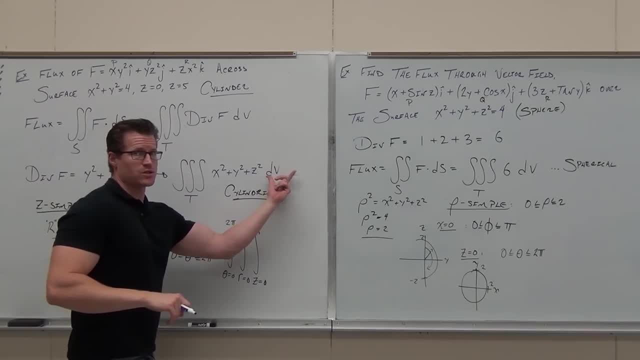 Crazy how that works. huh, Now the d. that's got to change. Come on, folks, let's get this right. You've got to match up your variables with the d of that variable and we also have something up there. 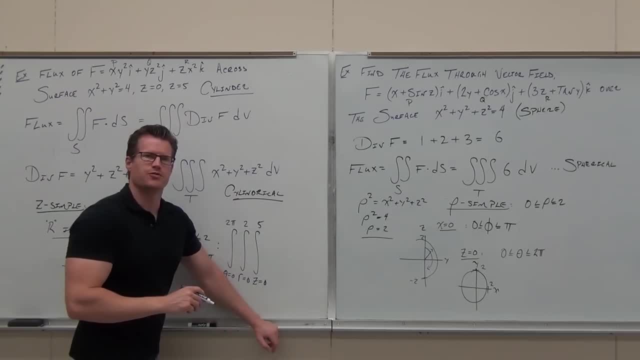 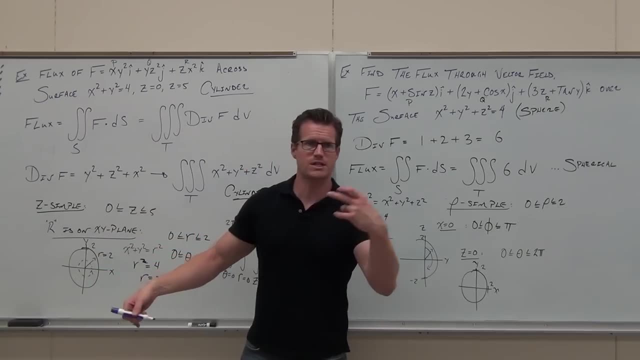 What's this going to be over here, Rd? Where's the r coming from? The r's coming, yeah, Jacobian, but r's coming from polar When we did the polar here. that's what, given that r dr. 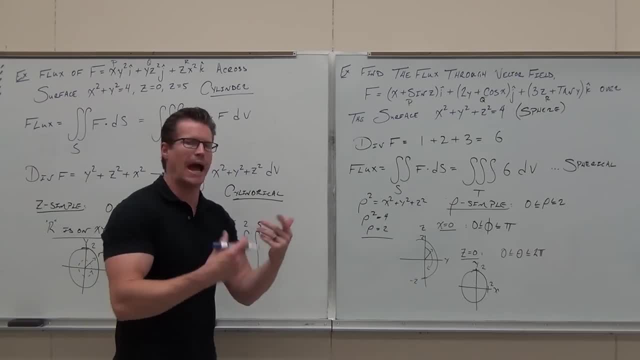 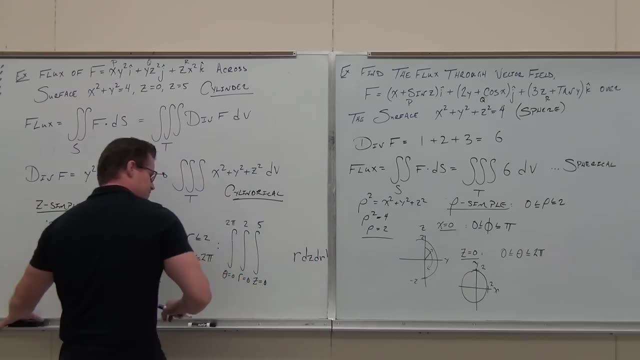 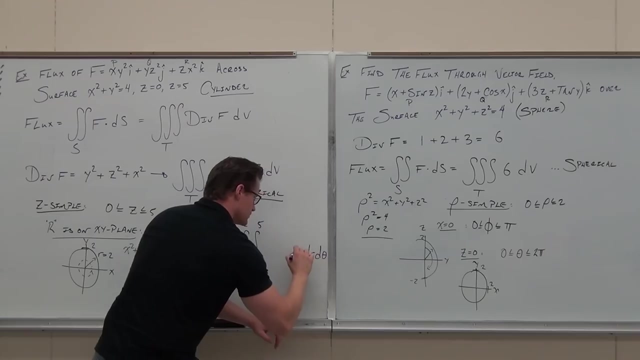 d theta. we just put the r in front of the dz so we don't lose it. you don't have to do that. But we have a r? dz dr ah shoot. We have a r? dz dr d theta. 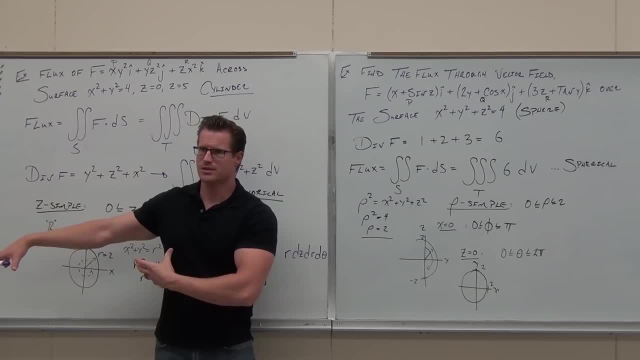 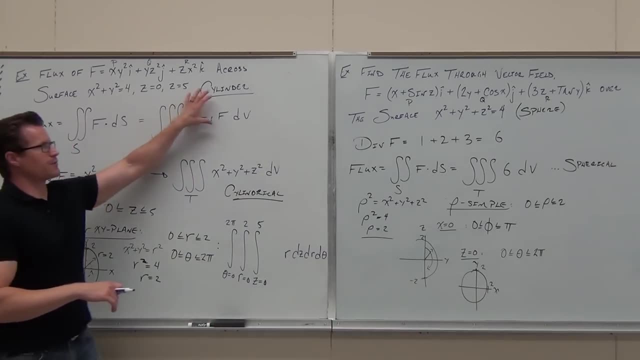 The r dr d theta is just the polar. that's what's happening. The cylindrical works, z first, then polar. that's about it. I don't know if you're okay with that one. Now. As soon as we determine, divergence, theorem works. 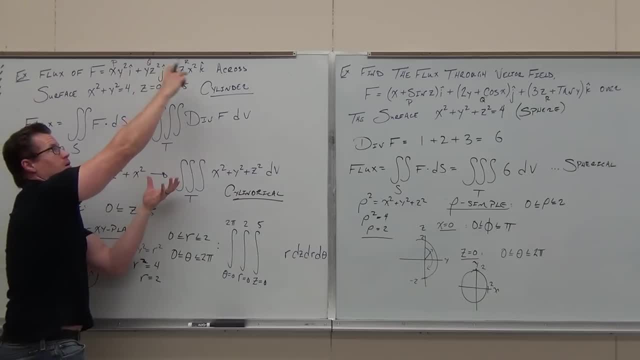 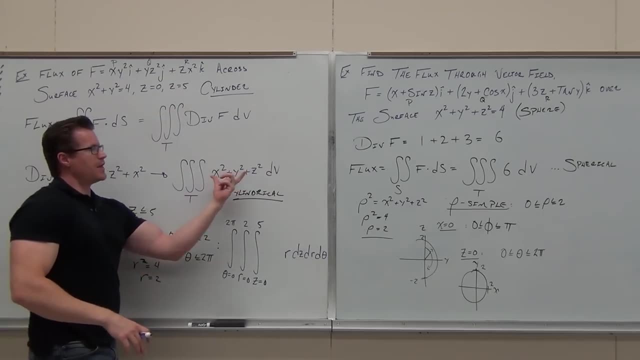 we find divergence, we put it here. we deal with the 3D region, that 3D simple closed surface, we identify it for a triple integral and then we change these pieces. But you have to keep in mind that these pieces only change. 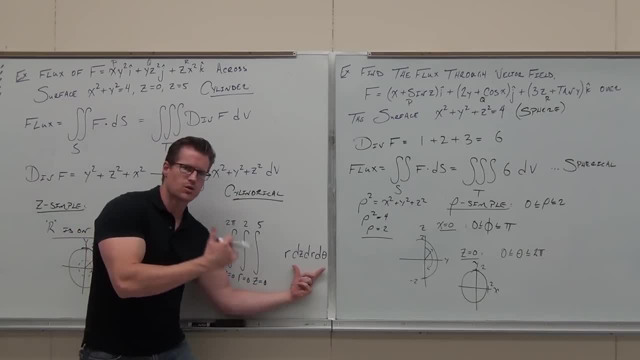 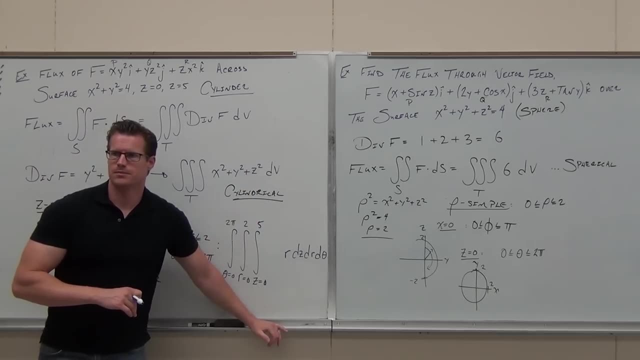 to match these variables. As long as you're matching those variables, you're good to go. So here's the question for you: Do you change this? Do you change the z here? No, No, No. It's real common for people who don't know what they're doing to go. 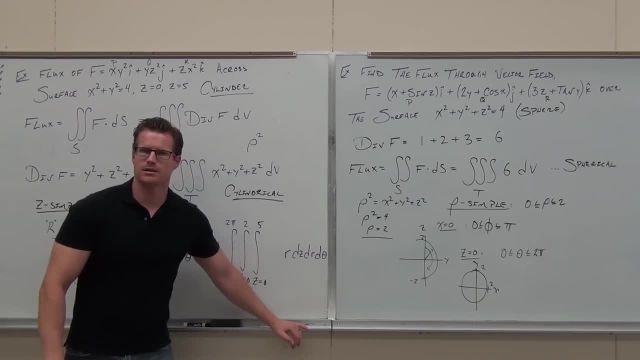 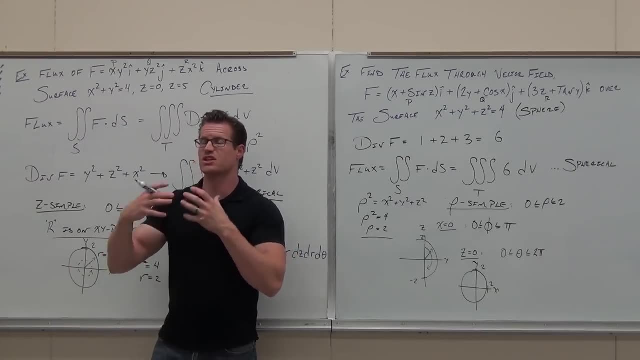 oh, that's row squared. yeah, I'm done. Would that be a good idea? No, Do you have any rows? No, That's hey, that shape, that's not spherical. Spherical doesn't work real well with cylindrical or cylinders. 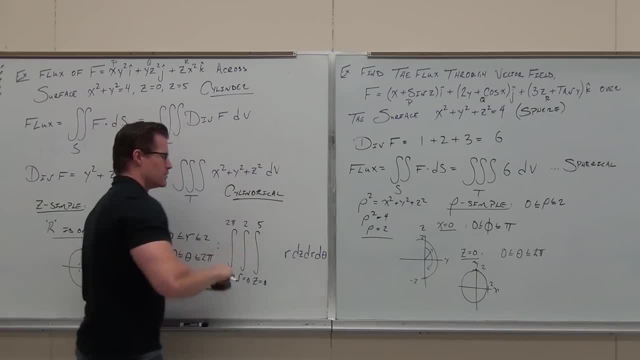 Cylindrical works real well with cylinders. Do I have to change the z at all? No, Should I change the z? No? No, In fact, that's the first variable that you're going to have to integrate with respect to, so don't change it. 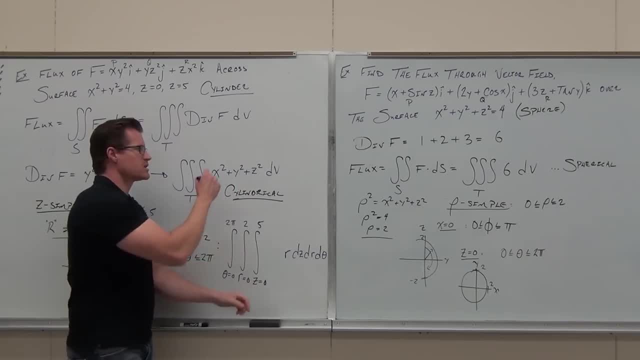 Do I have to change the x? Yes, Yes. Do I have to change the y? Yes, So change them both at the same time. What's that become? R is more or less By the polar definition that you just put right here. 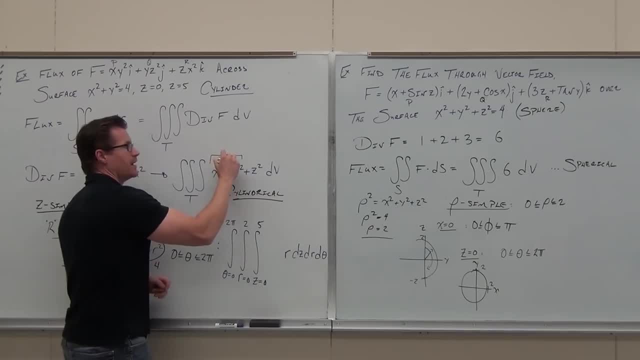 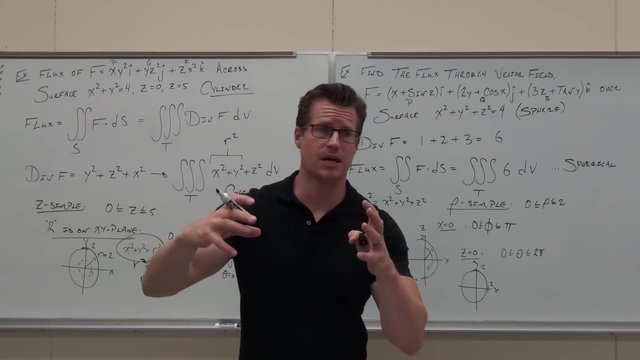 so why we put that stuff on paper, not just do it in our head? You already have that. You change this to r squared for your region. therefore you have to change it to r squared for your integrand What's inside of there. 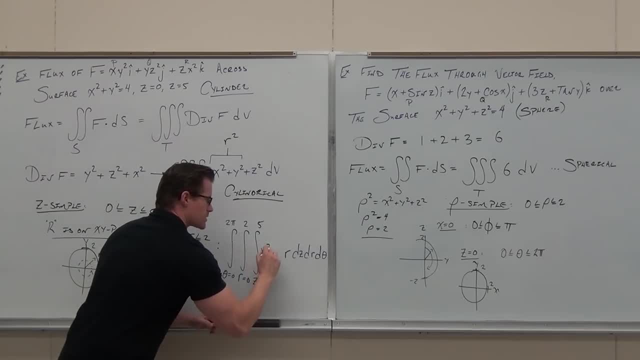 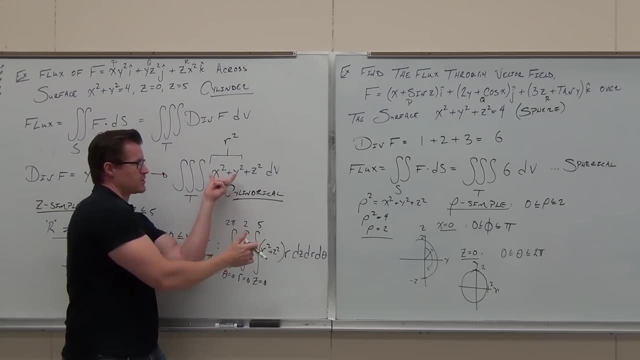 You've got to do that. So this becomes r squared plus z squared, and then we have that times r. Just keep in mind you have to have parentheses. Here's your r squared, here's your plus z squared. and you multiply the whole thing by r. 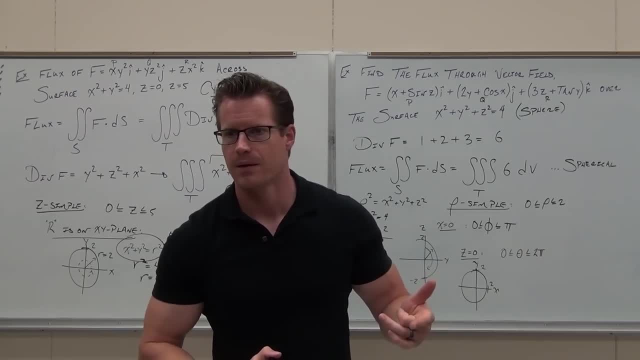 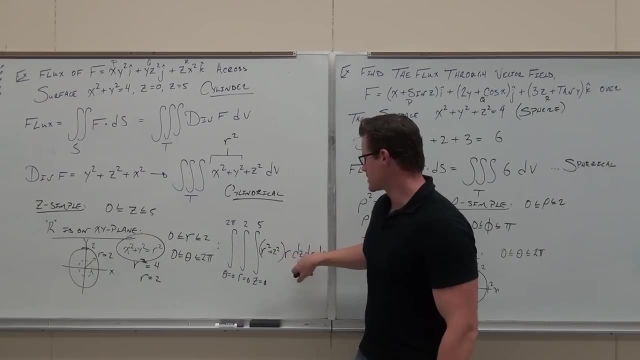 Does that make sense to you? I want you to start working with it. What's the first thing that you would do right now? Yeah, you distribute before you integrate here. So distribute the r. You technically don't have to. You could hold that out until later. 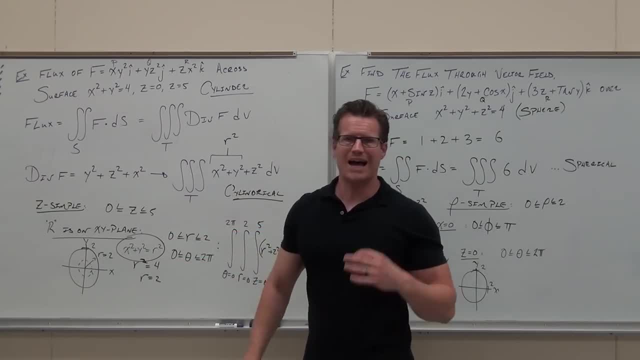 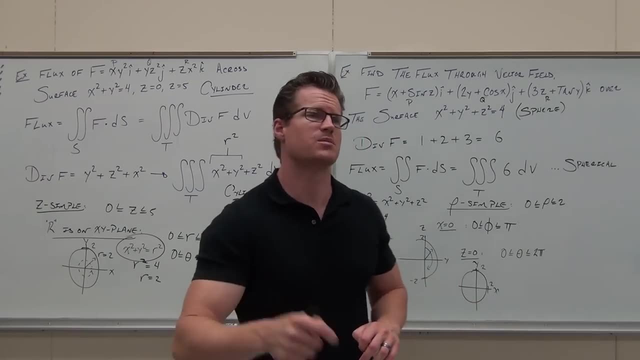 and then distribute the r later. It doesn't really matter, It's a constant with respect to z. I like to not lose it, so I like to distribute that one. So I want distribution here. I want you to work it through the dz plug in some numbers. 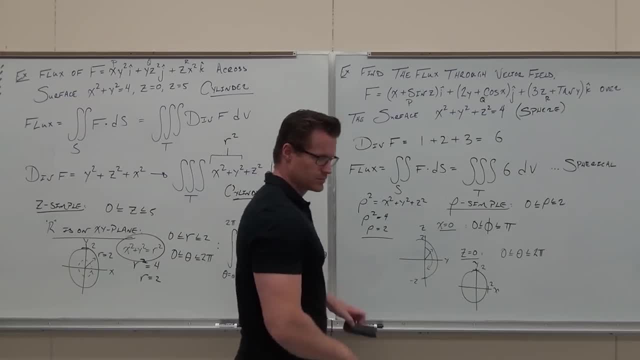 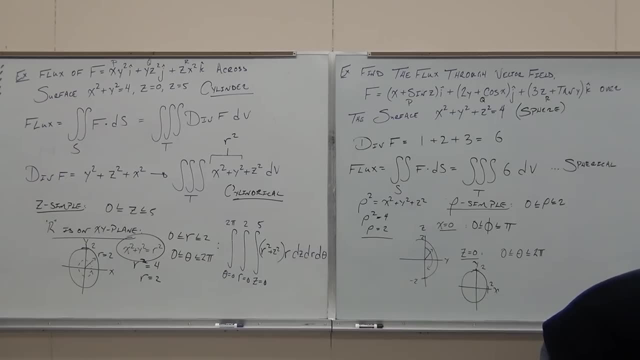 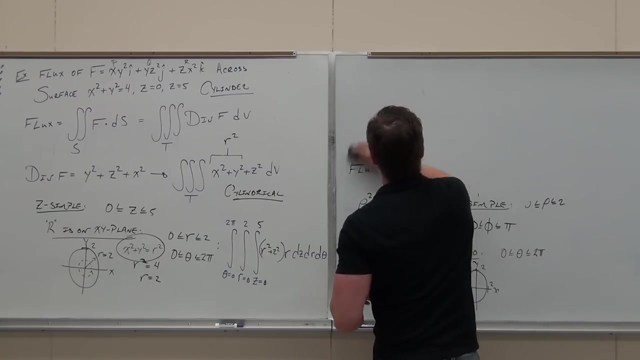 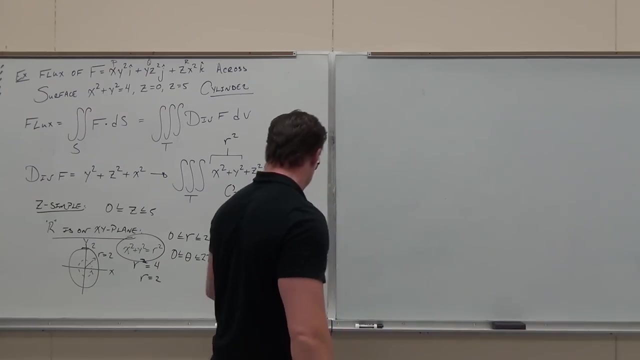 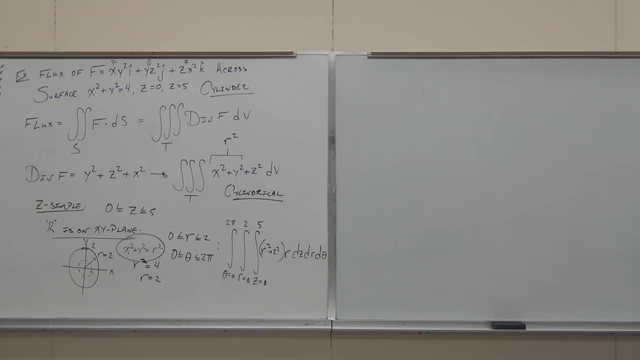 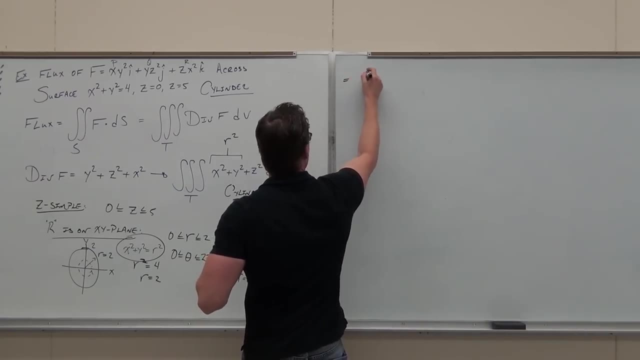 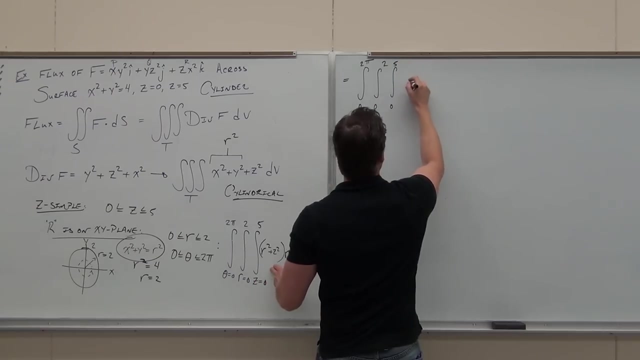 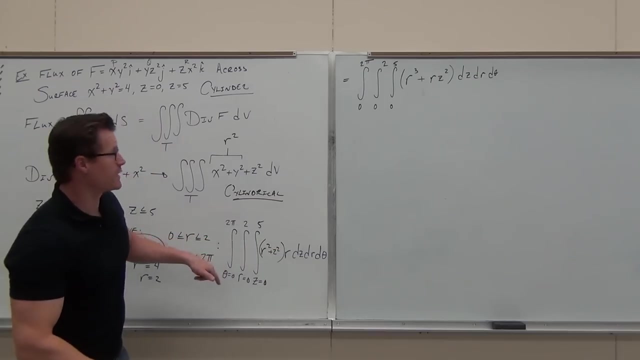 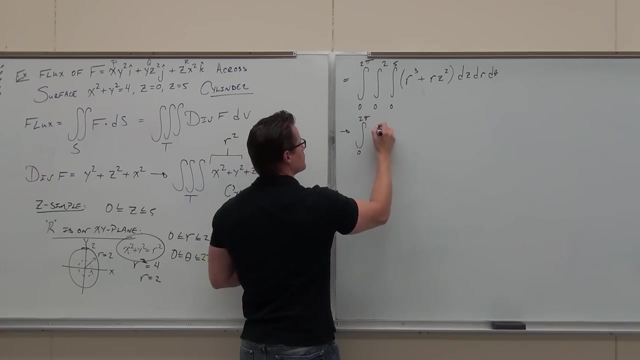 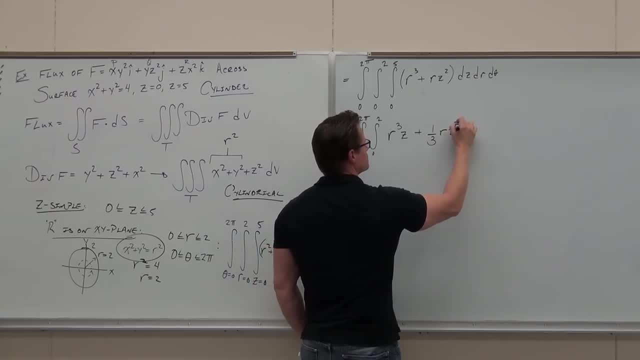 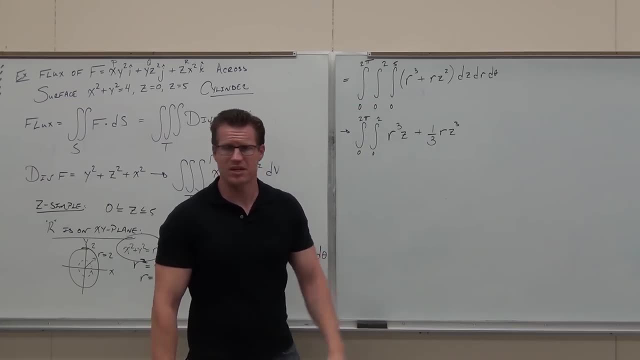 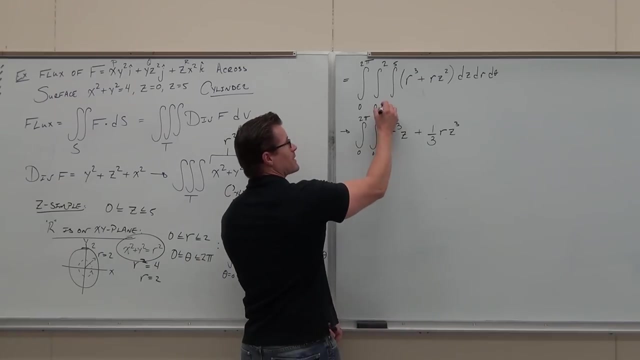 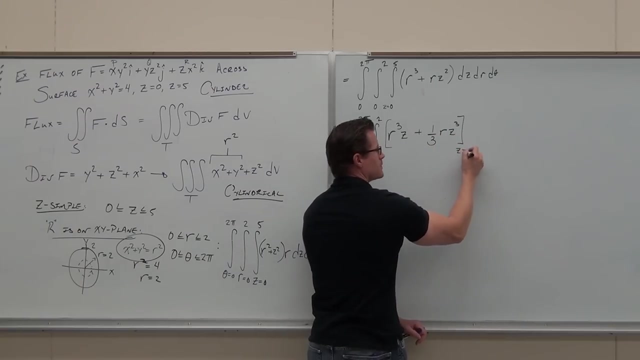 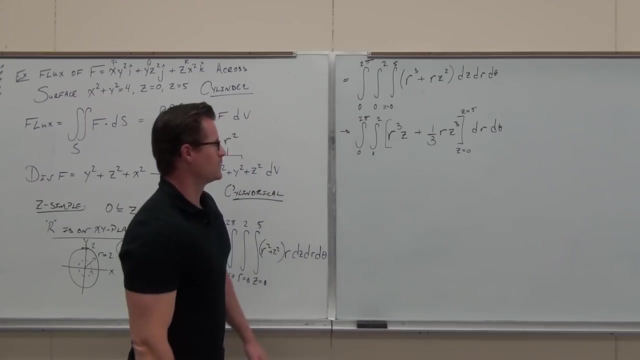 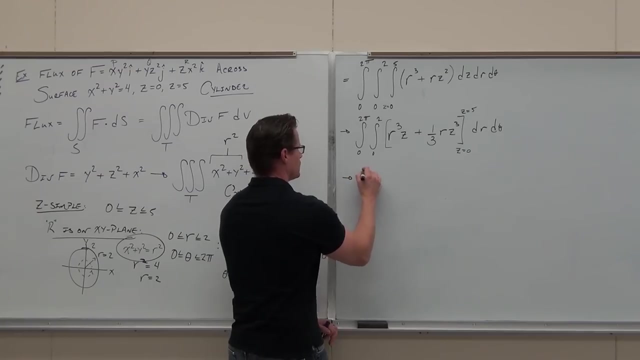 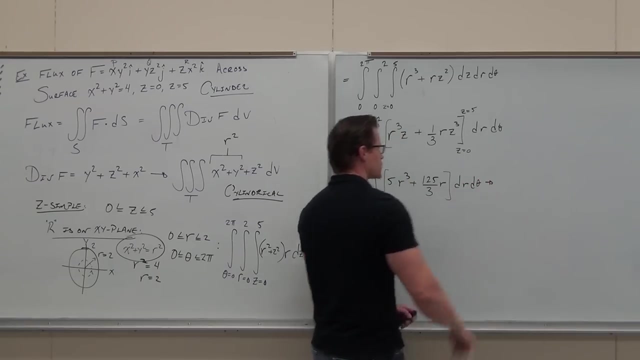 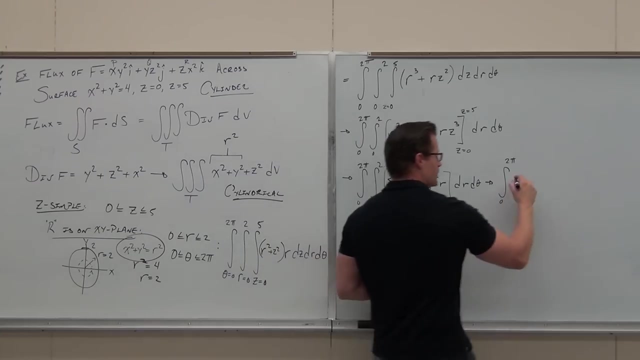 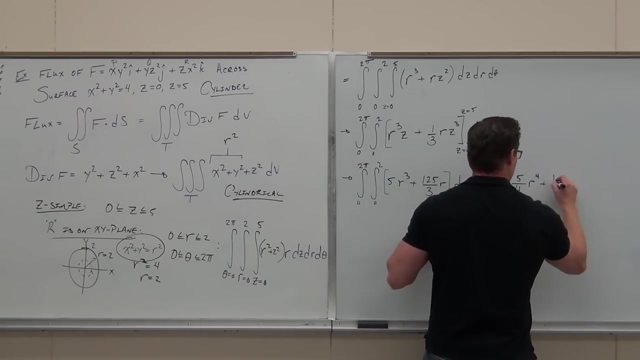 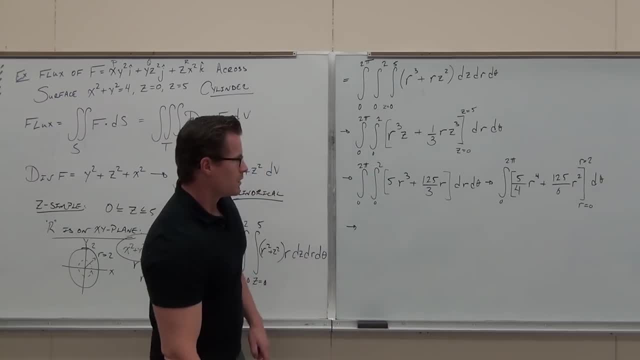 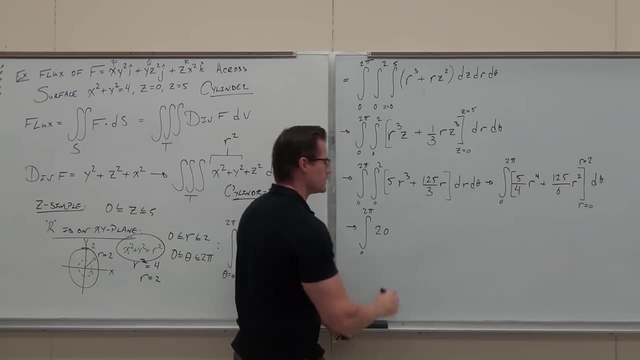 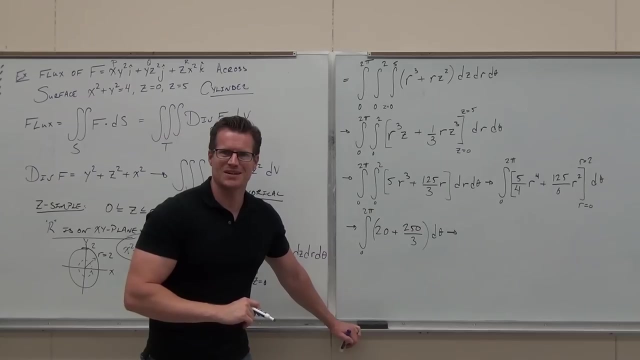 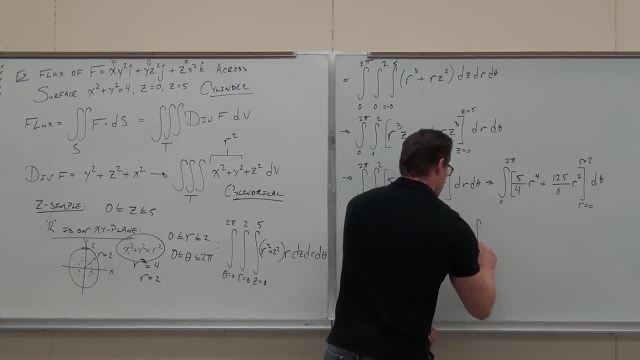 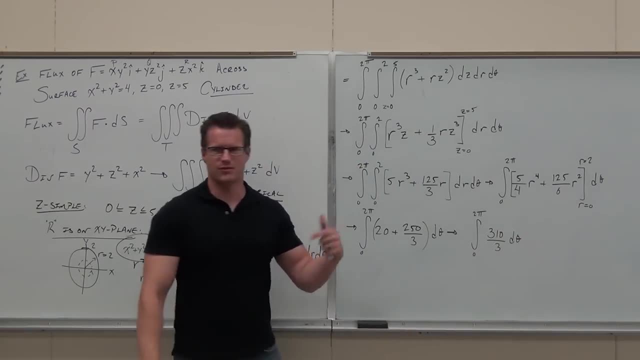 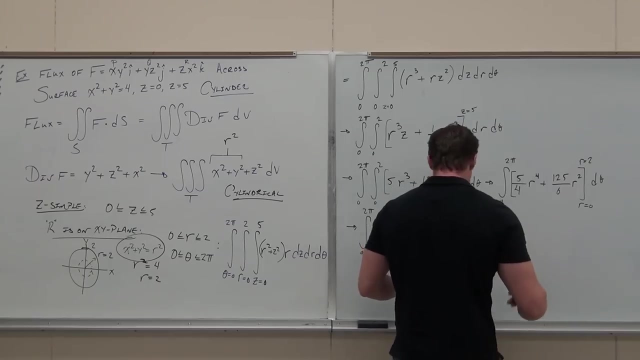 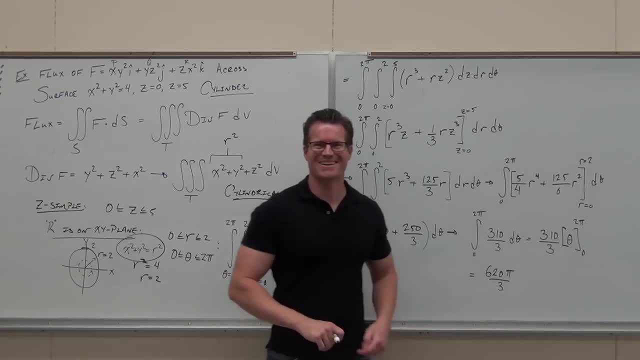 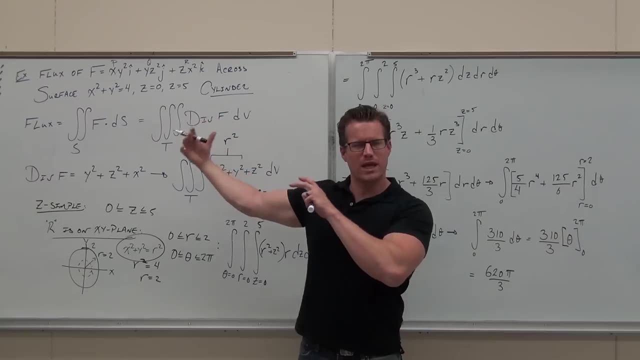 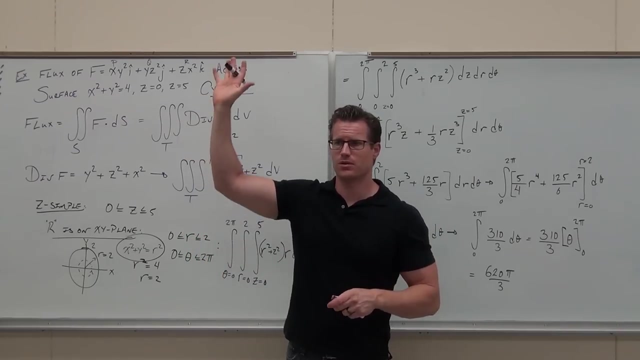 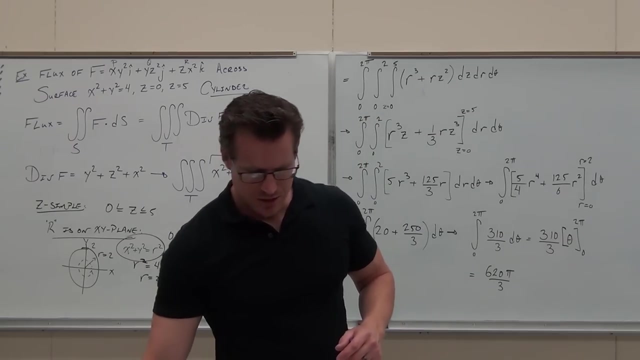 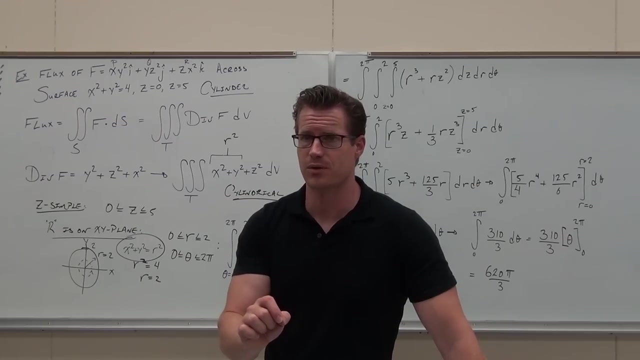 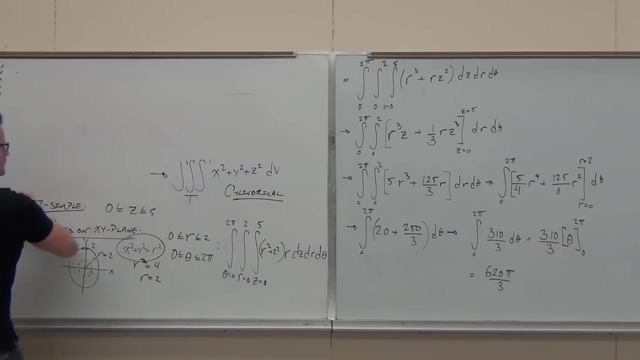 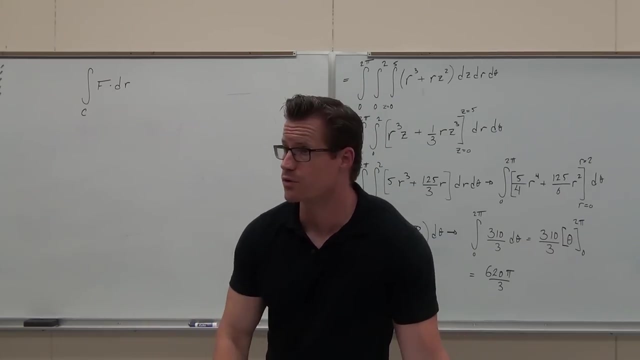 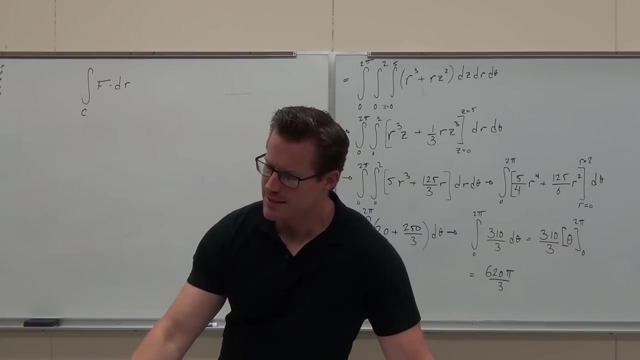 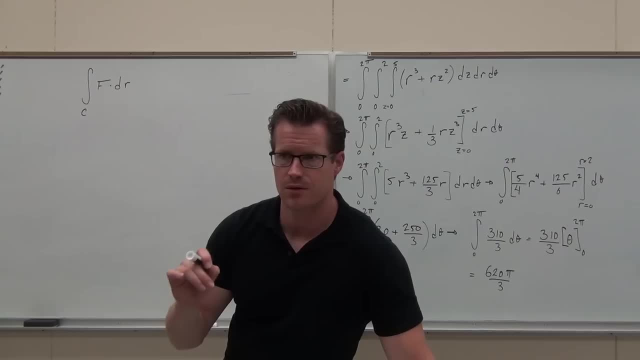 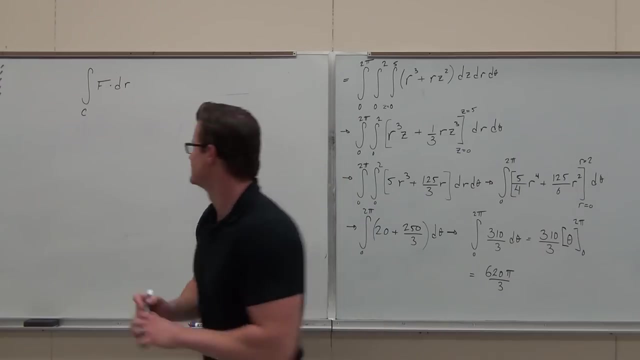 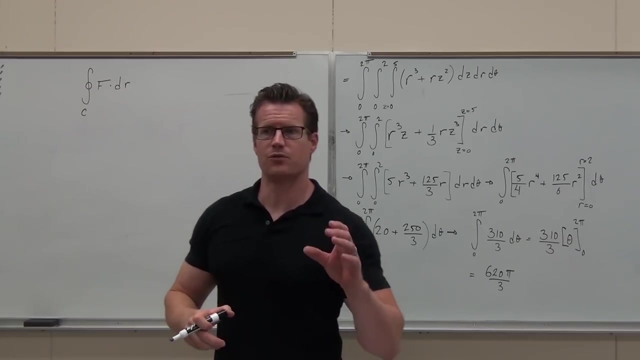 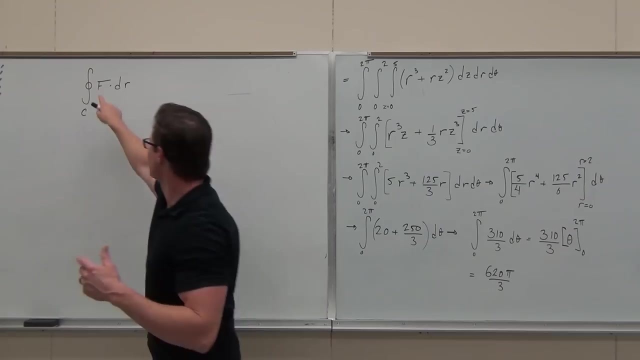 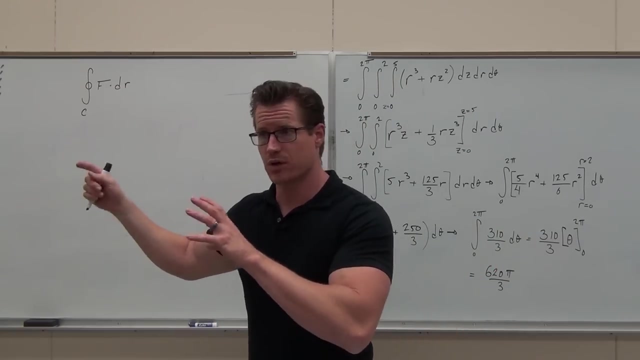 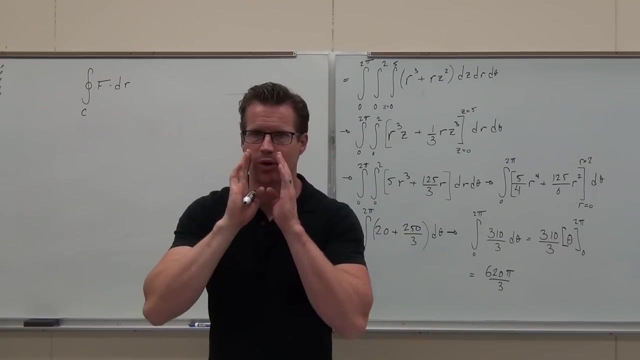 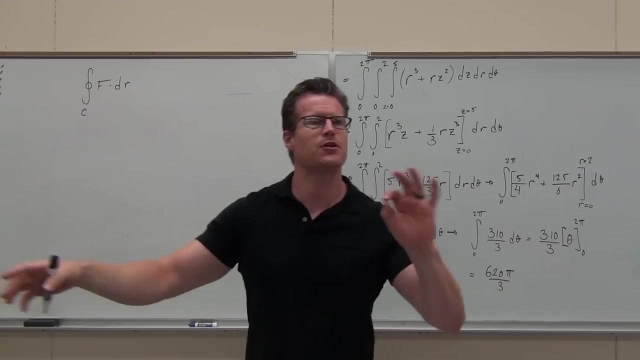 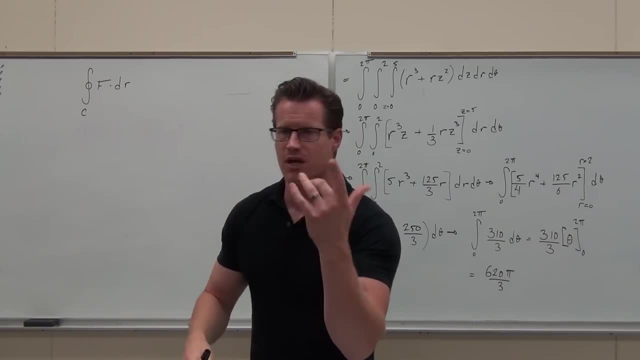 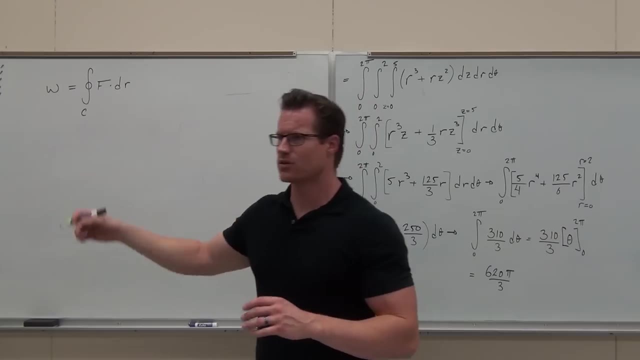 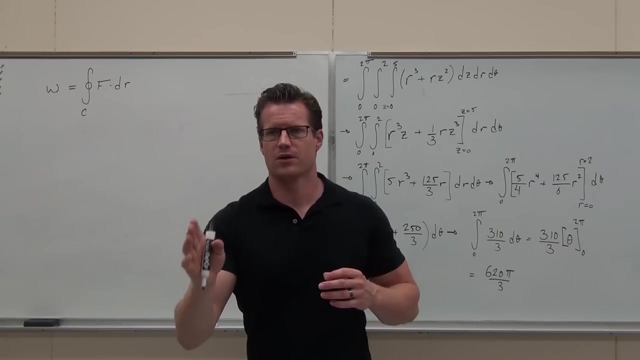 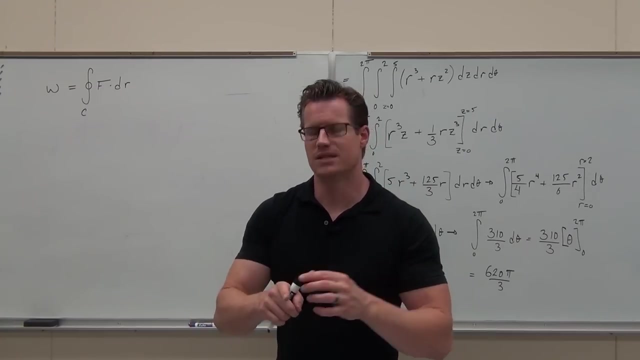 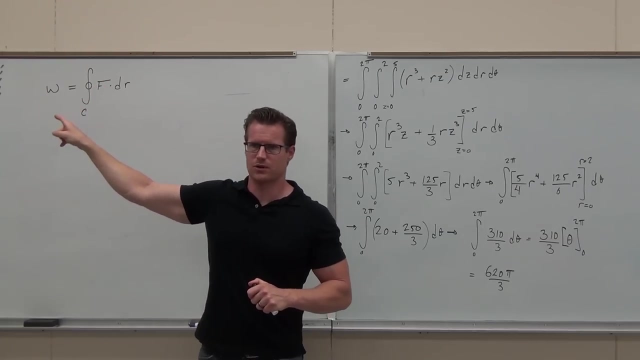 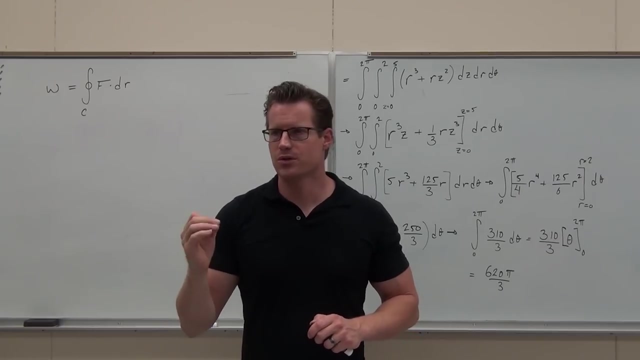 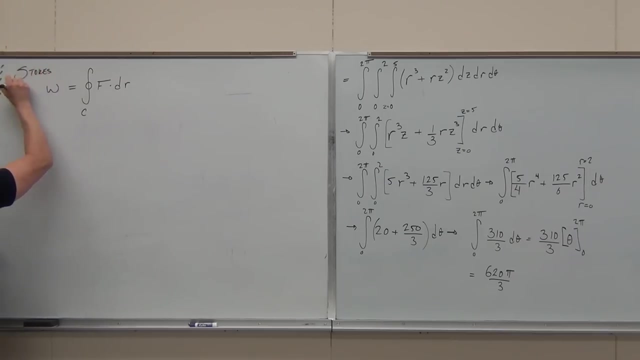 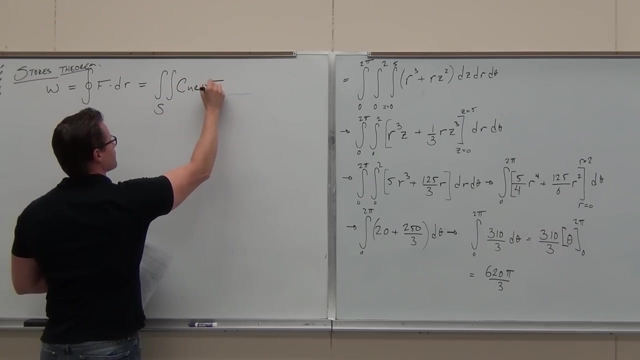 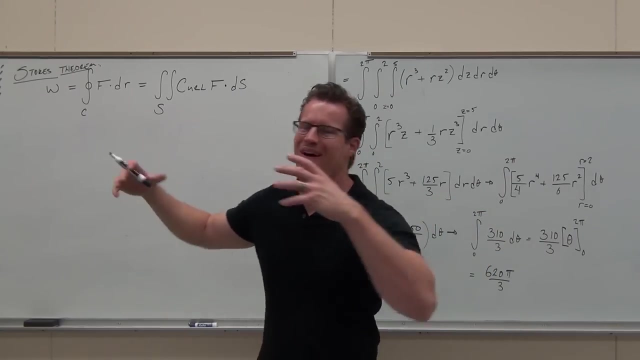 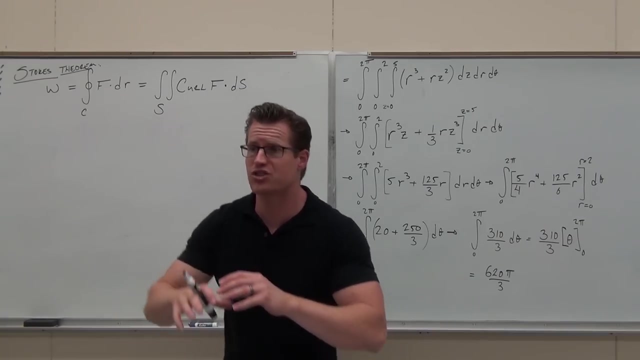 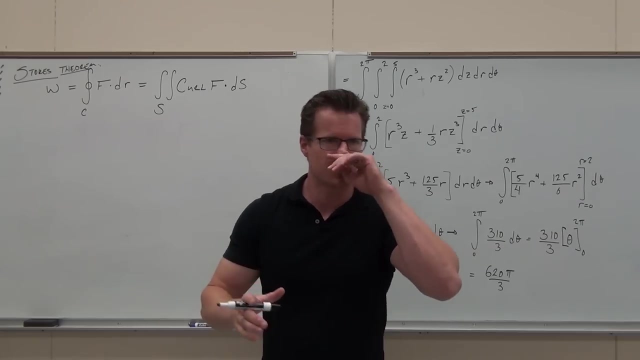 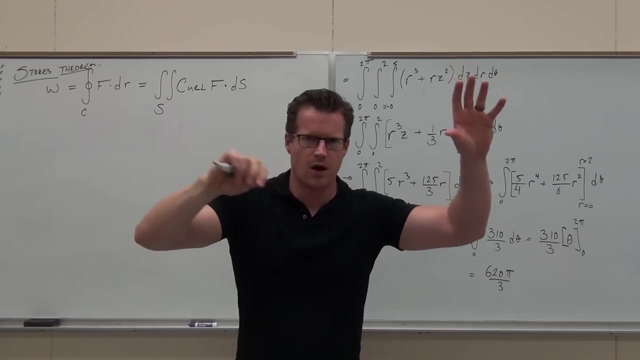 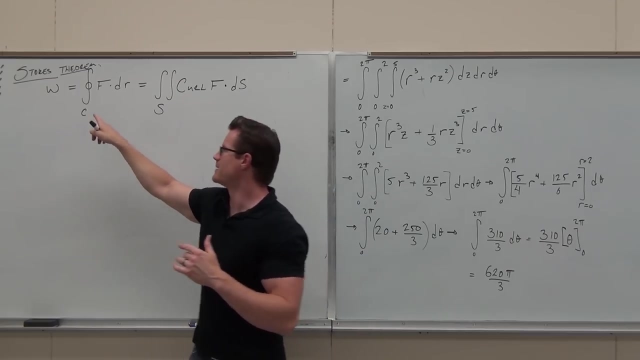 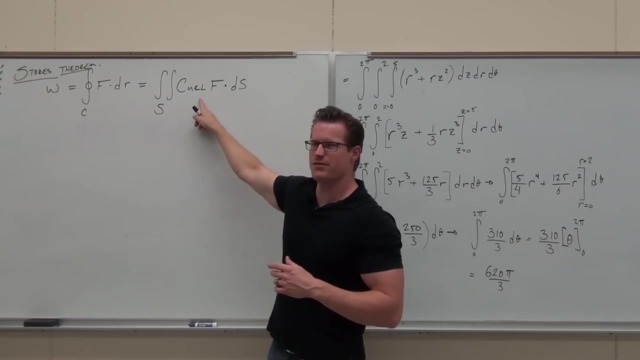 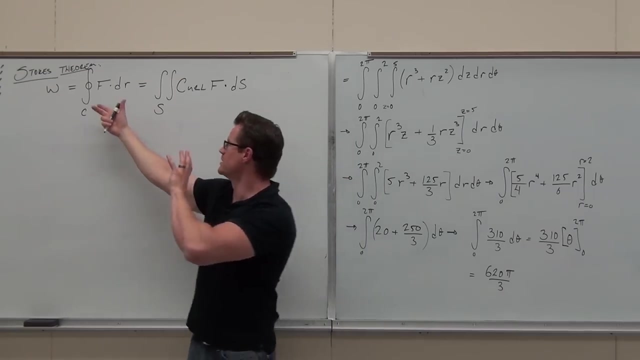 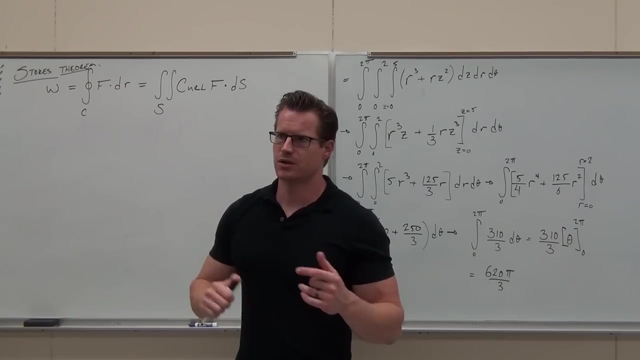 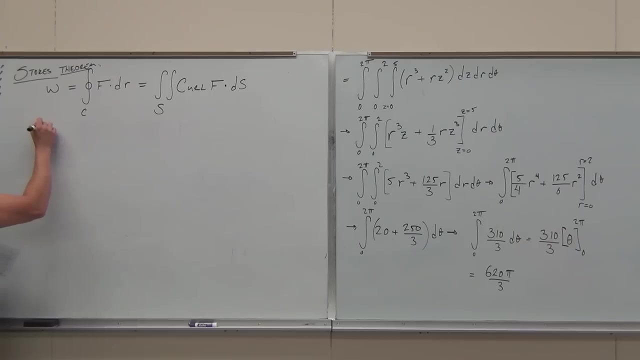 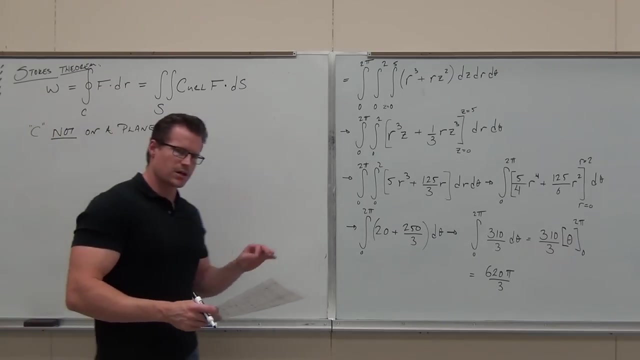 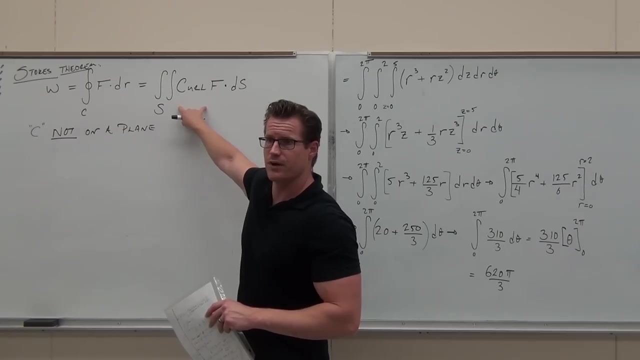 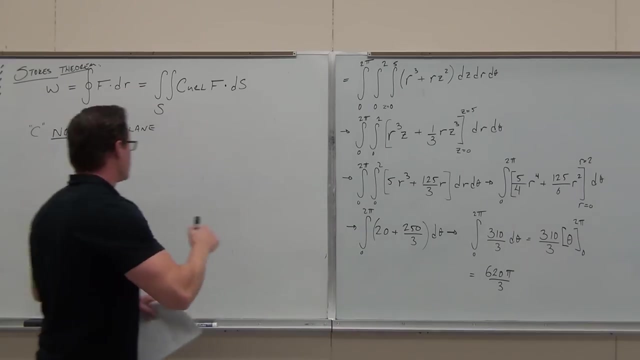 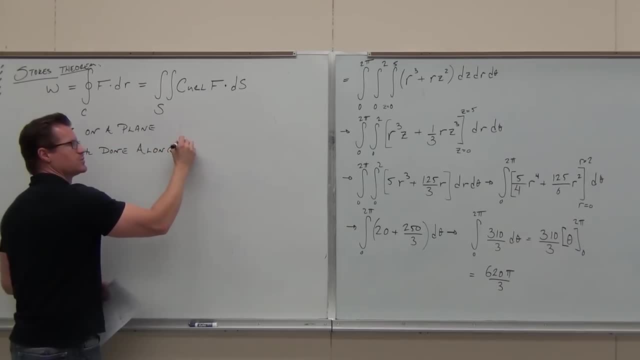 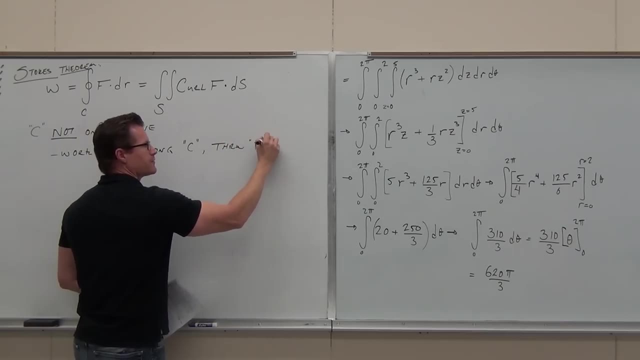 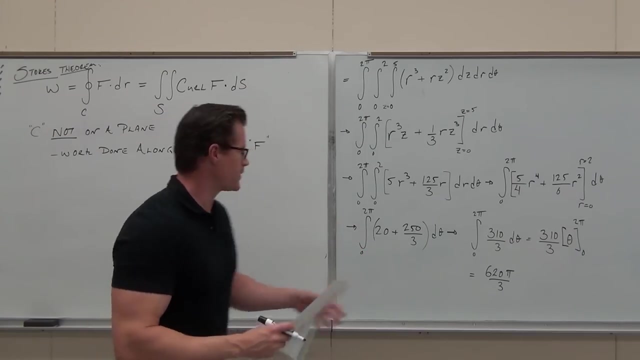 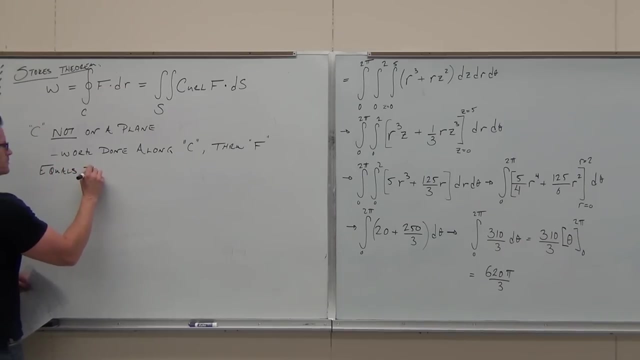 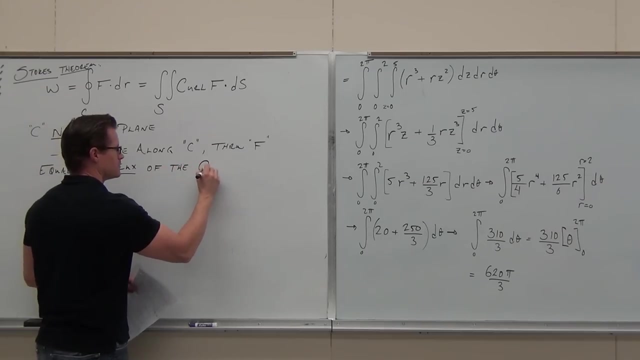 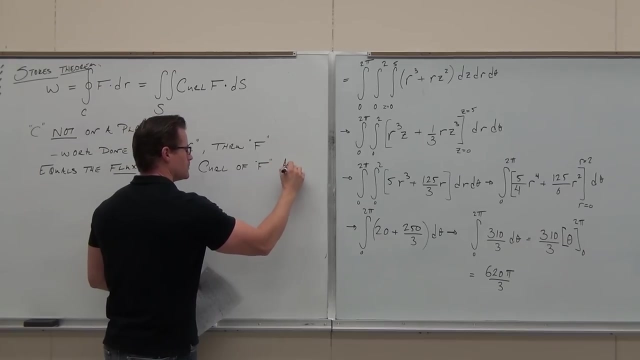 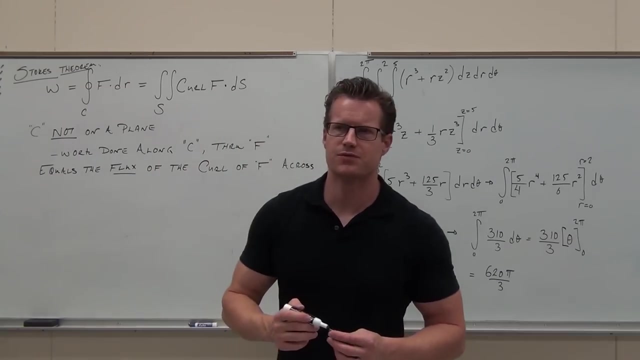 We're done along our simple, close curve C through the vector field. F equals the flux of the curl of our vector field Across, across, across what. Let's unpack this for just a minute before we do our very last example, and then we'll be good to go. 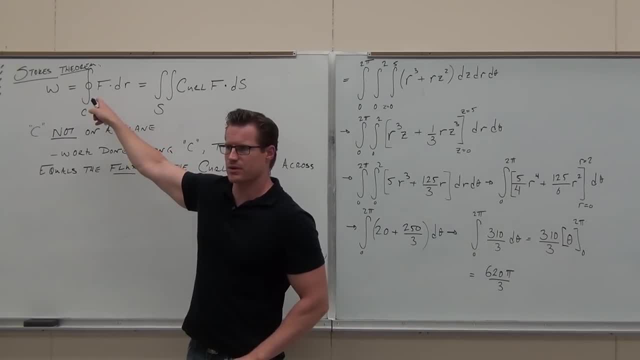 Let's unpack this for a second. Do you guys understand the idea that we're back to line integrals and still calculating work through a vector field along a simple closed curve? just not on a plane anymore. so it's 3D. So what is equal? 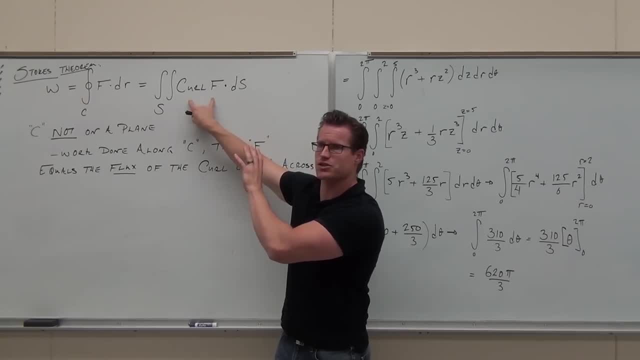 It's equal to a surface integral of a vector field. Is that a vector field? Yes, it certainly is. I'm going to show you how to deal with that in a second. This is the flux: Surface integrals of vector fields. is the flux that says that the work done? 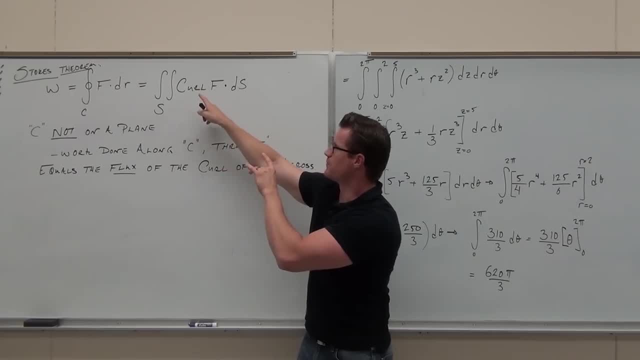 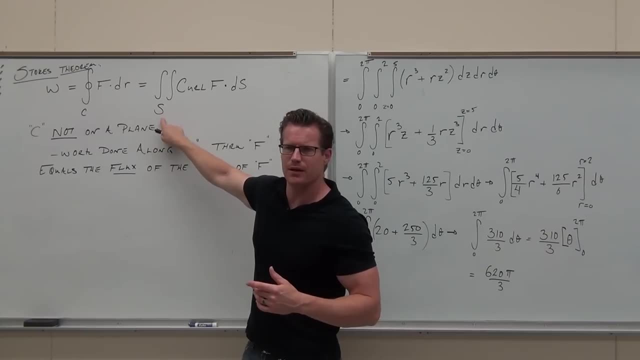 on that line. integral is equal to the flux of the curl of F. Oh, but wait a minute. Over what? What, Over what? What is that thing? Surface, What's surface, What's surface? I don't have a surface. 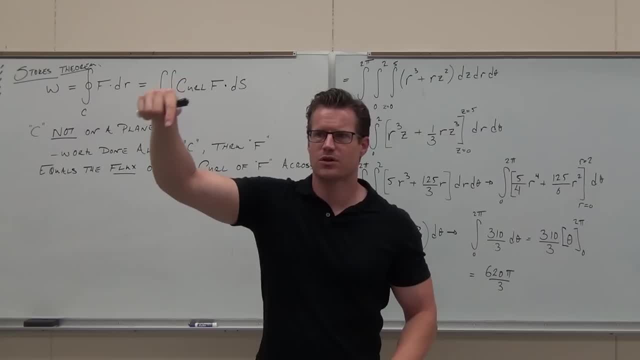 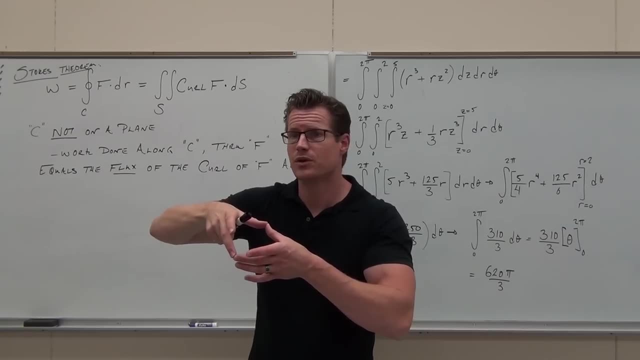 I've got a. I've got this curve. I've got this curve. Is that curve connected? No, Is that curve a simple closed curve that makes like a loop? Is that curve a simple closed curve that makes like a loop? Yeah, yeah, yeah. 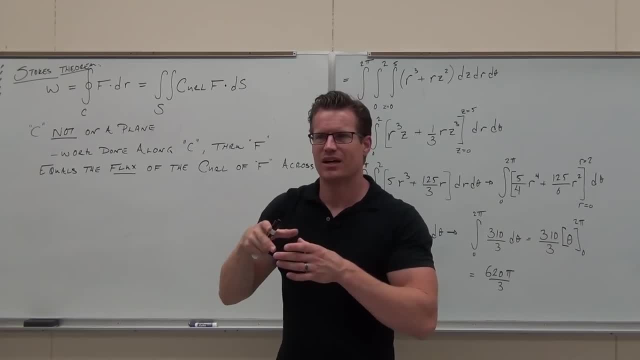 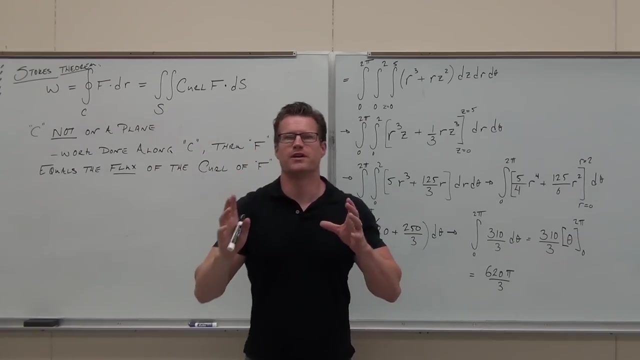 Okay, Like Green's theorem, remember that. Do you remember how Green's theorem you remember? You remember? Remember how Green's theorem dealt with the region, the region that that curve encompassed. Do you remember that This deals with the surface, that that simple, closed curve bounds? 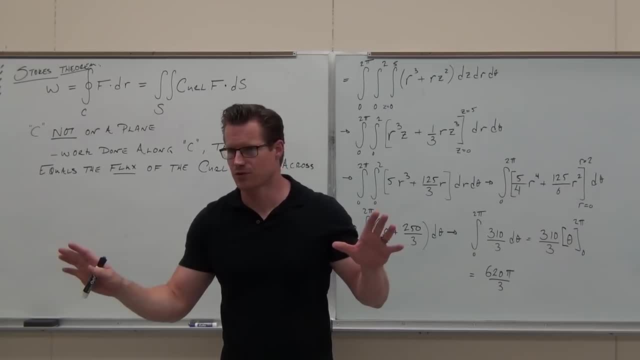 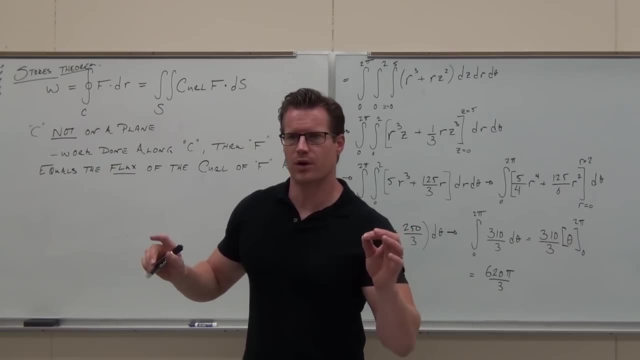 Not only that, it deals with any surface. where this curve is, the boundary Stokes theorem is. the boundary Stokes theorem is very impressive. Do you remember that whole independent path thing where you're like: hey, you can go along any curve, it gives you the same work done. 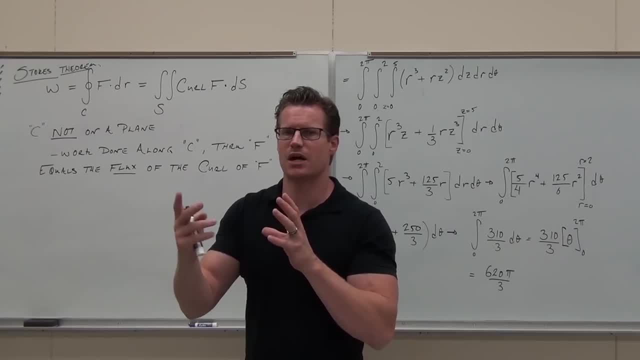 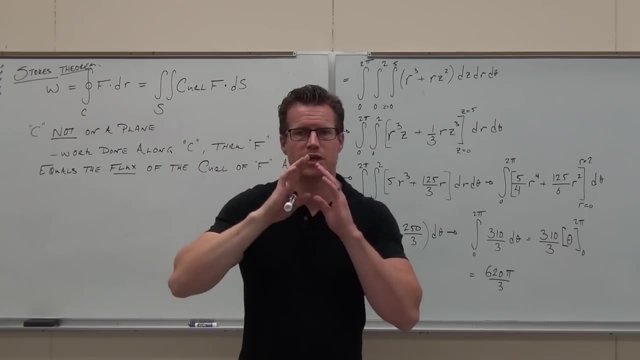 Do you remember that Through conservative vector fields? This is similar. It's not the same thing, but it's similar. It says that as long as this curve is a simple closed curve in 3D, you can do a flux integral. 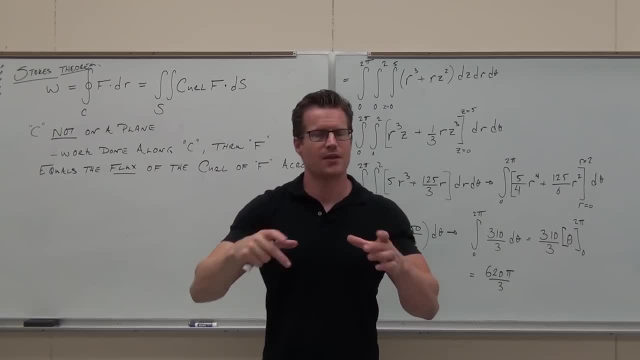 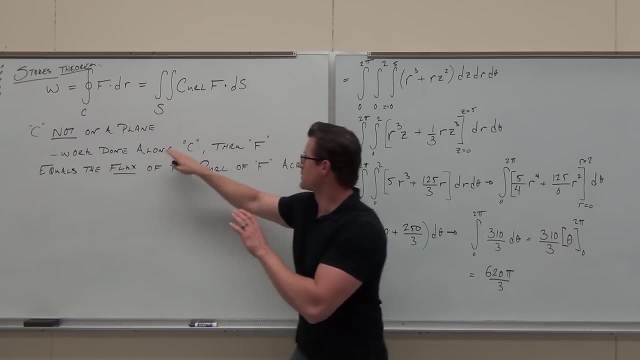 a surface integral of a vector field for any surface that has that curve as its boundary and it will calculate the correct flux for you. So this: this says That the work done along C, C through F, F equals the flux surface integral of the curl of F. 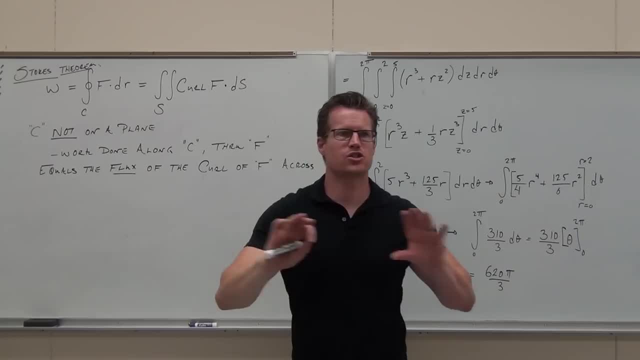 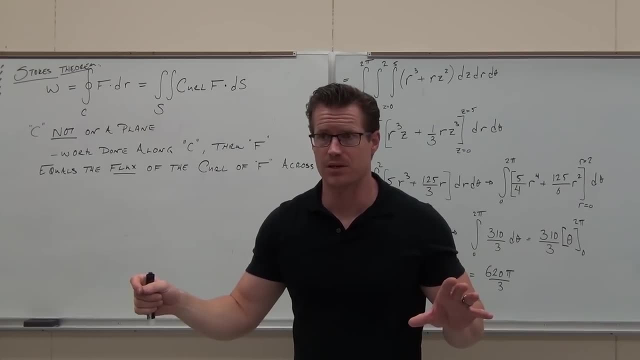 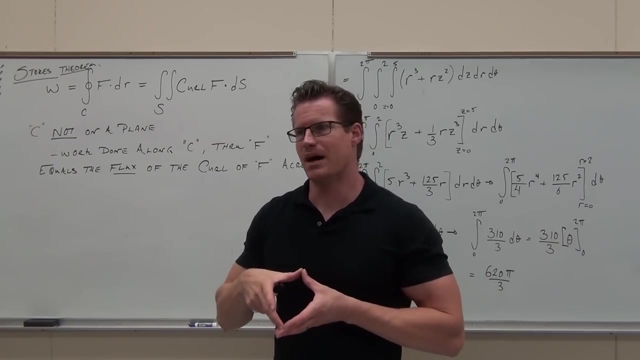 it's still a vector field across any surface where C is the boundary of that surface. That's freaking cool. Does that mean we need a surface? Yes, Does it mean that any surface will do? Yeah, As long as C is the boundary. that's what's important. 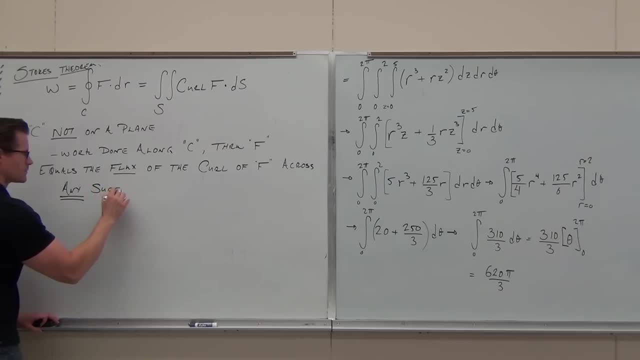 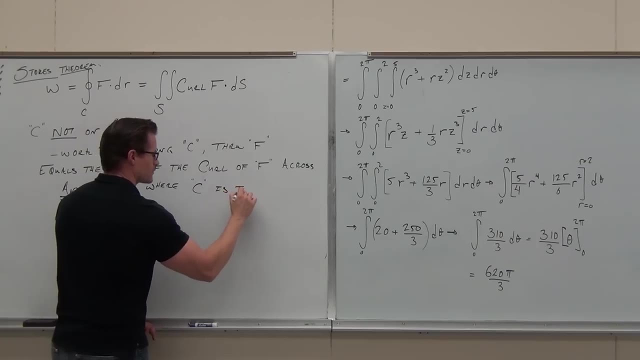 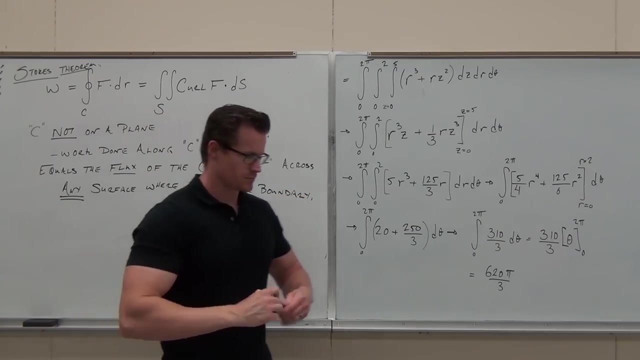 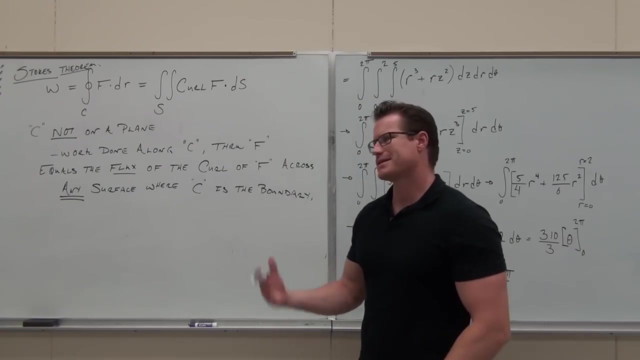 Okay, All right, I'm getting one more question. I have a question about the. Now, I made a statement a while back. It said that like maybe five minutes ago. as we were going through it, I said: wait a minute. 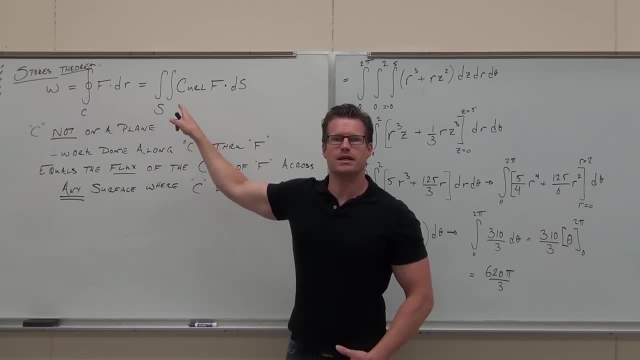 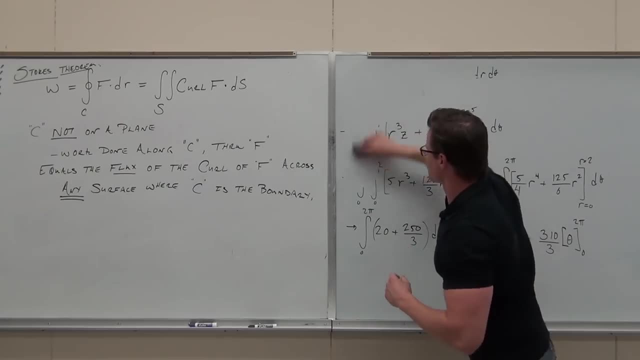 If that's a flux integral and that's a vector field, then it's old stuff. It is old stuff. Here's the idea, and it's a beautiful idea. It says: well, wait a second, If we do the curl of F, verify that the curl of F comes from our vector field. 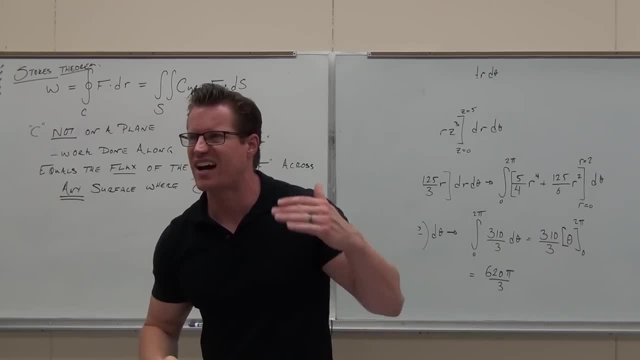 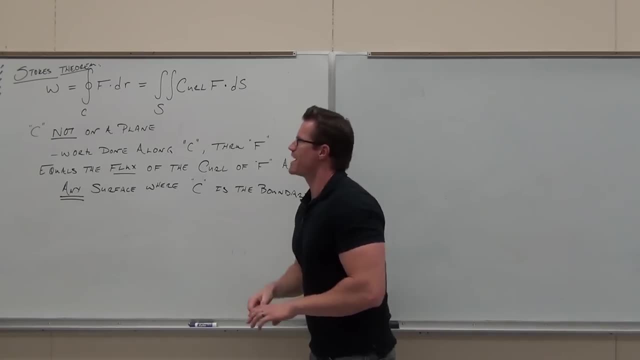 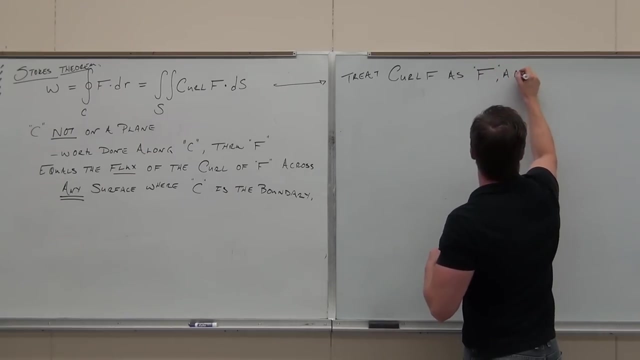 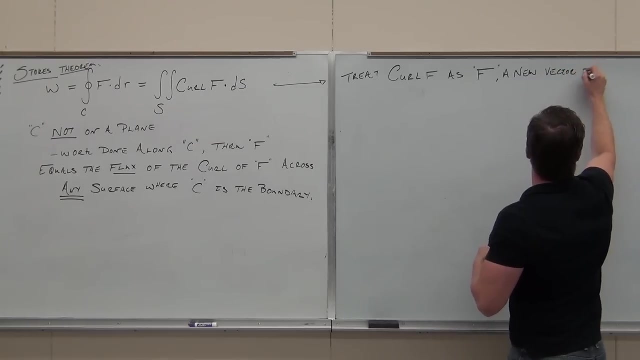 and still gives you a vector. Remember that curl F still gives you a vector, has I's, J's and K's. Then if we do just a little mathematical maneuver, treat curl F as F, as a vector field, Then this thing: 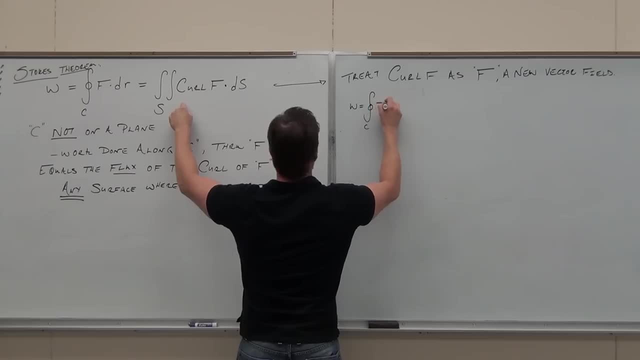 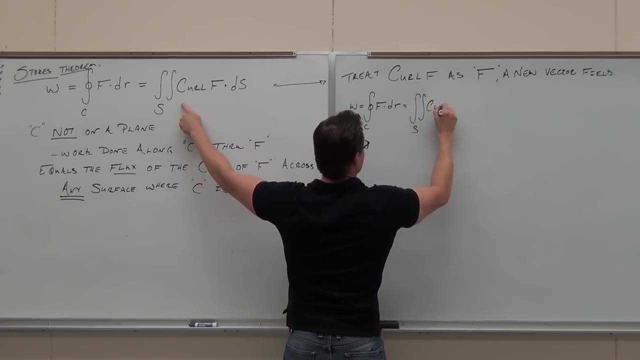 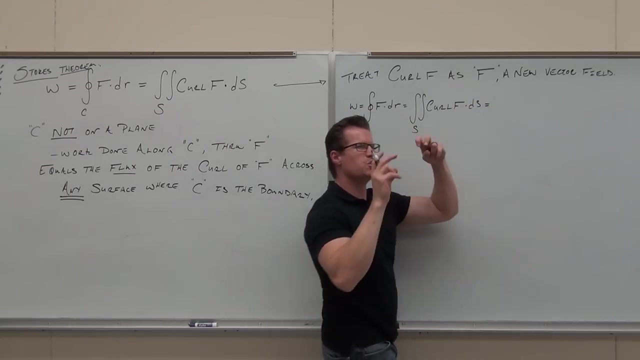 If I treat that as this new sort of vector field, I'm going to put these little quotations around. so you see it's a different F, It's a new F. I know I'm using the same letter, but it's a new F. 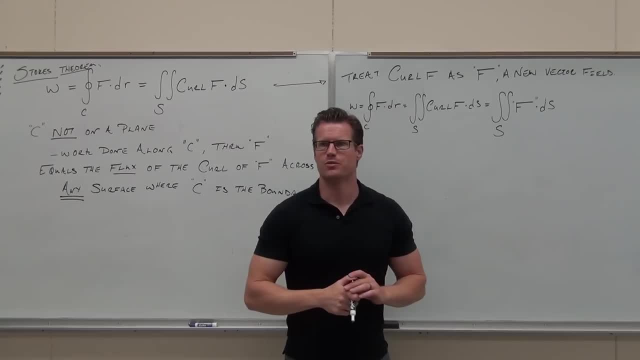 Well, that looks pretty darn familiar, doesn't it? In fact, that's exactly what we had last, just the last- I don't know- hour and a half of this lesson. Tell me two ways that we can deal with this right now. 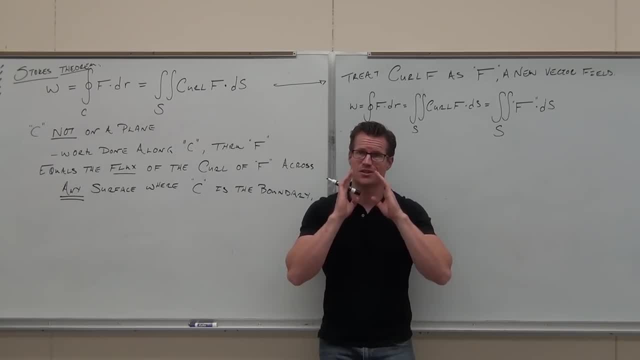 What if S is a simple closed surface? What could I do right now? Divergence theorem. Divergence theorem could apply to this. If you have S being a simple closed surface, If you can define it like that, then we have a simple closed surface. 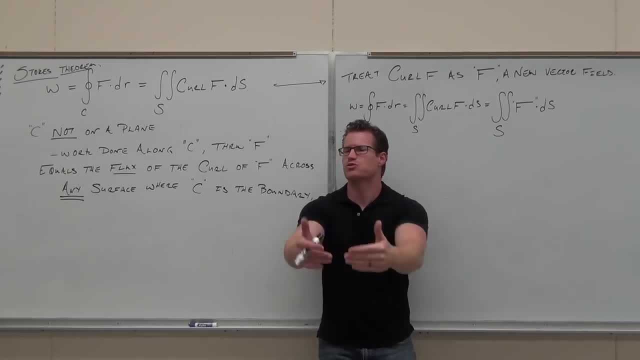 You could use divergence theorem. What if it's not? Could we do it? Yes, that was right before that. when we did flux integrals in general, We said: well, this could also be, so. this could be divergence theorem if S is a simple closed surface surface. 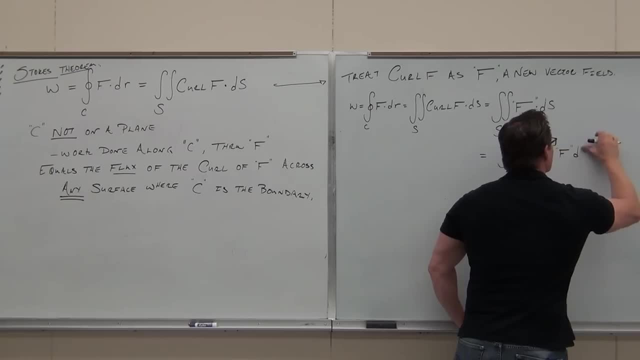 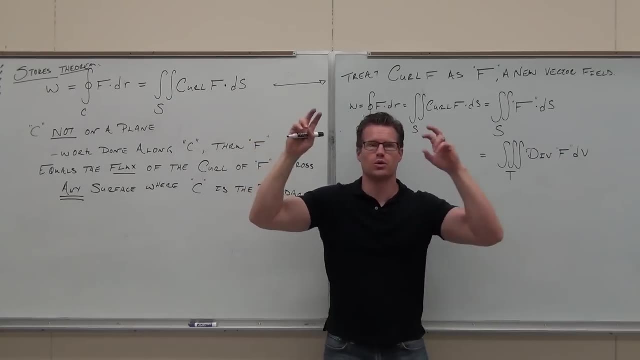 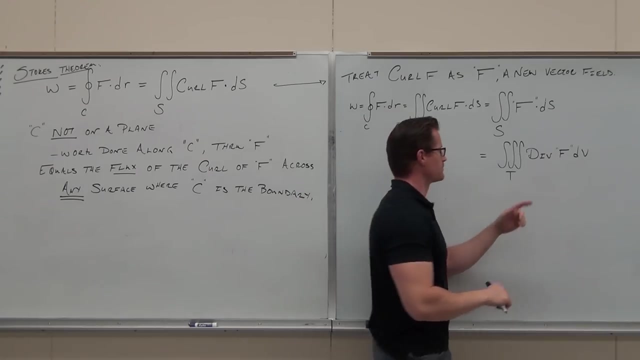 This gets a little tricky, though, sorry, Because this F, where you'd find the divergence, is not that F, It's the curl of that F. Does that make sense? So you do a, you do that the curl, then divergence. if you have that simple, closed surface. 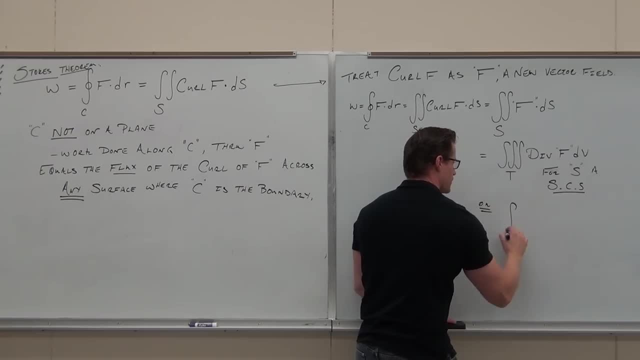 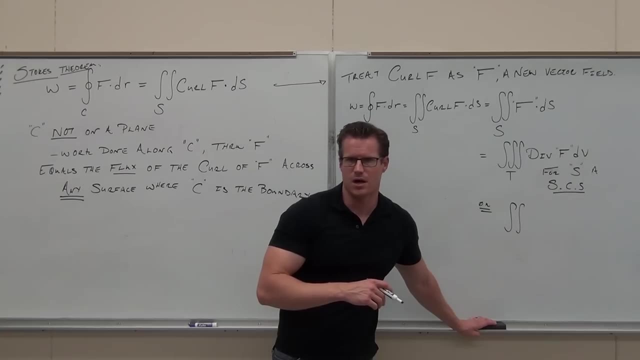 Simple closed surface. Or we go back to this: Let's suppose that S is not a simple closed surface, which in general it's not. It's just a simple closed surface, It's just something where- and it's it'd be very unique to have this, because can you? 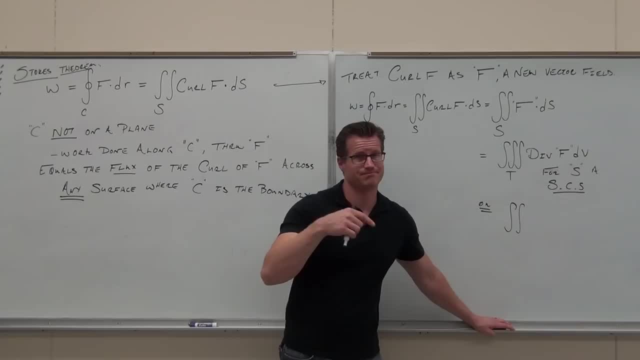 really talk about a curve being a boundary of a simple closed surface. It doesn't really have a boundary. It'd be very unique if we had that. Generally it doesn't happen. I'm just saying in generalities that you make connections here. 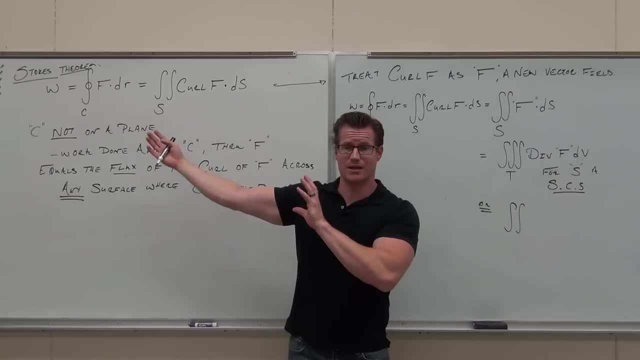 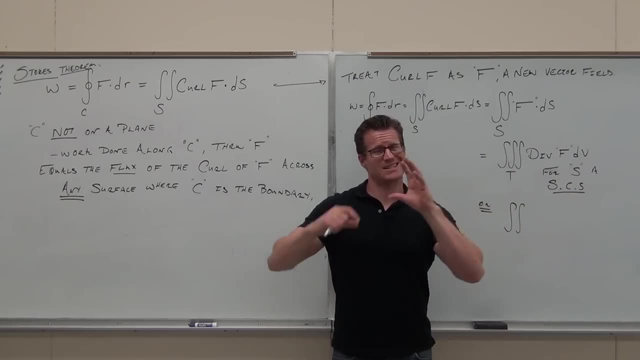 Okay, the connections are: we are getting a surface integral out of a line integral. That's pretty impressive. How do we deal with them? One way we deal with surface integrals is divergence theorem. That's one way. But if it's a simple closed surface, then C boundary kind of falls apart a little bit. 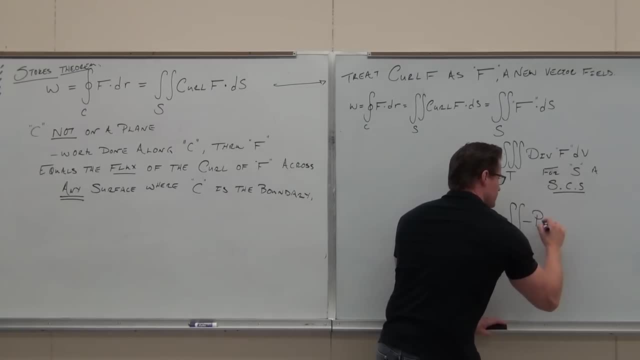 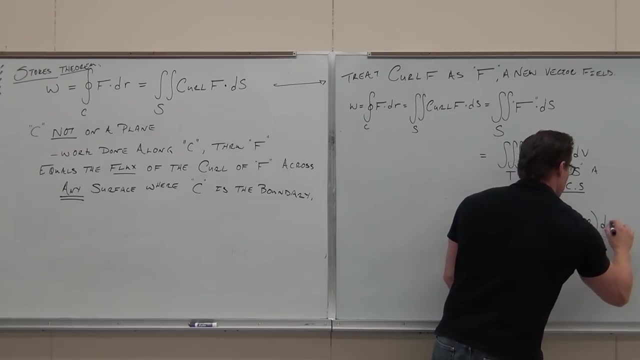 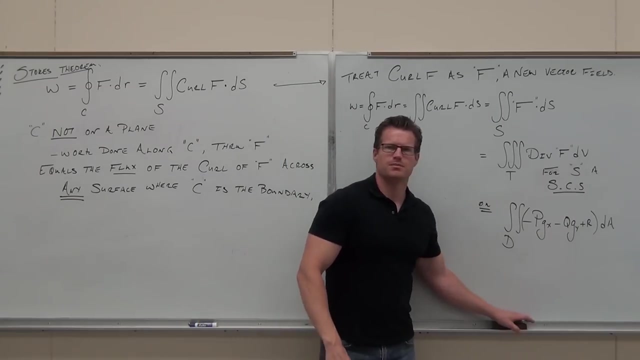 So in general, We deal with this. This was the other way that we dealt with surface integrals of vector fields, flux integrals. But this also means that, hey, how about this? Can you figure this out? This is implying that our surface is defined in a certain way. 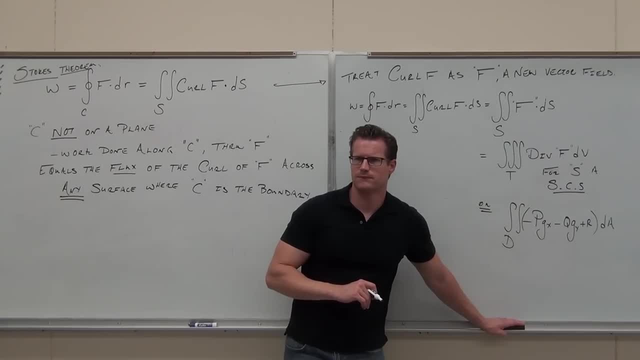 How is our surface defined? Not vectors, They're not parametric surfaces. I want you to look at the partial derivatives. What are the partial derivatives with respect to? So this would be a surface defined as Z equals. Perfect, Yeah, that's exactly right. 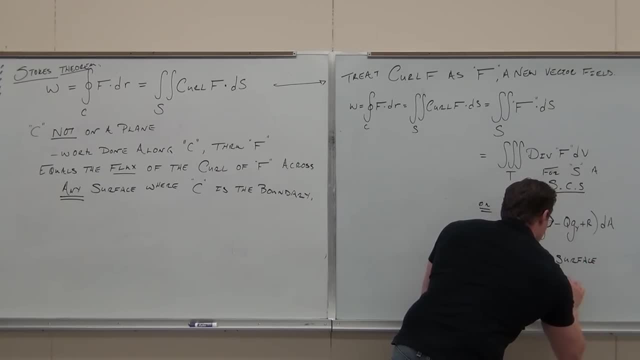 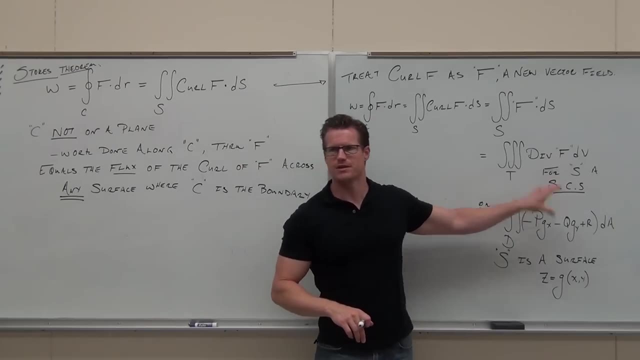 Just like it was before. this is what happens every time. This doesn't really happen with the Stokes theorem, at least not very often. This happens every time. I'm not even sure if that can happen, but this happens every time. Shall we try one. 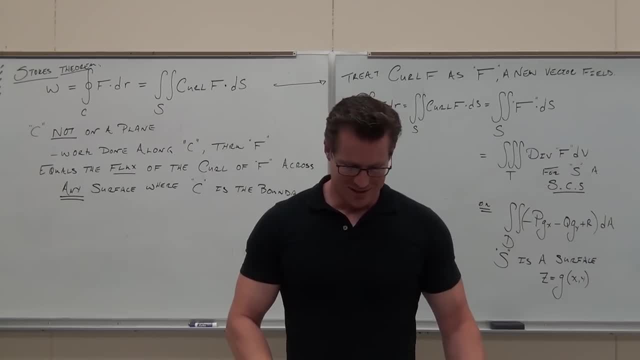 One, Seriously one. I have no more written down. This is the last piece of paper. It's almost sad. It's going to make me cry, Not really. Let's go to Costa Rica, man Woo. See you all there. 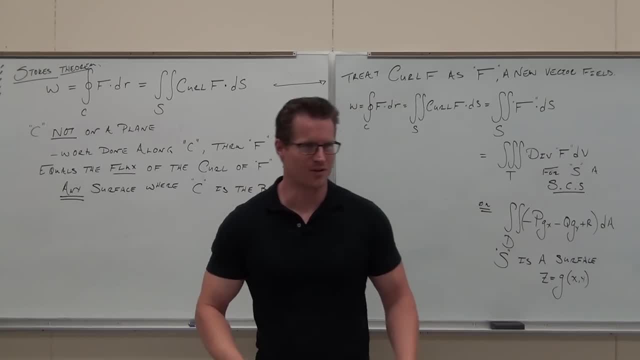 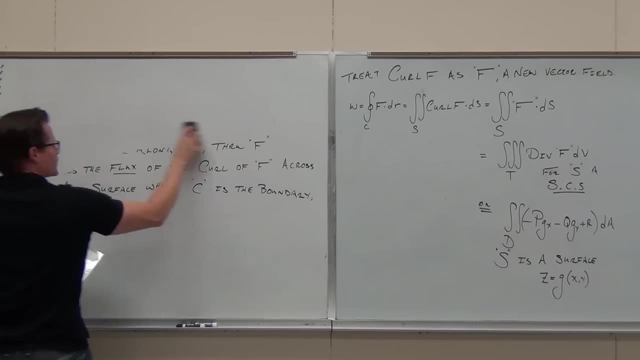 I'm building a house. I'm building a house for 12 hours a day, But it'll be fun. What was that question back there? I just said that one's the last example you had of that book. no, It's there. 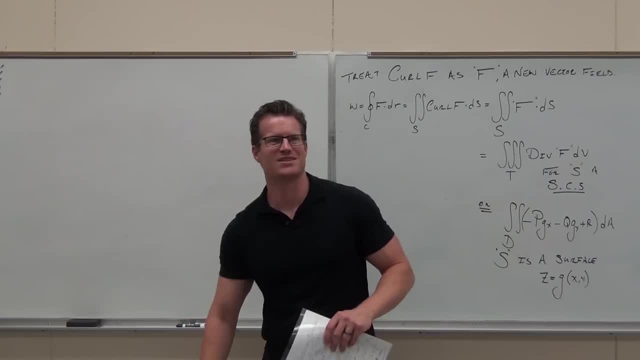 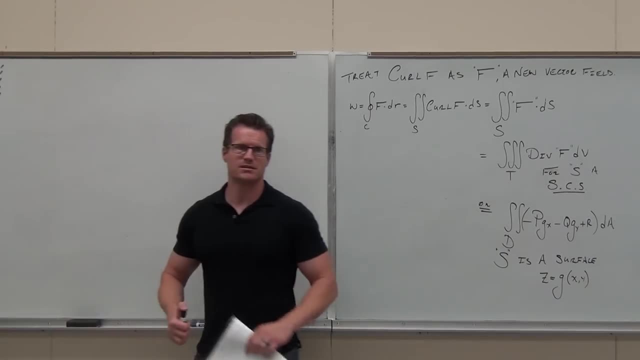 Wow, Right there, Out of 750 pages of notes and done homework, we end up the last one. You actually went through your guide, sat down for this. did you prepare for this class and write that out, or just I mean. 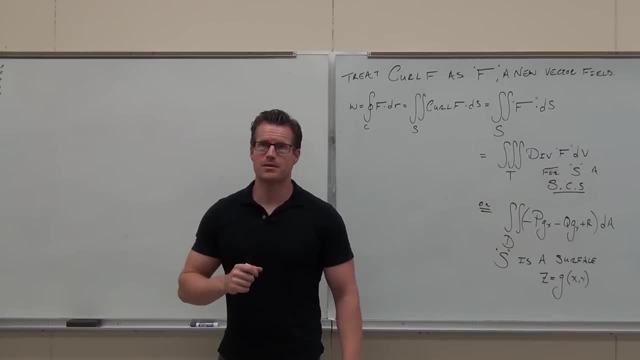 that's part of when you do it as a professor, I spent three months eight to ten hours a day creating this class. Wow, I gained 15 pounds. All I did was calculus and eat cookies. man, I gained 15 pounds. 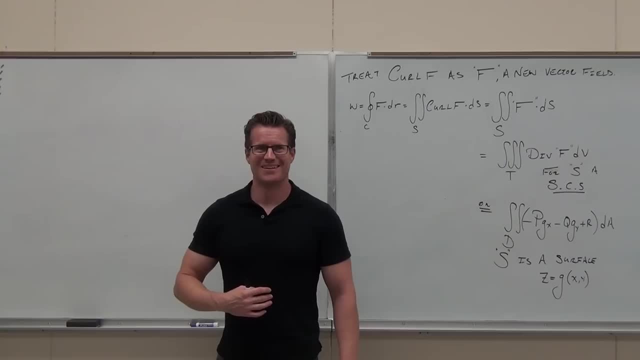 I'm just finally losing the last five. right now. Someone online was like man Leonard: lost a lot of muscle and gained some fat. Something must have happened to him. He must have had a kid. Well, yeah, I did. Well, I didn't have a kid. 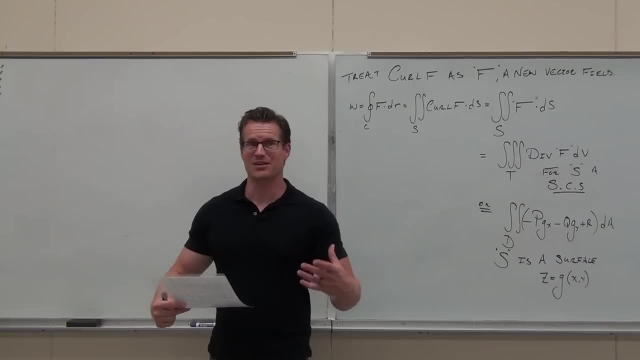 I'd look good if I had a kid. But yeah, I did calculus. That was my baby that I produced. Am I right? Here it is, I'm delivering it to you right now. It's kind of gross, You can think about it. 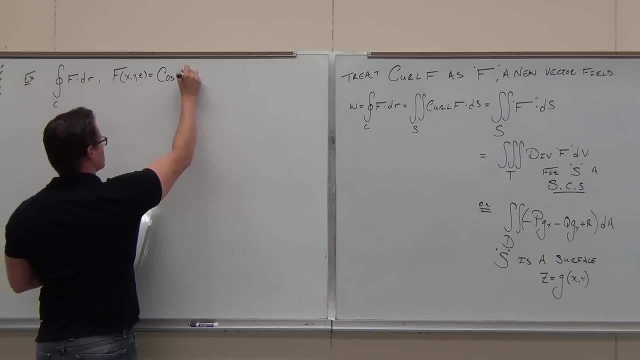 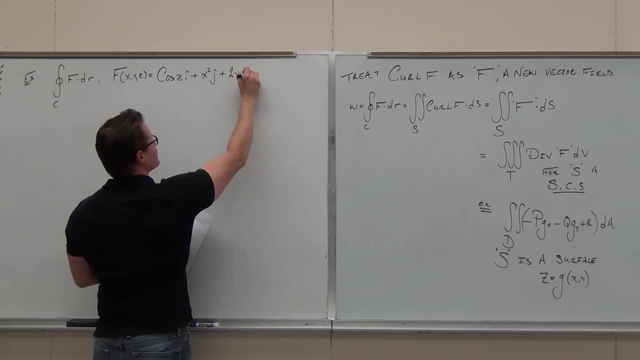 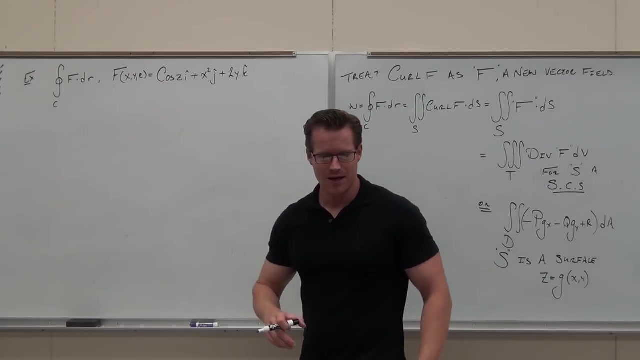 You know I'm going to milk this for all it's worth, though, right, We're going to go Leonard speed on this one. You're going to understand everything about it before I. let us be done with this stuff. So let's find the line integral of this vector field. 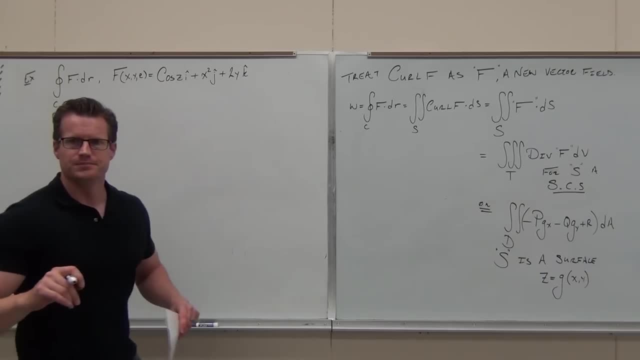 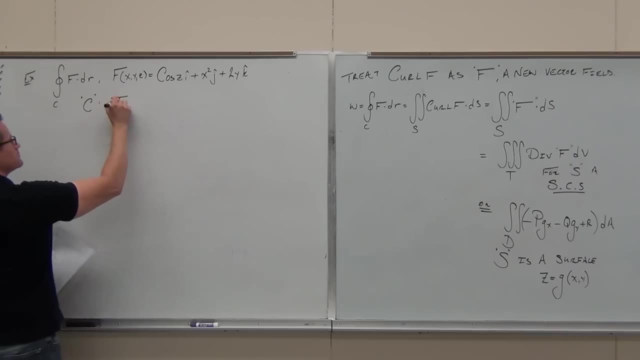 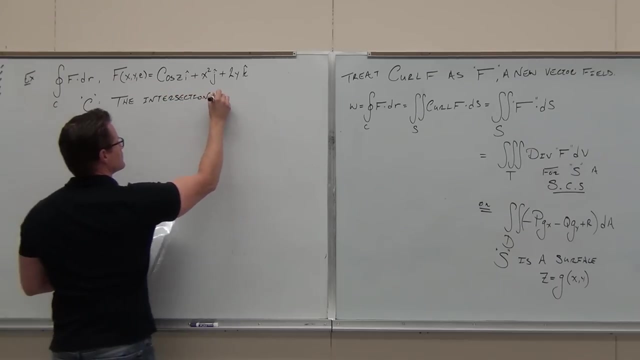 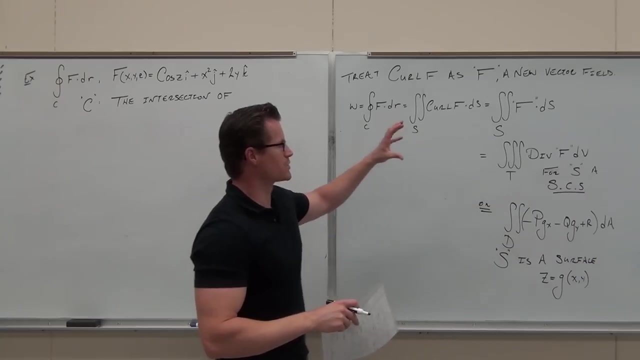 I've given you a vector field. What else do I have to give you Curve, Curve. I have to give you one curve. Yeah, you know what That would work if we had two surfaces coming together. that created a boundary. That created that. 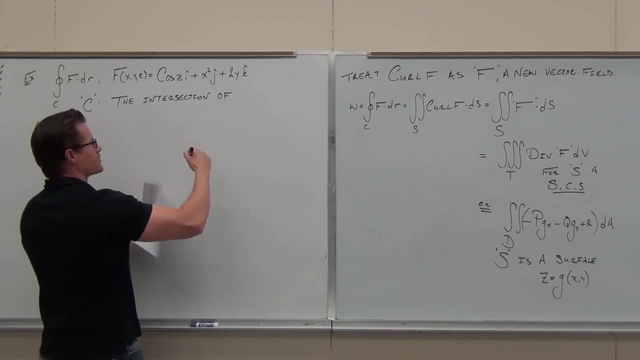 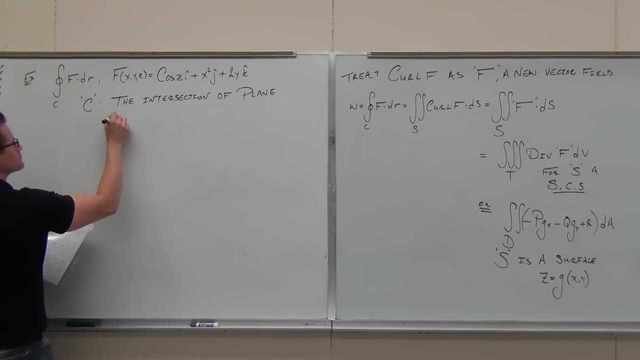 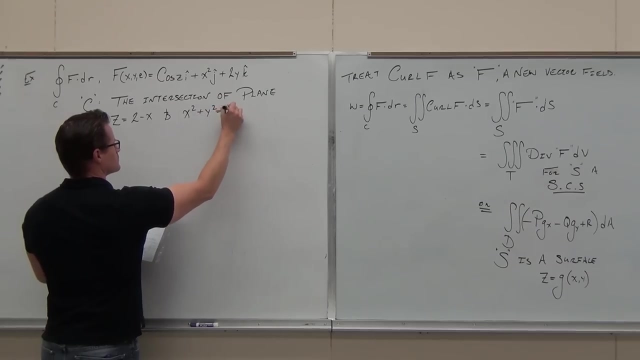 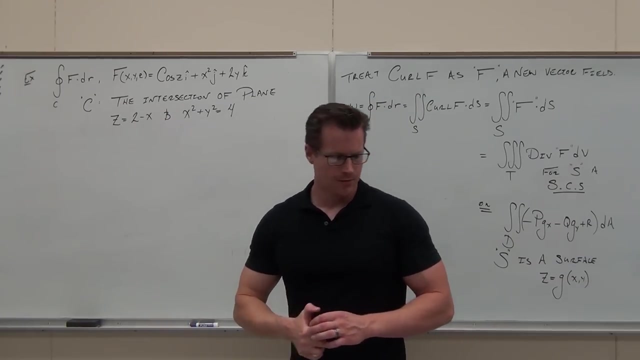 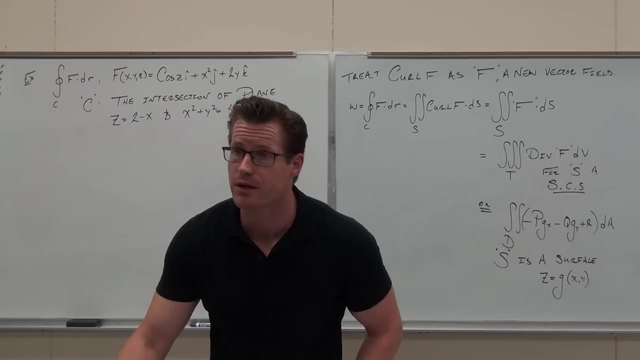 That'd be fine If you could define them as two: the boundary of two surfaces. There we go, Of course. what I've been preaching the whole time is that you get the setup correct and understand the fundamentals of what's going on here. 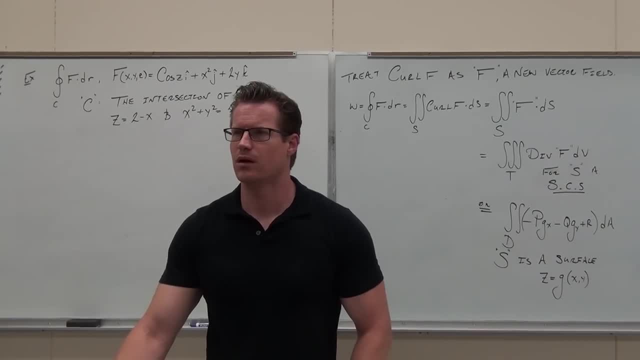 So let's read the first part. What am I even asking you for? Line integral, Very good, Somebody else? A line integral, A line integral, A line integral of a vector field where we have a simple closed curve. What two theorems could possibly apply right now? 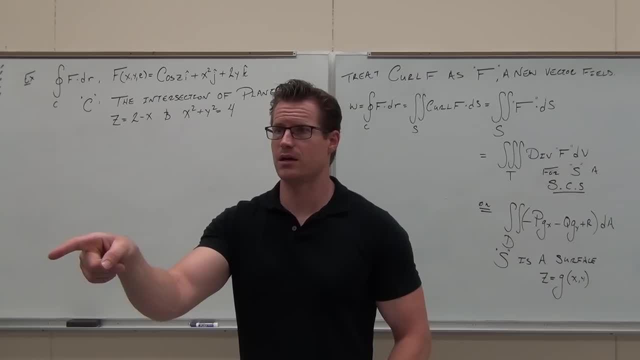 Green's theorem could possibly apply. if the curve happens to be on a plane, Very good. Is it on a plane? No, This is a plane and a. do you see the cylinder? Here's a cylinder, Here's a plane. It's not the curve. while it could be looked at as flat, it's not unequal. 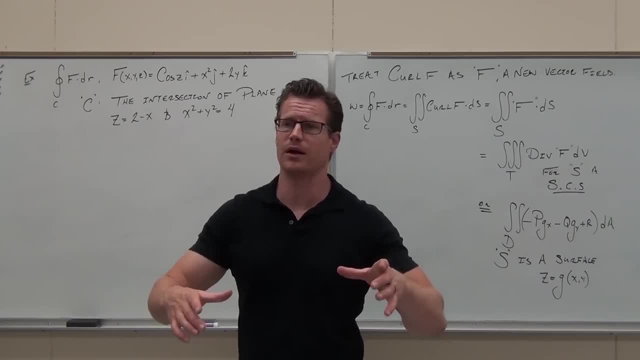 We can't do it with Green's theorem. It does not apply. Does that make sense to you? What other theorem would apply? Stokes' theorem, As long as we have a simple closed curve. So you think about this. This is what I'm trying to get you to do with divergence theorem, with Stokes' theorem. 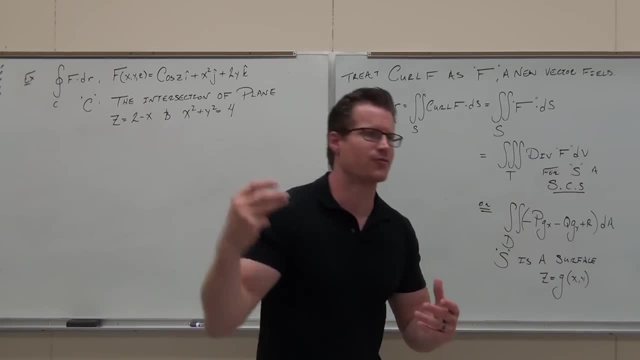 Look at the region. Look at the curve that's created. Now, I'm not talking about a 3D surface here. This is not what line integrals do. Line integrals talk about a curve through space. Well, let's look at it. 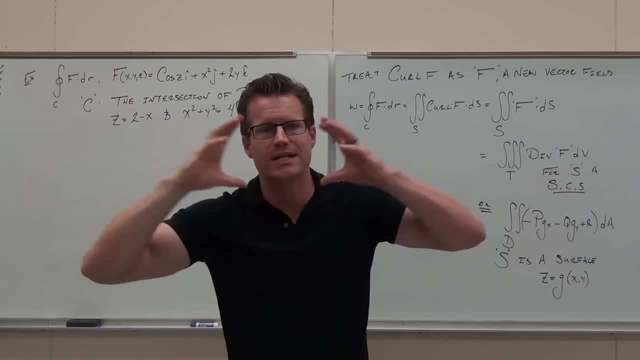 The intersection of a plane through a cylinder. What's that give you? Well, it's the intersection of a plane through a cylinder. What's that give you? It's the intersection of a plane through a cylinder. What's that give you? 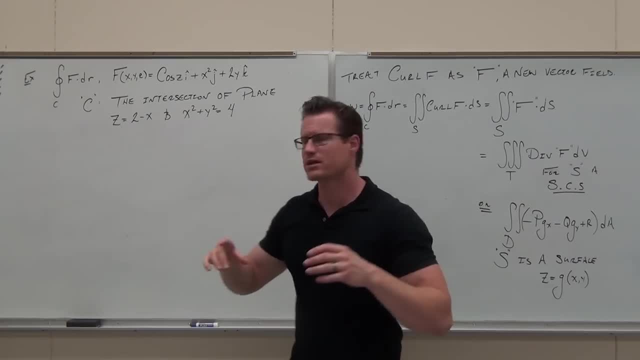 Line integrals. do Line integrals talk about a curve through space? Well, let's look at it: The intersection of a plane through a cylinder. What's that give you? It gives you a curve. It gives you this curve that's cutting out the edge of that cylinder. 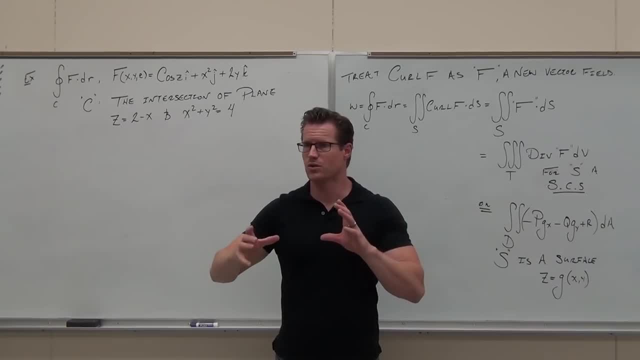 Does that make sense? That's what's happening. It's not a surface, So a surface integral right off the bat doesn't apply, but a line integral does. It's a simple closed curve in three-space. Now what Stokes' theorem says is: 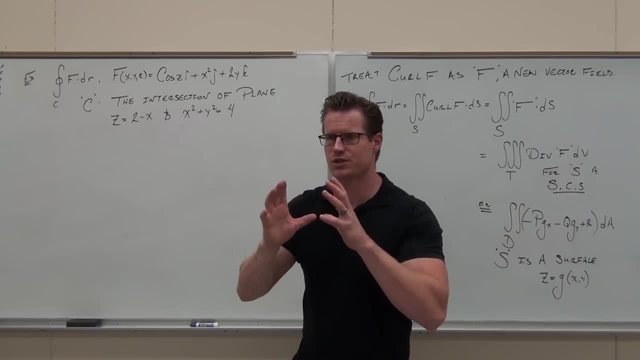 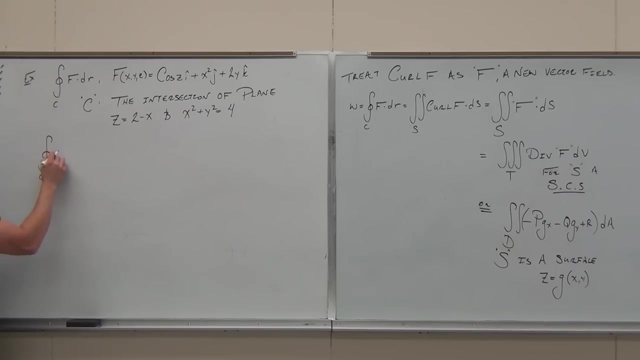 a line integral. I can use a surface integral of a vector field to do it. I can use a flux integral to do it. Does that make sense to you? So right now, write down Stokes' theorem. All Stokes' theorem says is that this thing can be calculated. 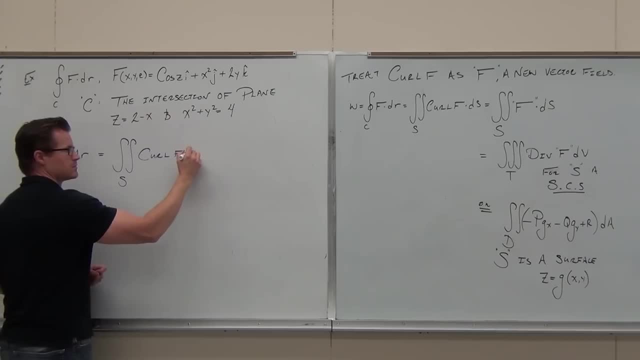 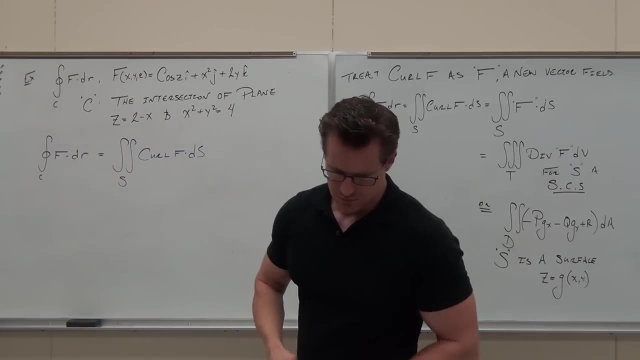 as this thing. That's all it says. And now, if you see that Stokes' theorem applies and that that is what it says, And now if you do you see that, Okay, explain to me then why does Stokes' theorem apply? 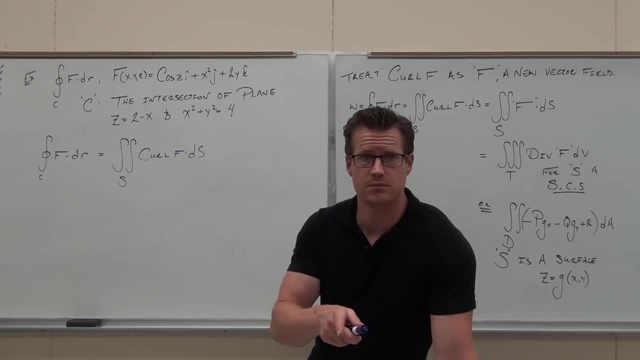 Simple closed curve. that's not on a plane through a vector field- Non-conservative. I don't know. We can check it, I guess, But I guarantee it's non-conservative. Why? Why do I guarantee it's non-conservative right now? 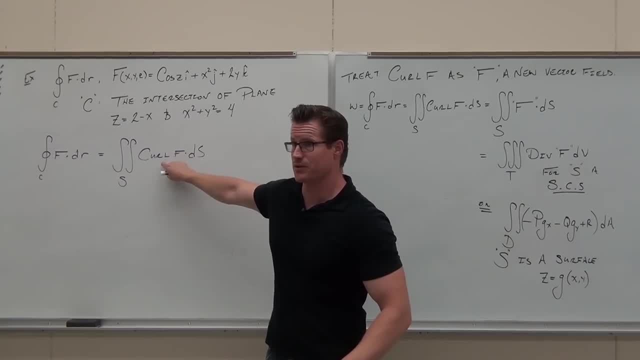 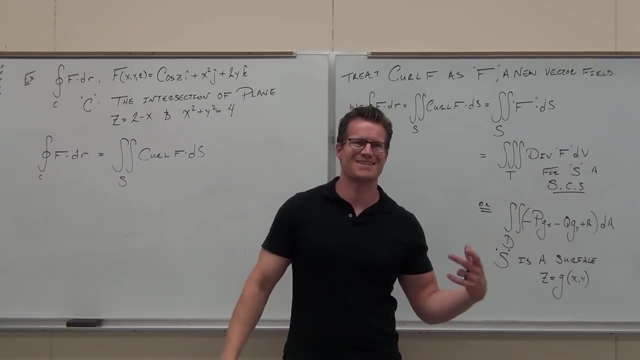 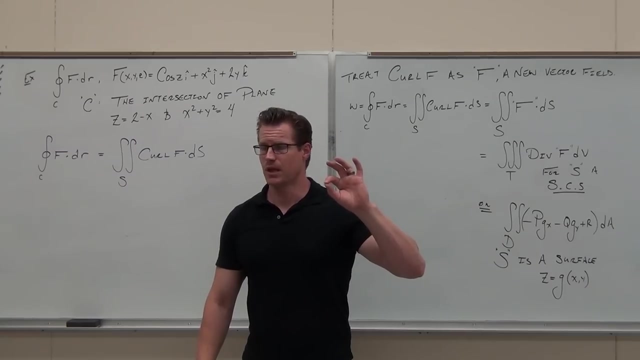 Why do I guarantee that that vector field is non-conservative? Because the curl of F is zero. What That generalizes something: It says that through any conservative vector field, line integral of a simple closed curve will be zero every time. 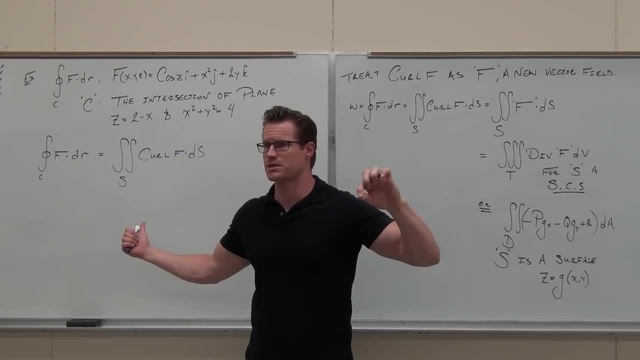 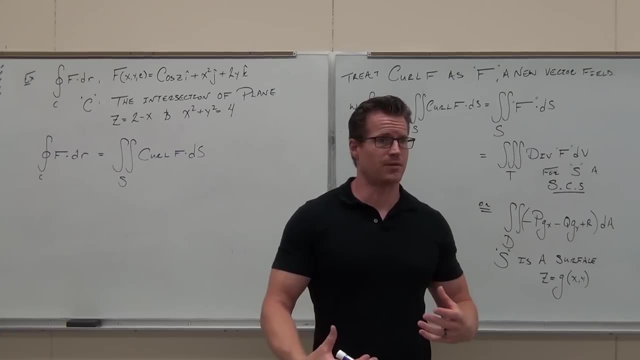 Because Stokes' theorem says it will be right there. Does that make sense? It's pretty cool, Because if curl F is zero, it gets zero Impressive. Now do you remember how to find curl F? Because it's going to kind of depend on that right. 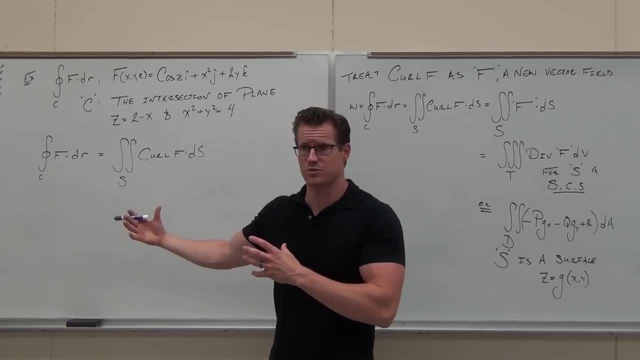 You're like curl. Who needs curl and divergence? We do These theorems, rely on them. If you cannot do that, you cannot do these theorems, And they're very important that we would be able to do this to find work done through vector fields. 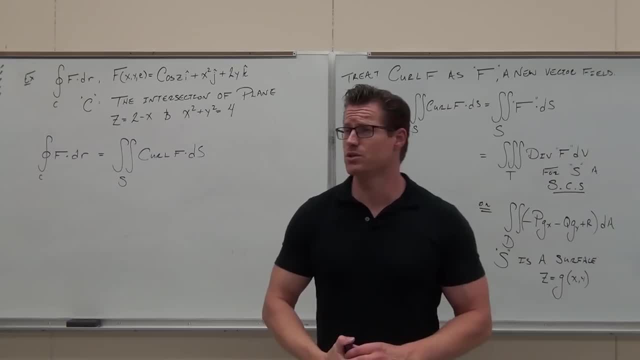 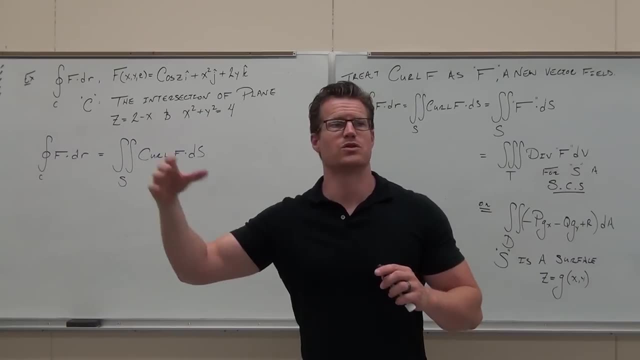 Can you please calculate curl F for me right now? If you remember how to do it, it's that like a determinant of that matrix that we created. We have i, j, k, We get the del and then we cross it with p, q and r. 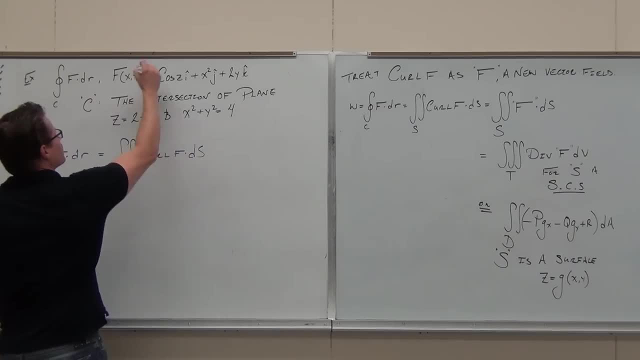 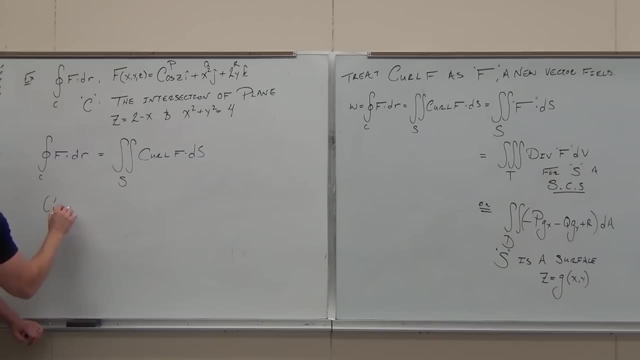 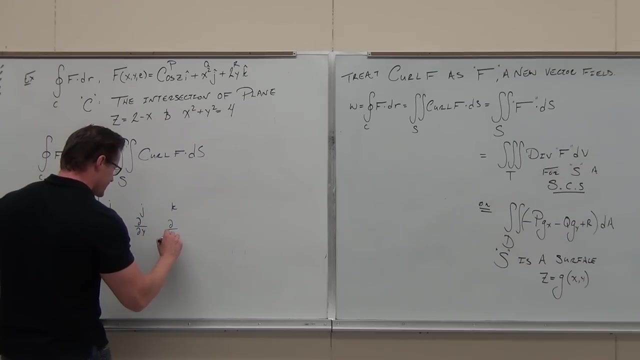 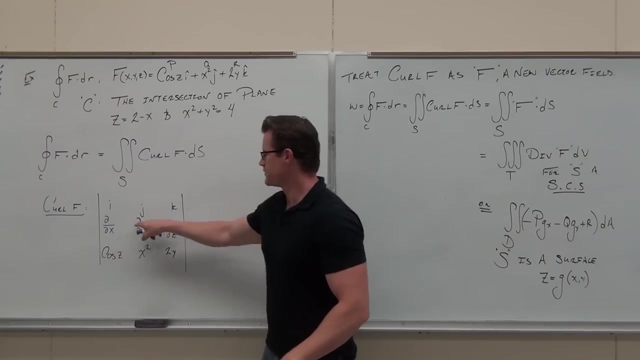 So probably pretty useful to be able to identify p, q and r. Okay, that's on, you guys Go for it. I've done this setup for you. Hopefully you see where it comes from. Partial derivatives, that's your del, p, q, r. 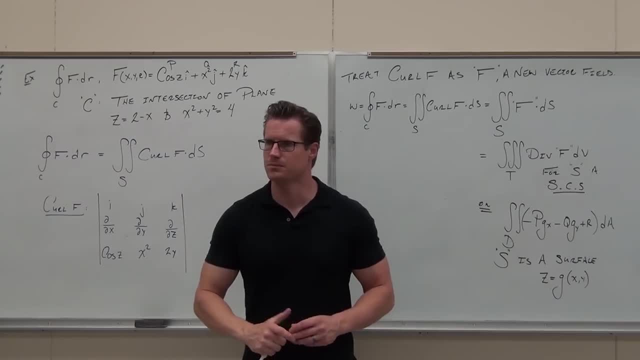 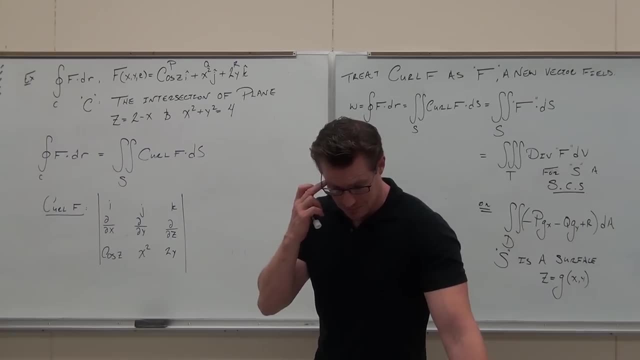 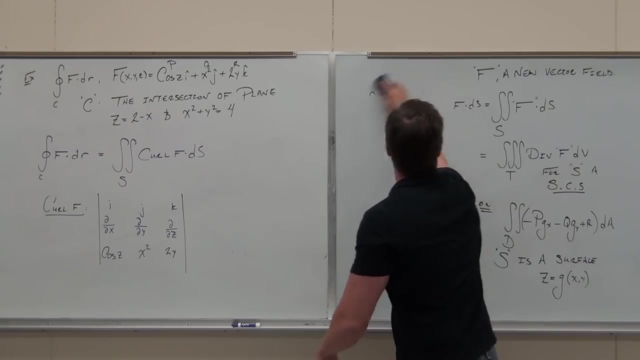 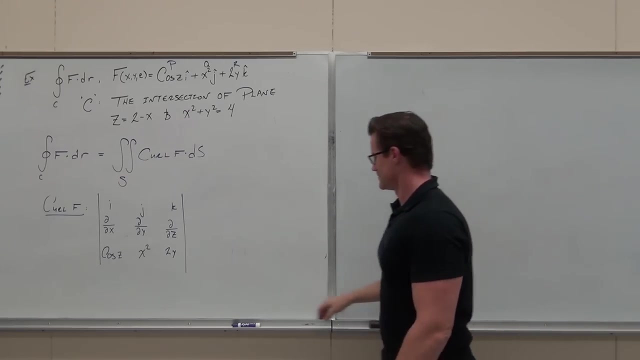 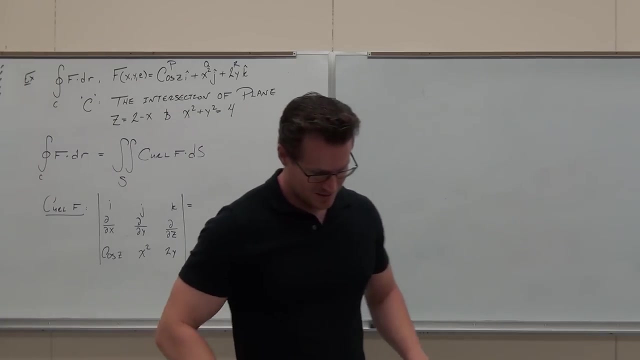 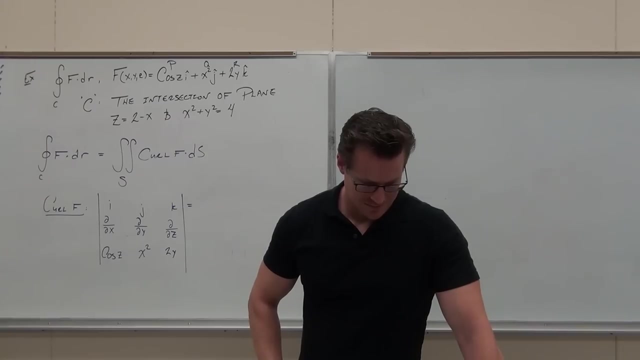 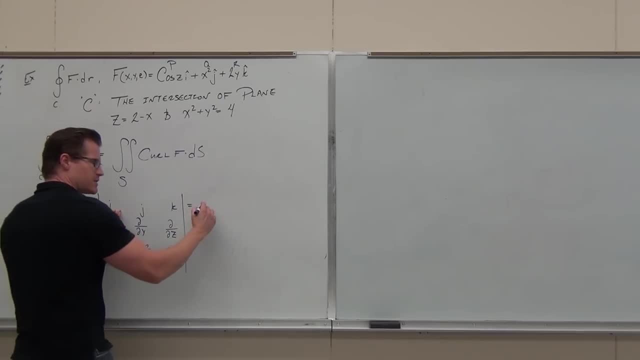 Cover this: partial minus partial. So what's the difference between partial and partial? What's the difference between partial and partial? What's this? give us Two minus Two minus Two minus Zero. We got a partial derivative of this with respect to z- zero. cool, love it. 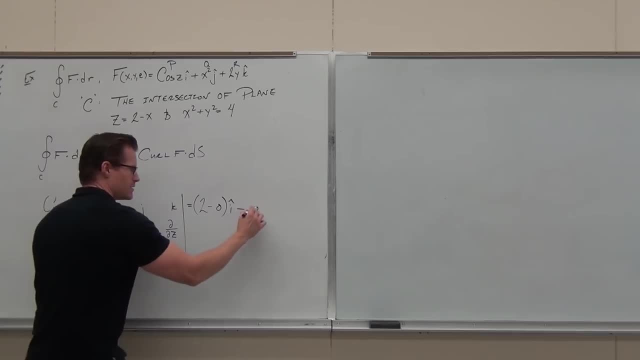 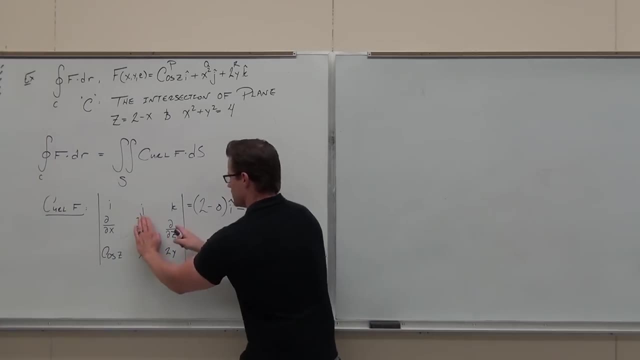 Minus sign. cover that up. Partial derivative is Zero, Zero, Minus, Minus, Minus, Sine z, Sine z. Let's be careful about this. one Partial derivative of this with respect to z is a negative sign and I'm subtracting it. 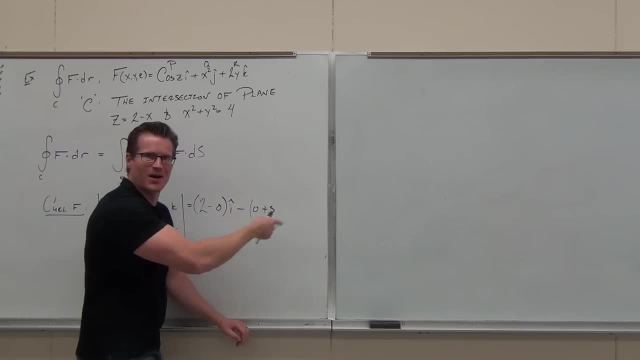 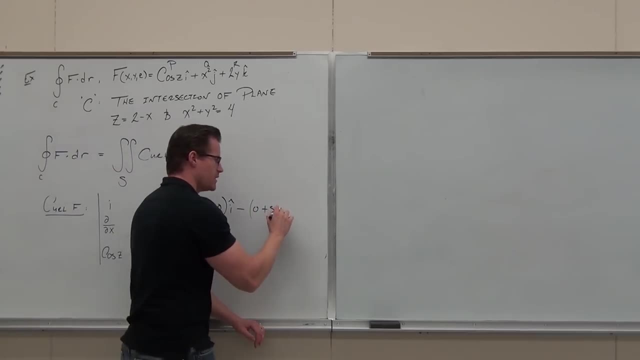 Plus sine z, which is gonna change to a minus. That's why we write this stuff down. You know that sign errors are the biggest thing for us, right? sign errors in algebra. Write this stuff down, don't put too much in your head. 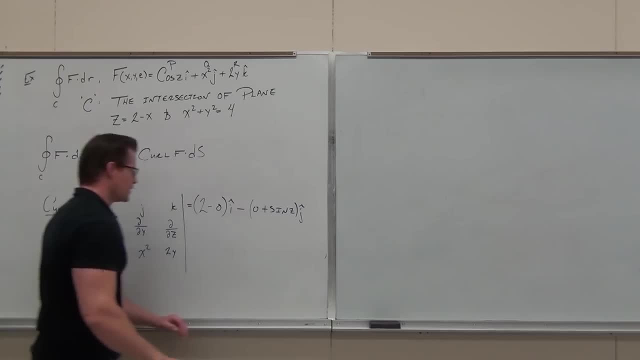 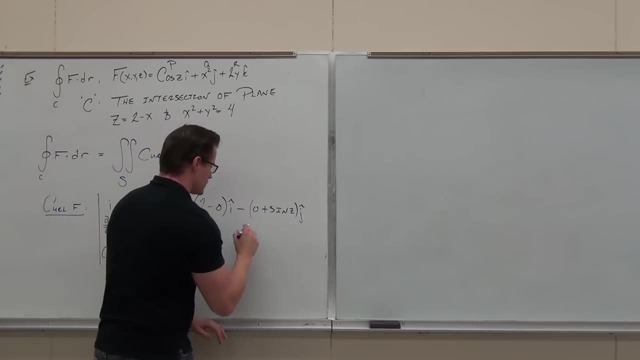 or we start making errors and then nothing works out right for us, and that's a bad thing. The last one: we covered that up: Partial derivative here: Two x Two x Minus Zero. Did you get it? 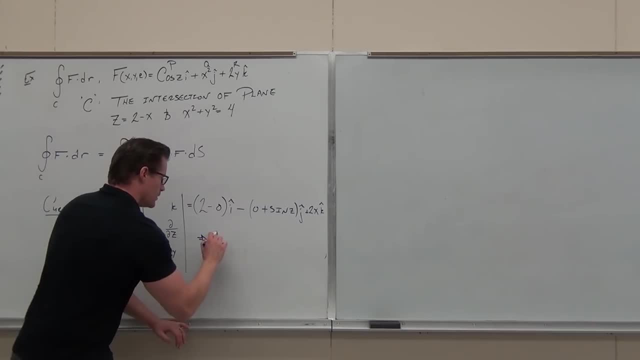 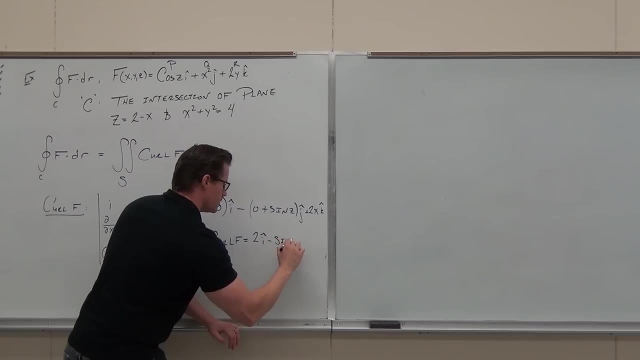 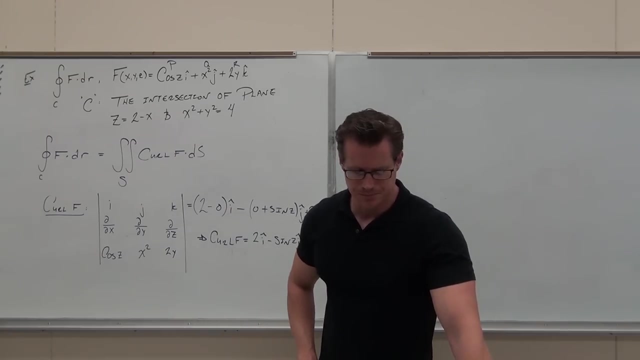 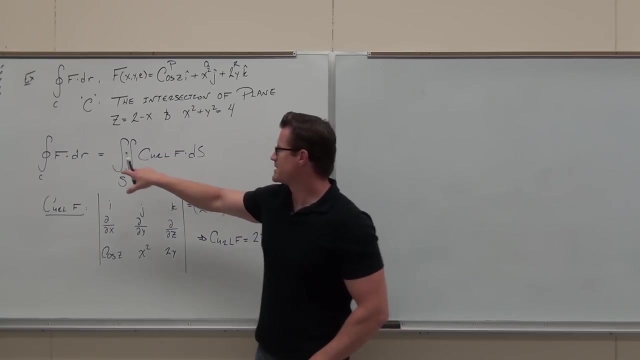 Simplify it a little bit, Ladies and gentlemen. are we okay with that so far? for real, Now what I'd like you to do whenever you have to do this right now: redefine this. You see, if this is a surface integral. 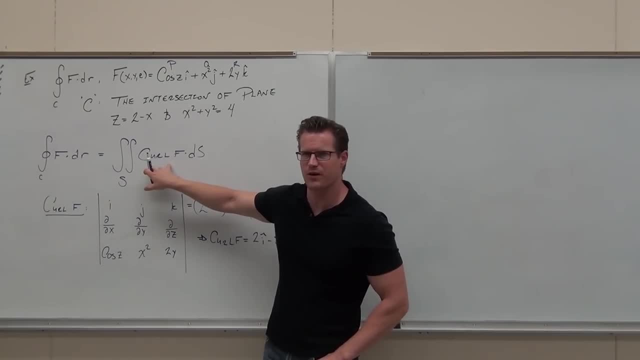 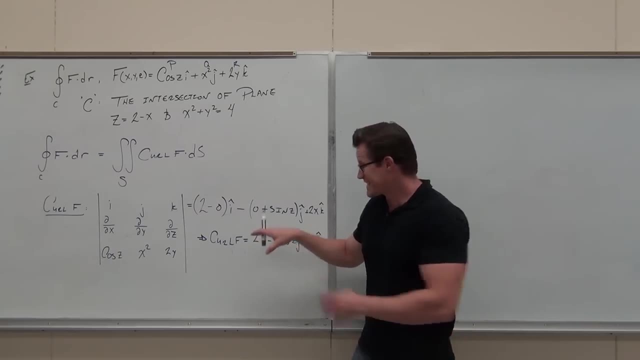 then that has to be a vector field, and some of you guys didn't catch it. you've seen it before, but verify this: This is a function-defined vector field. It's giving you a vector at every single point: x, y, z. this is a vector field. 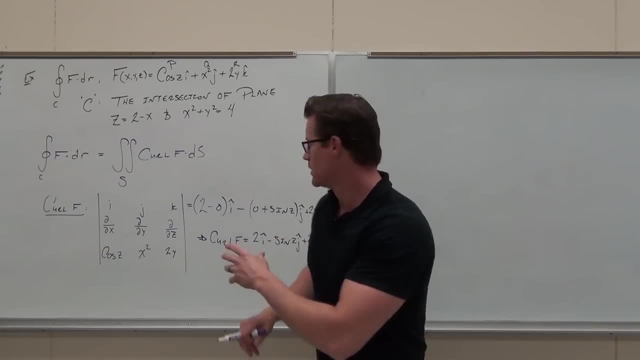 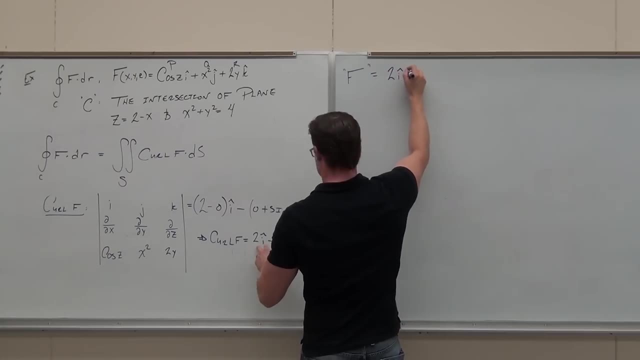 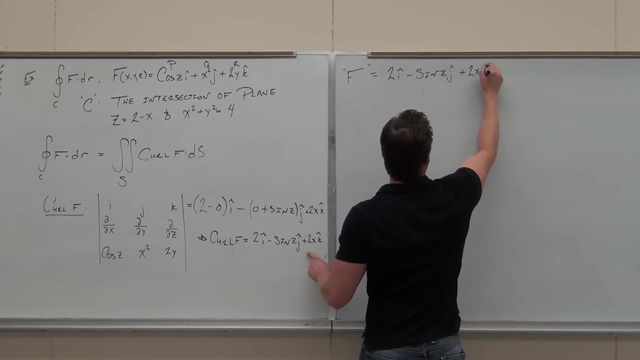 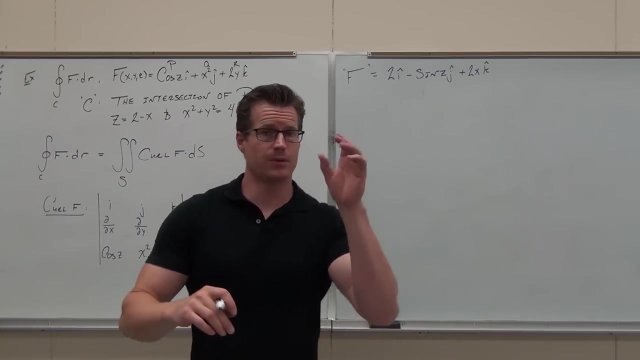 Redefine that as your vector field. So now our f, our new f, is that: Why, Why, Why do we want to do that? Well, if we do that, then we can start labeling p, q and r. 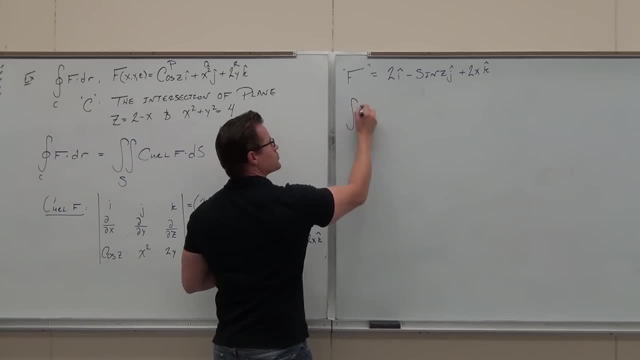 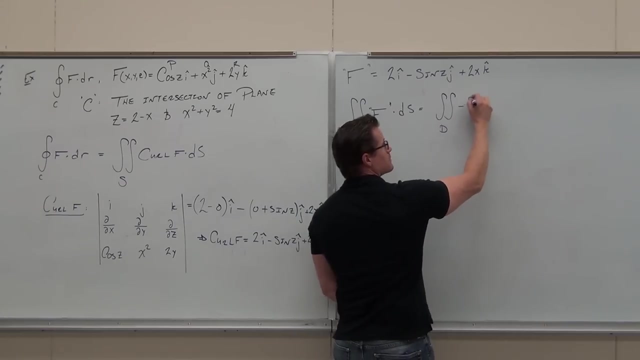 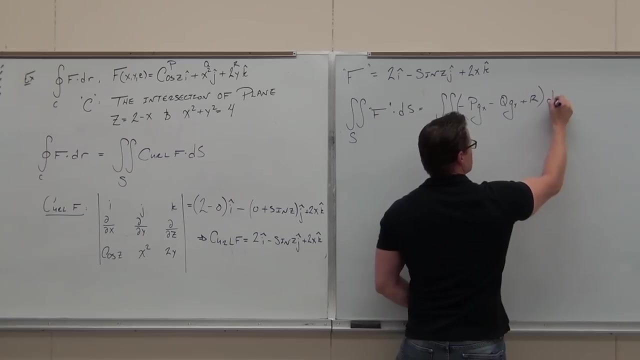 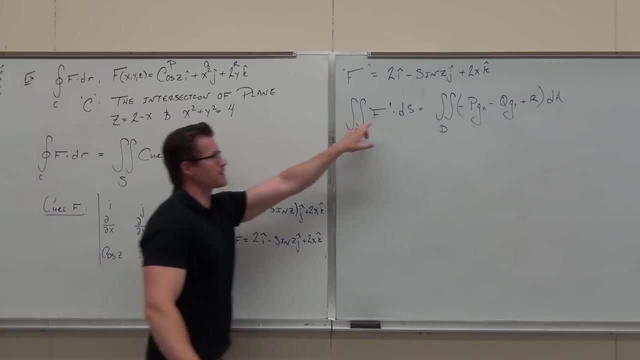 Then we can start doing well, changing this into this, Because if we have a vector field and if we're finding the flux integral of that vector field- which is exactly what we're doing here- then we can start using this old stuff. 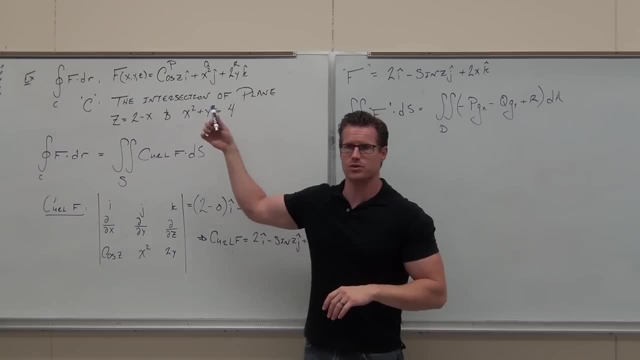 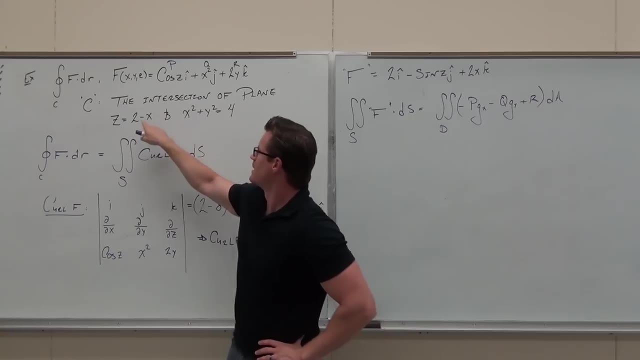 By the way, we're not using divergence there, because we do not have a simple closed surface, And I can't- I thought we, I can't think of an example where we would have one This one. well, let's look at the surface. 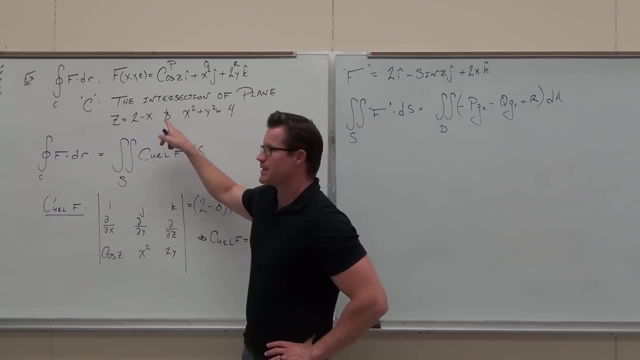 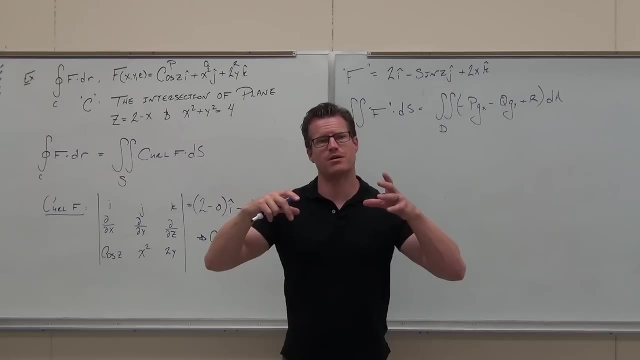 Let's look at the surface. If we define the surface, what's happening is all. I need now be careful here. All I need is this: All I need is for some surface to have a boundary of this curve, this intersection. Are you listening carefully, please? 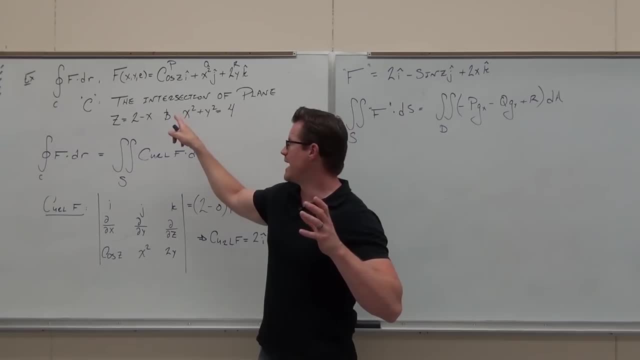 Please listen carefully. All I need is any surface that has this curve, the intersection as a boundary. Does that make sense? This can be used as that surface if we also look at this thing as the region that contains that, as the projection. 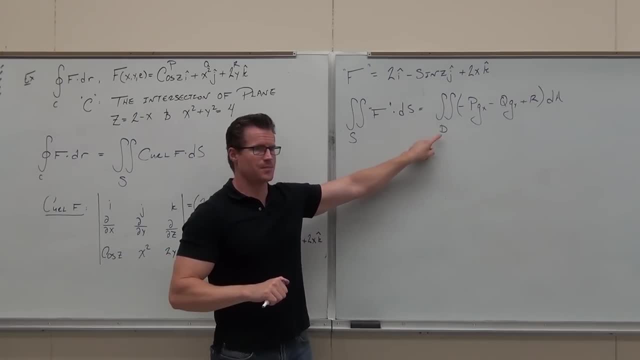 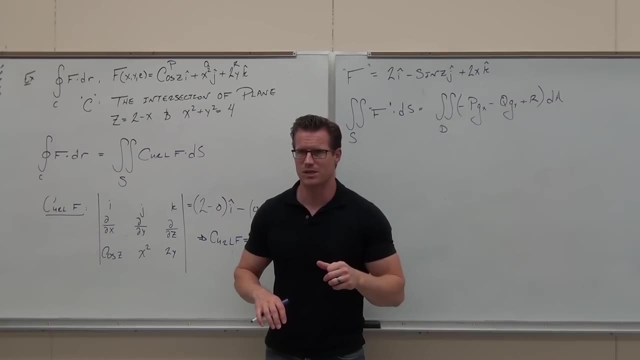 Because remember what this does. this says that d is the is the region as projected onto the xy plane, where z is a function of x and y Is this. is this making sense to you? Say it one more time: The curve has to, has to bound, whatever surface you have up there. 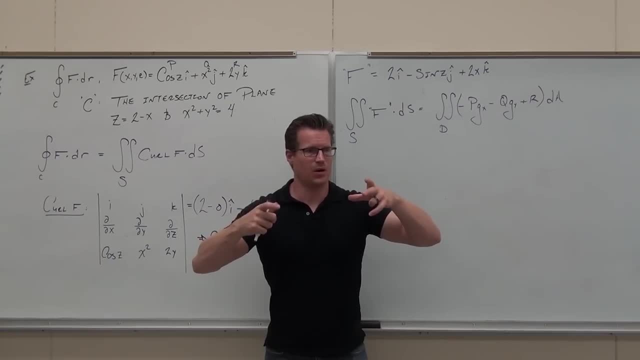 It doesn't matter what surface it is, It doesn't matter, But it has to bound that surface, okay, So define some surface where that is a boundary, but then, when you do that, the region that you get on the xy plane comes from these two things as well. 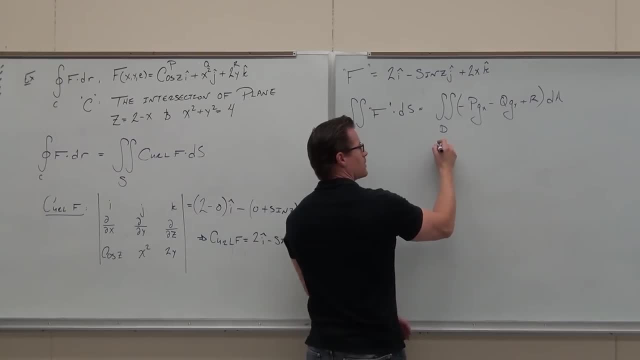 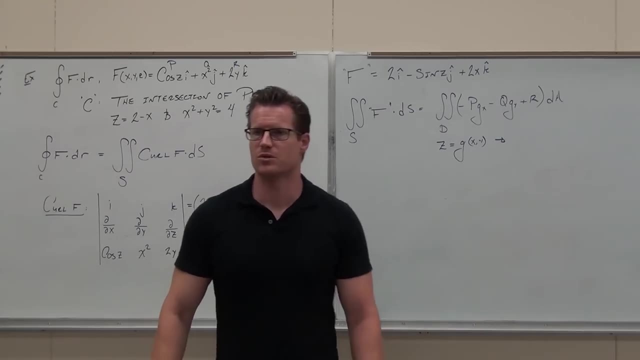 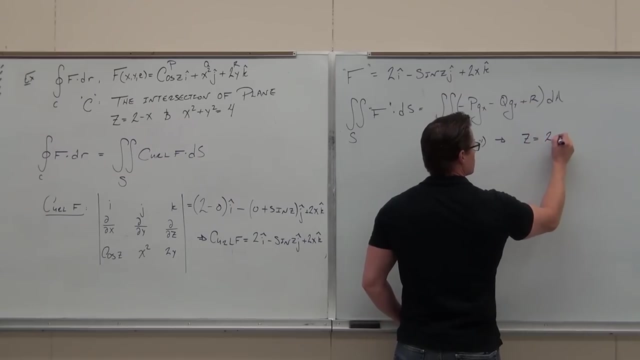 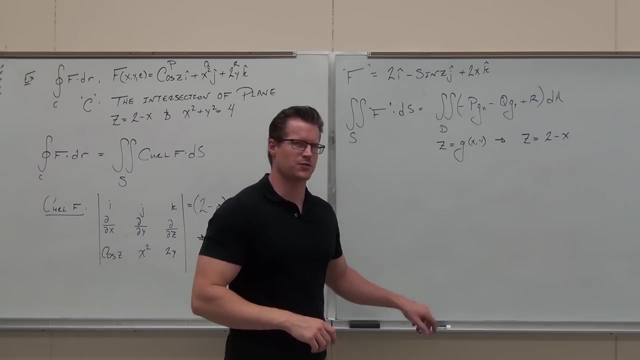 They have to be there. So let's define our function of x and y. Do you have something up there that's defined a surface in terms of z equals x and y? Do we have that? Yeah, what is it? Can you right now go back to your vector field and identify p, q and r? 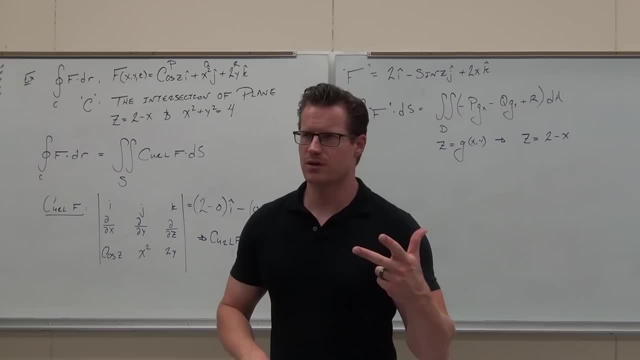 Let's see if you know what you're doing. Identify p, q and r. Can you do that in your pay-per-view real quick? Just try it. Try something, Put something down. Here's the question: Is this p, q and r right now? 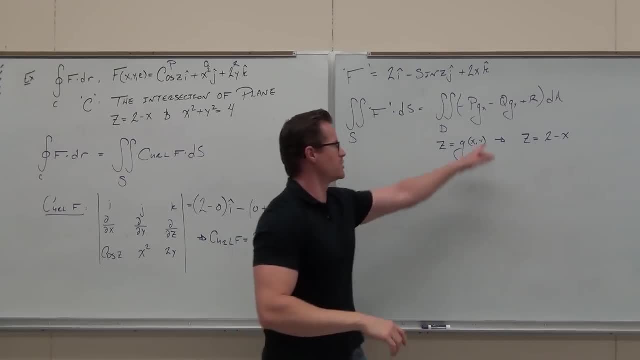 So there's a change to it. A lot of people get jacked up on that. They go: oh, you're using p, q and r, It's got to be that one. No, That's what we use to find the curl. 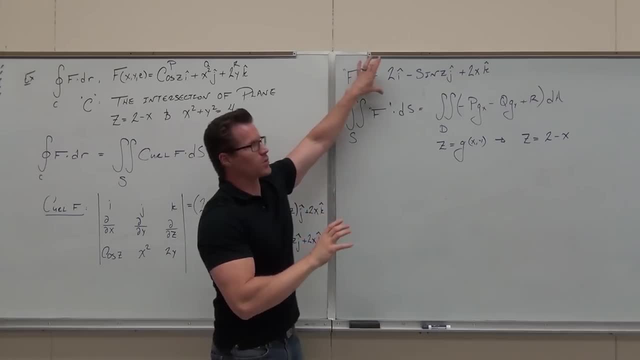 And then we make this switcheroo and we say: hey, that curl, that curl of f, that becomes our new vector field, so that we can even do this. This right here, This right here is my new p, my new q and my new r. 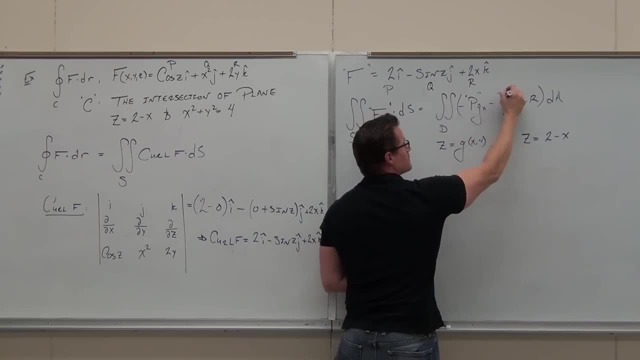 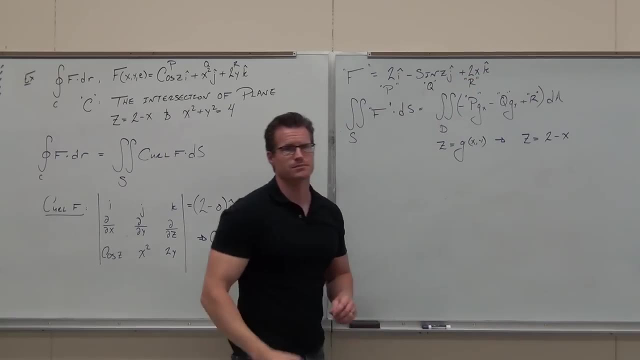 If you want to do notation, it's horrible notation, but maybe this. See, this is coming from that new vector field: My new p, my new q and my new r, Otherwise you're going to have to find new letters. 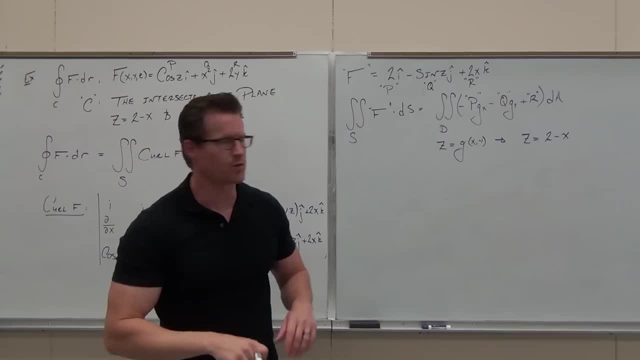 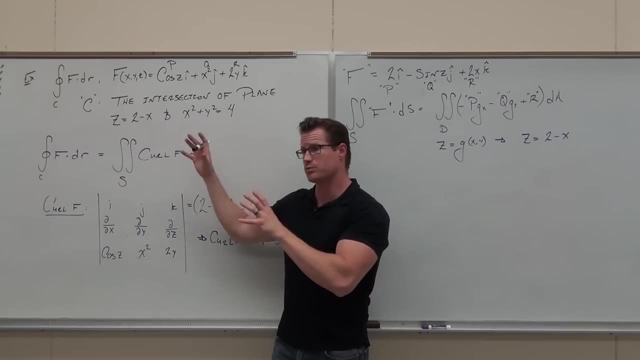 It's up to you. I don't really care. That's my notation, So use whatever you want, But that's how I think about it, so I don't get confused between my new vector field and my old one, my new p's and my old p's. 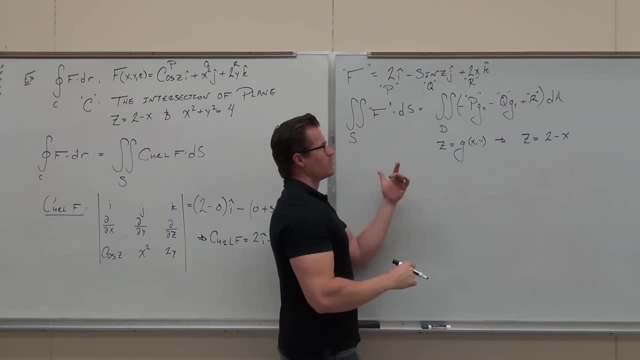 Does that make sense to you? So let's try this stuff, Let's go ahead. What's the two other things we've got to do before we set up this double integral? What do we have to do? Yeah, partial derivative of what. 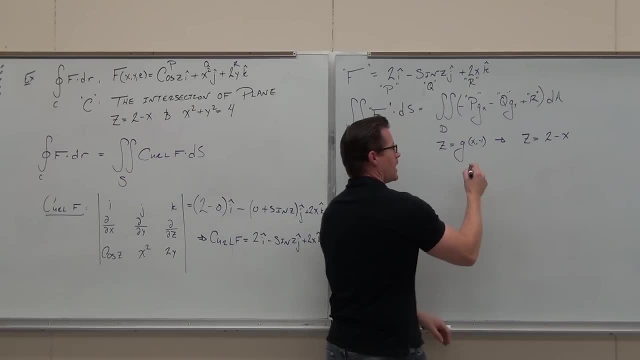 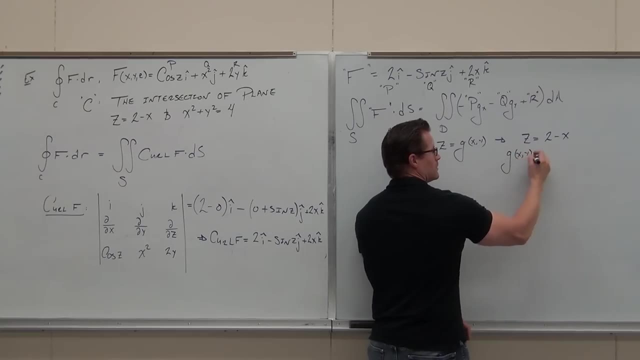 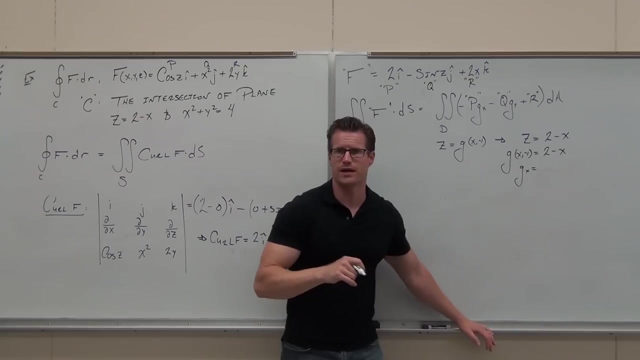 The surface that sees the boundary of. So that's this surface I want to find the partial derivative of, and if you want to write it as this so it looks a little nicer, that's fine. The main goal is to take the partial derivative of that surface that you defined. 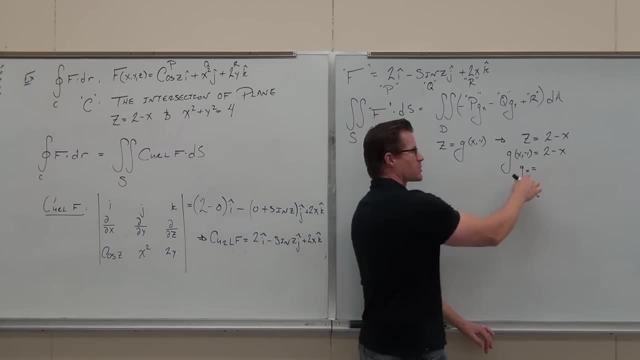 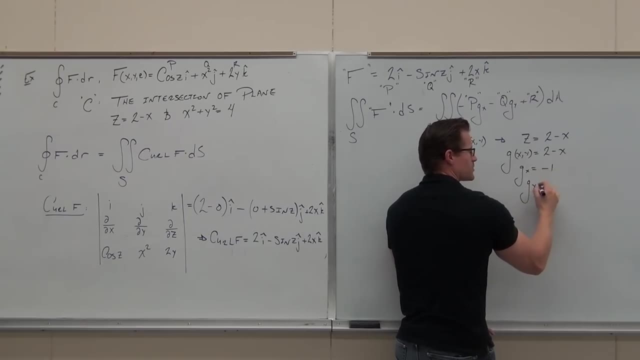 z is a function of x and y. Take those partial derivatives. Can you take the partial derivative of the space to x? please Come on, don't let me down now. And the partial derivative of the space to y is Zero. 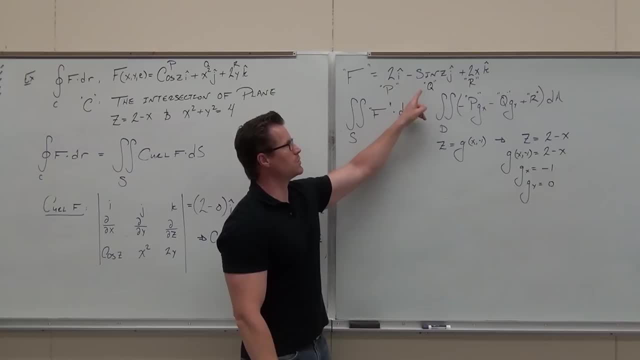 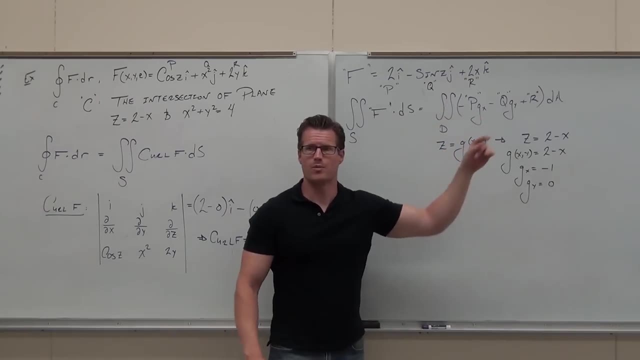 Okay, Can you take your new p, your new q, your new r, your partial derivatives of the surface that we just defined- z is a function of x and y- and put them in that double integral? Remember, we never look at the region until we set up the double integrals. 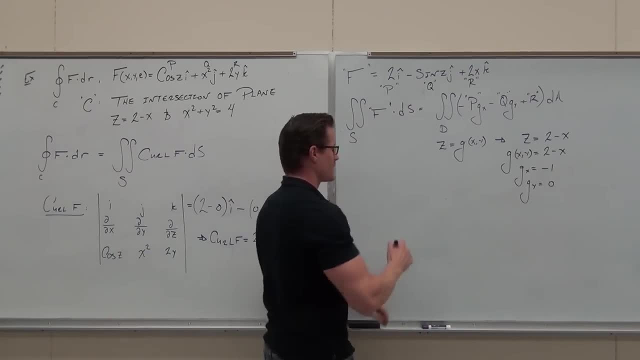 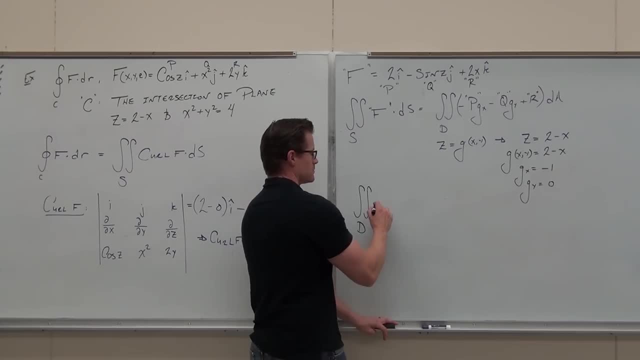 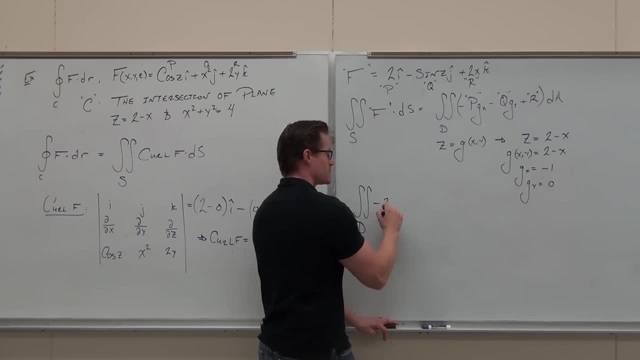 Negative, 2., Negative, 2.. I like the negative 2 because it says hey, negative, and that's my 2.. It doesn't, it doesn't matter that way, Keep going. Times negative 1.. Times times negative 1.. 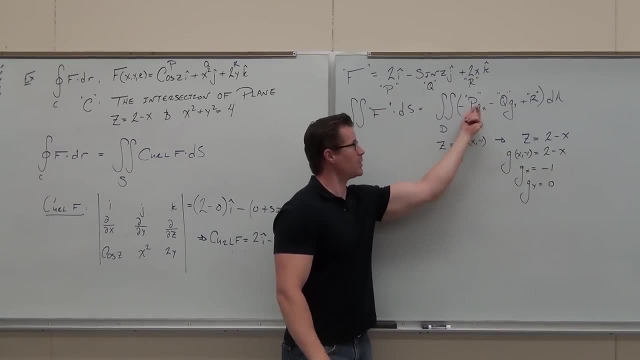 Times negative: 1. This, this, multiply it with negative. 1. Make sense, Okay, null it Minus sine Good. it would be negative sine z, because it goes with the sine. No pun intended, I mean it literally goes with it. 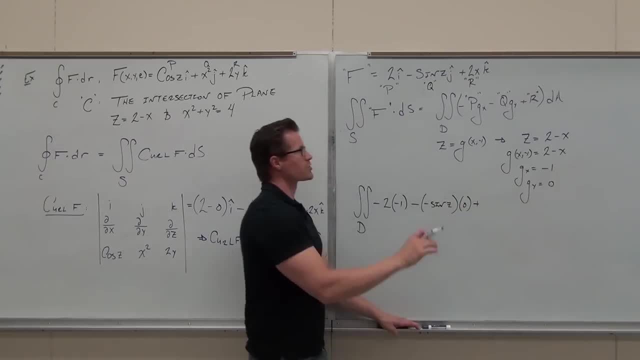 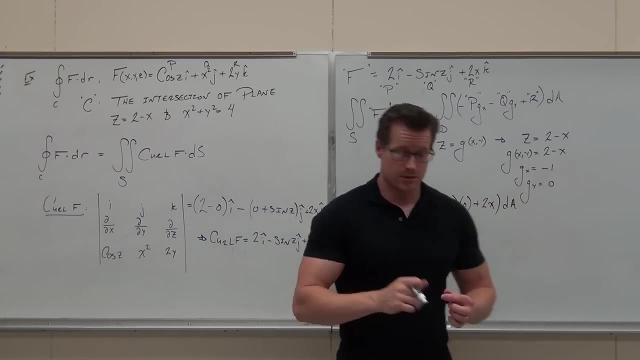 Times. oh, zero love when that happens. Plus no partial derivative. just give me the r: Two x, two x, two x, yeah, yeah, Man, we've done a lot on this problem. Sine integral, not on a plane. Stokes' theorem applies. 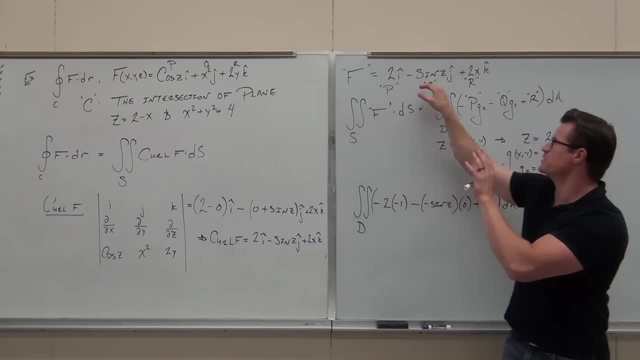 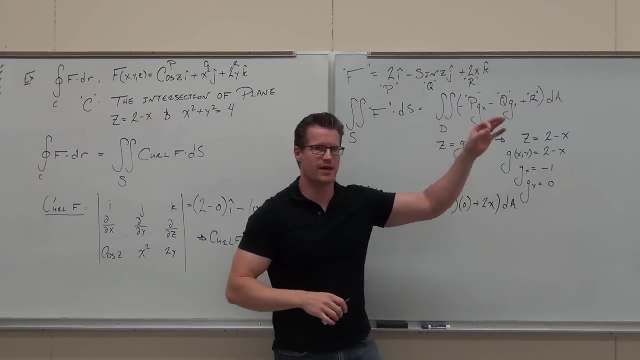 Find the curl of your vector field. treat that as your new vector field. a new p, a new q, a new r. Take a surface that has this curve as its boundary, which we have here define in terms of x and y. 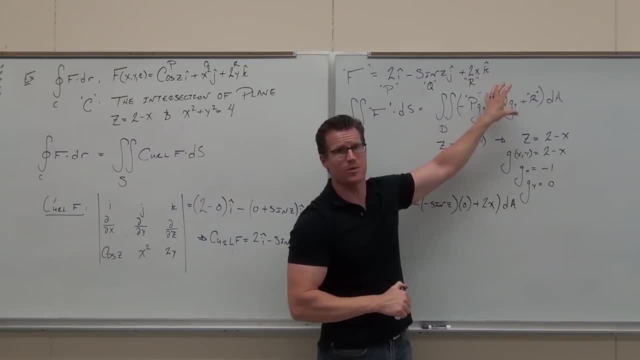 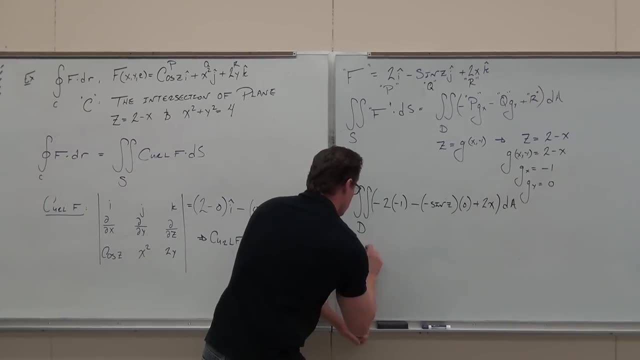 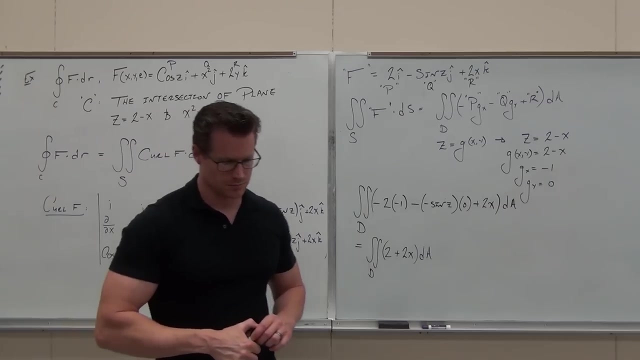 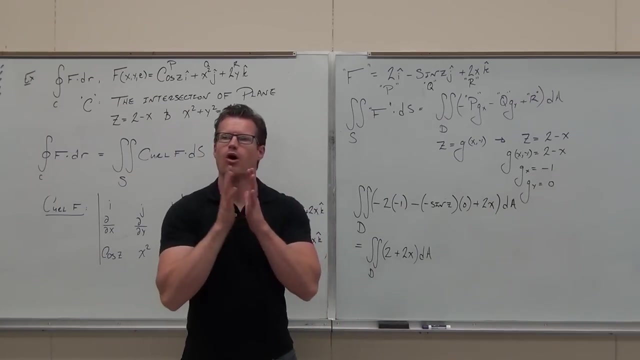 take your partial derivatives and plug it into the flux integral formula that we created a long time ago. And now, now simplify it. Now, simplify it and I'm really hoping that you remember what to do now. I'm really hoping you remember what that region means. 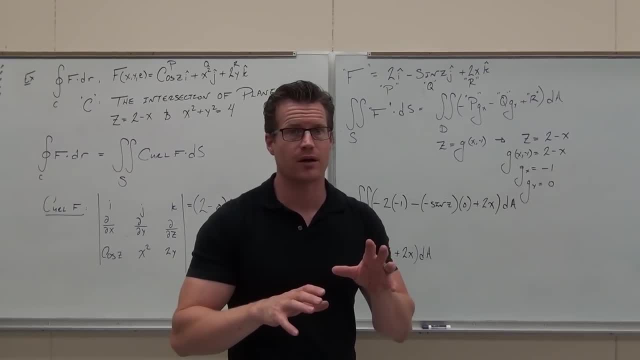 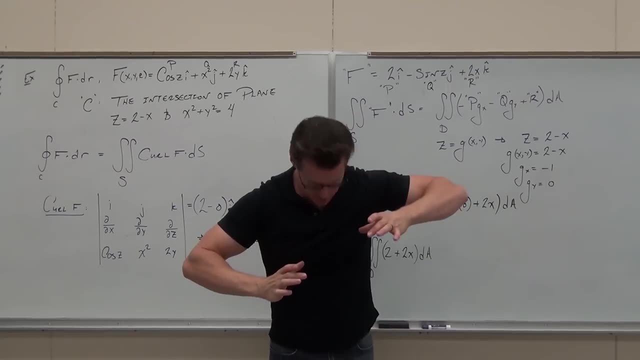 What's that region? What plane is that region on The xy? So it works the same way as everything else we've done. You look at the intersection. you say, hey, look at that intersection from the top, like that, What shape is it going to make on the xy plane? 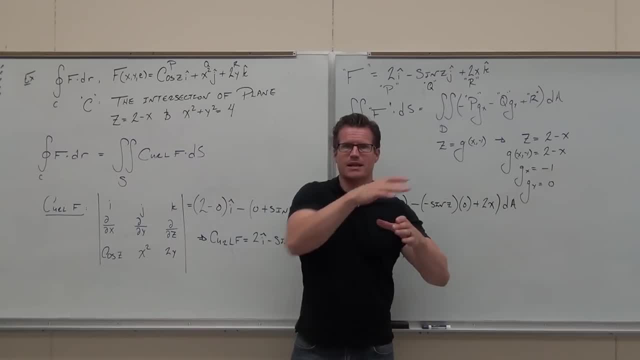 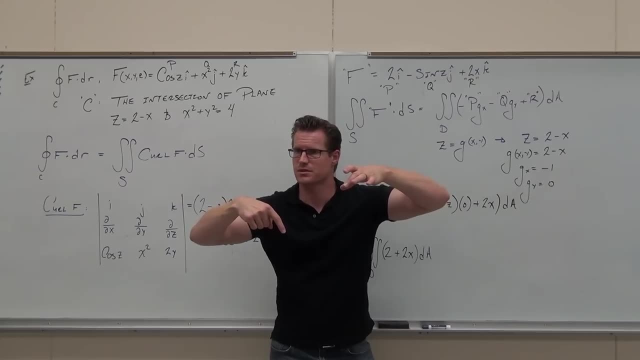 Well, if that's a cylinder along the z and that plane's just cutting it, then that shape, that surface, that that curve encompasses through space, when you look at it from the top, that makes this projection of just the cylinder itself. 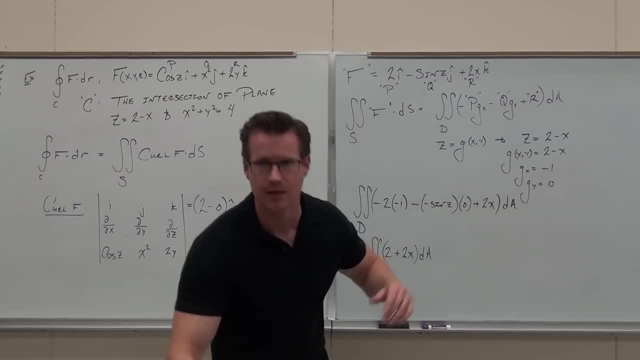 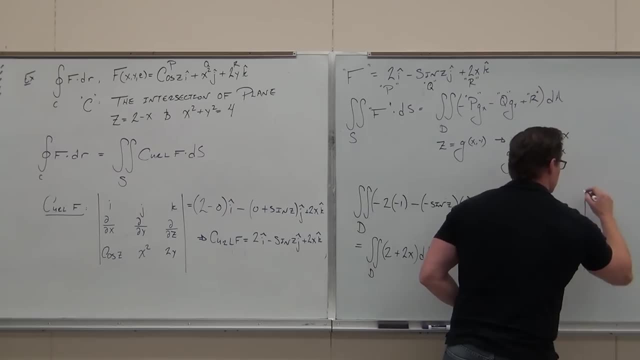 on the xy plane. And if you're like man, I can't get that, draw them all, That's fine, But just recognize that when you draw the region on the xy plane, what's the value of z on the xy plane? 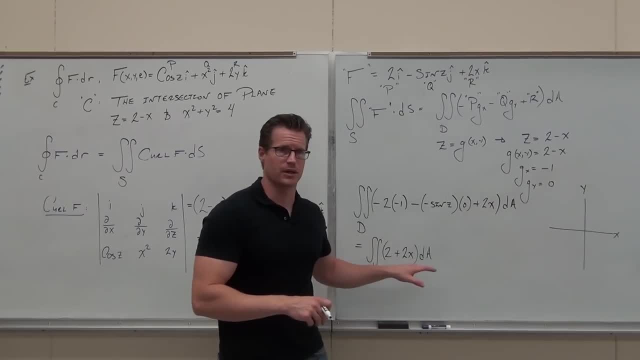 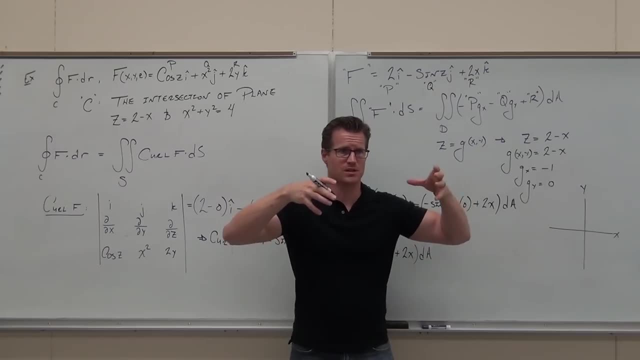 Firstly, are you guys okay that the picture we're looking for, the region is on the xy plane? We're basically making it z simple here, if you will. We're making the function z equals function x and y, which means that the domain, the region there. 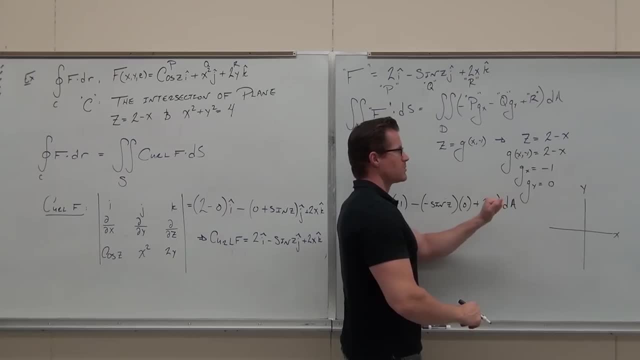 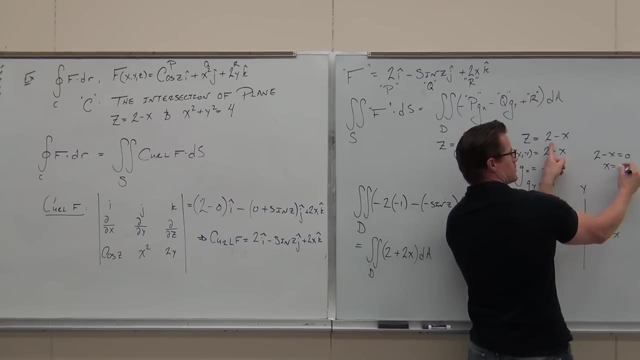 is going to be on the xy plane. That's what we're trying to do here. So if z equals 0,, then 2 minus x equals 0, and x equals 2.. Can you draw that on the xy plane? If we're on the xy plane, z is 0, man. 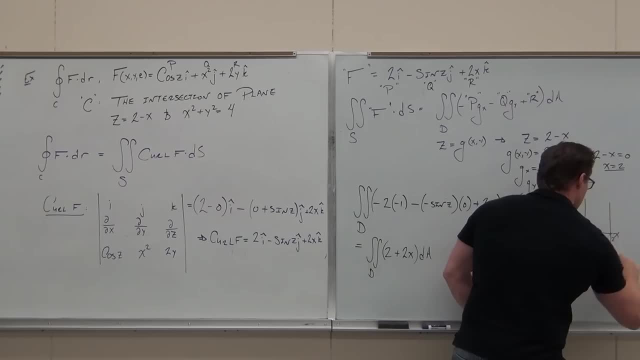 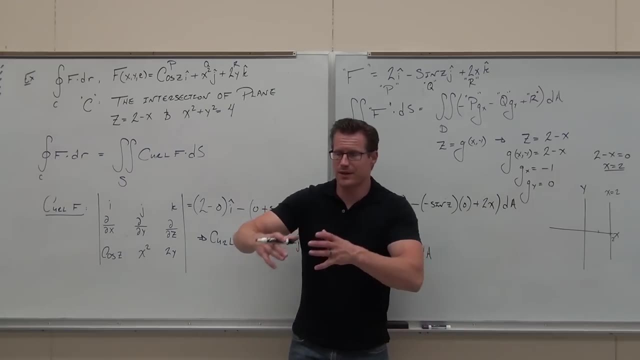 So we got 2.. I don't know if you're okay with that one. Let's look at the other thing. that's basically creating our boundary here is this: Let's draw that too. What's that going to give you? 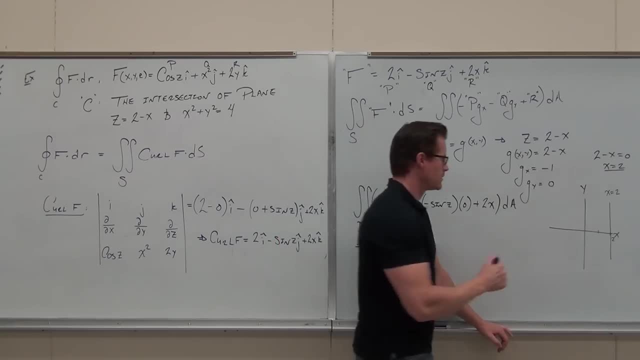 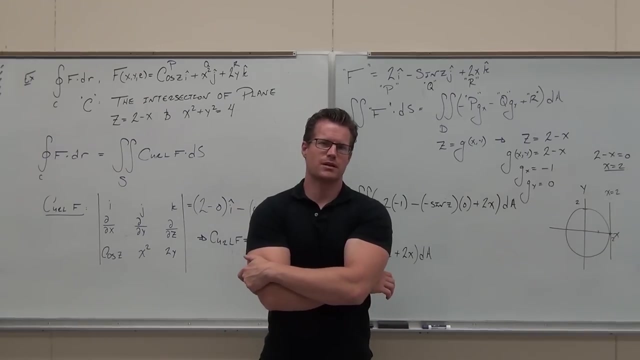 How many circles have we had in this class? huh Radius of. Let me ask you a question: Is the line x equals 2 relevant to the region that's created on the xy plane? Is it relevant? What if it would have cut through it? 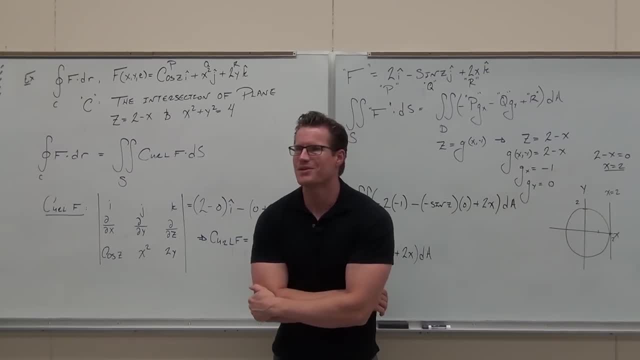 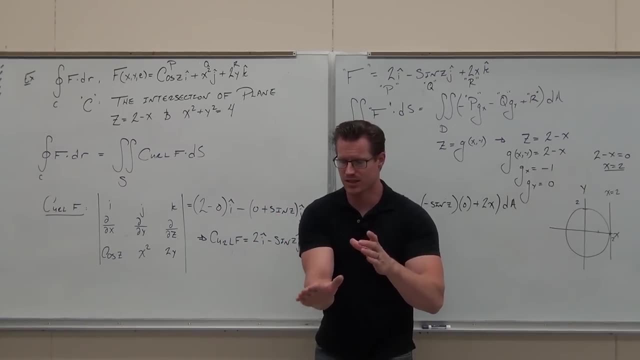 Would it be relevant? Yes, But if they don't intersect, why don't they intersect? We had an example like this a while back. We got this cylinder right And we got this plane that's cutting it. That plane intersects the cylinder. 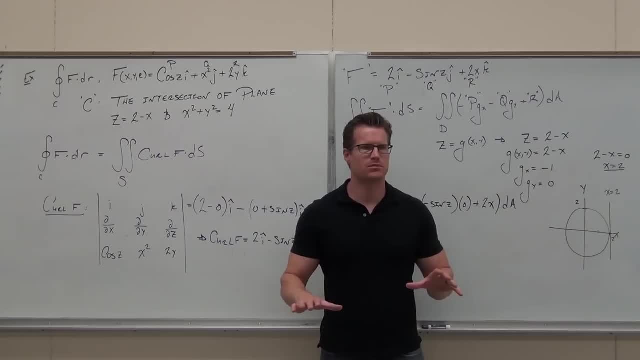 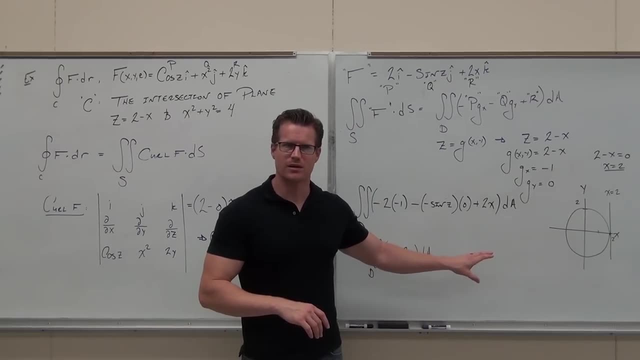 right at the xy plane, right at z, equals 0.. Hey, now that's your op on that one. Okay, now can you finish up the rest of this problem. Try it. What do you think you're going to do here? 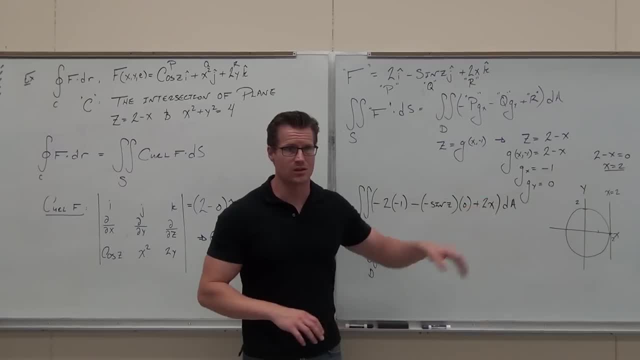 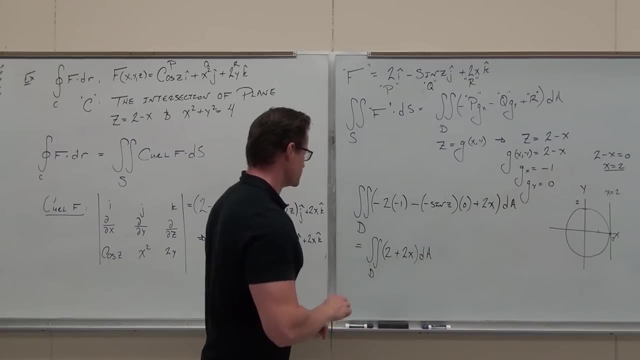 for that region. Remember d just means the region. What do you think you're going to do? Convert it to polar, Yeah, Why would you convert it to polar Circle? Beautiful, Do it. How would you do it? Don't mumble at me, man. 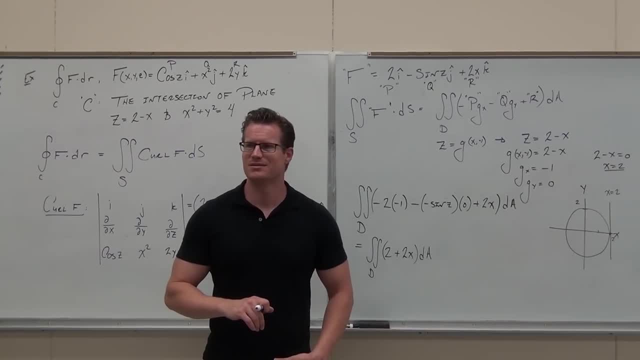 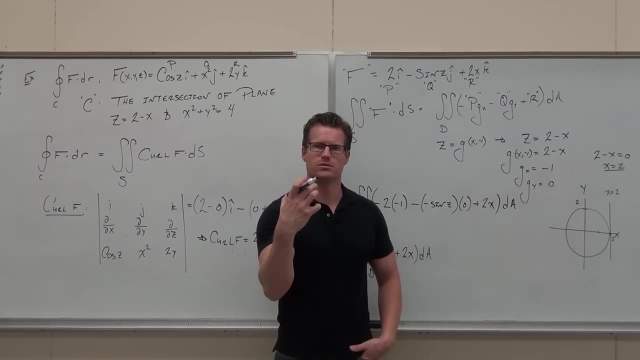 I can't hear you. I hear you mumbling at me. How would you do it? Define the r and the a. Define the r and the a. Okay, okay, What two variables are going to give you the circle here? So those are the two variables that you want to call r. 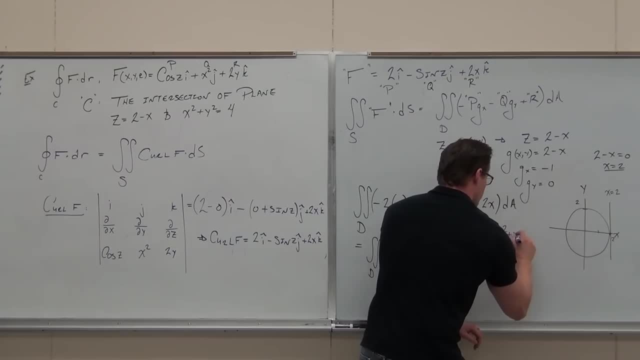 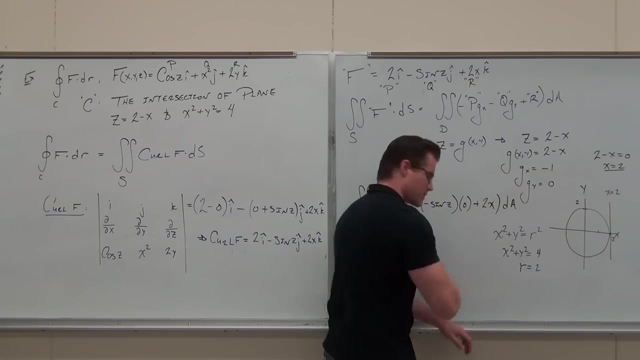 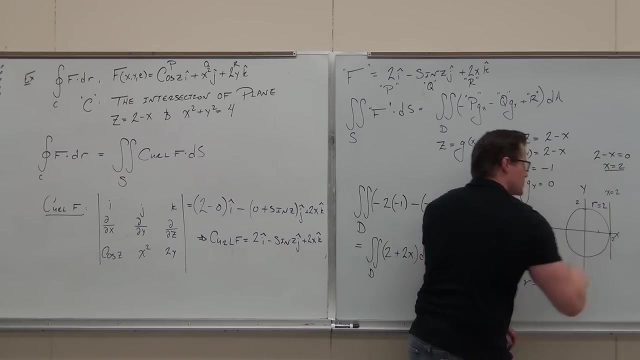 So let's do this Like this: yes, Yes, That means that x squared plus y squared, in our case, equals Four, Four. so r equals two, R squared equals four. r equals two. This is the circle: r equals two. 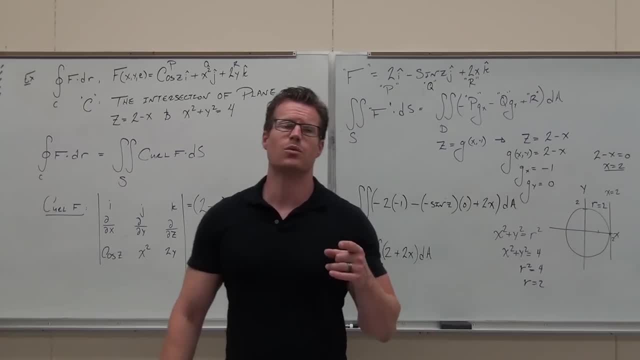 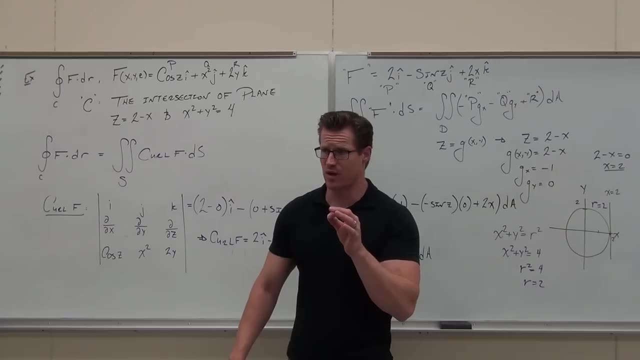 No big surprise, It's a circle with a radius of two. Now I also told you to do one more thing: Every time that you have to define something in terms of polar, that necessitates a change of parameterization for your x and for your y. 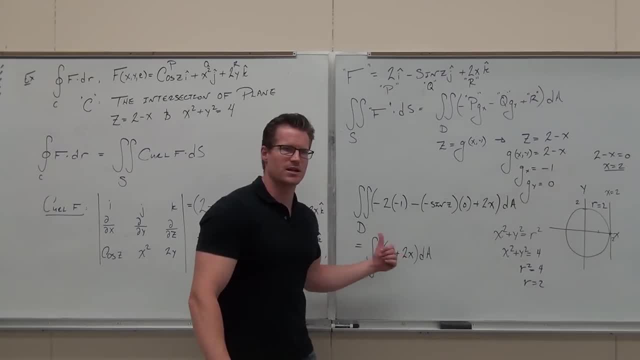 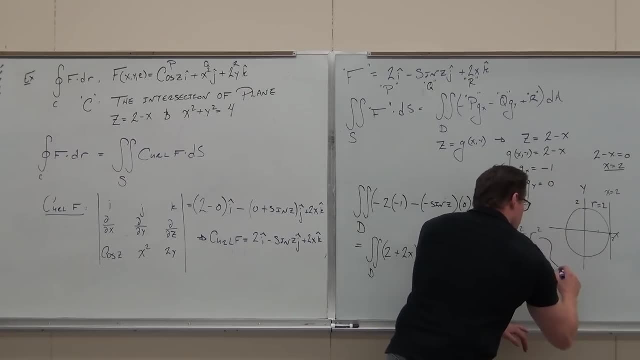 Write that down. Write that down. That way, if you have any extraneous x's and y's floating around in your integrand you can change them okay. So as soon as I do this, what's our x become? 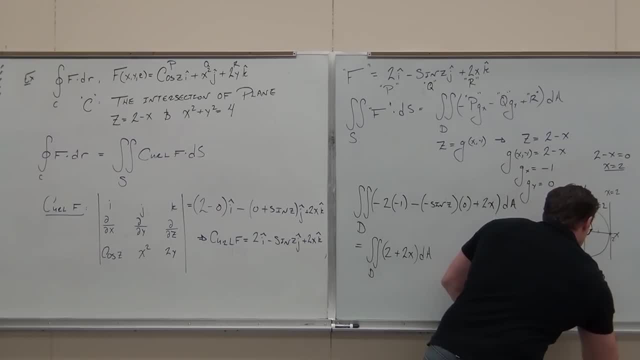 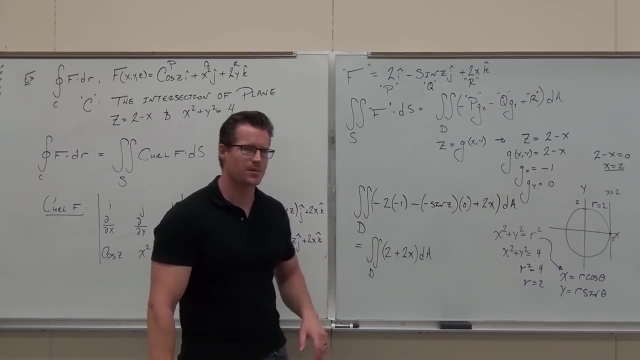 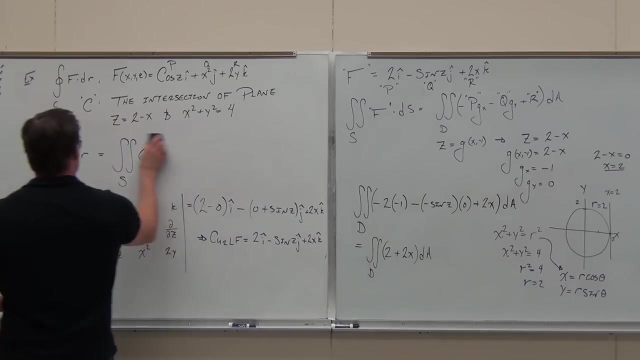 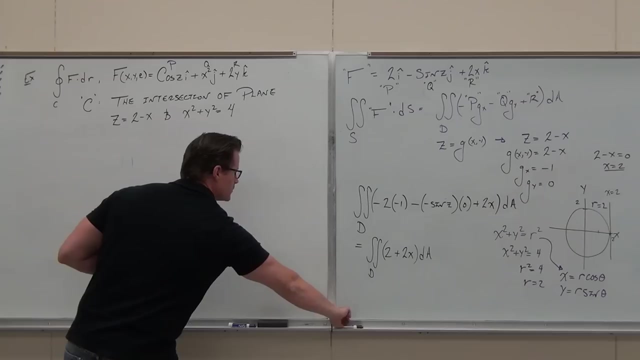 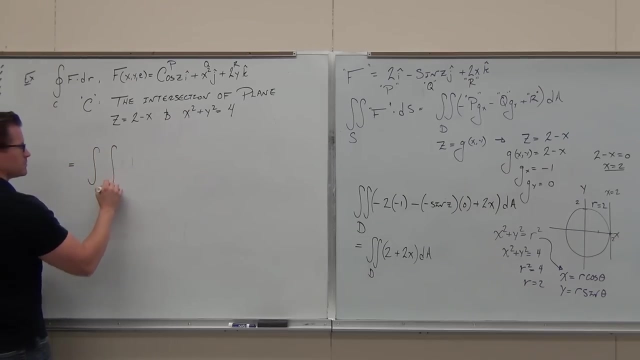 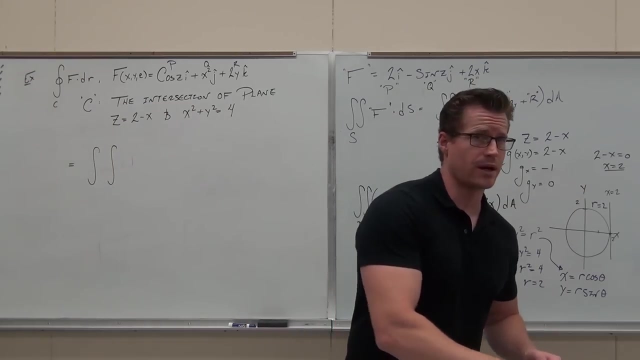 R squared, R squared, And that allows you to change it. So I want to see a proper setup and then let's check that. I'll give you about 30 seconds to give you a proper setup. Remember, this is just a double integral. right now. 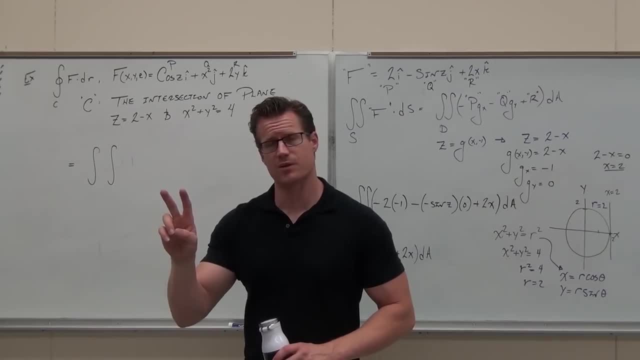 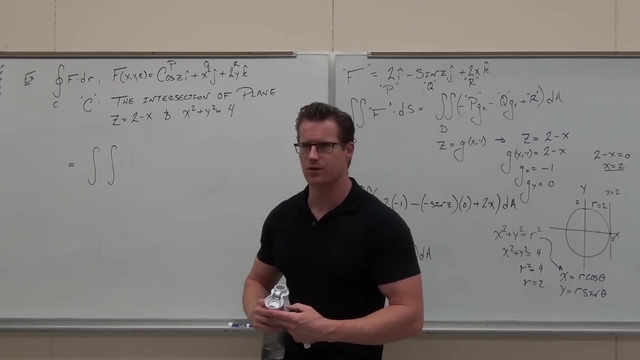 So all I need is two different variables. All I want is two variables. All I can have is two variables. And you're changing a dA, not a dV, So you're not doing like cylindrical, You're not doing spherical. 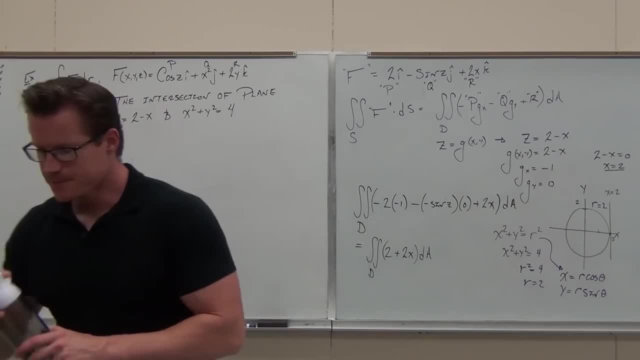 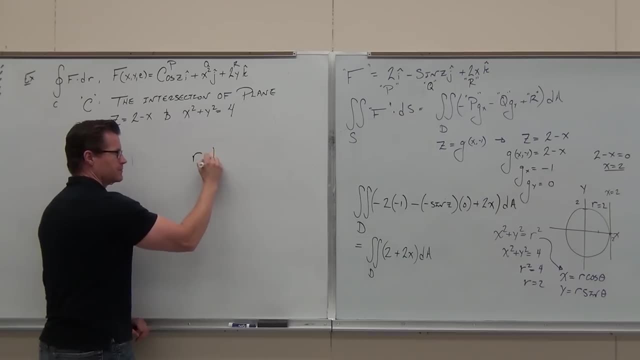 You're just doing basic old polar. What that means is, with that circle in the region we're doing polar. I know at the very end I'm going to have a what R squared Beautiful. That means that I have to go r then theta. 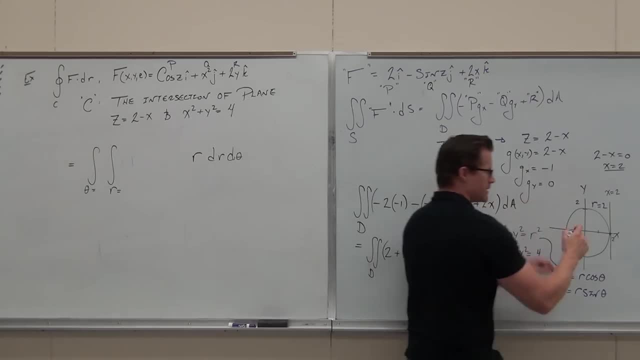 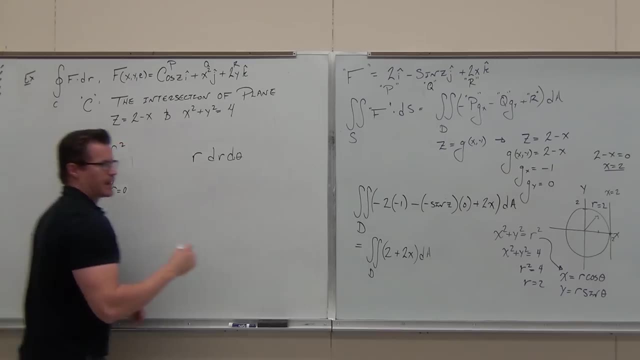 I know that for this region that was projected from that surface onto the xy plane, my r goes from 0 to 2.. Sweet, And it's a full circle. So our theta is going from 0 to 2i. That's changed our bounds of integration. 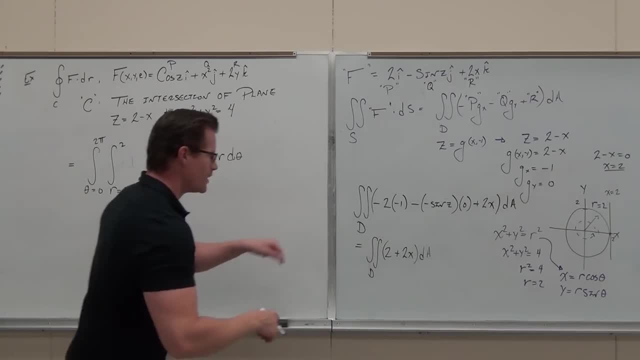 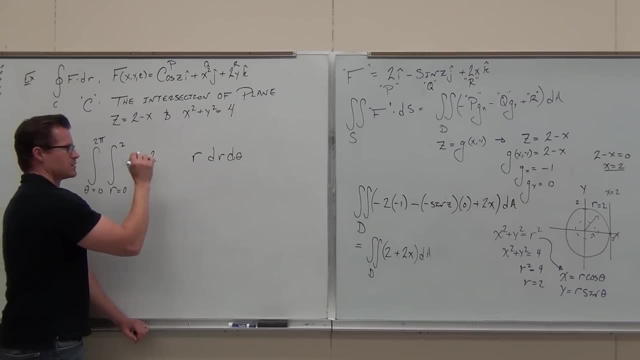 It's changed our dA to what we want. That already already theta is region polar. Now we look at the inside, the integrand What's got to be in there. 2 can't change. That's why we define that. 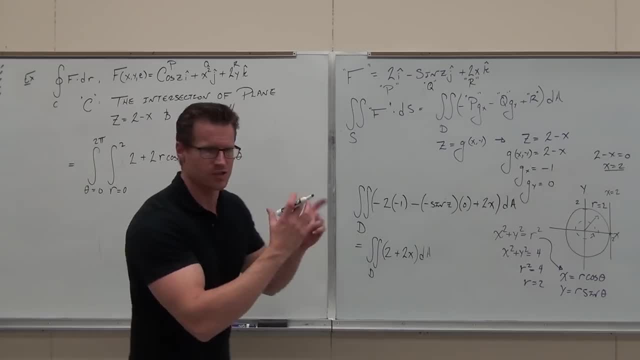 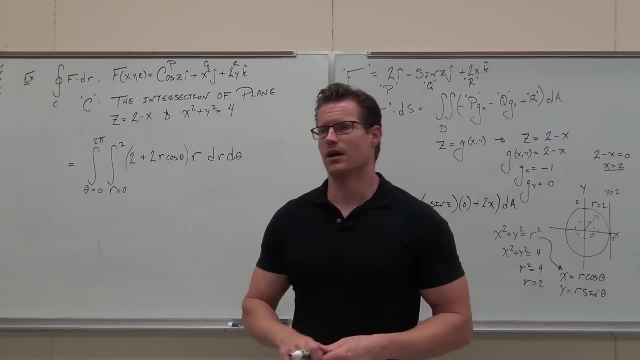 So you know what to do with any x's and y's that are in there that aren't like x squared plus y squared, And you've got to have parentheses. Did you make it that far? Good, You've learned a lot. 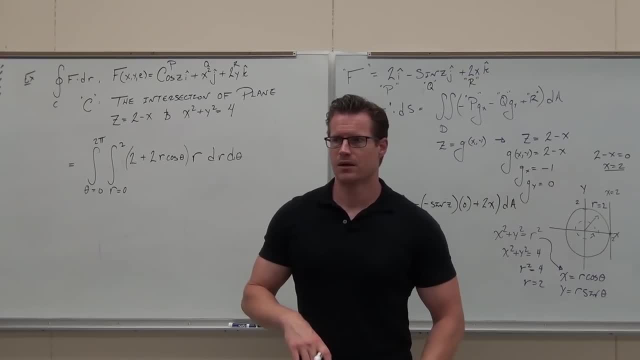 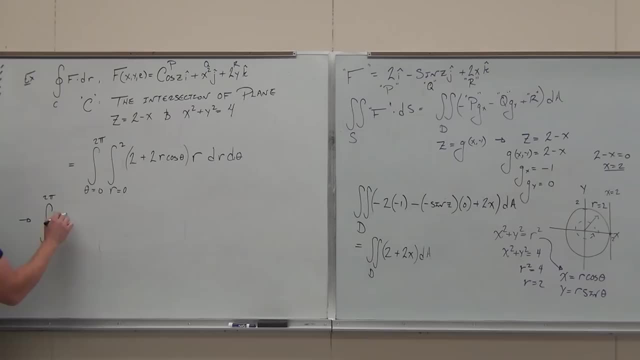 That's fantastic. What's the next thing you do? Because we're going to work through this one. Do what now? Yeah, let's do that. You could also factor out the 2 if you really wanted to. I don't think I did that, but you certainly could do that. 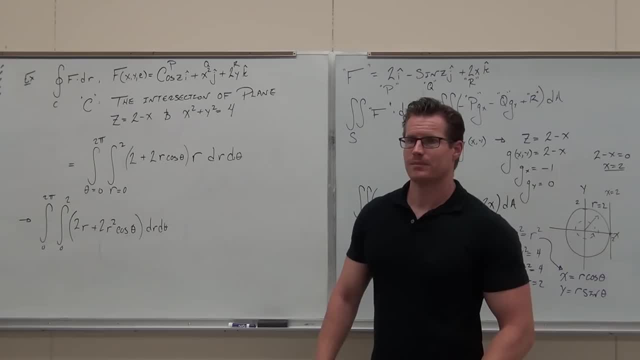 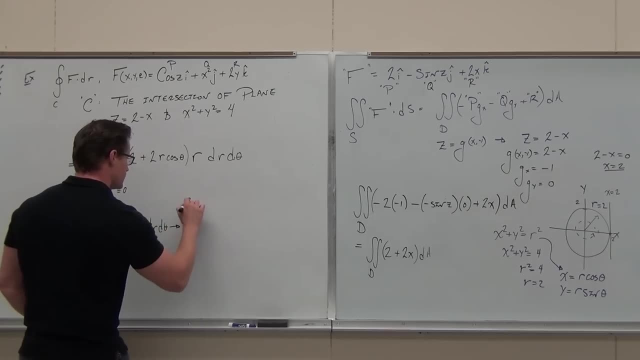 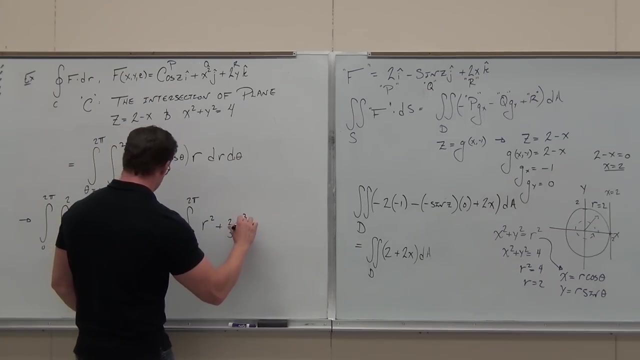 Well, now let's end with some good participation here. What would I get when I start integrating r squared And 2 squared is r cubed. Okay, right-setters, we're plugging in. for what variable please? 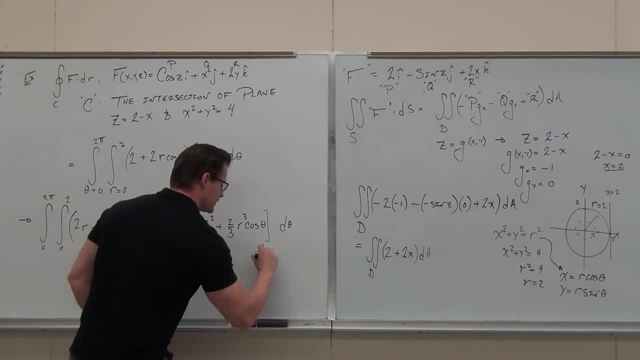 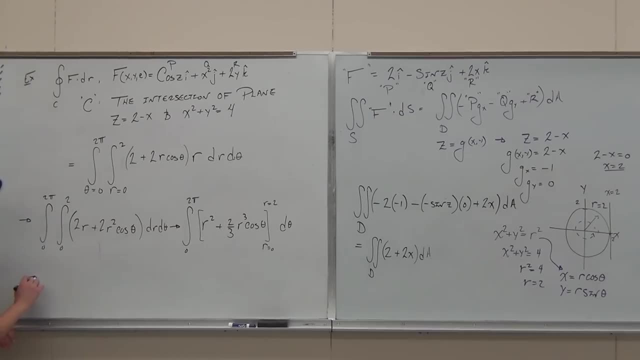 r 0.. Yes, for what variable r? So if we do that, we get this. Looks like 4, 16 thirds d theta. Plug in 0,, you get 0.. After that one, come on, stick with me. 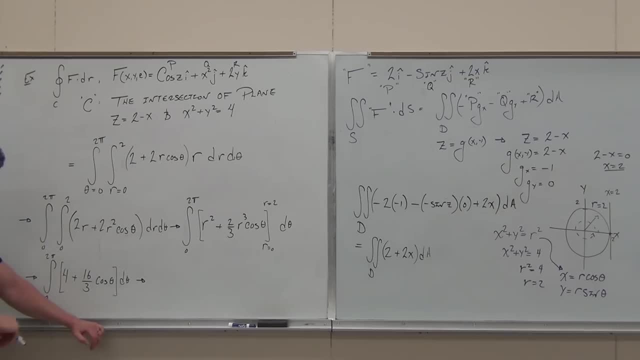 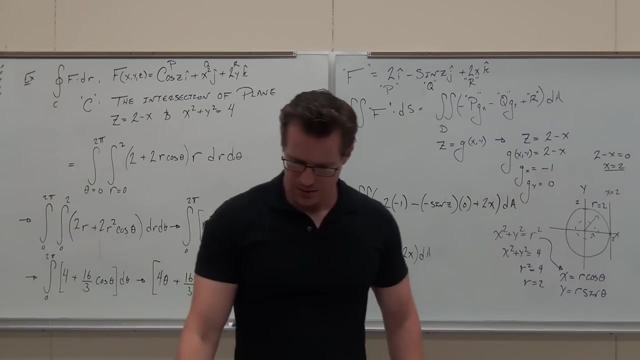 Middle people. how about you guys? What do I get when I integrate, respect theta 4, theta Plus 16. Plus, yeah, Is it going to matter? No, No, but Say what now? You get 8 pi. 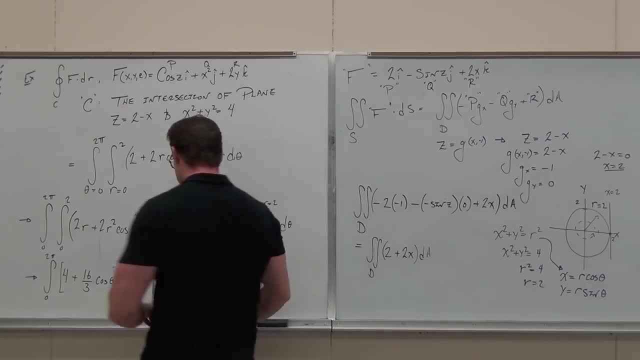 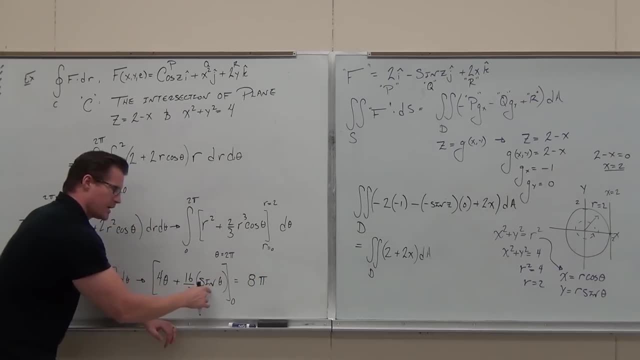 Do we? Yes, That's good to me, 8 pi is 0.. Yeah, so plug in the. definitely plug that in. We're going to get 8 pi. Plug in 2 pi here. Sine of 2 pi is 0.. 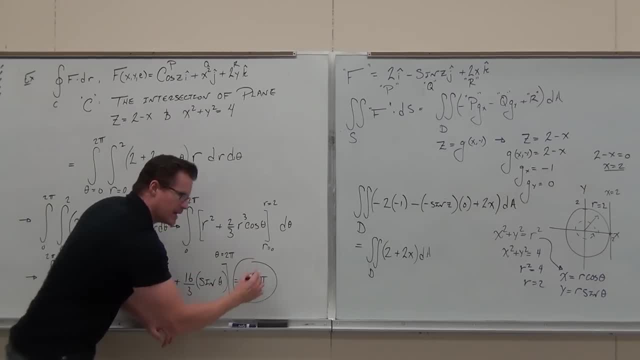 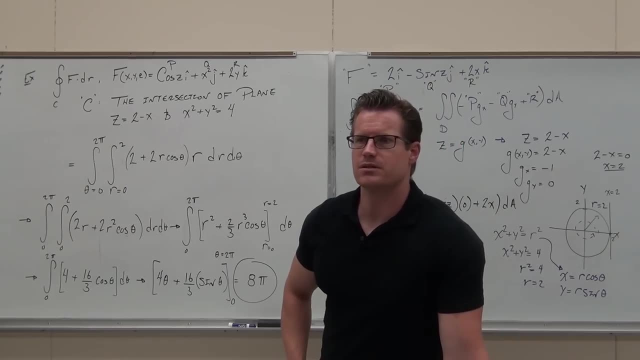 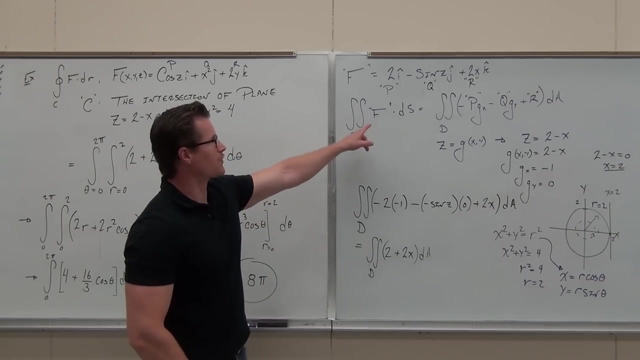 Sine of 0 is also 0.. Theta with 0 is 0. We get 8 pi. Now you tell me what it means. Is this flux? No, No, Yes and no. It's the flux over that vector field, if you want to consider that, of that surface, that plane, that little disk.